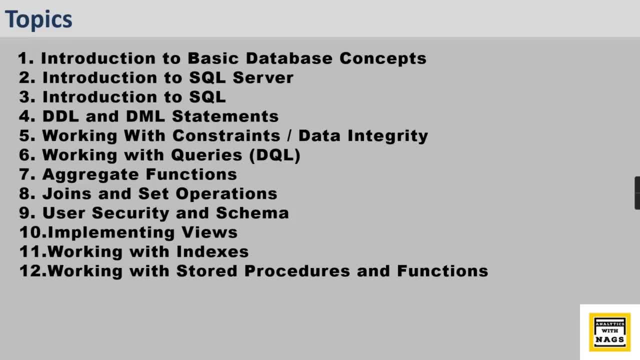 But, to be honest, understanding what things you will learn as part of this video. I am sharing this slide over here So you will understand about database, why you need database and what is the DBMS SQL Server and what role SQL plays in it. 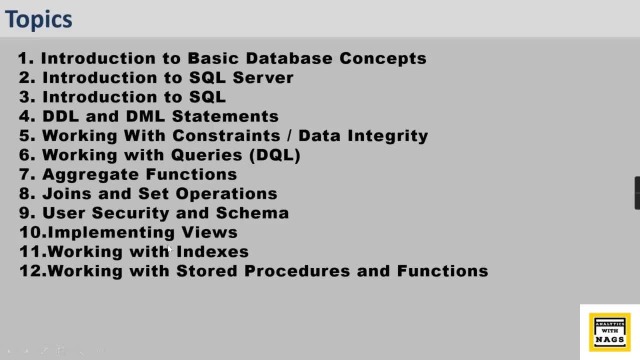 Then followed by all other topics related to SQL only. So initially you will understand all these concepts, Then you will deep dive into SQL language. So this is the main agenda of this video. With this note, let's move on to our core topic. 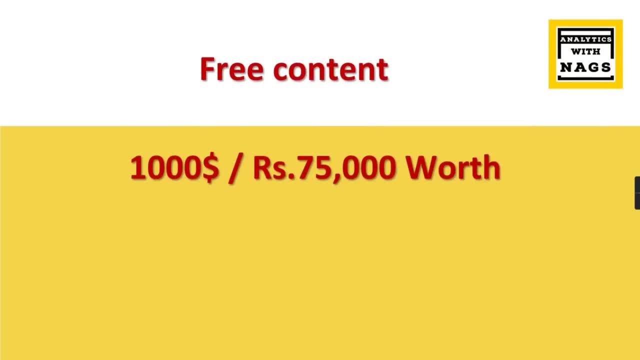 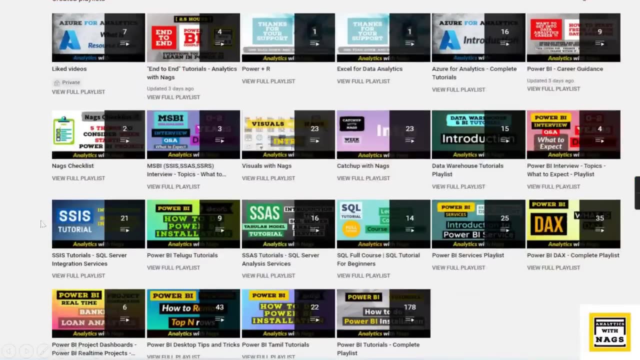 And this channel contains INR 75,000 worth, or $1,000 free content. Just utilize it. as you can see from this playlist, This is the analytics with luck playlist, where you can able to learn SSIS, SSAS, Altogether, you can call it as Microsoft BI. 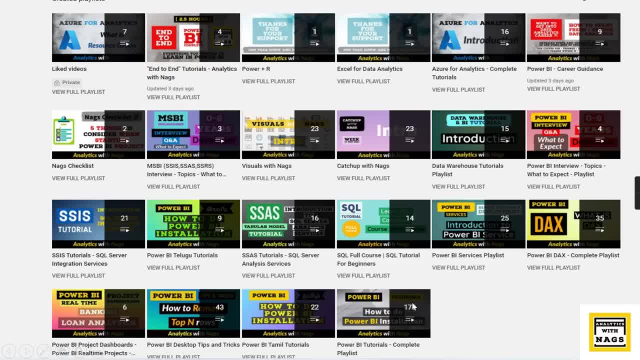 And also this channel is predominant, Having a Power BI content as well, And lot of people ask for career guidance, whether the resume preparation, how to crack the interviews or how to move to this technologies. So for them, I've created career guidance. 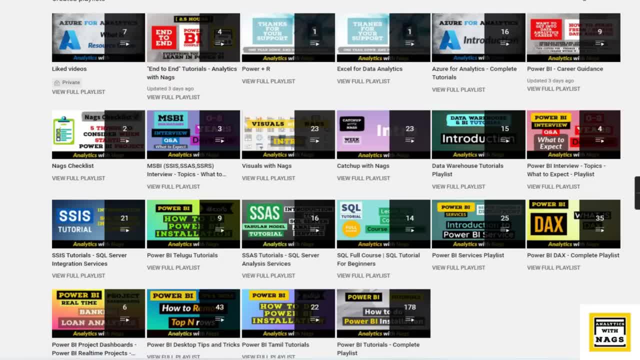 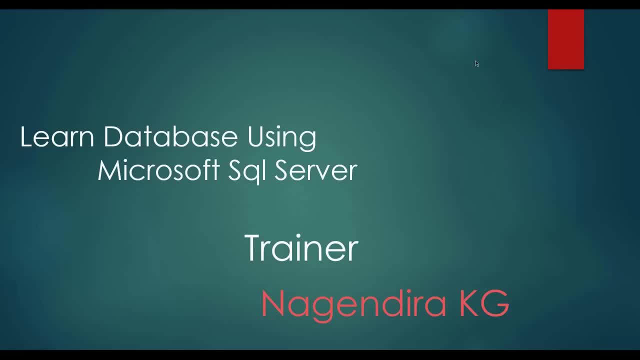 So please utilize this free contents as well. Let's begin our today's topic. So it's all about data, And you have any examples of data like whatever we use to store is called your data. It can be a customer information. 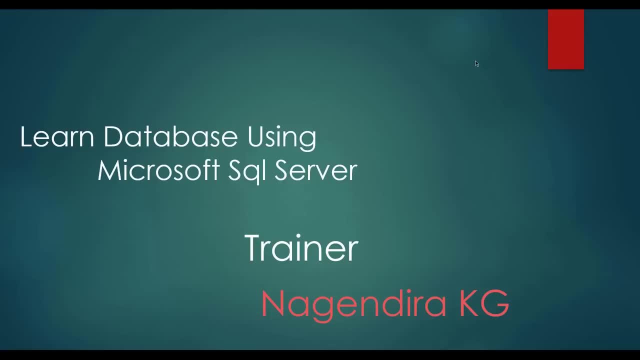 Customer information in the sense customer name, customer phone number, All those things are considered as your data. So this course is intended to have a database. So database purpose is to store your data. Okay, So just going to a history. 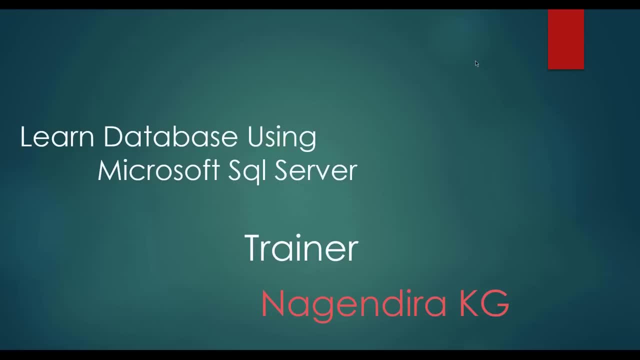 Why you need a database Before inventing a database. what was there And what are the difficulties or disadvantages on storing the data before the database? What kind of system they used- Okay In that system. what are the disadvantages they face? 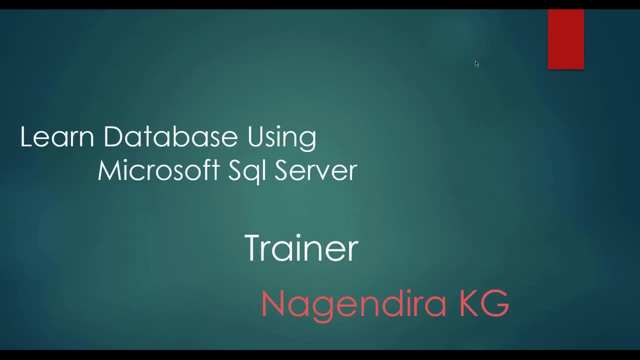 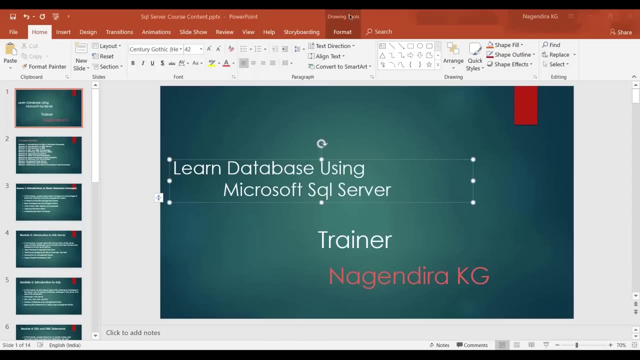 For this. only they came up with the concept called database. Okay, So let's see that history first. So, as I said, you can see my screen. You can see my screen, guys. Yes, Yes, We can see your screen. 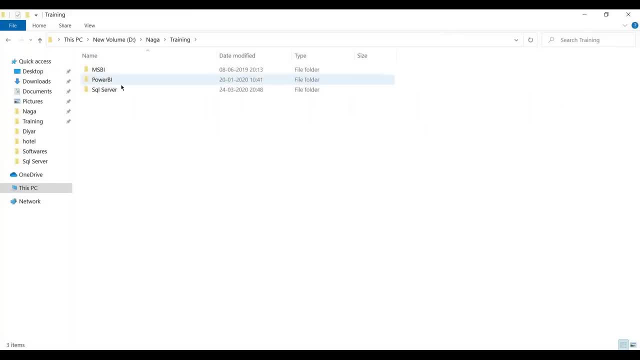 Yeah, See, like, See, you have a data right, As I said, the customer data. So earlier, before the database invention and all how they are stored, They started storing using a file system. Say, for example, I can store this file as a customer info. 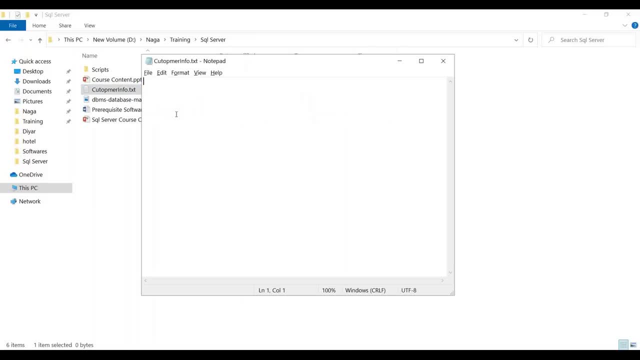 Okay, So customer info. So say, for example, I have a customer name and I have a phone number, Something like that. So name can be Naga and my phone number can be 98674, something like this. 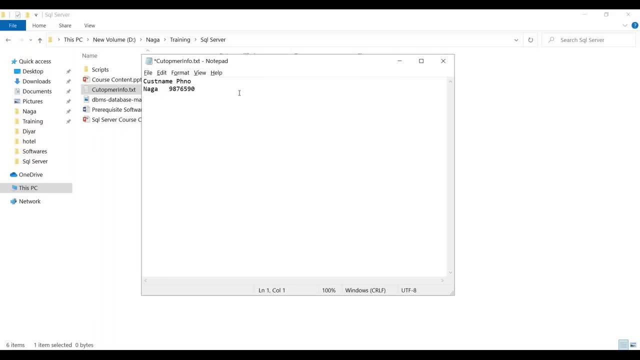 And even I don't need to store in the same way like this. I can store in the same way like this, like Naga and 98765.. My address can be in, say, for example, I'm in Kuwait. Maybe someone else say, for example, Varun. 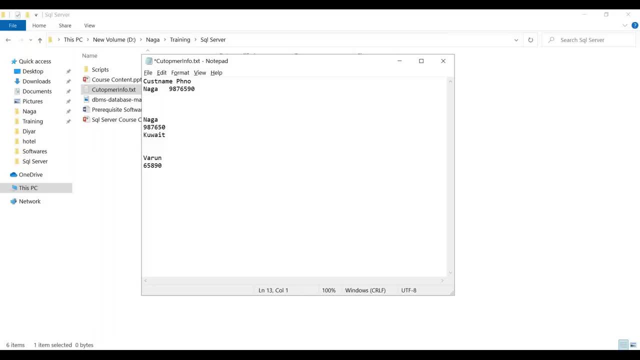 His number is. phone number is like this, So I can keep storing the data in this file system as well. So this is how the conventional storage of data has begun. Okay, So when you keep storing the data like this, 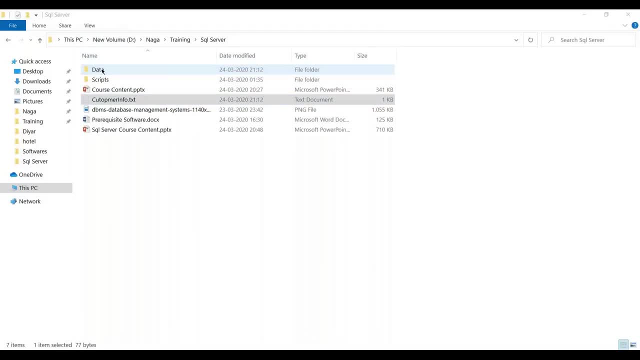 Data. So when you have your data stored in a file system And what complexities arises. Like Windows have a restriction, Like you cannot have a storage of a file more than 10 GB, 5 GB. I'm not saying about today's high technology. 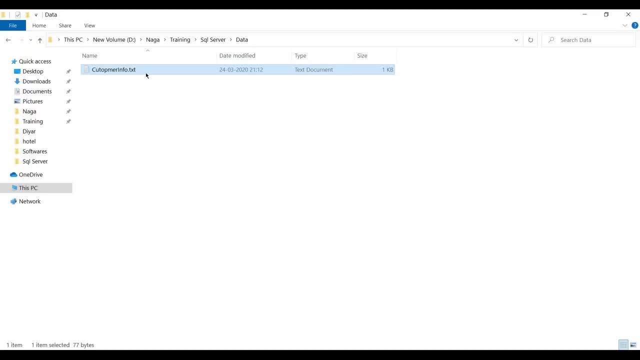 I'm speaking 20 years back. So they have a storage restriction of a file, individual file. So they have a restriction. We have a restriction of storage of a file, Okay, So that is why you have The file. system has other disadvantages over our database. 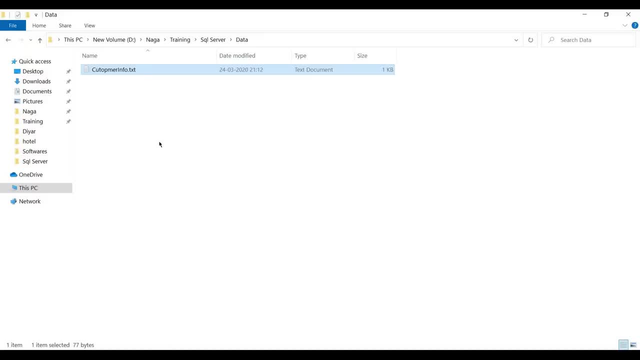 Okay, Now just a minute. Sorry guys, I'm getting repeated calls, Let's continue. So earlier they used to store the data in the file system. Okay, So you have a notepad or you can create an Excel spreadsheet over here. You can keep storing the data in Excel spreadsheet also. 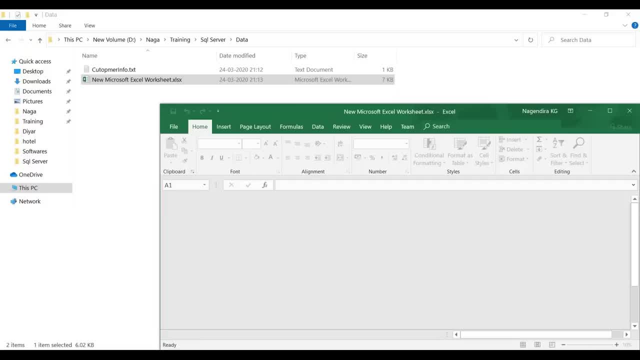 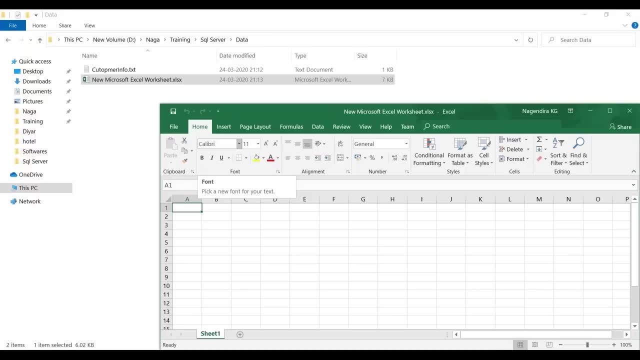 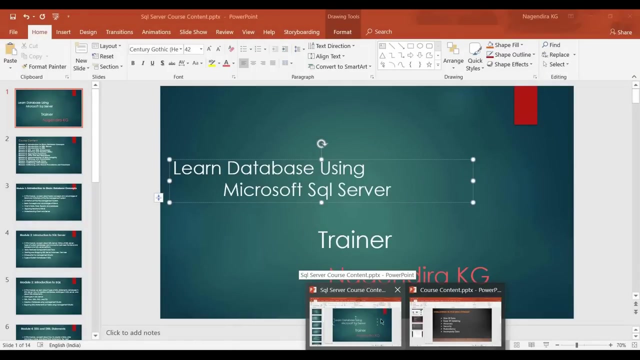 So this is the file system you have and it's used to show the data. It also saves the same purpose. As I said, database used to store your data and you can even store the data in the file system. So what disadvantages that it had in a typical file system that makes you to create your database environment. I mean that makes you to create binaries. 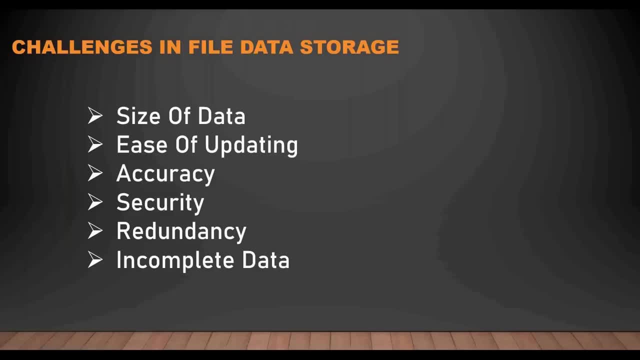 Something like that made you to evolve the database architecture. Okay, So challenges. what we face is like size of your data. As I said, if it is for a small environment, if you are managing for your own purpose, then it's fine. 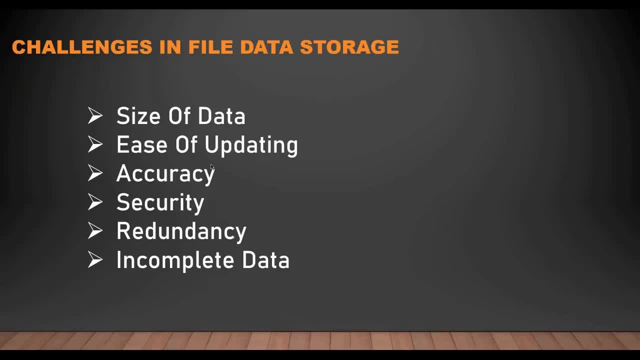 If you assume as an organization, you will keep on adding the files, You will keep on adding multiple files and you will, as you see, like you can't able to take the backups, You store it here and you put it in a drive. You have to try. Someone asked you to verify where it is. You find very difficult. So first is size. 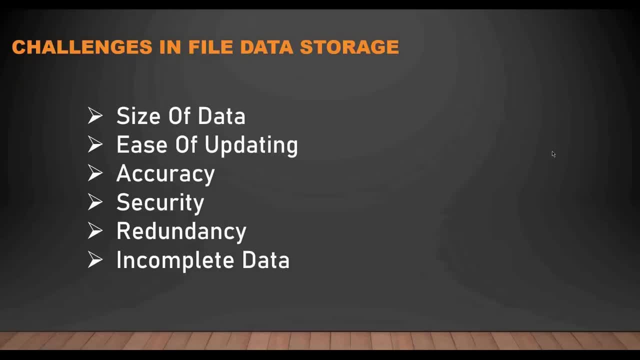 Hello, Someone is speaking. Okay, So ease of updating. So ease of updating means you can't able to easily update. Say, for example, in the same file you have hundreds of customer, The customer information has changed, He has changed the phone number. You need to go on such assume you have multiple files like that. You have 80 to 90 files. You don't know in which file the customer data is stored, So updating becomes very difficult. 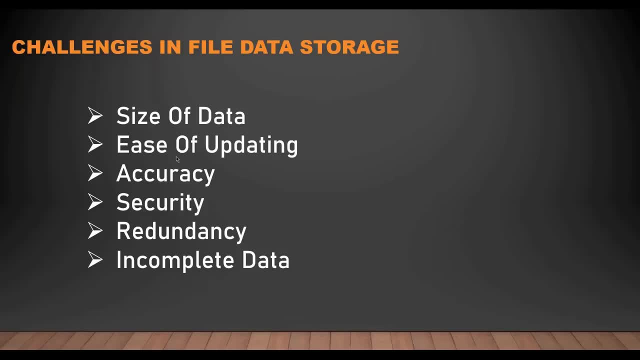 Storing is easy. Initially you start Okay, Accuracy, as these are more or less related accuracy and updating Everything is same- and security. So when you have a data stored in the file system, securing those files, You can save. for example, as a manager, I need to access only the payroll. I can access the payroll, but the other employees should not access the payroll information If I have all the information stored in my desktop. 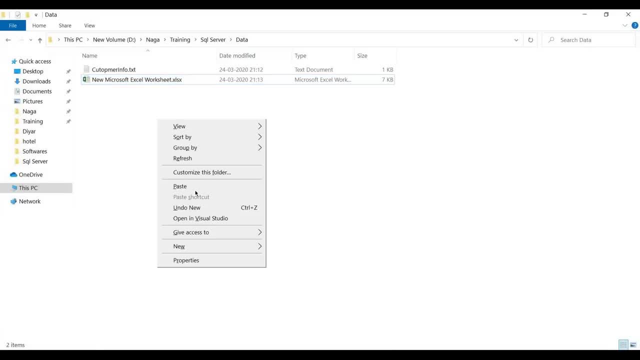 Like this: this is your data and you have payroll information over here. Okay, So you have payroll information. So, if this folder is access to everything everyone say- for example, from the manager, from the deal or your employees- everywhere can go and see their payroll information, how much they have paid, what is the salary of. 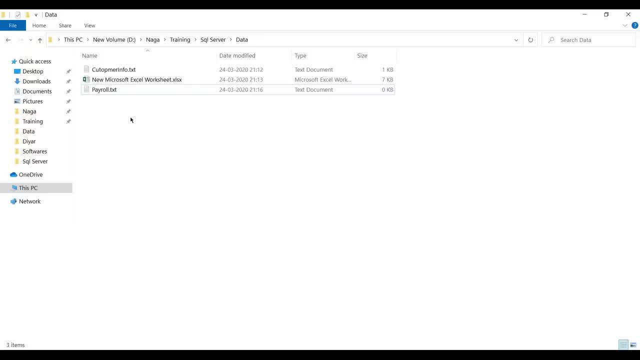 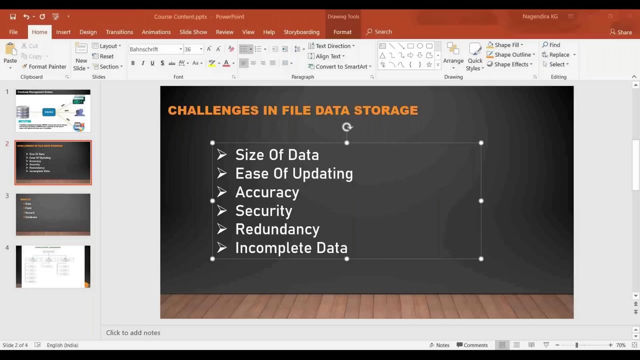 my colleague: what is my manager's salary? then that becomes unnecessary conclusion. so that should be some restriction to people. who has to see what? okay, so security implementation is very complex here. can't switch between the screens. hold on, can you able to see, guys? i will teach you in this manner, because switching between the 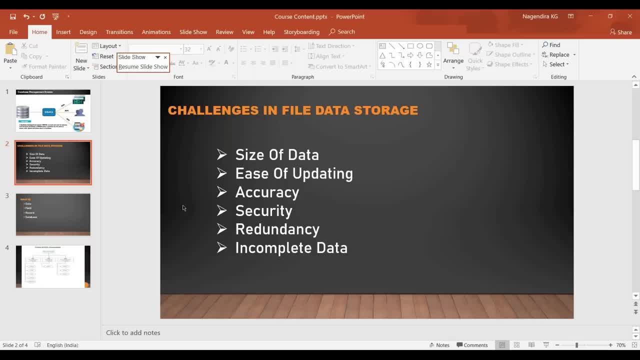 screens will become very difficult, so i'm going to show you how to do that. so i'm going to use is whichever version you need to use, you don't know after some time. So this redundancy of data and you will not have accuracy. 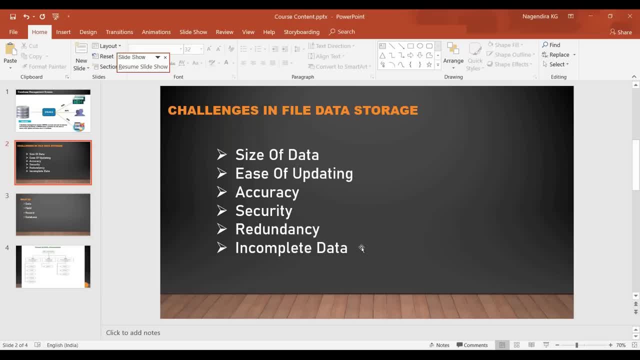 This is closely related- And incomplete data. So incomplete incompletion in the sense, if that is like some constraints are not defined in your file system. Say, for example, your employee or your customer should always have some phone number so that you can able to create. 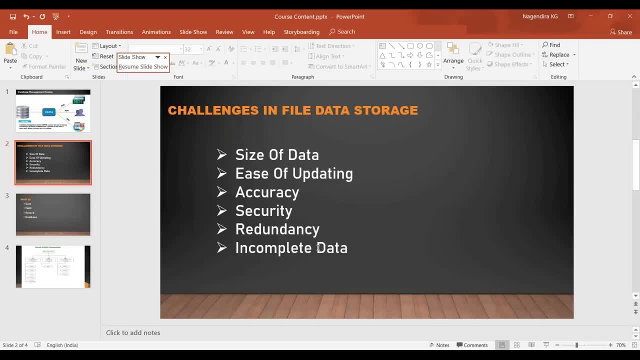 If the in a file system you do not impose an restriction to it Without having a phone number, you can start creating it. So those kind of incompleteness you will keep on adding. That becomes very complex when you have your data stored in your file data storage. 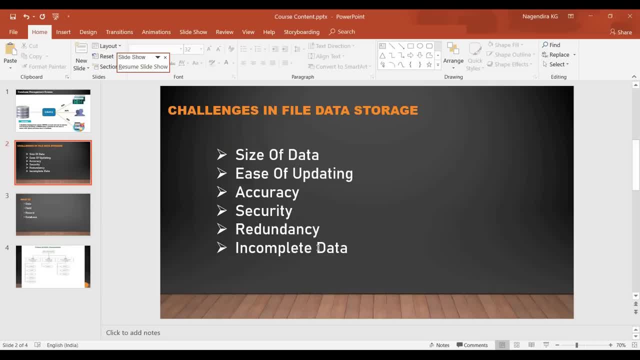 So this is the main disadvantages that earlier systems faced, or earlier organizations faced, so that it made us to evolve and move towards the storing your data in your databases. I think till this it's clear: Guys, Yes, Nagar, Yeah, yeah. 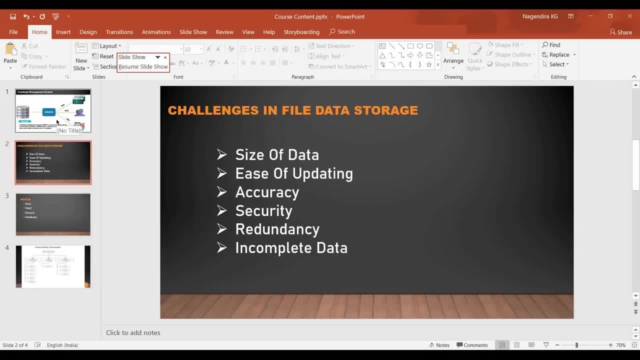 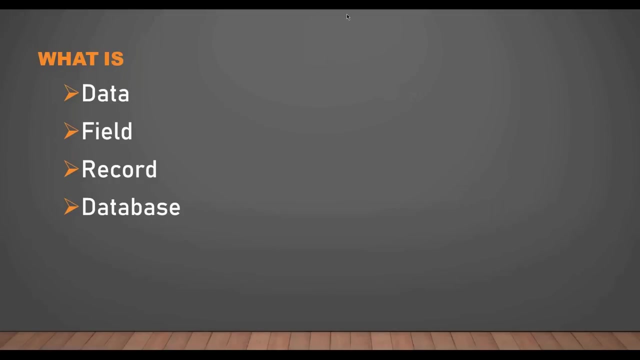 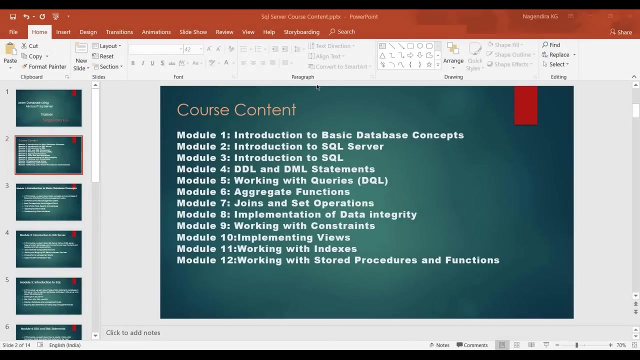 Good, Fine. So coming to the modules Now, with this note, let us see what are the things we have in this session. So basic database concepts, So basic database concepts, and we have introduction to SQL Server. So these are the things I'm going to cover. 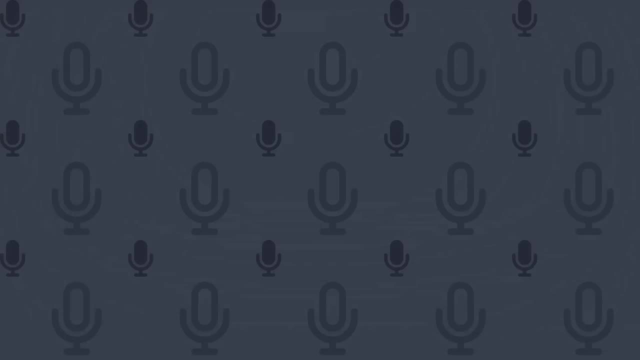 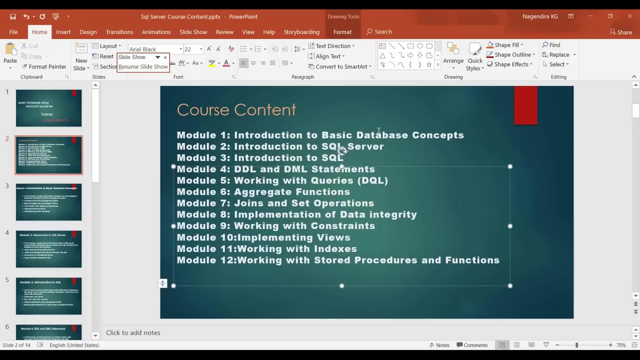 Let's keep changing. So, introduction to SQL, DDL, DML commands, working with queries, All these things will make you to have a full SQL developer, That is, SQL Server developer, Once you learn all these courses. okay, So I think Rabani Rahil wants more on the module six. 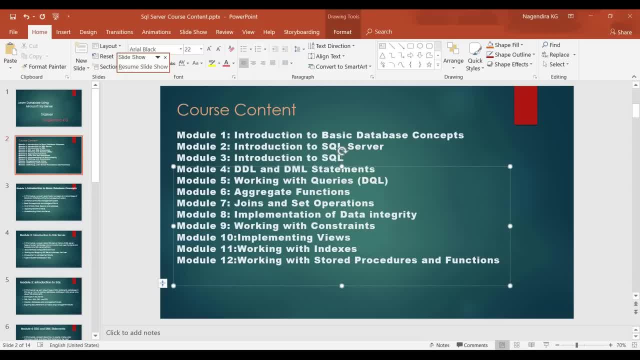 two, seven, eight, nine, 10, those things. So they are familiar with the module till first five modules. I think Let's see. Yeah, Nagendran will. this course will also cover the SQL fundamental about data query. 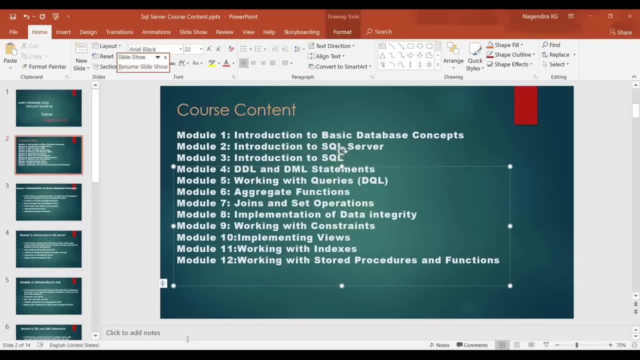 Yes, yes, yes, yes, That is what- working with queries. You have a module six over here. Hold on, Select, direct insert, update and delete those and joins. Yeah, yeah, So you see here working with queries. 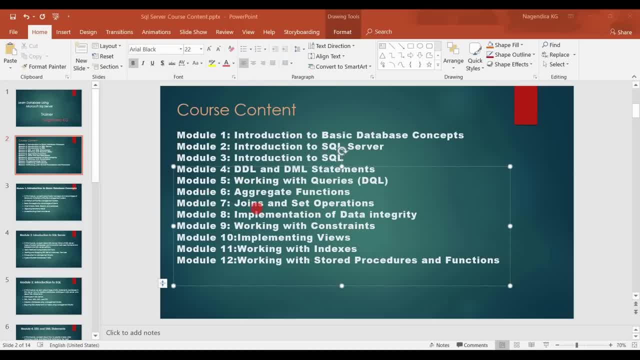 aggregate functions joins- You can see my mouse pointer there- Joins, Yes, yes, So implementation of data integrity. So basically it involves know about the database and using SQL. okay, I mean using SQL, and we use SQL Server as the DBMS. 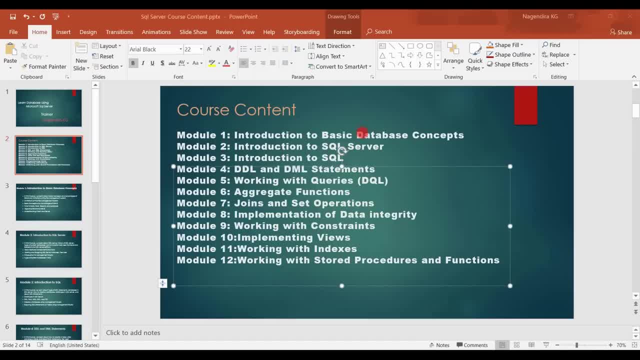 I'm going to quickly start that session now that DBMS, all those things. So this is your course content. Just go through it, Okay, Because my job- primarily to retrieve the data- is on if anything need to be updated or something. 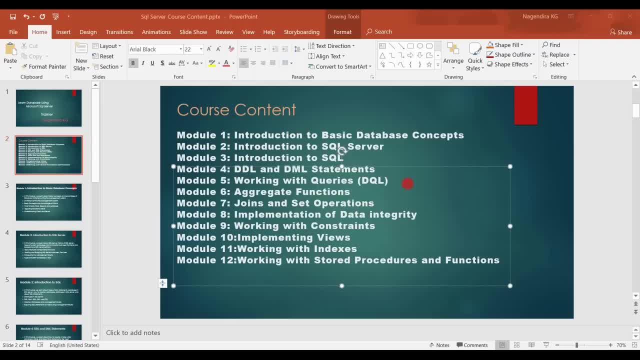 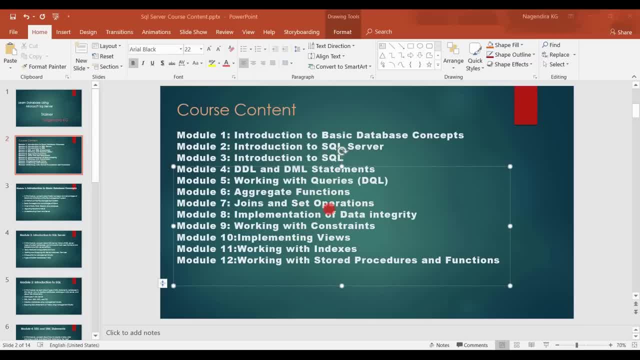 I'm going to take each module one hour and I will have another half an hour to for I mean it will not complete in one hour. Some classes will take more than one and a half hours. So that's what I told the 14 hours session. okay. 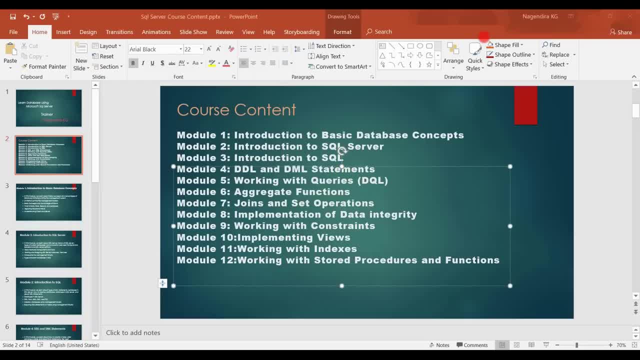 Let's see how it goes. Let's see how it goes. Okay, give me a minute. Database management system. So now I told you about database. I mean data. We discuss about data. Anything, any information is your data, okay? 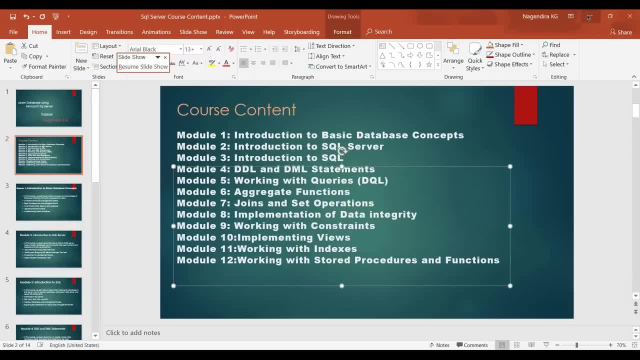 So it can be customer information, It can be your transaction, It can be your what to call it? payroll information, employees. Just you say mobile information, EMI number, I mean IMUI number, your mobile model, everything is your data, okay. 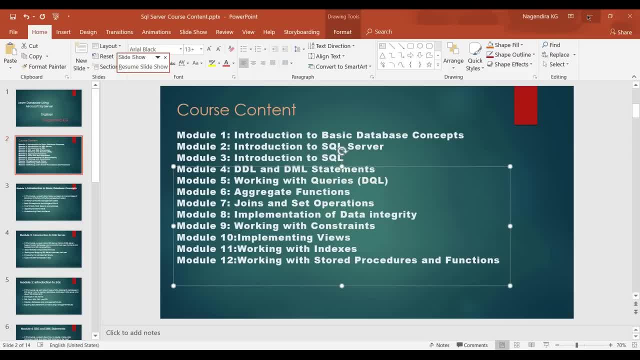 Anything, any information. definition of data is nothing but any useful information is called your data And database that is used to store your data. That's simple things. okay On where this database management system comes into place. So if you read through the definition of database, 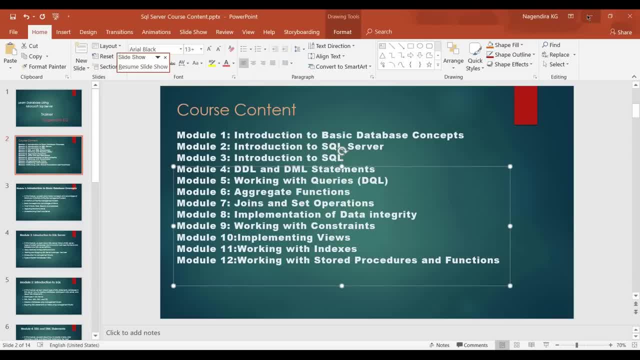 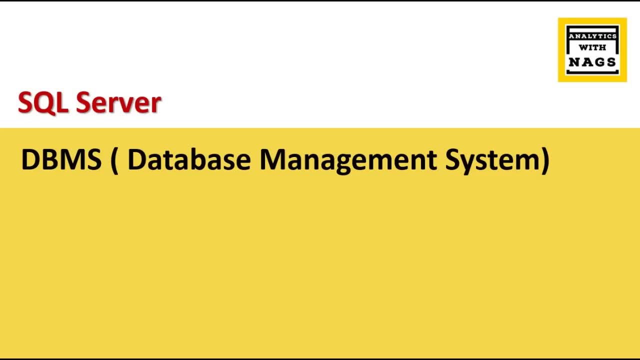 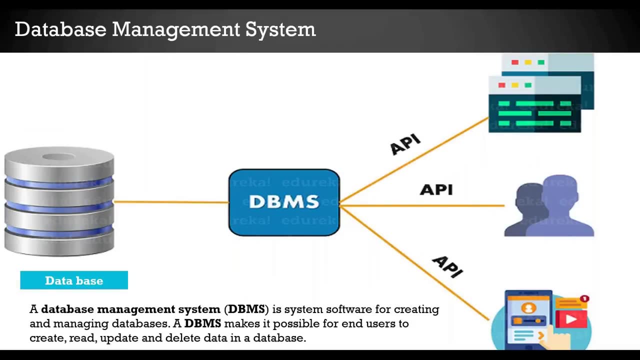 There's a lot there. They're all data. They're only as far as something else. I think I'm not sharing the screen. hold on. so database management system. if you go through the definition it says like it's a system, software for creating and managing your databases. so first I 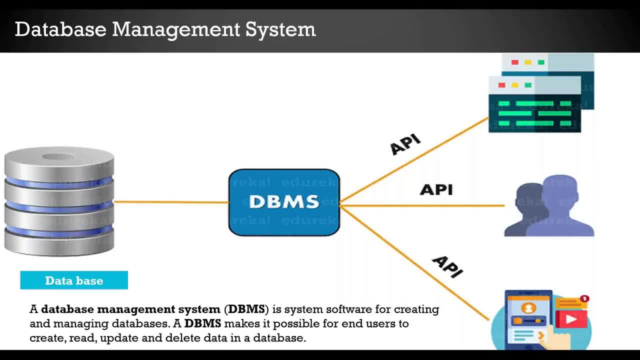 started with data. then I told what is a database that is used to store your database. then I'm telling another term called DBMS. so this DBMS is nothing but that stays in between your database and your user. so it's a software that is used to collect the data and store it in our database. it acts as interface. so 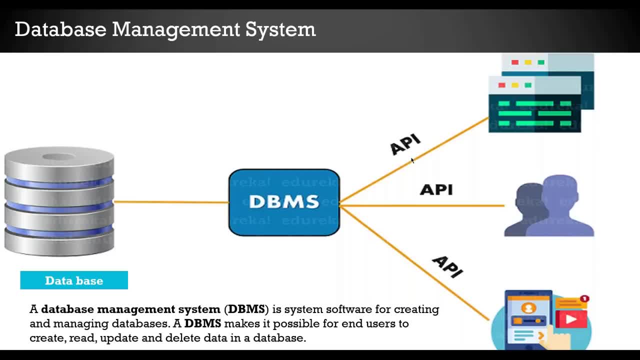 basic logic behind databases. but database management system okay. so DBMS makes it possible for end users to create, read, update and delete database in the database. so it's nothing but a software written. it's a program that makes you to create the database and modify the database. so in general term you will say databases only. but 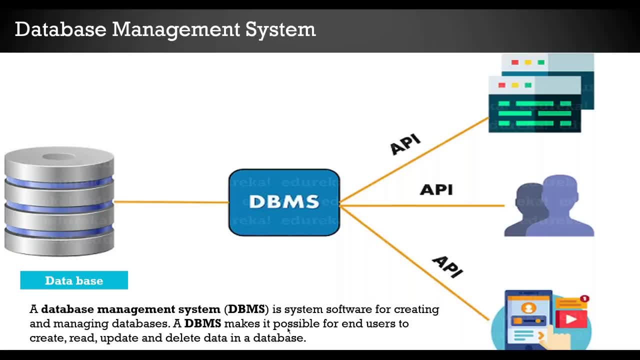 indirectly, the all the works done by database management system. it's nothing but your software. so now i said like i am teaching this database course using microsoft sql server, so it is one of the vendor, that is, microsoft is a vendor providing this software. so sql server is your database management. 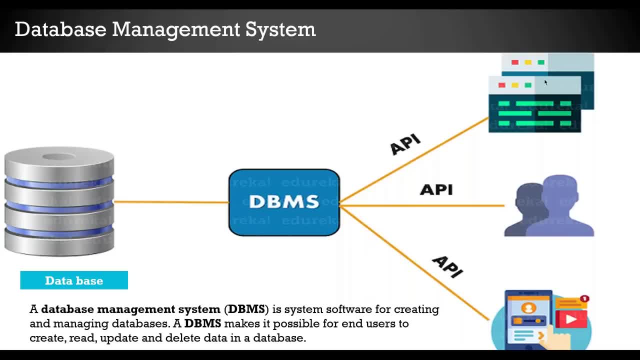 system. you got the point. and oracle is your another database management system and ibm db2 is your database management system. underneath what we'll have, you'll have databases, so databases is common. okay, that doesn't matter. so, ms sql server, oracle, all these things are database management system. 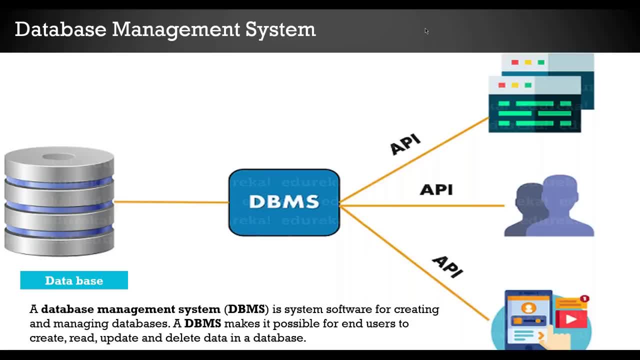 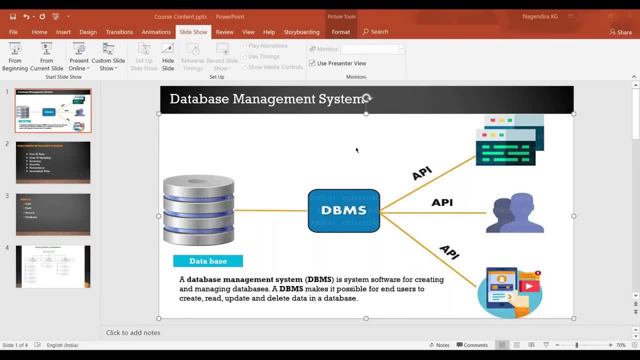 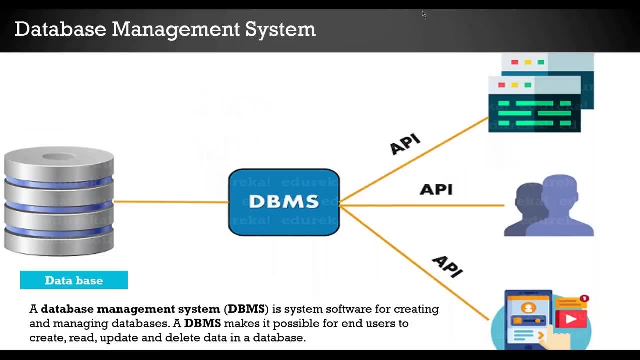 i hope i'm clear in this point. so how this database is architected in the sense people will have our data, okay, so people has to insert a data in different ways. like this: the user can use the client tools or hold on. so user will either use the 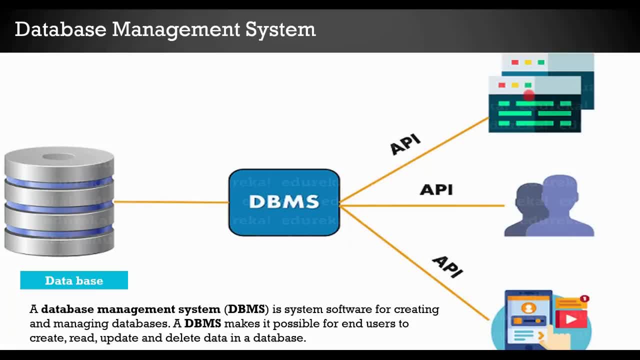 client tools or they. they will use the apis like application programming. if you assume you are going for any online shopping, they will use to collect your information. it can be a card details or any online application. so this api is nothing but this top screen, is nothing but your screen front end. 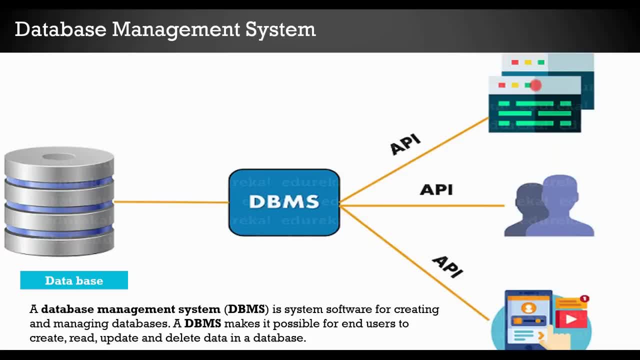 screens. okay, using that, they will gather the data. then, using the dbms software, they will store the information in the tbms. i mean database. okay, it can be a mobile application and it can be a video or any other things, so your data can be anything. basically, it is not only a text. 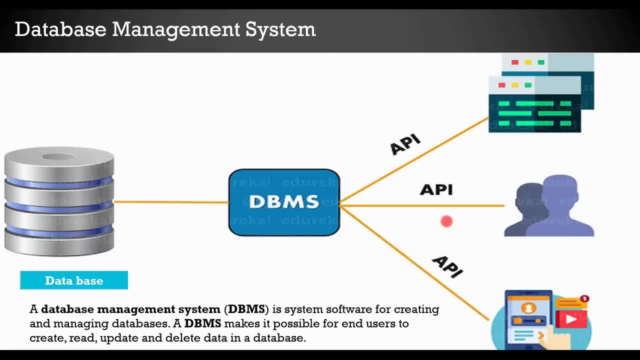 it can be a image, it can be a video. those things also can be stored in the database, okay, okay. so, nagi, uh, one question here. yes, so these are db. you said like ms sql server and oracle. uh, so, like in in the real-time scenario, like who decides like what should be? like mongodb, we have. 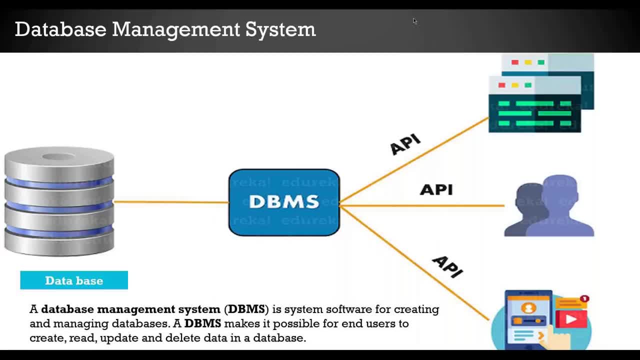 different dbms. so yes, yes. so who decides which rdbms to go correct? yes, yes, yes. so it's a business call. basically, if you have all your products built in microsoft, they always go for microsoft skill server. in some applications they used to go for oracle. so purely based on the uh. 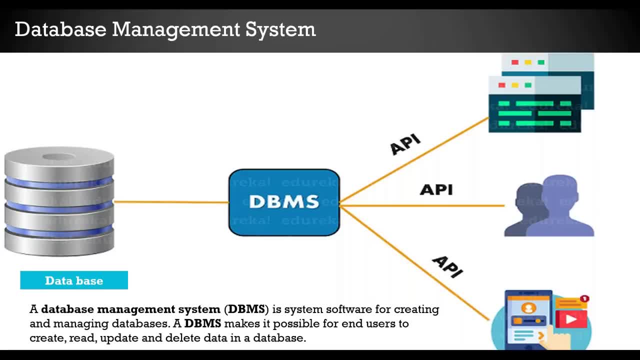 business analyst, or i will say architects. so architects will decide based on the volume. each rdbms has its own advantages and disadvantages. they need parallel processing, they need multi-level tasking. those kind of strings can be applicable only in ms sql server. oracle will not support that. then they will obviously go for this. so based on the business scenarios, situations, 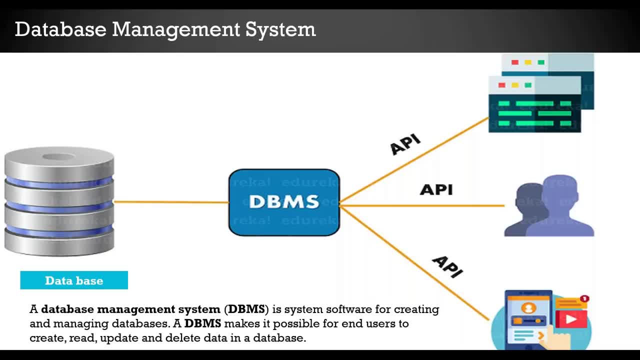 they will go for a chain. i would say rdbms. i mean microsoft sql server, because i know that one i don't know about article. this is a human mentality. you know what i mean. whatever you know, you will project it. that is how it works most of the companies. as simple as that, okay. okay, in my organization also. uh, using 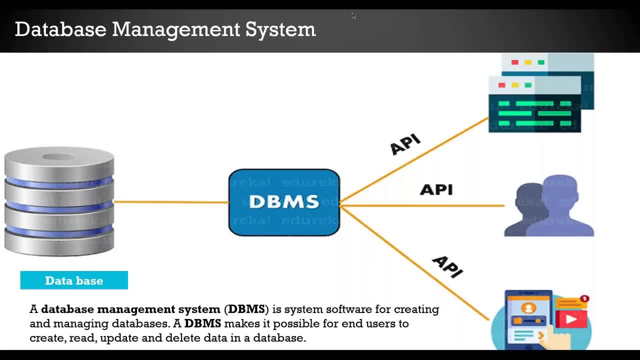 toad toad oracle- yeah, toad. and mysql is open source. so it's- uh, i mean it's a free, open source software. so mysql you, they will not charge anything. so that is rdbms that is. i mean, that is nothing but your dbms database management system. so this thing you need to be clear in mind, okay. 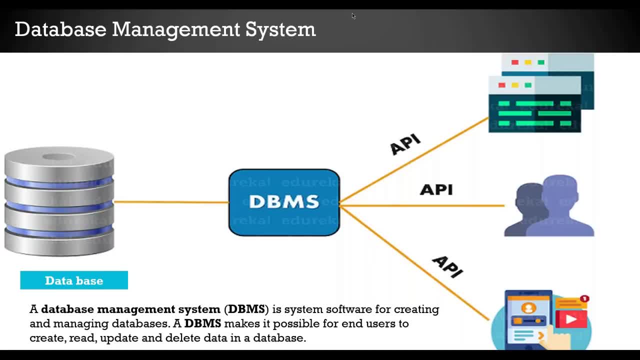 so the base concept will be any different: syntax or stay in the sql when you retrieve the queries or something when we work on with sql, microsoft sql, and when you work on with oracle. will there be any difference? no, so the concept behind this is: database is common for everything and they, if they use sql. 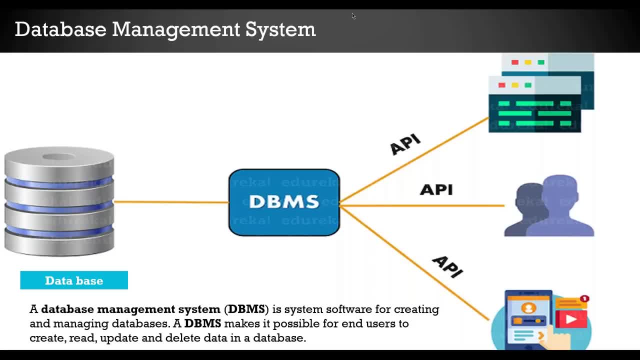 structured query language. okay, that is common for everywhere. maybe the syntax may be different if you know the programming languages like c, c, plus, but any programming language, it has its own syntax declaring a variable, like you mentioned, the data type: integer, a, r, a comma integer. it differs between: 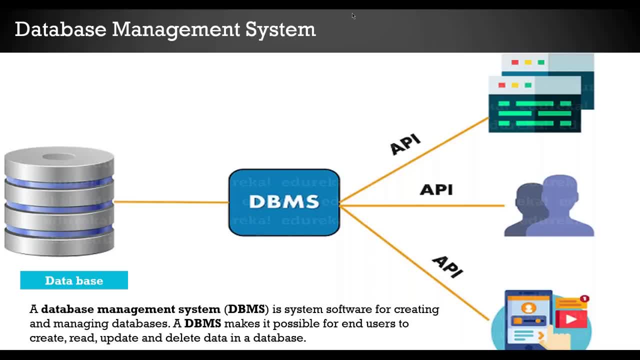 the programming language. similar syntaxes will differ but they follow the sql, then the syntax would be same. slight differences will be there in some cases. uh, i would say in article and sql server we have 80 same syntax for most of the cases. there are some cases who are providing access? 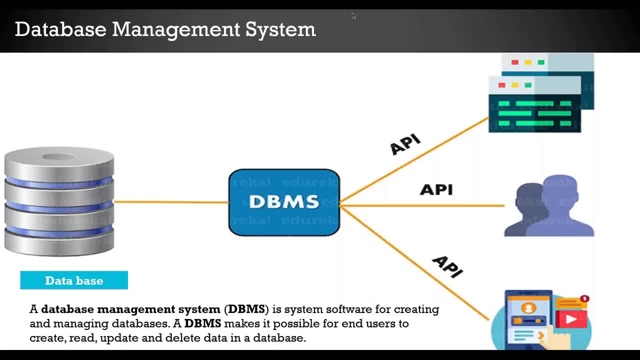 those things. the syntax will differ. even if you learn this sql, it will be applicable for oracle and mysql. everywhere, you can use the same code, okay, okay. so with that note, let's move forward. so now you understand what it is. microsoft sql server is nothing but your dbms and what it will do. it will enable you to create databases. the databases will 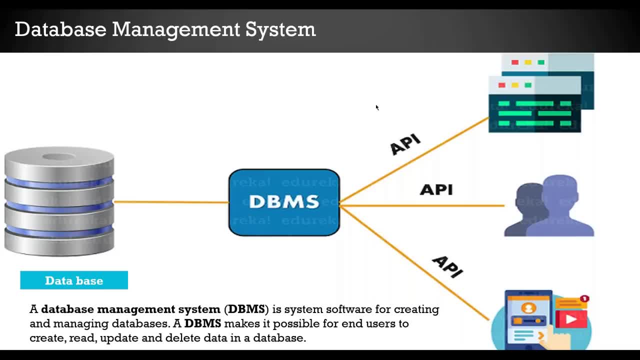 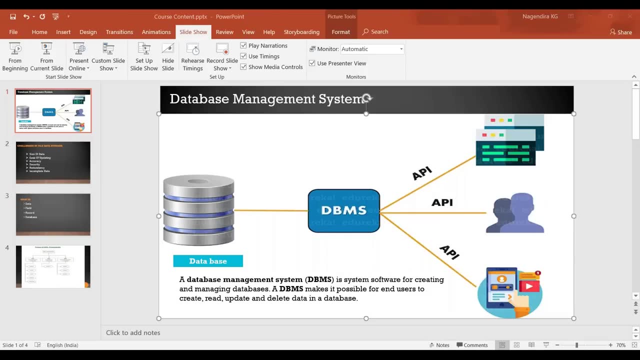 store data. now the question arise, like when you have a files- okay, you are storing any type, whatever i typed earlier. okay, yeah, i typed in the notepad i. i can store it in excel like this, or i can store it in notepad like this: move this window away. 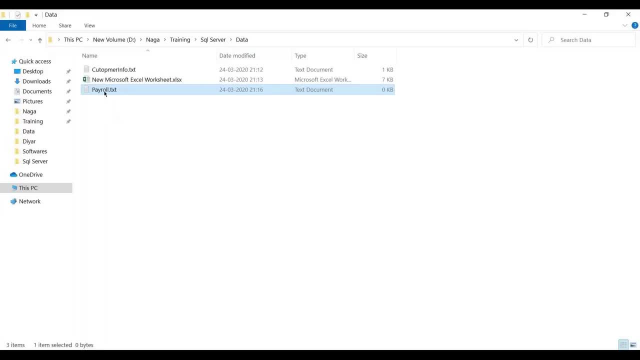 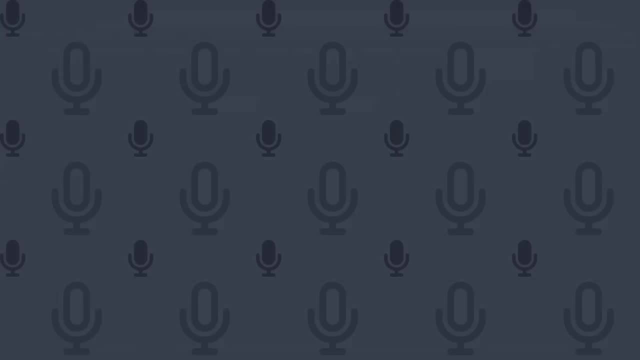 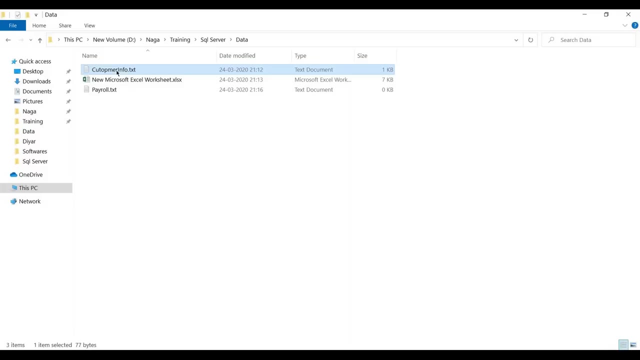 so i can store anything like this. i can store like this. i can store like this. come on, i need to fix this one. what i'm saying is: you see here, i can store here, in this format, any other format. so, in case of database, how the data should be stored. 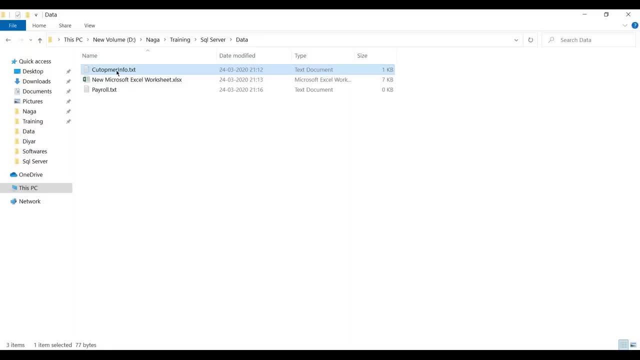 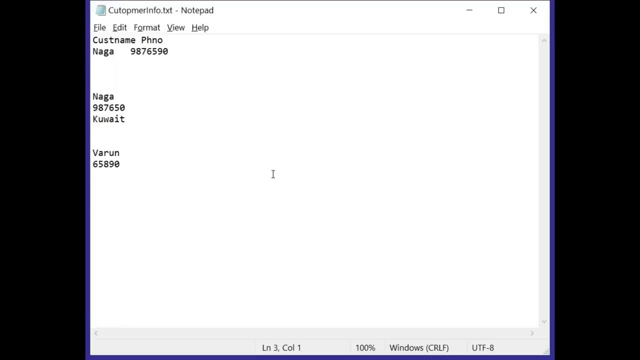 so you, you got my point. you can see my screen. i'm pausing this one. okay, fine together. hello, yes, can you able to see? yes, yes, you can you know? yes, yes, yeah, one minute, i need to fix this guy. i mean, uh, it's sharing, uh, share everything, something like. 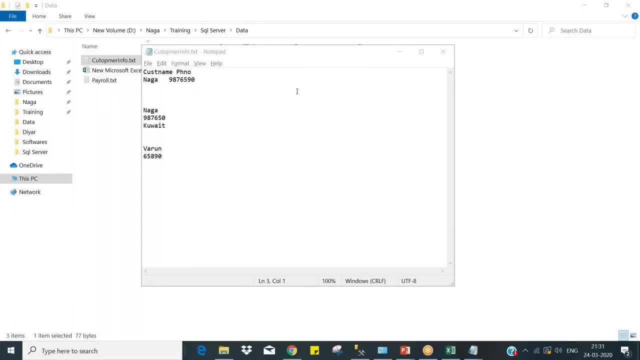 that screen hold on now. i hope it's fine, i don't want to. each time i'm switching it says okay, fine, yeah, yes, share screen is fine now. okay, now you see, like uh, here you have a customer name, phone number i can store like this. i can store like this. so that is uh. any way i can store if it is a file i can. 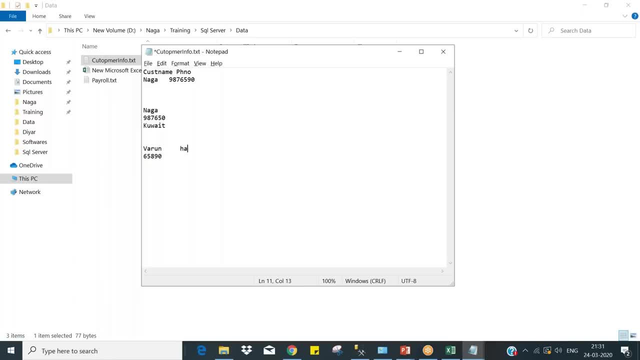 store like this. also one, one customer i will store, i will say harry, and i will say like phone number here i'm storing phone number here, uh, after his name in this next line. here i can store like this: it's my wish. there is no restriction in the file system, but in the database perspective, how you. 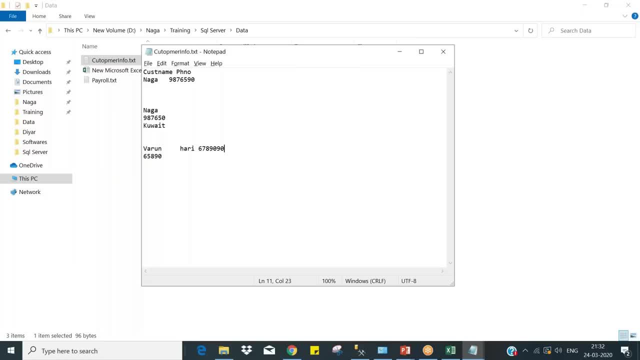 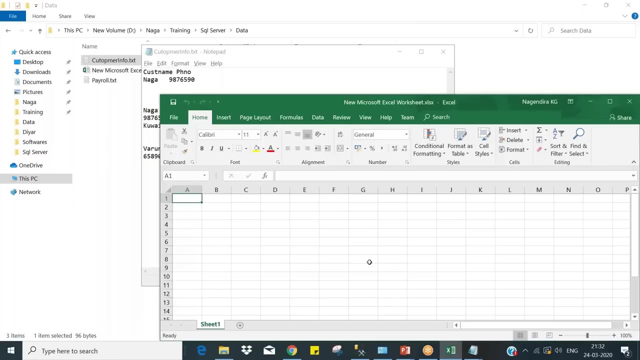 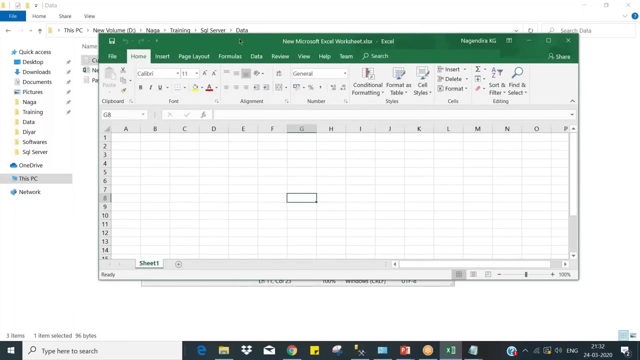 need to store the data. so there is a thumb rule like in dbms: you need to store the data in tables. it's pretty much clear. okay, so the tables are nothing but your spreadsheets to see here. yeah, so this is. your spreadsheets are nothing but your tables. if everyone- i hope everyone- worked on 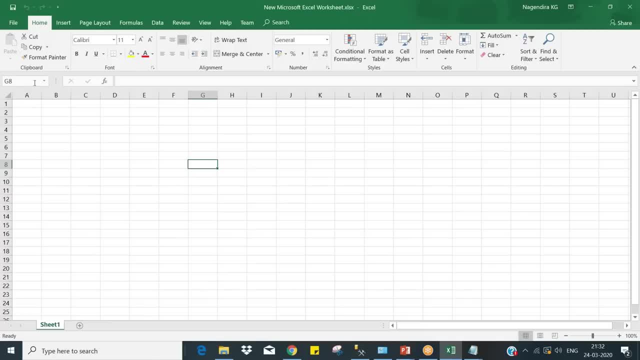 excels. so table is nothing. but you have a rows, you have columns. okay, this is how the data should be stored. so, in order to store your customer detail, you need to define customer name, you need to define- i mean you need to define- this column. call a customer name, phone number. 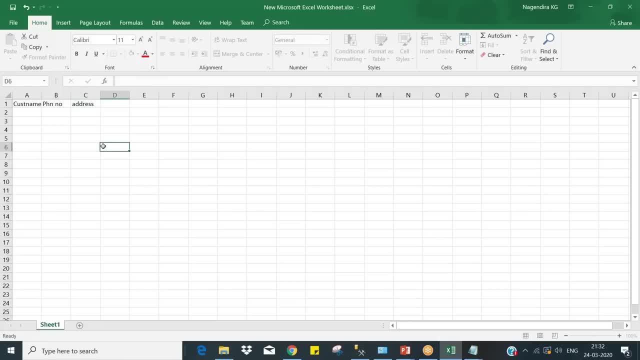 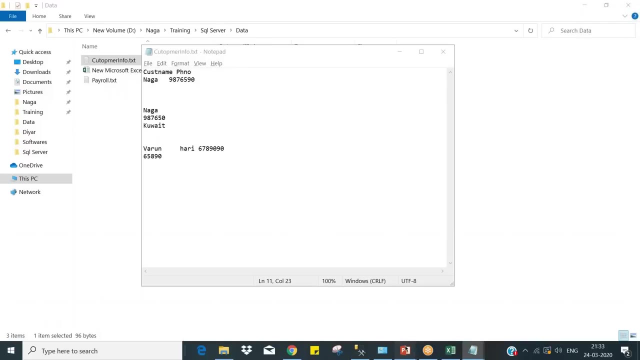 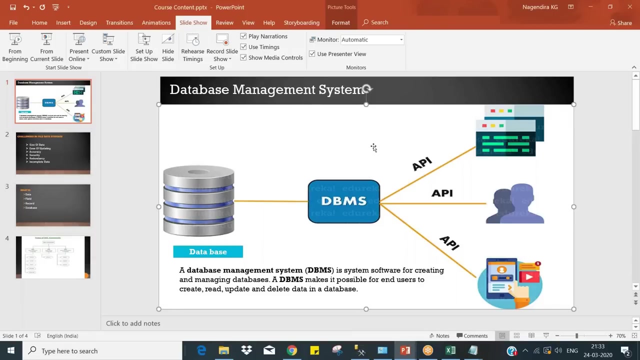 and address. okay, this is the thumb rule: where your data should be stored, i mean how the data should be showed. so your data is stored in a table that is called your relational database management system. so i'm i told about database management system. so there are different types of dbms. object: 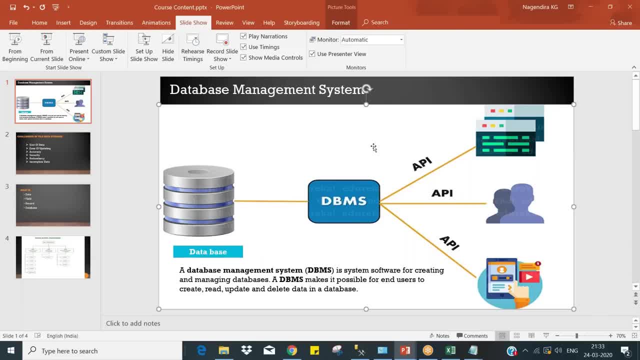 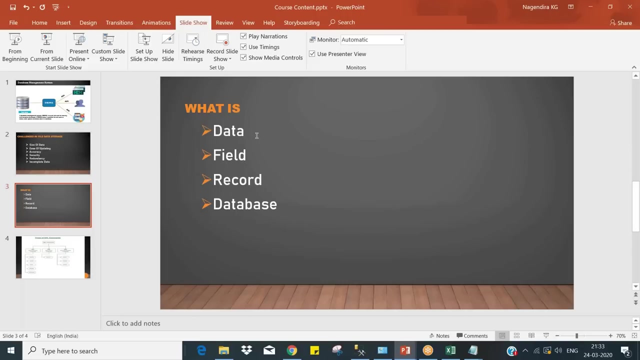 oriented, hierarchical. no need to put much into it. now the full farmers. everything is like rdbms relational database management system, where your datas are stored in a table- pretty much clear. okay, now what is data field record database? this is the hierarchy we need to follow data. as I said, any information is your data field. 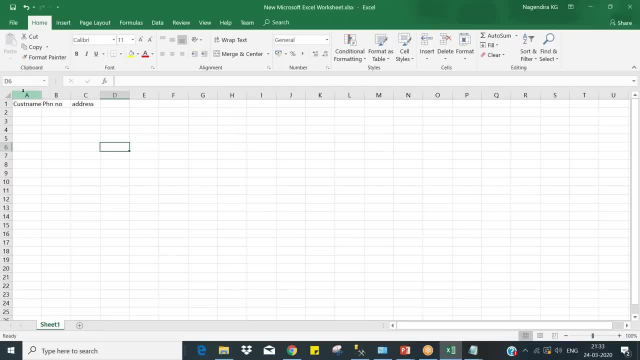 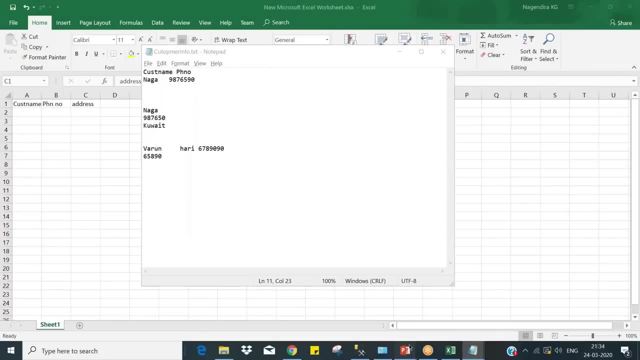 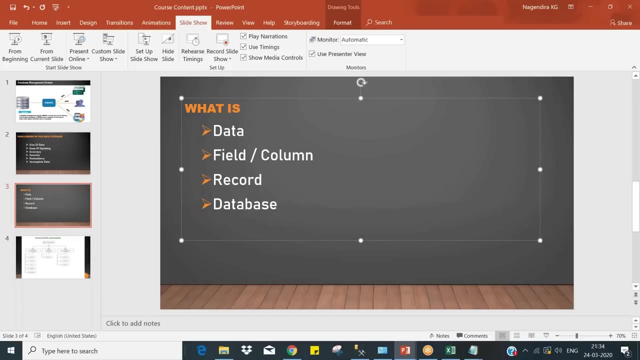 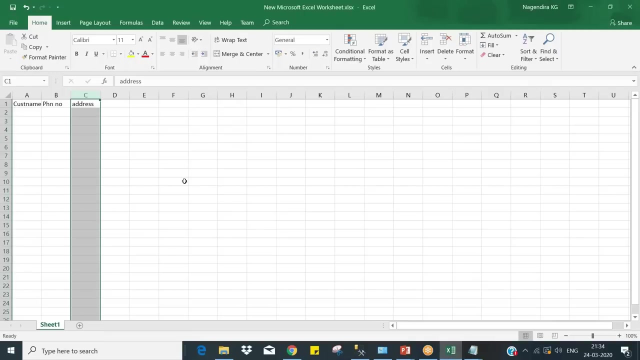 is nothing but your column. each column is your field, technically speaking. when business perspective, any application user will say it has a field. okay, in database world it should be considered as column. okay, so it's a column. then record. so record is nothing, but you have defined the. 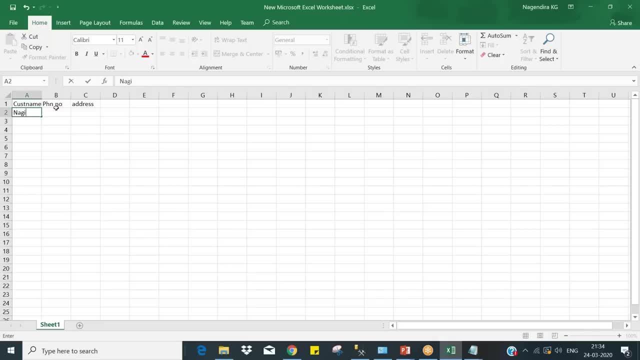 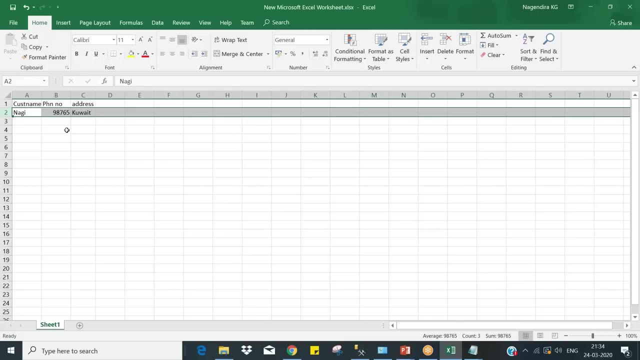 headers. so I am having one record here: Nagi nine, eight, seven, six, five, and I just quit. I'm just typing just country name here in address. so each row, one row, is called your director, or I mean it's it's called a row in a table, or it's a. 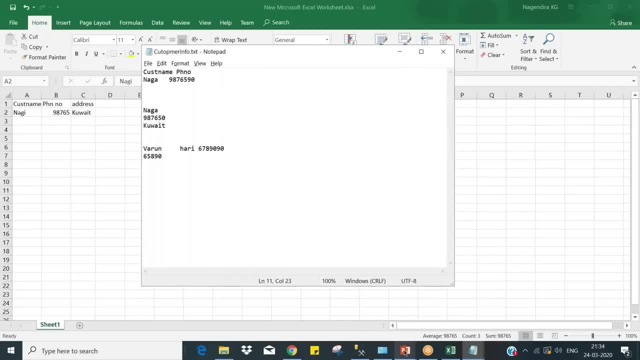 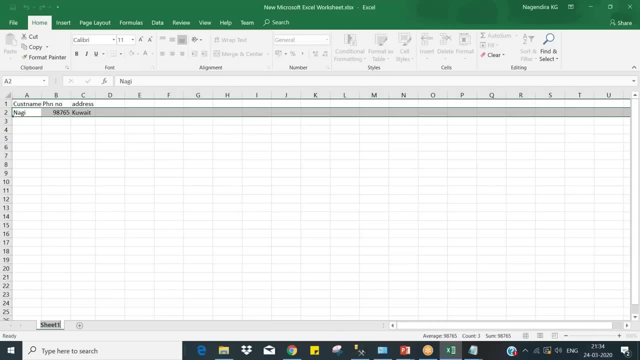 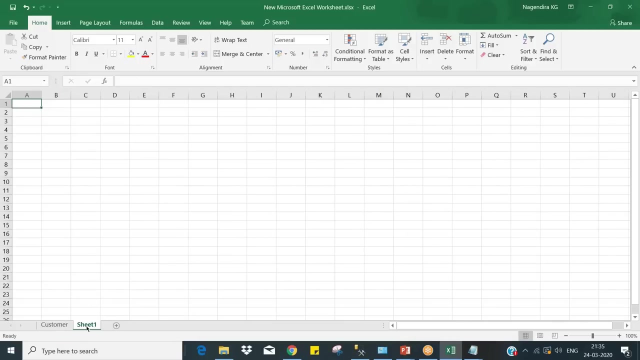 record: okay, that is what you say. it as a record, then database: okay, so I created this. I will name it as customer. so, whether this is considered as a database. now, this entire thing is considered as a table. so this thing is considered as a table. okay, now I create another table like payroll. 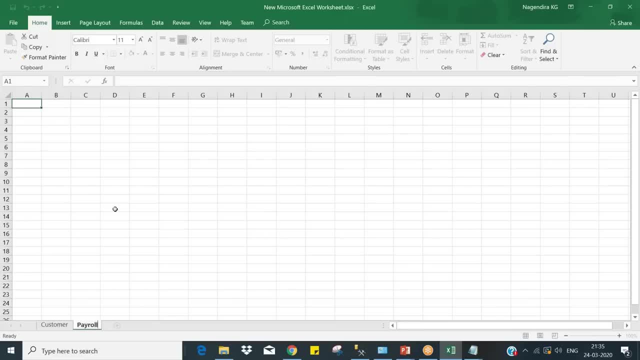 here I can maintain another information. so this is how the group of tables, so your database, can contain multiple tables. this maybe i can say like entire excel sheet, this single excel sheet considered as a database. so this actual sheet is the database and can contain multiple tables. okay, got it, it is simple. 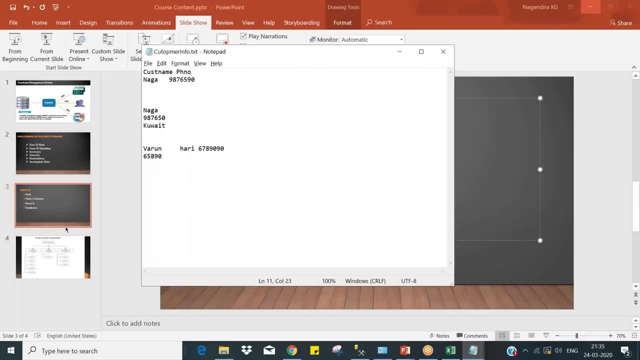 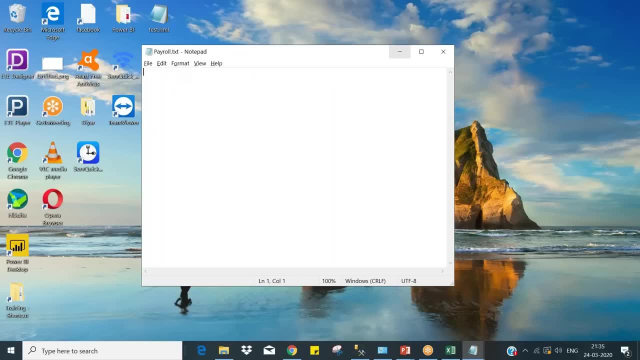 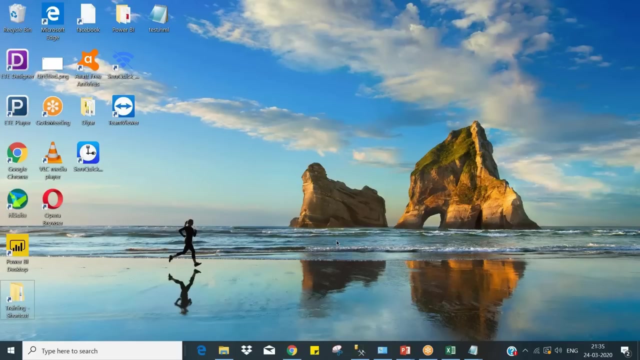 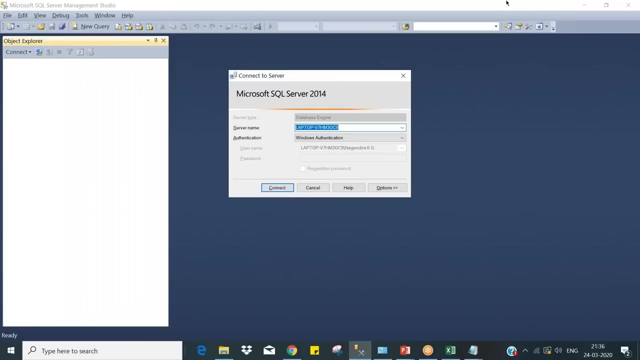 as that. now, with this, all these informations, okay, let us quickly know what is a skill server, all other stuff like this. come on. so you, you got now every idea about data database tables, dbms. okay, as i said, microsoft sql server is your uh, dbms, rdbms, relation database management system. so 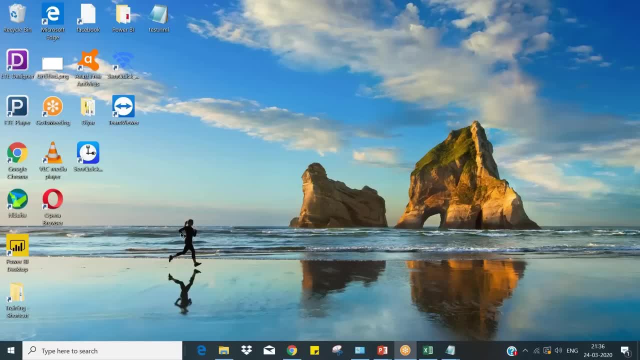 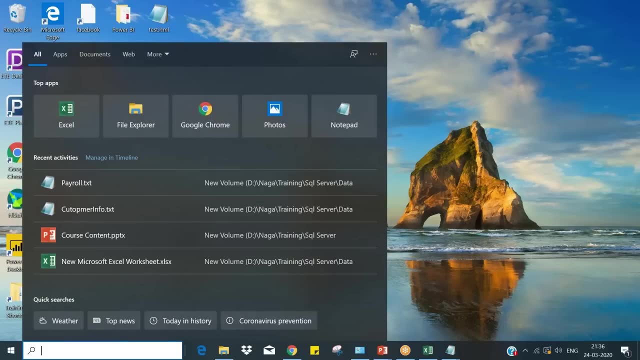 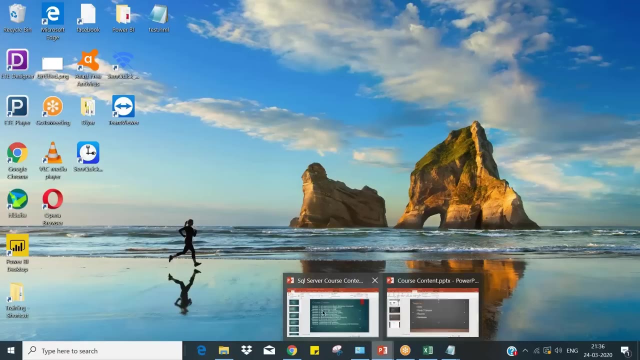 i have probably the link to you guys in the email I have sent. you need to install the softwares so that it will install Microsoft SQL Server engine. so the architecture comes like this. okay, I need to go back here, say for example: now I am saying about: 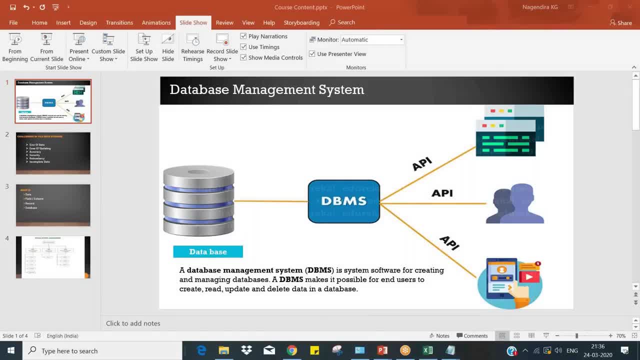 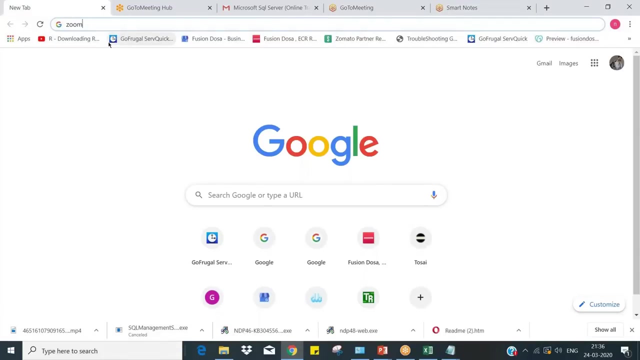 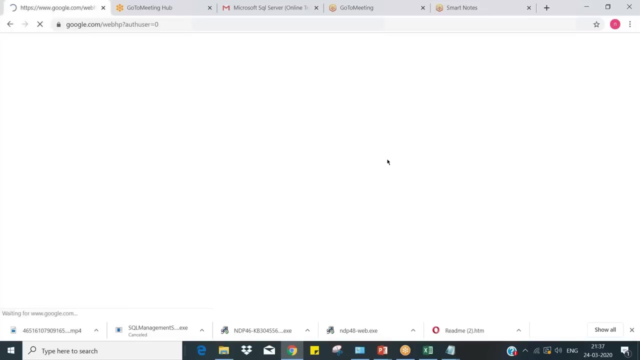 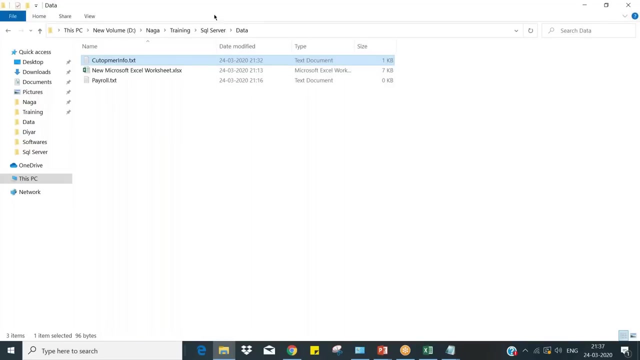 this two-part, this two-part, okay: database and DBMS. so whatever link I provided in the email, that will install your SQL Server only. okay, this alone, the center part alone. it will install the second software. maybe I will quickly show you, guys I need to go to make. 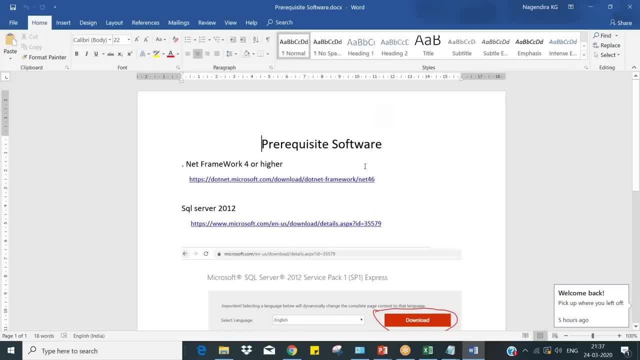 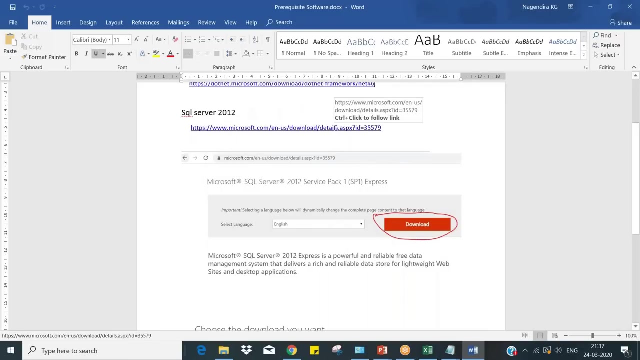 I need to expose the system name, as my blog would be, so that it can tell me everything I need to know about your data. okay, so thisnet framework is. forget about this. there is no concept related to a SQL Server. all this SQL Server built-in dotnet code. so that is why I 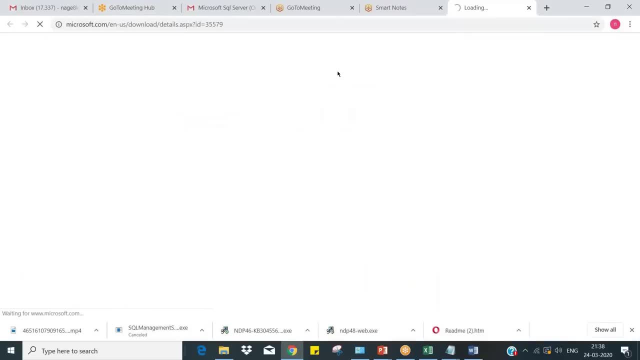 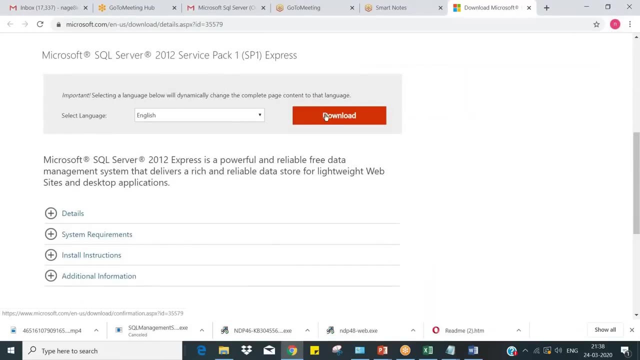 Microsoft asking you to install. forget about this, this is not related to our topic. then a SQL Server- see this link- is nothing but your SQL server as a DBMS. it is nothing but your RSS code. it is nothing but your DBMS, your server, the dbms software. okay, this is what you need to install. download now, as i said, you. 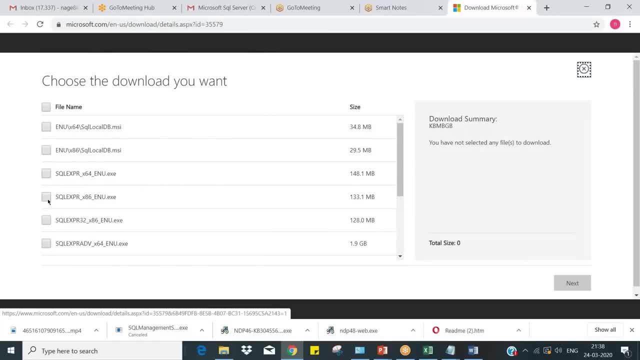 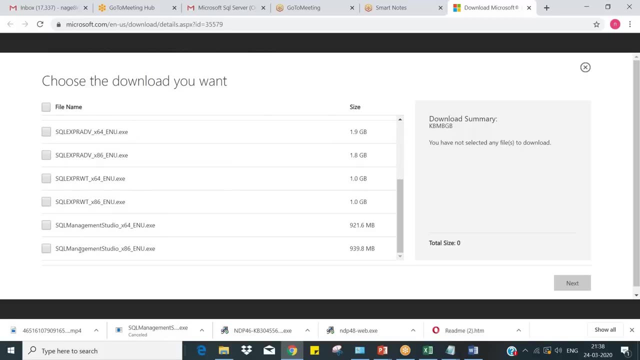 if you have a 64-bit, you choose this one. if you have 32-bit system, you choose this one. so this will: these two will install your dbms. then what about this management studio? it is nothing but your client tool to connect see server is the software. as i said, it's a software, just a software. 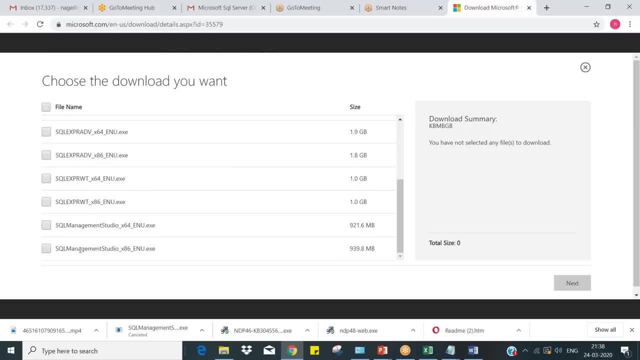 that will sit in your one desktop or server system- i mean any server, dedicated server- then you need a management studio to connect to that server and you want to manipulate it, create a database, or you need to query it, as you asked. you want to select, create tables, whatever operations. 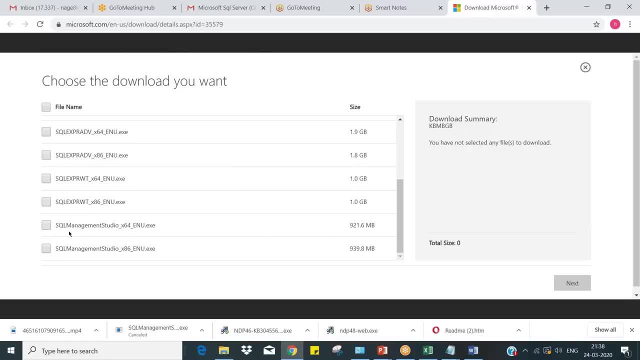 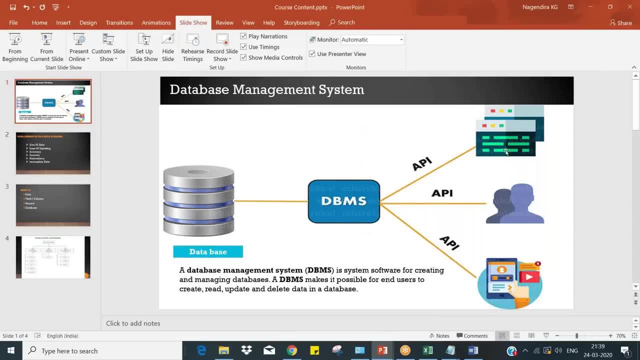 you do. you need to have a client. this is management studio is nothing but your client. okay, so in this picture you don't have that uh cap. you assume this particular picture. uh, maybe i'll say this one has, uh, your management studio. so first link will enable you. 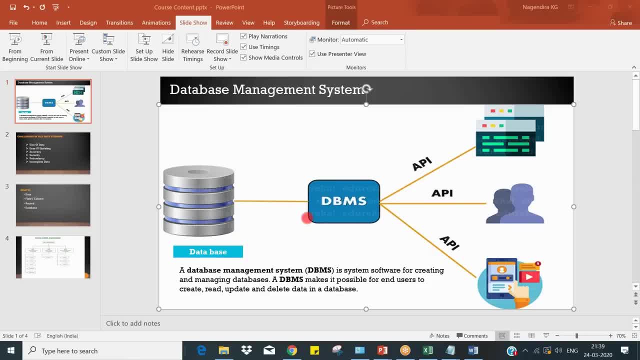 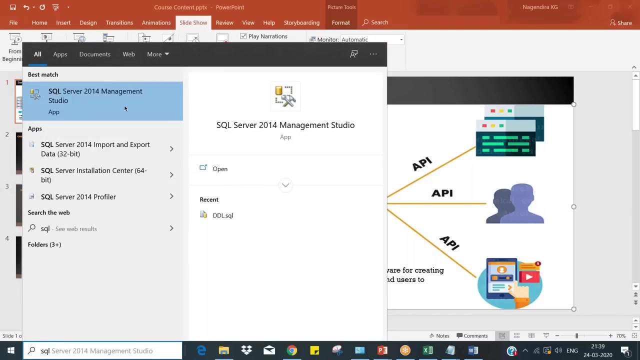 to create the dbms next link management studio, you need to create and database or all of the strips. okay, so i will help you if you find a difficulty in creating. i mean installing. now i already installed dbms database management studium. that is nothing but your sql server. i am trying to connect with your management studio at that client once you install. 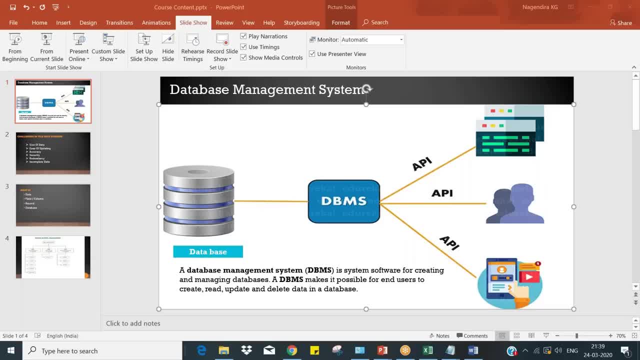 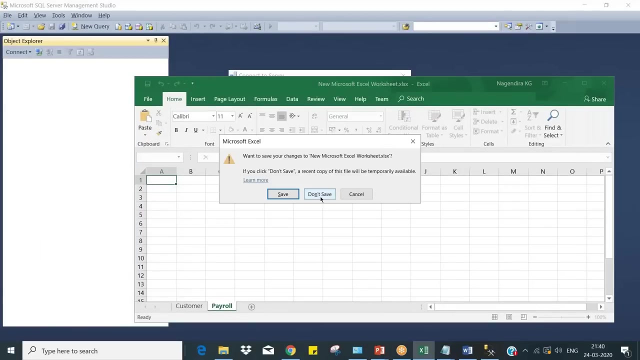 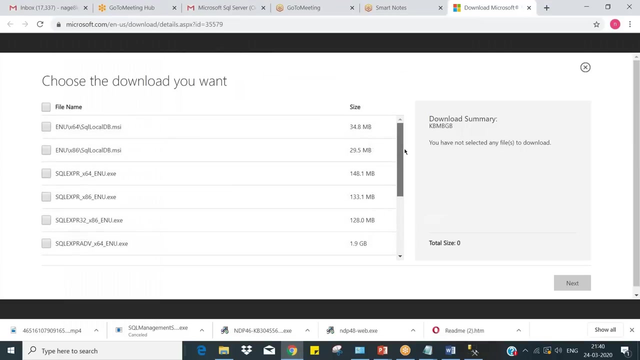 it. so we need to choose 64 or 86 according to system requirement, right? yes, yes, based on your system, you need to choose either of those. i have selected four options. you choose any two. that's enough. what are the two options? right? just see, i told you like here i mean x64, x86. you no need to install both, i mean download both. 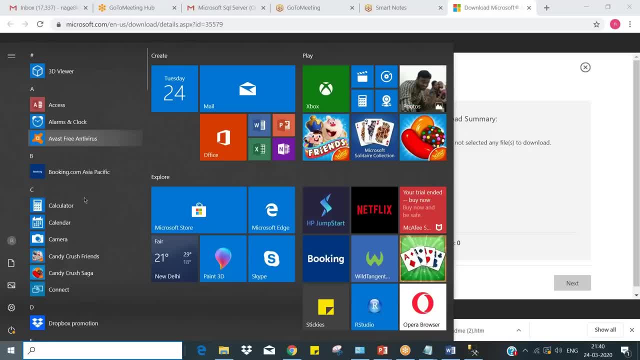 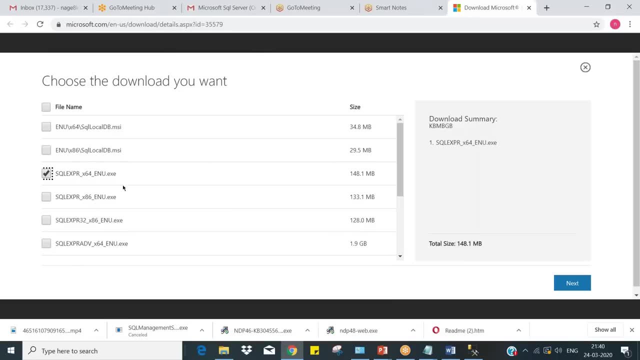 secure system configuration in my computer like here: yeah, i can find. okay, whether it's 32 bit or 64 bit, you choose a, in my case it's 64, i'll choose this one and, uh, this one. that's enough. then click next and go for. 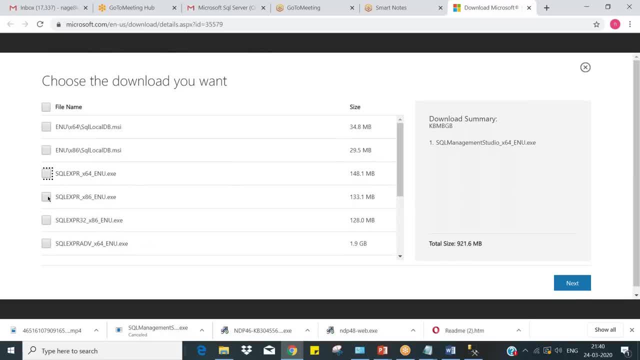 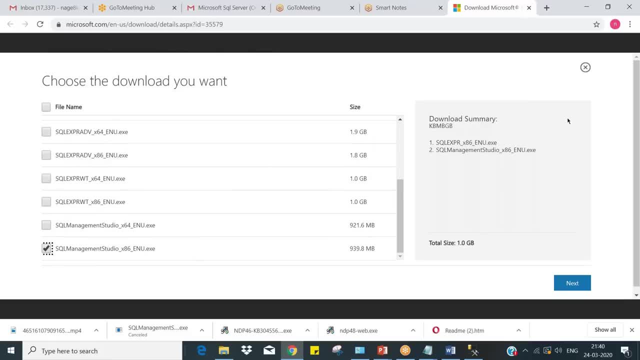 it one gb only, and uh pravin told uh he's having 32 bit, so he installs 86, this one as well as this one. you need to choose these two, then go for it. okay, just download and install it, uh, by default options. next, next. next. 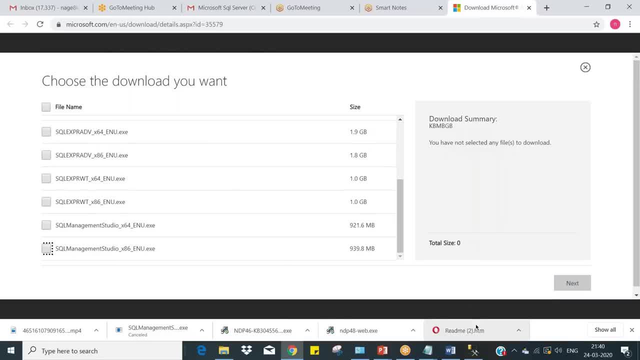 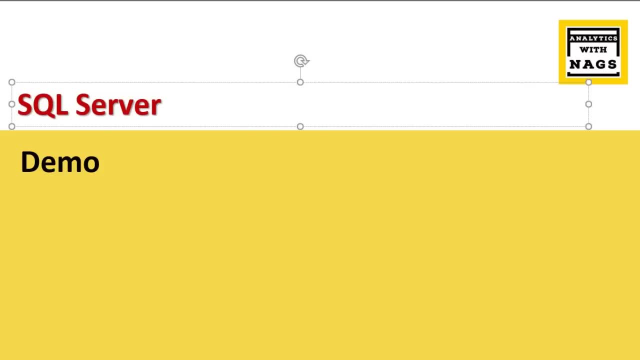 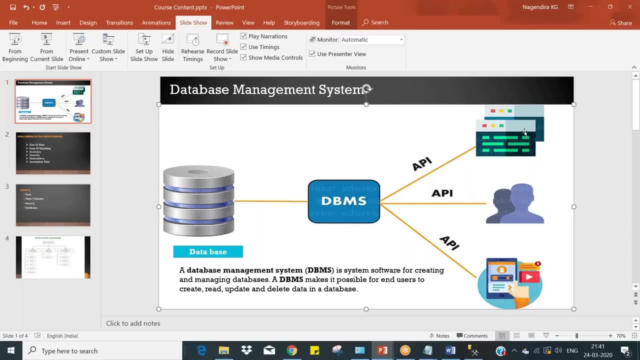 then you will get all the environments like this. okay, now, this is the client, as i told. see, this is my dbms. i already installed it will go and sit. you cannot see this one unless you have the client. just you have to connect the now this part, uh like. 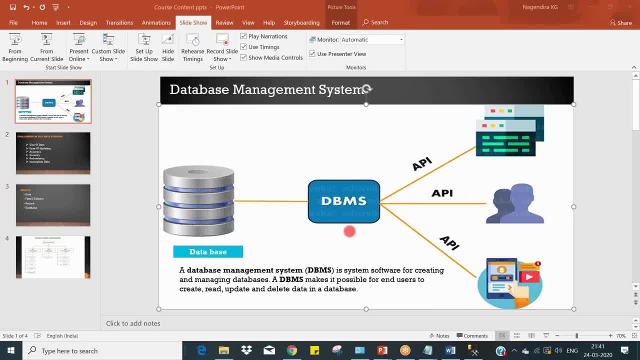 this database won't exist. only this one is existing. okay, dbms software. now you are connecting to the dbms software and you are connecting to the dbms software and you have to use the dbms software to go and install it. okay, then open up the dbms software and you will see the dbms software. 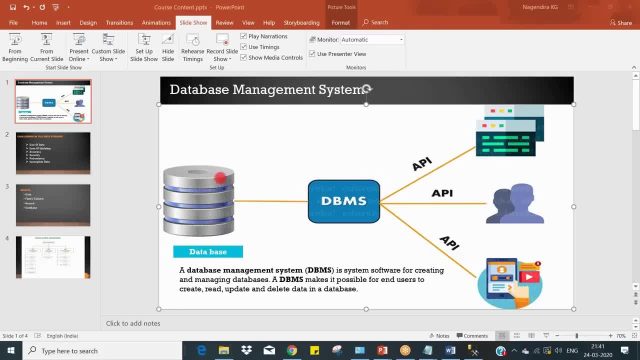 are connecting to the client, then you are creating a database, then you create table inside it. okay, all these things you need to do manually. once you install the dbms, it will not have database in place. you are doing only the dbms at first place. okay, now already installed, so this is my server. 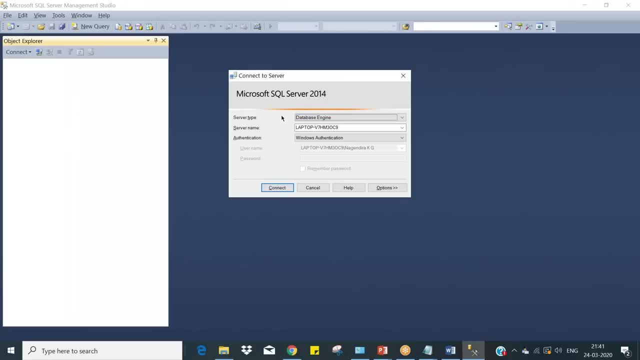 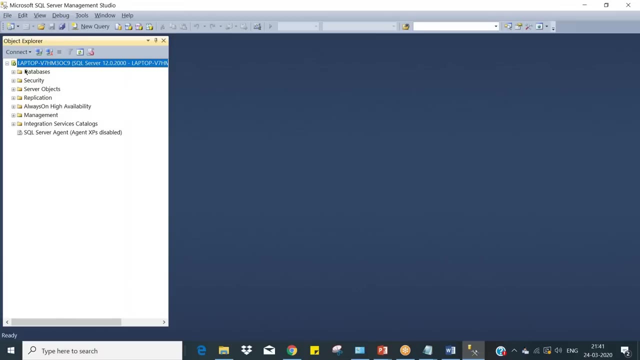 name. as i said, this is the server. you go to other engines, you forget about all those things. server name: i will give my server name, then click on it so it is connected. so this sql server management shooter is your client. it's connected to your dbms. that is sql server laptop. this is the server name and this will have all this architecture. okay. 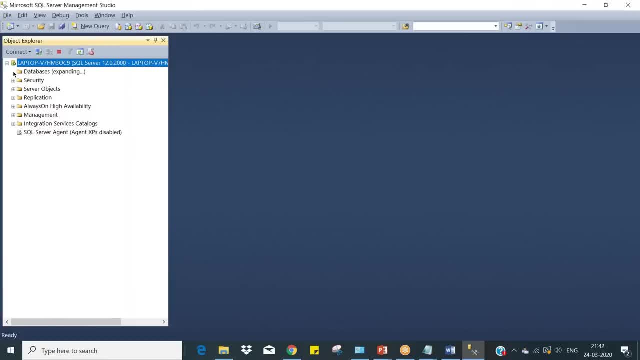 i mean, we will go through it later now in order to create database. i already have some databases, so in order to create databases, one of the main advantage of michael soft product is that you know minimal coding. you no need to write coding much. instead, you can write. 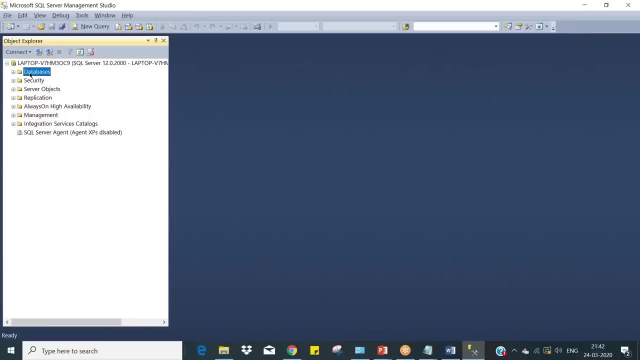 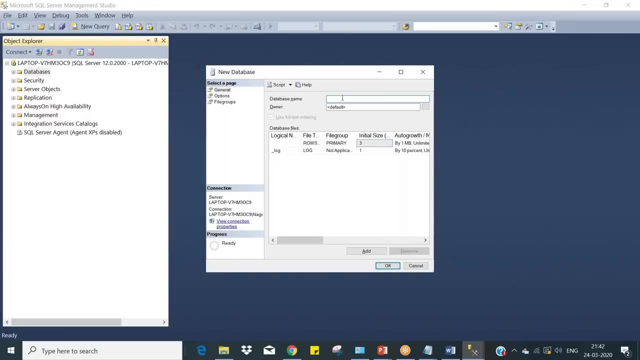 i mean you can create using a gui, so just right click on it: new database. i will say, like sql training, it's feeling this wrong? sql training, corona, all right, so this. so it's as simple as that, just for the name. these file groups we'll explain later, just click on okay. 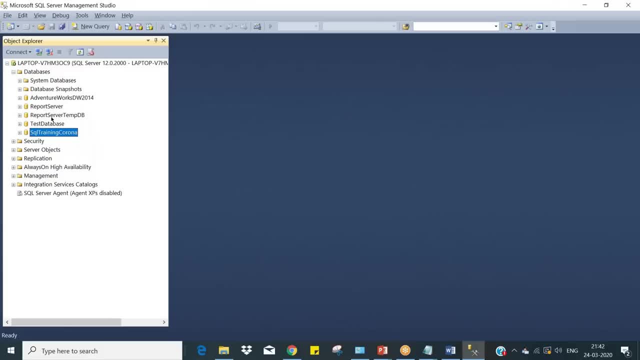 then you can see like sql training corona here. okay, these are database i already created. so once see, this will contain the folder. i mean databases inside this. what will have inside this one database? under the database only you will have tables views also. also this one only will be the真的 database. fighter only. you'll have tables views also if you just want to directly organize it. also. another average��: acontece, we won't generate more database. it will take out for that. you know, put in a cool, a little bit extra space on pokebank under the database. will you just want to create more database? 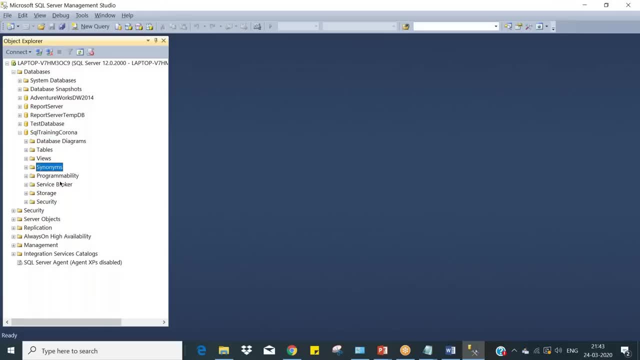 those things, the disadvantages, whatever we face in the file system, like security and you have a consistency, i mean the user should not have restricted access- those things can be implemented using these uh options. okay, we will. while going through the sessions, we will, you'll learn that one. 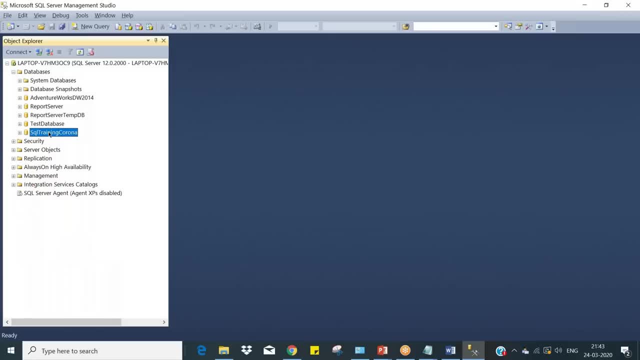 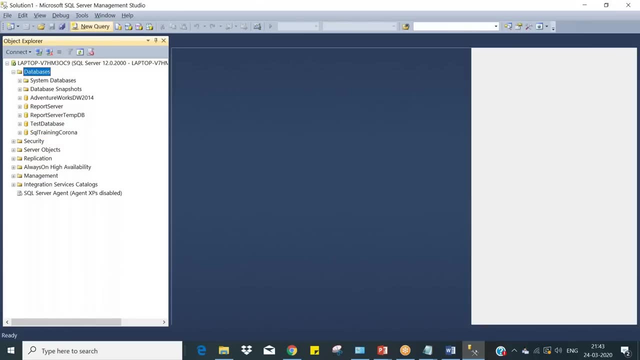 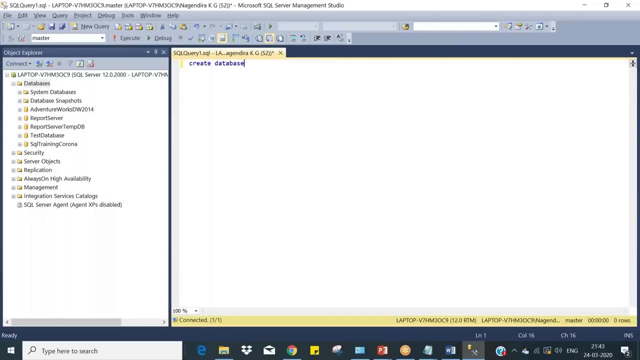 now. so this is the database. uh, you can create it like this, or you can choose this one. you can create a new query. a new query, i'll say create database. i'll say test two, something like that. okay, this is also way of creating it. it is as simple as that. so 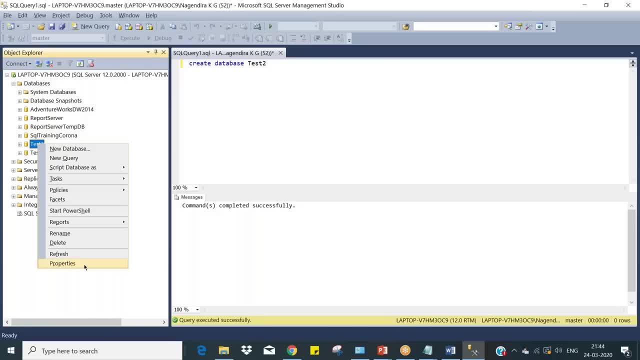 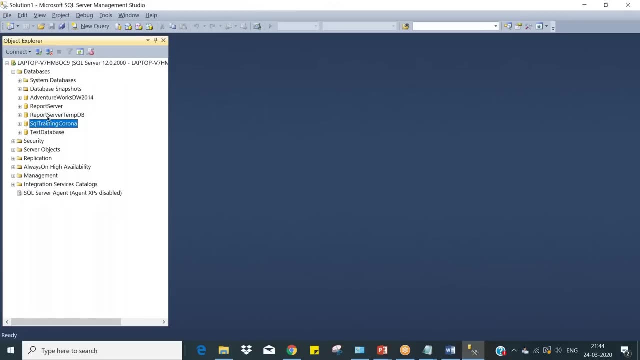 you have test two here. okay, i don't want it. just i want to show you guys how it has been created or how it should be. now we'll stick to this. so, how to navigate: see once you have your database in place. okay, here, you choose that. 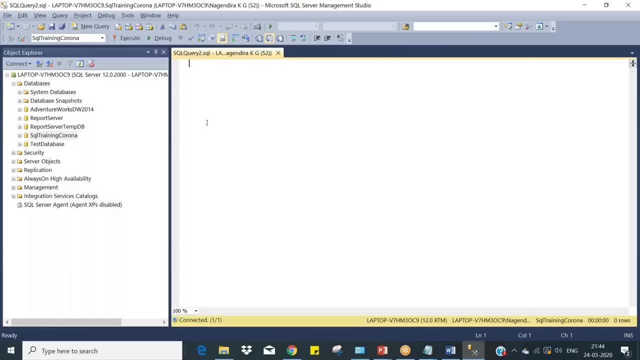 database, then press new query. okay, so now you see, this is highlighted here i mean: um, let us have a spotlight. you see, uh, highlighted here i mean sql, training the database. then you can start writing it code. now, as i said, you need to have the table to store the data. so, as i said, like here you have. 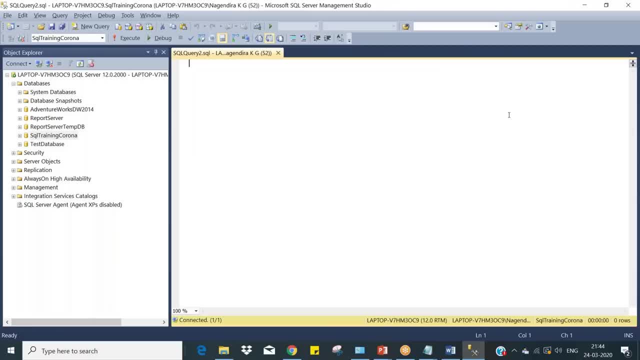 customer data. so these are my customer data. so you cannot copy and paste and store it. you need to create a table first. that table only shows the information, okay, so instead of wasting writing the codes, i already prepared some kind of uh scripts over here. i'm in module three. 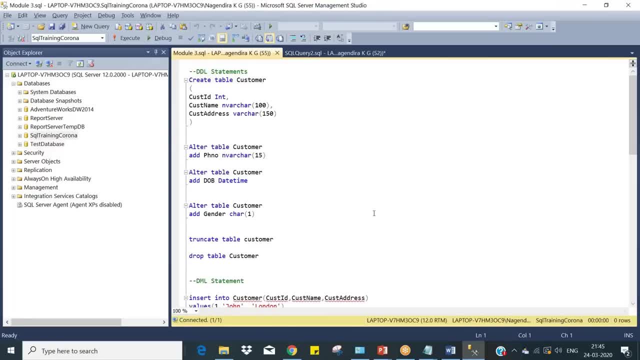 okay. so first, as i said, it's a customer information. so this is the syntax for creating your table. so it starts with create statement and what you are you are going to create: create table, customer customer id, customer name and address. so these are the things i want to store. so just imagine with the excel example: these are nothing but your columns. 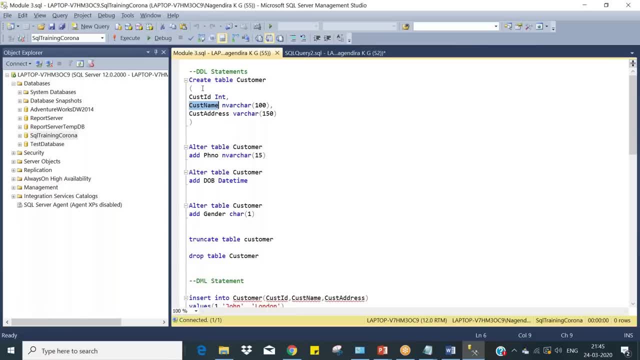 or fields. so you are just creating a metadata that is headers. okay, uh, so that these columns is going to hold this information. okay, this is the column name. and what about this? these are very important part. nothing but your data types. so any programming language or anything which have a data type, meaning, what is the type of your data? 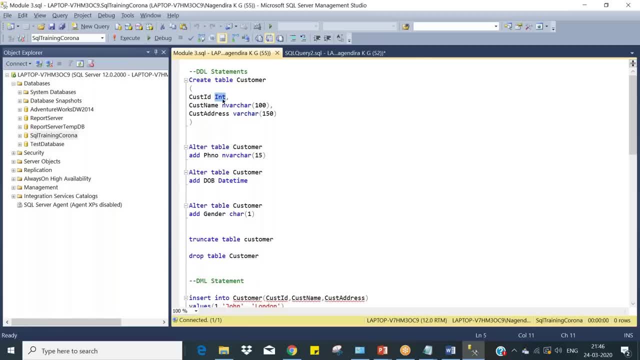 say for example: this customer id is set as integer int. integer is nothing but numerical values. it will hold the values from one, two, three, four till, uh, some limits, three million or some million it will hold and the customer name should be back here. that is character. it should not. if you put. 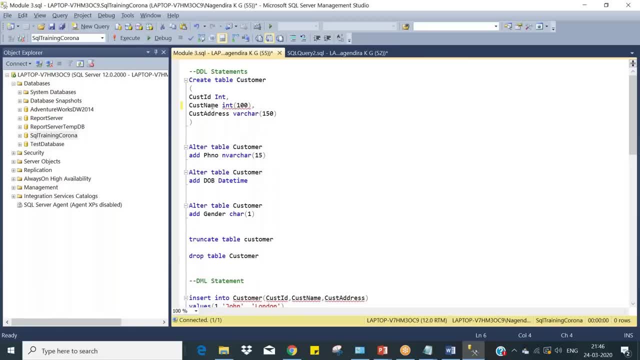 integer over here. it will throw error in this place. if i want to insert nagi, it will not allow. so it is saying that restriction to your data. what data is going to hold? that is your data type, type of your data. you need to declare it. there are. 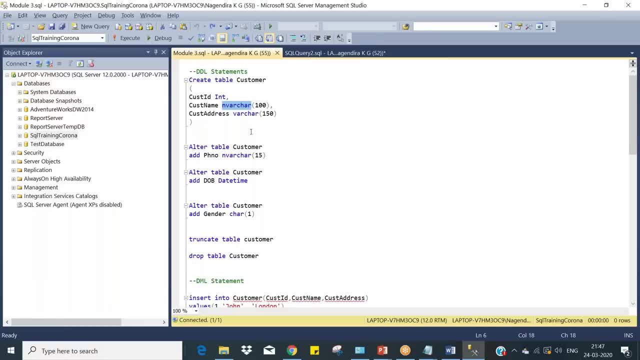 number of data types. mostly we will use integer and worker. we will go through it. i will share you the link there you can uh study what are the different types of data types and when we use this, when to avoid this, what is the difference between work and work, and we'll go through it just. 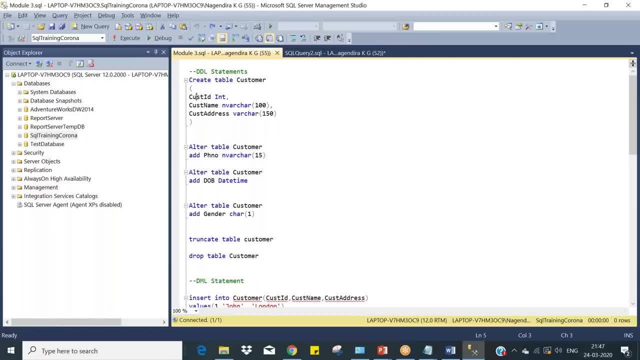 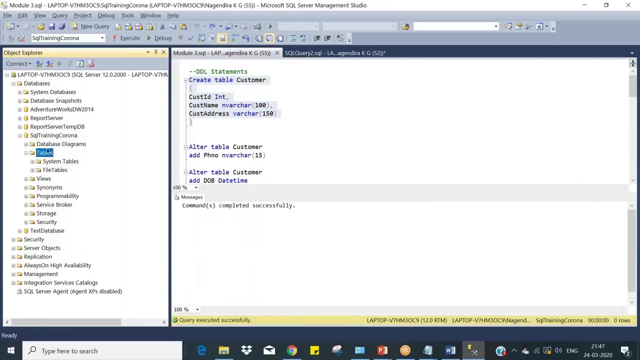 for now you focus on table. this is the column names and these are the data types. okay, now you see here i don't have any tables. now it will, by default, it will have system tables, so i will just go ahead and select this. once i select this statement and do execute, it has. 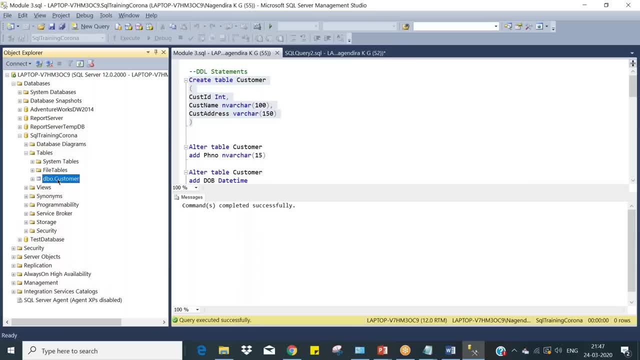 said completed successfully. then do a refresh here. you find a table here. okay, this is the customer table. now, as i said, how i can see a data inside the table? i cannot see like this. i can see the columns. what are the columns, all those things, okay, but i cannot. 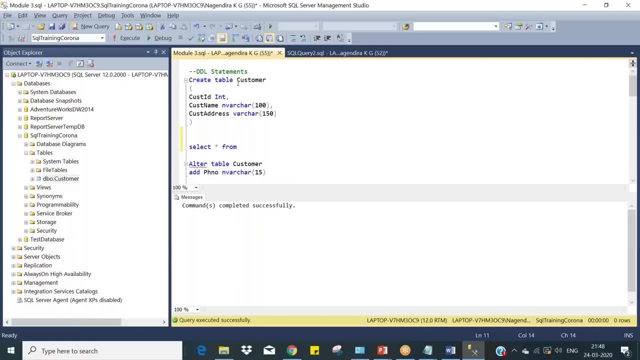 have any data. i mean, i don't have any data. it just creates the structure. now you see, this is the data: customer id, customer name, customer address. okay, so there is no data, and how you want to store it. wow, i'll know the answer. it's okay. fine, so basically, you created a schema or structure and you want to insert. 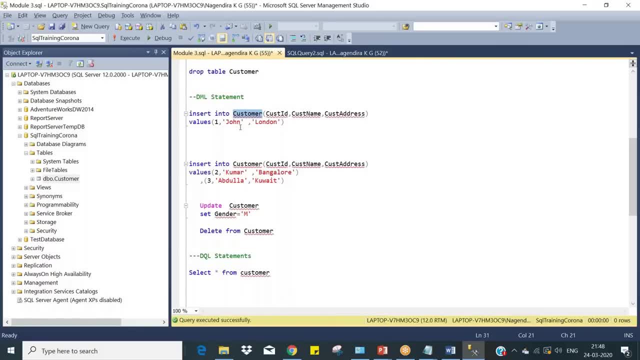 the data. this is the only way you can insert into a table. i mean, you need to explain this by insert into what is that object name? that is, object name is nothing but table. then you need to mention the columns. so this is john and he's from london. now, when i select this statement, 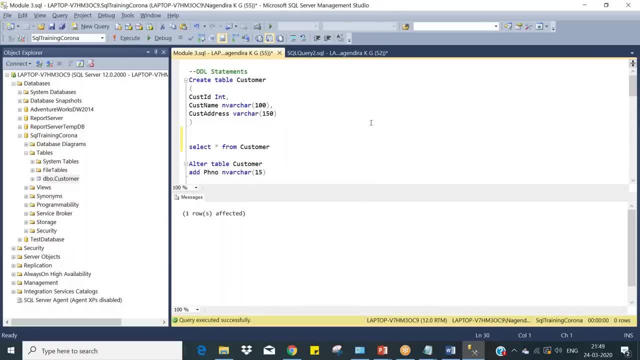 you're gonna need. okay, now go and see the data here. so one customer information is stored. so this is how your datas are getting stored in the database. it's flat. I mean it flat in the sense it will be row by row, so this is called a row, this is called a field, this is called. 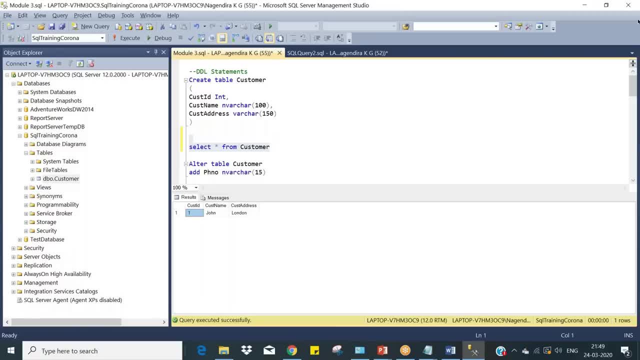 a field, and this is each cell, is data. okay, this is how it is related. now let me insert some more values so that I can find something useful. so now I have inserted two more accounts, so this will have. So now you got a clear understanding about how you can still do. a semicolon should be at semicolon- end of the query, some. 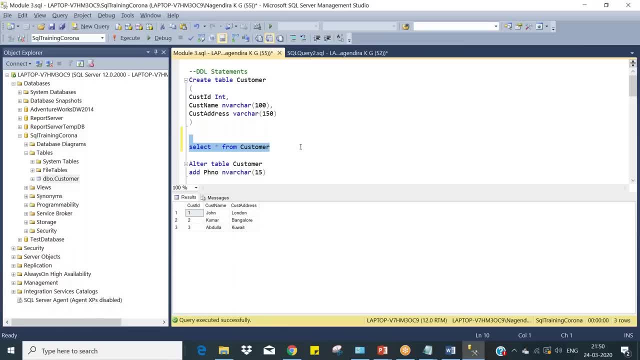 other. should we had any at the end of the query? yeah, as I said, so it depends upon each DBMS. our DBMS in Oracle, you need to do in mysql, you need to do what I studied. when I studied, actually, I was forced to. yes, that that's what I said. so syntax was go ahead, go. 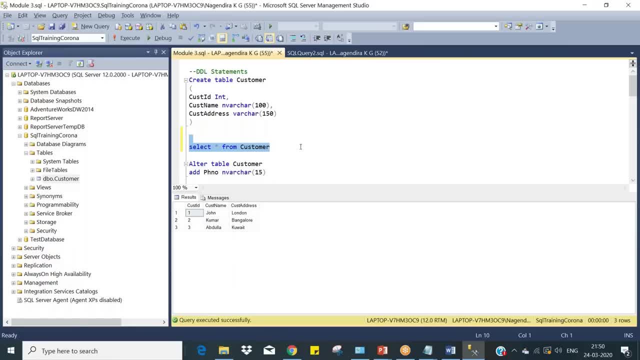 ahead, but I you did not add a semicolon at the end of the query. yeah, that's what. so, as I said, this SQL is a standard. I mean, whatever I written here is the skill. each and every RDBMS has its own syntax, so in SQL server there is no. 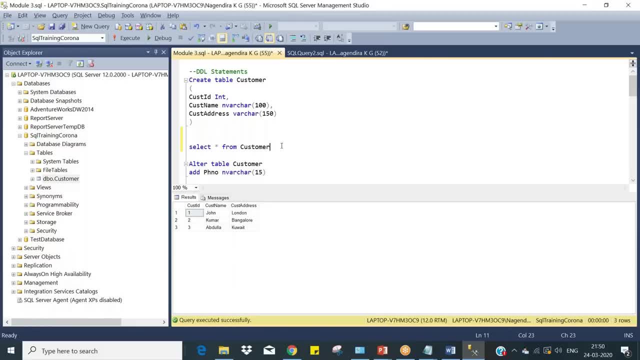 semicolon in mysql. even in Oracle, I'm not sure there might be a semicolon okay. so that is no thumb rule. so you need to focus on one particular technology or querying or RDBMS if you, once you are familiar, then you can compare while learning. I recommend you focus on this for now, then 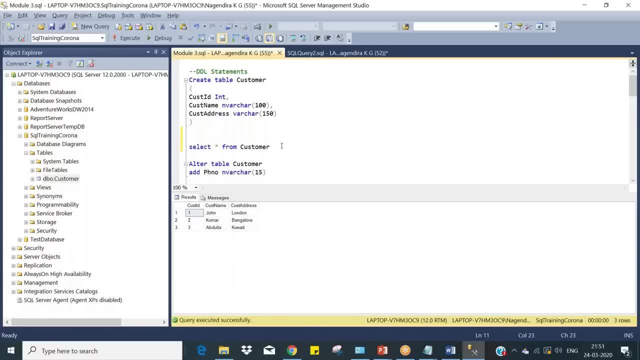 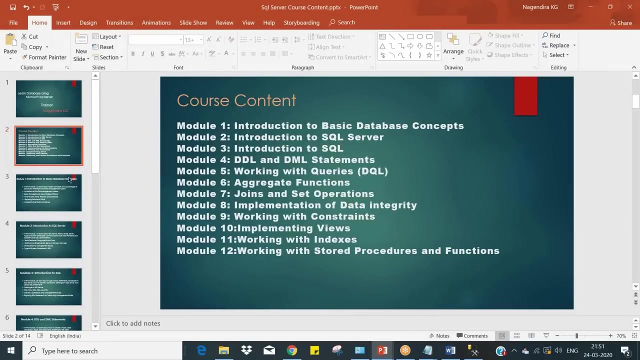 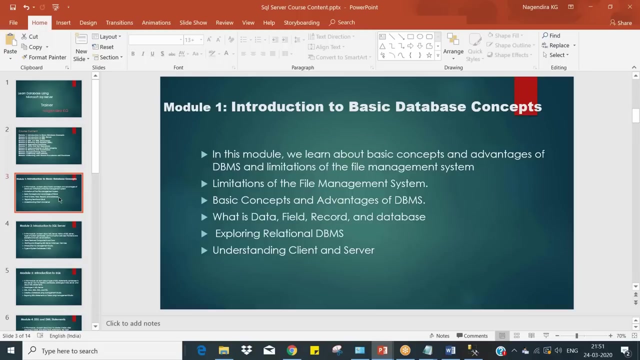 you go for a comparison? okay, because you already did study on that, that's fine. I'm saying here in SQL server: no need, okay, you, okay, guys. so this is your about the table. okay, now let's focus on your syllabus. so you see, like limitations of file management systems, I have covered. 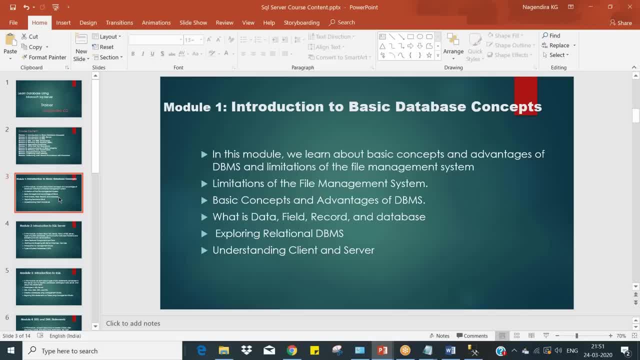 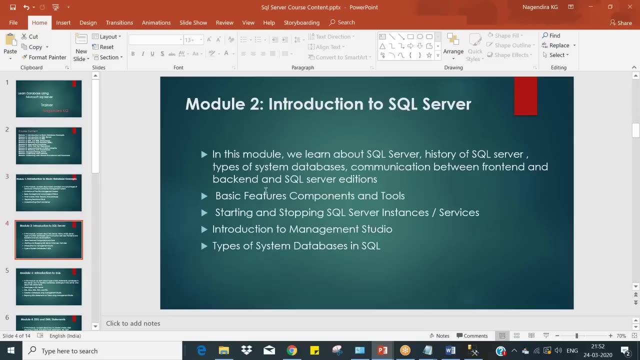 basic concepts and advantages. basic concepts is like a server client architecture. what is different about a server client architecture? what is data field record database, exploring relational database, management system, understanding client-server? so mostly this. this is history. basic futures components and tools. yeah, so you need to starting. 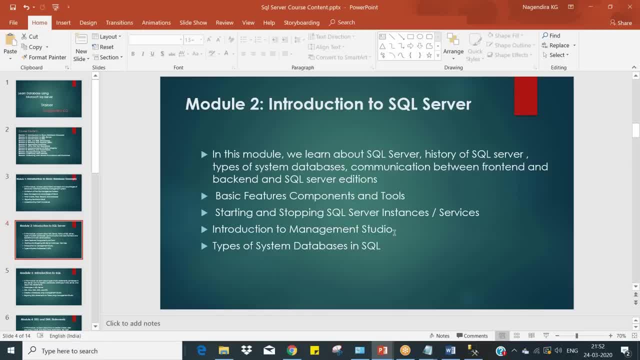 and stopping. these are very small things. introduction to management, should you. whatever I use, this is the one types of system database in this field. okay, fine, this is a typical value for data table, identity data and specific data types. now you are left with one and one, and this is what I will explain in the next. 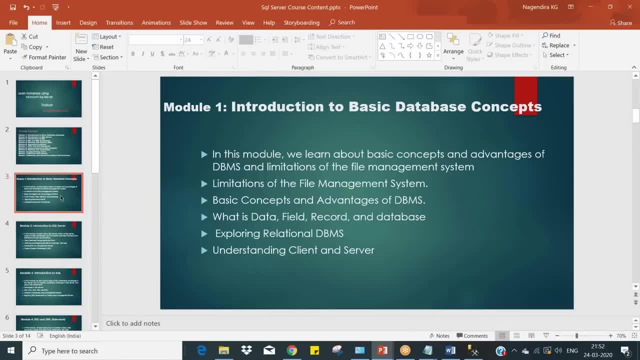 slide on how to use dynamic entire data database management system so you can check and see how it works. so when you are working with a new data system, the first thing you need to do is to find a specific database, and how do you know where is it located and what is the database location? 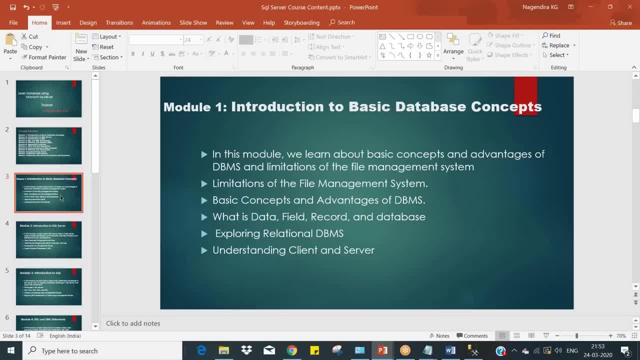 uh, to rephrase my sentence, it's a software. okay, then what comes a relational database management system? you need to store a data in a relation manner, so how? it is relational manner if you need to store it as a table, so every table is a relation. that is what it's: a relational database. 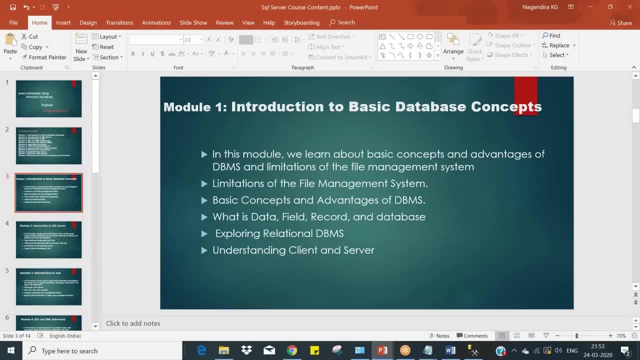 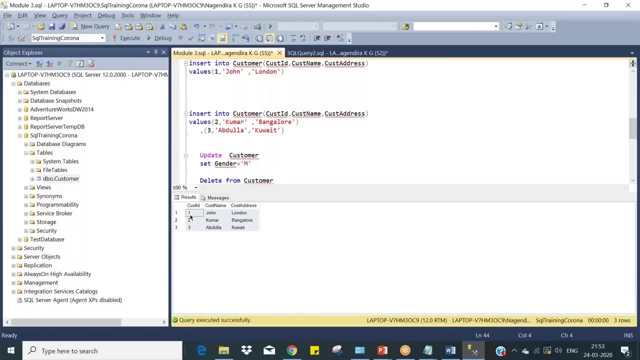 management system. okay, so how it is related. let me explain with the. so, basically, rd dbms, i explained. now you see the customer id. this london is related to this id. this london is not related to him. so every table is a relation, every column is specific to this particular person. it is not. 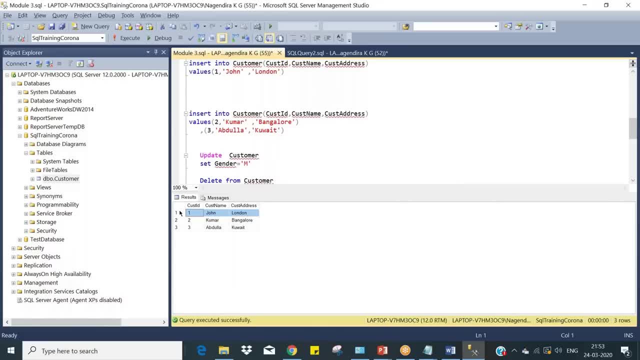 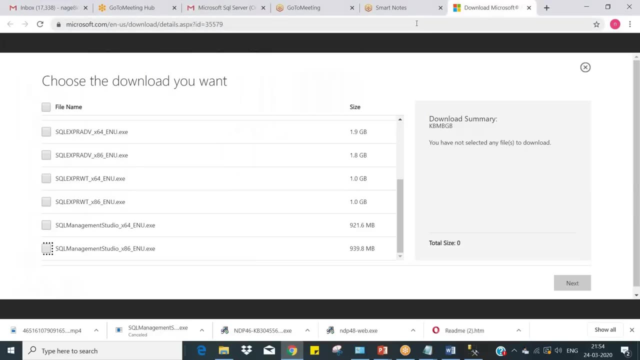 specific to this guy or this guy, so this entire row is called a relation. they are building a relation, so this entire table is called your relation. okay, not satisfied, i think. okay, no, no, i'm saying there are other ways of managing dbms: object oriented, hierarchical, relational. so they consider everything as object hierarchical, all those things. 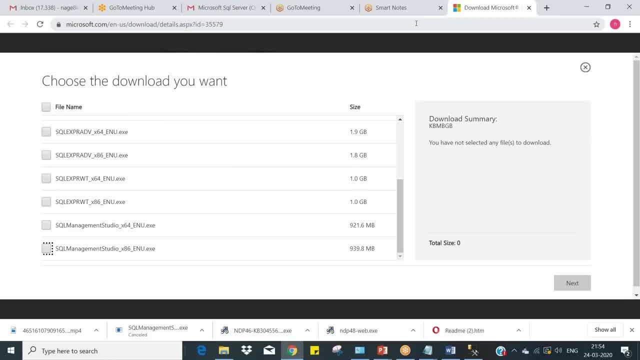 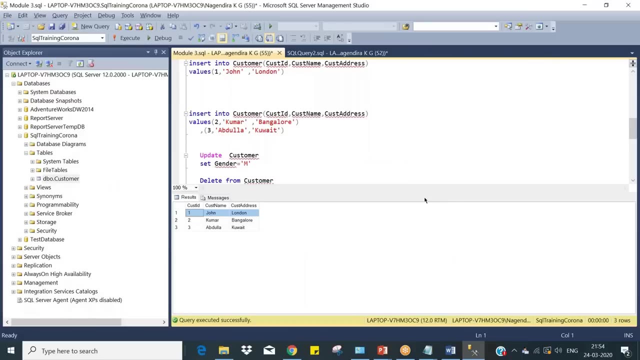 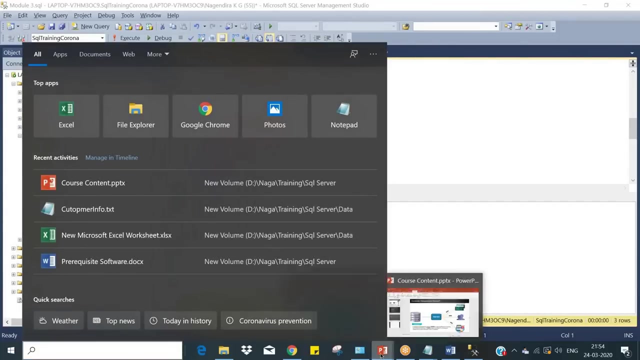 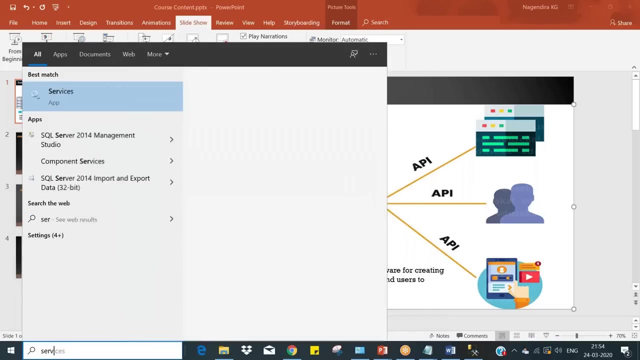 now, relational management system is nothing but purely. you need to store the data in a table that becomes your relational database management system. that's what the definition of it, and every table is a relation as the thumb rule. okay, now let me explain some more thing about services. so back to this guy. so this guy just sits as a service. you see services. 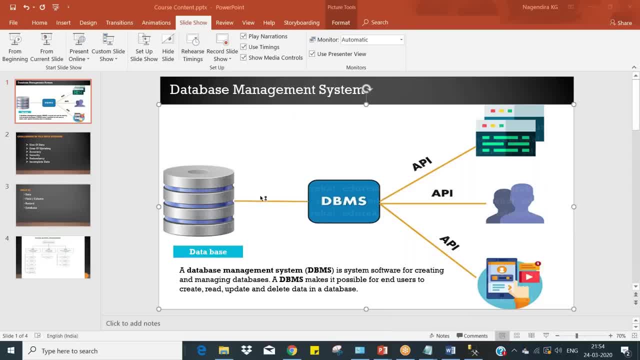 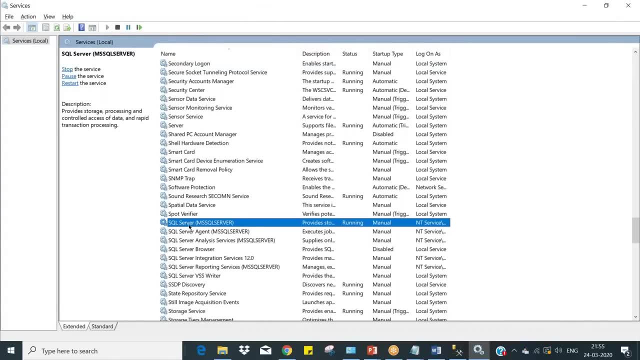 dot msc. you see here this is the guy. sql server is nothing but your dbms database management system. that will run as a service. this is running okay. now he is the one i mean. uh, we are running. now. when i stop it? just see, just see. 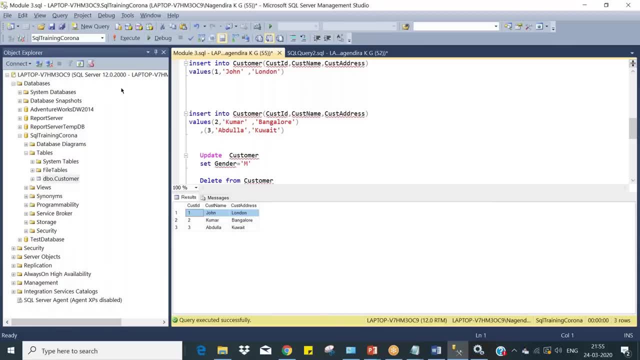 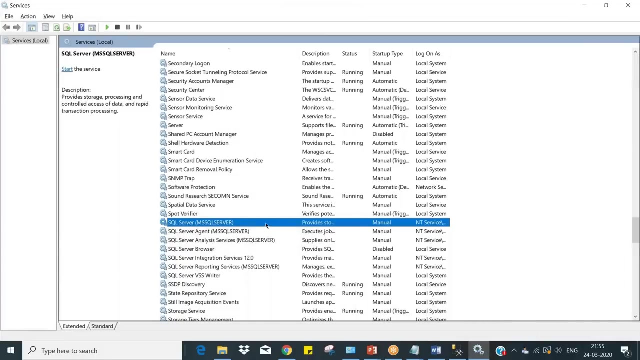 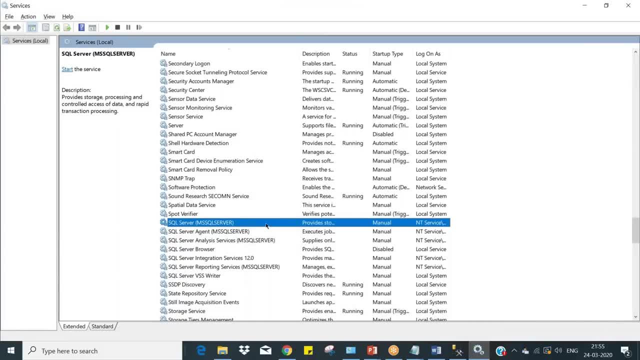 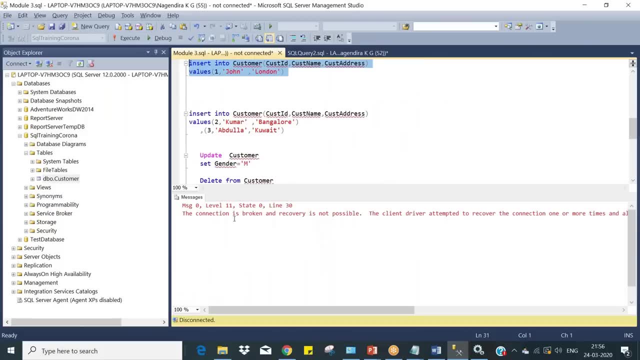 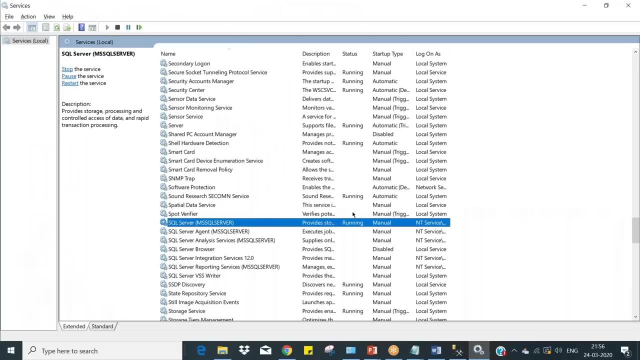 enabling you to run the management. should i mean dbms? so this is the service you if, if there is some issues like this, just go and check the services. connection is broken, recovery is not possible, something like that. okay, let us start that. so it is already running. now, when i go and uh, run something, i, instead of 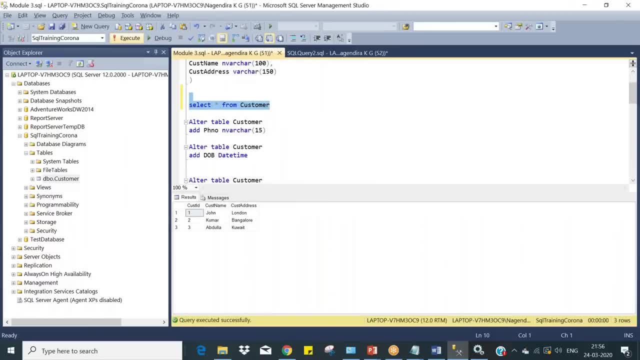 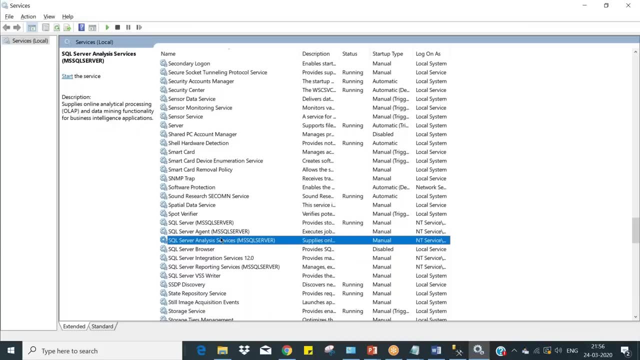 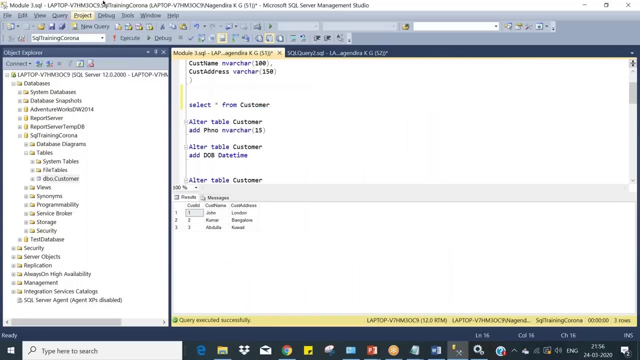 that i'll select this statement that will run immediately. now it's working, okay, and uh, your management should. you also will run as a service, i think. wait a minute, microsoft sql, not sure? okay, that is not as a service. so this is your service and management should. as i said, 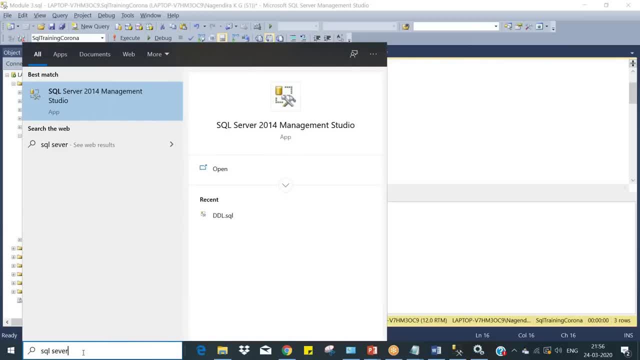 you can go and check it here. sql server. this management should do. this is your client tool. that is what you want to understand using this. only you told about toad. toad is a client tool to connect your article, so it's not a database toad, i think. 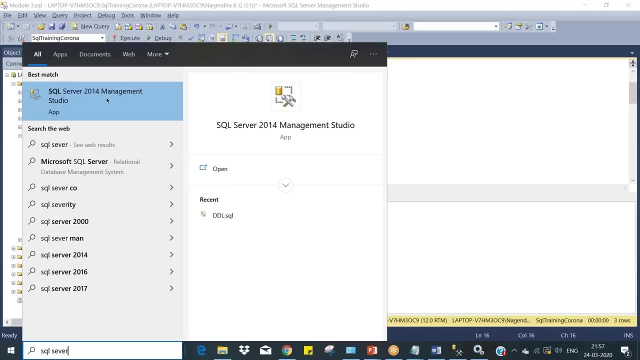 if i'm not wrong, varun, can you tell me article you use toured as some other client but toward? i don't have much idea. i heard about it. clear toad is a client tool, tool to connect, I think it's otherwise. it's like ID integrated development. 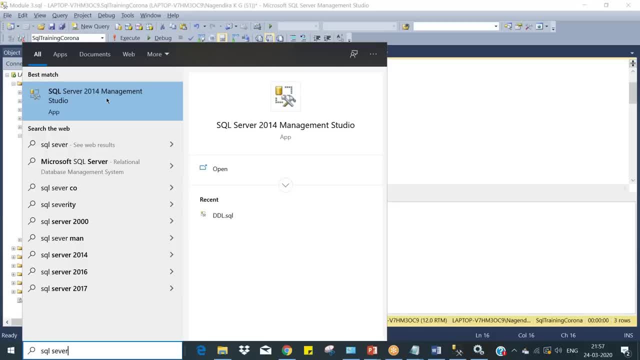 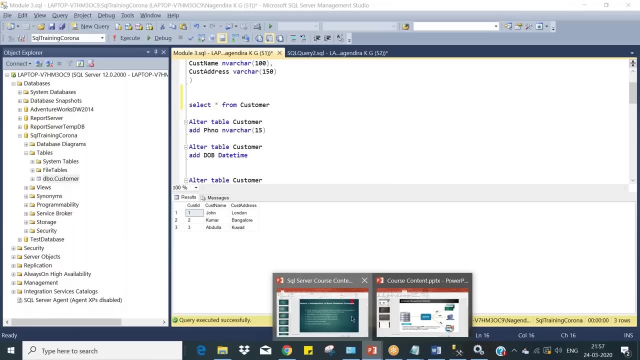 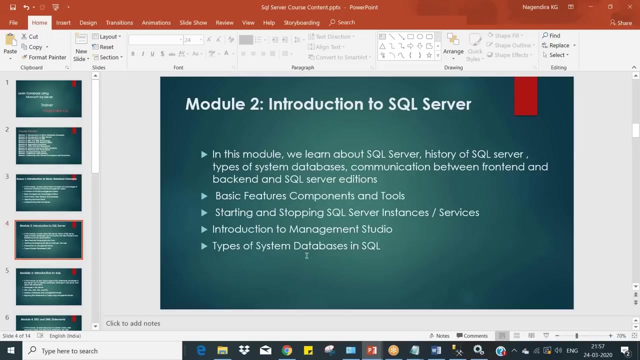 environment kind of thing, so you can connect to server clients, all this thing. so it's a client tools. okay, it's a client, basically. so management should use your client and your SQL services done on underneath, okay, so this is the things you need to know about then. what system databases? 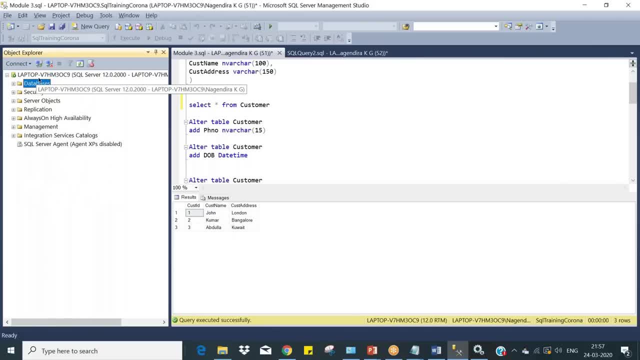 okay, now see, and I say, like I connected, this is RDBMS database management system. when I right-click on it, okay, create new database. it has created me a SQL training database with all the schema tables, view, synonyms, all these things, how it creates, basically, the system. 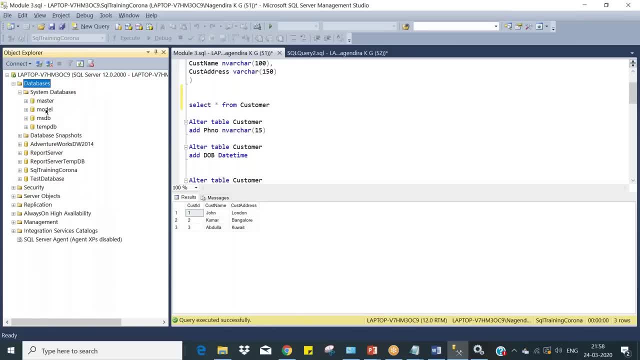 database. if you expand it, this internally create a model database: master database, MSDB, temp DB, all those system databases to process. basically, this model will have the all the content to be created when I just create a name, so this will create a one copy. this is taken as a copy, then this database is created. so 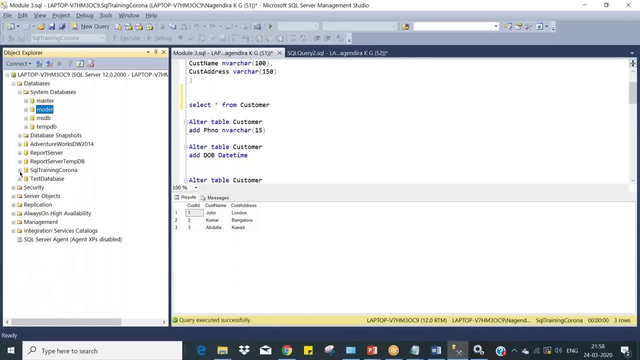 already they have defined how it should create all the metadata over here. okay, so just a copy and paste and renaming it to whatever name we provide. that is what your model database and this master information. by default, all the data should be stored- metadata, if you see. like what is my system configuration. 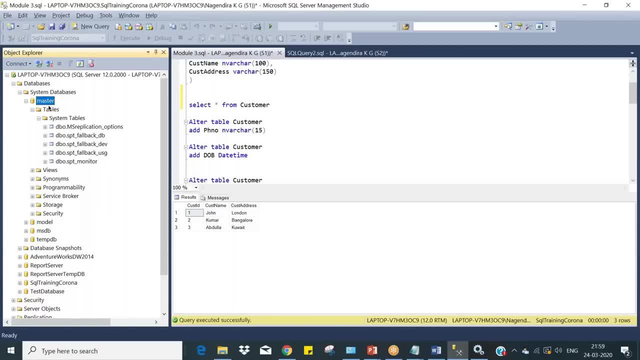 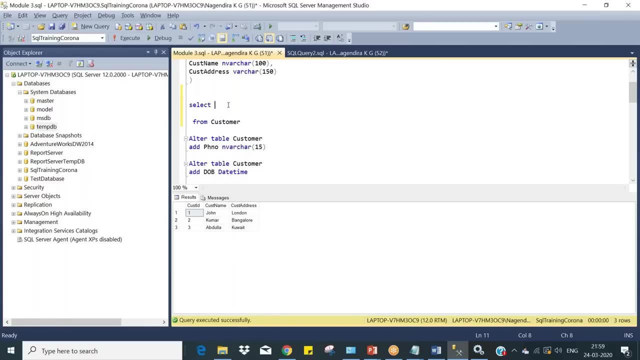 all other stuffs. okay, this should be stored in some key database that is called your master database and I'm not pretty much sure about it, but temp DB. whatever processing you are doing, say, for example, it requires select 70 plus 80. okay, 70 plus 80 is 150. very easy answer. so I'm running this. so 150 is your answer. so 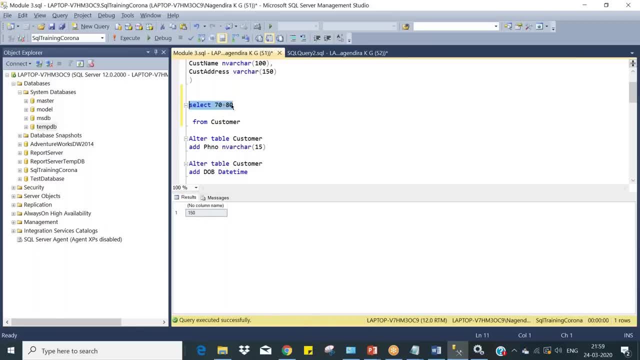 this requires some computation, some memory power to calculate. so those calculations will reside in your temp DB. so basically, as a software it doesn't do anything on its own. all the things is doing using some kind of system databases. okay, so these are the main purposes. we will, it don't? 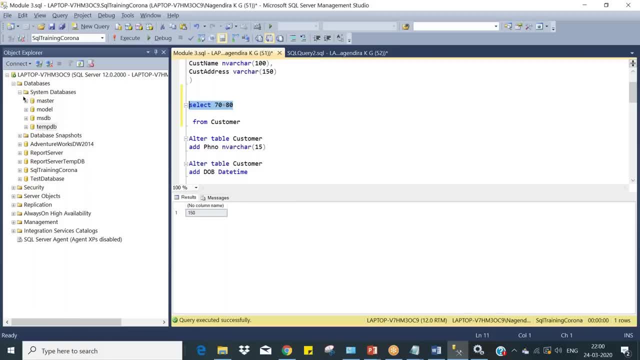 look much into it. okay, if you look into much into it, you will get confused. we are never going to use that one just to for your understanding how they will create all those things. questions will arise. for that I'm telling you: forget about all these things. you just focus on your data and the history. there is a 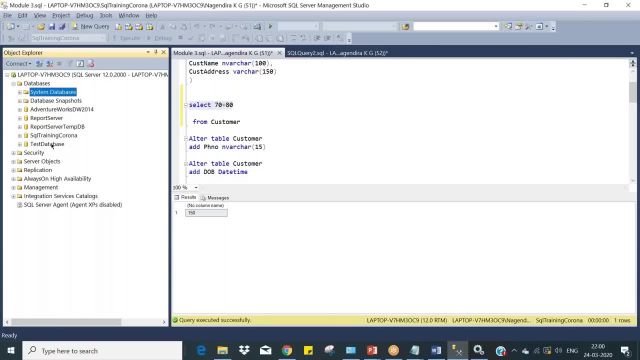 disadvantages for using a file system. that is why we came to database, and in database it is not just a database. we have a database management system underneath that will use it to create databases and all your- and it is called relational database management system- and your data stored in a table. so this 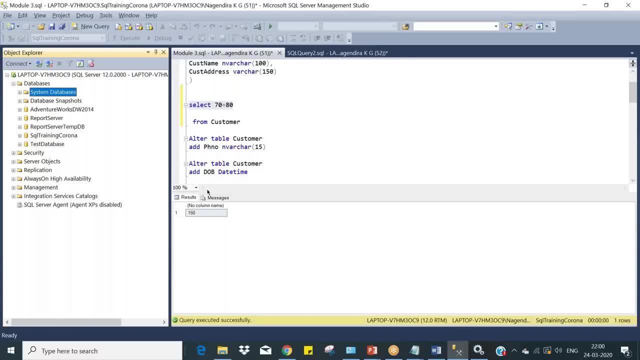 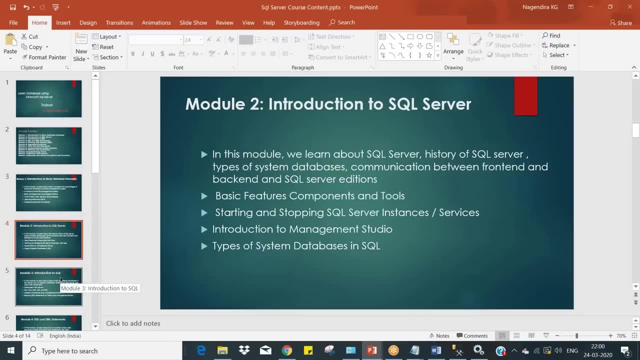 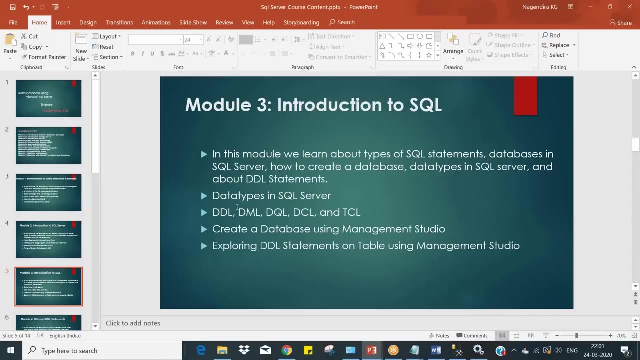 is the flow you should remember. okay, I think today I can stop, so these are the things I covered today. tomorrow I touch these things. data types, all those things we will look deep into. what is your data types? DDL, DML commands, when to use this one. create all other. 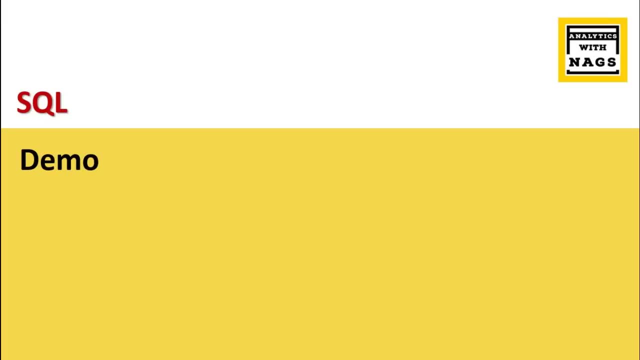 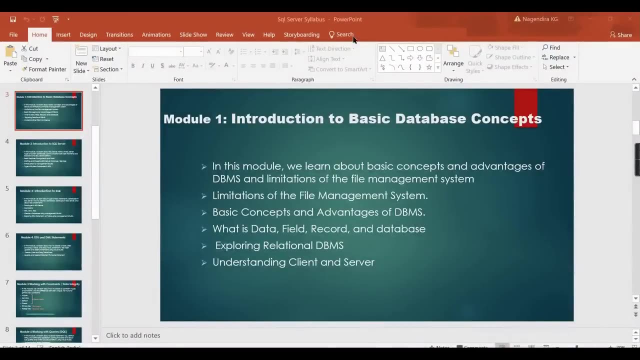 stuff. okay, so in our previous session we have seen, like what are the basic concepts of DBMS and why we need go for databases and i have introduced sql server. that is, sql server is one of the rdbms. and we have seen sql server management studio, how to create a database and all other basic things like what. 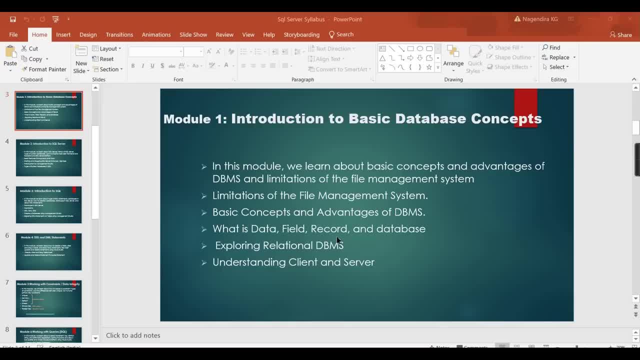 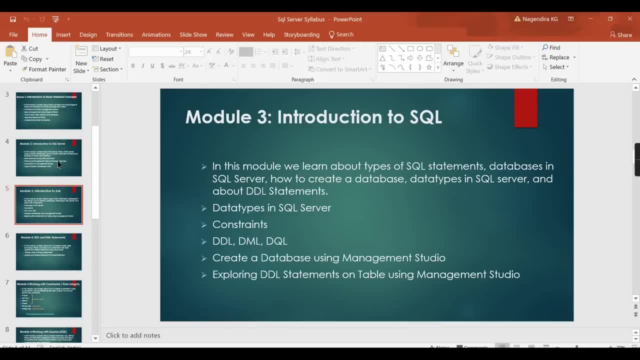 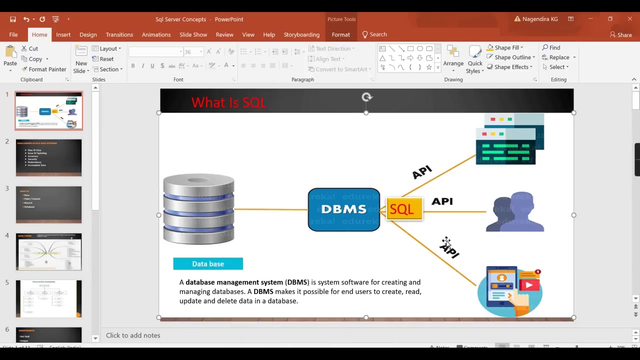 is the data field record and we have seen module 1 and module 2, and so in today's session we will see the sql basics. that is introduction to sql. let's see where this sql sits in this database world. so basically we know that dbms. 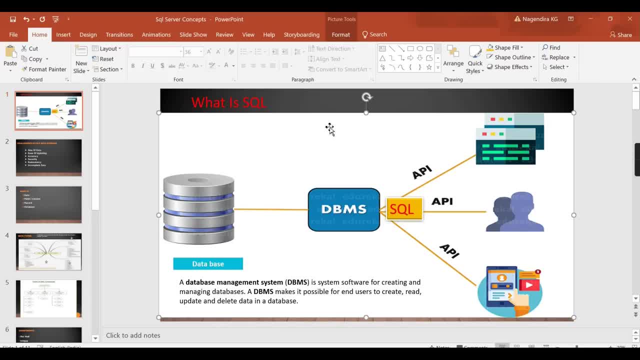 management system is a software and we need to install and we can access from the client systems. so this client systems- either it can be from application or from client sql server management studio or any apis should communicate to this dbms. so sql is nothing but a structured query. 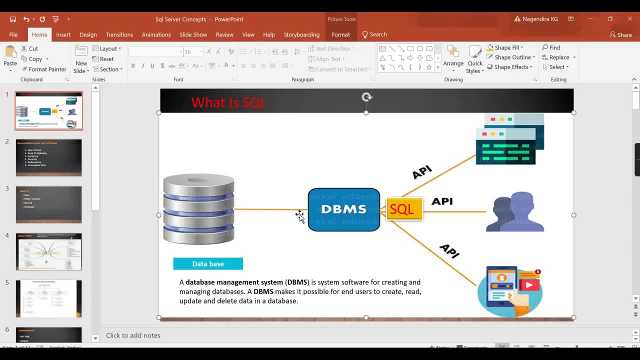 language that is used to communicate to the database. that is as simple as that. as it says the language, any language is used for communication. sql is a language to communicate to the database. this is the definition of your sql. so when you say it's a language, then sql consists of: 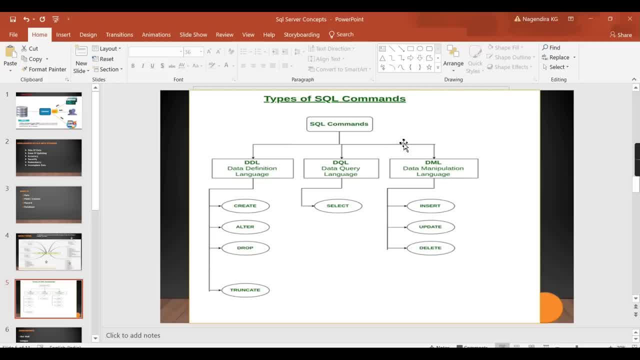 three kinds of commands, basically. uh, they categorize the sql statements, or some kind of query, into three main categories. there are other categories to kickstart your sql knowledge. i think this is fair enough. so what are the different types of statements? we have ddl, dql and dml statements. so what this will do assume the data definition language, which is nothing but. 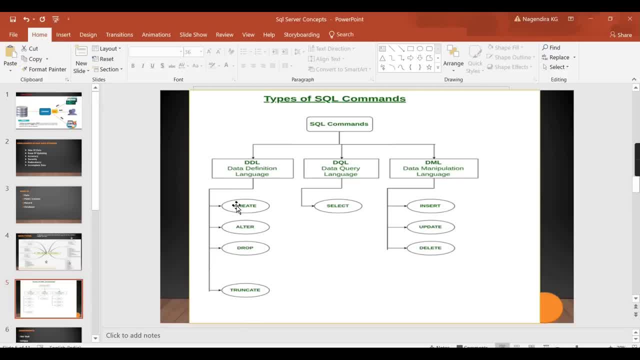 use it to create the structure of the objects. when i say objects, it can be a table, it can be a view, it can be a stored procedure, functions- those are considered as objects that are used to create the structure and modify the structure. that is your alter once you created a table. 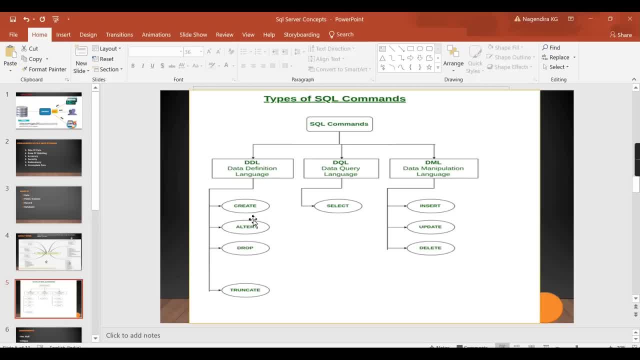 you want to include or exclude some columns. in that case you need to go for alter. you want to remove the table or drop the table from the database? then you need to use drop. so these are the different commands. truncate used to clear the records. commands use it to define the structure of the object. that is why it is called ddr statements. 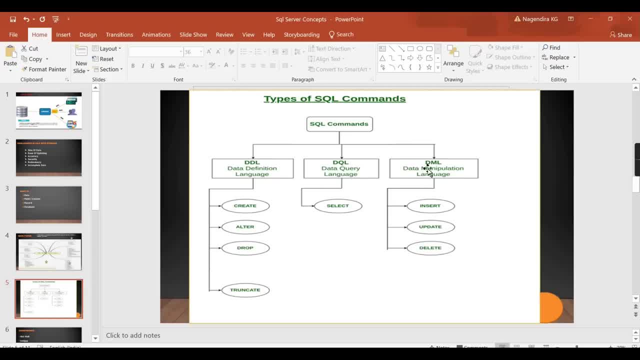 and then dql once you created. uh, this should come second, like data manipulation language. so, as soon as you create the objects, the data is not available. you need to insert the records into the created object or you need to add some content. okay, then you have to go for. 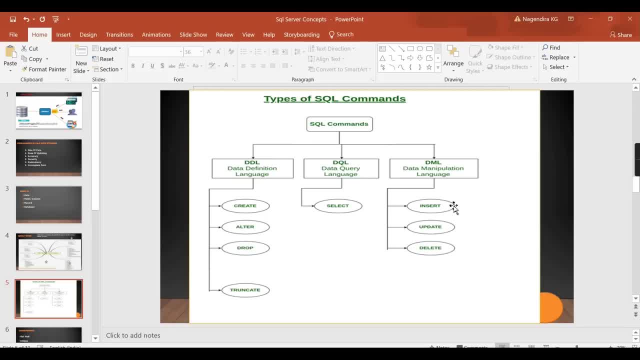 insert a record, i mean into, insert a data into your tables. that is what your data manipulation language. what are other operations you can do? once you integrated you, you find like you are adding some data to be modified, then you forgo for update, some data to be deleted, then 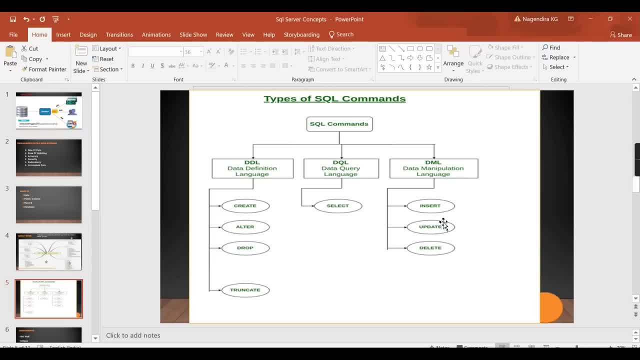 delete statement to be used? i will explain it with some examples. what are the different statements you can use? once you inserted, everything is done and you want to see the data that is you are querying. so most of the part you have to be familiar with select, so it is not a single statement. 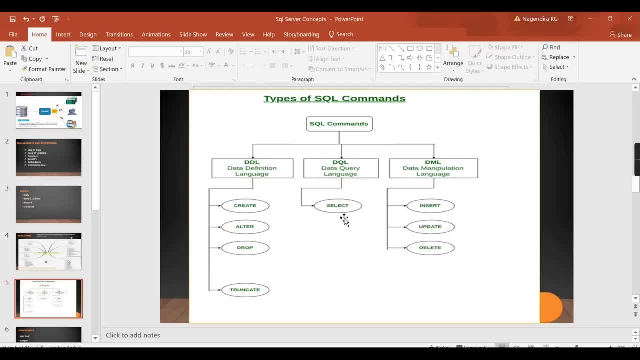 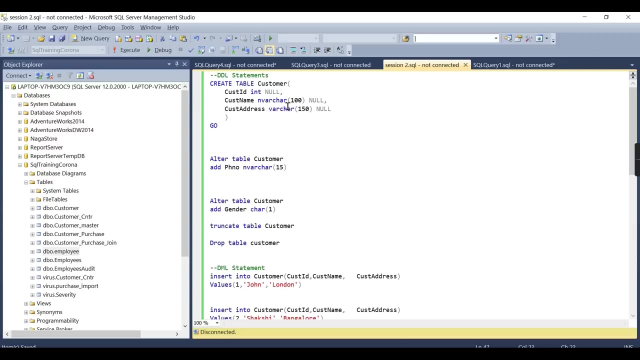 are a lot of other options in data coding, like grouping, var condition. everything will come here, but basically everything comes under a single statement called select. so these are fundamentals of your sql data definition, data manipulation, language, data query language. let us see by creating one table. then i just want to explain the some other concept called data types. then we 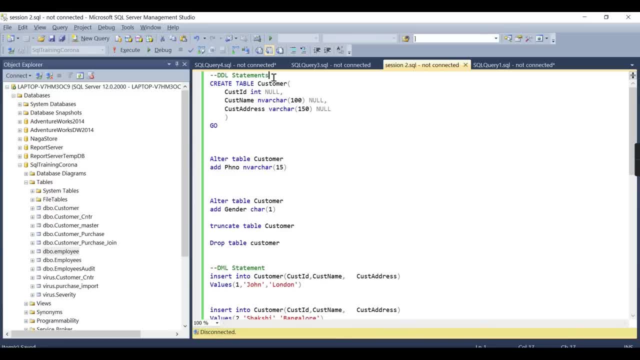 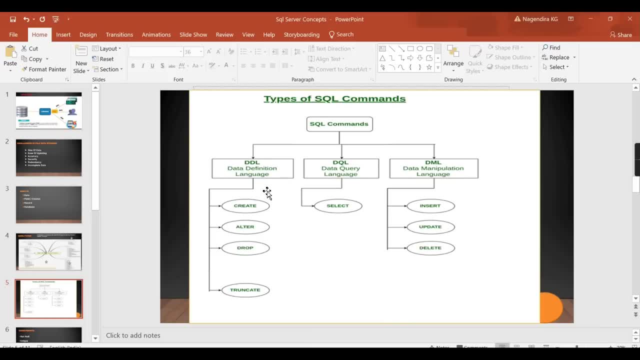 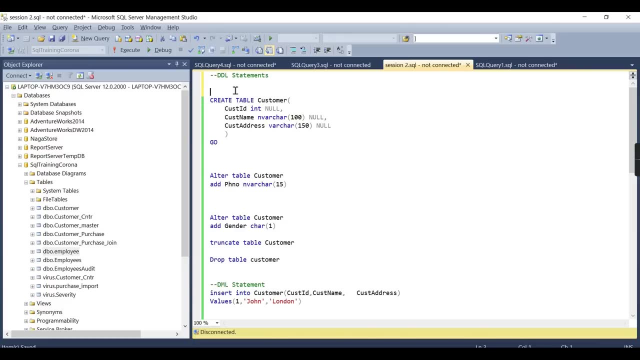 will go through all these statements one by one. so the first statement: i'm going to create the structure. okay, i'm going to instruct what this statement, this statement, i'm explaining. so what i'm saying here is i'm instructing the database management system from my client. that is this my 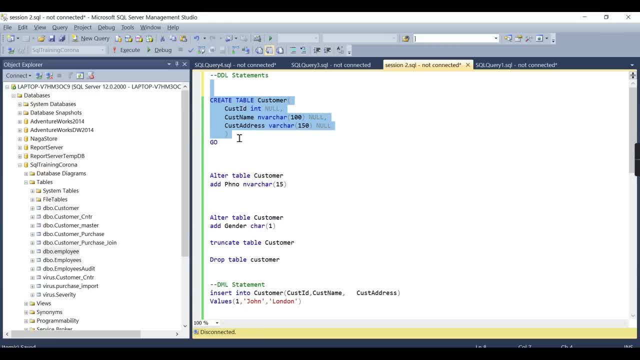 management studio is my client. from the client system, i am instructing the dbms create the table. so it has to understand right? this is the syntax. okay, the any language has some syntax and programming language, i mean. so this is the syntax to create your table, which says like: create: 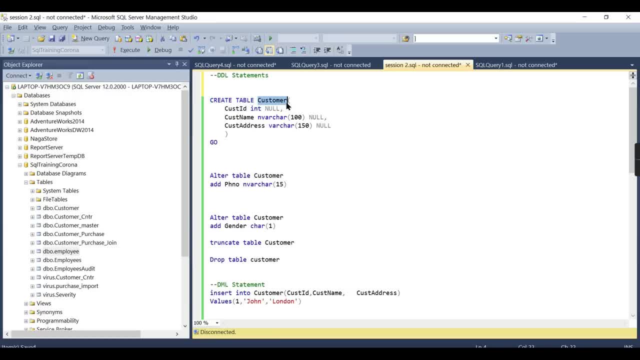 a table and your name. you can give any name. uh, they have certain rules to give a name. you cannot have a space here, so some rules are there, okay, so you need to follow those rules and you need to provide the column name followed by the data type. then this is the constraint: whether it's a 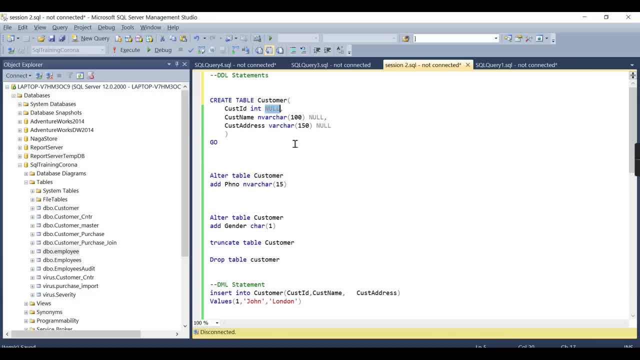 null, not null, all those things. i will cover it later in later modules. so to understand it, this is the syntax: create table- table name, followed by column name and data type. this is the second column name and its data type. this is the third column name and its data type. okay, so once. 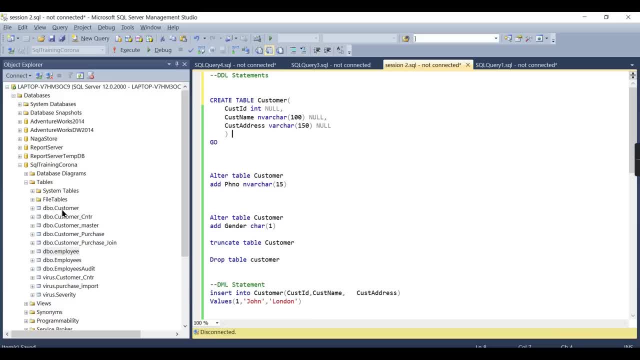 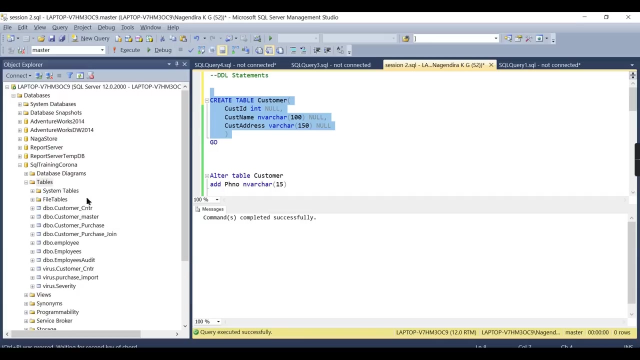 you do this. okay, now you can see, already have this table. so let me drop this table, delete it. so i do not have this table right now. okay, the customer. so when i say execute, select the statement and click on execute, let me connect it. command completed successfully, so now you can go here in your database. xql training corona. 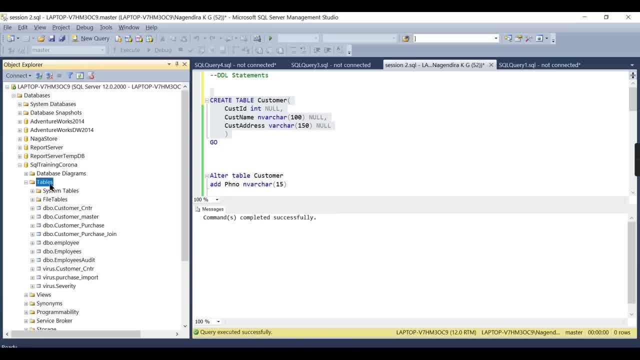 and refresh it. so as soon as you do that, okay, sorry, see, there is a issue here. i i didn't created in the sql training corona database, so you need to choose it first. you choose this database and execute it. that is created in the master. we need to delete it. i can drop it later. 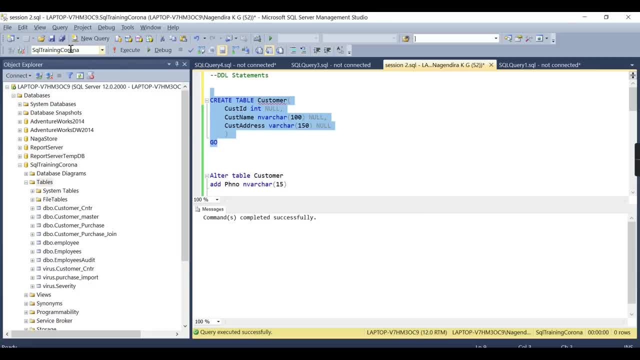 now i created in this database instead of this. okay, you can use some class like use. use. if i want to create this table in naga store, okay, okay, when i use this one, it will automatically change it to naga store. so, first statement you need to use: uh, that is, use the database name. that is the best practice. 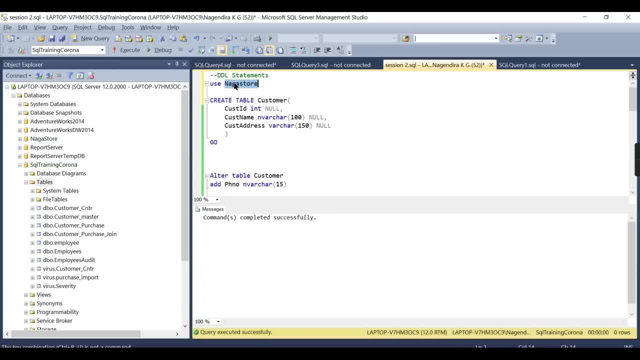 let me change it to sql training corona. here also: sql training corona. let us keep like that. so by mistake it will not uh. you will not uh create in a wrong database. so this is fine. now, once you see and refresh it, you can see that apple created and. 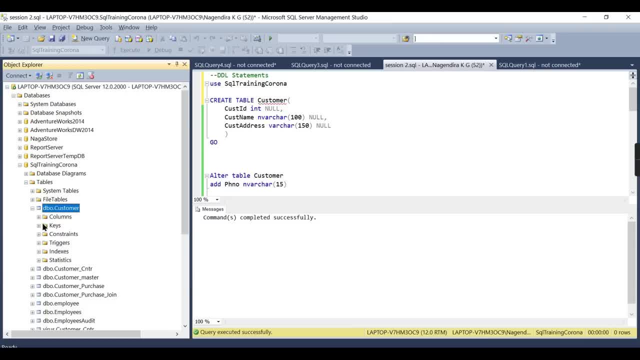 soon as you create it. okay, there won't be any data available. you see what are the things it has created. you mentioned only this. now you can see what are the columns available are created in this table then. is there any constraints, triggers or keys? you have created all those things will. 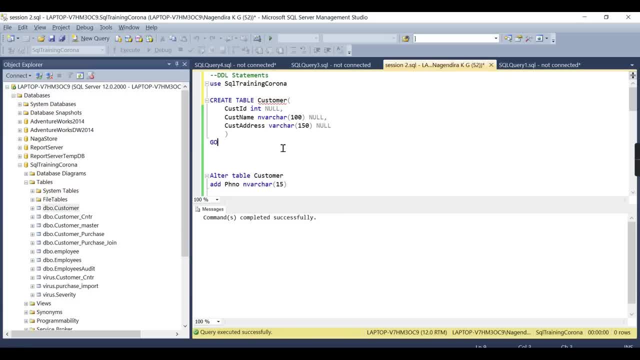 automatically fall under this table. so, uh, let us stop this. uh, i mean break for some time for creating this table. or ddl and dml statements- what are different? sql statement? i want to cover important topic like this- integer and nvac, or what is this data type is all about? so i quickly try to insert: 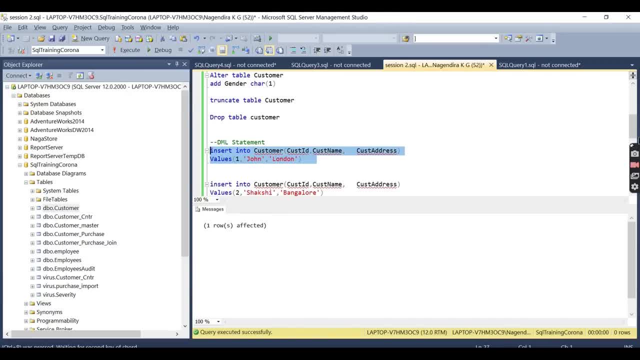 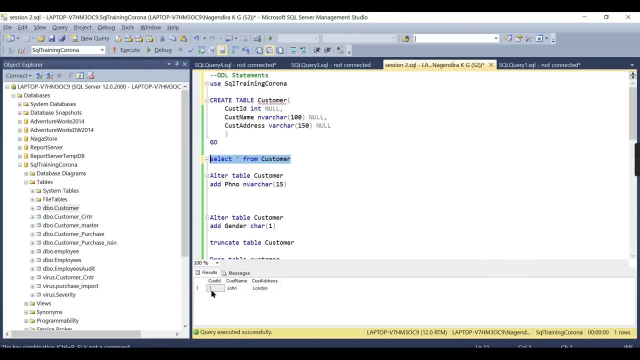 one record. so this is how you need to insert a record, and i can see the record here: select star from the customer. okay, now you see, here you have your customer id, customer name, customer address, right? so in this you have something like integer and nvac. what are these? these are nothing but your. 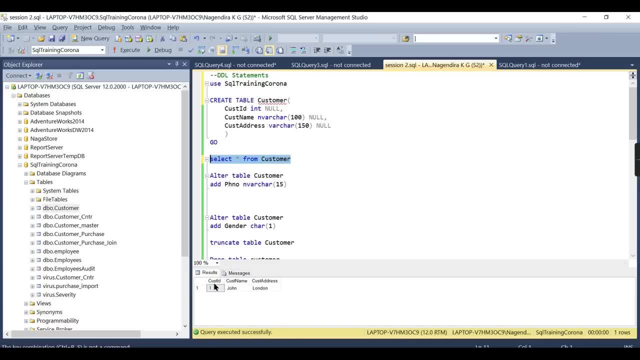 data types, which defines what data this column should hold, whether this column- customer id- is an integer or text columns or any other binary or numerical column. so those kind of what is the type of data you are going to store? that is your data type. that is what you need to mention it here. 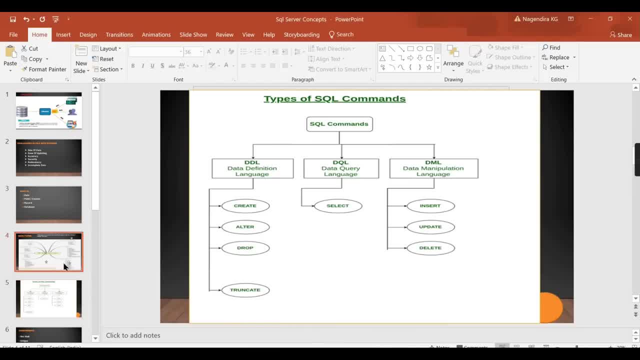 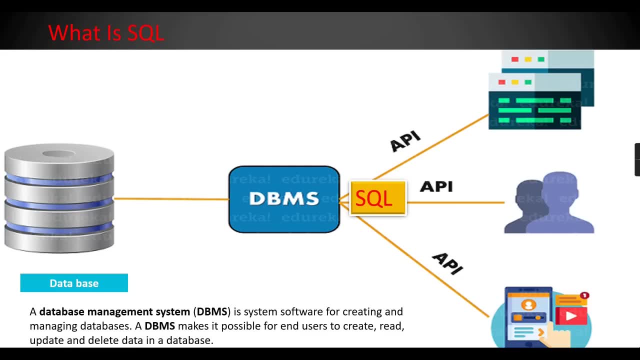 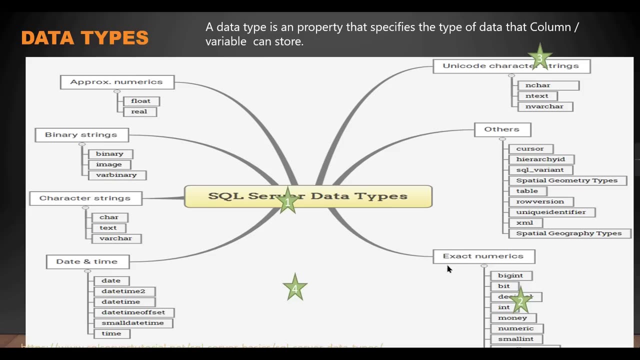 so what are different types of data types available? let us see it here. let us see it here. it is very small, let me put it in back screen. so now you see like basically most of the time, exact number numeric. you see here, the first preference is like here: 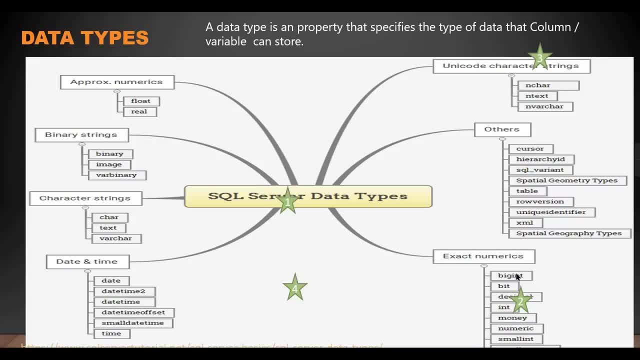 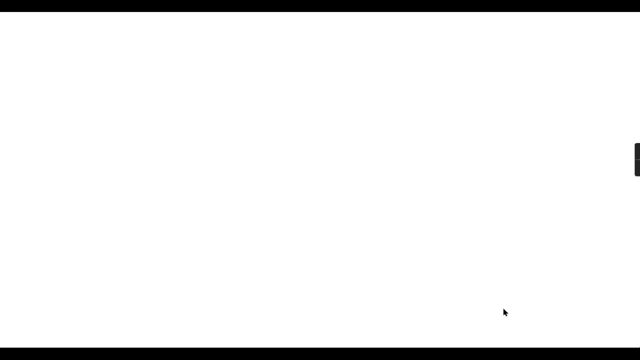 the big, int, integer, numeric small and all these things are used to store the numerical values. uh, there is a limit for each and every data type. i have given the link over here. i will share it in the description so you can watch that one. so each data type has the limit if you want to store. 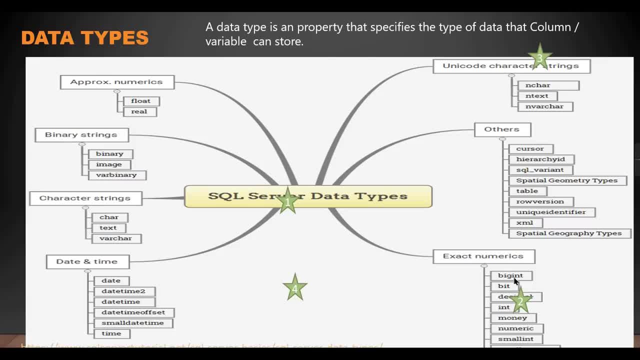 big numbers- okay, it's more than a trillion or some big numbers- you cannot store it in integer, and if it is something between 0 to 128 numbers, you can use the small int instead of using the integer. so, based on your type of data, as well as the volume, how much? 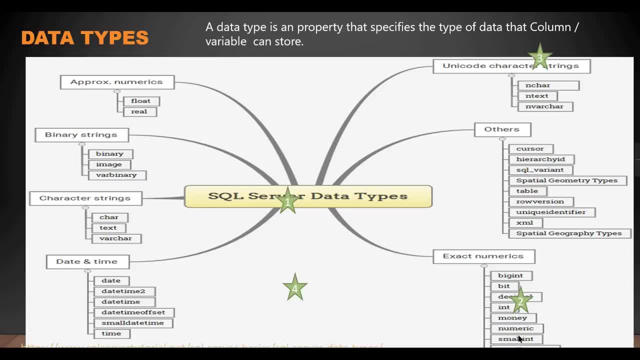 data it is going to store the limit- okay, minimum and maximum limit. you can choose appropriate data types. so if it is like strings, that is text. there are three varieties. i mean three types: character text, worker. and in worker is a new data type that needs to be added. 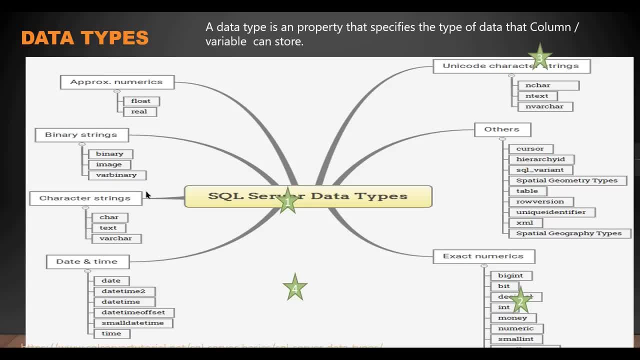 then last is: i mean there are other kind of data. like you have a date time here. if your column going to store the date related uh data, then you can use uh date date time to small date time, our time. so, based on what, what kind of data you're going to store? so each uh, what is the difference? 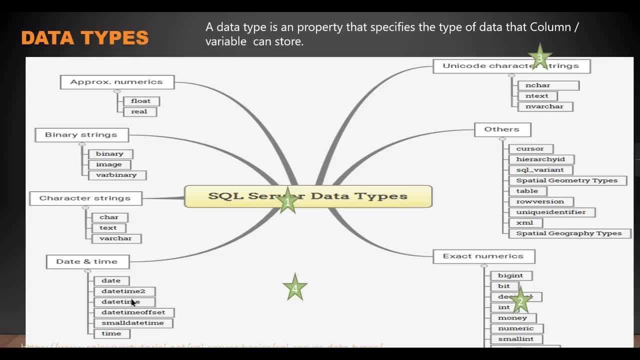 between date, date time and date time two, we can uh check it later. i mean, uh, basically, uh, this will have only the date, this will have a date time and this will have date time with some utc kind of them. so, based on your business scenario also, you need to choose appropriate data types for the columns. 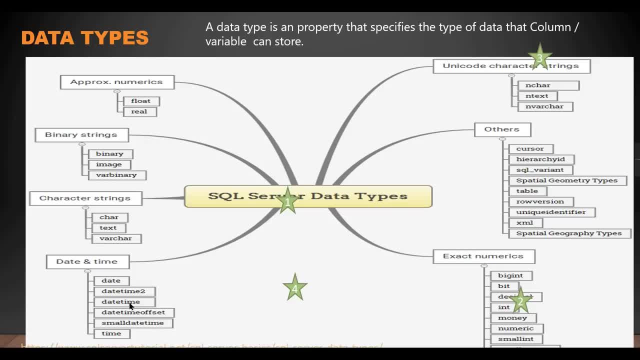 so mostly we will use integer and in worker and date time and there are certain things like: uh, you have um boolean values, right, whether it is true or false. you have kind of binary zero and ones, so those thing you can show it as a binary. then you have: uh, it's not. 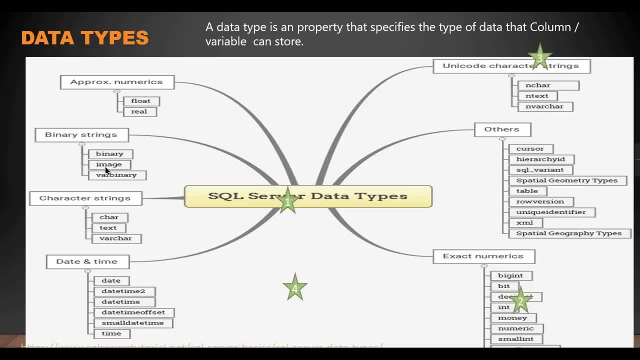 a binary- i think this is for uh var binary and images for uh big numbers. i mean you can store an image in this data type. if i mean sql server can store the images in in a column. so image how images will be stored using this data type. when you store it in var binary you can retrieve it. 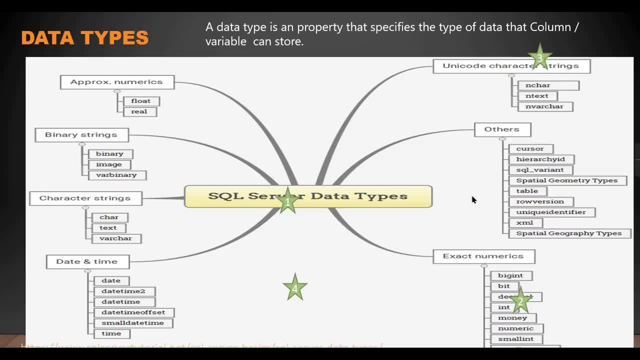 okay, that is what. so there are some special data types also there xml spatial geography types. so these are some special character, i mean data types that you can use. uh, here you see the character string worker and you see the unicode character string in worker. so what that differs. 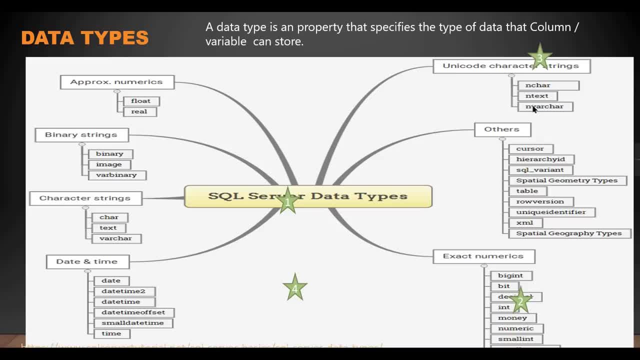 from car and n. car n stands for unicode and which is basically nothing but uh. unicode characters are multilingual. like these will store only the ascii characters or only alphabetical characters in only english language you can say and, whereas the unicode characters will support the other languages, like um chinese language or arabic language values, if you want to store so. 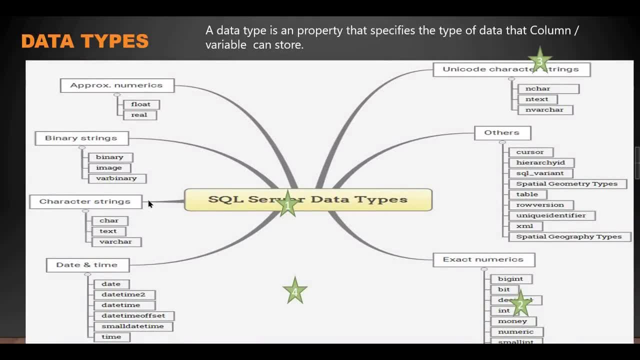 the purpose of these data types is to enforce certain rule, like if you define um a type of a column like a date of path as integer and you cannot store the uh- your date of birth- in that field, so you can't store your data in that field. so you can't store your data in that field. so 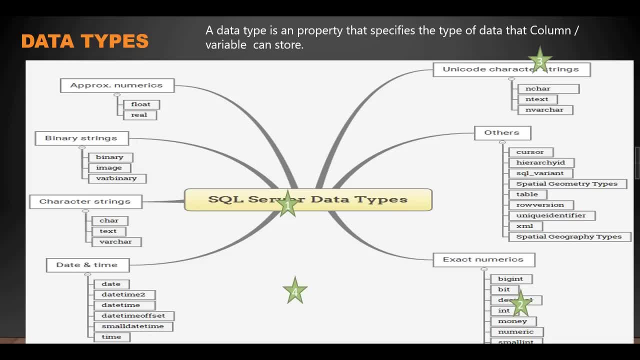 it's type of some kind of checks you are doing and to enforce, because, uh, another main important aspect of having a proper data type is like, uh, certain functions you will call to say, for example, you want to get the first four characters of a string. okay, then some string functions will work. 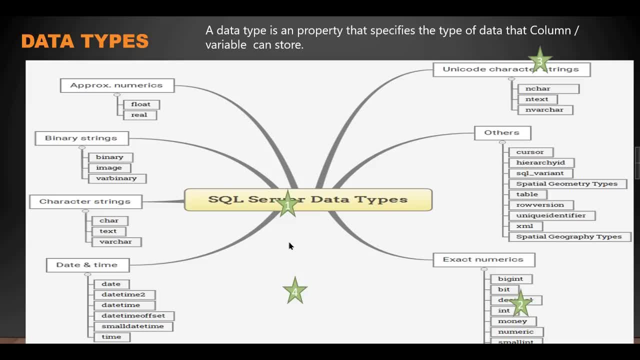 only based on this data type. whatever you define, these are the main purpose. you need to define a proper data type. so another example i can give is: like you want to add five days from our subrack, five days from the current date. uh, i mean to say 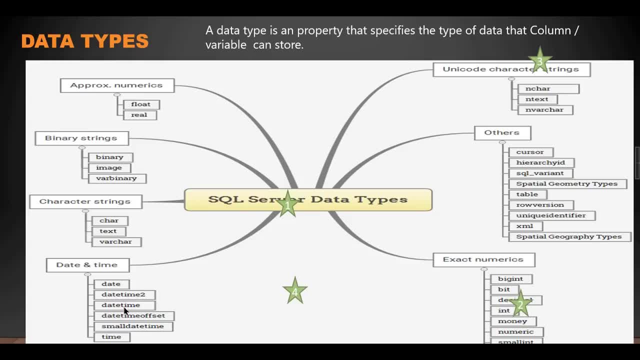 from the date in that column, then in that case you have to use the date add function that takes the one of the parameters: date column, date field, date data type. so if you are not defining your data type properly, then some of the functions won't work. so with this note i have explained. 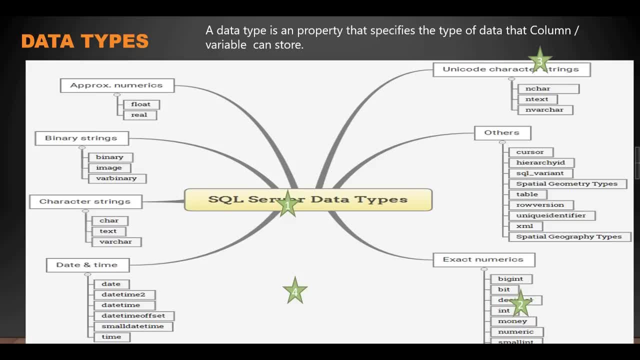 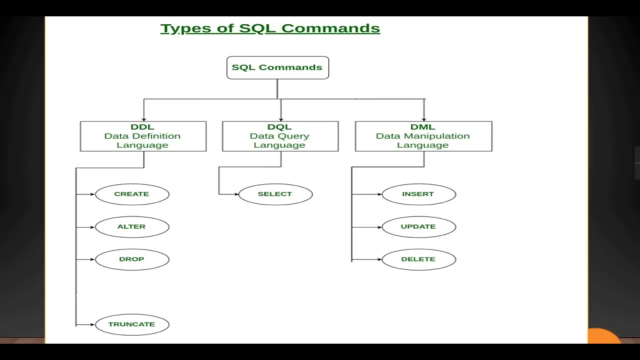 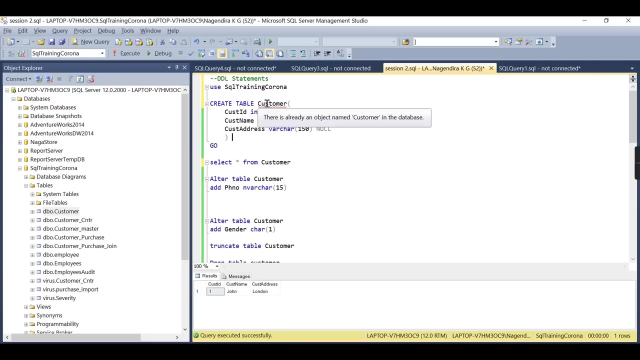 the purpose of data, data types. uh, how important it is to make your database proper design. moving on to the sql statements, once again let me start creating it. so this is the create table that we have already created and added one record into it. so now we have defined uh, integer and worker and worker. so i have mentioned. 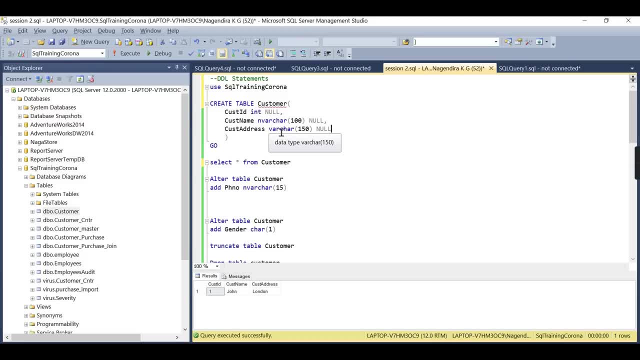 both here in worker and worker. so now, if we insert some other characters other than english characters or ascii characters, this will not support, whereas this in care will support your uh, chinese characters or your arabic or other other than english language. that is where unicode stands, for there are mainly other differences as well, but understanding i am. 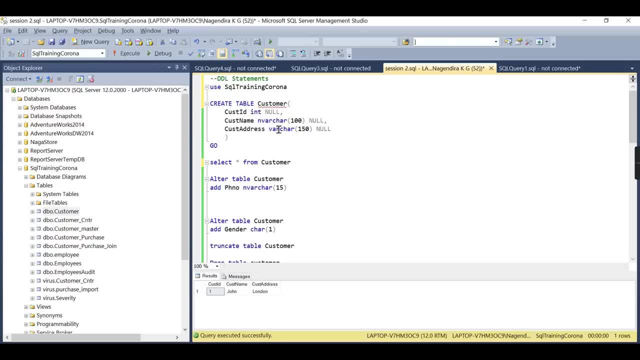 mentioning it to you, there are some storage, uh reasons as well. i mean, that is storage wise, it is optimal. that is unicode character. for, to begin with, just try to understand. there is two difference. I mean difference between worker and it and worker. so I have inserted a record. I 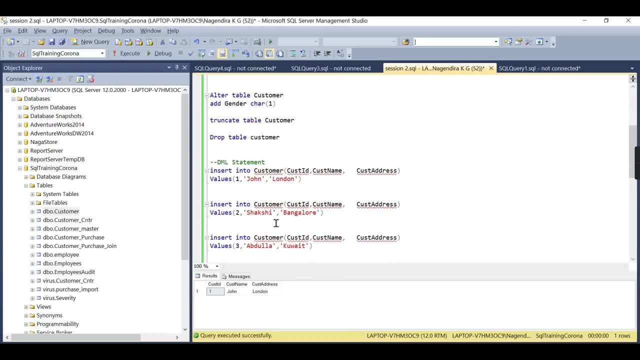 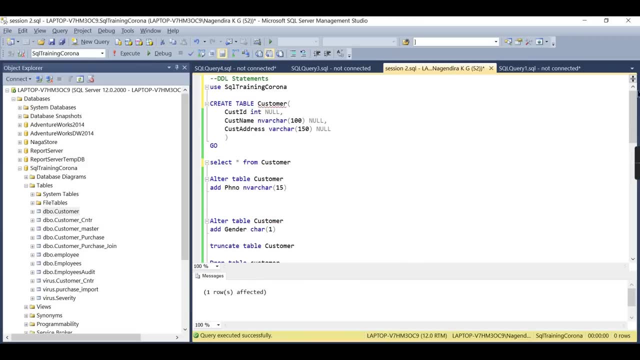 want to insert a few more records, that is two records here. okay, to Shakti Bangalore and let us try to query it. okay, now you can see here customer ID, customer name, customer address, everything was there. and then what happens when I try to change, you know. 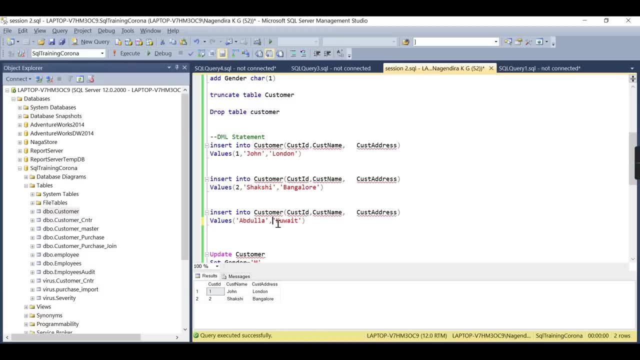 what's happening? I will try to insert it in improper adder, like I mentioned, customer ID here, which is integer column, but I am trying to insert a character value here and this is the character. okay, I mean, that is a string and this is a grain a string. okay, what happens if I do like this? yes, it. 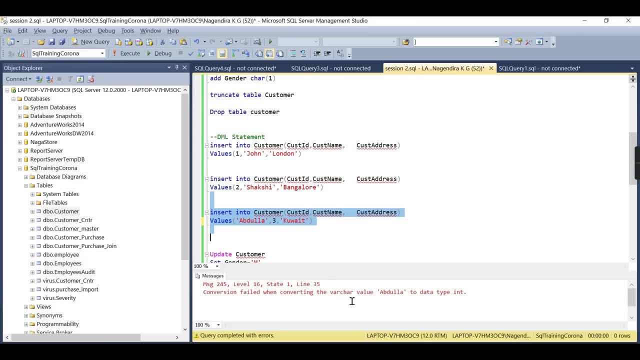 throwed a error. conversion failed when converting a worker value, Abdullah, to data type integer. it is trying to convert this value to integer because customer ID- whatever you defined here- is integer right, so you cannot insert character value in the integer field. so it's it's a kind of one check. 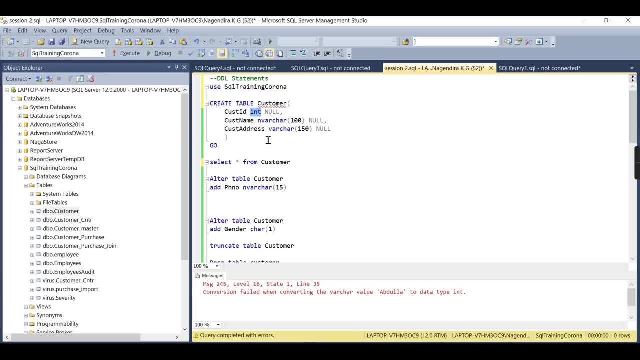 you can't insert a character value in the integer field, so it's it's a kind of one check that it is imposing. these kind of checks that you cannot impose in file system, right? if you in Excel, if you are having one value- 1, 2, 3- then again you cannot. you. 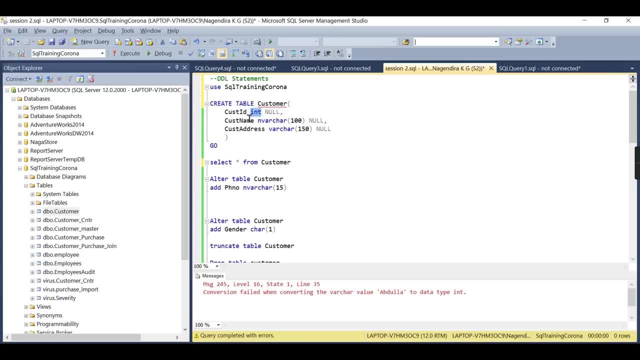 cannot impose much. okay, that that is what the people can start typing, the name or whatever they want. so I am NOT. I'm not saying only in Excel the file systems. they maintain notepad or other files. so this is one of the disadvantages in file system that. 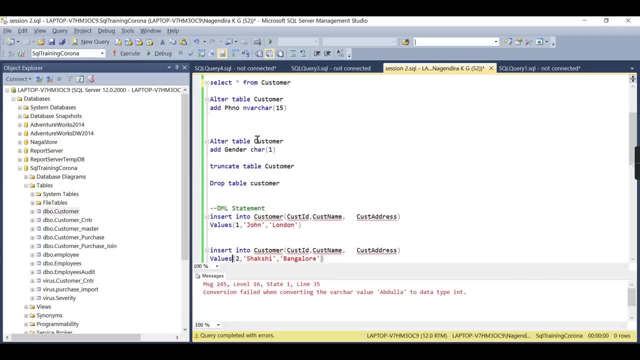 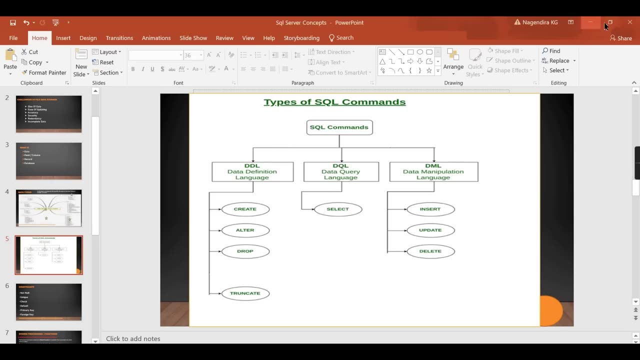 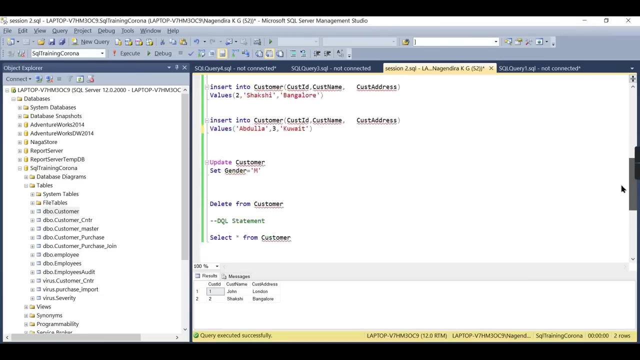 will be overcome by database. this is a classic example why we need to go for databases as well. so the next statement is like in the DDL is to alter: now you see, here we have two records. let me insert the third record now by replacing it with proper order. 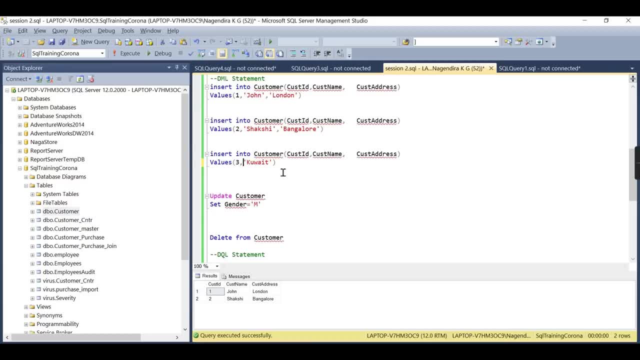 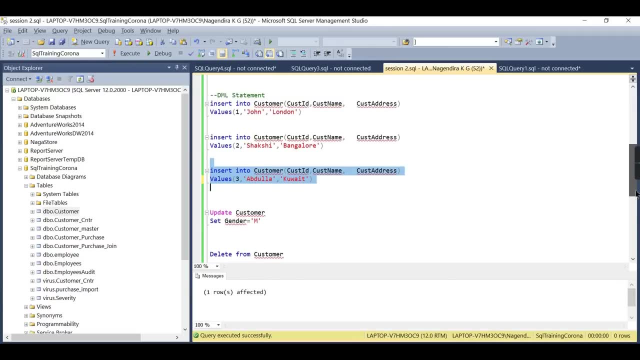 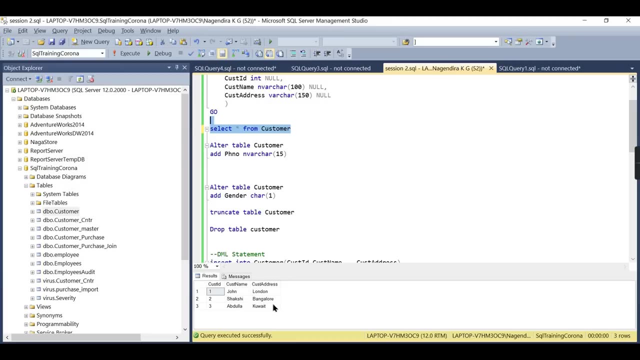 okay, yes, so I'm inserting the third record. there you go, let us see this: one, two, three: John, London, shakshi and Abdullah, and now, after I insert, and now I want to add a new column called a phone number and a gender. okay, so how to? 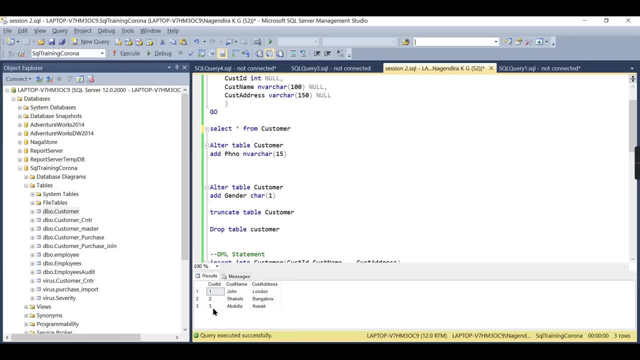 add a new column called a phone number and a gender? okay, so how to add a new column called a phone number and a gender? okay, so how to do that? it is like altering the structure of the table that is object. the customer table is object. you are trying to alter the structure, correct? so 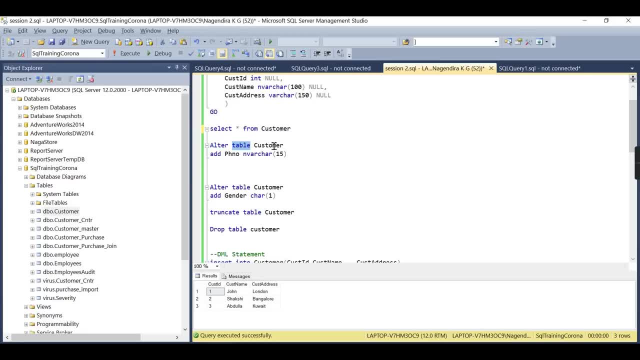 for that you need to use: alter table, the table name, that object name, then add the column, whatever the new column you are specifying, then the data type. okay, so this is the way to alter your structure of the object. for that, just execute this. now you go and see. so whatever changes you, 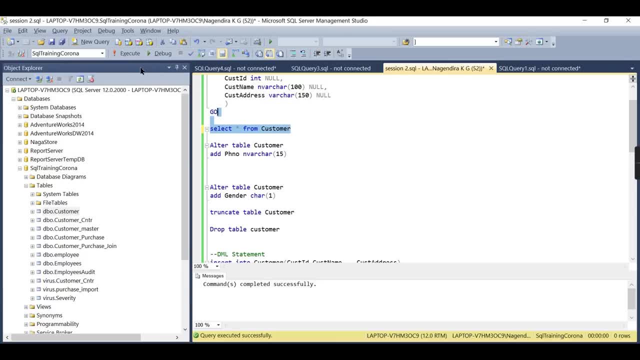 do. in order to see the result, you need to use select star from customer. that is your tqr now, as soon as you add it, it doesn't. we didn't say anything about the data. we are just adding a new column to this table. that is what this altred. 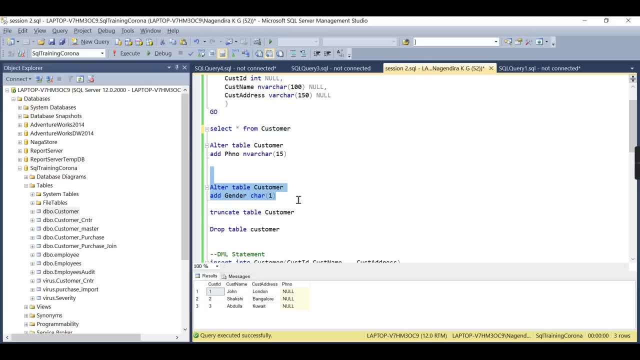 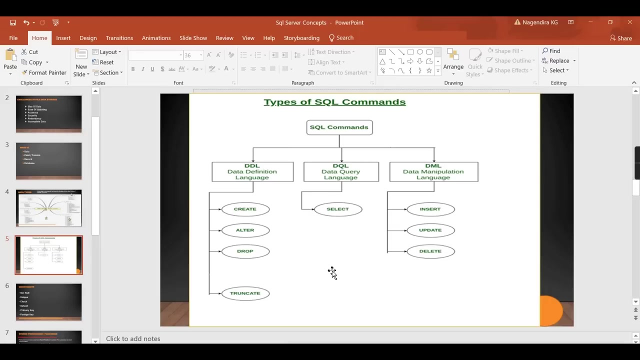 table will do similarly. I want to add another column called gender, which is character one. let me correct: now there are two blank columns. fine, let us keep these two later. okay, drop and truncate. let me go to another important dml statement. now we have seen create and alter. then we have inserted the record using the insert statement. 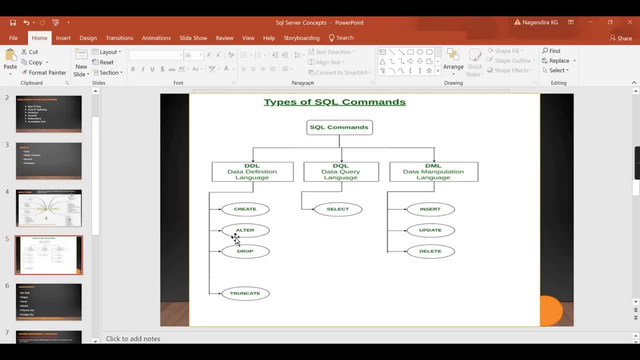 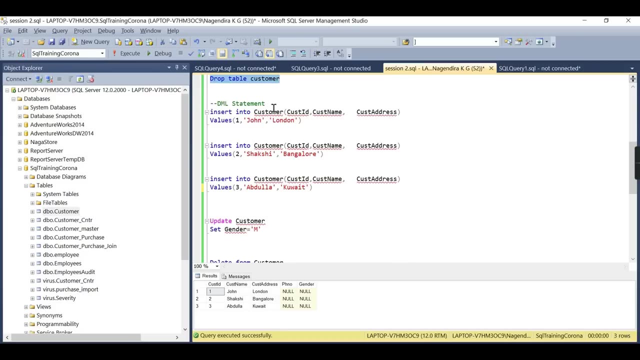 now. i want to alter the structure means you go for alter. i want to modify the data means you need to go for update. update is for modifying the data. okay, so the another important statement here is update. customer set m. so what will be? the result of this query is like: irrespective of your gender, you are. 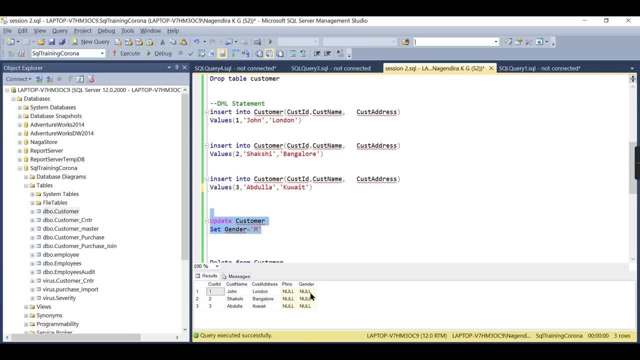 not seeing anything over here. just update m for all zeros. okay, that is what it is saying. let us try to update it. let us keep it like this. then you see the result. now, once again, you see here, one, two. everyone got the gender as m. let us have it like that. 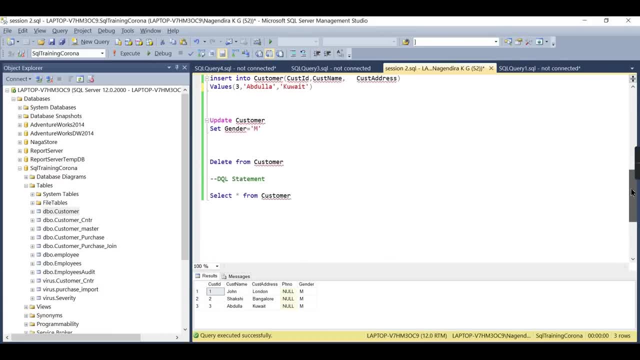 then what happens? i want to update the phone number. let us keep the phone number as well as such. we will do it later. now you understand the concept of update. if you want to modify the record, then you need to use the update statement. i am not modifying the existing record, i am just modifying. 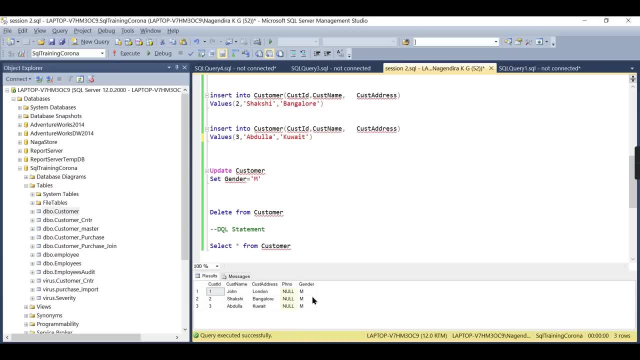 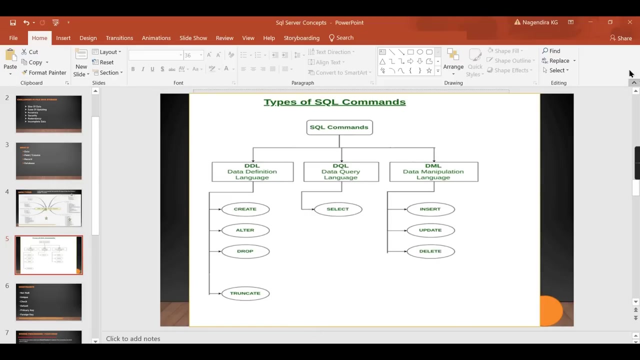 the existing column value. there is no value. i have added new value here. okay, so if you want to change for this particular london, i will do it later by using a var condition. we need to do it before that. so i want to show you the last dml statement here. delete. so when i want to clear this. 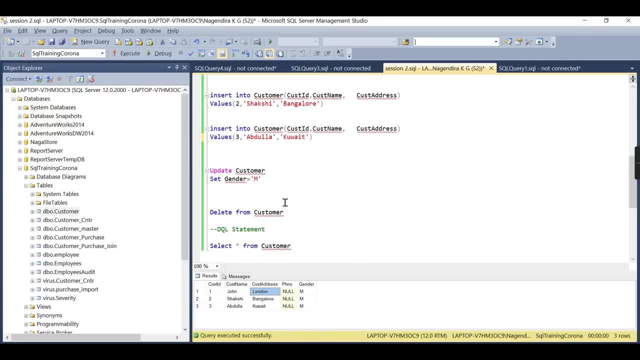 record. okay, everything. i want to clear it what i need to do. you need to use a delete from customer, that's it. now you go and select this table. now there is no record. okay, so these are different statements you need to understand to work in your databases. okay, so first to begin with create, then you not to alter. you need to 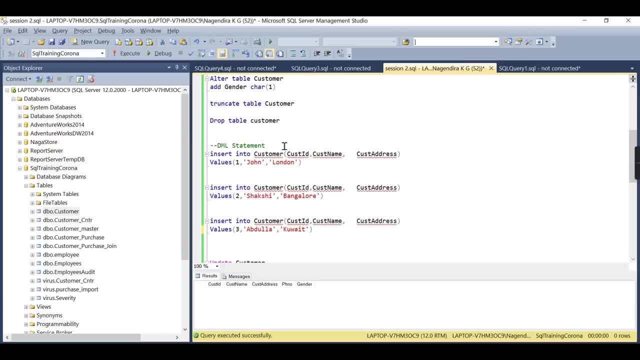 alter it, then in order to insert the record, you need to use insert statement. if any record or data to be updated, you need to use update. then, removing the record from your table, you need to go for delete. this is the core, key concepts. then what about these two truncate table and? 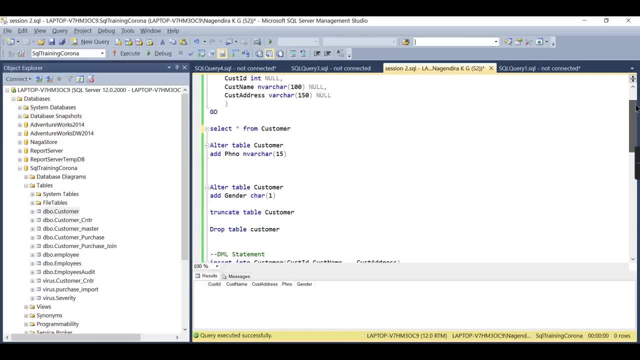 uh, your um delete table. so these are one of the important um interview questions. let me put the data once again into this table so that you will understand. so now you have us three more records again. as i deleted the record now, i do not enter the gender now, so again it will be blank now. 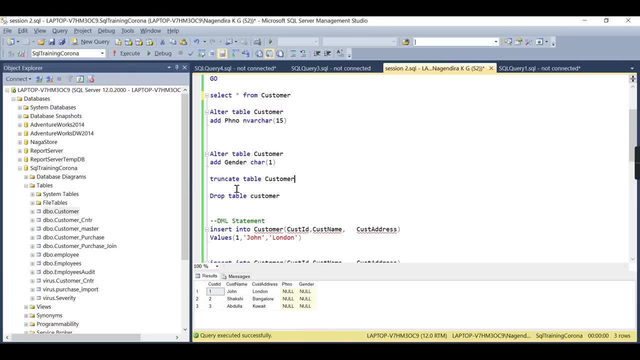 what is this truncate table is doing? it will also clear all the records from your table, but, uh, some indexes. if the table contains that, will also to be reset. okay, the identity column will also be reset. there is some few difference between delete and truncate. where delete the key difference between delete and 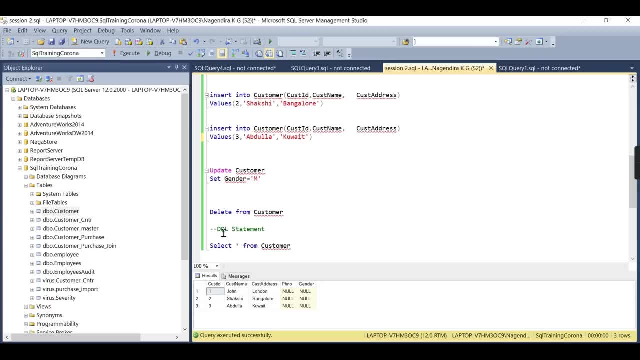 truncate one of the important differences. in delete statement you can use a var condition. what is var condition? to view the records, you are using a select star from condition customer right. i want to see only this customer id 2 for that. in order to filter it, you use a var. 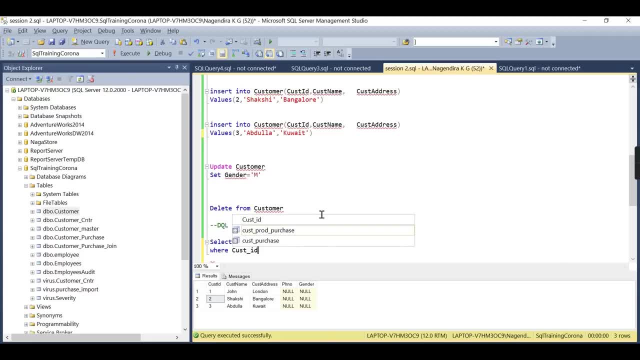 customer id. customer and id equal to 2. so i want to see only the customized 2. so let me hold on a minute. there is no underscore, it's only uh custody, so i i can see only the customer id 2. when you use select star from table name, it will display all the records in your table. 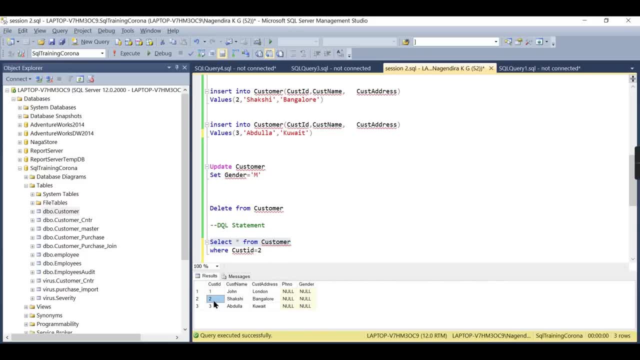 i want to specify or filter out certain records, then you can use a var condition where customer id equal to 2 will give me only this record. so similarly, in order to delete only customer 2, i can use a var condition here where customer id equal to 2.. so this will delete only sakshi. 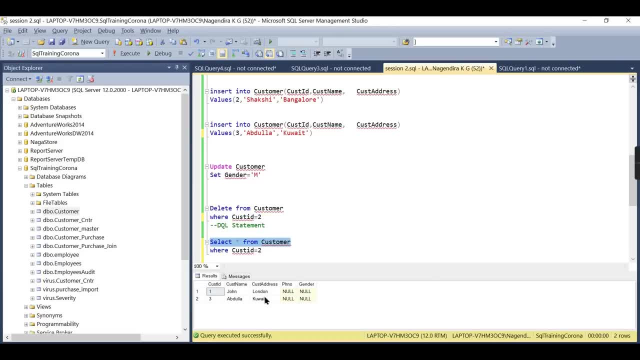 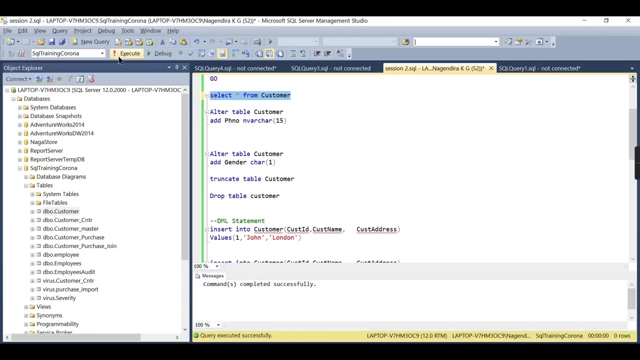 now you can see in your customer table you will have only the two records over here. this is the key difference. but whereas the truncate, there is no var condition. whatever records you have, even it contains one million records- it will clear it very fast. that is the main difference between delete and truncate. now you there won't be any data in your customer table. 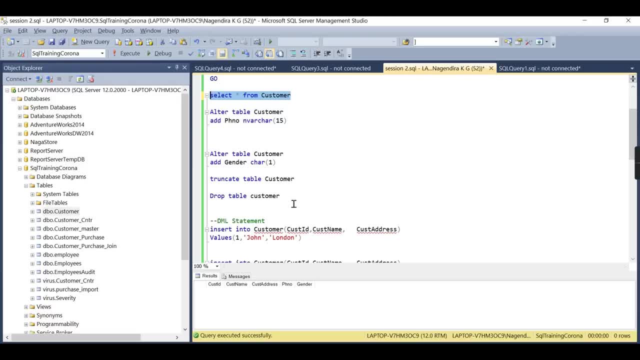 and there are some key differences as well. and what is the drop table will do so. drop table is nothing but will remove. this will delete the table itself. see, uh, delete is deleting the data. okay, what drop will do is drop will delete the table from the database. there won't be any table anymore, okay. 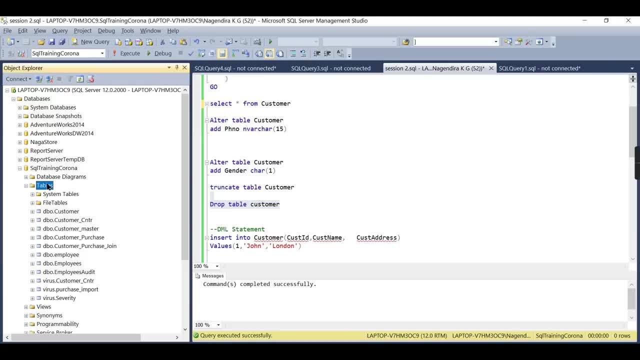 drop table table name. now, if you see customer here, when i go to click on tables and refresh, customer table is gone. there is no more. now, even you create it won't be available. invalid object name: the object itself dropped. that is what your drop will do. i hope it was clear like what is. 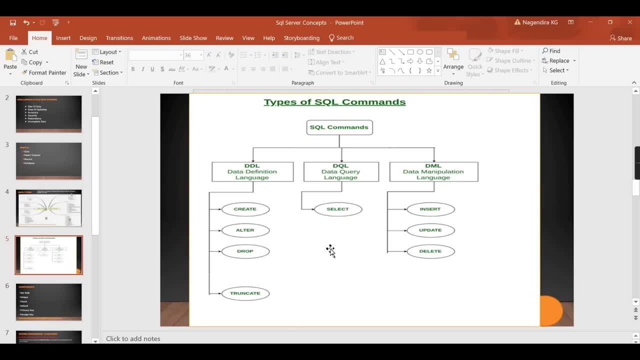 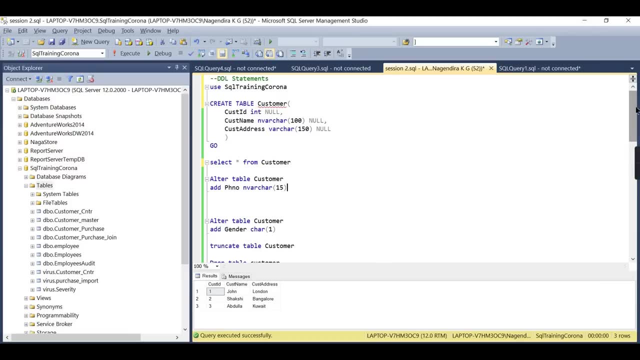 sql. what are different sql statements? uh, to manipulate and what is its purpose as well. let me uh walk you through certain um other um examples, as i mentioned before, like we have seen, if insert wrong values like abdullah and um in three and four, then i mean. 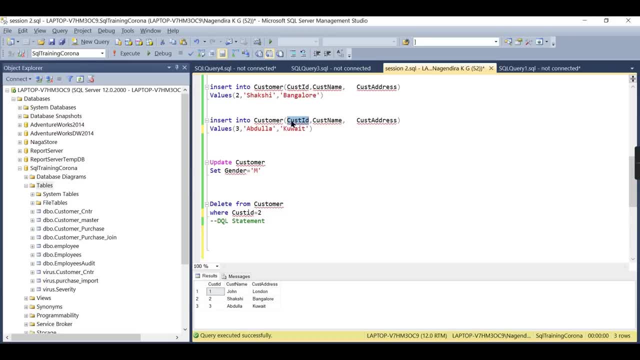 to say, in the customer id is integer, i need to insert an integer. and what happens if i'm not mentioning the column order like this: will it insert? yes, it will actually the column order. if you are not mentioning the column, however, you have created it. you see here the this order, you. 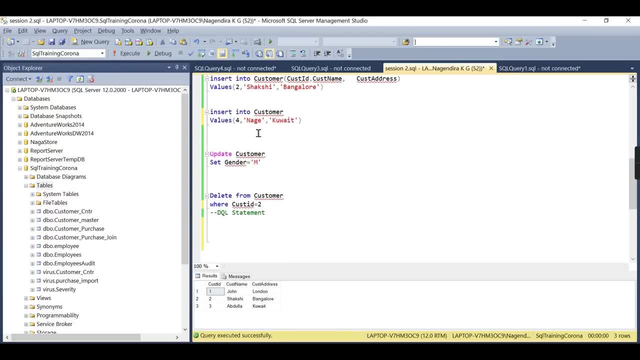 have created it, that in that order this will get inserted. insert into- now i am saying naga and uh, i'm in- say for example, jubai, let me insert now. okay, let us select this. select star from customer. okay, now, i didn't mention any order, but still i can insert a value. and what happens? by mistake? 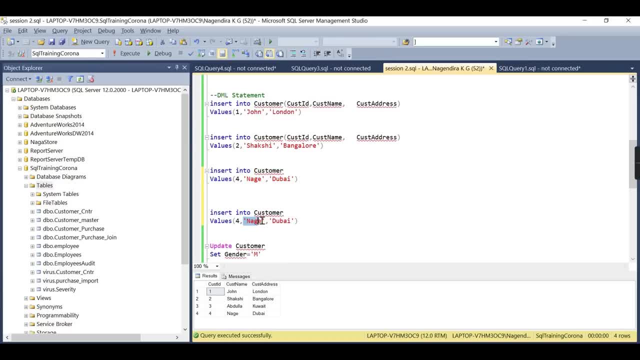 user inserts a data like this, dubai, and he says: is mr kumar, kumar kumar is not here. fine, what happens? let us see. okay, so now i have mentioned, i will just move it a little up. okay, now you see here, this is a statement i have executed. insert a customer, phi and dubai. now what happened here? so the 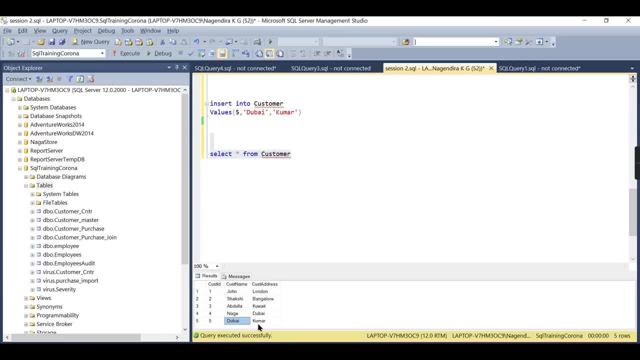 number is of eight, Ü3 is one of NUM or our object block, but the value as susbcribe: kumar. this is a very common cross ated addressing function. so the custom address has also to buy, but inserted in the customer name column, whereas the customer name kumar is inserted in the customer address column. this is because the order you are not mentioned here. okay, you see here in one of the example, customer id, customer name address and this order should be the same and in order to do a proper insertion of into particular column like this, okay, you can mention the value. so this prayer it is you, as i can say, add a cash number to the customer. 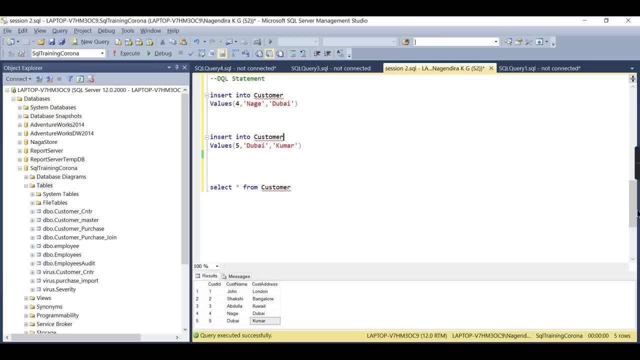 in different order, but what you need to do is you need to mention it in this insert statement as well, as we do not mention it in this example. it is inserted in the created column as well, in this order it has inserted. now, in order to work this one, I'm again inserting this record, but what I'm doing 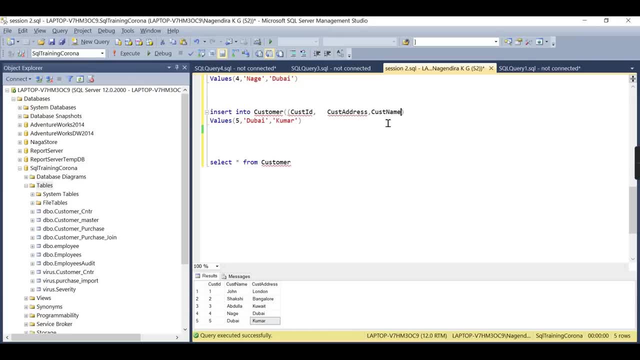 it here. customer address- customer name. so insert into customers customer ID, customer address and customer name. here layer. we used to give customer name and customer address, so this is the proper order now in order to give different order you, because once you create a table, you don't know which order you. 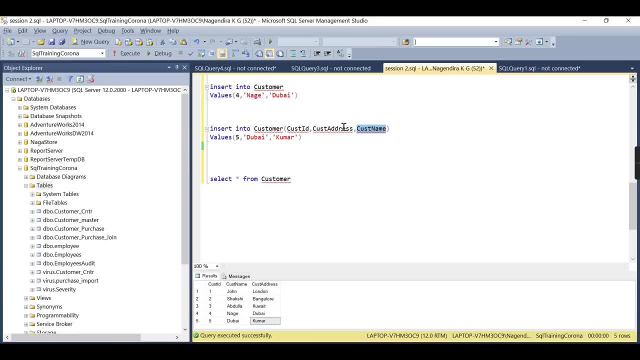 have given. so you just pick up the column names here and, based on the column names provided in the insert statement columns, you can mention the values. so now, once you insert the same record, let me put it for six. okay, again, I am putting for Kumar. so what happened now? 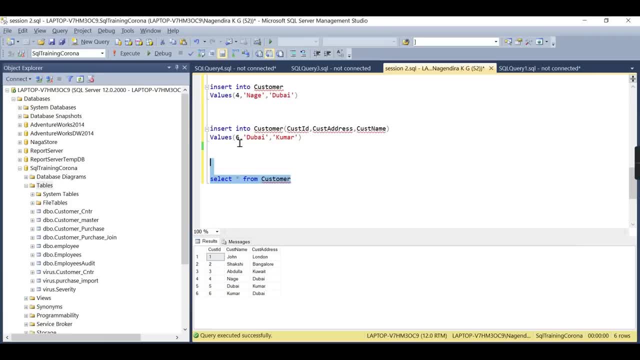 yes, so now, even though I mentioned, like six, Dubai and Kumar, the Dubai value is inserted into customer address properly, you see, for six, right? so this is how the some of the basic things you want to understand and, synthetically, this is syntax and you need to follow it, and how. 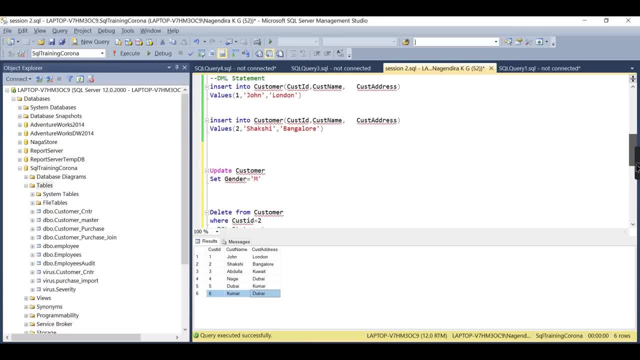 about your one of the update statement I mentioned, like select star, from where condition? we have seen similarly even in update statement we can use a variable condition. now let me add gender again. you will see, always once you do some statement changes you just try to select, start from. I mean select the data and 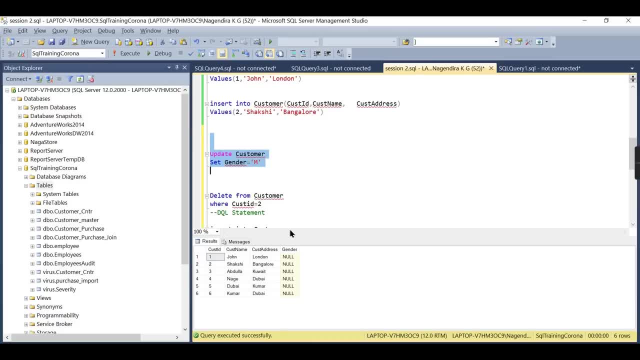 see, once you do this one, what happens is like it will update M for every, every individual. I hope for Sakshi. we need to update it as female, right, so what? the one of the simple thing I can do is where I will say: customer ID okay, customer ID equal to two. I want it as Jeff. okay, I want to put it as Jeff. 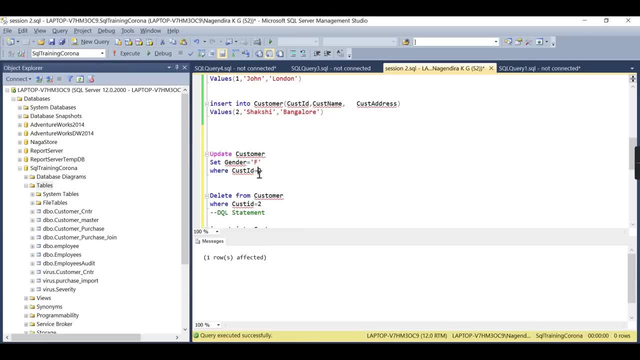 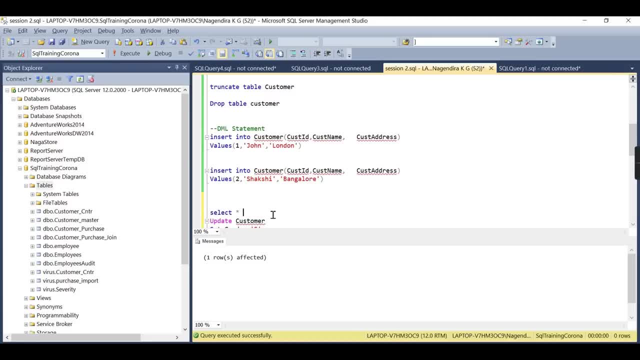 female now once you do the update go and female now once you do the update go and select. it always, always select star from select. it always, always select star from select. it always always select star from customer. so your life as a database customer, so your life as a database. 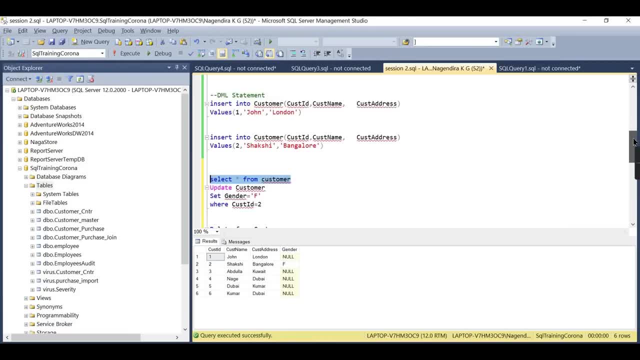 customer. so your life as a database developer will be in select star from developer will be in select star from developer will be in select star from table. only now you can see like of our table, only now you can see like of our table, only now you can see like of our- only for Sakshi I want to update. so where? 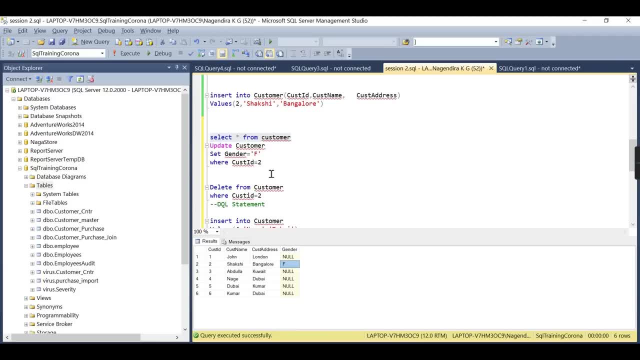 only for Sakshi, I want to update. so where? only for Sakshi, I want to update. so where condition is basically: condition is basically. condition is basically restrict your data rows to filter it and restrict your data rows to filter it. and restrict your data rows to filter it and update or select wherever it is possible. 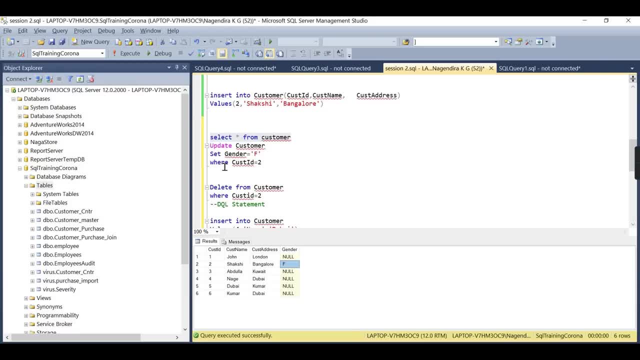 update or select wherever it is possible. update or select wherever it is possible. you want to apply it to filter a rose. you want to apply it to filter a rose. you want to apply it to filter a rose. you want to use where condition now for. you want to use where condition now for. 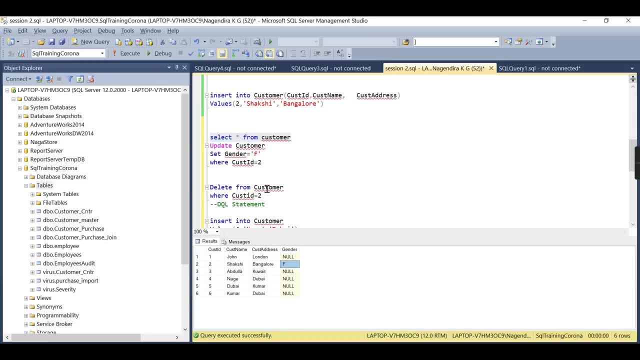 you want to use where. condition now for other than two, everyone is male. so in other than two, everyone is male. so in other than two, everyone is male. so in that case I need to go for not equal to that case, I need to go for not equal to. 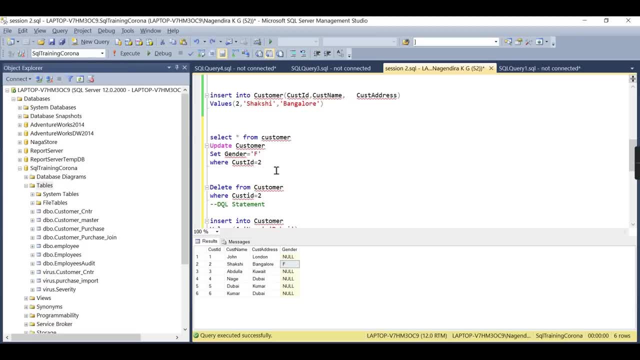 that case, I need to go for not equal to two. make it as Jeff. let us have this one. two. make it as Jeff. let us have this one. two. make it as Jeff. let us have this one as such. let me copy and put it here as such. let me copy and put it here: 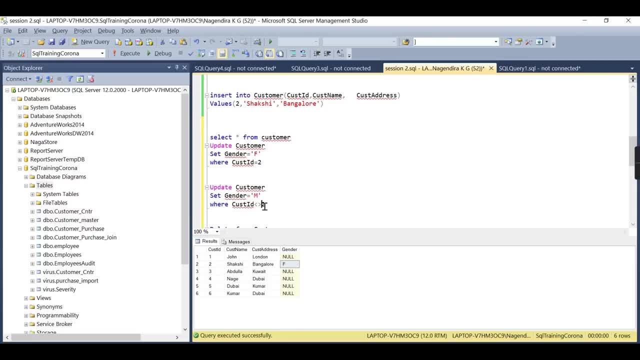 as such. let me copy and put it here and I will say: not equal to 2, so this. and I will say: not equal to 2, so this. and I will say: not equal to 2, so this condition, this condition will evaluate condition, this condition will evaluate. 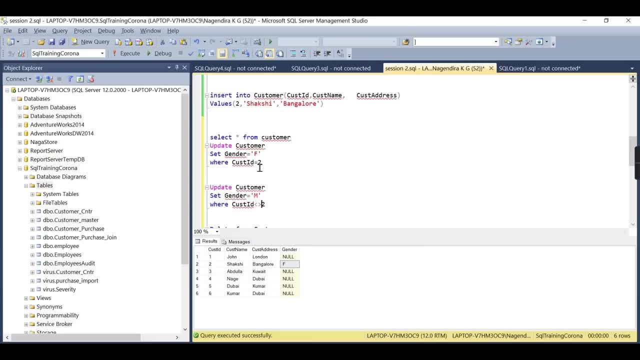 condition. this condition will evaluate for each row. okay, and say, for example, for each row: okay, and say, for example, for each row: okay, and say, for example, this is 2, so it will check for customer, this is 2, so it will check for customer, this is 2, so it will check for customer ID 1 equal to 2. no, 2 equal to 2, true, then 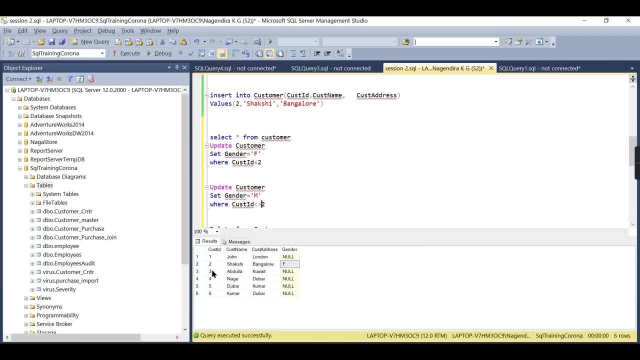 ID 1 equal to 2. no 2 equal to 2: true, then ID 1 equal to 2. no 2 equal to 2: true, then update this particular gender column. update this particular gender column. update this particular gender column. and 3- it will say false. so like that it. 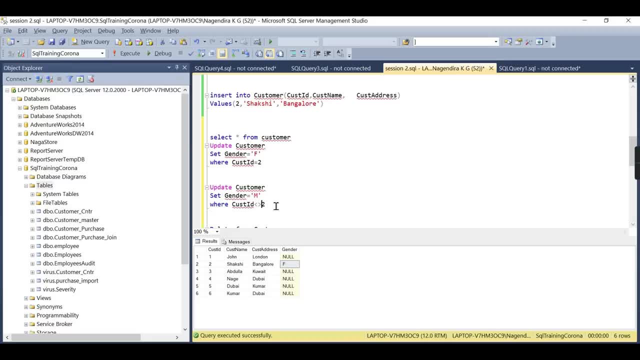 and 3. it will say false. so like that it and 3. it will say false. so like that. it will execute whatever rows having a true will execute whatever rows having a true will execute. whatever rows having a true value for that, it will execute this set. 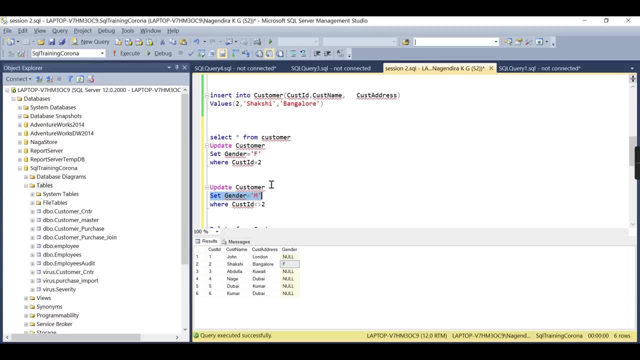 value for that. it will execute this set value for that. it will execute this set statement. that is the syntax for update statement. that is the syntax for update statement. that is the syntax for update. now, other than 2, every row will become. now, other than 2, every row will become. 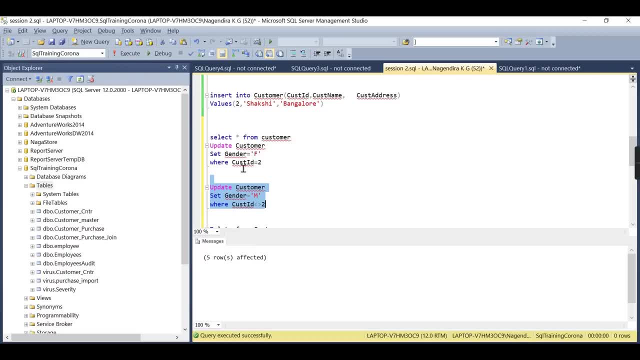 now other than 2. every row will become true for this, let us see. so. it says 5. true for this, let us see so. it says 5. true for this, let us see. so. it says 5 rows affected now. let us see. so this is. 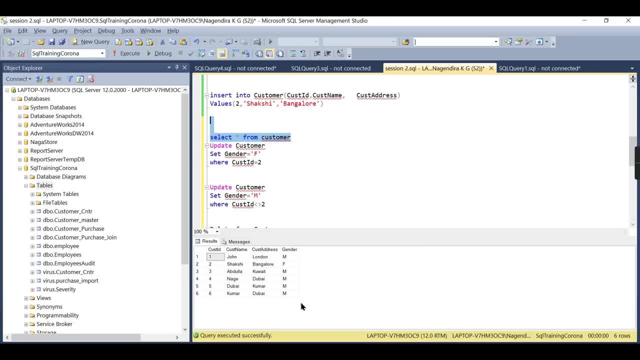 rows affected: now let us see. so this is rows affected: now let us see. so this is how you can update a newly inserted. how you can update a newly inserted. how you can update a newly inserted column for different combination: you need. column for different combination. you need. 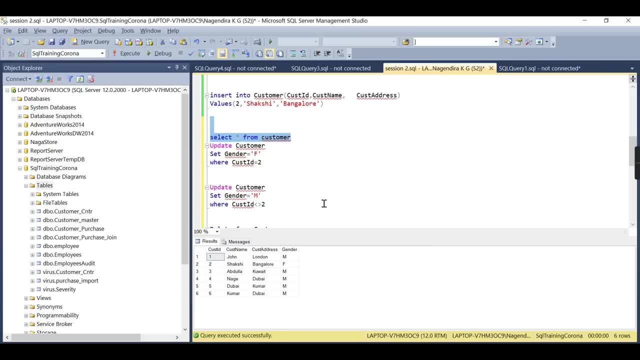 column for different combination. you need different conditions. so this is one of different conditions. so this is one of different conditions. so this is one of the important aspect for your. the I mean the important aspect for your. the I mean the important aspect for your. the I mean what you called SQL statements. so there, 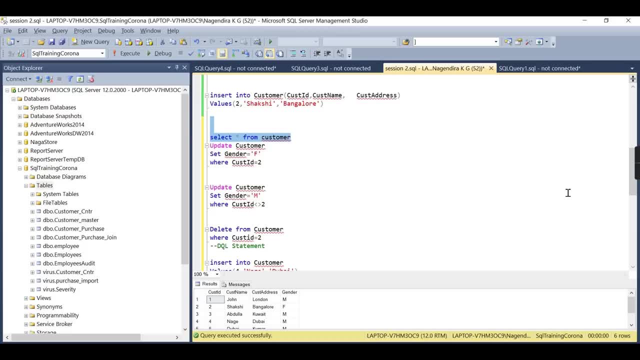 what you called SQL statements. so there, what you called SQL statements. so there are two things, so I've covered it today- are two things. so I've covered it today are two things, so I've covered it today. one is about data types: how it is. one is about data types, how it is. 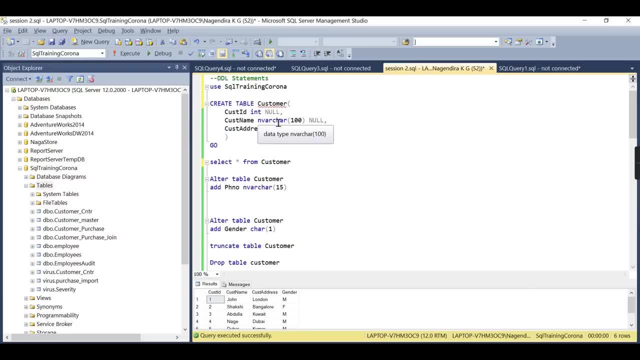 one is about data types, how it is crucial and whether it's integer in crucial and whether it's integer in crucial and whether it's integer in worker. you cannot insert a numerical worker. you cannot insert a numerical worker. you cannot insert a numerical value into integer and 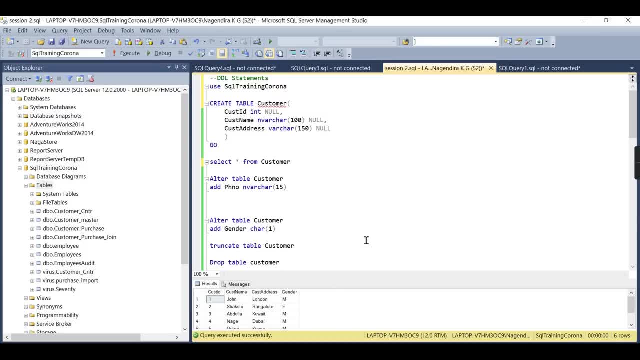 value into integer and value into integer and the different SQL statements, and we will see another important and we will see another important and we will see another important concept here in the SQL, in the table concept, here in the SQL, in the table concept, here in the SQL in the table, it's like you can see here and null are. 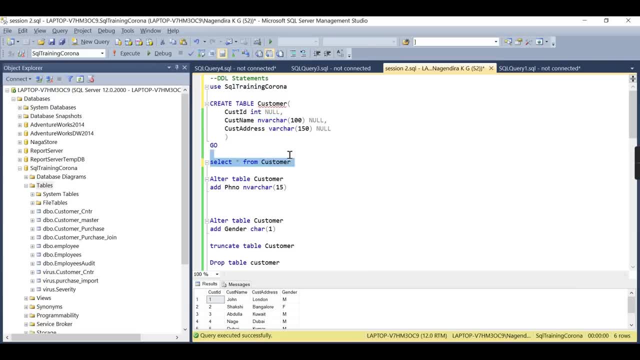 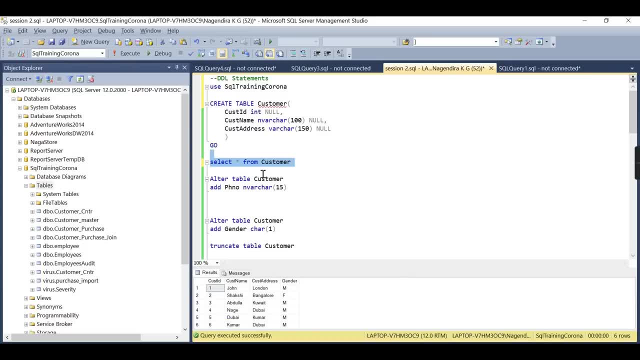 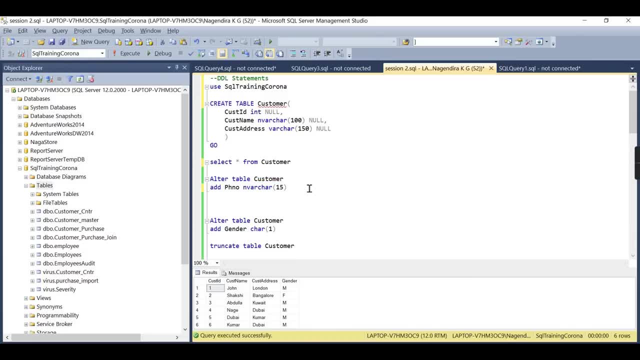 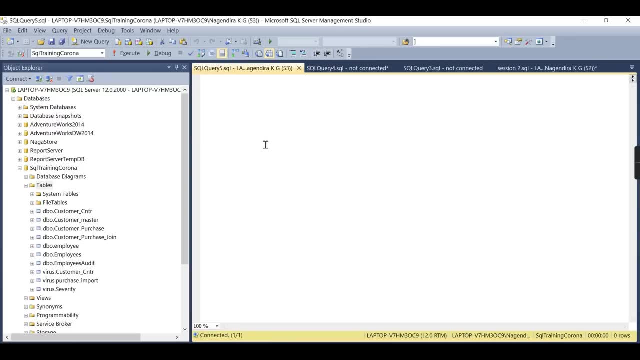 column here, like phone number, okay, and which I'm defining it as. let me add one which I'm defining it as: let me add one which I'm defining it as: let me add one more table. create table gender and what more table: create table gender and what. 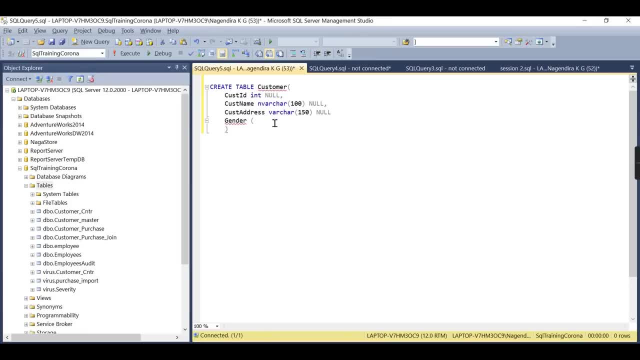 more table, create table gender and what you have like come home in that care of you, have like come home in that care of you, have like come home in that care of it's. again it's a care care of one and I it's again, it's a care care of one and I. 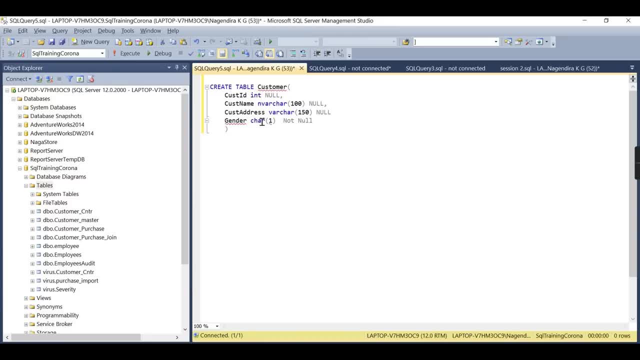 it's again, it's a care, care of one, and I will say it as not null: okay, put it. will say it as not null. okay, put it. will say it as not null. okay, put it. come on the customers, not not just for. come on the customers, not not just for. 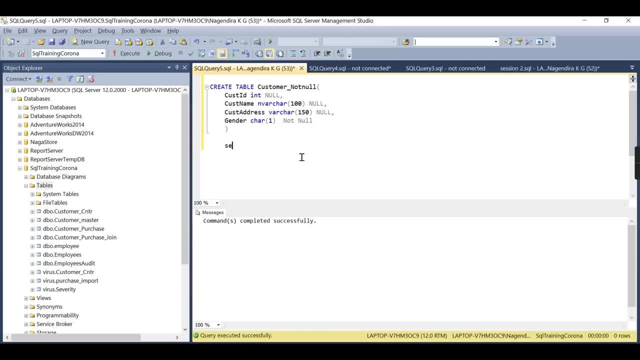 come on, the customers, not not just for understanding and putting it here and understanding and putting it here, and understanding and putting it here and now you see select star from. now you see select star from now you see select star from. I'm trying to explain how. what are the? 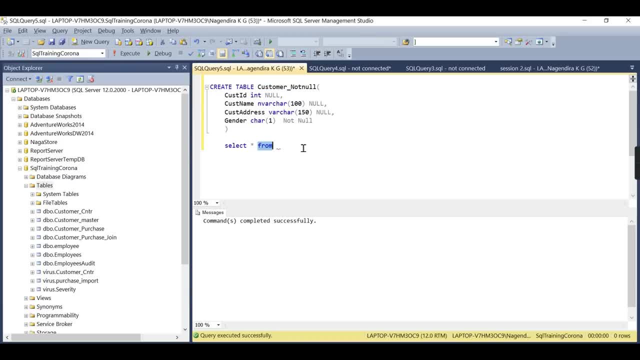 I'm trying to explain how. what are the? I'm trying to explain how, what are the different things? you have it in your different things. you have it in your different things. you have it in your table creation step. that is core. table creation step- that is core. 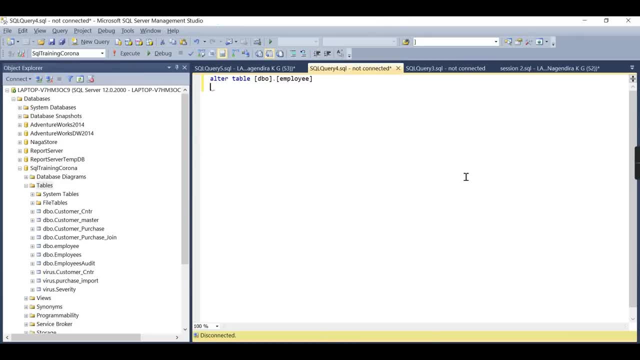 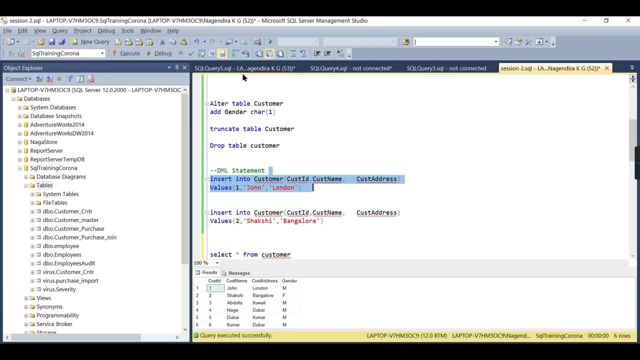 table creation step. that is core. important select star from customer table. important select star from customer table. important select star from customer table. not null is null. now I want to take. not null is null, now I want to take. not null is null. now I want to take insert table script and this is a. 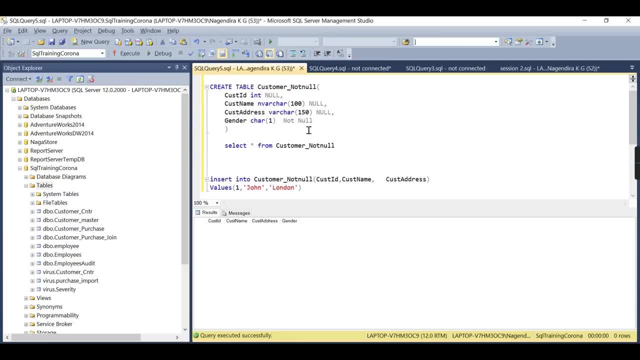 insert table script and this is a insert table script and this is a customer table. not now customer table, not now customer table, not now. let me put it here now. this I defined as. let me put it here now this I defined as. let me put it here now this I defined as not null. okay, what happens if I'm not? 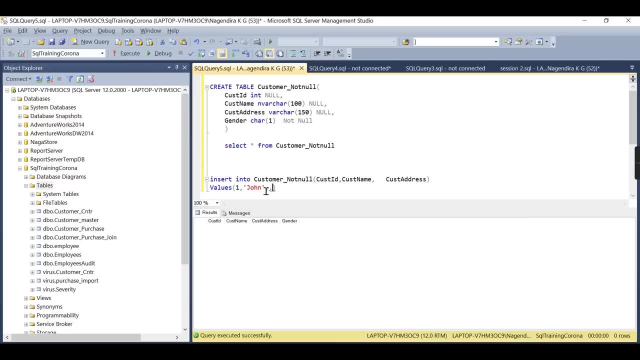 not null? okay, what happens if I'm not not null? okay, what happens if I'm not putting this value at all? that is, I am putting this value at all. that is, I am putting this value at all. that is, I am putting customer addresses null. okay, putting customer addresses null okay. 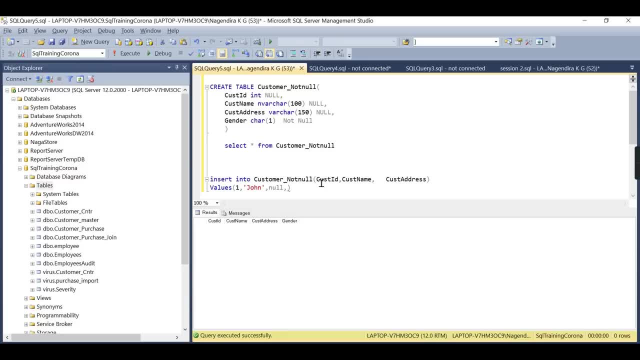 putting customer addresses null. okay, even I can ignore it. let me show it to, even I can ignore it. let me show it to, even I can ignore it. let me show it to you what I'm trying to say here first. you, what I'm trying to say here first. 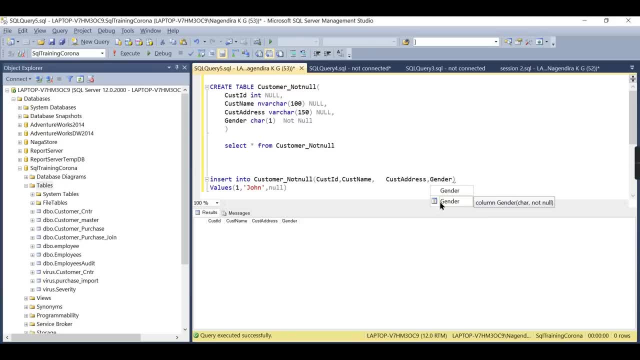 you what I'm trying to say here. first, I'll put gender. I'm trying to insert the. I'll put gender. I'm trying to insert the. I'll put gender. I'm trying to insert the value over here. what was it? it was, value over here. what was it it was? 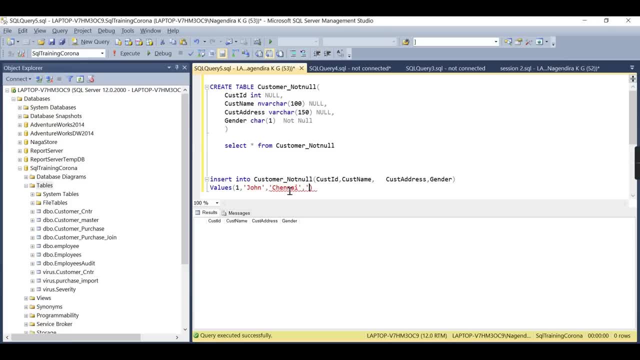 value over here. what was it? it was whatever Chennai, and I will put him as whatever Chennai, and I will put him as whatever Chennai and I will put him as male. okay, this is fine, now one John male. okay, this is fine, now one John male. okay, this is fine, now one John Chennai and male. okay, now, what, what this? 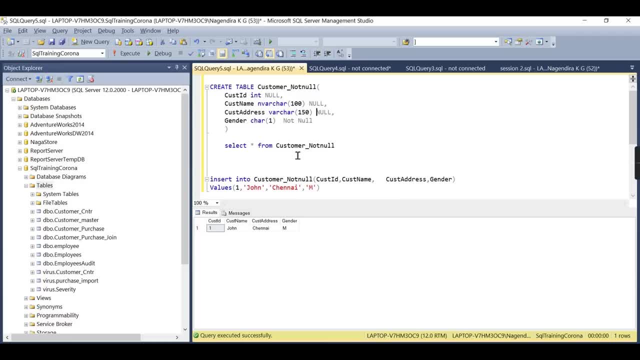 Chennai and male. okay, now what. what? this Chennai and male- okay, now what. what this is saying is like this one: null are not. is saying is like this one: null are not. is saying is like this one: null are not null. this column should have a value, not. 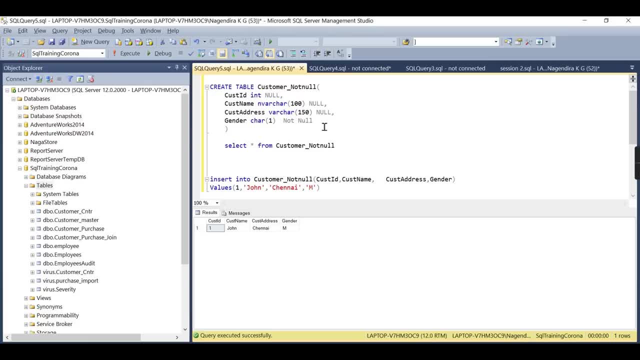 null. this column should have a value, not null. this column should have a value, not null means this column does not alone. null means this column does not alone. null means this column does not alone. else this always should have some value, else, this always should have some value. 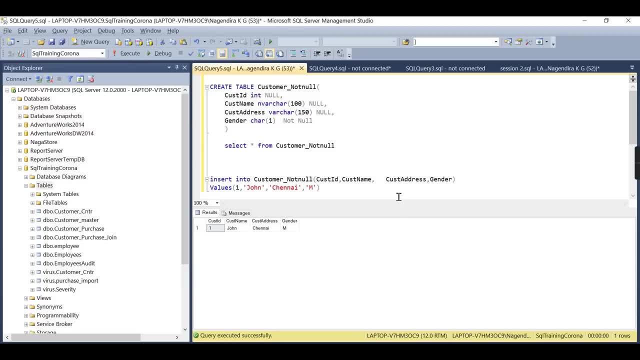 else. this always should have some value. that is what it is say. so some columns, that is what it is say. so some columns, that is what it is say. so some columns are optional meaning like this. maybe are optional meaning like this. maybe are optional meaning like this: maybe some customer can give the address or 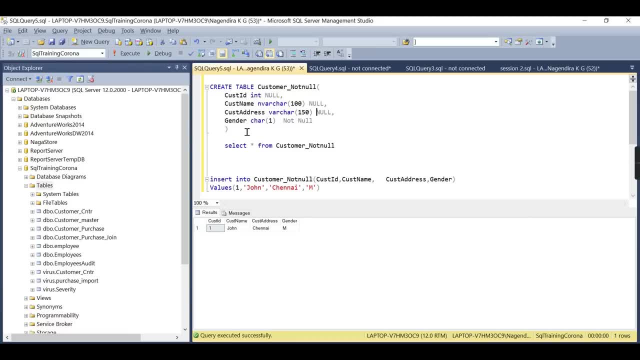 some customer can give the address, or some customer can give the address or not, that is fine. but in your case, like not, that is fine. but in your case like not, that is fine. but in your case, like phone numbers and genders, maybe it's phone numbers and genders, maybe it's. 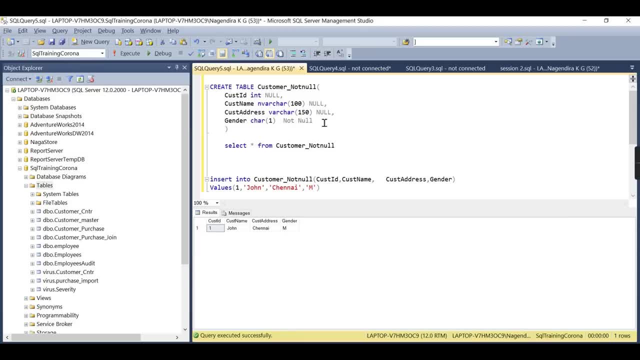 phone numbers and genders. maybe it's like dressing company. I mean the retail like dressing company. I mean the retail like dressing company. I mean the retail company. or they want to understand the company, or they want to understand the company, or they want to understand the customer base, whether they are female. 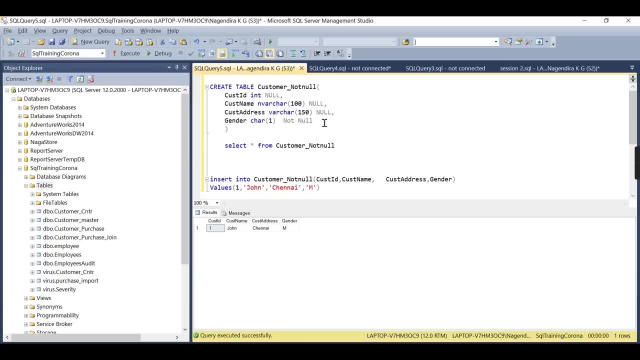 customer base, whether they are female customer base, whether they are female customers or gents customer. they want to customers or gents customer. they want to customers or gents customer. they want to record it, then they will make that test. record it, then they will make that test. 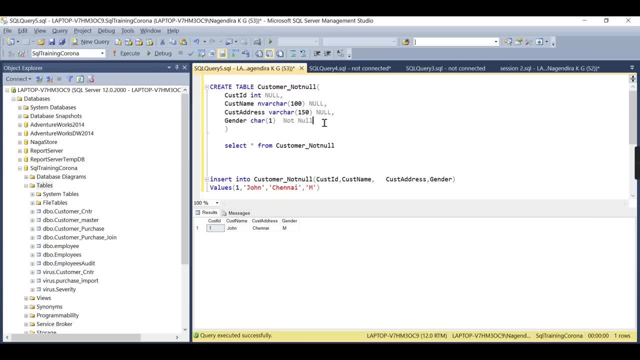 record it. then they will make that test. not know. they want to understand. make not know. they want to understand. make not know. they want to understand. make that as a mandatory field. in that case, that as a mandatory field. in that case. that as a mandatory field. in that case it is compulsory. so now you can skip the. 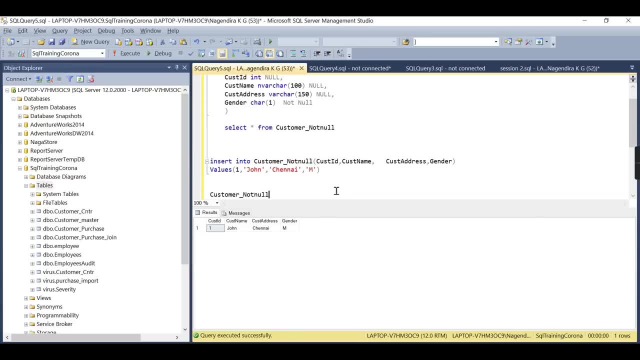 it is compulsory, so now you can skip the second value. what i'm trying to say is: let us copy this once again: i'm i'm not providing this customer address now. okay, in that case, instead of address. i'm not giving any value over there. what happens? let him be two and his skimmer is a male. 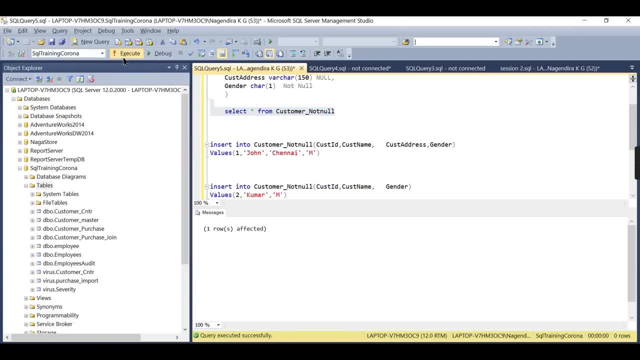 let me insert it. what happened now? now the customer address is blank, there is null. this is allowed. so this particular null is a constraint that says this column will allow null, that there can be a value or you can skip it, whereas if i am not giving a value for the gender column, 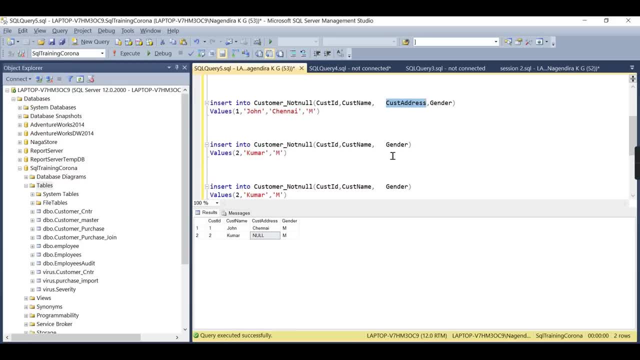 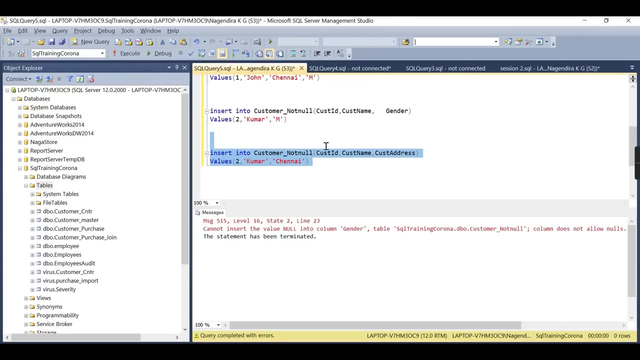 okay, now i'm saying custom, i will give a customer address. now i'm not going to give any value to the gender. instead, i will give only chennai. okay, what happened to this statement? you understand this two difference, uh, statement difference. now the error says: cannot insert a value. 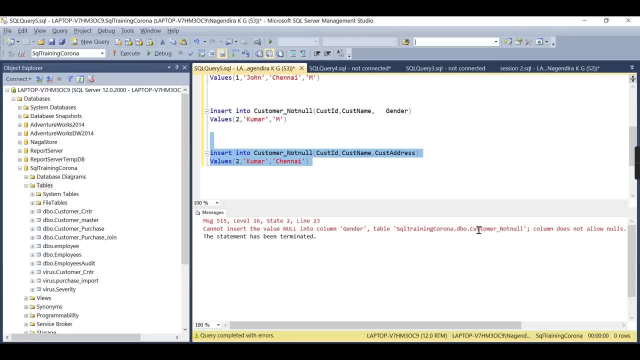 now into a column: gender. because of this constraint, column does not allow null. how this error comes is because of this single constraint. okay, so you are defining some, imposing the rules. as i said before, these kind of rules are data in integrity. you cannot impose in the file system. that is why 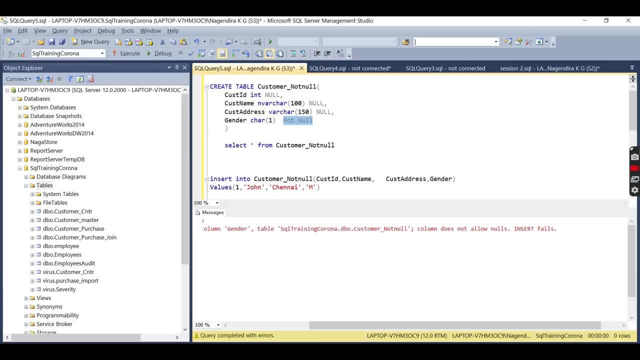 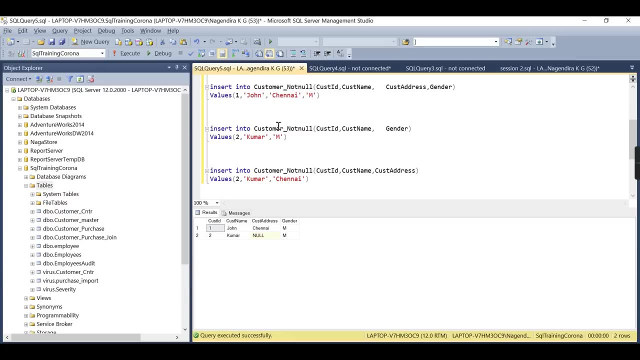 you are going for this database management system. now you understand this point. now this record is not at all inserted. that is, two kumar chennai is not inserted. you can see this: one, two kumar blank. that is, this statement is executed, two kumar blank and mail is executed. but whatever you mentioned, 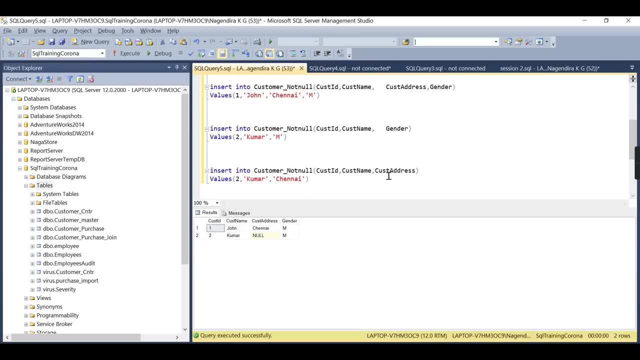 only chennai. two kumar chennai is not executed because you are not giving the gender. in order to insert two kumar chennai with he, maybe again, i will insert just as a duplicate. that's fine, i want to. i have to put this column here. 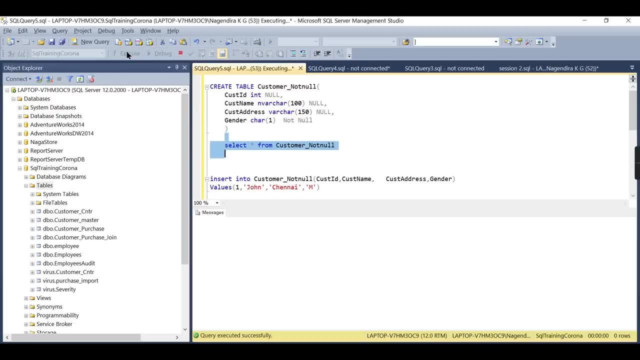 so you need to correlate this to any business scenario, as i mentioned before. so these are the some of the constraints: null, not null unique check. so i will cover more on to uh next session. uh, we will stop it today, okay, i hope. uh i covered uh two of the topics. one is 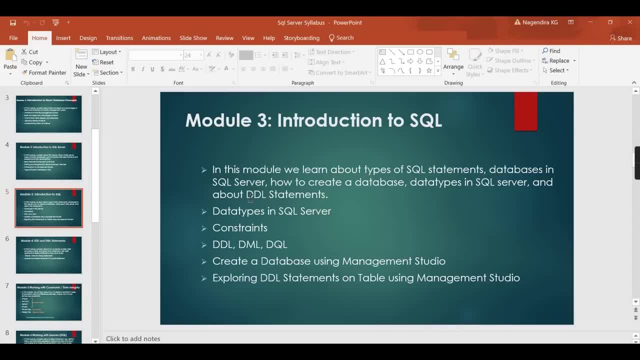 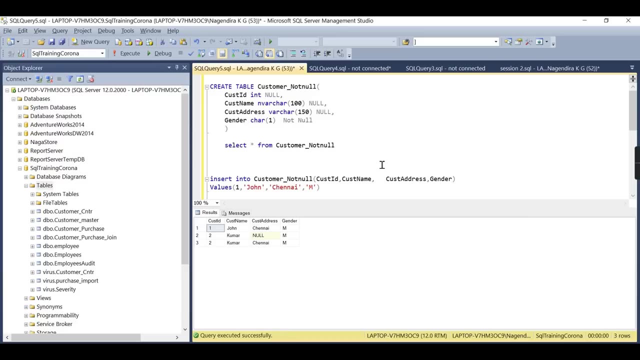 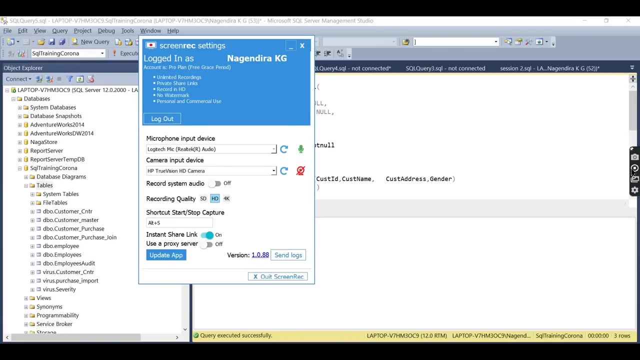 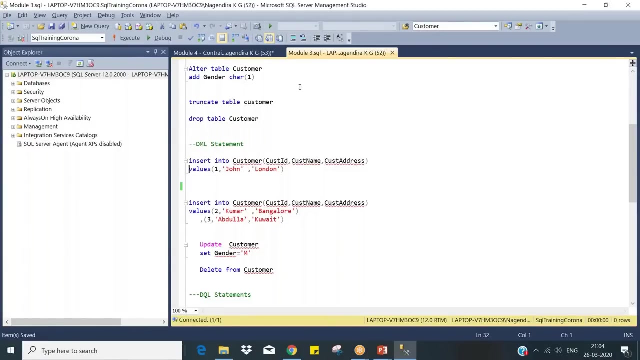 about um, um, introduction to data types and ddr, dml topics, then constraints. i will take it on next session, okay, so uh, yesterday we saw about uh, not null constraint, so we have a table over here, dot home, let's see whether this table exists. so there is no data and we have only three columns. let me do once again. i'll put phone number as not. 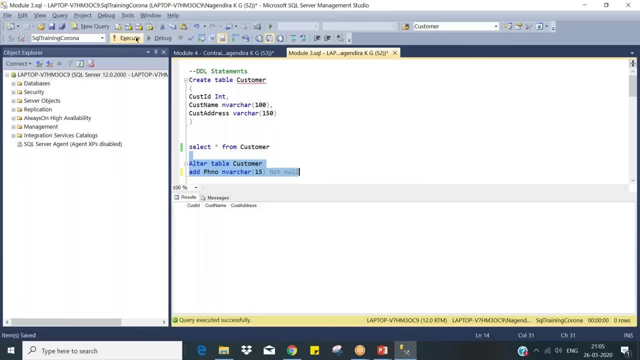 null. so i'm adding a column here. now let's have phone number. so, and yesterday i mean uh, till this time- i had only three columns inserted, see, uh, i'll first come to the normal part. so now i have a phone number defined as not null here as a constraint, not null. now what happens when i try to? 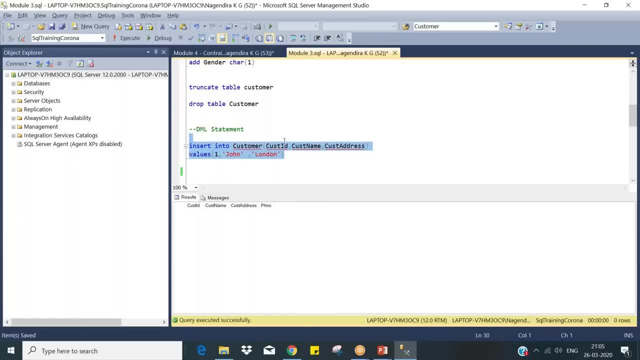 insert without a phone number. okay, i have mentioned only three columns here, so phone number is not included, meaning null is inserted. it says: cannot insert a null value into a column phone number. that that part i have seen yesterday. now when i want to insert, i'll go and check. 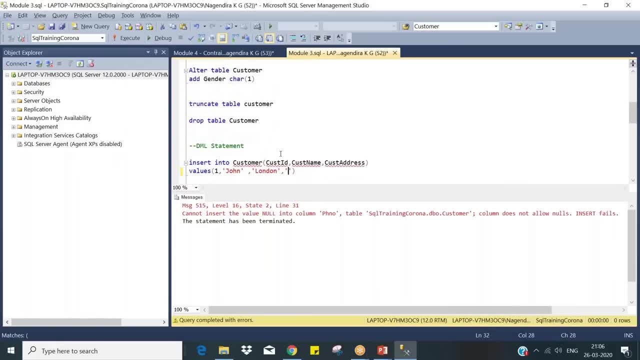 what is the varchar? only i put. so i put just, uh, my quiet number. it is eight digits, it's one. okay, now when i do the same thing here, it get inserted. there are fewer. yeah, see, this is another important factor i want to inform you: there are fewer columns in the insert statement. 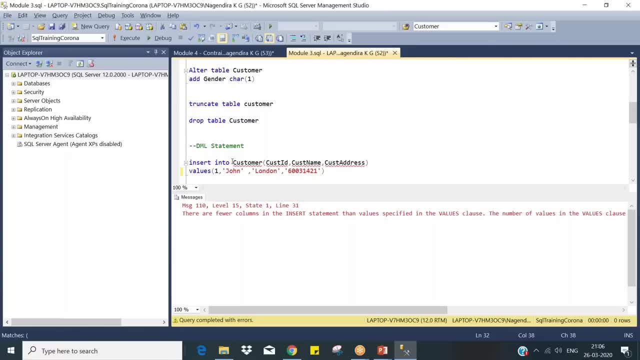 than the value specified in the values. column meaning like see i first statement indicates insert into customer. i am saying you insert customer id, customer name, customer address. okay, only three columns i mentioned. but while giving the value i gave four columns, including a phone number. so it wrote the error. so you need to add the phone number as well. now you see phone number. 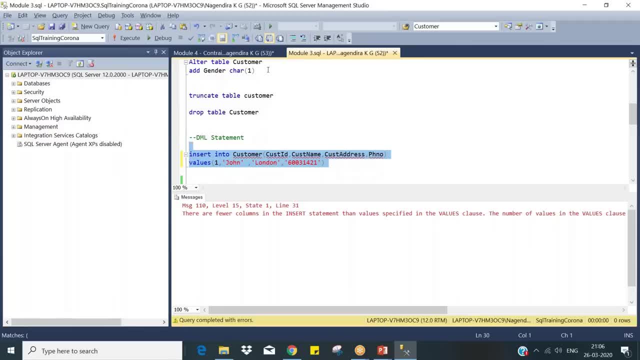 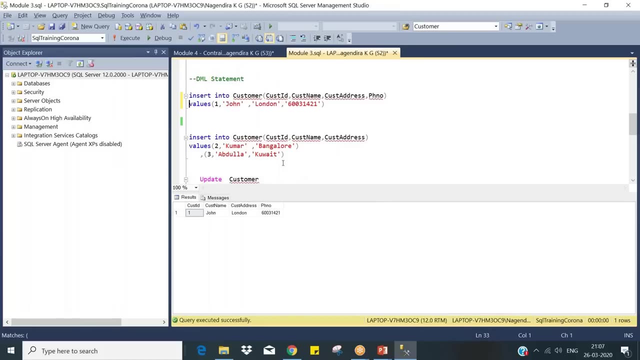 i have added now i will insert it. it succeeded. so now you select the data. you got the phone number, so you might have a question like whether i need to mention the columns always. if you remember the column order, people won't remember what columns order that created in the table. what i'm trying to say is, if you are not specifying the 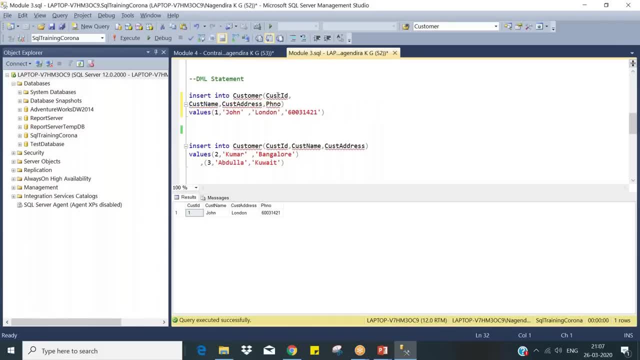 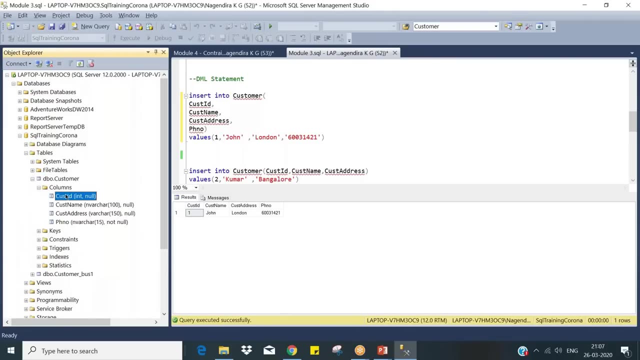 column order. here in the insert statement, the sql will take the default order how you are created. you see here this is the customer. so this is the first column, second column, third column, fourth column: this in this order it will take. okay, now what happens if i remove this order? i mean, uh, this column specification. will it work any guess? 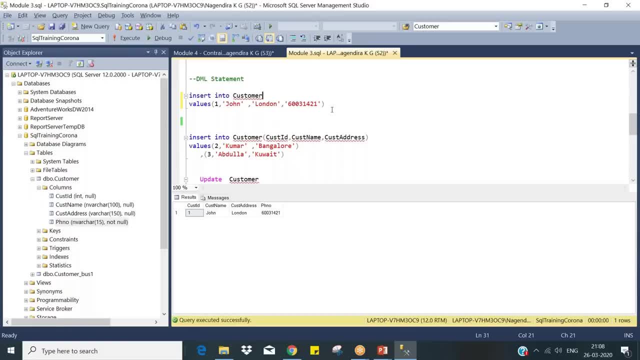 it should work. yeah, you are expert, i know, so it will work again. i will do insert. yes, it worked good, but what is the data here? see, i have two records already. i inserted already. this is the case. but what is the big challenge in this is like: 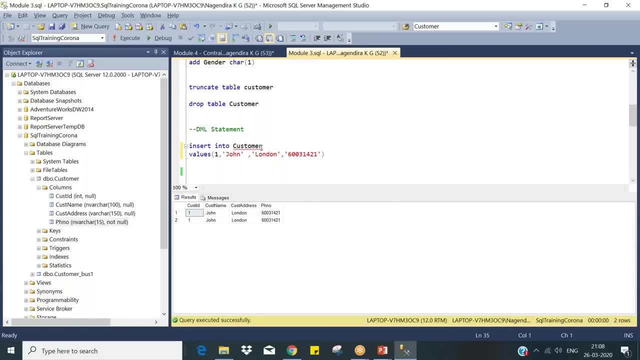 you can't remember what is the order of the column and until you know this one say, for example, by mistake: if i do like this, the order is changed. okay, will it work? yes, obviously it will work. now what happens? so in the customer address place i replaced okay, see the issue over here. 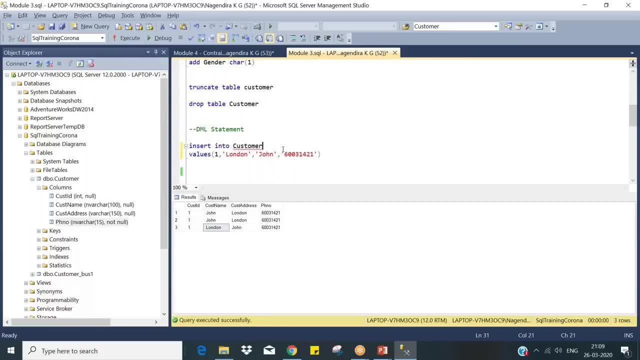 if you are not specifying what column i am setting was inserting here, by default, it will take whatever order it has created now in order to achieve the proper ordering. now i will say: see, without specifying, this london has went to customer name, this john has went to customer address. now i can do a proper if i mention. 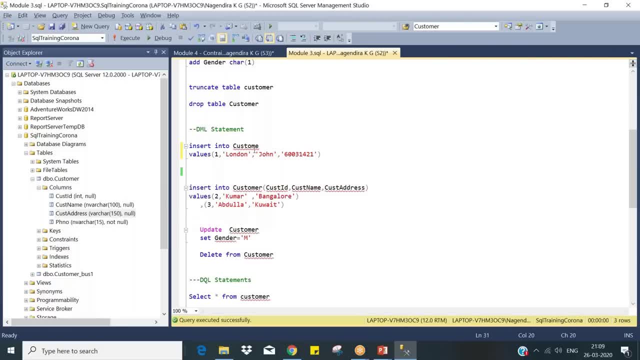 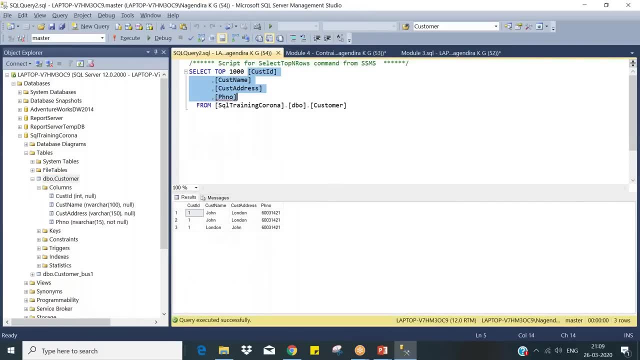 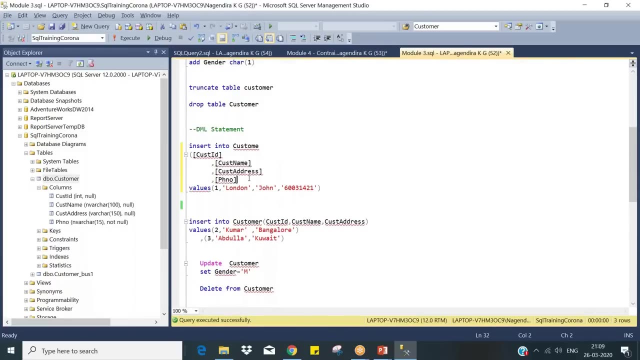 the column names over here. give me a minute. it will be two basics for someone who already knows this. so specifying the column order is very important. now i can say whatever order i want. okay, so this london is nothing but my customer address, so it should go in the second column here. 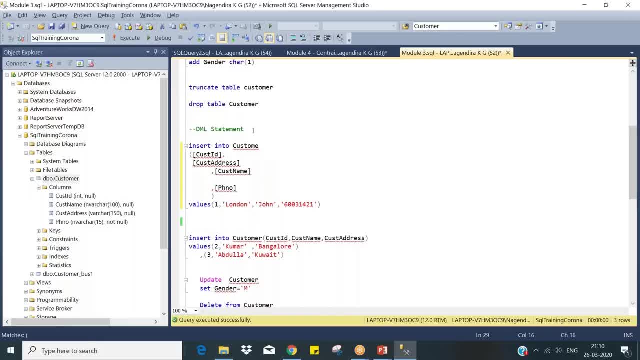 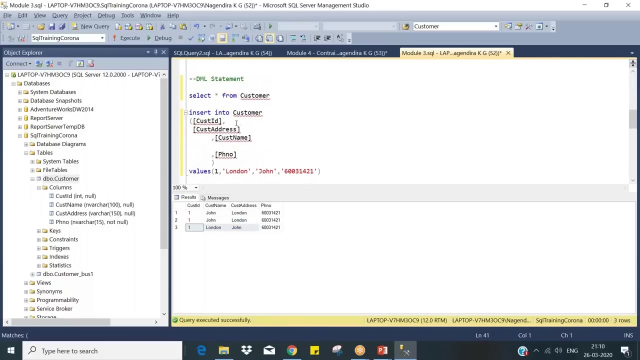 and customer name. now you see, let me select and show you the results first. see, now, this record is wrong, wrongly inserted. okay, now what i'm trying to say is: whatever order you are specifying here- customer id, customer address, customer name, customer phone number- same values should be represented in the values as well. 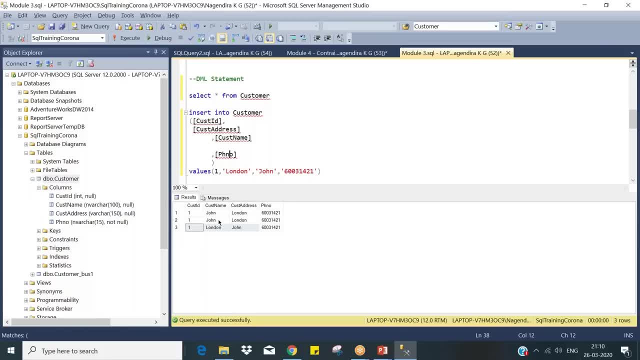 so now, when i insert it, instead of this wrongly inserted record, i can have a proper record here when i select it. let me see, let me show it. okay now. you see, now you got london. even you have a one london john over here. the column order, whatever you inserted, it doesn't matter. 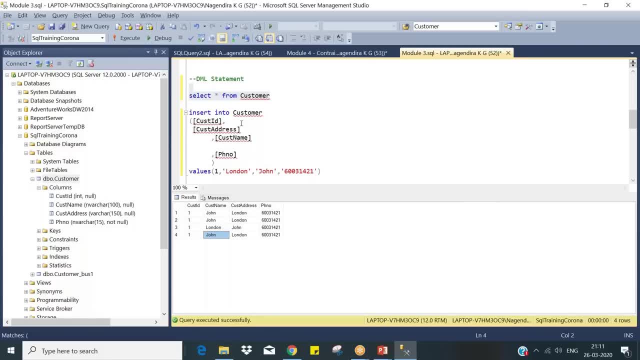 when you select it, it will properly insert into proper values. so it is always recommended to specify the column names while you are inserting. okay, just you cannot skip it, because people will forget what is the column order over here. whatever you created, okay, that is the thing, it doesn't mean. 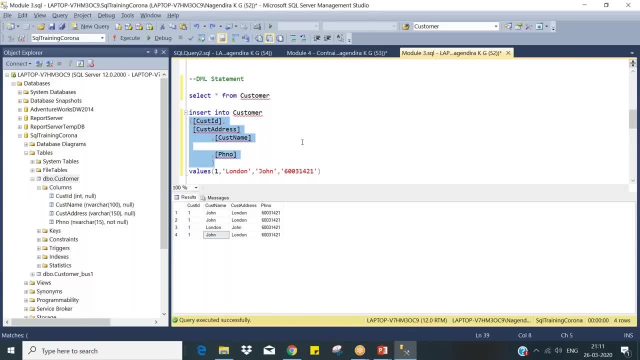 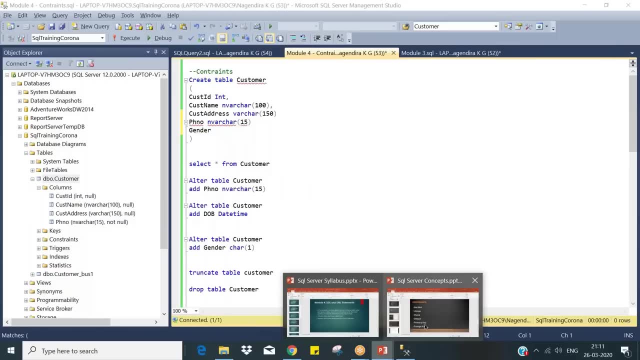 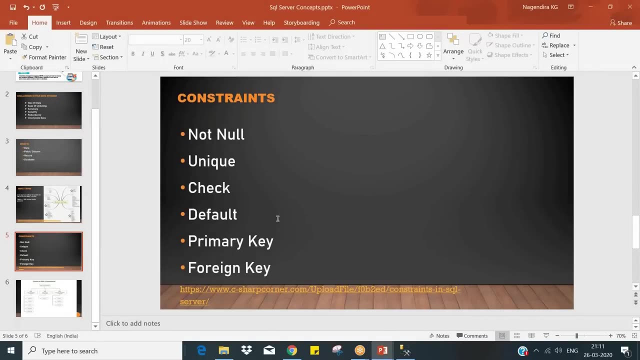 anything about the constraints. just for your understanding. i told you back to the topic, not null we have discussed now what are other constraints we have? we have a unique check default. we will discuss these three now. i will take primary key, foreign key, later when i use joints. 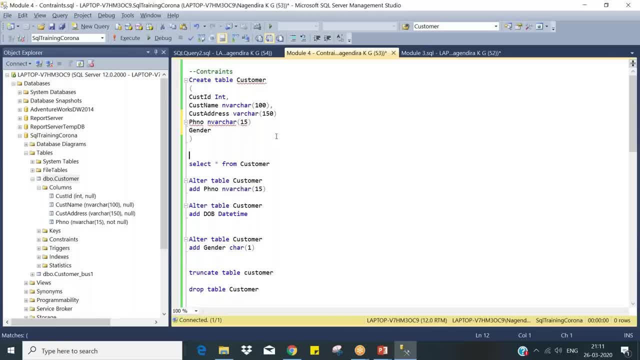 so unique. so now i told: not null, always i need a data, say for example: uh, not. now i said the phone number i need mandatory, okay, but i don't want to get people won't give phone number. sometimes you as a customer, i will say like i will not give you a phone number because you will send me message. 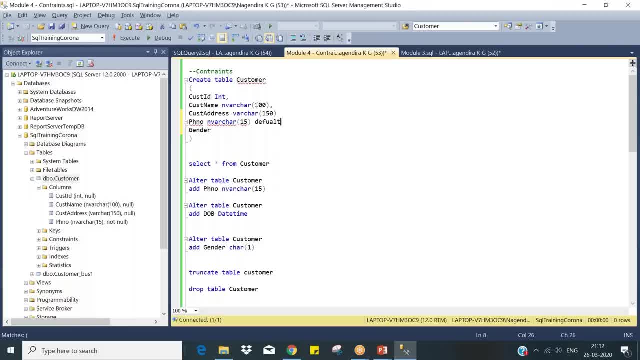 but i want the phone number by default. application design like that, so you you'll put some dummy numbers over here. default nagi. one question, uh, for inter. can't we give you any constraint like in? uh, like size integer, that is the size i mean. yesterday i gone through this. i mean in this website you can go and check. 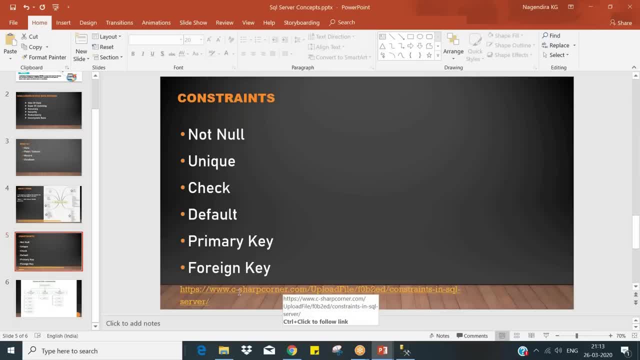 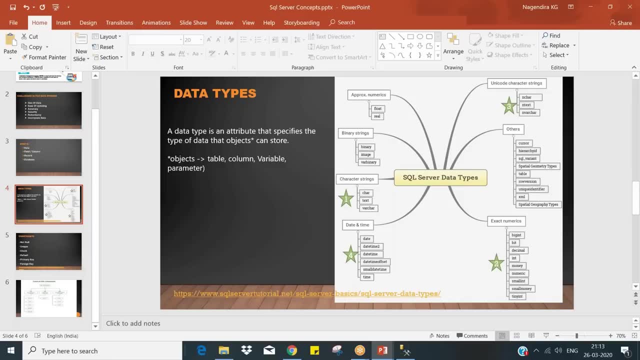 it out and see what is the size, maximum size, uh, it will have like: uh, yeah, i'm not asking maximum size, can we define the size for an end? now, integer, by default, it will have its own say. for example, let us go and check it here- it will have something like 2.3 million, something that is the maximum. 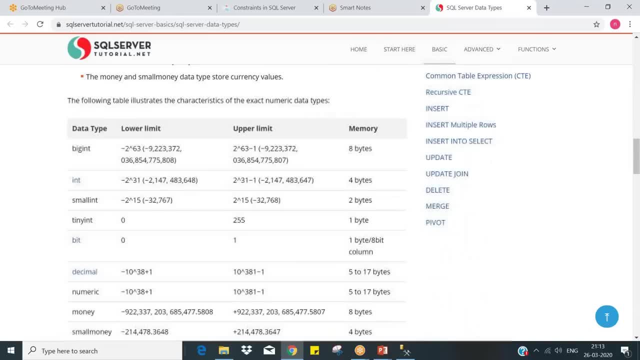 limit for integer. so, but it is understood it is a whole number, big end int data type value. it will allow this much. well, this is the maximum size, but it is, it is defined, it is internally understood. small it means only: uh, 28 characters, something like that, 128. so three, two. 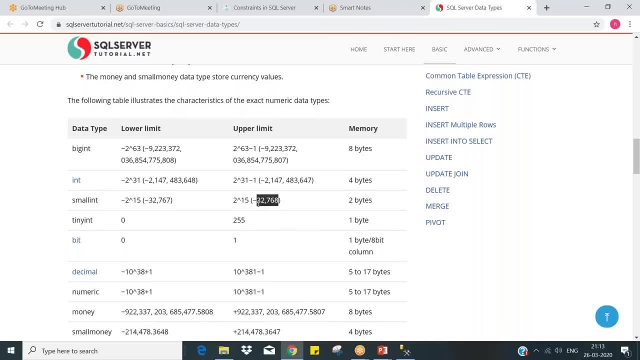 seven six, eight. thirty two thousand seven sixty eight. you can. if you uh type it as thirty two thousand seven seven seventy, it will throw a limit crossed. it can store up this value only. i got it so. but integer, it will show this one, so no need to specify the size. 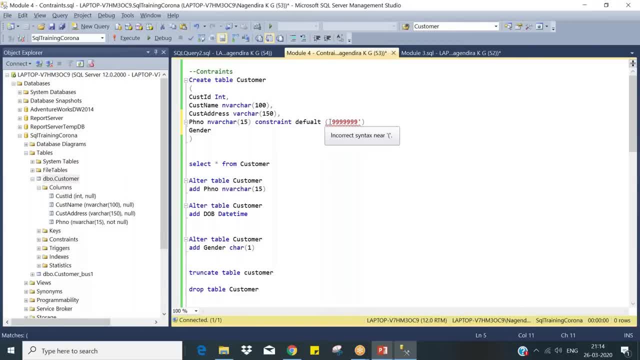 okay, now i always i used to have that feeling spilling mistake- got you. thanks, shrabani t. thanks so phone number. i want to make it as default, okay, what i'm trying to say is now you saw a not null constraint one. only if the, if it has a value, then only it will allow. if doesn't have a value, then, as i need to put, 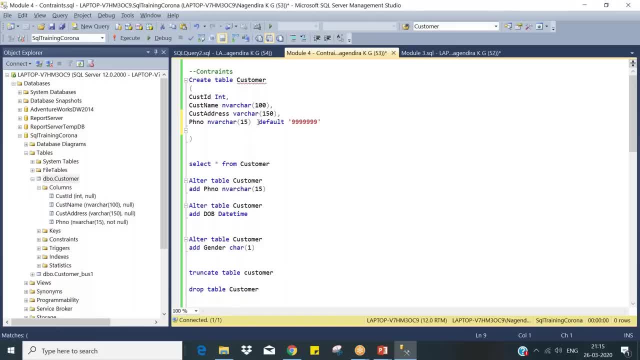 something in that place. so it's combination of both. it's a, not null. you need to specify a value, but if someone is not specifying, make it as a default. that is triple nine. some some values say, for example, some phone numbers. okay, this is your default. let me create. 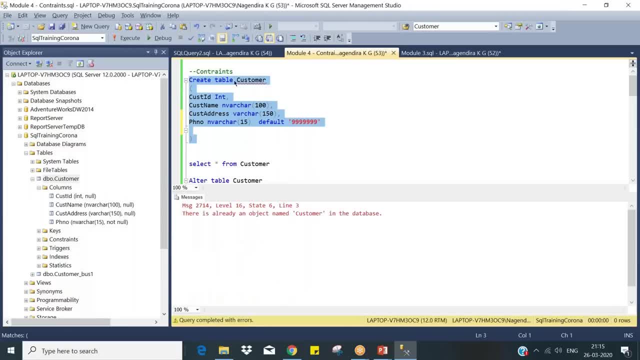 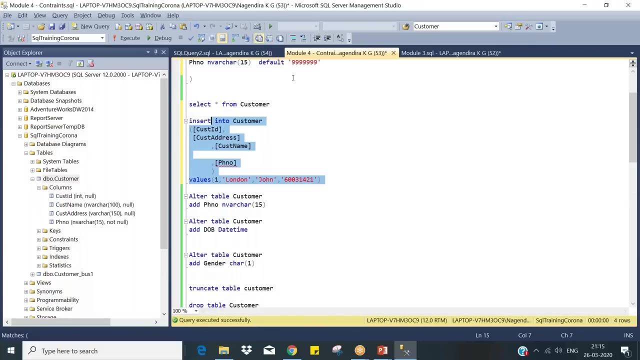 and you can understand the data constraint: create table, customer constraint. okay, now you don't have data copy. this guy. see guys, i'm i'm trying to insert the existing record here. i want to add something, i want to set a set up. so now you see, my data is created. so i have. i've got, uh, six, double, zero, three, one. now what happens if i don't specify my data? so just type in six, twin, two, three, one, well, and majored. so now i've already get my data. so call out feature the instant desire configuration and it will automatically, in Kansas City, block the pizza creator. if you have an internet английic program, then there will be a different app. so if you have a open c? c local network and regardless of theeeателя, pass through these calls if it's not operating. this important process, so you can remember, in the next session i'm going to do is soldier payment, and i will also have another issue to cover in the second session i'm gonna do, which i will answer: Wolof, WHY and what for my service. 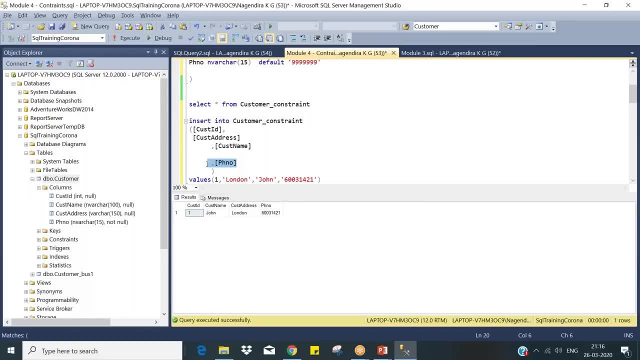 phone number, say, for example, i'm saying i'm removing this phone number, then i didn't specify phone number. earlier case: what happened? it is inserting a null. when you see, when i create a column, empty column, it has created a null values. now you see, default is nothing but. 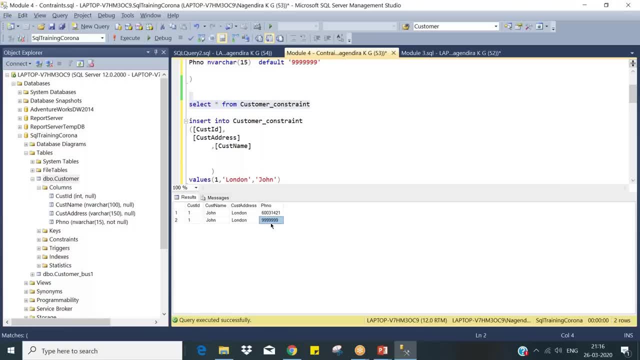 you are stamping some values. if it is missing, some value is missing, you default it. this is a constraint, default, constraint, okay, it's a default. and we, moving on to check: constraint, okay, check is like you say, like you want to have certain rule, impose a rule, say, for example: 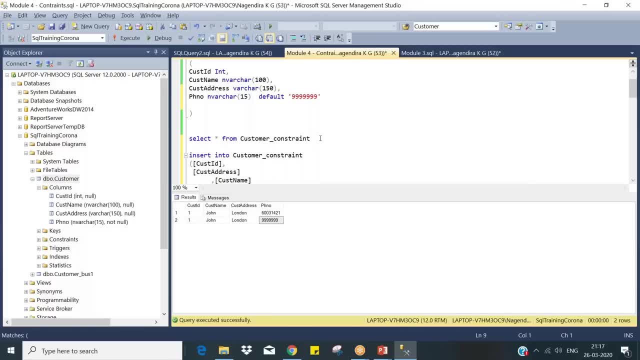 someone is registering uh for a college and whose age should not be uh greater than i mean should not be less than 18. so this is the rule you want to impose. then i create a rule like age integer. you cannot default it here, but you can set a rule. 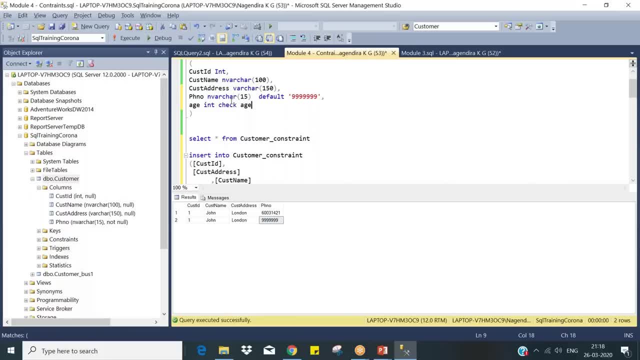 and you say, like a check, if age is greater than 18 or greater than equal to 18, so that's all our problem. so i'm just dropping and recreating these tables, okay, just so that. so all these things i'm dropping and recreating because just you. i want you to understand. 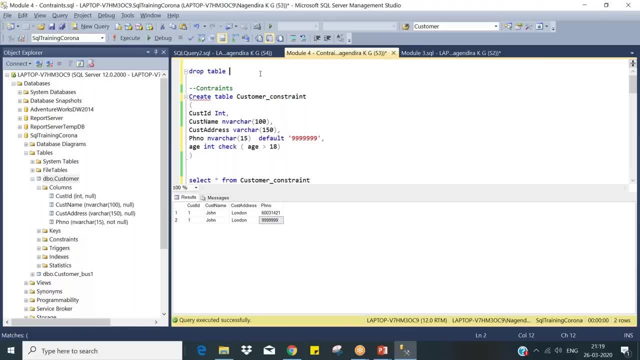 from the beginning, all these things, while creating a table itself. you need to decide, so that's why i'm doing one by one. so now i again created this one. now i'm selecting it. okay, so i'm going to insert this one now. uh, i'm putting only the age here. i'm i'm going to insert age. 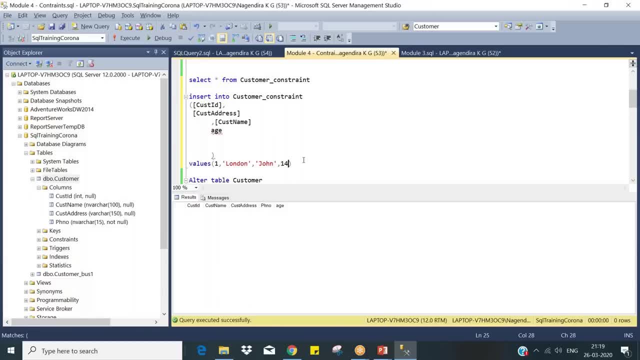 i have two cases, one failure, case 14, and i mean it should fail insert check 14.. come on, insert statement conflicted with the check constraint. so it says like, uh, it is failed. it doesn't inserted value anything right now. so if i use 22, 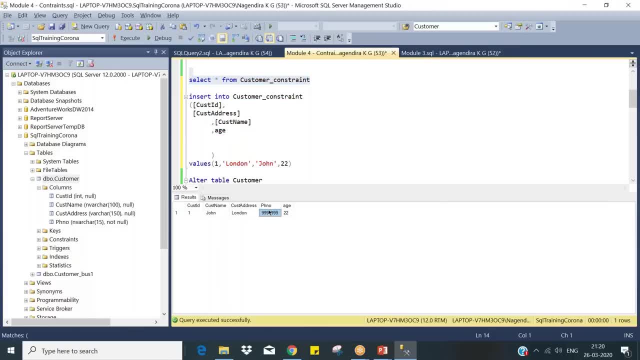 then fine, okay, and it has default to my phone number. i didn't give my phone number, so both constraints worked. so this is about check, default and unique. so there are certain things like my phone number in this case defaulted to triple nine, say, for example, my name should not be. 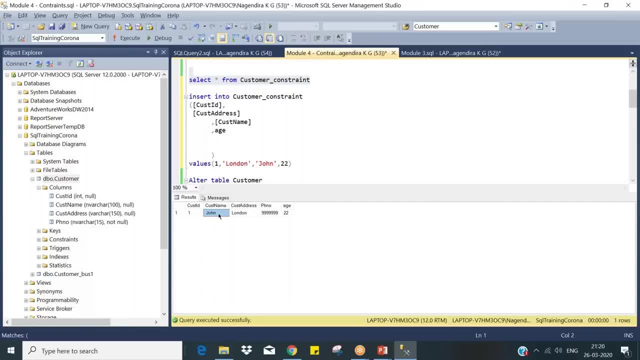 repeated, i should not have any other customer. the perfect example should be a unique constraint. other card, so i have a other number. that should be unique. i cannot repeat for different customers. same other number cannot be applicable to another person, so in that case i will use unique constraint. 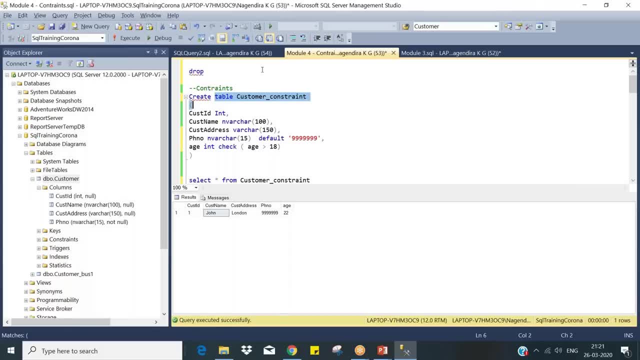 so let's keep this one here. i say other again. other is integer only. so i will put integer. okay, i will say unique, just say unique. it should be unique betweenêteer. this is document and扰 exactly what they are saying. so this is a commenting out, meaning that will not be executed. you need to put two. 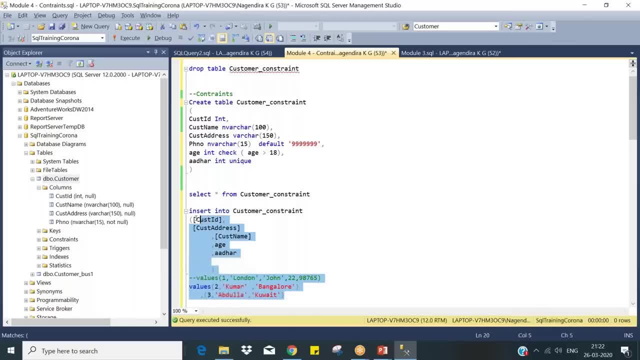 hyphens. okay, that will be commenting out that code. so I commented out now other: I give eight, six, seven, five, something like this AJ didn't put for him, so that our message will be really clear. see, there are message. there are more columns in the insert statement than the values. so I 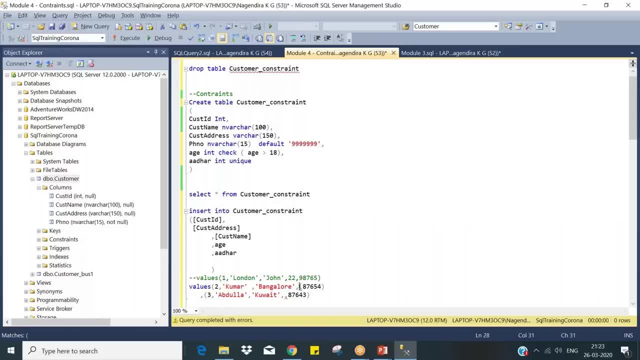 have mentioned the age. I didn't spend sway age here, that's why. so I say that before I will give 34 for him to six. now you see, like each other is your unique: nine, eight, six, eight, seven, six, eight, seven, six, four, three, something like that. what happens when I try to insert a? 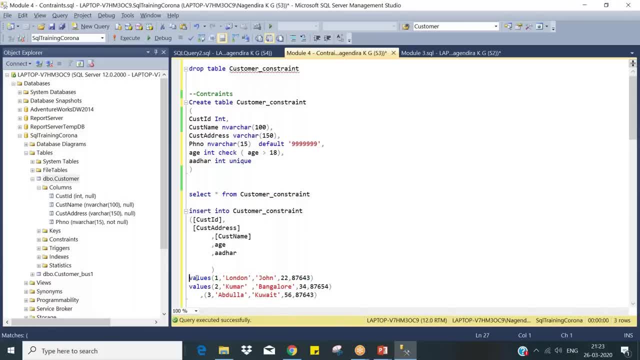 rectangle record with the same value over here. I'll say: I can have one over here. I can have repeated here, repeated here, repeated here. this guy is repeated same. okay, when you use this constraint. okay, violation of unique key constraint cannot insert duplicate key in object. so if you see here: 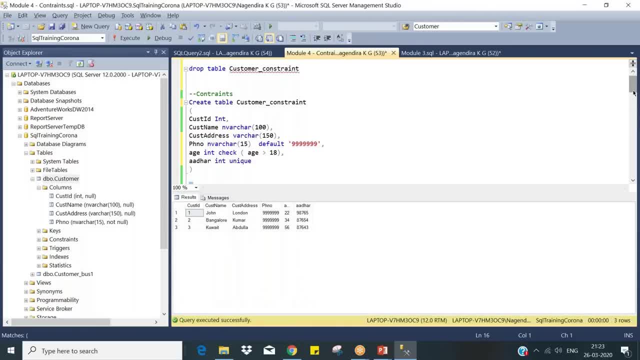 compassion. let's go back to the sketch: render the same and the first one, the constraint's. okay, the constraint now can, if I create other constraintập, sunrise in this case- I have to create another constraint over here, Ceilomaster, okay. so again, you will find that after this text, this6743 pointer. so that means we have 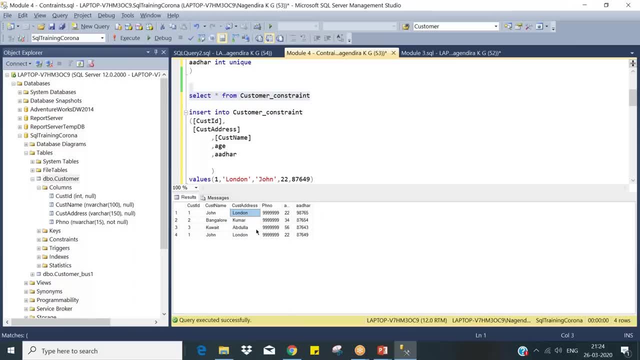 this unique constraint for this particular column. okay, and i i had a default for this phone number, so it keep on adding the default even i didn't mention. if i do mention phone number, it will update and age- i put some restriction that is greater than 18 either. it should be unique. so 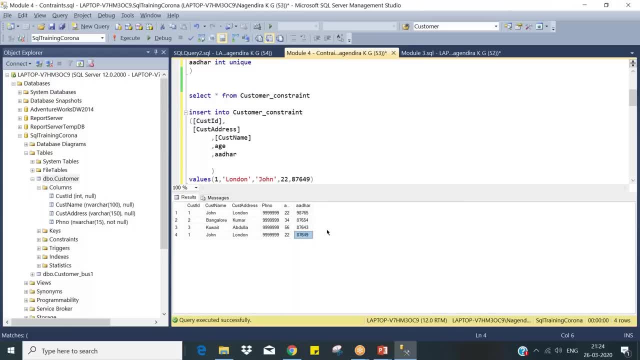 if it is repeated then it throw error. so these are the things why you need constraints. just imagine, in a business world, guys, okay, so that there should not be any duplication of other information. if someone is claiming some, um, some- now you say corona, claim someone, government is. 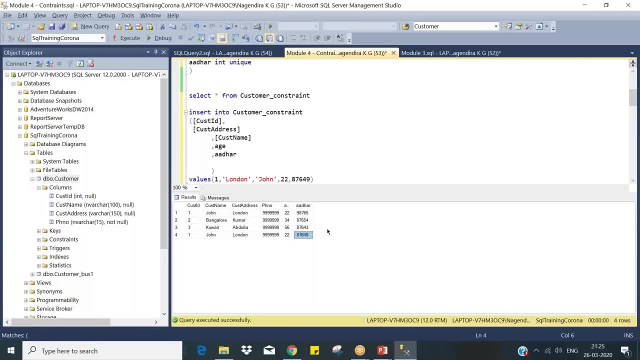 offering thousand rupees, so they will come and whoever collected, so those other will be recorded here. assume this guy again. you are going in some other state and you can claim. people think like that, but if it uh shows this unique constraint, already you have claimed. instead of this error message, i can show: 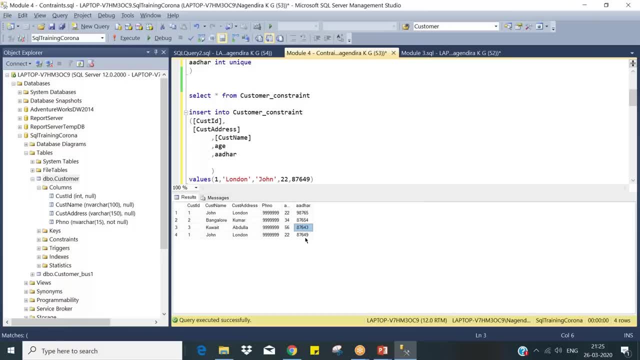 like: uh, you already claimed in this particular location. don't come again something like that. okay, these are the things you impose in database level that will have uh impact on your real business. so that is why you need to have concentrate on this constraint- how you is related to your business. okay, i hope uh, this example. 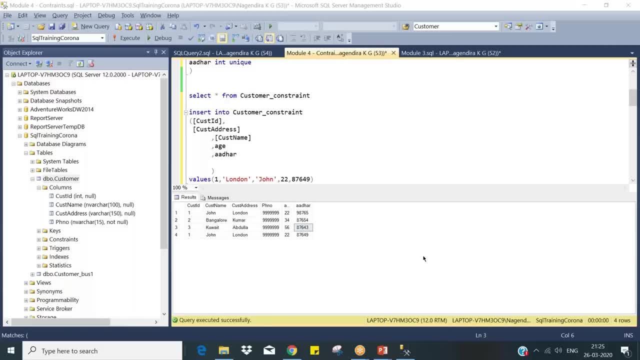 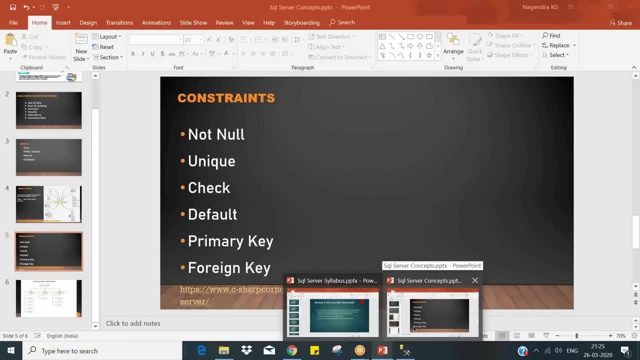 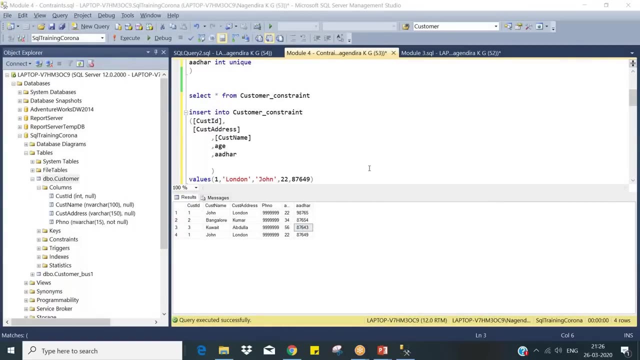 says anything else, guys for, uh, constraints, no, right. so now it's not only for numbers. even like in some websites, work, create this with the same email id. they already tell us, like ordering: yeah, exactly, it works on the same thing, right, exactly. so it is not for a particular number. i'm saying integer is easy to understand. so it is not an integer, it is a. 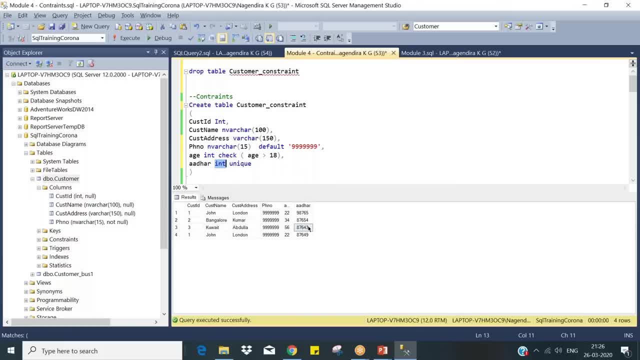 is for the data type. any column that column see, it's for the column, so understand about the column column will have its attribute. this is the attribute of your column. there is nothing but your metadata. i mean to say this: the rules are for the columns, not for integer or character email, as 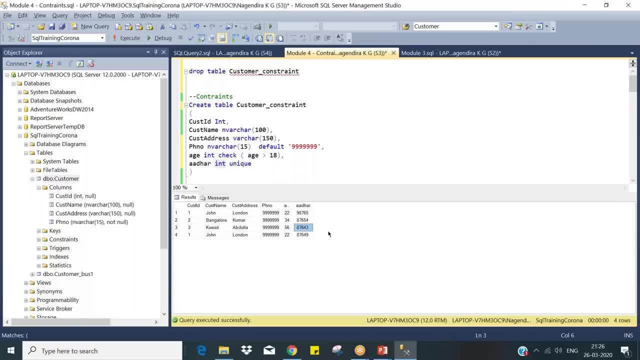 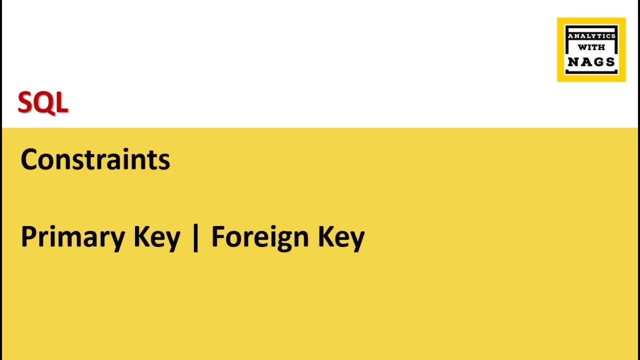 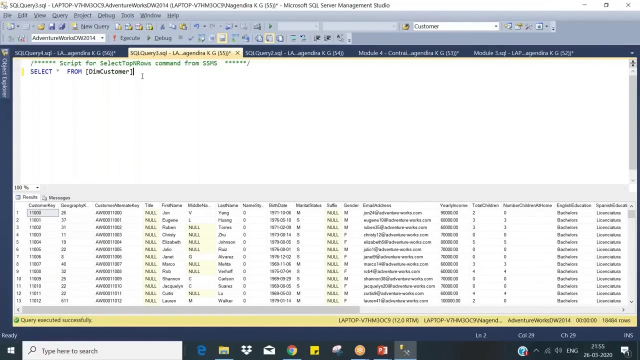 you said email: perfect, since you cannot register same email id in netflix two times. something like that same thing. okay, guys, uh, i will take this primary key, for basically, the primary key is defines your record. okay, i mean to say, if you want any information for that customer, you need one key to identify it. that is what your primary key. 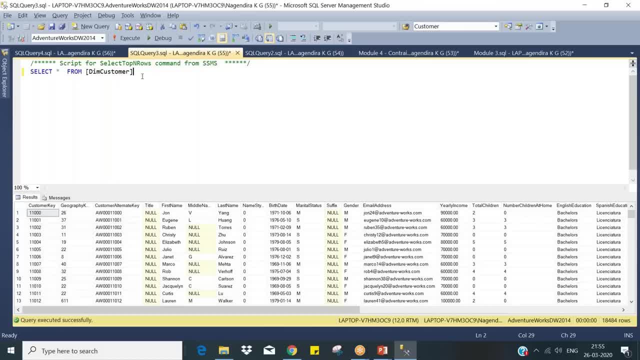 got it so like: um, you have a other id for a customer, then you have other id to be defined as your primary key, then you have your name, all other things, okay. so what about if you do not have other id before other id? what will be your unique? 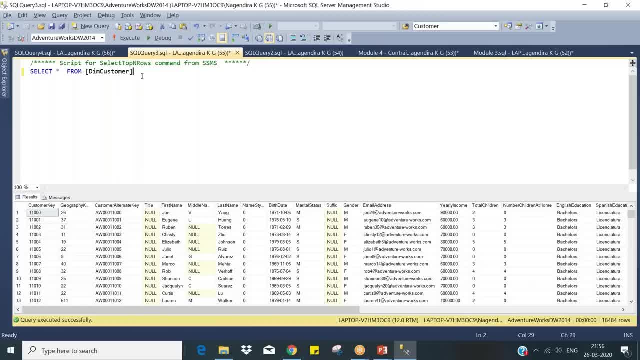 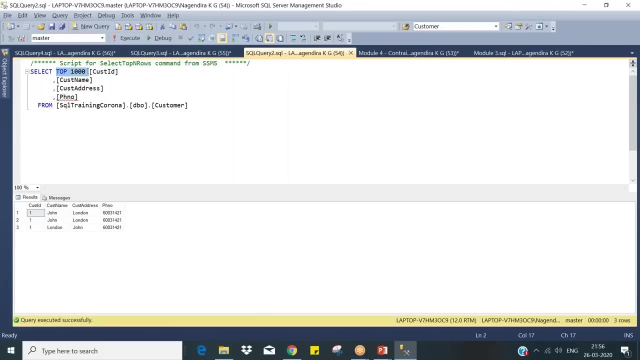 combination to create a record. i mean to identify a person and then, after knowing the name of the customer or the type of person that you'reréfusing, then i will label it and like, if i need nowadays a certain item, a particular department, i can add it and i will do that. you can include a name or a different. 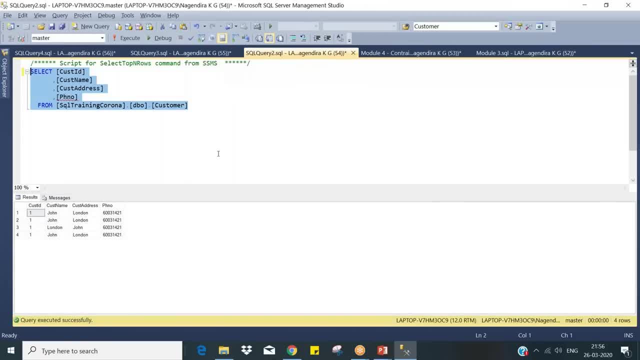 username so that i can easily apply a name to it. i will not need it. you can see every zettai line can open every domain and design and upload content in it. and there are others house decisions. you know there is like you work in if you are not оф shipper. 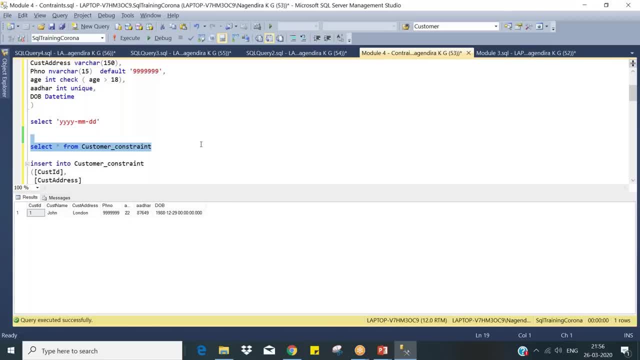 sunil, warun or raga. it's a regional name. it will be common, or some in case of arabic countries like muhammad is a common name, so you cannot create a primary key based on the name here. you see, you have a customer id defined, okay, so customer id is there. customer name is there. 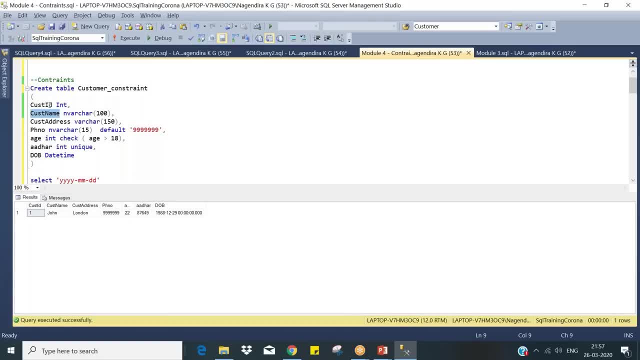 so customer id is nothing, but whatever uid you generate, if i don't have this guy, i have only name. so the names are so common everywhere, so how you can distinguish that one? it's like: just give me a minute, i will drop this guy again. drop table. 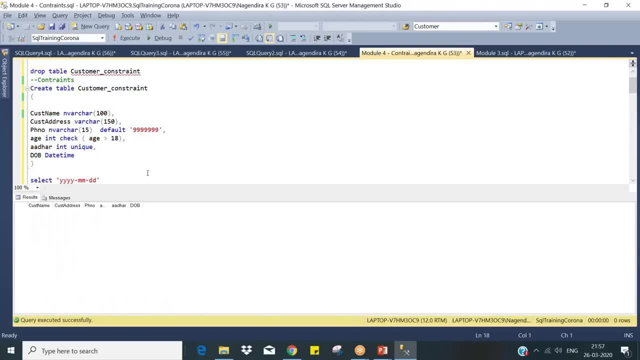 okay, what i'm trying to explain here is the purpose of primary key. so i have a name, a customer address, phone number, other. now you, in case of uh, even a person, have multiple phone numbers. how to handle it? i, i hope everyone has two to four, four, four, four, four numbers. so can you repeat the record? no right, 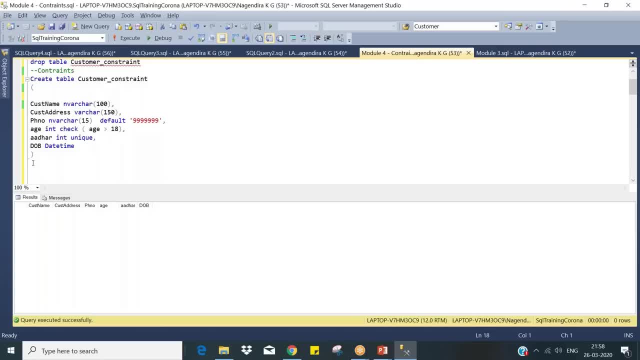 okay, questions about: please think now, what is the primary key is like? a primary key should identify a, a record in a table. if you want a uniqueness to be maintained in your table, that key should be: identify that particular record. once you give that primary key, then that record is for that. 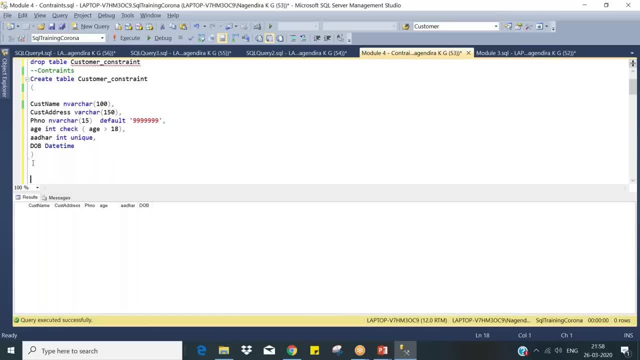 there is no duplication. it is a unique key as well, internally. okay, that is the definition of your primary key. so, in case of customer name, uh, you, what you need to do is like, you need to have, but you cannot have a unique name for the customer. it will repeat: so you need. 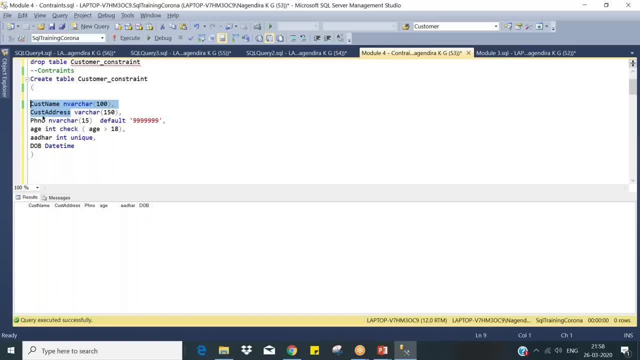 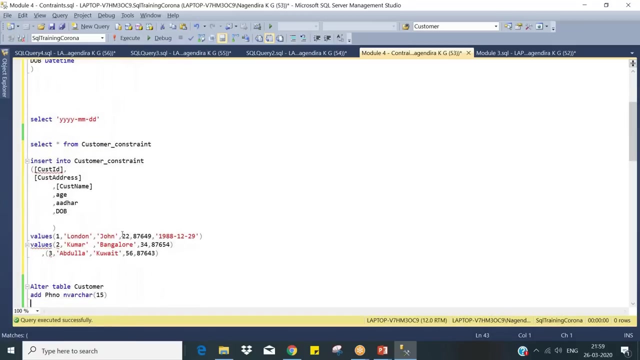 to add two possible combination: combine these two columns. he cannot be. I mean, a person from same street does not have same name. okay, you need to find such a combination. then you create a primary key. I hope somewhat little bit confusing, let me create and show it to you. so here, instead of ID, I will replace: 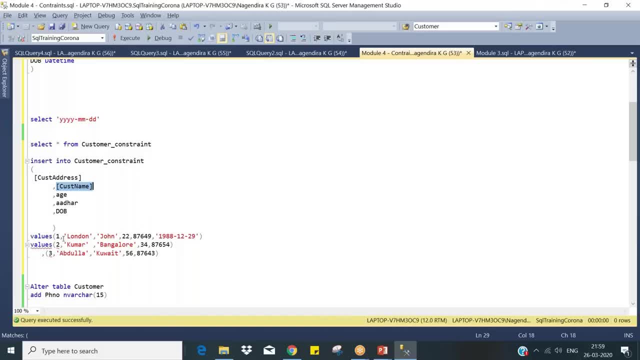 customer name: John is the. it'd be here. the order doesn't matter, since I mentioned customer name here: visiting. okay, I'll copy this guy, put it over here. I'll put same data. but now you see guys: John, Kumar, London, John is London and Kumar is from Bangalore. okay, now I can. 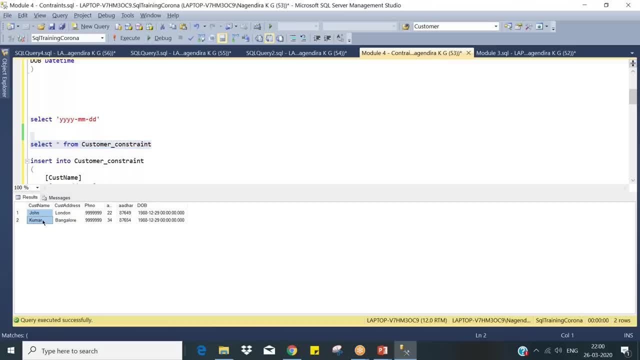 have another Kumar from Bangalore, okay. so what makes me to create a unique key over here is I mean if I use the primary key over here. is I mean, if I use the primary key, so now I can to create that action, now click on priority here and then say just: 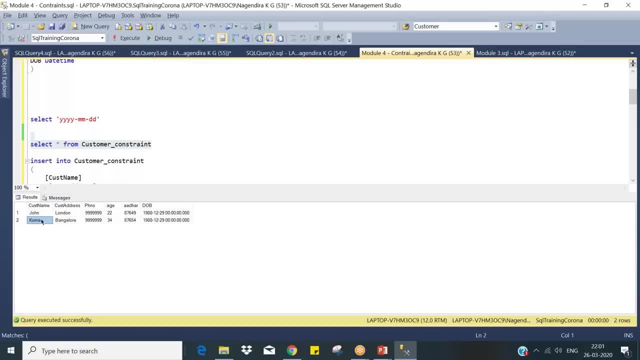 click on choose someone, so if that's you or another customer here. so now I am going to create a combination from present כा, my table up, so now I can create a combination of these two and create it as a primary key. now I say like I create a primary key here. customer name over here. 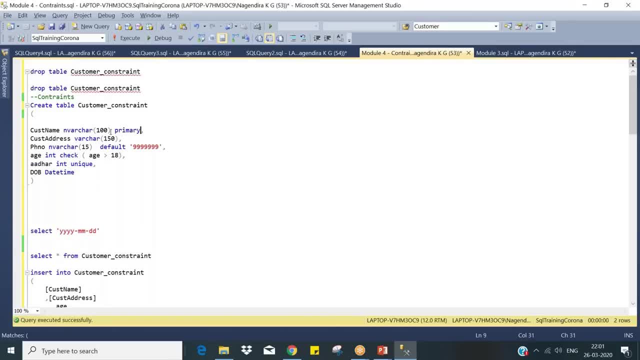 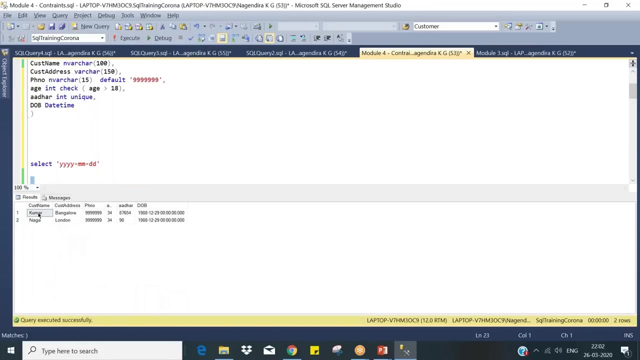 I cannot have another command, so I will create a combination and also a combination as primary. keep proper constraint, create table I've created as a primary key. so there is no difference once you create a primary key, no difference in the table structure and all of its same. and I insert a value inside Kumar. here I say like Naga: okay, now you have a Kumar. 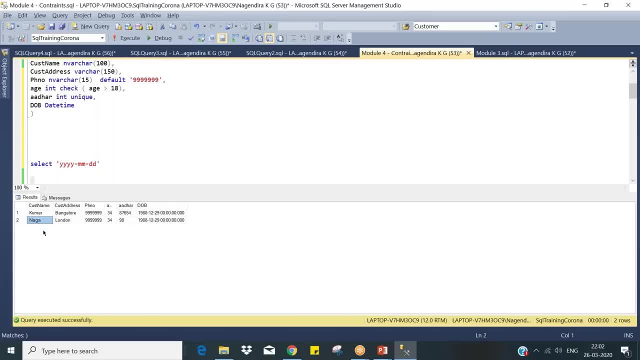 and Naga. now imagine I would I was. there is another Naga comes into place and he is from Mumbai. here I need to change this. says like violation of primary key constraint cannot insert a duplicate key in object. okay, so basically you need to have a primary key that defines if he is from. I mean just 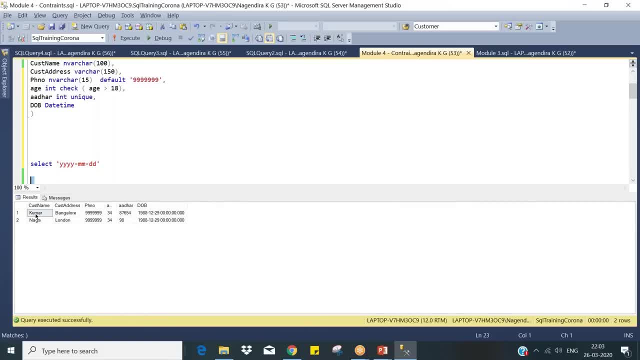 imagine you need to have a primary key that defines if he is from. I mean just, instead of this customer you imagine as an employee- okay, employees, you can have a names as a unique values. and if you say that employee say, for example, in this session we have eight people, eight people have a unique name. no, just no. 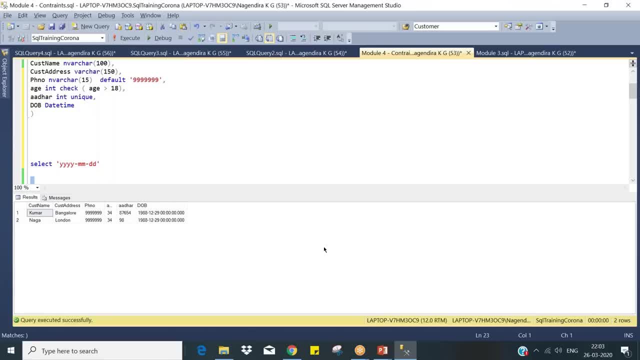 confusion at all. but if someone is having a name called Ganesh, Ganesh is joining from quite, Ganesh is joining from India. so what makes them unique? look, location: Ganesh from quite and Ganesh from India. so you need to distinguish Ganesh based on the location, so you will combine these two location. I mean a name and the location as 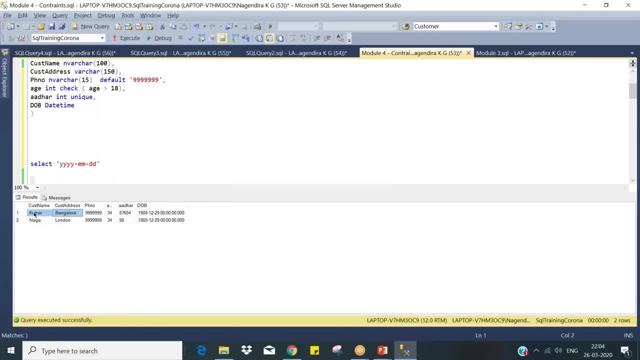 your primary key that makes you a unique value to identify a row. okay, simply a primary key. usually you think like only one column is considered as a primary key, using a name. now, if we, if username has different values like this: Abdullah, all other things, then no issues. but in practical world, okay, Abdullah Kumar. now you have inserted. 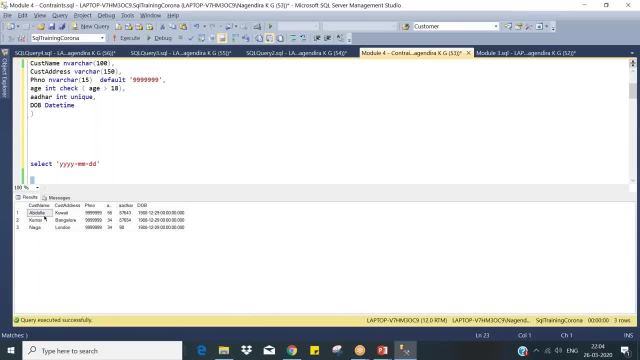 now, that is why people always have a customer ID generated got you. so, in irrespective of location, all this possible possible combinations I need to create. instead of that, what I will do is I will create ID for you, customer ID. then I will generate it as a primary key. okay, so that will identify me- individual record. so this is. 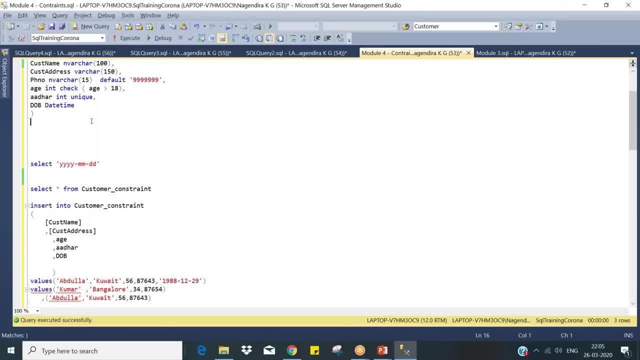 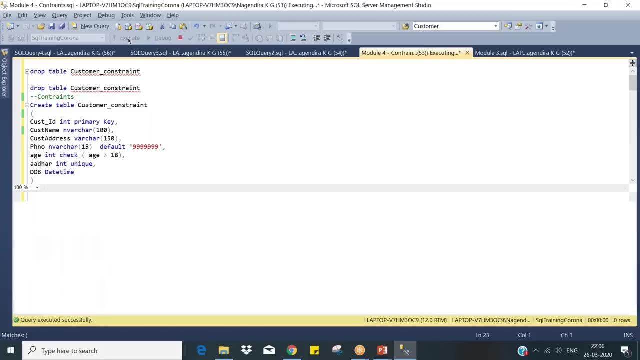 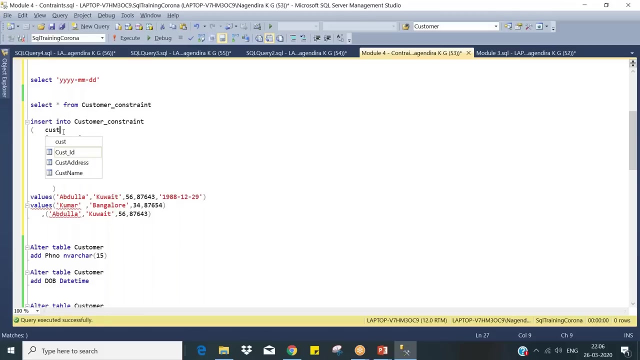 your primary key concept. now let me tell you what I am trying to explain: the customer ID. so there's no records. guys, I think damn silent. you are there, hello, yeah, yes, okay, any confusion, guys? are you getting the point what I'm trying to convey? any condition? no, you got what is a primary key. now you see my medical care. one, two. 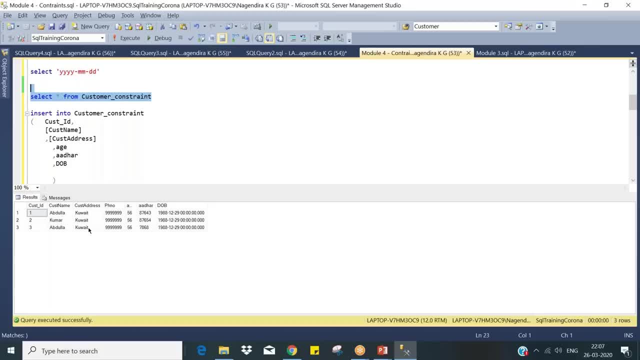 three. so now, instead of saying if i have abdullah abdullah here, it should be abdullah from bangalore, is like verifying it in another table, right, like that is foreign key or primary key. okay, see, now i am trying to insert four. okay, let me now wait. 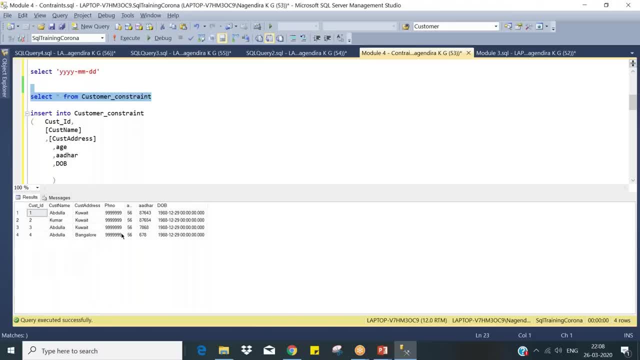 guys, as i told, i have three abdullahs here. okay, so what makes you to differentiate from this sub i have, if i created a customer id as a primary key, i will generate, i will have a logic to generate this one, two, three, four, five, and i will give this customer id to the. 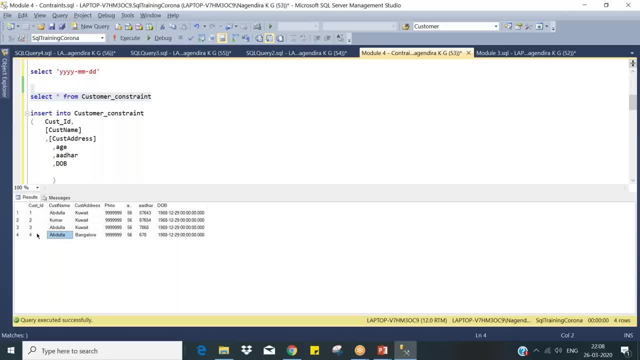 abdullah. always if you come back to my store you give me customer id or you swipe in using your card. that card is tagged with customer id. so all buildings will be against this abdullah. so i don't confuse with this abdullah that abdullah. i am at least bothered, okay, so you? 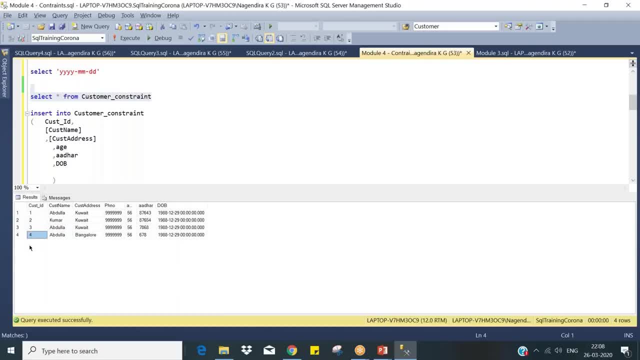 need to generate a primary key to identify a record. so this four is your abdullah bangalore. it doesn't matter whoever abdullah here, it is okay. that is the main purpose of your primary key: how you will create based on the combinations you choose. are you new customers? they come, they create a new record that will have auto. 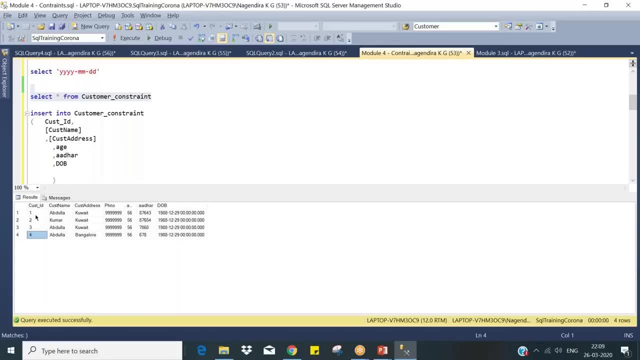 incremented values. that i will explain it later, later. so this is your primary key. now i say for is abdullah bangalore? even abdullah can be from kwai, but which differs him? other car differs sim. so it doesn't matter how many abdullahs, whatever data does they have? 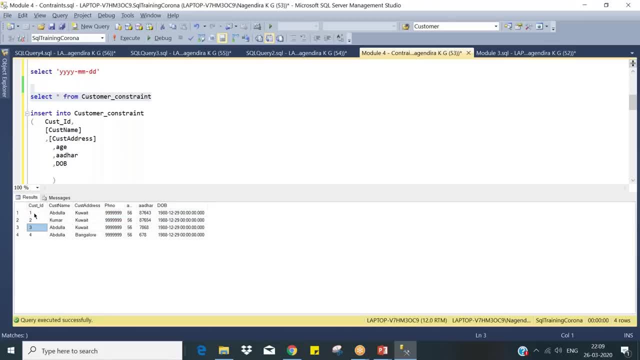 I mentioned only the primary key. so primary key purpose is to identify a record in a table. okay, any doubts? is primary key always unique or we need to specify unique? yes, that is why I asked a primary key. but I mean when proven answered he said, like primary key is used to identify a table record and it. 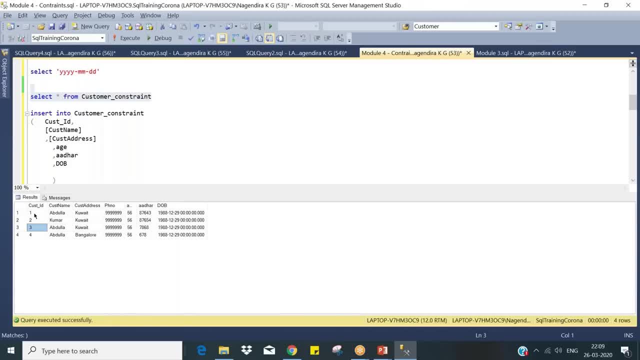 is unique. then I asked: what is the difference? that is why he can't able to answer. so this is nothing but the difference between your unique and primary key. primary key is not a unique. you cannot switch between both. I want a unique value. whether I can have a multiple primary keys in a table? no, not. 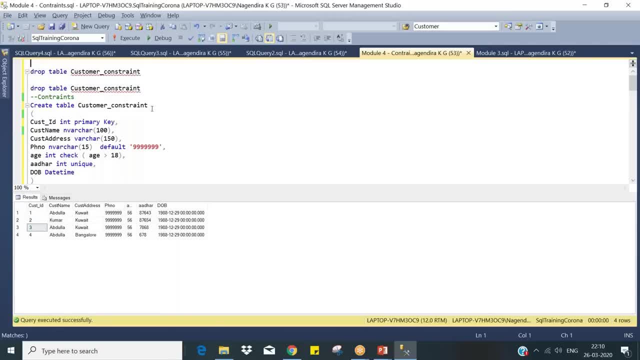 at all. you can have multiple primary keys in a table. no, not at all. you can have a single primary key. single primary key in a table that defines a record. okay, you can have a multiple unique constraint. say, for example, either I have a unique and phone number I have a unique instead of default. I can also. 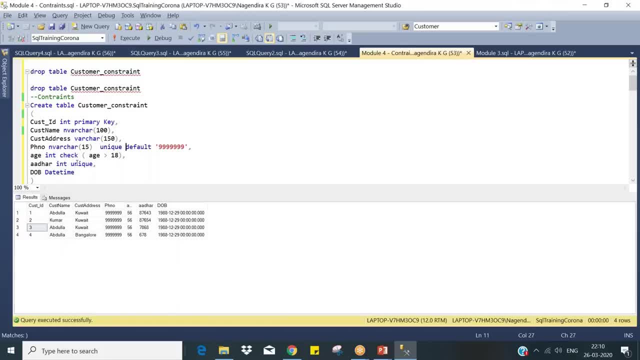 have a unique, unique phone number. okay, so multiple unique key constraints can be applicable, meaning like unique is for a particular column and your primary key is for the entire table. yeah, this is what is the main constraints and primary key. all those things so far in key. we will take it tomorrow already. we. 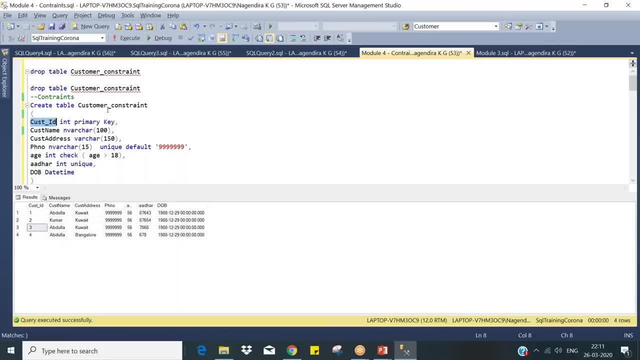 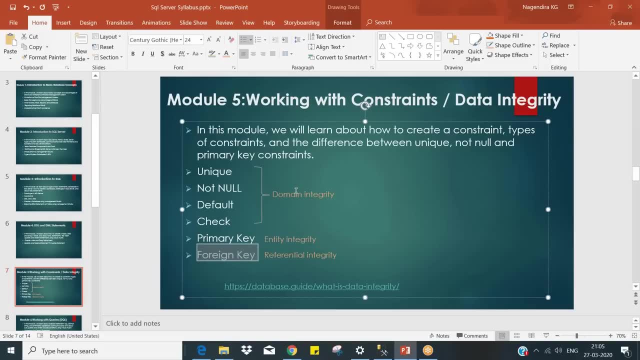 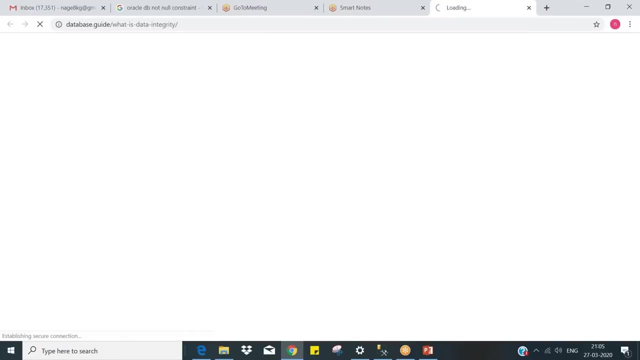 are 10 minutes over time, so with this we'll stop. today we focus on foreign key and before heading to foreign key, so what are these things? says like it is used to implement a data integrity. so what is says data integrity? so that our definition says like it is used to. 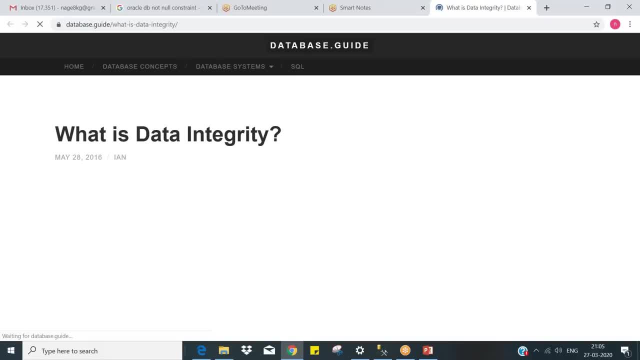 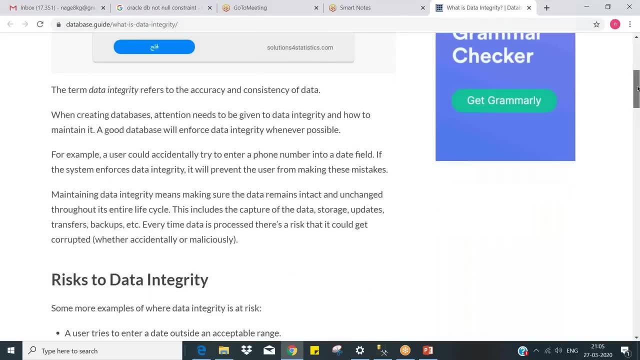 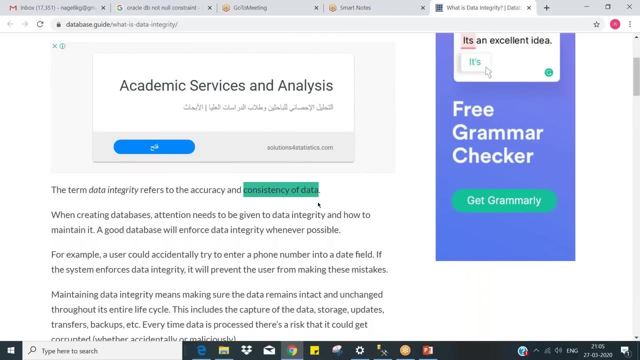 maintain some data consistency or relation between the data's like that. so the definition is like here. so it refers to accuracy and consistency of data. see the consistency in the sense: once you have a primary key and your check constraints, so your data will be consistent. otherwise you miss some kind of rules, if not imposed. say, for example, someone who 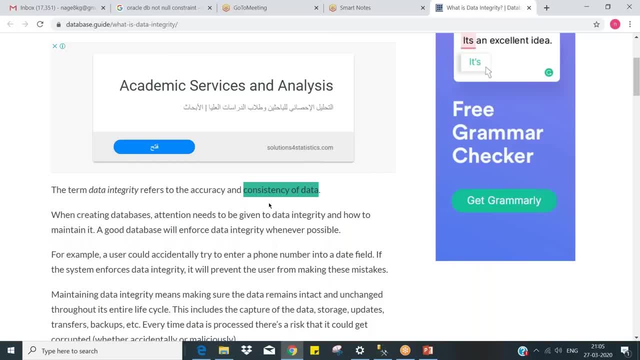 doesn't have any age limit, who are applied for college, then you will allow them to apply for the college. it is wrong. so you are imposing certain rules so that your date is accurate and your data, consistency of your data, is maintained. that is what a data integrity means. okay, so there are. 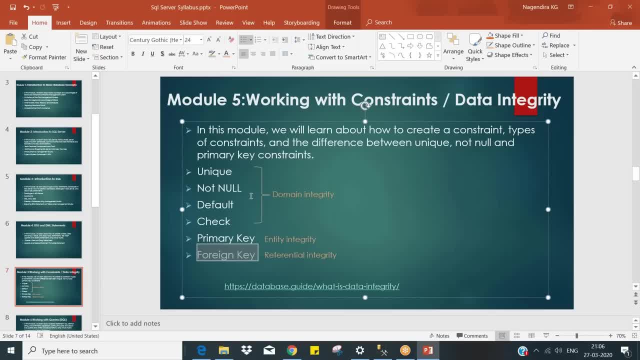 different types of data integrity, domain integrities, all these things use it to create for a column, particular column and entity integrity. entity is nothing but for your table, for entire table, you are maintaining a primary key, then foreign key. that just now I'm going to explain. I mean, I'm going to explain next. so 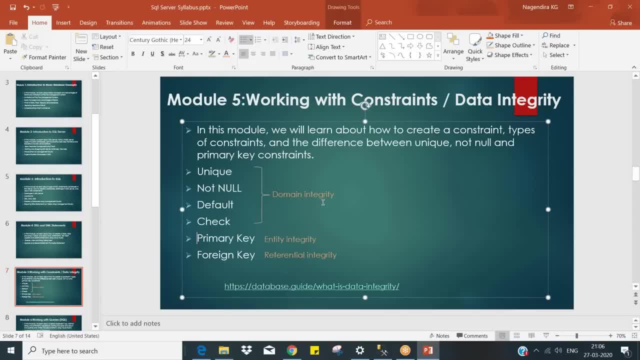 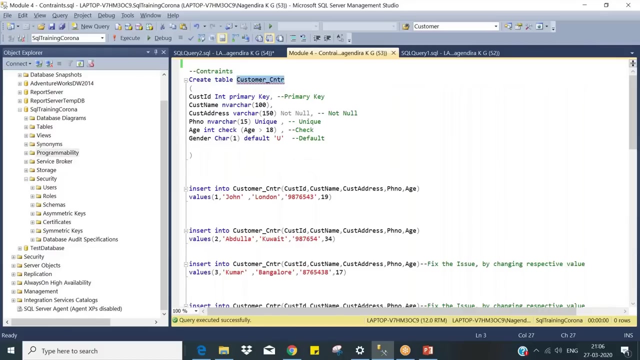 referential integrity. these are some kind of integrities, data integrities that you can construct to be able to achieve only in the database. all these things are challenging features in your file systems. okay, so with this, no, let us move on to foreign key. so we saw about these things like yesterday, we have constraints, all this. 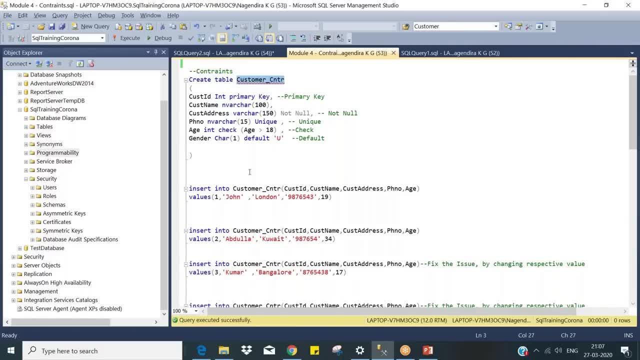 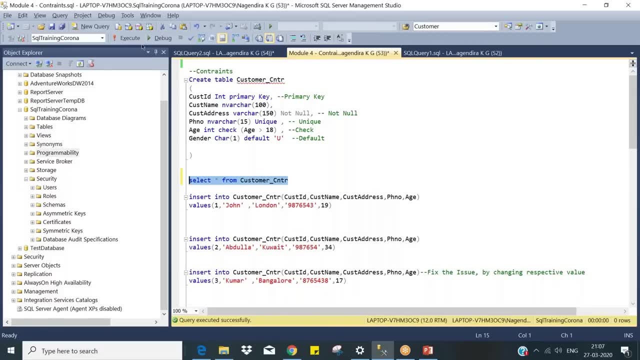 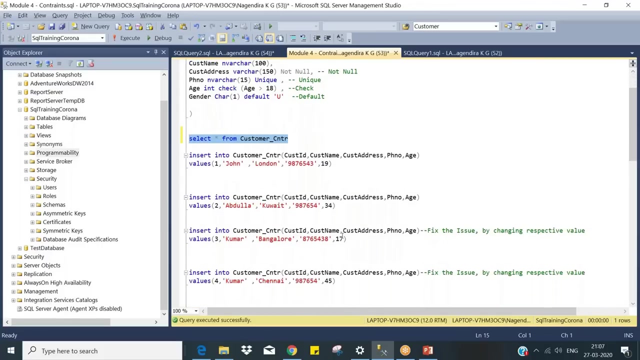 concerns primary key, not null. unique age limit, check and everything default. so whether this table exists because I work on some, something might be deleted, So we have a data. So, customer John London, this is the guy And I tried to to refresh yourself. I just trying to give you some fix over here. I mean. 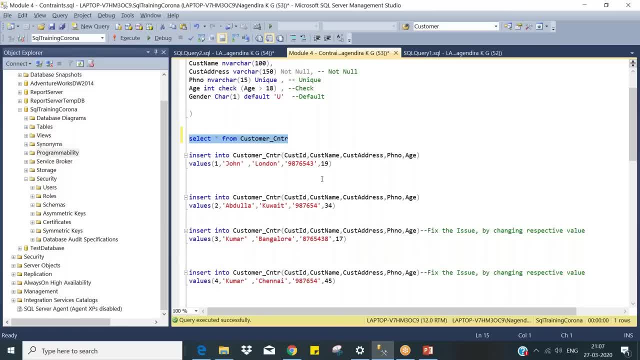 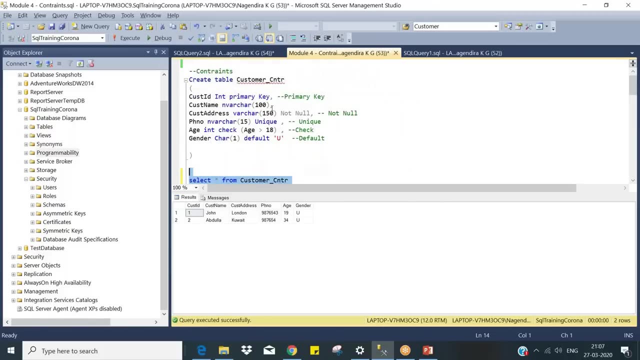 this queries will throw error and you guys have to answer it. Okay, So this contains the one record. I'm going to insert another record now. So this is also done. So two records Now you see. you just see the constraints once. Okay, Quickly, So address. 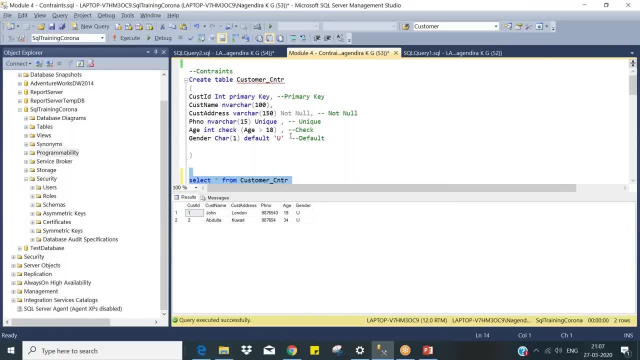 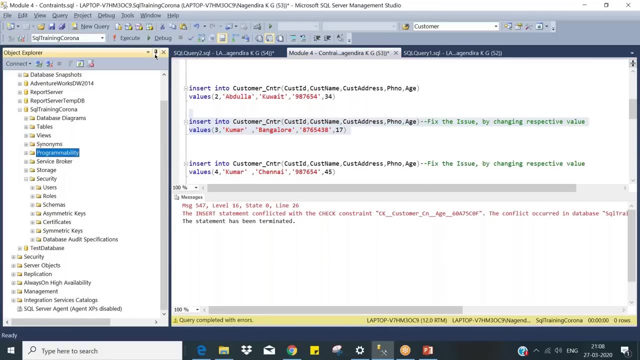 is not known. One number is unique. Age is greater than 18.. Gender is by default to you. So these are the constraints I have. Now this guy fix the issue by changing the respective value. I'm going to run this one. I will get an error. So what it says. 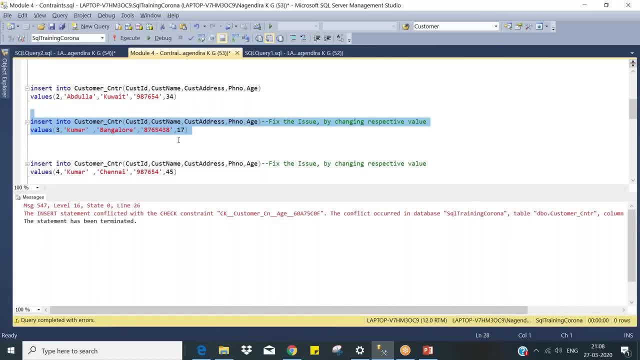 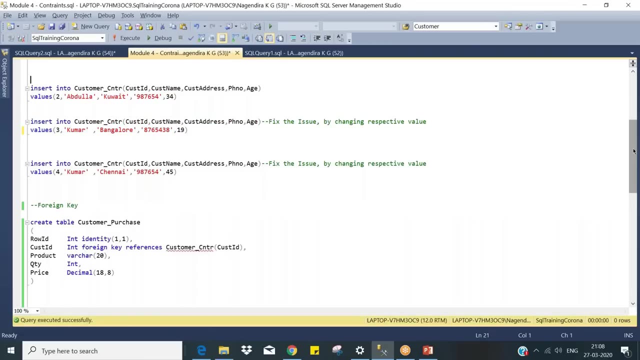 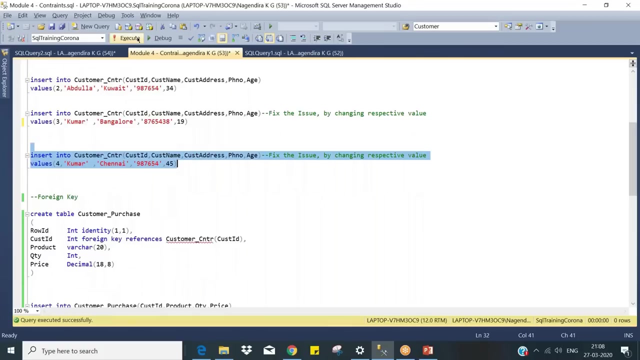 Age of age, Any age. So so throw out an error, So let us give it as 19.. Okay, Now you try to execute. Okay, So again. So this record will be inserted. no, fix the issue. by looking at the value itself We can say Violation of unique key constraint, That is: 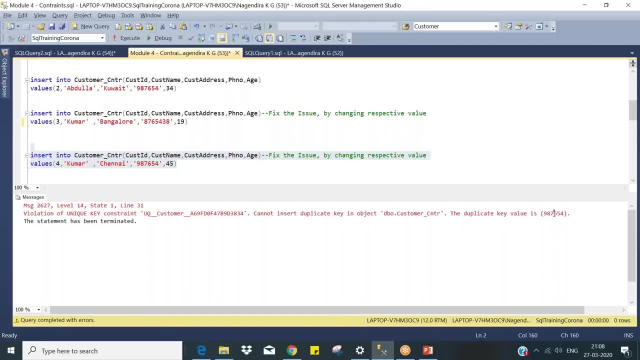 uh. insert of duplicate object, duplicate key values: 987, that is your phone number. phone number here it is repeated. so i put phone number already here. this guy already there. same phone number. when i try to insert it is throwing me error. so this is kind of integrity, data integrity you are imposing. 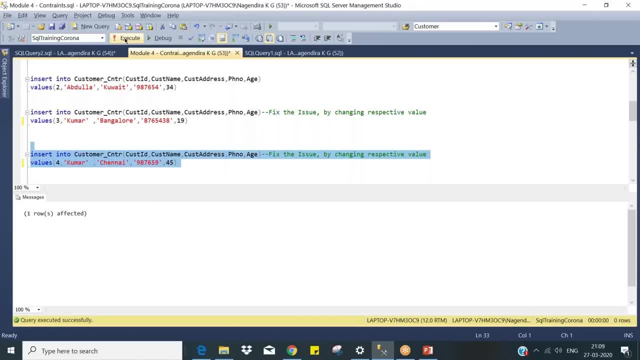 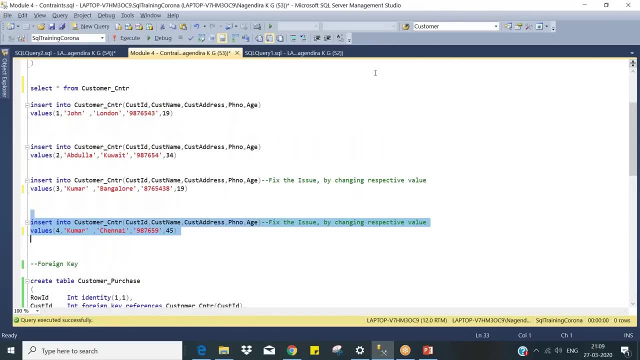 i just change it to nine. something else done. okay, now i have this, uh, customer table guys: customer id and name, customer address, phone number, age and gender. okay now, uh, what is the reference or foreign key? what is the purpose of foreign keys that you, you need to? 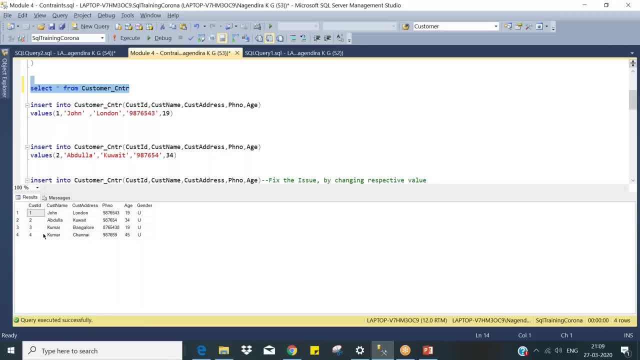 ensure that whoever is the actual customer, those entries only should be available in the other table, or those those valid customers should be allowed to enter in the table. so that is why you impose certain rule: whichever is a foreign key here, he should be the- I mean primary key here. this guy should. 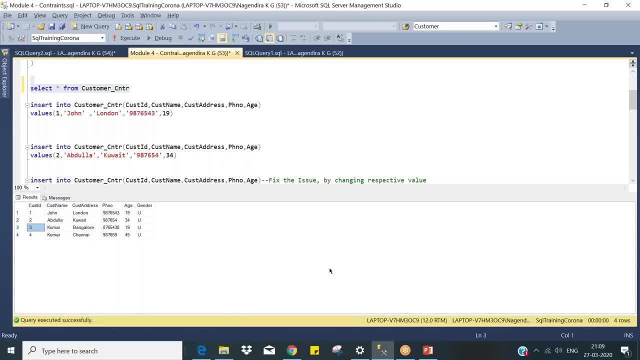 be the foreigner of another table. okay, that is a rule you are trying to impose so that your data is again maintained in the integrity manner. so I have another table. say, for example, I have a purchase table here. okay, so this is a customer and I'm having a purchase table, like you are. 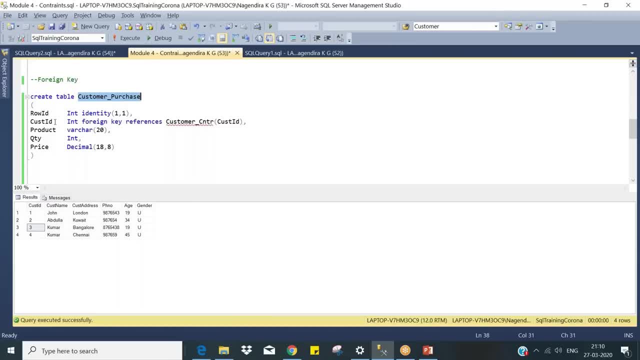 going to a supermarket purchasing some items, okay, so what I do is like I need to track bill. that will generate a bill. now you have a he. this customer is nothing but all those guys. okay, over here. customer name, so I don't need to maintain the same. 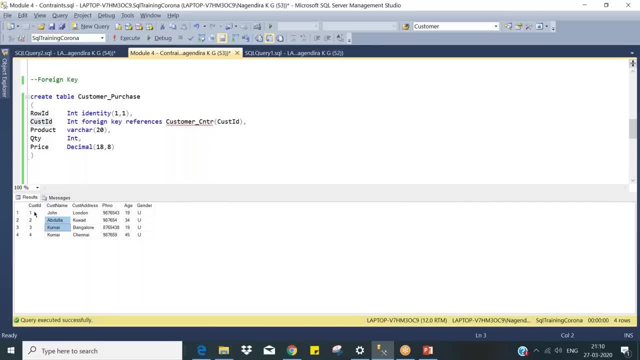 information over here in the customer purchase table. just I will refer the customer ID, then what? whoever purchases in that particular bill, I can refer its location, phone number from another table. that is customer table, customer constraint table. this is the consumer constraint table. so whatever you are seeing here is nothing but your customer constraint table. I am going to create the. 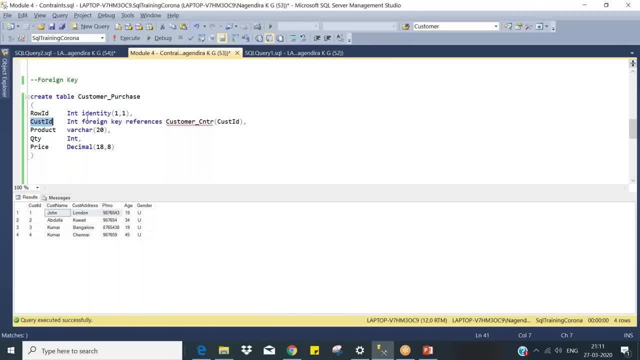 new table: customer purchase. okay, with the customer ID referencing to the customer consent customer ID. let me create it okay. I already created it okay, so I'm trying to insert the records. it was affected. now let's see both the tables together, so let's start from customer constraint. 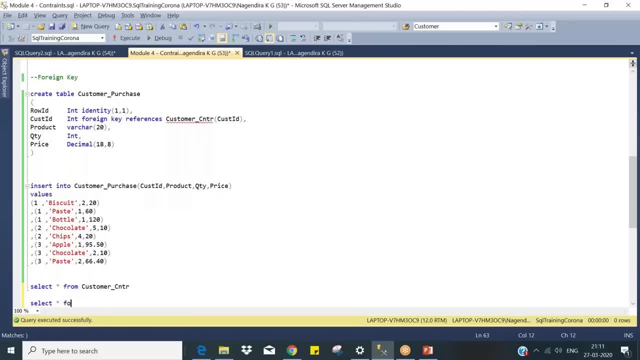 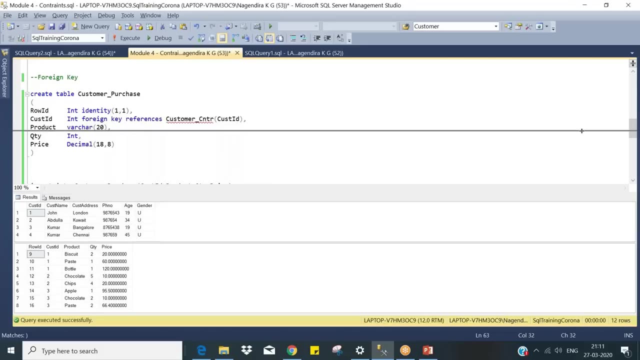 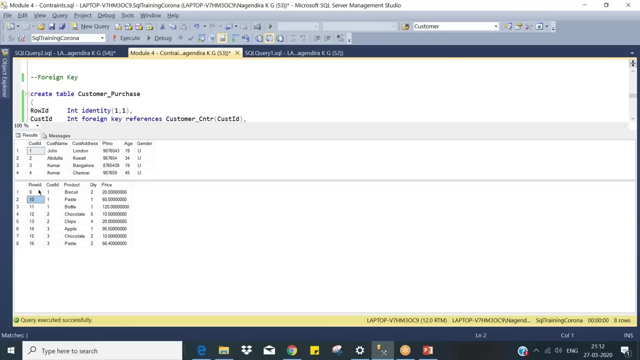 from customer purchase. now you can see from this table. so this is the customer master table which is having a customer information and this is nothing but assume. it is something like serial number, line number in each will you have some number? so what it says like says John, what indicates: john don purchase biscuit paste and bottle and 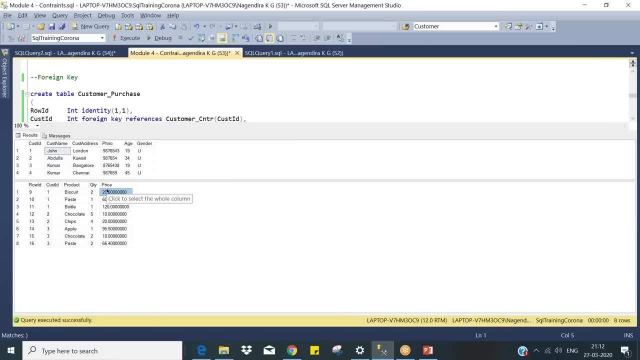 he purchased biscuit paste and bottle. he purchased list blessings and bottles and he purchased ice cream, oradı, and he purchased two quantities of biscuit, and which is having a unit price of 20, and paste 60 piece, body, 60 piece. So these three rows belongs to John. Okay, next two rows. 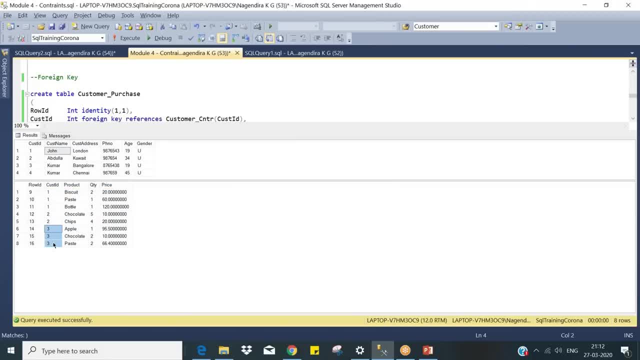 belongs to Abdullah And these three rows belongs to Kumar, from Bangalore, not from Chennai. Okay Now, this is a customer ID having a primary key here: unique information that is for a single record, but I mean single record per customer, This particular row. 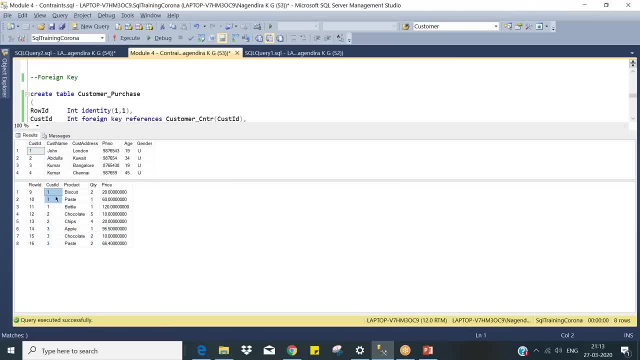 and for this customer. but here it is repeating. Okay, So from this you can see like foreign key and be having duplicate, or it can have multiple values. foreign key, Correct. Now what is the main advantages of having a foreign key? As I said before, you cannot have a customer. 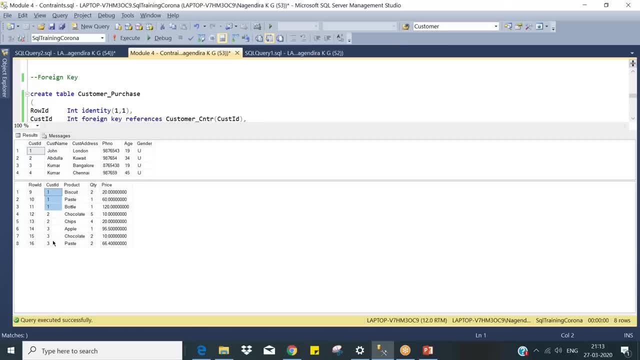 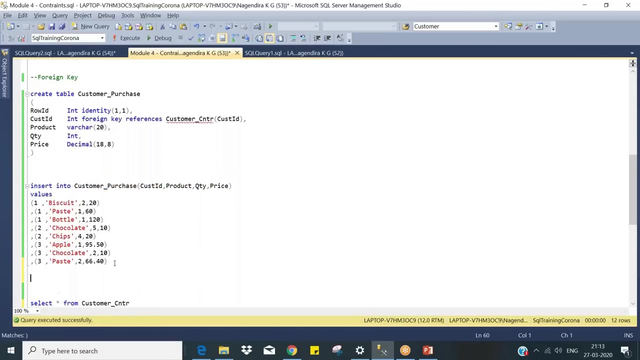 ID Five. Okay, You cannot have a customer ID here. Okay, in this purchase table. Okay, without having the information in the custom master table. So let us try to insert a customer ID five in this table. Okay, then let's see what is the issue happening. 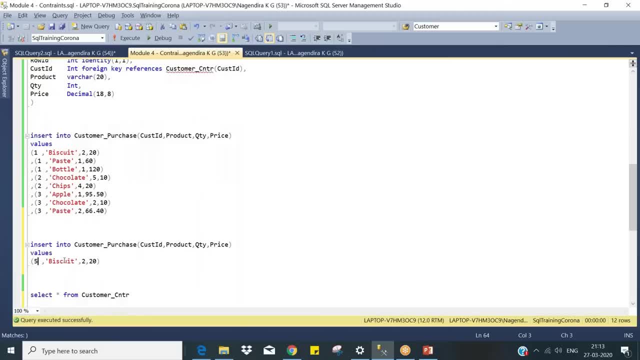 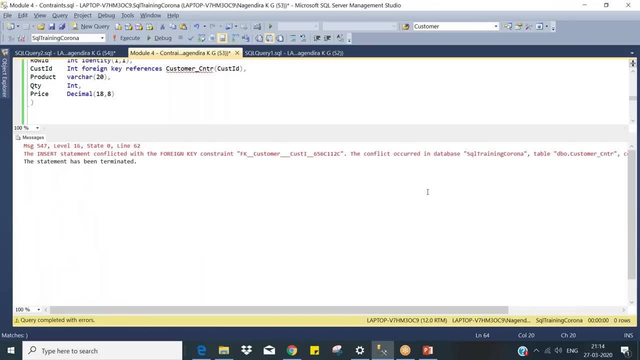 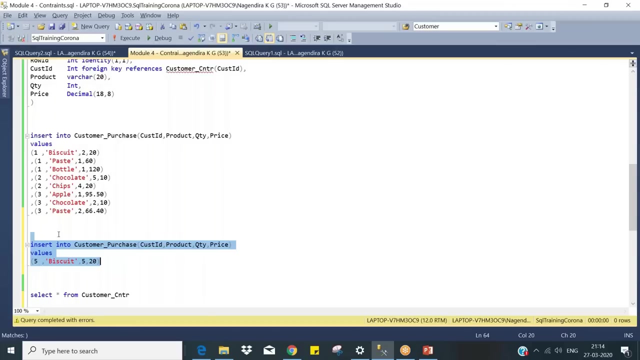 I say like customer five: Okay, He is purchasing this guy, Let it be three items, Five biscuits He is purchasing. Then I try to insert it. It says, like the insert statement conflicted with foreign key constraint. The conflict occurred in the database, Okay, in the particular column, customer ID. So what it does is that. 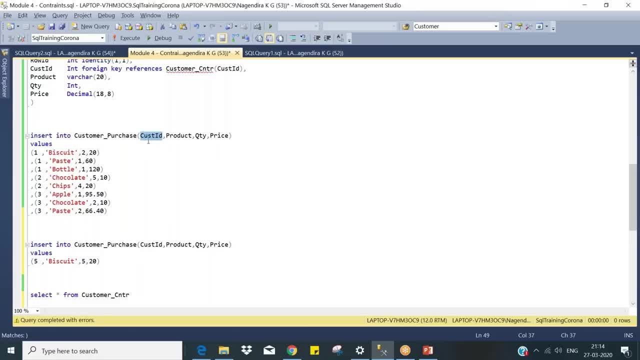 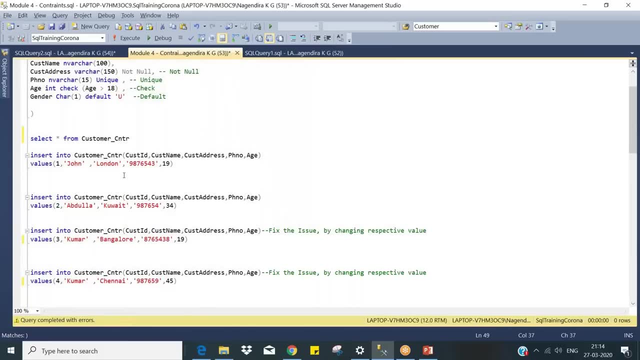 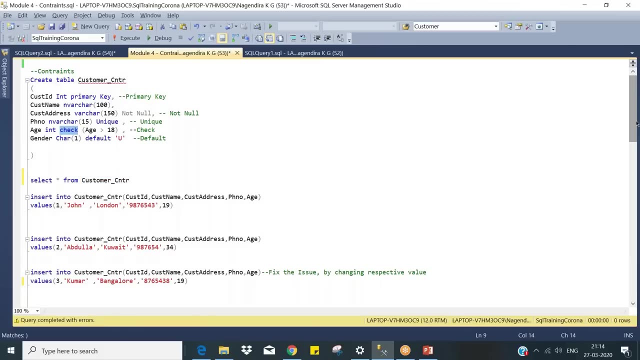 each time when you try to insert a customer ID, foreign key column, it goes and checks in this particular table- Customer contract. That is primary key- Whether that value exists or not. It does something like a check constraint. Okay, It is like checking each time when you do a insert whether 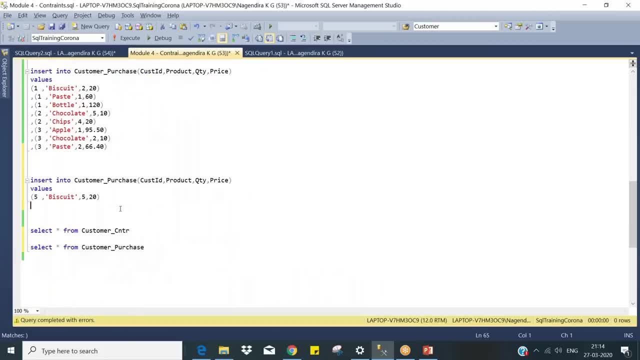 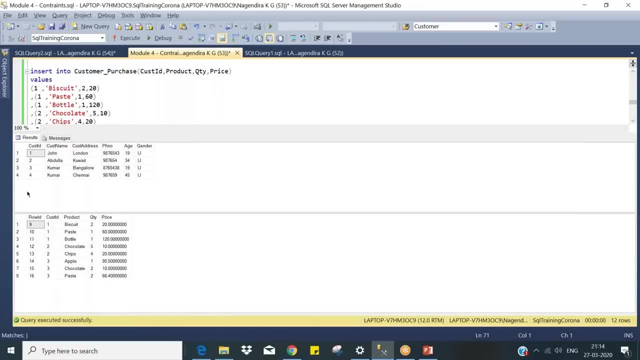 that value already exists in the primary key table. So let us select this guy once again. Now you do not have a five here. You can't able to insert unless you have a value in this customer master table. So let us insert a customer ID five here, Then we will try to. 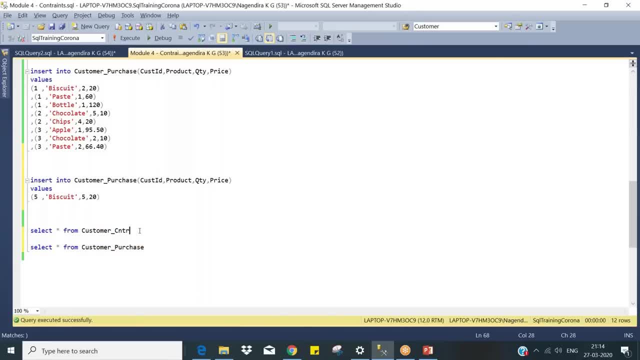 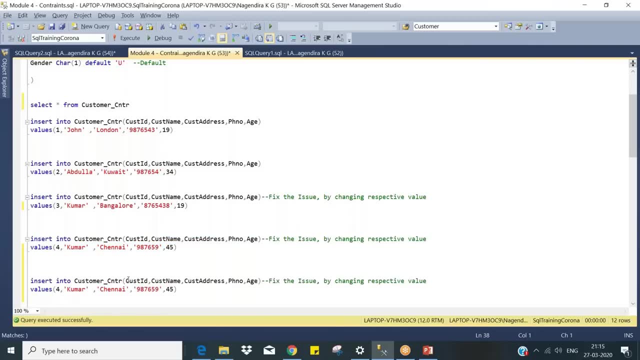 insert here, Then what happens. We will check. So we will take customer master customer control. I will have this. I will put it under: Deepak, from Chennai. His number is 67890 and his age is 32.. Let us insert him, Okay, Okay. 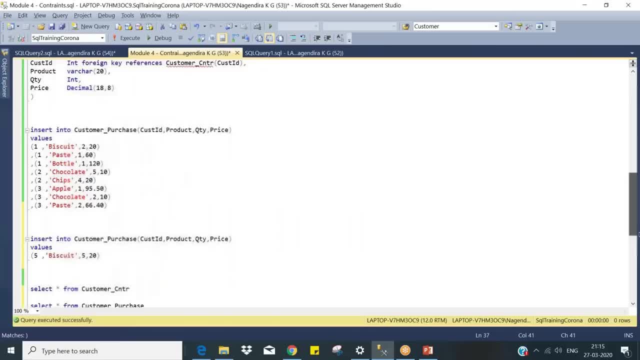 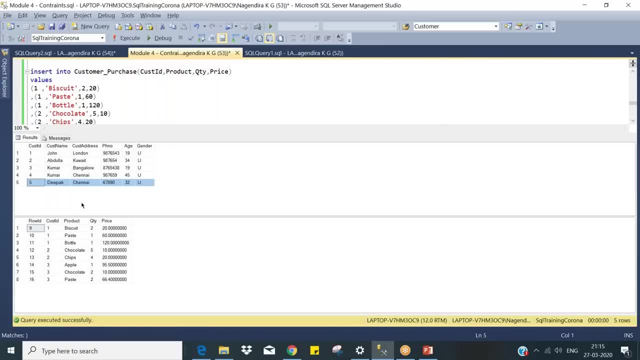 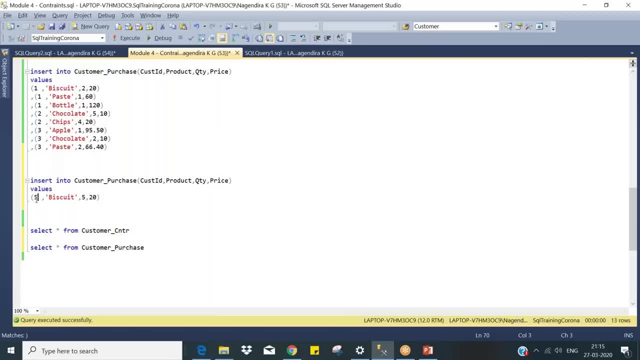 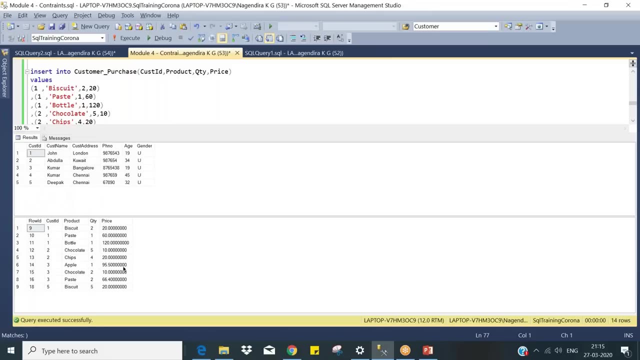 in the purchase table he budgets to. I mean customer ID five, purchase biscuit five, and each cost to 20.. Now I insert how it got inserted. Okay, got it guys. so without having a master information created, you can't do the transaction. okay, that is. 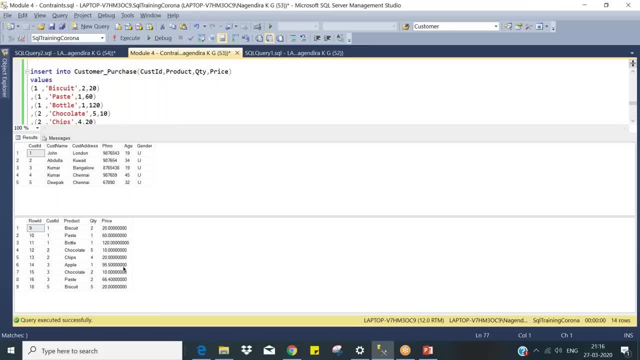 what, uh, the main purpose of foreign key, so why we need to impose all these rules to maintain the data integrity, okay, so that your system will be consistent. this is the thing any doubts. guys in this hello- the first one, john abdullah kumar- are from: yeah, customer constraint or a customer? 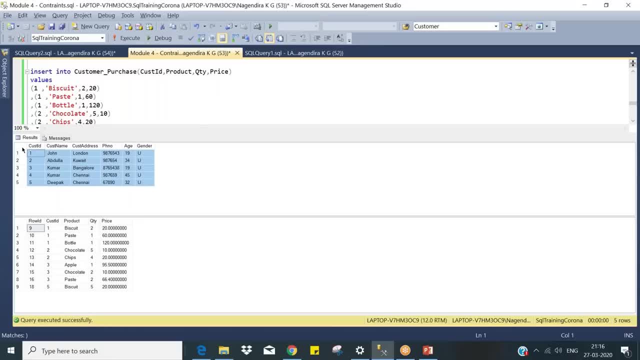 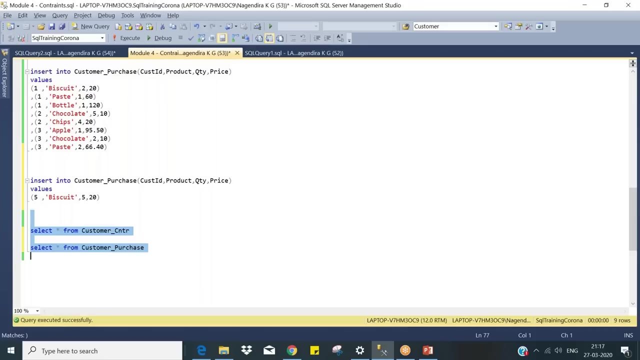 customer. customer. first one is you. you say like customer, interrupt customer concern. for now, you say like customer master: okay, customer master, master, okay, this is when you run this, uh, when you run the customer purchase, how this checks the customer master file, yeah, yeah, that that is what i'm saying. i didn't create, that is the purpose of 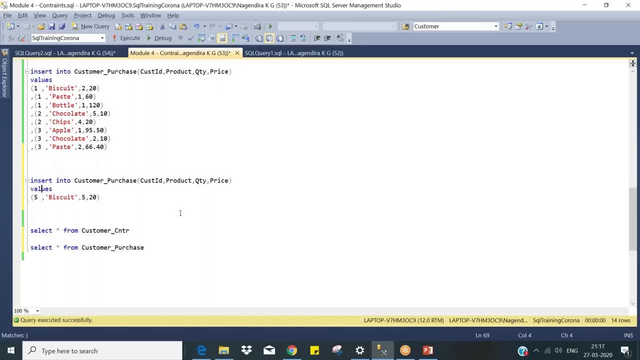 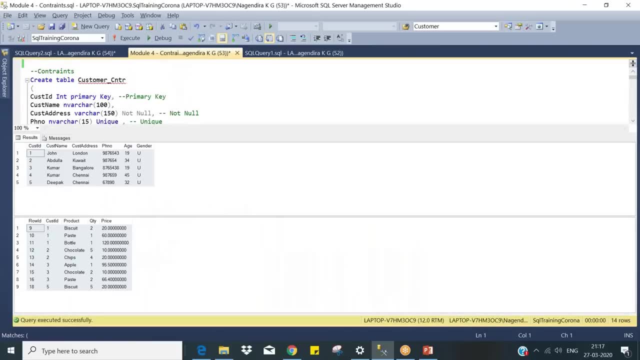 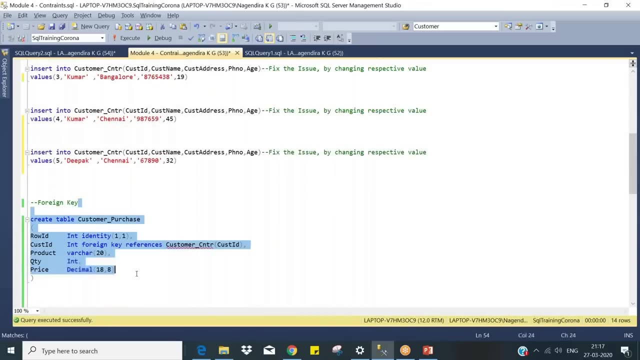 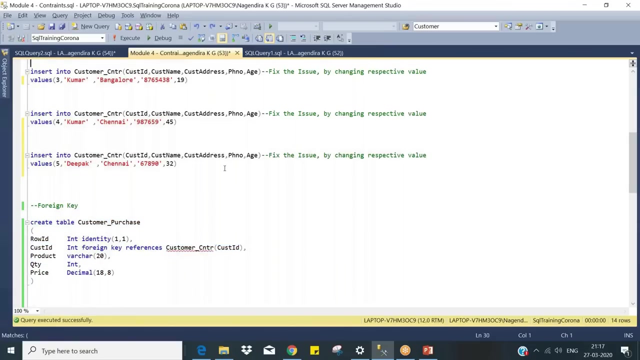 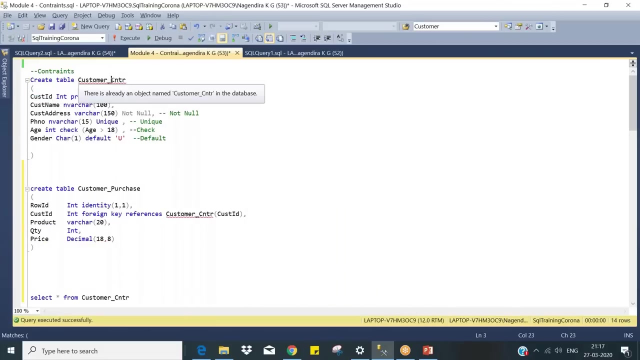 the dbms written program. they have written a program saying that. so that is what the definition says. you see, like, uh, here when you see the definition of these two tables, let me bring both the tables together: control, is it control c? so the checking happens internally. okay, that is the program written. so you see, like customer id in: 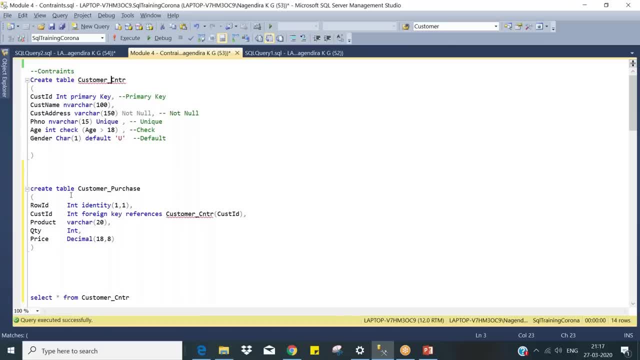 the customer master constraint as a primary key. now here, customer purchase table, i need to say this is the foreign key. foreign key always will refer the primary key of any other table. so foreign key references. i mentioned customer control, customer id, okay, okay, okay, fine, yeah, here you need to define. 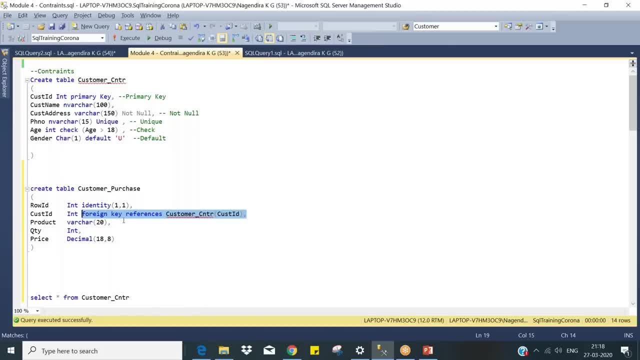 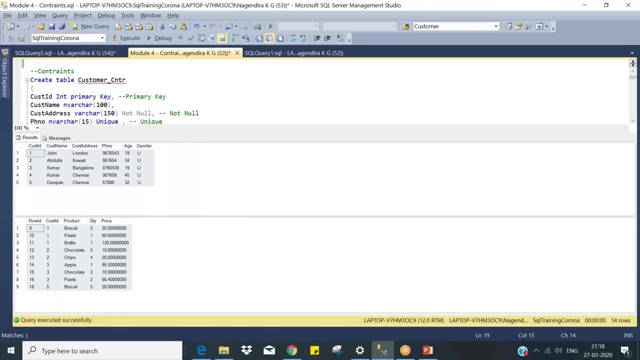 that is why i mentioned okay. so this is uh, this will be internally taken care by the tbms. that is the program it controls, that is the software duty to check. okay, okay, well, not in the customer. yes, yes, uh, in the customer purchase table, like you have given the warranty, like customer id. 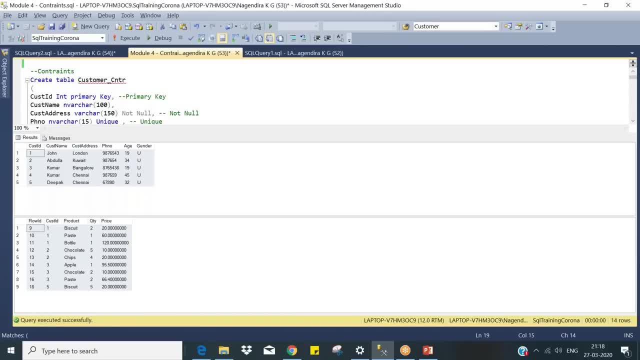 and it's a primary key, whereas if you have given like customer name one minute, so in the customer purchase table customer id is not a primary key. no, no, in the customer constraint it's a primary key. yeah, yeah, where have you given in that foreign key like uh? 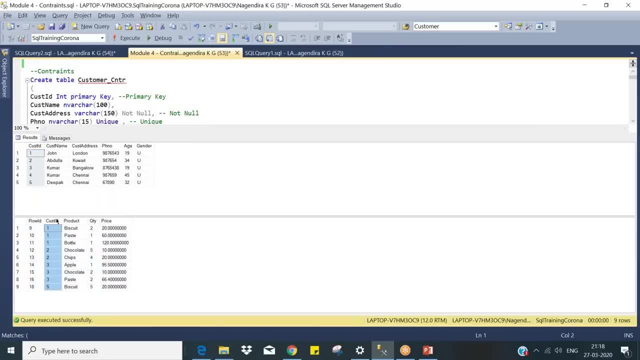 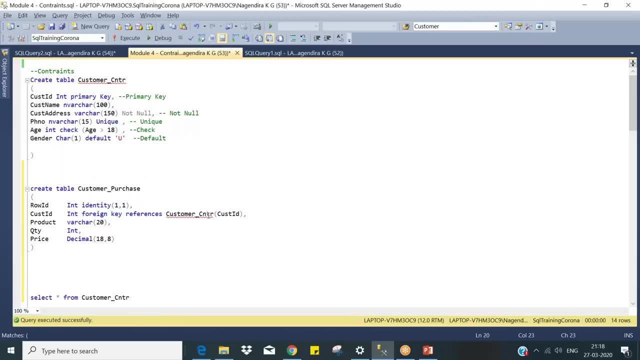 at last you have given the main ideas. so if i have given there the customer name like, that means it's not. it will not work right, it will not pick up. it will not pick up. see, there's your customer id. it will always reference to a primary. 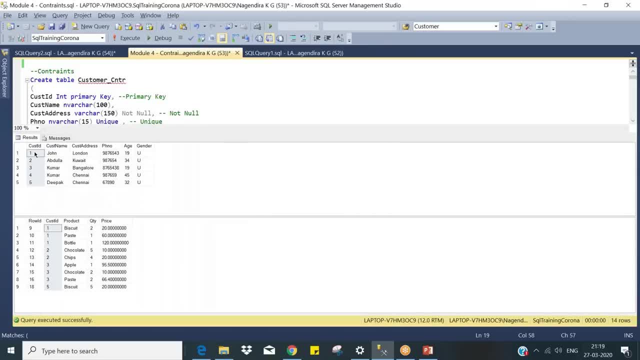 key only so you okay. whatever you defined as a primary key in another table, that column only you need to queue you. you can have a unique value instead of customer. you have other card? okay, that is fine. but whatever you define in this table as a primary key, that only you need to refer here. 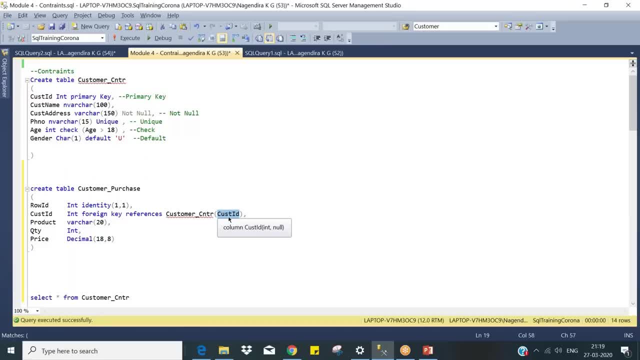 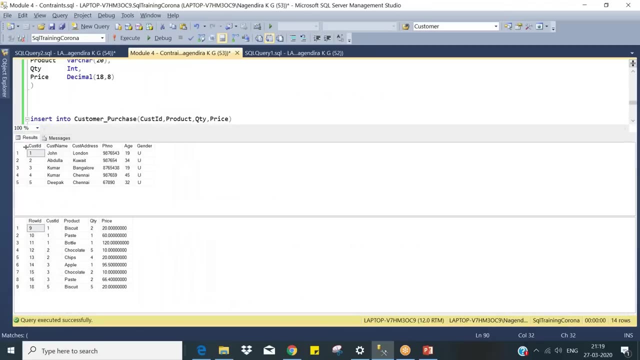 that is a thumb rule. there is no clarification. okay, okay, okay, guys. so the another important purpose is, like people always maintain, like the disadvantages of a file system, as i said. so assume like you maintain the customer information in this one file and the purchases in another file, what will happen if you lose some information somewhere? you are losing. 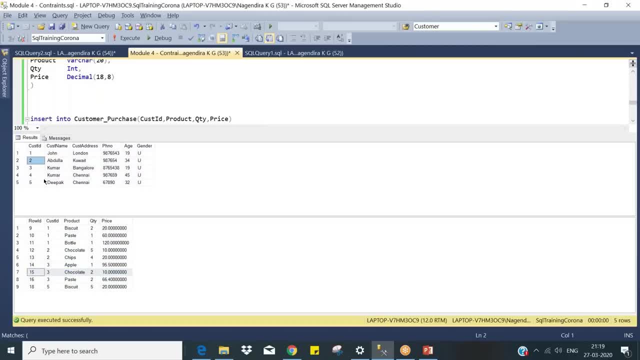 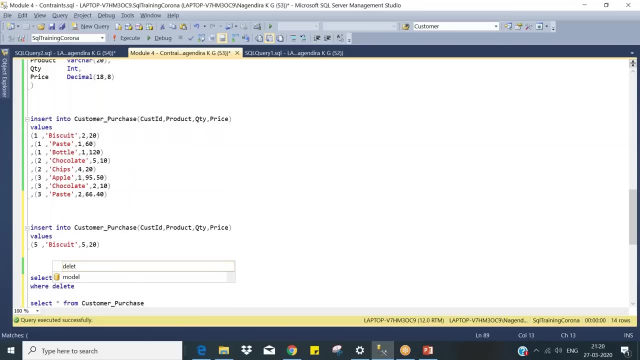 here or use it. you are losing here. um, let me tell you, let us uh delete this guy. try to delete the customer master kumar from bangalore. what happens? so any guess what happens now? who is that? please? okay, uh, delete from this guy customer id. so i, i want to delete uh customer id 3. okay. 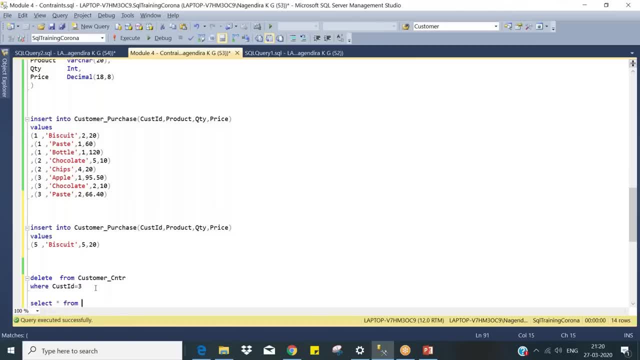 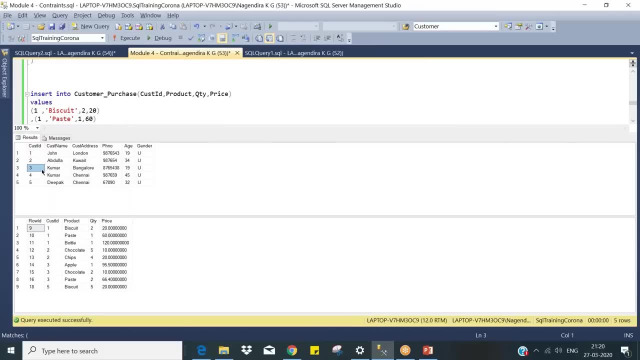 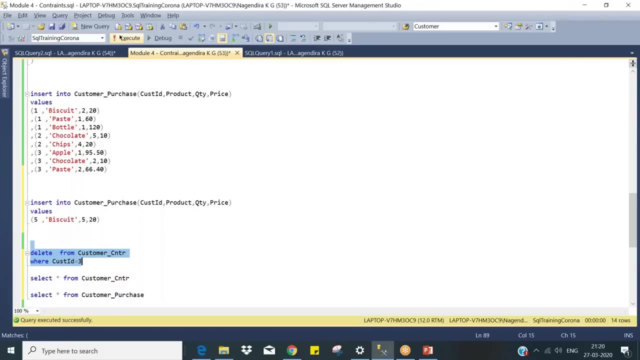 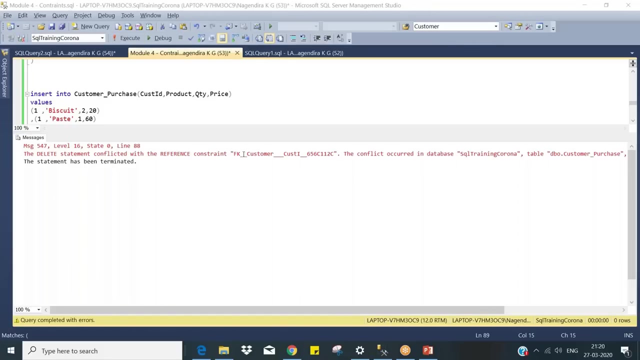 you see the data once again so that you it will be clear to you. so here i want to delete this guy, but this guy already have a transaction over here. okay, delete from customer master our customer constraint. it says like: uh, the daily statement conflicted with reference constraint- foreign key- because, unless you 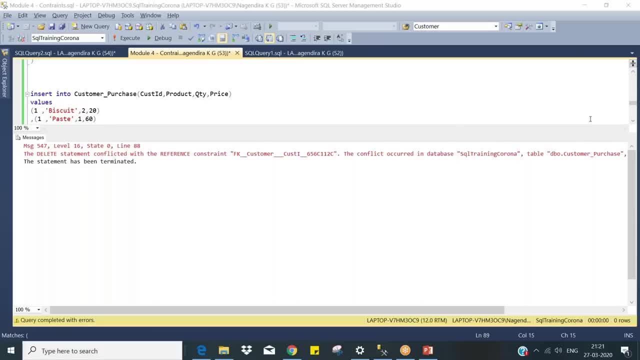 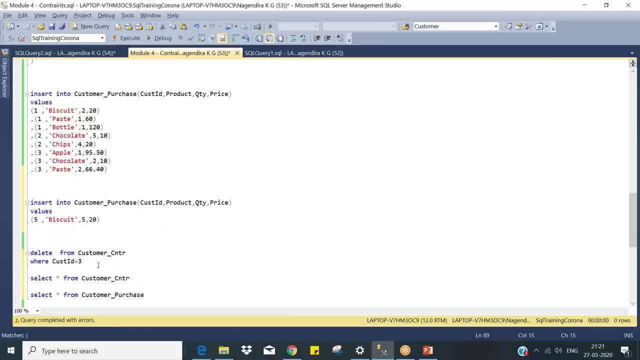 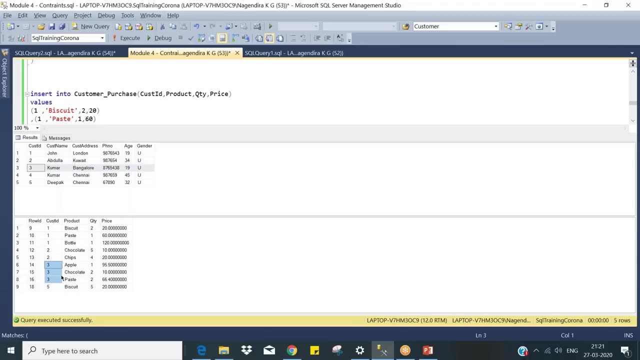 delete the related information, the foreign key information, the master information won't be deleted. okay, because once you delete this guy, this will not become any meaning because it always referencing this value. so when you keep on referencing it, okay if you, it will not allow you to delete. but when you delete this guy, then you 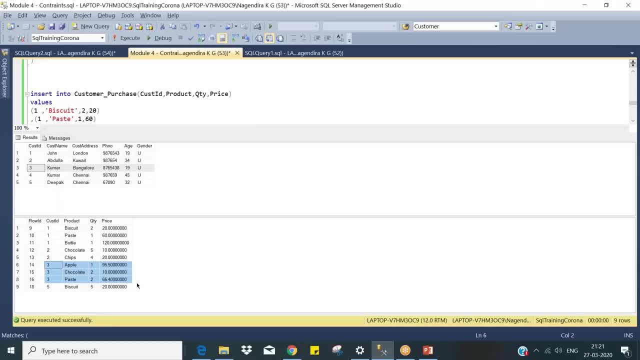 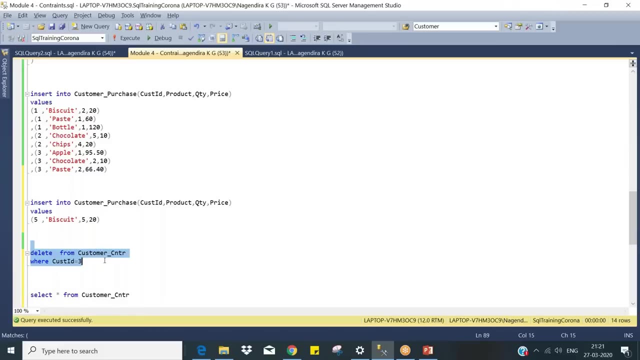 come and delete this guy, then it will happen. so always it should flow from this direction. okay, from foreign key you need to delete, then only your master information to be deleted. let us try that one. well, as gave one d that frying to fill this p, Joel, find why. 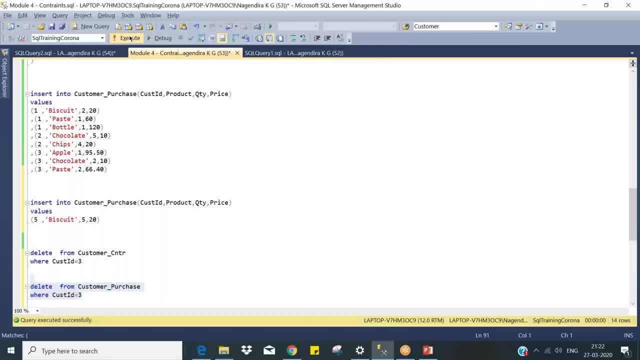 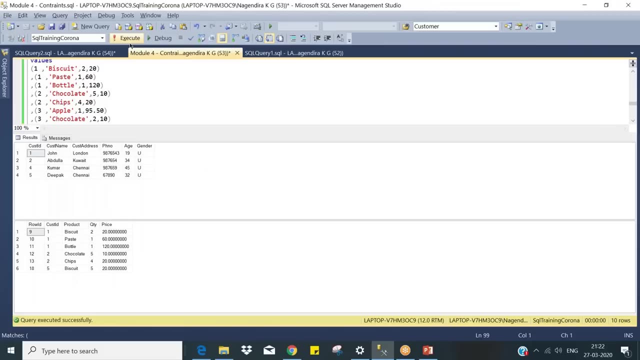 soldiers, customer purchase. now, when i delete from purchase, it will delete. then i when so earlier it throughout error. now it got deleted. so much only, yes, very much- will make you to maintain your data integrity. okay, now it got deleted, cleared off. i hope i'm clear, guys. so with this note, uh, we'll stop about constraints. let's focus, uh, more on. 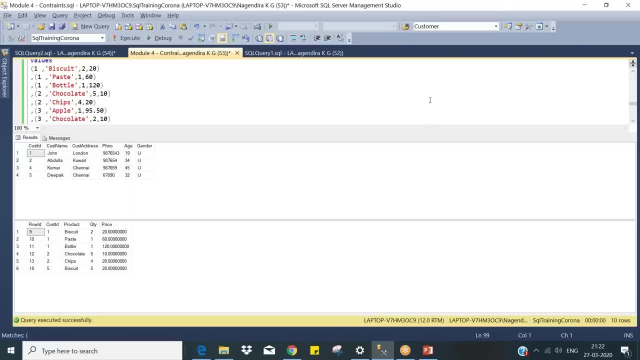 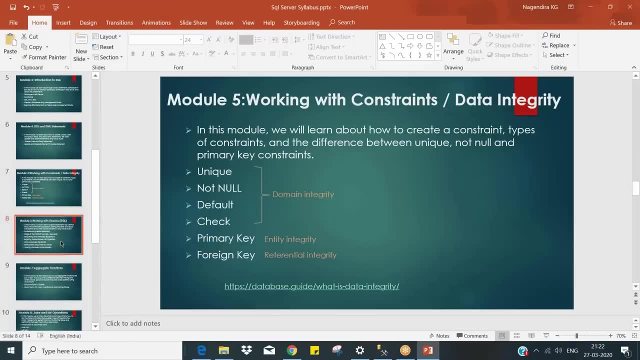 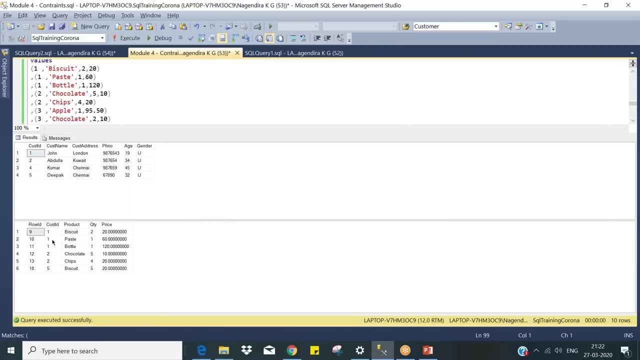 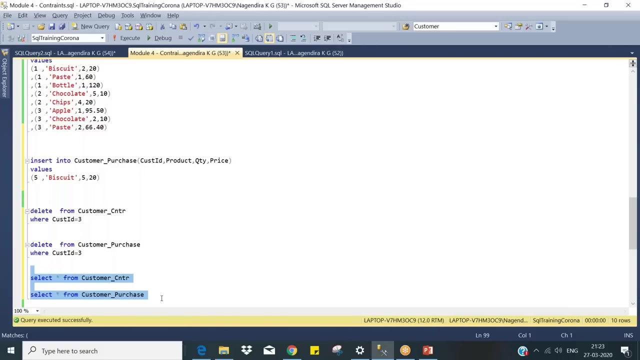 other models now. uh, you guys have any doubts? i'll give a minute and let's move on to next topic. so, uh, primary key. uh, in a table there is only one primary key can be, but we can include more number of columns. uh, we can add too many foreign keys? yeah, yes, in a single table you can have a multiple foreign keys. 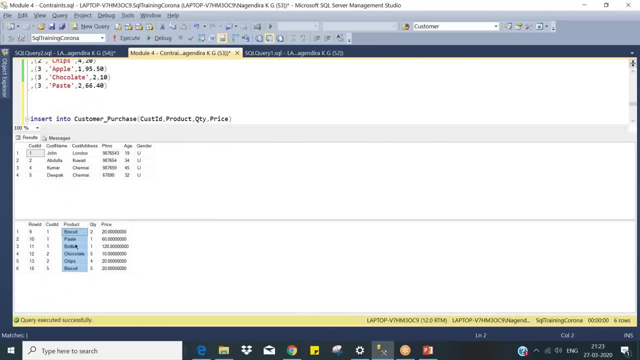 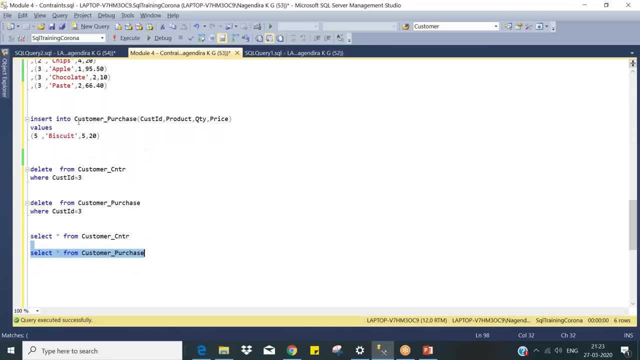 because your foreign key is nothing. but you can create this product, master. you can see that biscuit is repeated. that's why desperately put the biscuit two times so you see, like this customer also will purchase a biscuit, this customer also will purchase a biscuit. okay, so you assume you have another table for product. 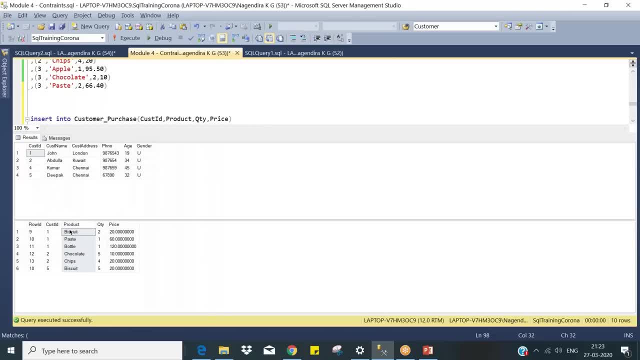 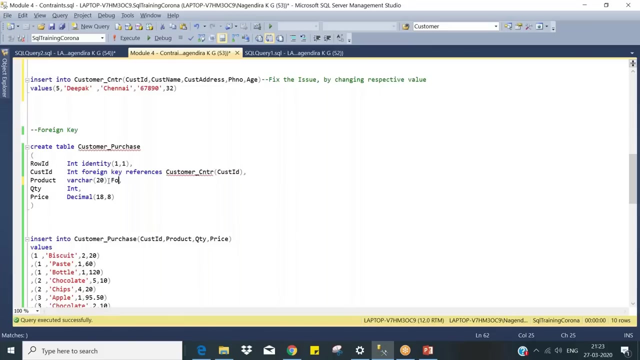 okay, and this product is maintained as- uh, i mean primary key, then you can have multiple foreign keys in a single table, no issues. okay, so primarily foreign customer id or phone number. yes, yes, exactly. so in this definition you assume like you have a another table, like product master. so here you need to define test foreign key references while declaring. 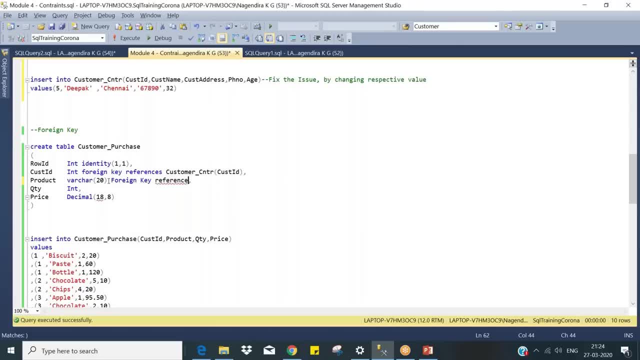 so these things, you need to be very careful while uh designing. okay, all these things comes when you're designing product master, product id or product name. okay, something like this. this table doesn't exist. that's why you throw here- now you see, customer id, foreign key references, customer. 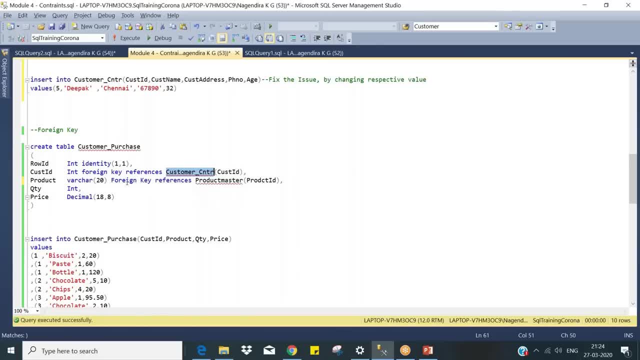 master or customer constrained customer id, product worker, foreign key references product master, productivity like this you need to define so as a. to summarize: a table can have only one primary key and the primary key can have multiple columns. and contrast, a foreign key will reference any of the other primary keys and single table can have multiple foreign keys. 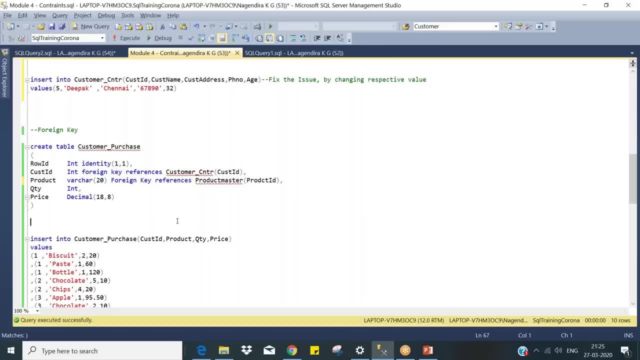 okay now. another point i want to touch here is: you see, like customer purchase table, i'm inserting only customer id product. and you see, like customer purchase table, i'm inserting only customer id product at quantity and price. okay, so each time when I do a insert, there is something. 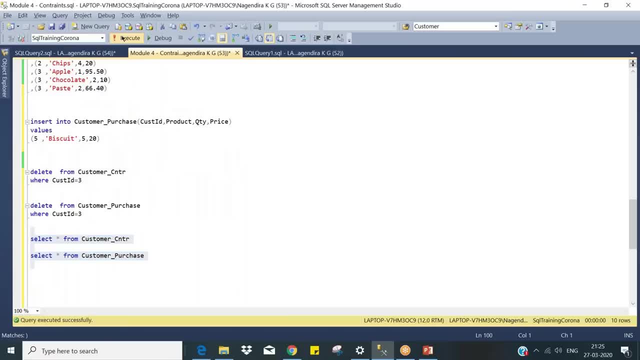 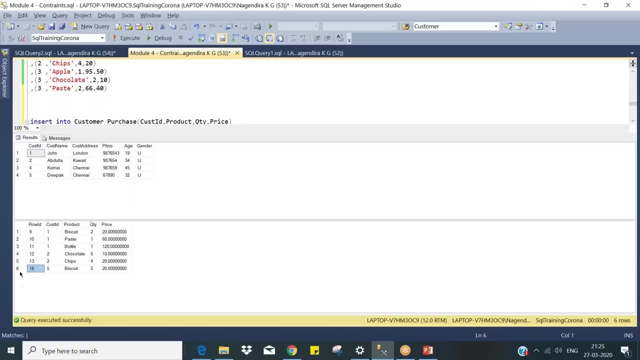 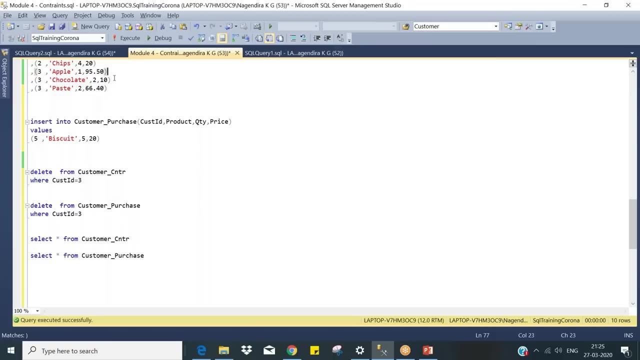 automatically. one counter is increasing. that is your row ID. you see 9, 10, 11, 12, 13, 14, 18, something. I deleted three rows, so in between three rows gone, so 18. when I do some other insert like this, I can do another insert also. this guy again came, the customer again. 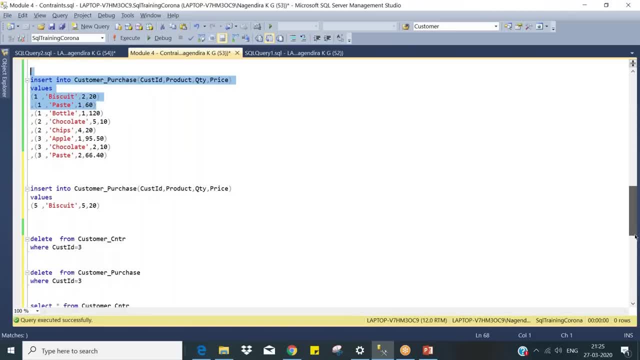 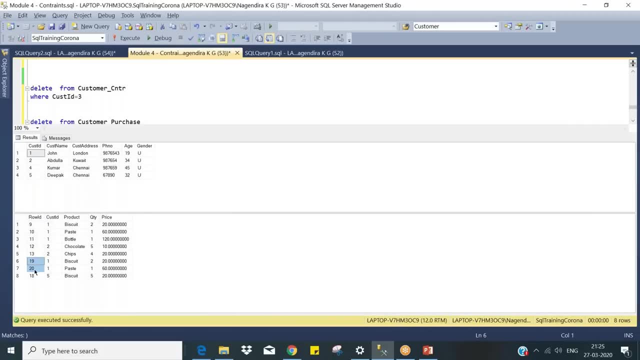 he can come. okay the show. so again he came. now, you see, 1920, this is I mean 19 today. these two records got in certain now, okay, so one, two here. initially it was the case. now again he came for the shop and he purchased a biscuit and paste again, so 1920. 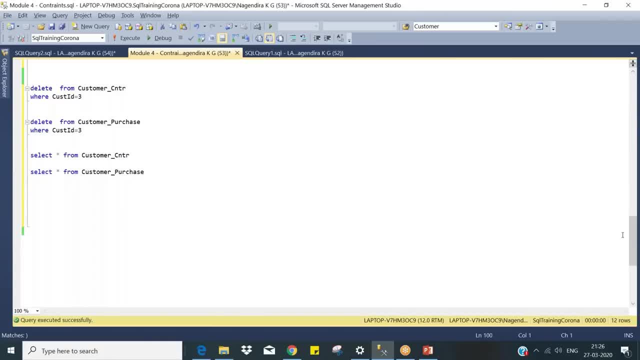 so this number I am NOT specified anywhere in my insert statement. okay, in such statement. so to auto increment some values based on the incremental values. it is similar to a default. default what it will do always. it will stamp a single value. so I want each time one row to be incremented. so for that, a function name. 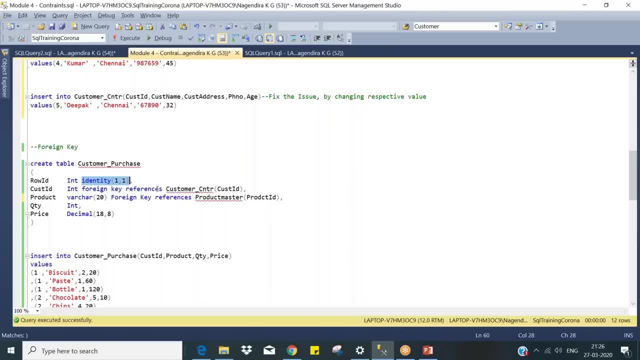 called identity identity 1 comma 1. so in Oracle we have sequence sequence 1 comma 1, something like that. okay, so some. it is a function you need to specify meaning that begin from 1, increment by 1. if I do increment by 2, 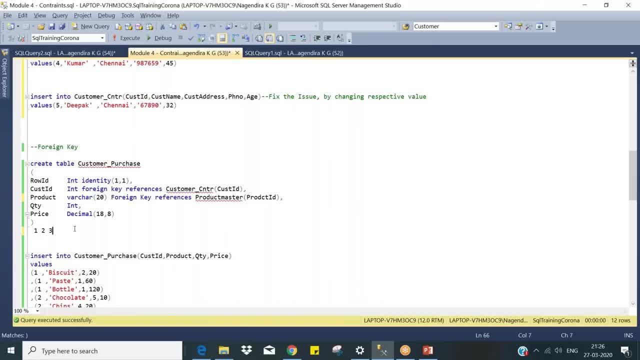 then it will go see. the sequence follows like this: 1, 2, 3. here if I say, for example, 3, 1, 4, 7, 10, 13, something in that, keep on adding from the last. whatever the digits, it's worth it. so this is the purpose of your identity column- any. 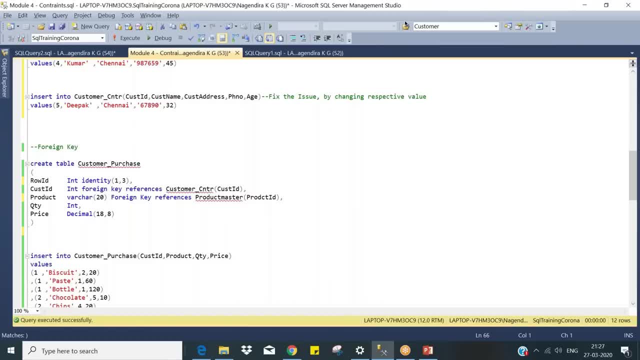 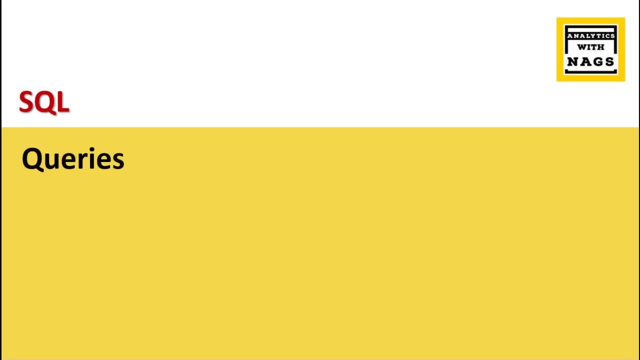 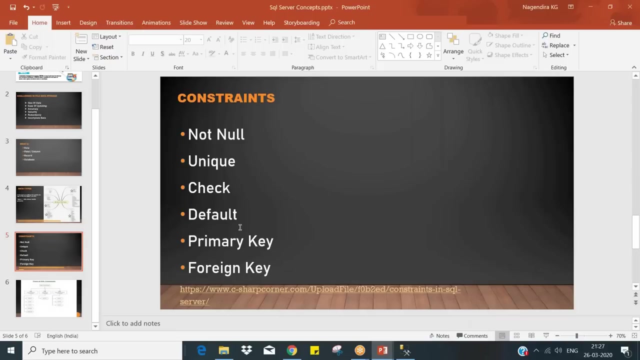 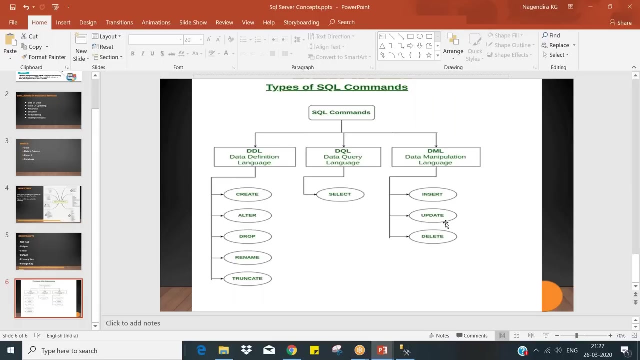 doubts in this identity. no, okay, let's move on to the next topic. you may have seen this one. I mean insert, update and delete slightly. we'll discuss more about this now. I'm going to go more deep into DQL, that is, data query language. select it. here it is written: only select, and we will do more magic. 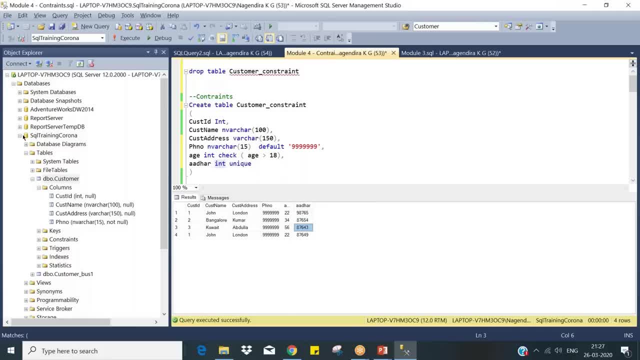 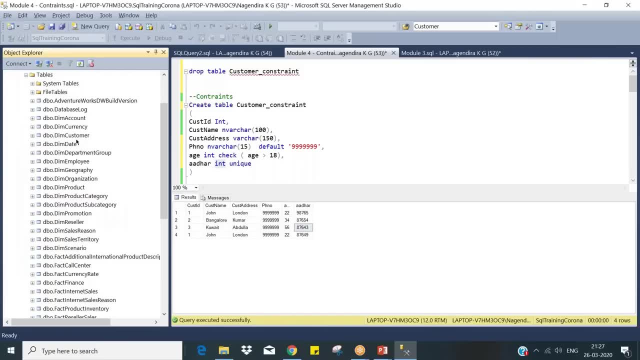 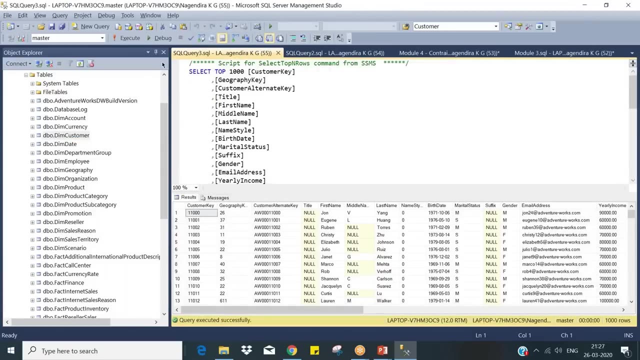 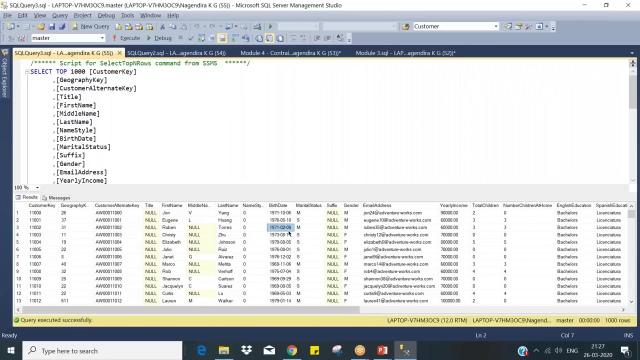 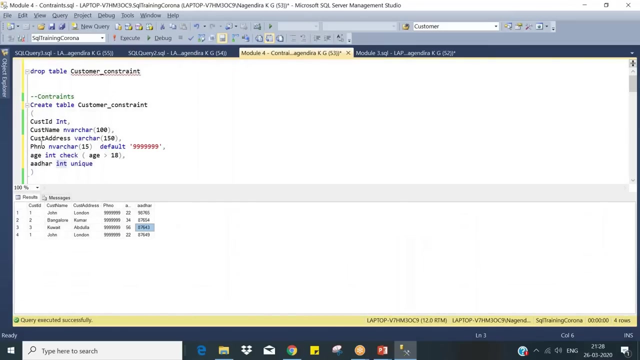 in that. for that I will try to go into the dashboard. so I'm going to go into the dashboard. we will do order and I will select the order on the left side now and we'll add the order and we will see what I get here. what I see through here doesn't mean I get the order. you can see it. 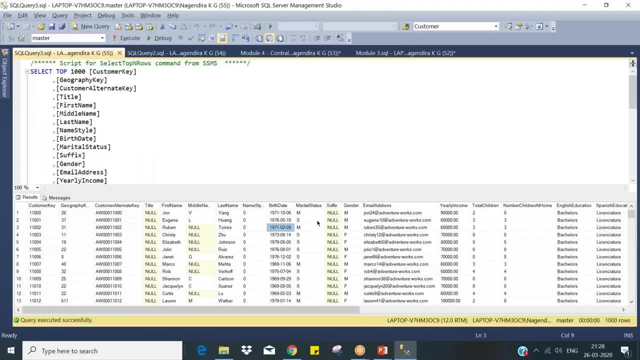 works well, so we will just keep doing it. we will just keep going. so let's go over, have a customer data with all these attributes. see guys, you have a customer, he's a john. okay, now you have got a customer key. okay, this is the actual key. i mean maybe a id for him, but this 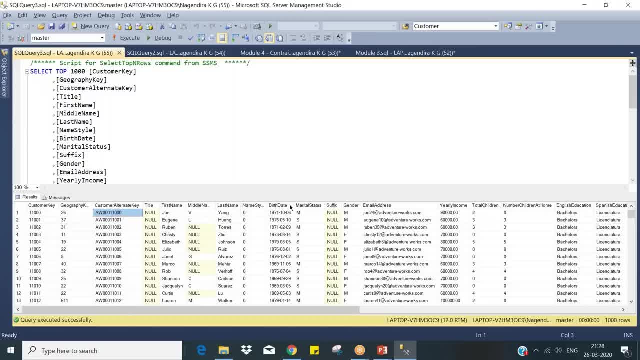 particular column, i mean this particular record. you have all the attributes, nothing but first name, birth date, marital status. all these things are belongs to this particular customer. as i said, this john is not belong to this guy, he belongs to this. so this is nothing but your record, okay, record. 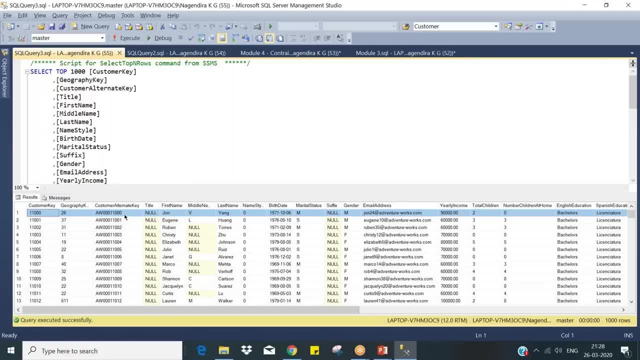 our row in a table now. so when i want something like, uh some, why so? when you insertion, updation, deletion, you know guys, now i want to have some queries saying that i want someone who has born over 90- 70.. i mean 90- 70.. 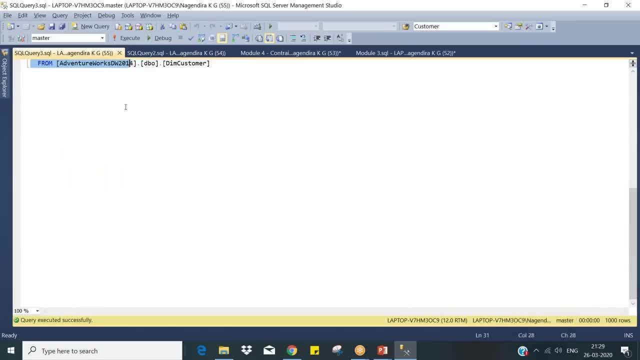 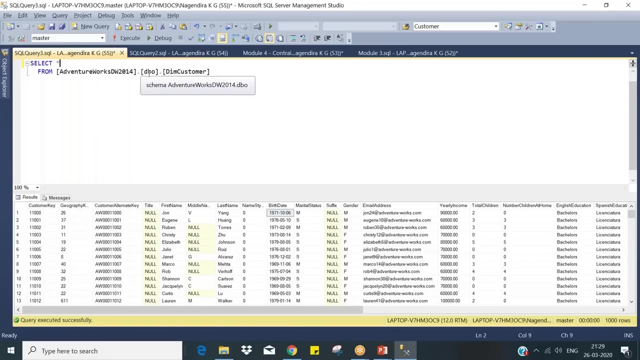 so then, what you need to do. like this business scenarios will come: select. i will put select star from this table name. okay, what i'm trying to explain here is you. you have learned about insertion, updation and deletion and all. now, after insertion, what it will do. you need to access the data. 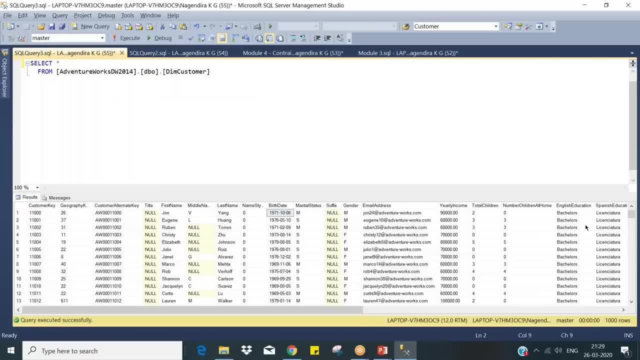 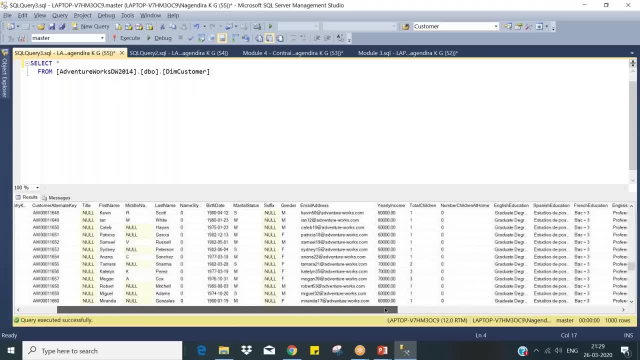 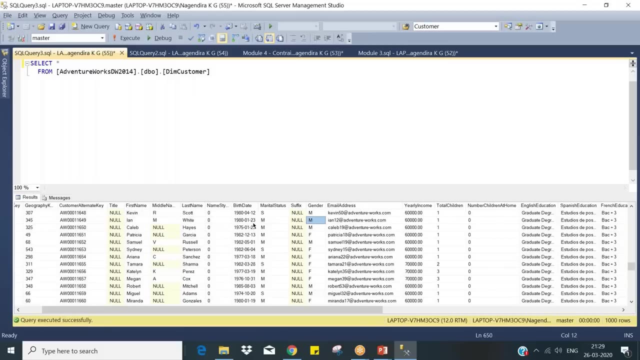 based on business scenarios. i want to know how many bachelors in my customers, how many married people in my customers, and i want to know, uh, whoever has not provided the email address, or whoever is male and whoever is male and it is married or single, something like that it should be. 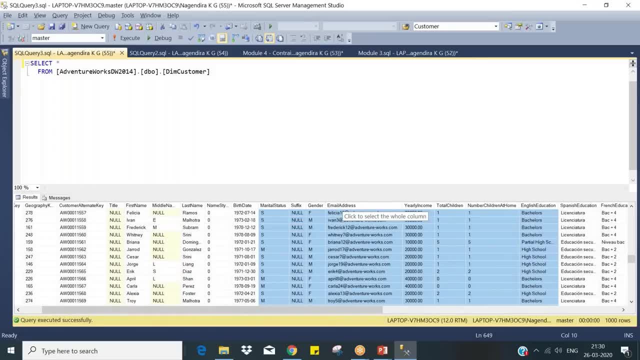 bachelor or college graduate, something like that. so business scenarios will come. they will keep on asking the question. this is where i think, uh, my colleagues find most of the time- i mean, they always go for queries- a lot of questions will come from the business and we need to query it. 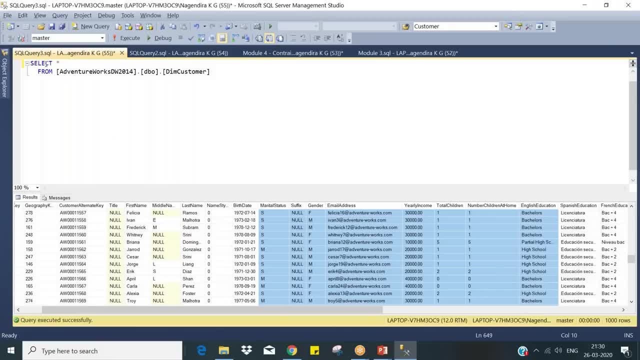 so the one and only statement is select. the syntaxes follows us like select star. this star is nothing, but if you see star when i highlight it, it displays the column. star means all columns in the table. specify a single column. also say, for example, customer alternative key. i can select only this. 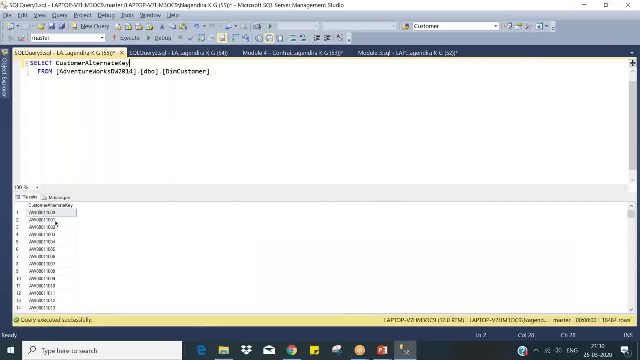 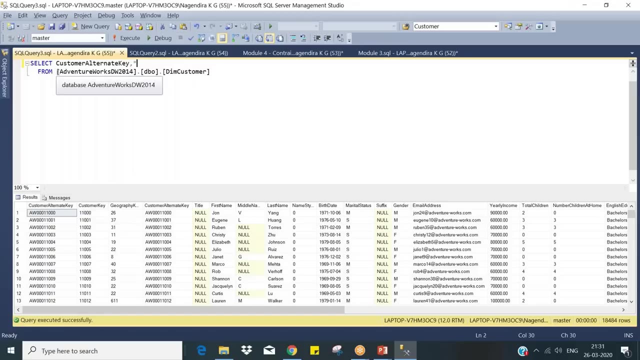 but it doesn't give me any view, just give me a data of it. okay, so i can put it like this: also, i want to bring some columns front. i can bring that column front, then go for it. so so this is you till this. we saw about only according like: uh, select star from table name. 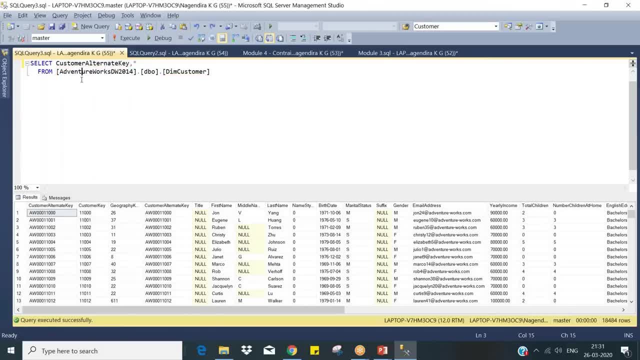 what about this? i mean, it was like that control. is it why it was three distinction values? what are those? okay, we'll take this later. this is nothing, but for now, explanation. this is database, this is a schema and this is your table. okay, i'll tell this later. 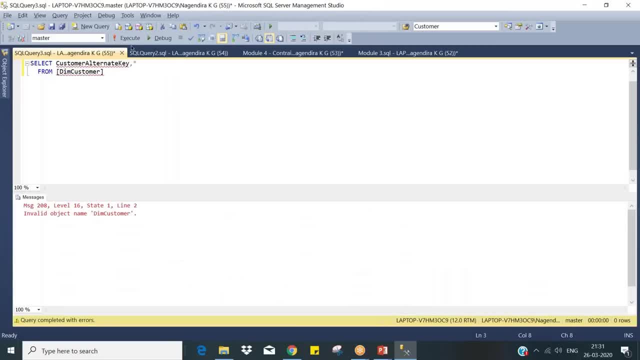 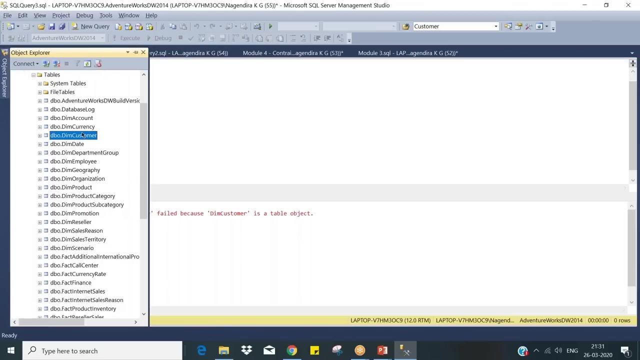 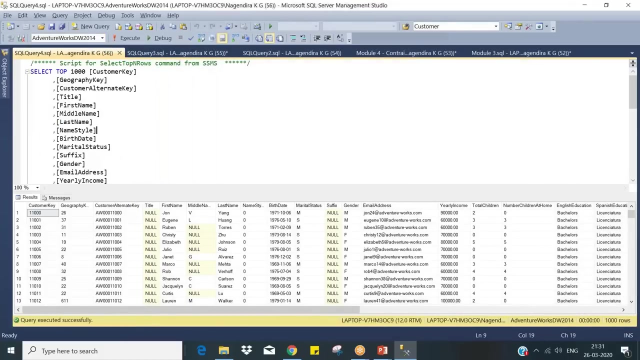 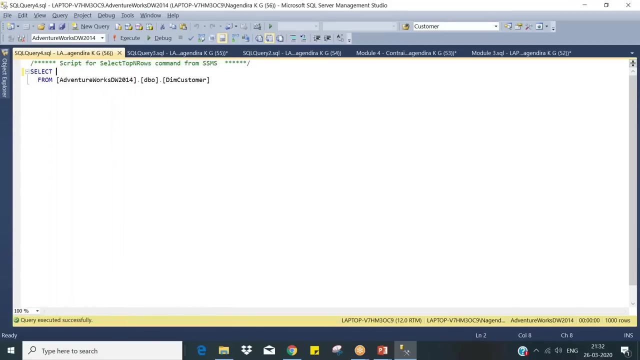 let us. you should use that condition. yeah you, you know better. i think you already learned. just hold on. okay, the request of procedure failed. bye, see, either i can choose. see, i can run from my sql training schema. this is the database it's going to run. if i use this, i can access the another database also. syntax error from selection. 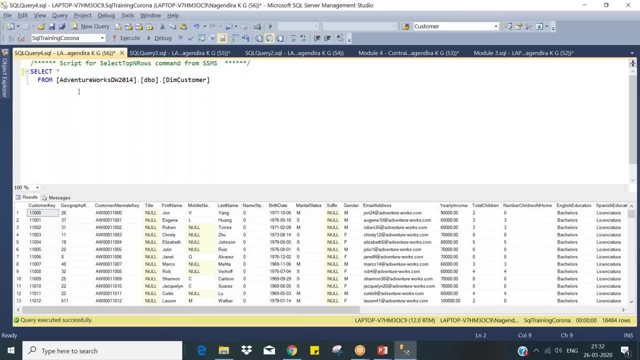 alpha. it defines inter database queries. okay, forget about that. just keep it simple as that. dbo dot dbodimcustomer, then var to filter. whatever columns you want to filter, you need to use a var condition. but i won't just say gender, i mean a male customer. you put gender equal to m. 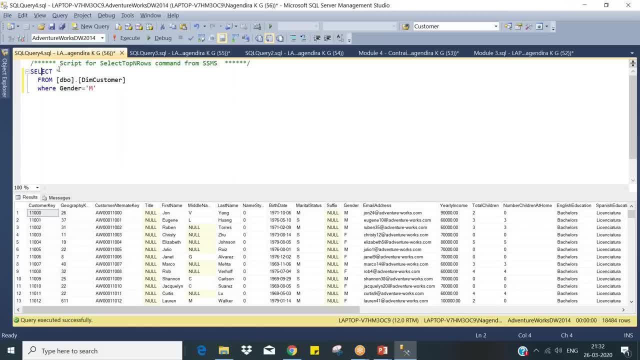 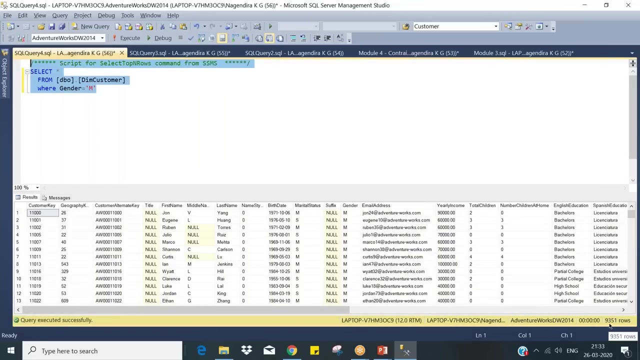 so this is the syntax: select column name or staff and from your table name, then var condition to filter. if you do this one, there is no filter. all the records, eighteen thousand records, will come. now you use var condition, that will filter only male customers. execute it. you see, out of eighteen thousand, nine, three, five one is your male customers. 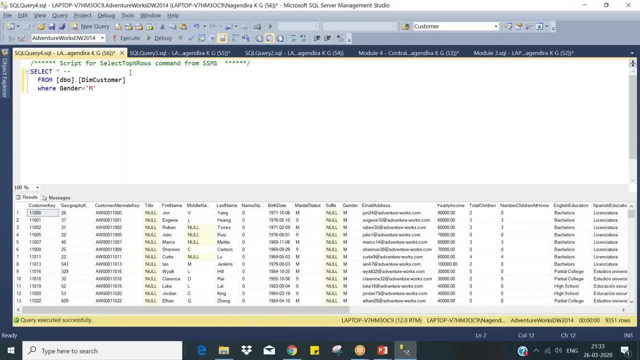 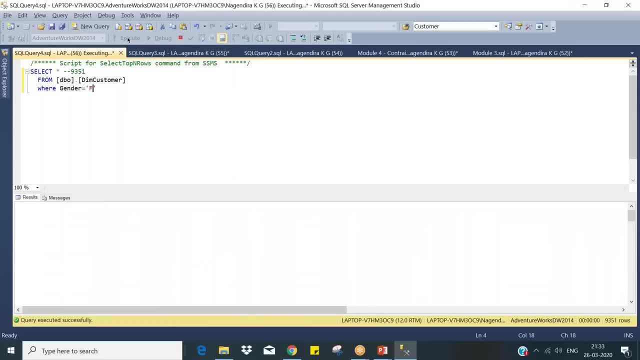 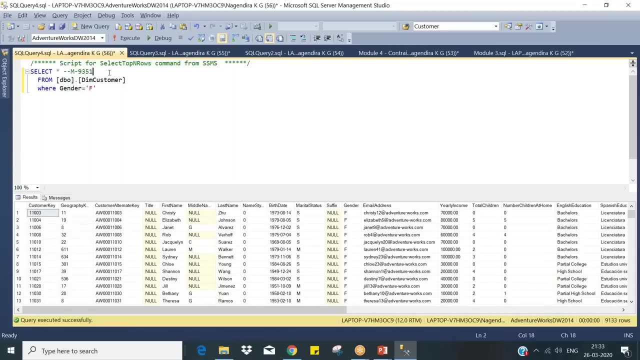 let's go for i'll take account here. nine three, five one. if it's female, how much? nine one? this is me, then it's female. nine one, three, three. okay, so this is just a typical query, how you need to um query your database, okay, simple basic query about uh select statement. now, when i have uh, 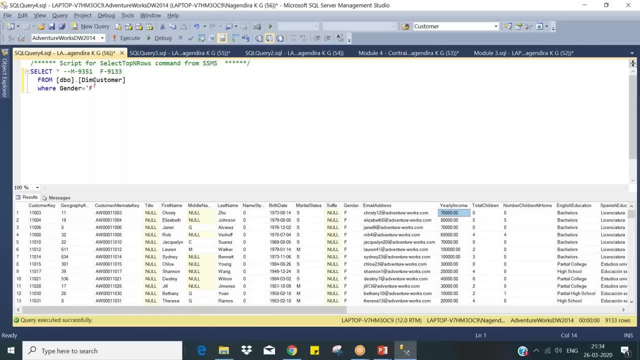 something like: whoever gets uh more than sixty thousand. so these are the operators you need to learn. i'll keep this query as such. greater than that is yearly income. yearly income greater than fifty thousand- i think this is in us dollars. again nine thousand. maybe i will increase uh slight. whoever gets most of it. eighty thousand: 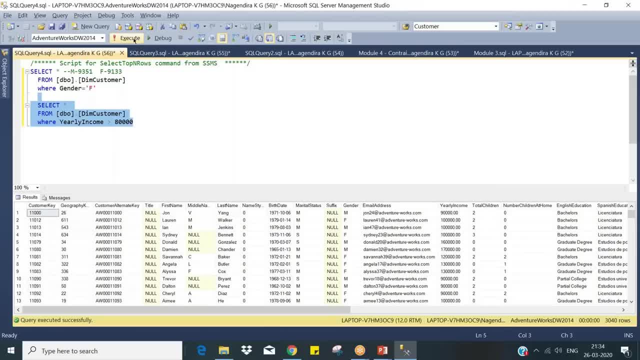 used investments. i think it's around six lakhs per month, so only three thousand people who has a yearly income eighty thousand, okay, so if you see the results, it filtered with eighty thousand greater than maybe if i use equal to, the result will change. three zero four zero. 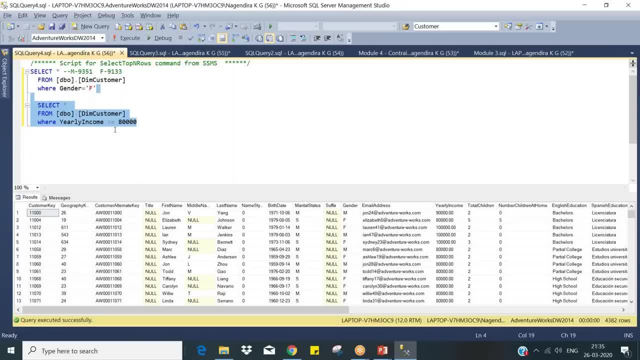 okay, four, three, eight, two. so everyone, i mean to say uh. whoever having, instead of having uh, greater than or equal to, i mean i can put equal to that- will give me thousand records. thousand, three, four, two. okay, you see the result now, exactly the matching. so these are the. 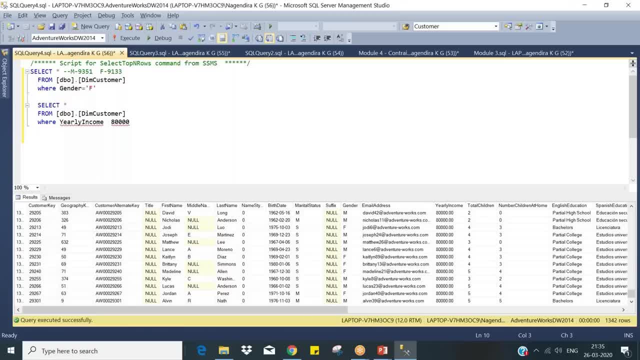 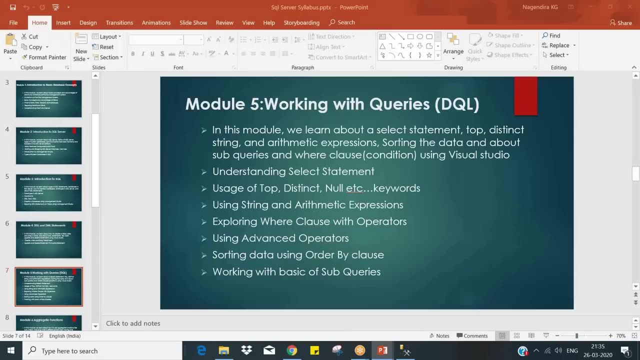 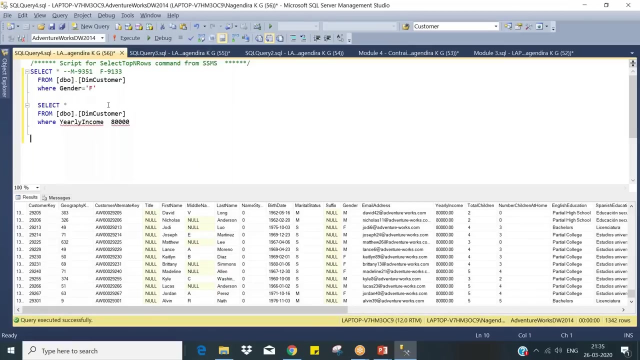 operators. okay, like what operators you have? conditional, equal to greater than less than these are the operators you use here. let's go to the syllabus select statement using strings and arithmetic operation, exploring where class with operators and i go for top, distinct, null, etc. okay, so now you see, like, uh, just just a basic understanding of gender and yearly income. 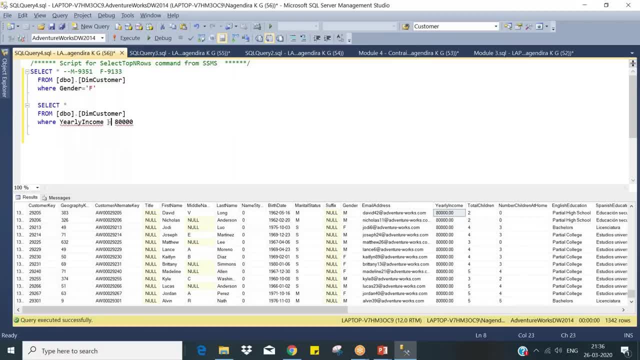 i saw, with only one column, what happens now: whoever gets 80 000. and also i want a female, a female customer who is getting a salary of 80 000. this is the condition. so you need to combine both the condition here, so you need to use and. 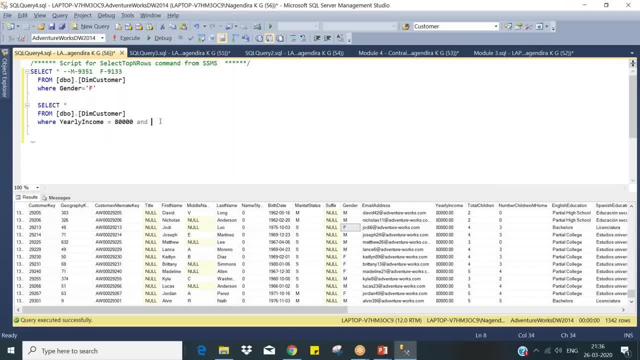 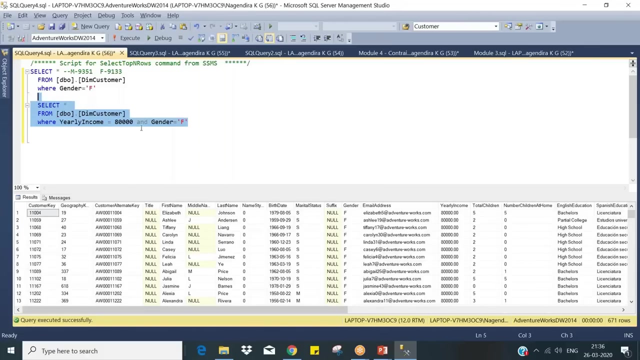 just apply in english: yearly income 80 and gender equal to female. so if i use like this, this will not allowed. always string values should be coated with single quotes. so i use both. so my results are drastically reduced like six out of five. so i know that if i use both of them, the results are being drastically reduced. 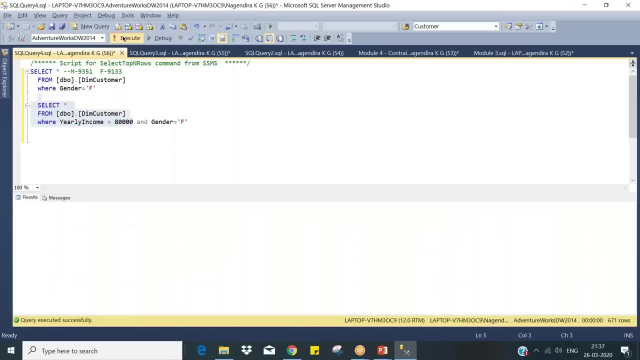 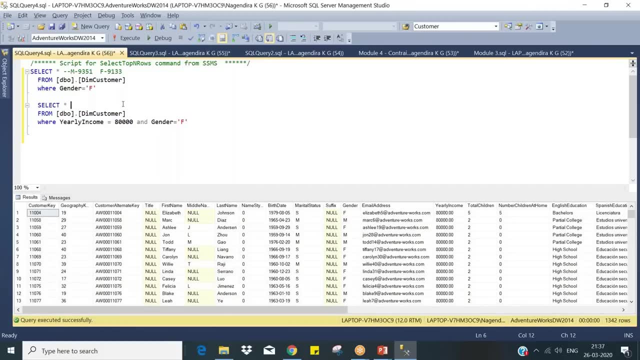 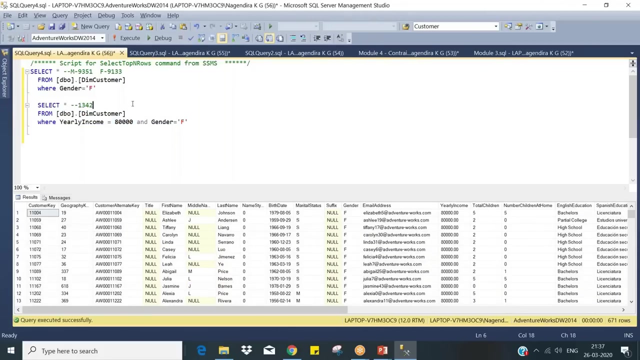 like 671. when i use this alone it is 1342. so i can say like it's one, three, four, two, and female is six, seven, one. so what about, uh, your male? so these kind of checks you can make by yourself while doing some kind of work. 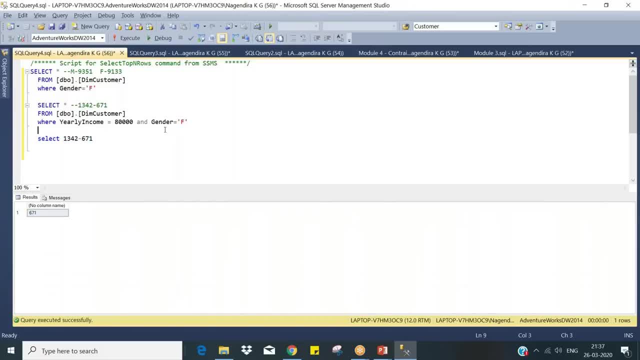 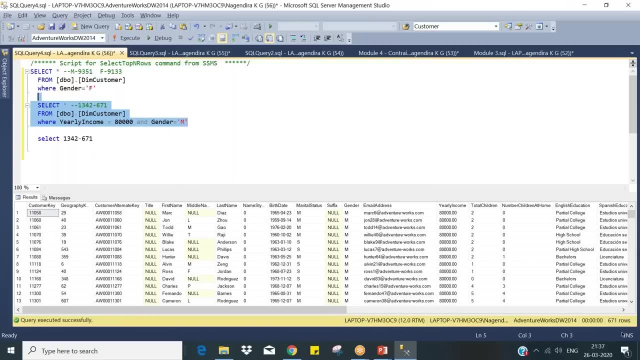 what i'm trying to say is 671, so it's exactly same. so even male is 671. see, i got output before. i know that data. when i subtract it it will come. so this is simple thing, okay. so how many conditions you can have, you can have many conditions. 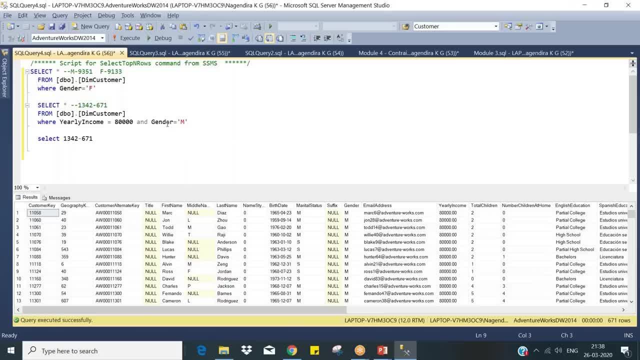 as such, based on your business logic, based on the request. there is no restriction, like only two condition, three condition: you keep on adding the condition. so this is like yearly income 80 000. gender, male and how many kids i want? only one kid or without a kid? something like that. 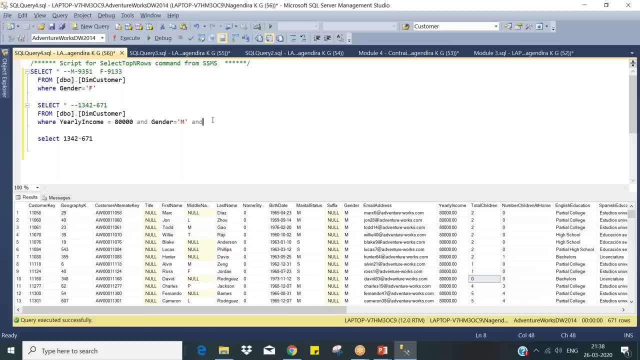 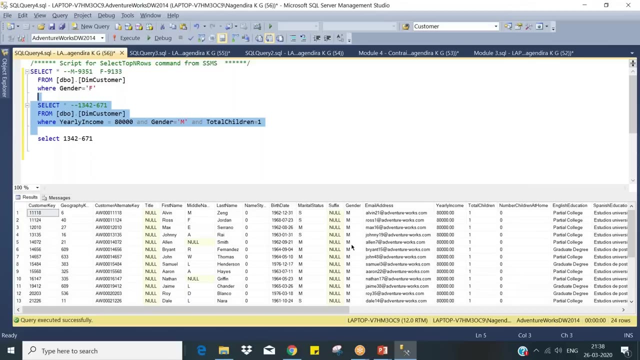 okay, so maybe i will add: and total children equal to one. it's like a question and answers you got using your query, so people will ask you a question: who, a male person having a one children and getting a 80 000 salary? how many people are there? 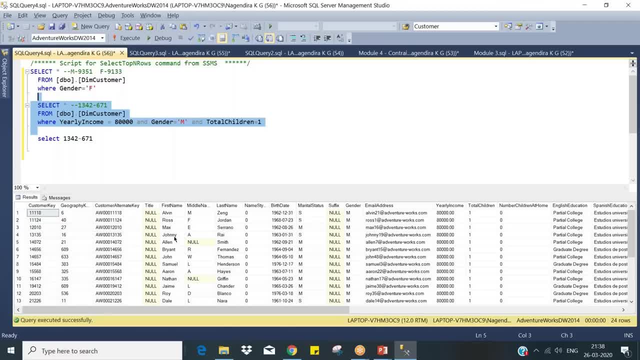 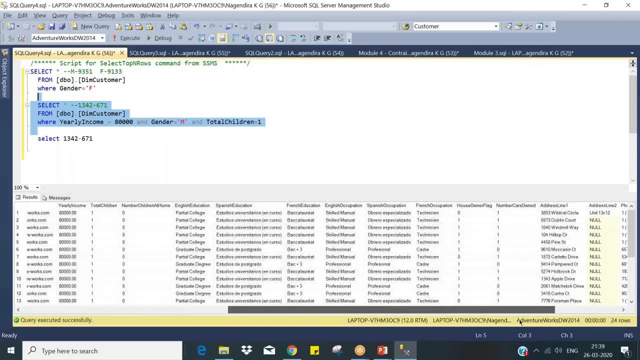 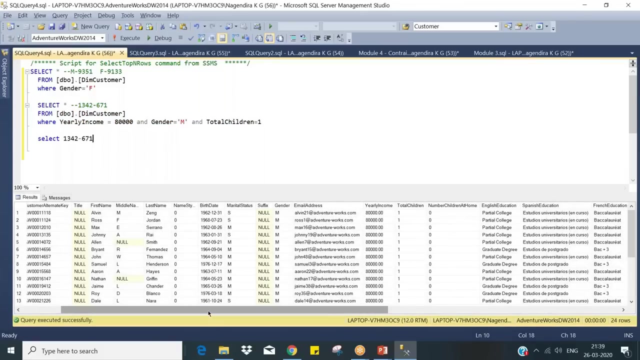 we will give this list. so what they will do using this. they will do some analytics on that. they want to promote some offers for these customers. who is having one- a child? okay, something like that. can you also tell me some specific period after which greater than or equal to yes. 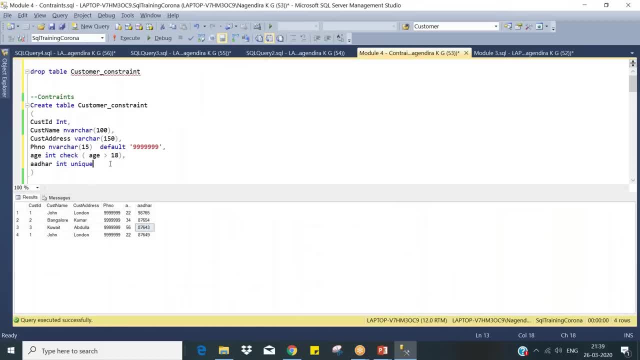 yes, yes, i date part i didn't cover so i will come to here first. so, date similarly, uh, integer n worker, this one. you have a date data type. like i will say, if you have a date data type, like a 15 month period, say, it's not even a date day day. 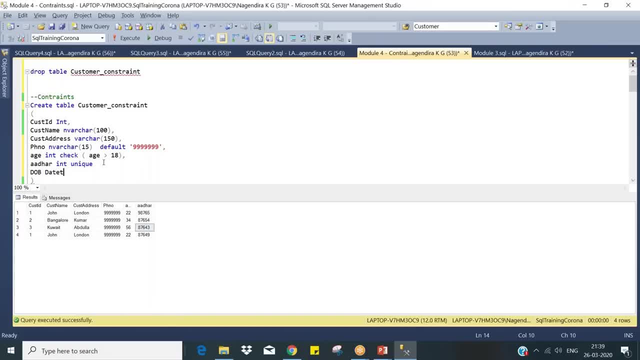 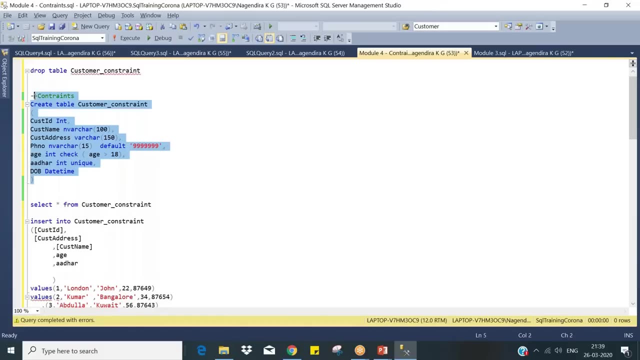 date of birth. i can go for um date time. okay, date time, then i'll drop. so date you can. uh, it's. it's little bit tricky. always you need to use the appropriate format: uh, ddmm, yy, mm. or. what i'm trying to say is: either you can specify yy, y, 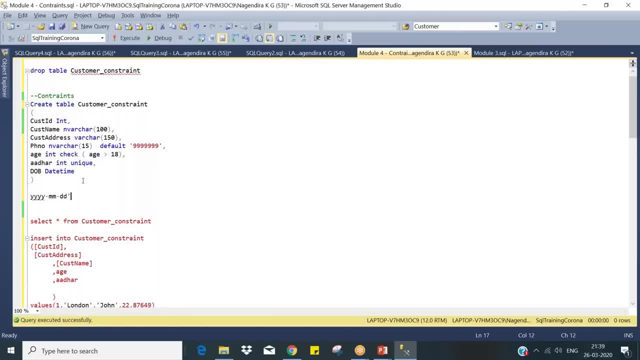 mm. dd. this is a standard format used to follow. okay, so in this format only you need to insert yeah, yy, y, mm. dd. so in the same example i will specify date of birth. so how you need to specify, either you can use the same format i mentioned: 1988. 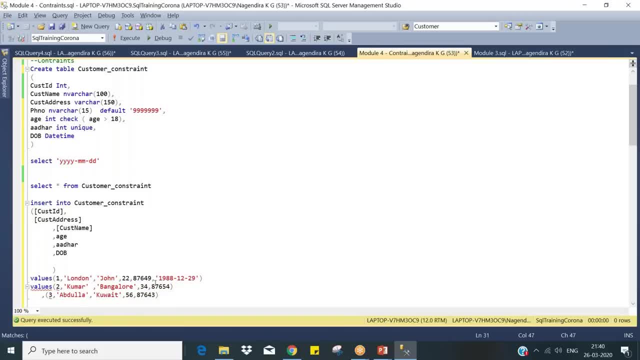 to work 29, say for, say like that: okay, i'll insert this guy. okay, so 1988, december 29. okay, this is the and time. also you can mention. i didn't mention the time, so it taken uh, the midnight, midnight of 29 000 000. if you born on a second, no one cares about. 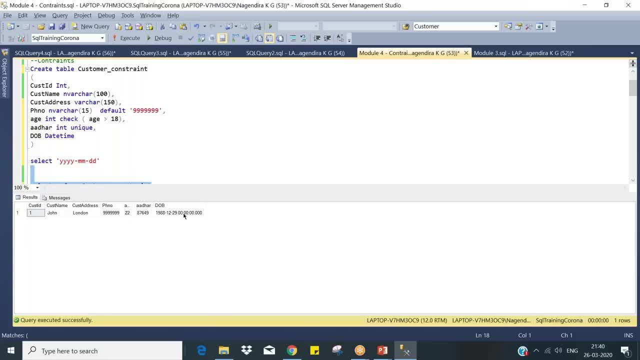 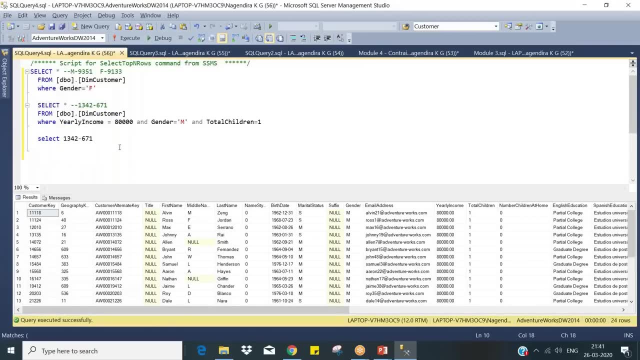 the time i mean typically recording, i mean in the database level only to astrology. i think we use time fine. so now to answer your question. so date is same like any other data type. now i want uh, some uh dates like uh, whoever born uh after 1970. so here we have something like uh. 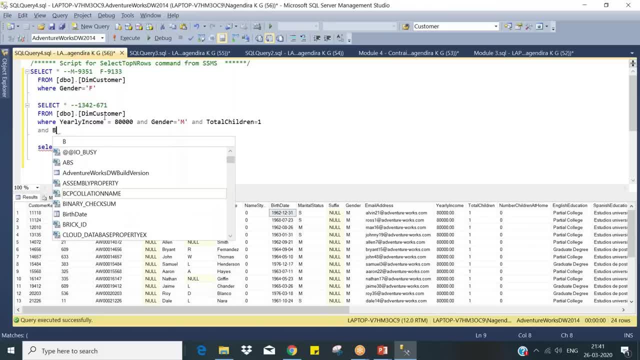 and you keep adding no restriction, okay, but date greater than. take a copy. you say like including. see, this will say like uh including 70. i mean to say first of january i'm in uh 1970. this is greater than or equal to means including: 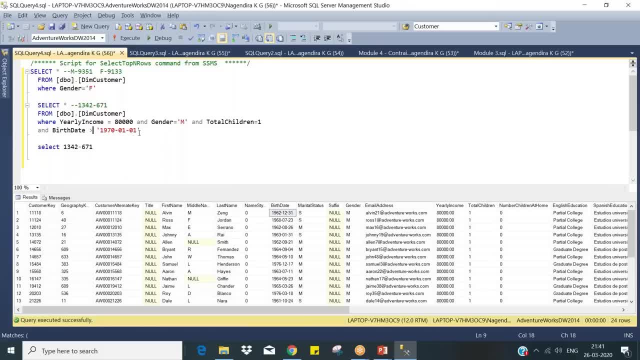 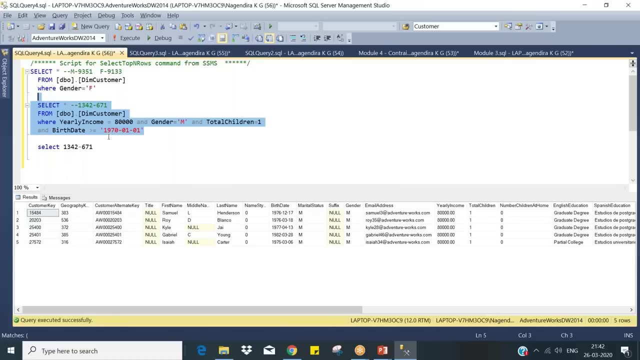 this date. if you remove equal to, this is excluding this date from the second of 1970. okay, january 2nd, so include means equal to. so there are customers who are born after 1970, so five customers over here. so this is simple, typical example. okay, and date functions, functions. we will come through. 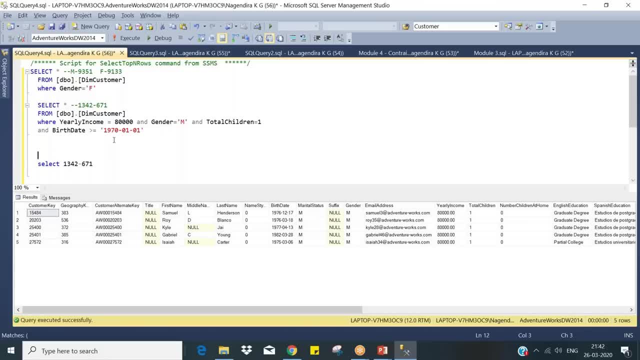 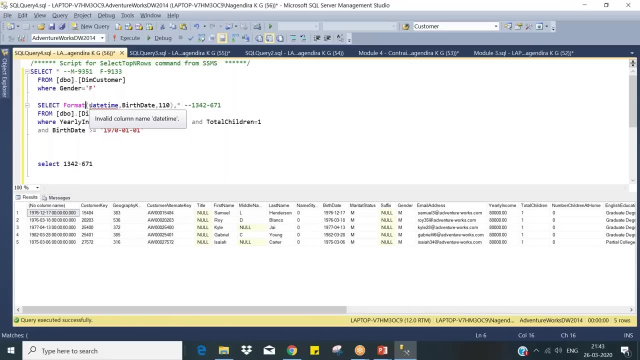 it now. yeah, if, if the database has uh, year, month and date and suppose if we need, if we need month, date and year format, it should just be displayed in the same the way which we require. we need to have appropriate function. there are a lot of functions. okay, i no one knows the syntax. see: 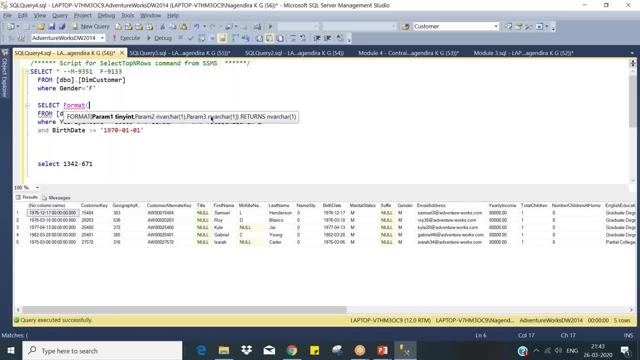 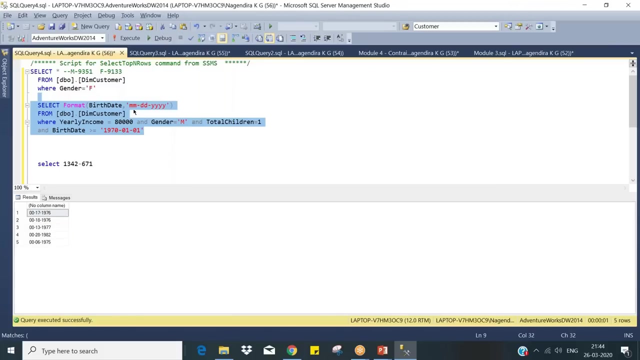 like uh format, param and param2 and param3, and we need to specify appropriately, see but date, that it can be either first parameter, a second parameter. now you see mm, mm, dd, y, y, y, something like this: let's try that one. now it worked. see, here went at last. something has happened instead of two or something it has. 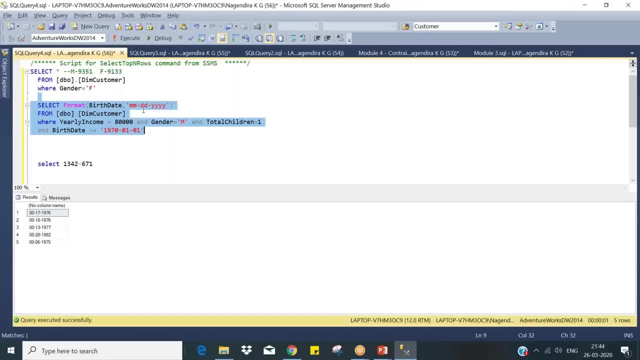 happened, so you can do it. okay, it's not uh doable. you need to find appropriate function. then do it. usually it will be like: convert, we'll use cache, we'll use format. so in article also, i think it will be format or some other function, so it doesn't matter, just for we need to find appropriate function, everything is. 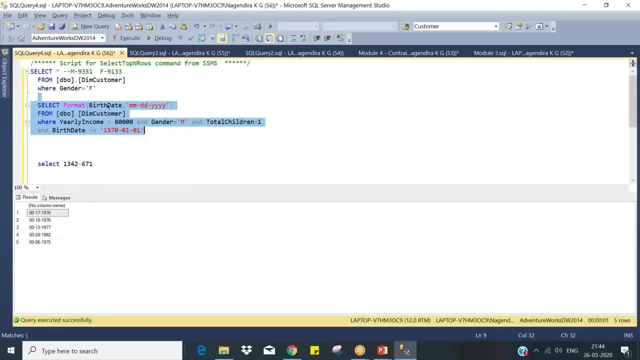 possible, okay? uh, when you see the birthday comparatively, you can see the result. what, what happened? so you can see the result, and then we will do that. so we'll do that, so you can see what the result looks like. so let's see what the result looks like. now. let's say m m, m m. what are the dates? 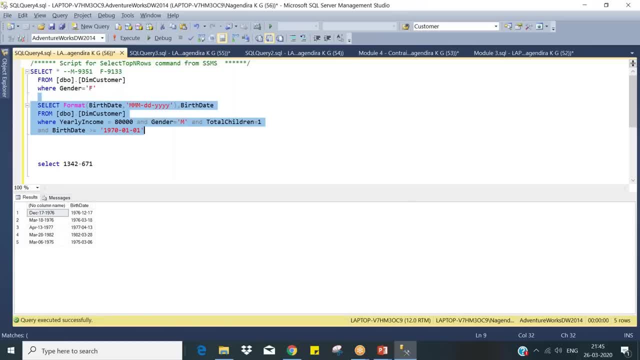 and mm. it is doesn't convert it. maybe we'll say m, mm, something like this: yeah, now it worked. december 17, 1976, march 18.. okay, we can do it. find the book. thanks, yeah, so now you got again. find the book. thanks, yeah, so now you got again. 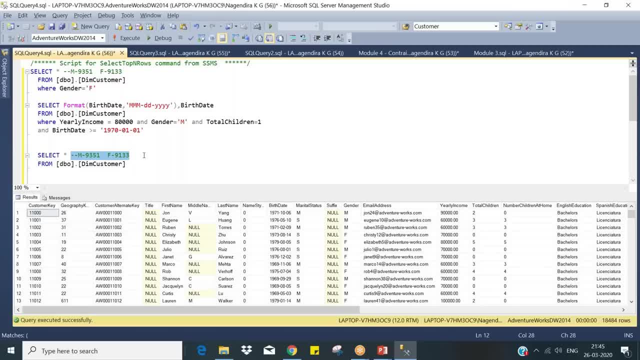 find the book. so now you got again. you want to work through the database. you always not going to work with all the columns or all the records. over here you have 18 000 or some tables contains millions of rows. it will, while running the query itself takes a lot of time. for that, what you do? you do the sampling of records. seeing this: 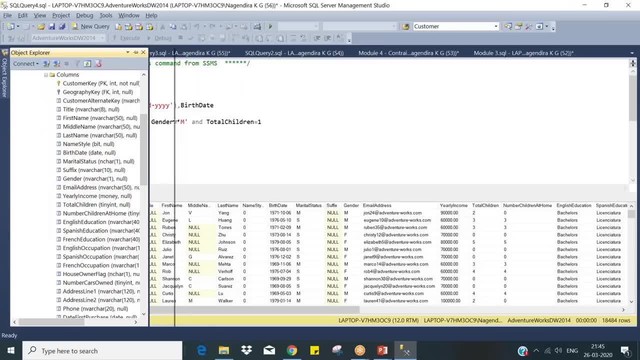 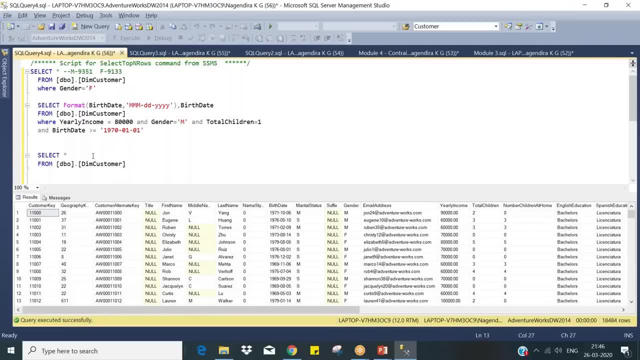 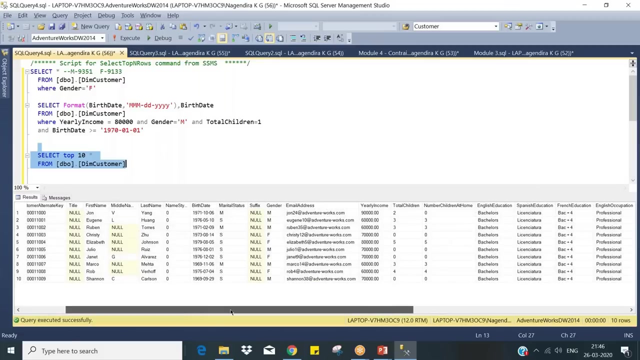 column definition doesn't make you to understand what is the exact data, whether some data is there or not, okay, so always you want to see the data at that time. you can't see the entire data, so you can use top 10- top 10 records, which will give you first 10 records so that you can analyze. 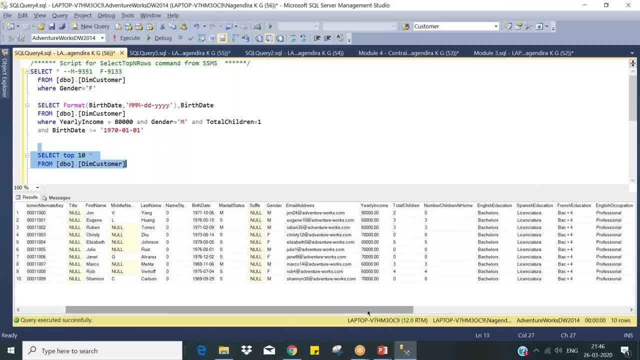 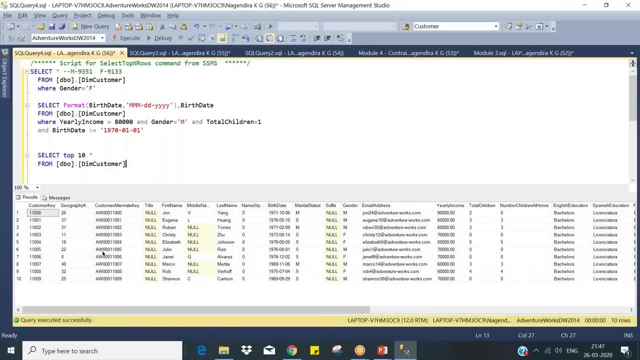 understand what kind of data it has, whether people are filling the email, whether yearly information, is there something like that? so top 10, just for profiling purpose. we will use this one. now you can ask me like: uh, you, i know that i, i have all these columns all in place. 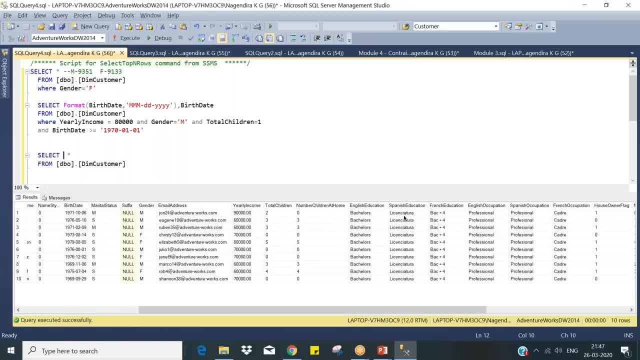 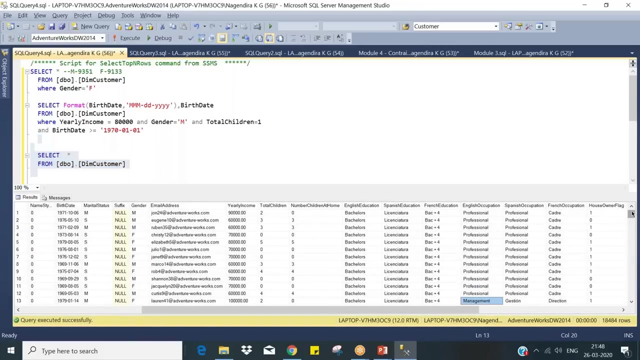 but what about, uh, this guy, i mean english education, or here you have english occupation. what are the different occupations i have? i want to only the. you see this is repeating. i don't want like this. i'm saying what are the different occupations? we have professionals, management and skilled manual. all those guys. 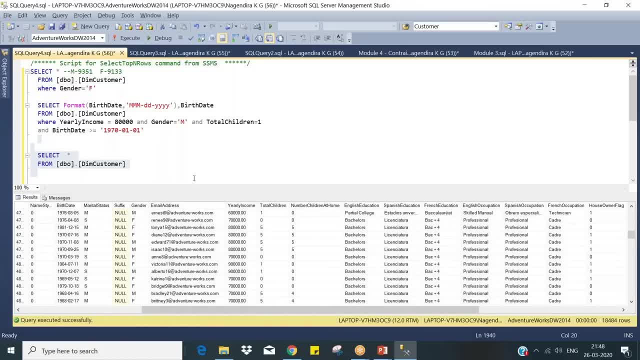 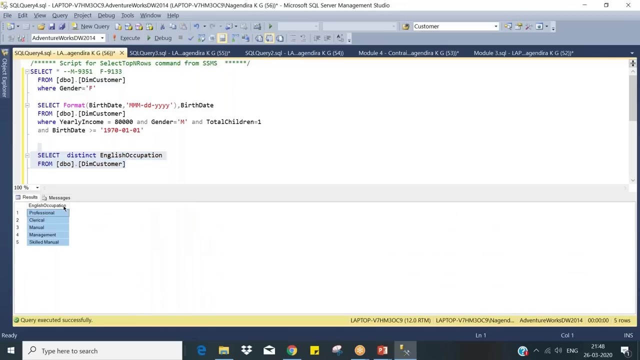 while inserting, they will keep on adding it. okay, then i need to get those distinct values, so just you can mention distinct of that column name- english occupation- and i use this one. i will get the five different values in this column: professional clerical manual and management skilled manual. so these are the different values. 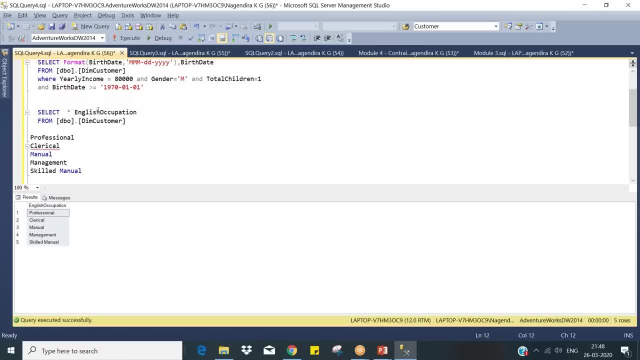 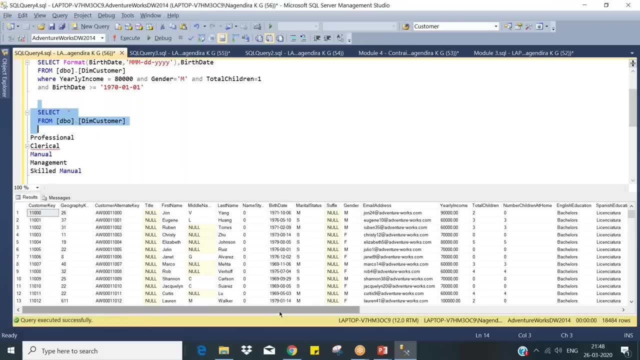 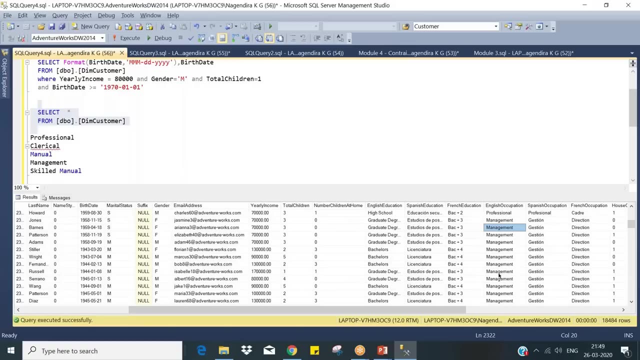 so no need to go each and every uh record over here and see, you cannot copy and paste. you got the point right. if someone asks you what are the things you can, you go and check, you take this value, then you keep on taking this value, you don't remember. 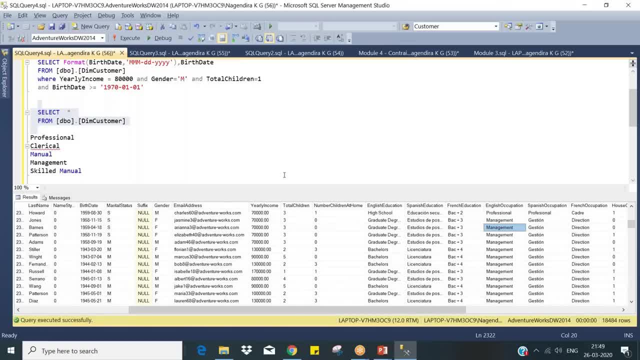 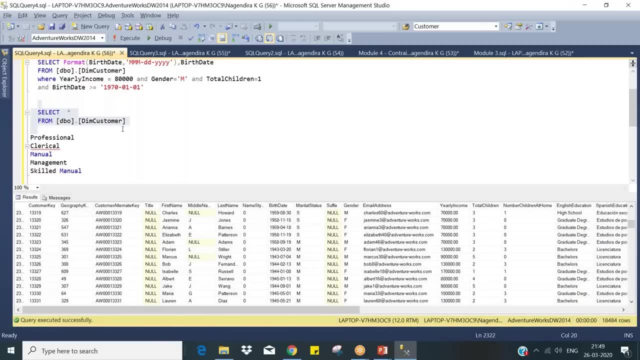 which one is already you have taken or not. so just putting a single query will give you what are the distinct values, unique values in this table, I mean in this column. so this is about your distinct. then, as you asked, as I told you, when you use this select statement you always see like 26, 37, 31, 11. again I'm. 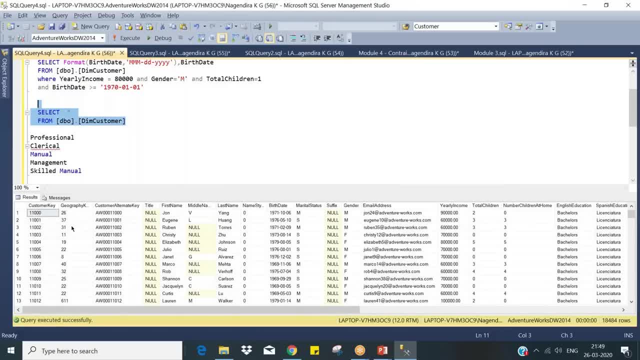 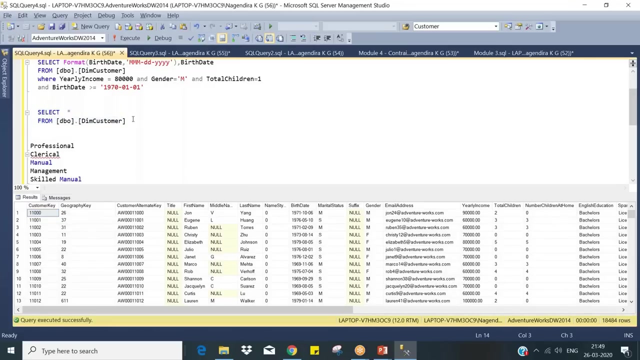 running 26, 37, 31, 11. okay, so, as I said, it will collect the data based on the order how it is inserted, based on the index logic. it work, but I want certain order, like geography key, starting from 1 to as sending, I mean so how you specify. so select shot from this one where 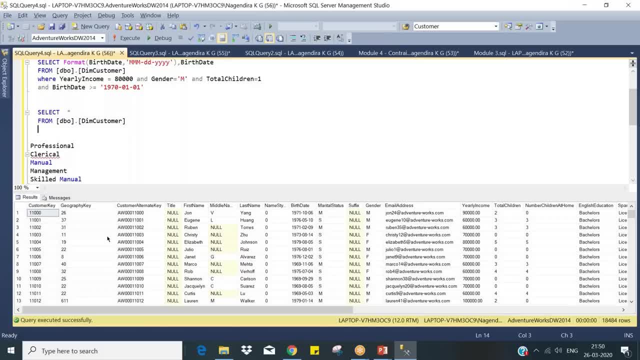 condition used to filter. I want to display the results in some order. order key ordered by see basically doesn't inserted by geography key and all you see the customer key. it's a custom based on the customer key that's inserted. I don't want to be displayed by a customer key. I want it to be displayed who. 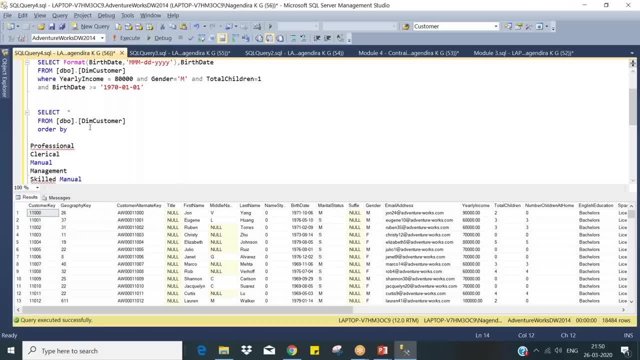 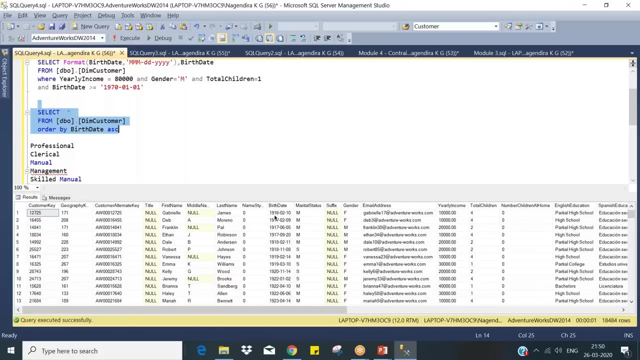 are based on the earlier date of birth. ascending order of date of birth. so order by birth date. you mentioned ascending. now you see the customer key has changed 1, 2, 3 instead. whoever has born earlier: 19, 16, 0 to show both the. 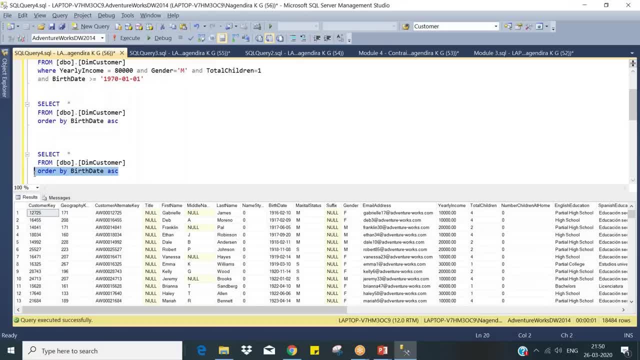 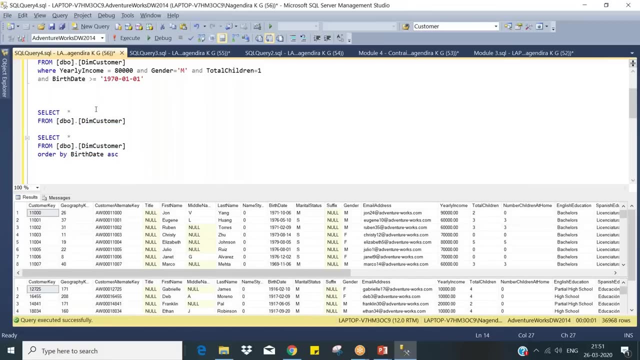 results together so that people will understand this should be top. okay now, this doesn't have first query, doesn't have order. this has order based on the birth date. you see the results based on the customer key. always it will fetch based on the customer key here the customer key. 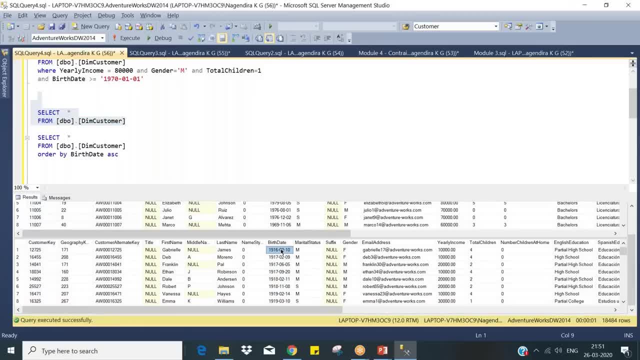 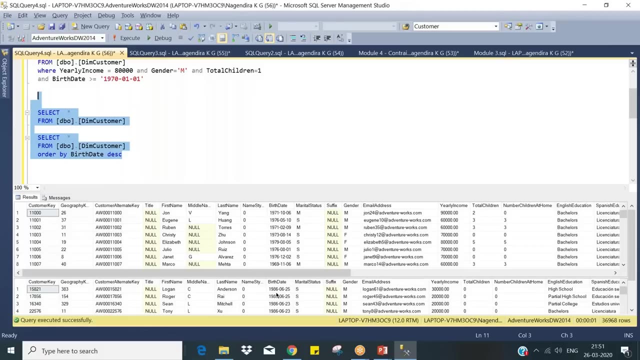 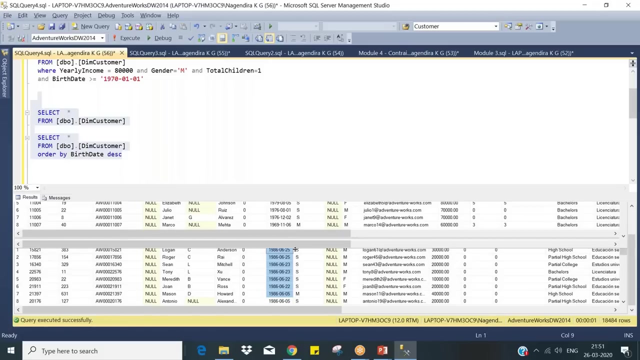 changed it, which it picked me the oldest but did. since it's ascending, I can use a descending also, so whoever is the youngest will come first. again, again. it picks up from the same order here 1986 is the latest, so from that it has picked me. so if i want to use multiple columns, 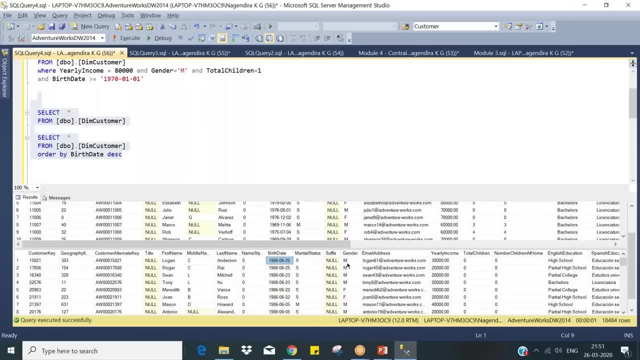 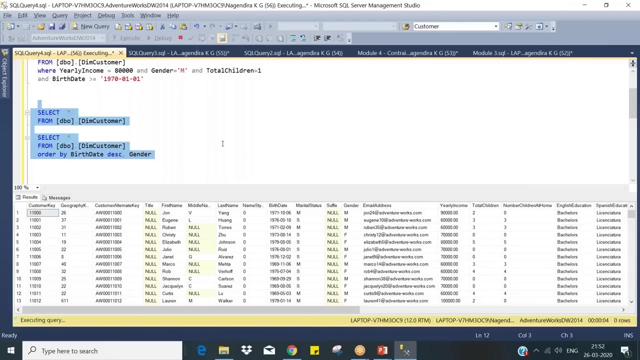 say, for example, birth date as well as gender, then put comma gender, descending or ascending. if you don't specify anything, then it is by default ascending. so ascending in the sense, f will come first, m will go next. see, if we use two columns order, it takes long time. 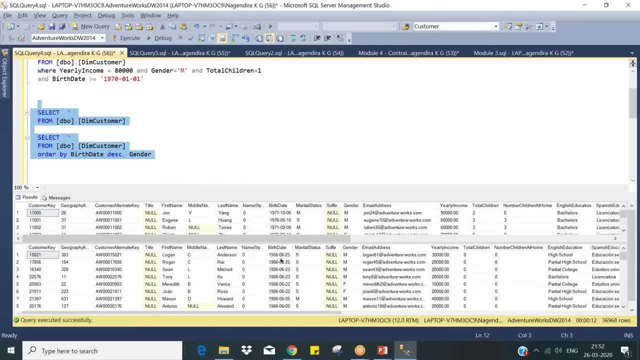 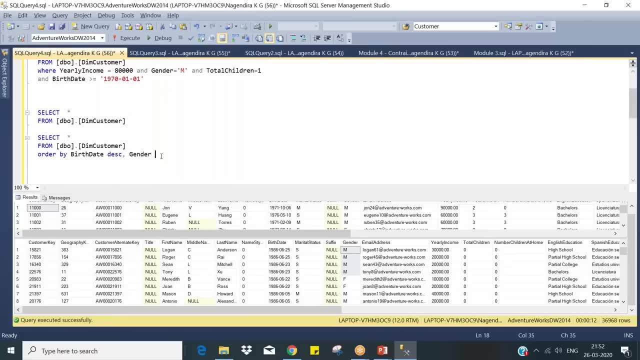 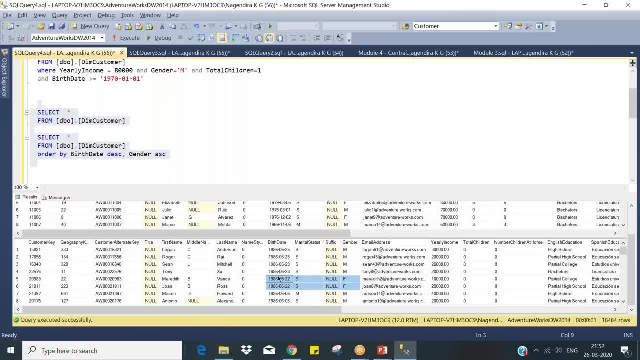 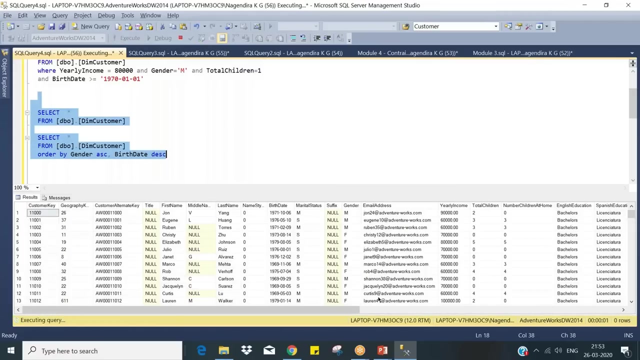 okay, and in 20 second, only female is available. so it filters by a group in this date first. it filters by date in this. if you have multiple columns, then f will come first, m will come first. maybe if i change this order you'll understand better. all females will come first, then. on that it will. 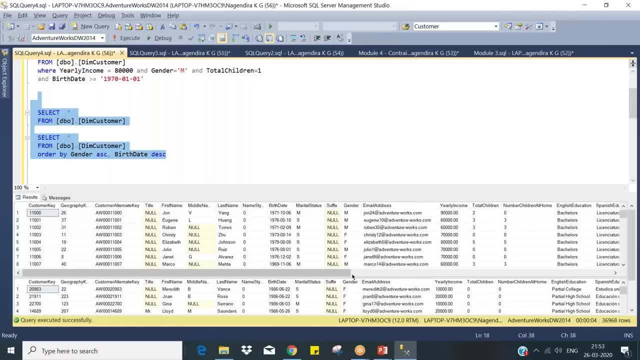 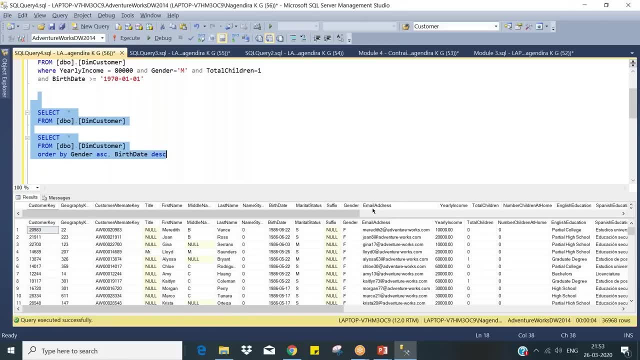 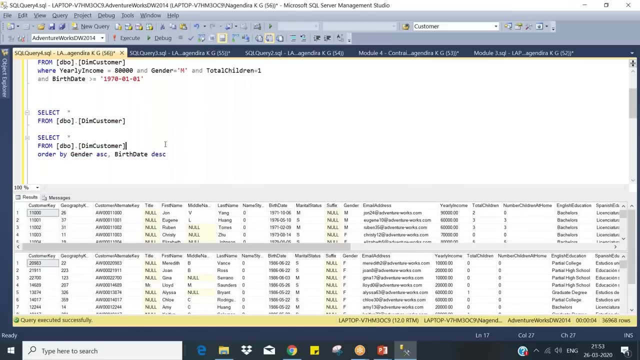 have a date- female, female, female- then here you have a date. forget about this. i mean in just ordering how you want to query or see the data, so the entire query, entire life in a square. you will work on this. you will have these things like select from where order. so this is the hierarchy you need to have. 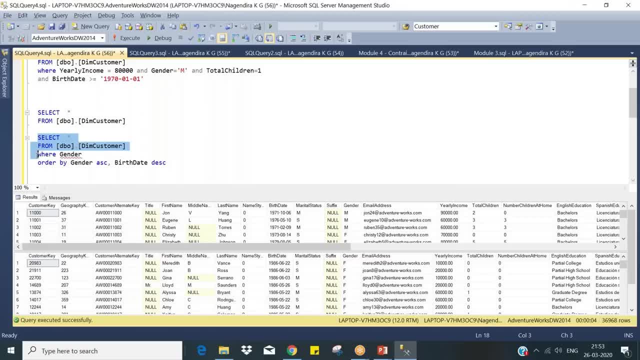 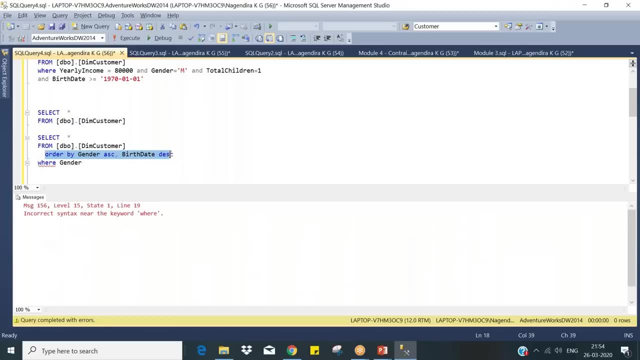 from where order. so this is the hierarchy you need to have: from where order. so this is the hierarchy you need to have to follow. you cannot put the condition before that class doesn't work. syntax error: okay, incorrect syntax. so always, you remember this order of execution: select from val and order by. so this should be your flow and in between you have 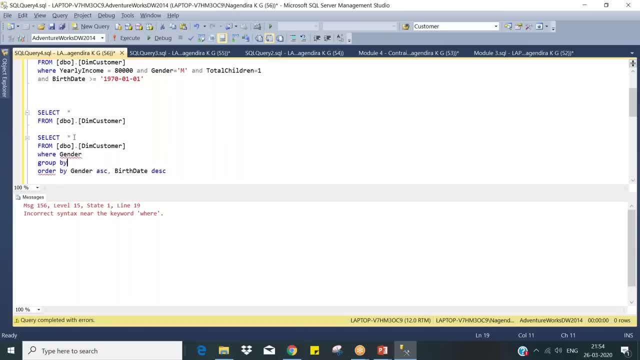 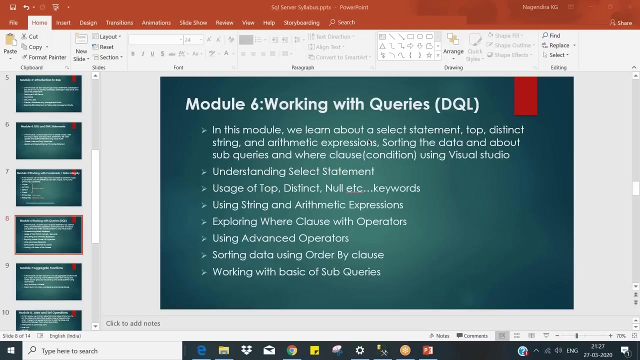 before order: you will have a group by also. okay, this should. this is the whole uh skill statement. there is no more uh addition to it. group by. i'll take it later. so this is the thing. got it guys. yes, yes, yes, we have touched a little bit about this. i mean: query stop, a distinct null. 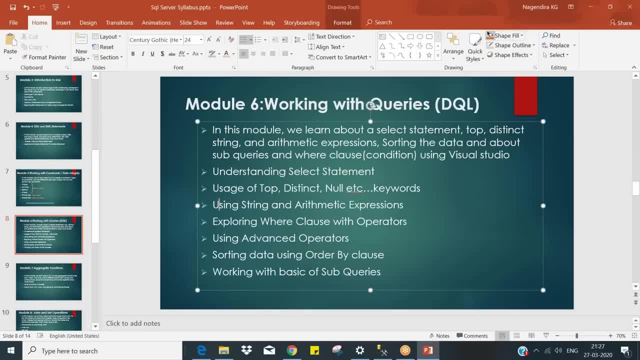 you will see some of the string and arithmetic functions. actually i thought of taking uh joints, but today i think varun has not joined. varun also wants to learn um joints, so let us focus more on these functions. tomorrow i'll take up um the joints, so 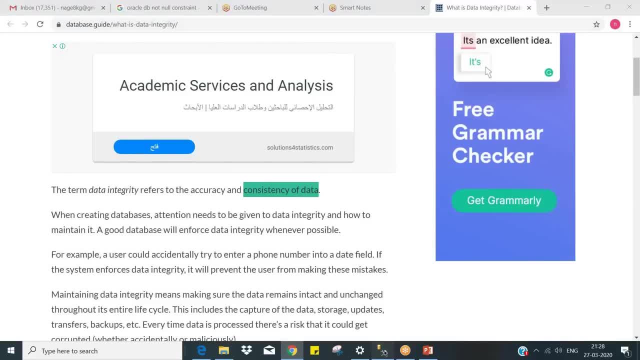 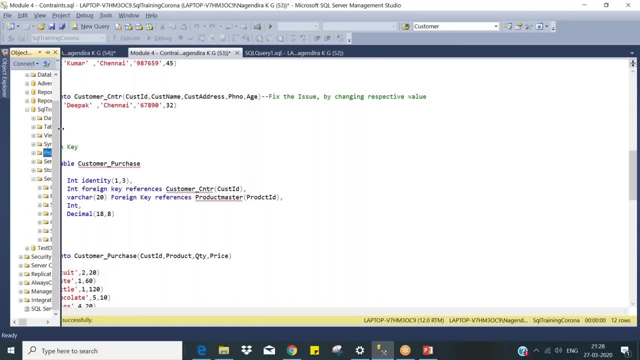 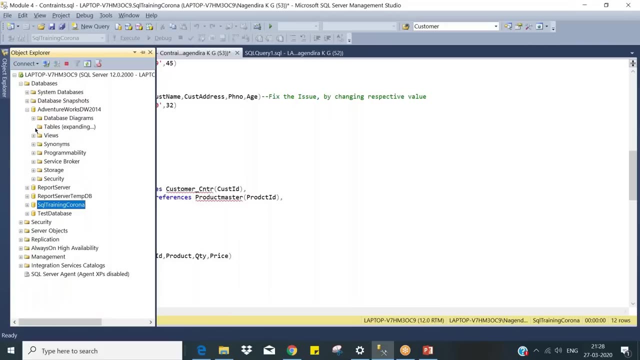 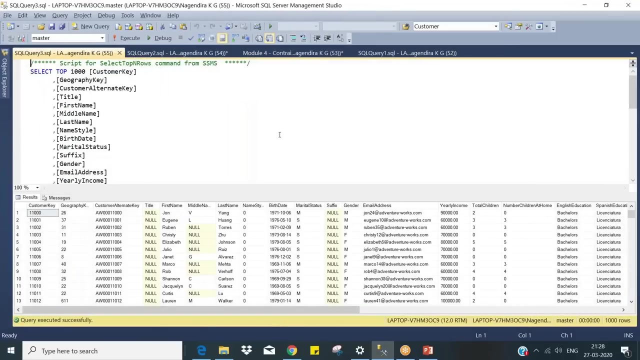 now we will stick to one table. okay, um, let us have, uh, yesterday's the big table, that we have some so that we can have multiple functions together. customer again, okay, fine. so now yesterday we saw about uh, uh, some of the operators- simple operators- in the back condition that we assigned. 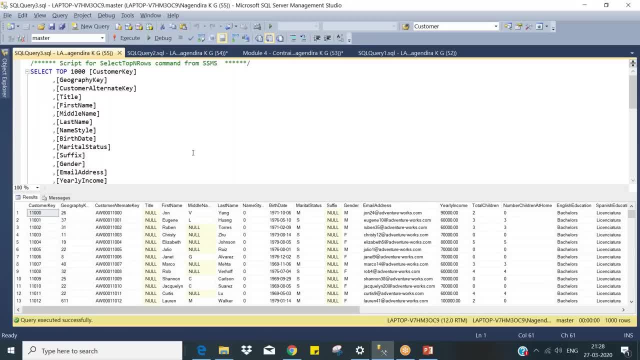 now i'm going to work on some of the functions that we have to use, always we need to have. it is not as simple as that. whatever you store, so say, for example, sometimes you may require only the characters from before this at symbol. if you see here from the email i: 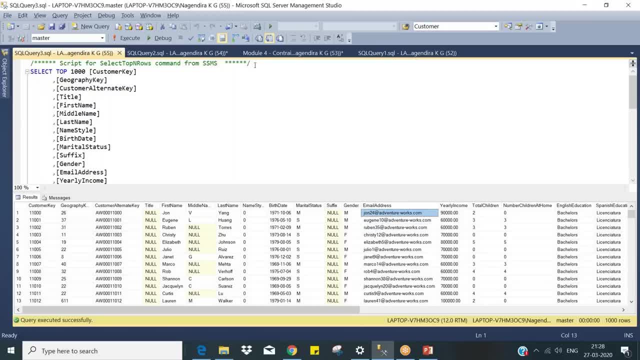 want to extract only this guy. i want to extract, before that part, this part alone. so you need to work on some kind of functions, you need to impose certain rules to it. so let us have a very simple uh example. now we can come to this extraction of the part before this at symbol. now i want from the email. i want from the email, i want. 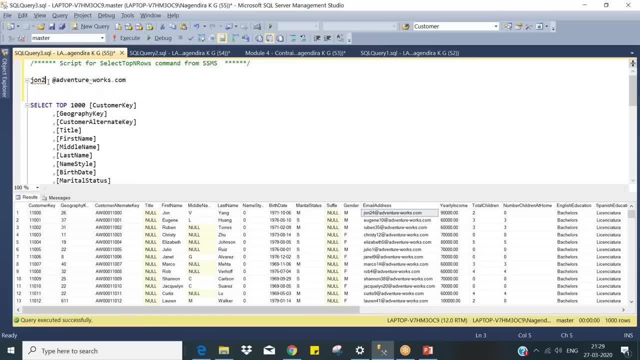 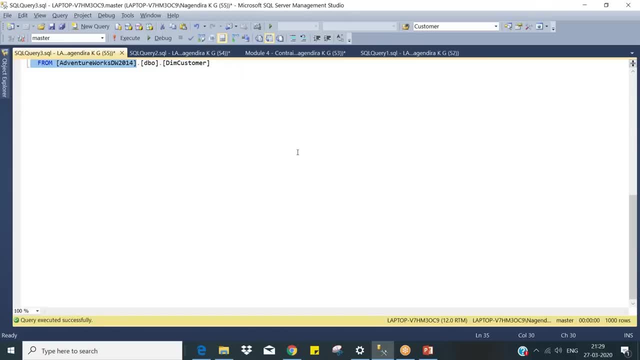 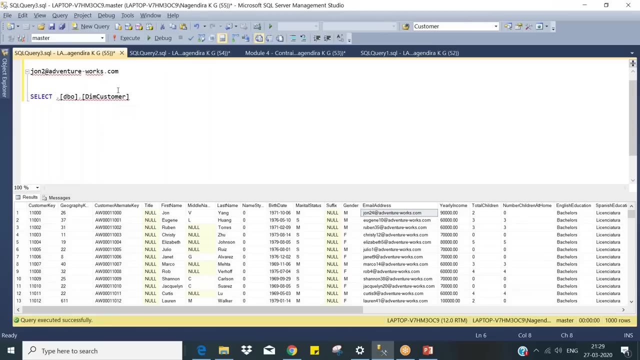 from the email. i want first four letters always to be written okay as an output. what you need to do. let us have um, we. we need to have only two columns now. i will have email address. other other columns i will do select email address here. so let's say, for a example: uh, 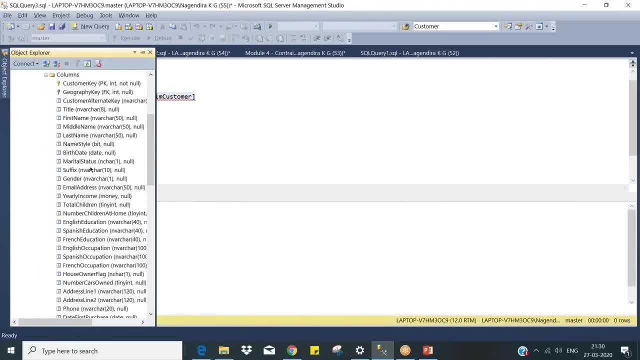 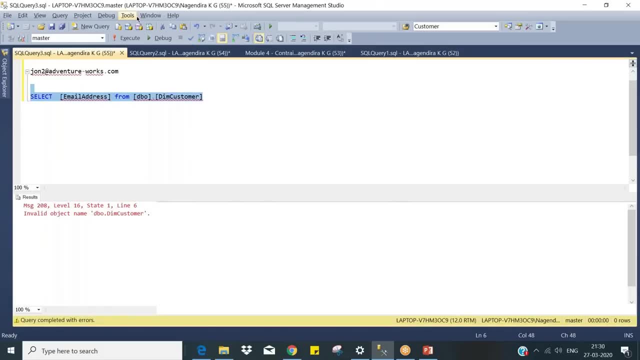 this is going to be my distributed email. wait moment to check. all right, so in order to sort out the biom axes, i'm going to work on one vehicle output, so two ves. kitchen is targeting farmer. okay, let's say, this one is our um. this so your window. you can switch between these two options. results to grid. results to text. 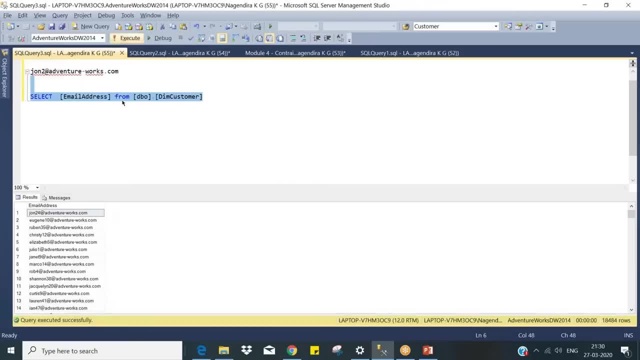 results to grid. okay, now, what i want is now: i want um first four letters from this email. so there is a function called substring. this is the substring of your email address, which column you need to specify comma 1, comma 4. so 1 is your beginning of your. 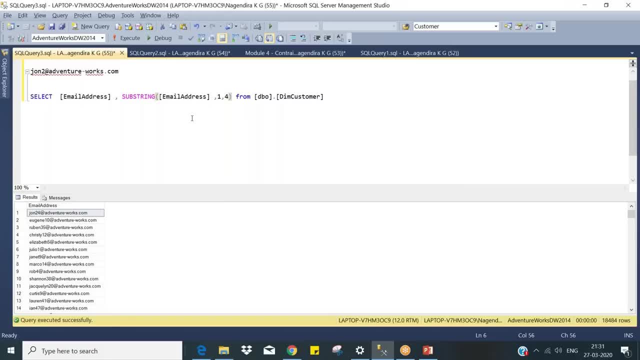 character. i mean starting point, and 4 is your length. so if i select like this, i got john 2 ego each, something like that. but i don't have. it says like no column, so to give a new column, so it is like a derived column. this is your actual column, which always have a column header and whatever you're. 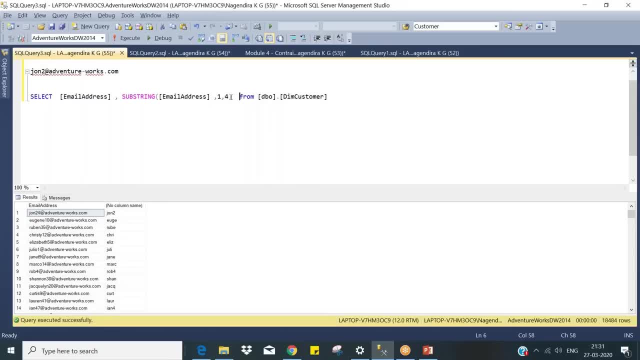 deriving. you need to specify some column name. so i will say first, first for care, or small email, small email, something like that. okay, so this is nothing but your allies name. allies name is nothing, but in going forward your queries you have, you can use this name as a reference. that is what allies name for this table also, i can have. 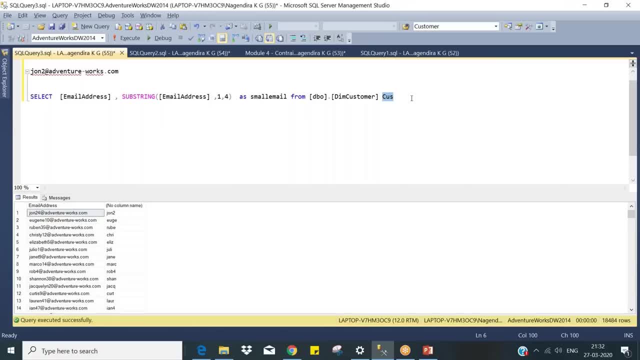 a nice name called the start name, because something like this: so this is going forward. instead of specifying the entire name, i can use this curse: this is your allies name, short name, uh, you cannot say short name, it's allies. instead of this, you use this name for reference. now it says no column. now it says small email. so this: 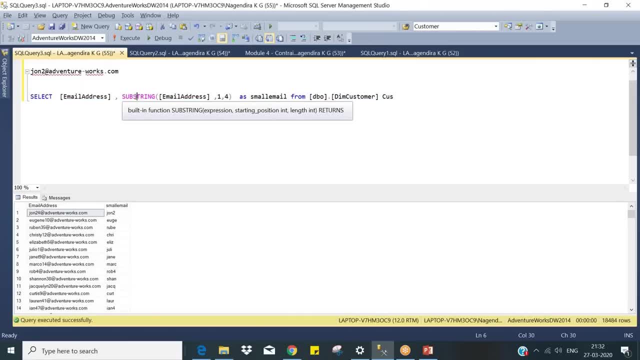 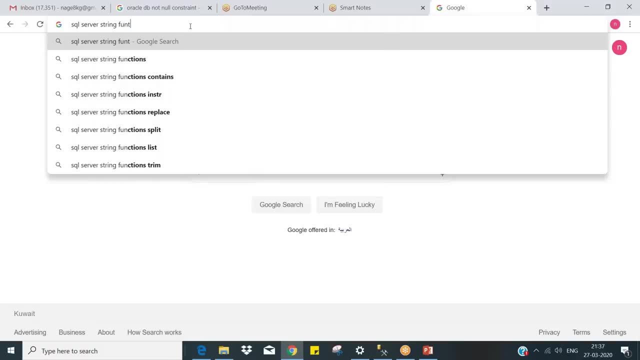 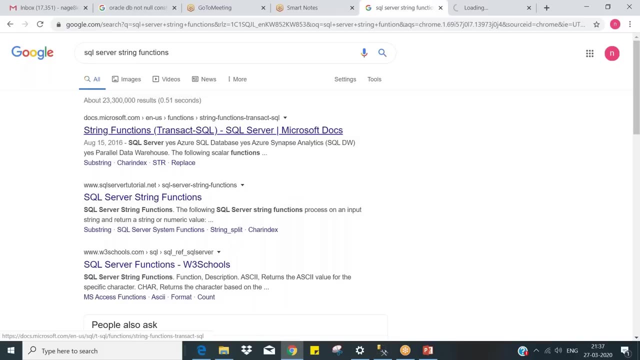 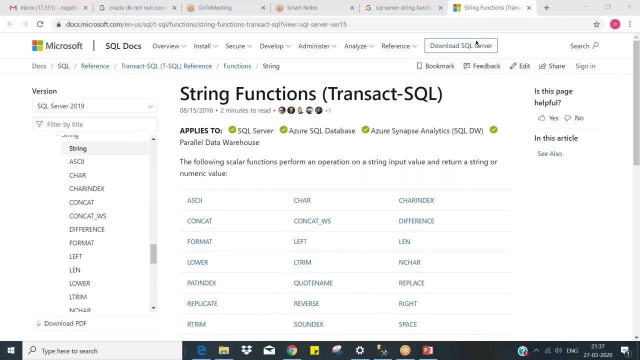 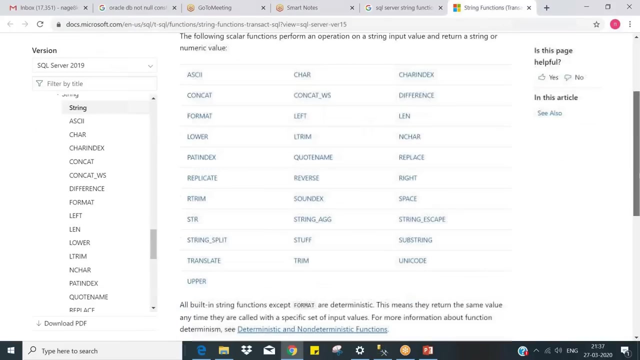 has came with a small email. so this is very simple function using strings. so, uh, you got the idea. guys, like you cannot have just a simple uh table, always you need to use appropriate functions. the requirements are very different. so now you have a lower upper r trim, l trim string split. so simple as that. 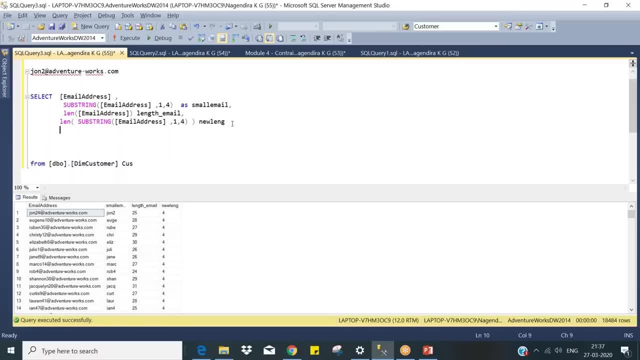 now you want everything to be upper lower. these are excel functions. you remember, guys? everything is available in excel. whoever worked in excel, they were off it, so i'm doing it for only single column. it is not mandatory. you need to work for a single column. everything turned into caps so you can use another column also, so each column you can derive. 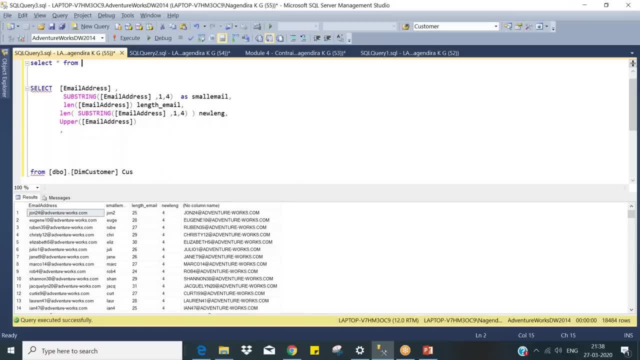 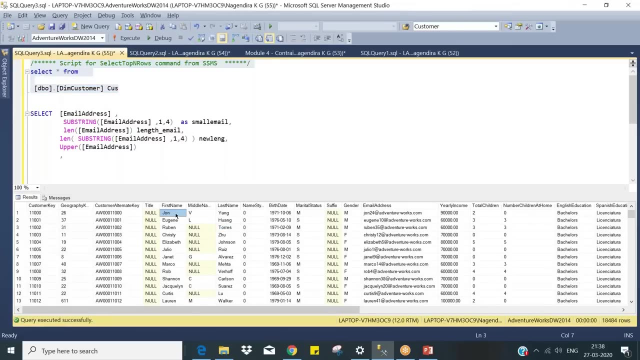 but everything works row by row. for each row, appropriate column. it will work. so say, for example: i need to concatenate these three columns: first name, last name, middle name. i just use uh plus symbol, so everything is a string. then this thing will be combined. if it is a numeric to string concatenation it will throw error. 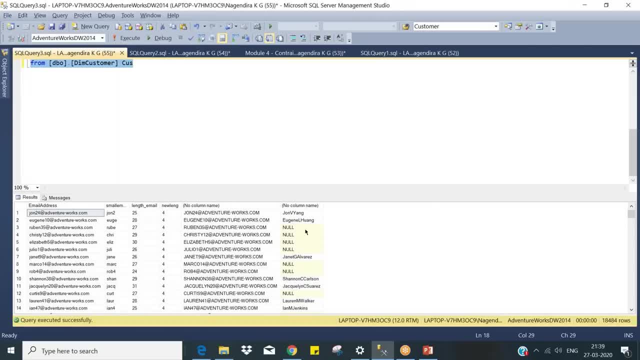 you see everything is joined: john v young. so this guy doesn't have a name at all. no, this guy has see another beautiful thing we got now. so this guy is written with null, so meaning that this guy doesn't have a name. come again. does is a output. 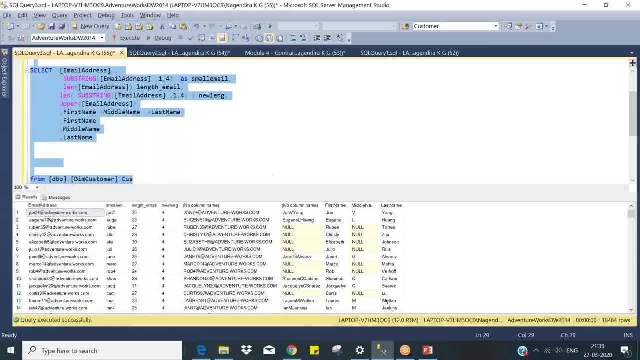 yes, this is the date of before. okay, come again. but guy doesn't have a model name, come again, come again. output something added with the null concatenate with null. then it becomes null, guys. so null plus anything is null, null into anything is null. so null is very tricky. so what? what to? 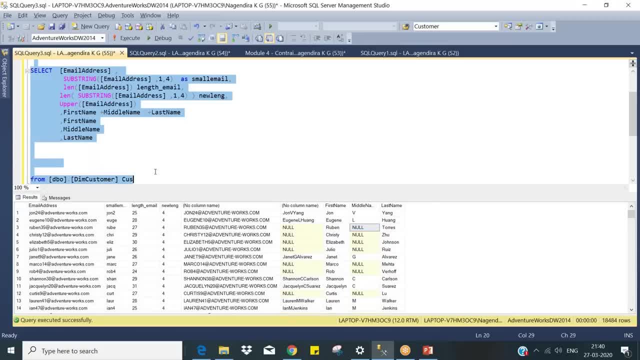 do in this case? any guess, i need to add all the three. so what i need to do if some column is null, so always first name. last name is make it as not but middle name. some people have, some people don't have. so if it is another, what i need to do i need to insert empty character here. so in database. 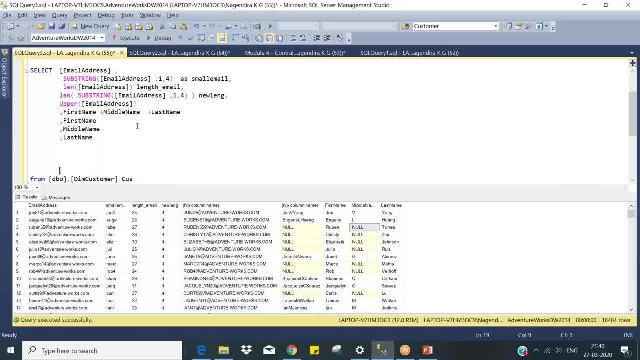 lever, you cannot add an empty character. so while giving the full name, what i need to do, i am saying instructing this: if is null, this guy is null, okay, is null of this particular column, then have some empty character. or you say hyphen, okay, so ruben, hyphen, taurus. for these guys there won't be any hyphen, okay, just times. 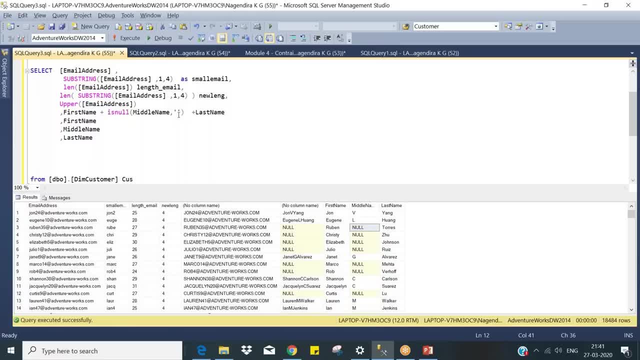 for your understanding. i i usually put, like this, empty character so you will not find a difference. that's why i put in hyphen now. now you see, this is the column we are deriving: full name. so it's like a magic, guys. it's like you playing a game. you can play with this data. usually we 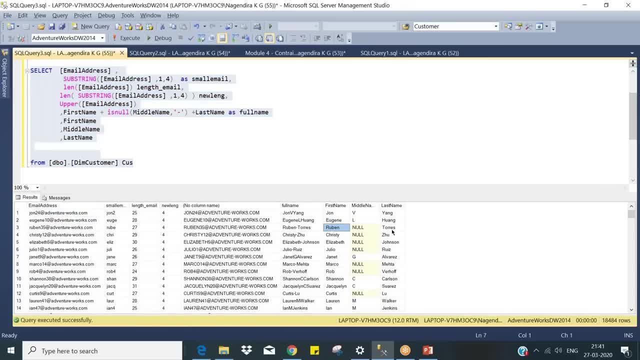 will say: like that, we will play with data. so you will see the difference here. so like this: you need to learn a lot of functions. when to use what functions appropriately, it will be used how to handle it. so most of the time we will face like that. if that we will ask: give the full name, then we 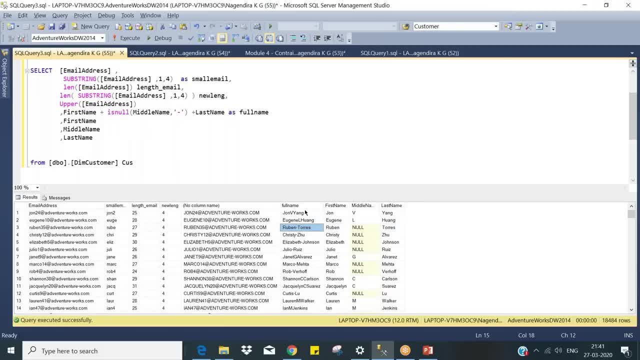 will give the entire thing without checking this character. we just need to check it and then we are things. so just check your output is correct. if it is wrong, then you need to use appropriate function. how to fix this? these rules you need to know. okay, let's have a look at some other functions. 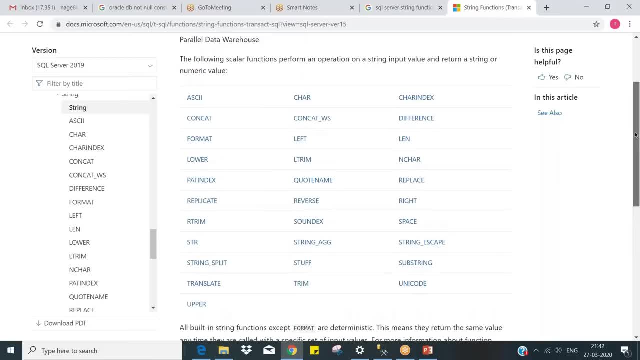 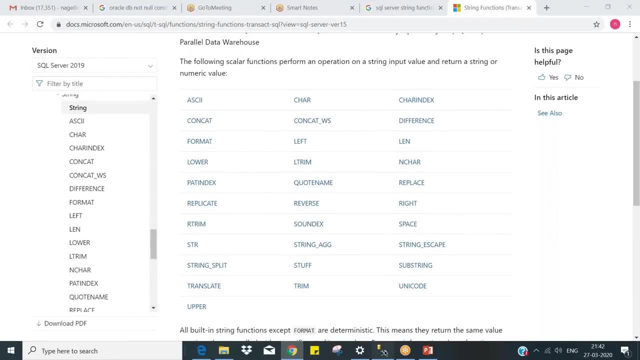 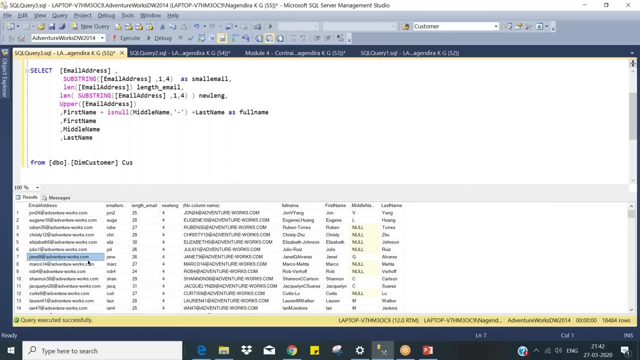 at index length: different care index. okay, care index is an interesting function, so now i want to find where this art indicates. some people will ask some you assume that is some feedback given- and some people say: like this particular string, i want to find some bird words or some things from negative reviews that, where it was there, i mean which, at what character it? 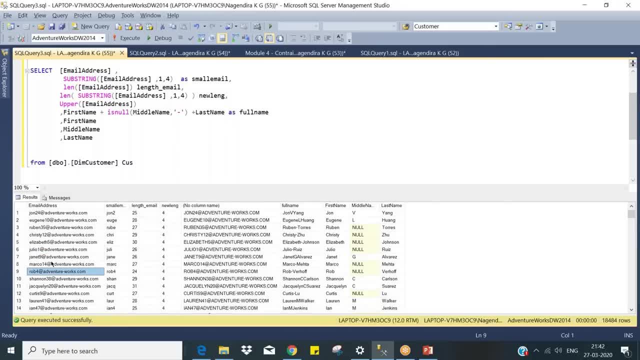 was there something like that you need to find some high form or some special characters, that where it exists, okay, you need to find one. so i use this at where this art exists. so for that car index, character index, you put comma expression. expression means you give that email address. maybe i'm not sure it can be. 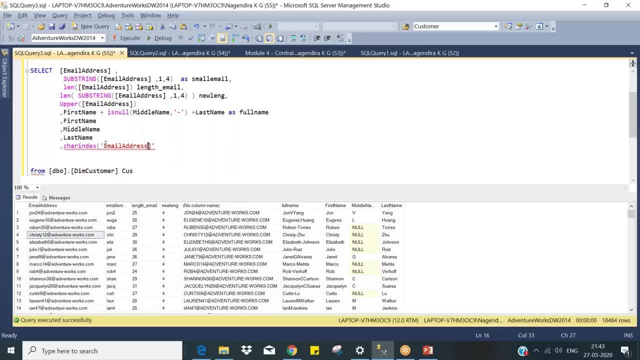 before and after. i mean either you should specify the which character you are searching for. i want to search for that and uh, it says like you need to find the syntax. i'm not sure about the syntax, i can't remember just lc expression, expression and start location. you can start. 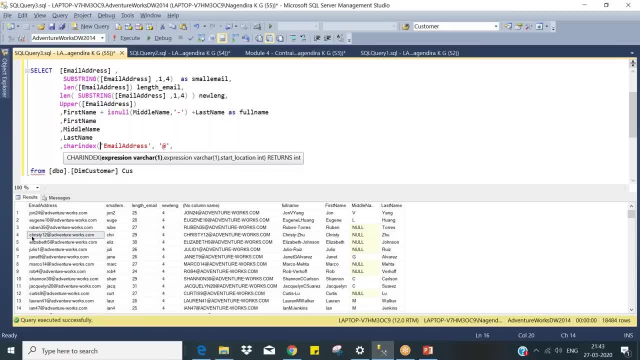 looking from uh, fifth character. you can start looking from first character. let's say like uh, one, two, three, four. see this guy, it is at right: one, two, three, four, five and it should return six. for this guy it should return more than 10 or 20.. say, i will put one here. index. 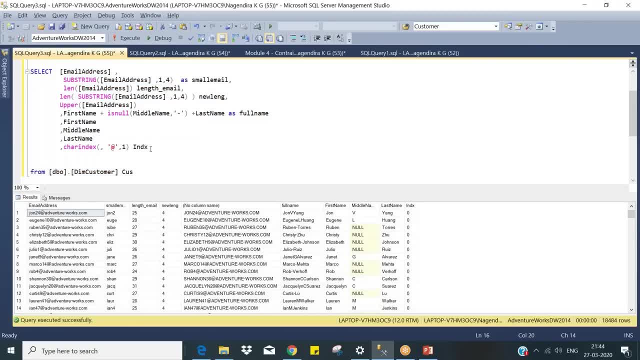 it is other way around. if it is not coming like this, then quickly i will change. so, first character is what to search next, uh, oh, sorry, this is. this should not be a course. it should be okay. let's try a column. this is the column input. okay, yes, so. 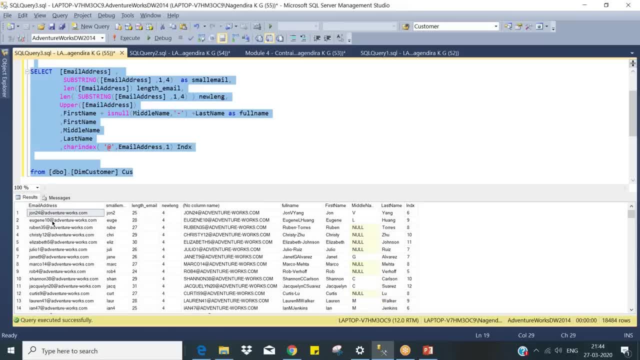 i have this sixth character here and here it is a ninth character and eighth character. when i say like, uh, start searching from a tenth character or here or maybe eight characters, when i change it to eight, these two will return zero. i mean, this will return zero, this will return one, or maybe let us see how how it works. 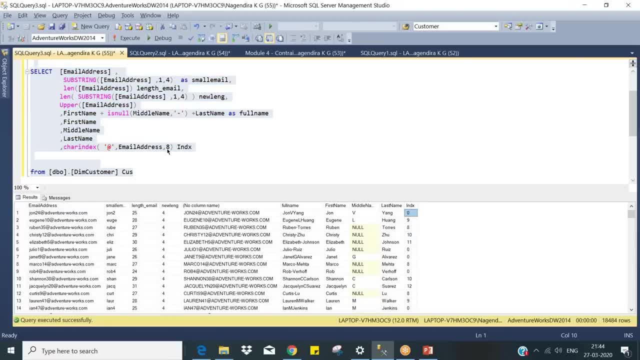 see, this doesn't find at all, because i'm saying: start the search from the eight characters, so from here. that is not symbol. so here it is: start from eight, but it returns nine, only so eight, and immediately it finds next character, it's nine. okay, so these are the scenarios that will come in your uh uh work life. so where you 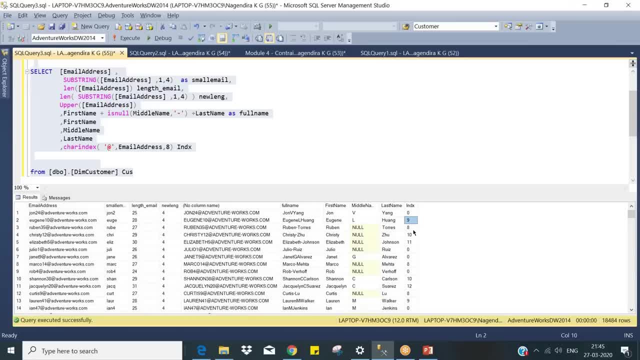 need to appropriate functions when to search, to skip, uh, five characters, then starts searching from the tenth character. so all those things, you, you, no need to write your big logics on that, everything is predefined. you need to go and search here, find appropriate functions. uh, what are the? 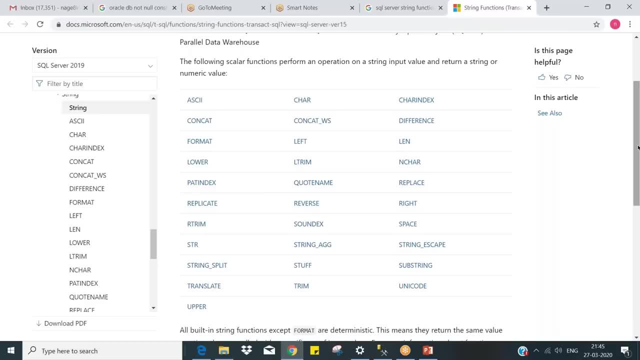 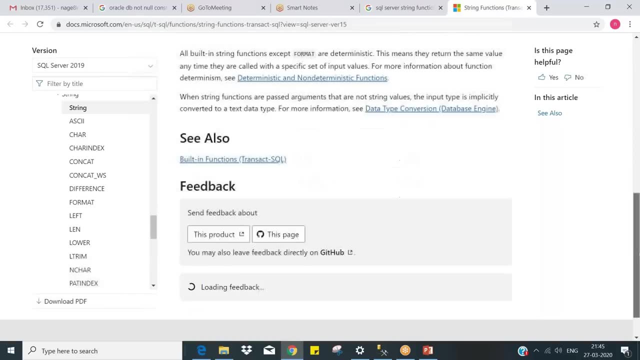 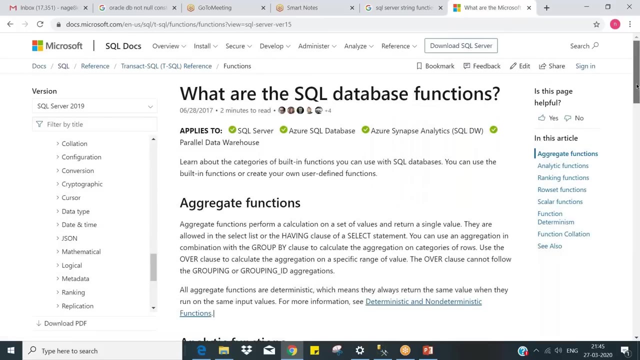 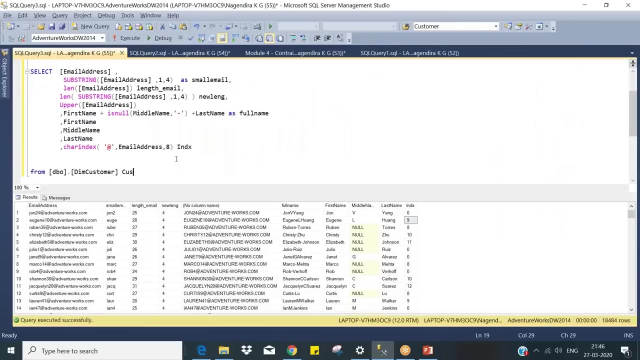 different functions available, then you will do it, that's all okay. so let's start with some of the functions that the nugget finally gave this indx right index. uh, just analyzing, okay, okay, fine. so just an example. if, say, if email address, i just want to retrieve only the at wherever, 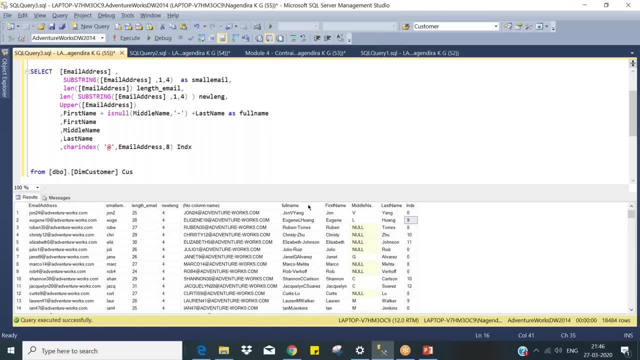 for this email that is facing at: if suppose, if anything, uh, we have some unique uh data, yeah, and some of the rows which doesn't have the unique data. in those cases, i need to retrieve only those unique data and wherever the it's not available, it can be zero or whatever, or something in those. 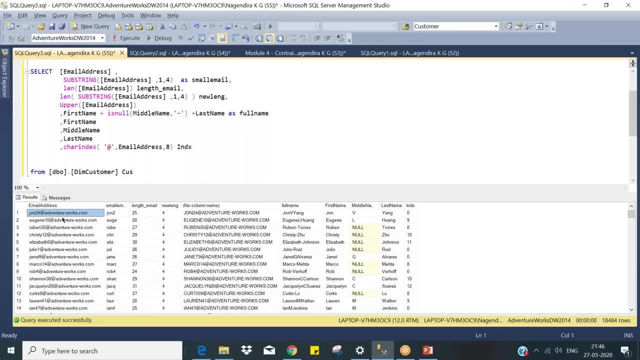 cases. how to you know? can you? can you refine your question? i mean you mean address we can say at is a unique, okay, so i need to retrieve only that wherever it's available. i mean you say you're saying i want to uh retrieve only that symbol, uh, over here. right, you need to write a combination of functions, okay. 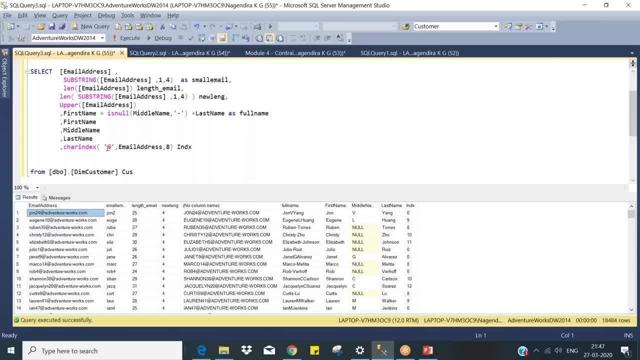 so let me uh write that query, uh, it will take uh, um, maybe at least 30 seconds. okay, so you tell me the logic, how to find. so in this case you are saying some, some, uh, in some cases you have that symbol at this expression. okay, you are having the at symbol at this expression you can able to find. 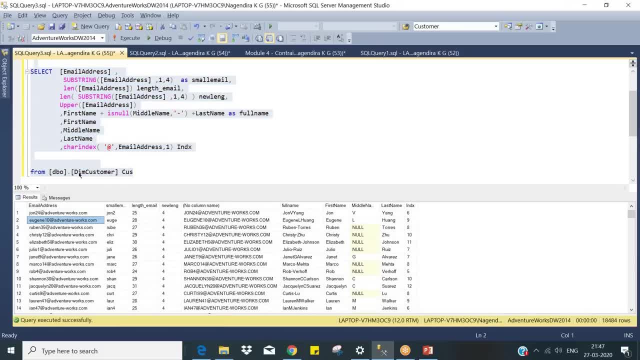 the uh position of the uh symbol using this current index. now i want that particular character, okay, in this position. so this should be the input of another function. similarly, what we did here, substring is of uh input to the length function. so now i need uh character index of this particular ad and i need the character in that. 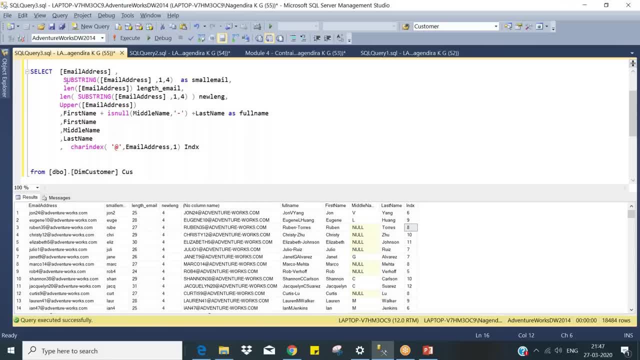 particular uh position. okay, uh, it is again. we can use substring here, i think. so substring of this will return the sixth position, right? so this is the starting position of the substring. okay, so substring. what it will do is so, in this position, you need to give this input and how many characters you want. only one character. 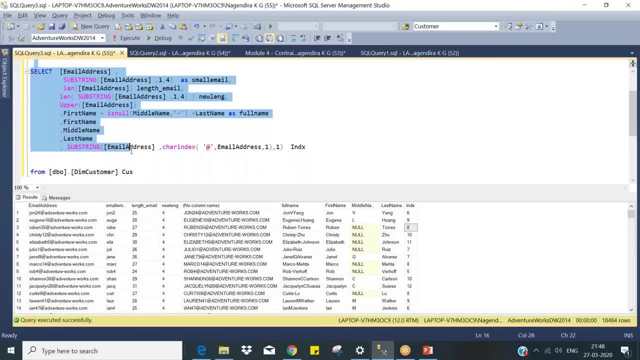 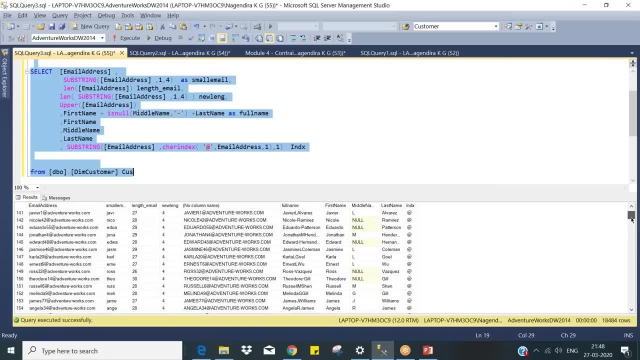 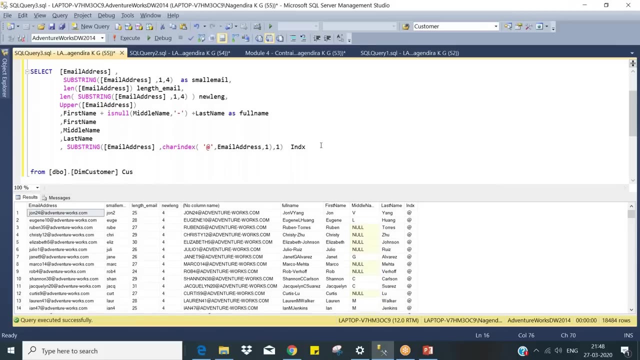 yes, that's the thing. so it's just a programmatic approach, how you work, okay, okay, okay, so you we need to use a substring, substring combination. it depends, uh, based on the scenario, how it has done your requirement. your requirement is: now i want add symbol and using 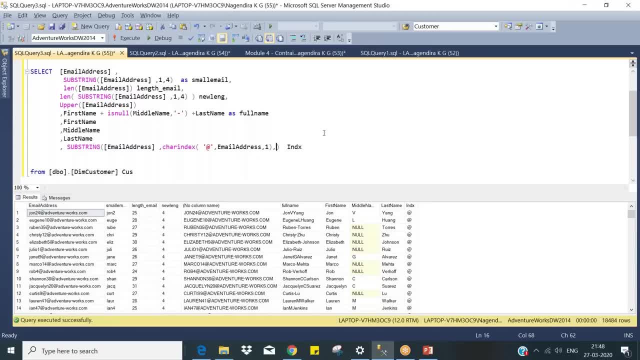 this: if i use two characters, three characters, i mean three characters- from that symbol, i can get next three characters. okay, is there any like? uh? yeah, i don't know whether it's in uh, microsoft sql or not. similarly, we used to give right like equal to this. yeah, like like percentage. 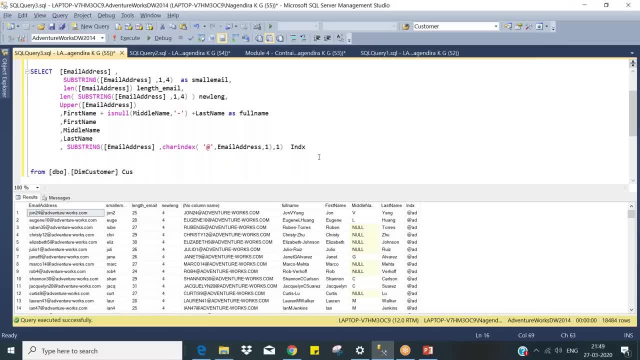 in that condition we can use those things. so it's like it's not like a like here, like it's used for something else. i will come to that condition now. so i just i want to cover some more functions in integer. then i'll go to like and where, conditions. what are the other combinations? 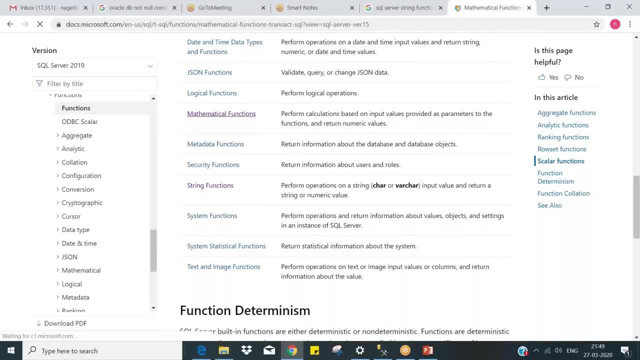 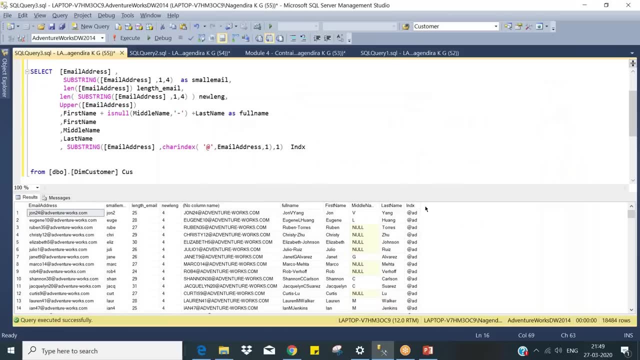 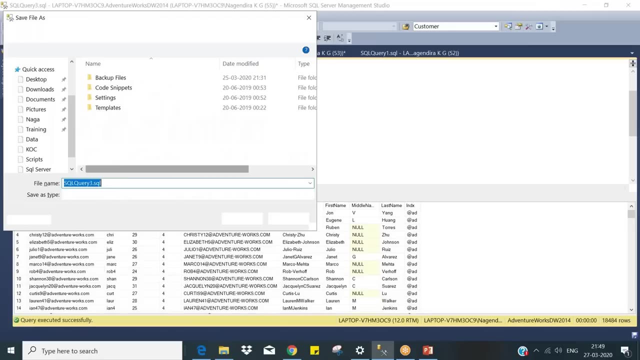 so i don't think: um, okay, math, math functions. so all the functions with any programming language, whatever programming languages you you use, those things will automatically applicable here. so what i'm trying to tell you is: let us save this guy as string functions, scripts, string function maybe. 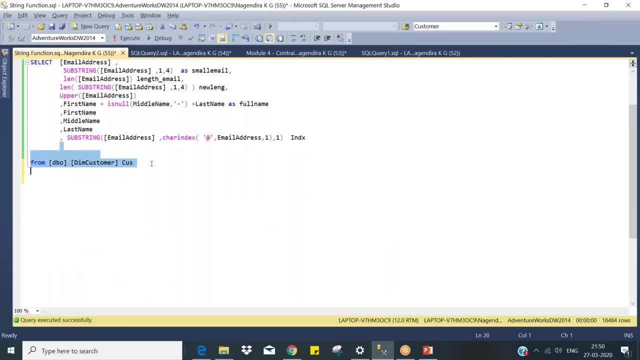 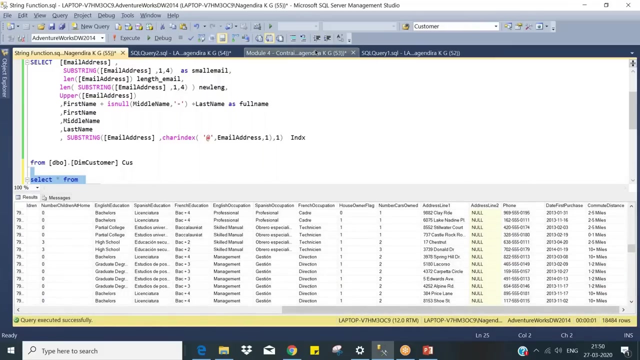 functions and say, okay, so everything, you can work only with your table. so there is no way of working any anything else. you have a p? l square there you can have a little bit of programming. i don't have any decimal values here. going back to our module right here, because we have 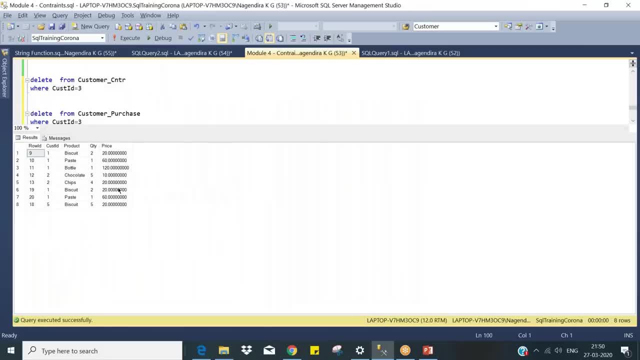 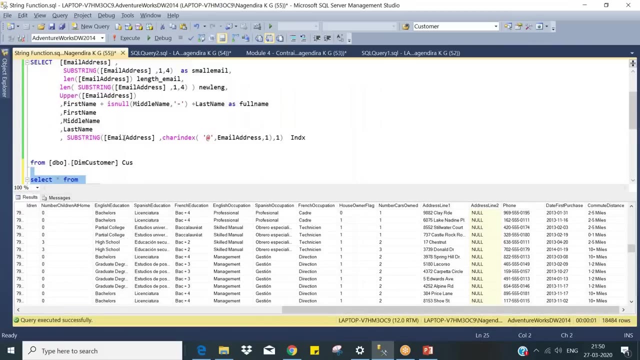 some decimal values here? you know, no, no way. why 28 comma decimal numeric. i'll finally try to fix that one. let's have um. okay, so let's, let's have a, some addition. you want to add these two, just one or two, this column plus this column. you can add it like this: so if it is string to string, then 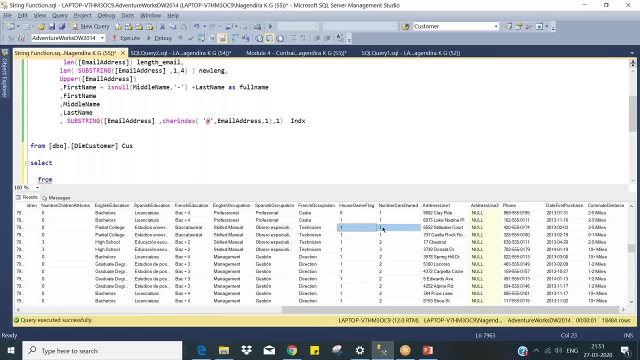 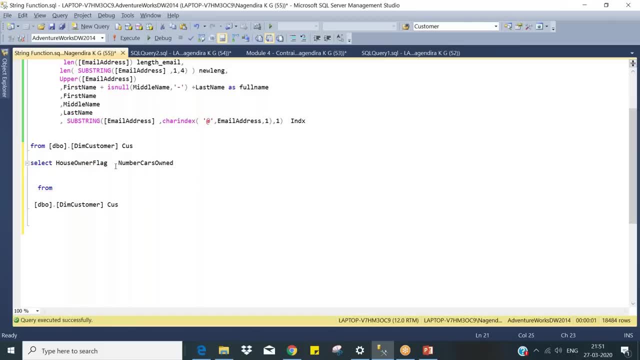 concatenation will happen, then if it is a numeric, then your addition will happen. so this is one comma, one. also- this should not be summed up, we don't know, just i'm saying so. so this will return only the values after addition. so just you need to ensure whether 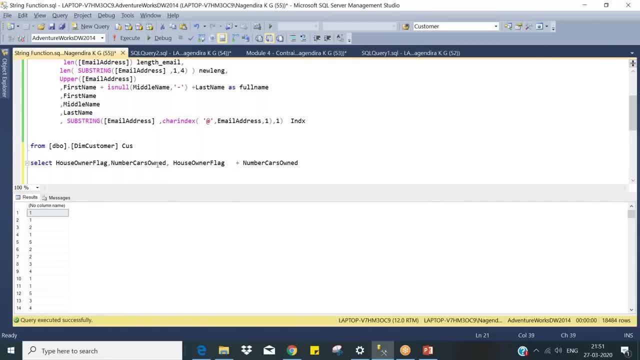 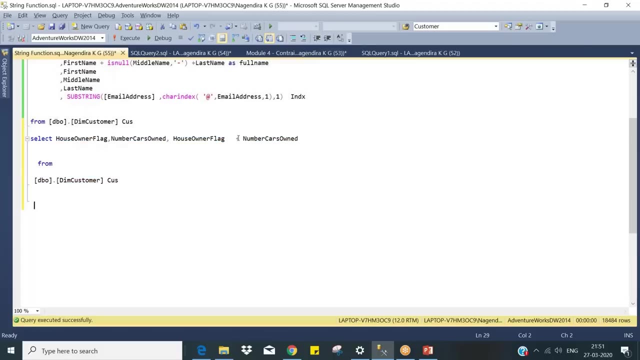 it's correct or not. so keep those columns before uh doing the calculated column, computed column. so i was like: one plus zero is zero, one plus uh one is two. so you are returning a correct values. so simple addition, subtraction, arithmetic operations using a row by row, you. 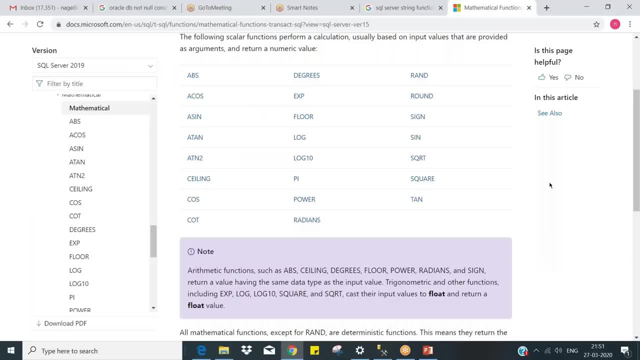 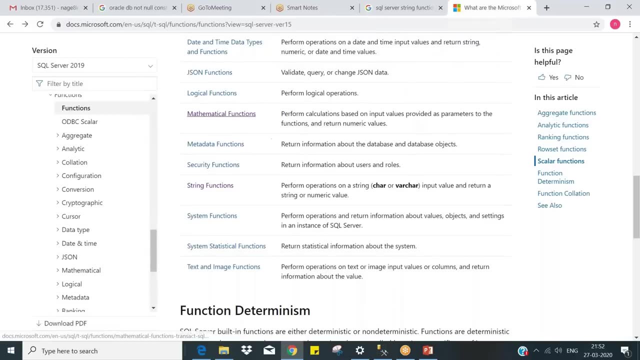 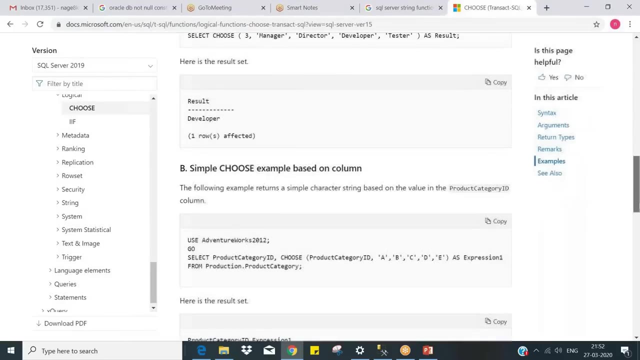 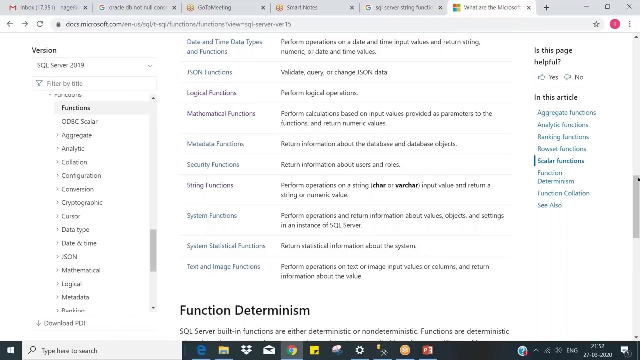 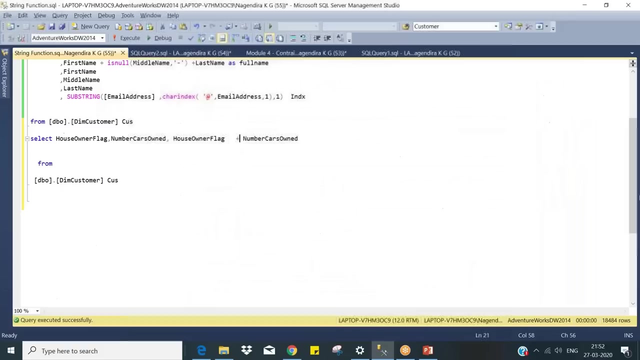 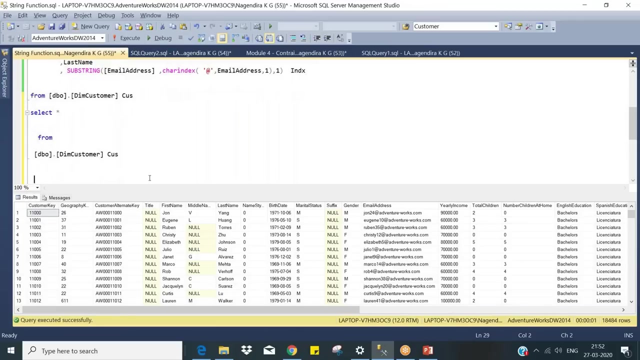 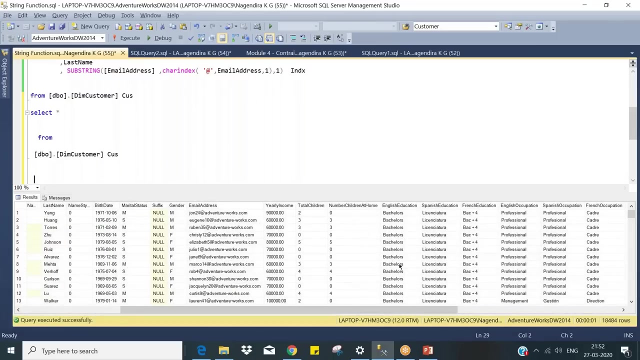 can use this one, okay, uh. so all other mathematical functions also- you can compute, wait, logical function, choose- and are not required. these are not uh for us. okay, now let's focus on uh var condition. use it like so. so now you have uh here. select star from dim customer. you ask like var condition. so when 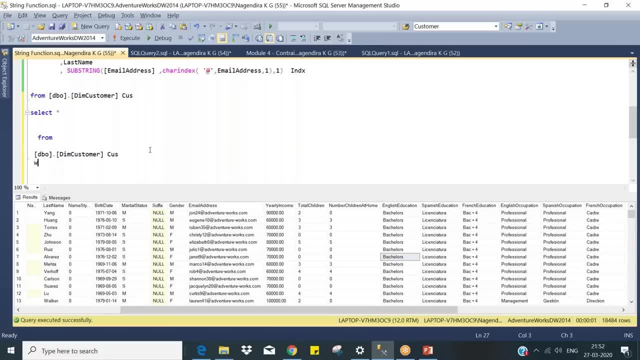 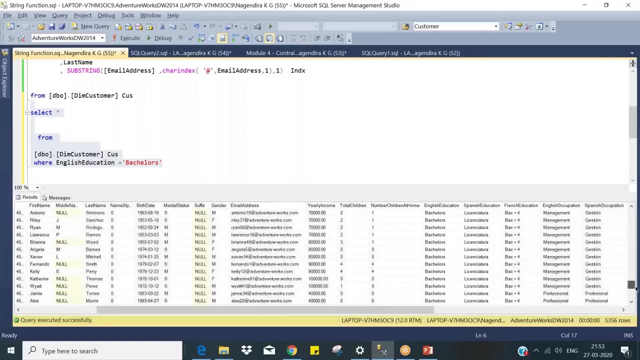 it starts from. so if you say like var, english education, equal to, you need to desperately specify bachelors. then you need to specify uh equal to symbol here. but most of the time we are not sure what is the spelling over here, whether it contains a proper value. you need to search in appropriate approximation. 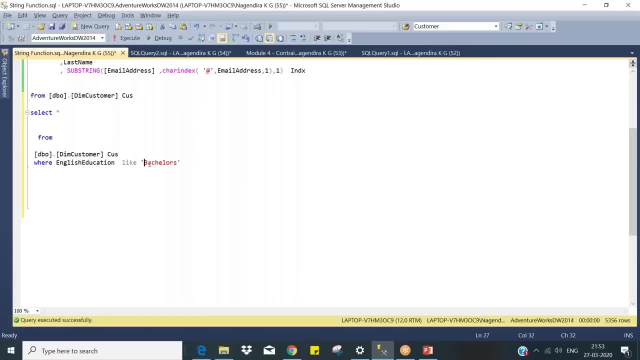 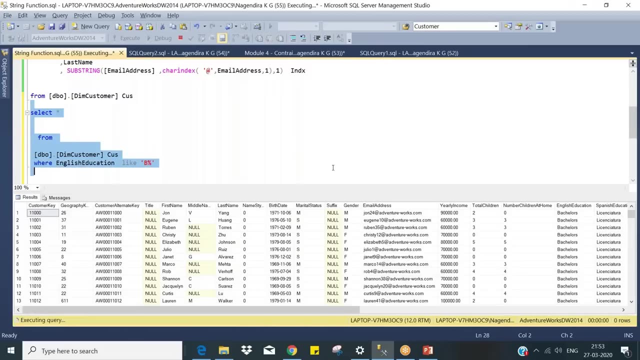 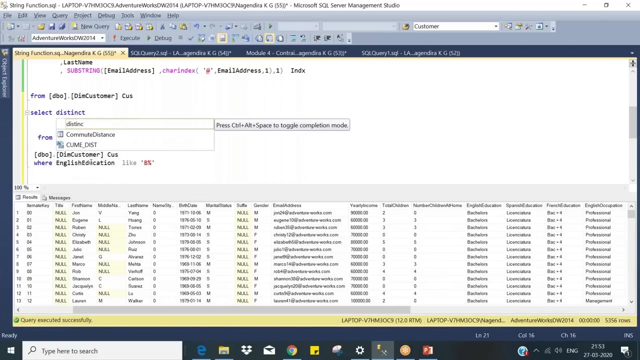 so in that case you can choose like. like it starts with b, b- then you need to say percentage. percentage means it can have any values after that. so so whichever starts with b, all the drawings will come. let me put distinct here, as we see yesterday, distinct english education. 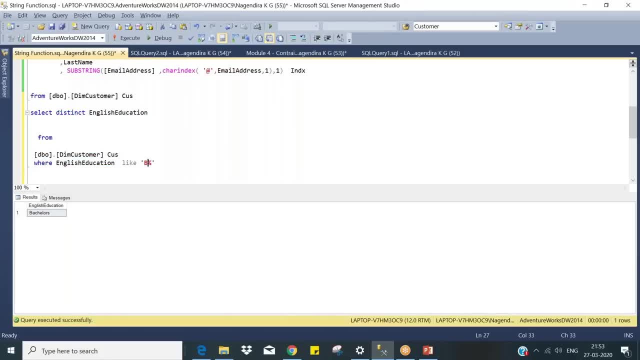 bachelors only. so when we say c, no, english education starts with c. let us see now you have partialize franchise, the branch aсьuxir switch. we are not searching it, just looking at what it says. at least it shows engl c, partial high school and partial college. so when I put here that starts with P, 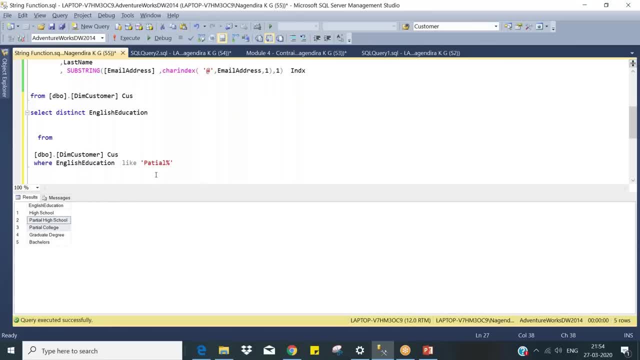 partial. okay, both the things when come. okay, my spelling is correct, wrong, partial- only these two will come. so when I say like little bit further, I want only starts with C, it can be a college or high school, only C will come. take some time. only C is coming. I am excluding the edge, so this is the way. 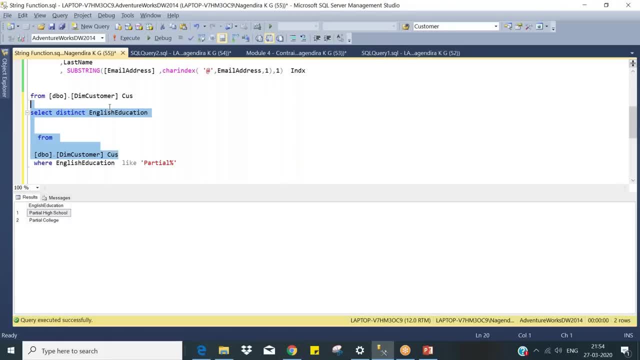 how it works. now I want in between the text with the common okay, that contains all in any of the values. I mean in between any of the texts like. what I'm trying to say is: I want the English education where it contains a text like: Oh you. 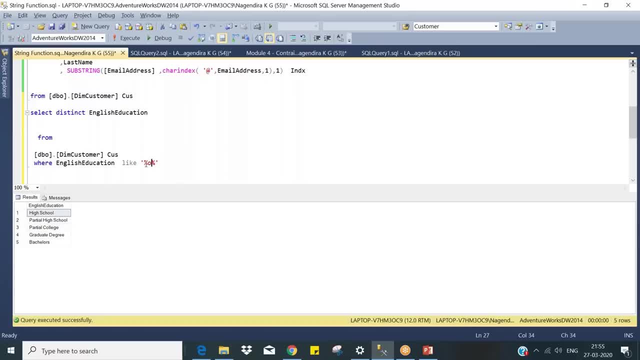 so you need to put percentage before, percentage after. so, Oh, wherever it is, it will pick it up. so it excluded some other part, like if you see here, and graduate degree doesn't have all, so it excluded it. it brought me four cases, so this is very important. 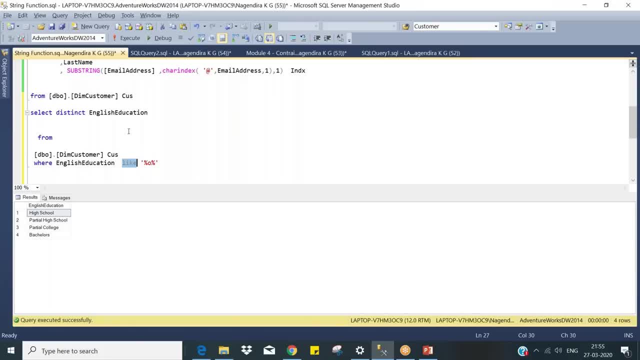 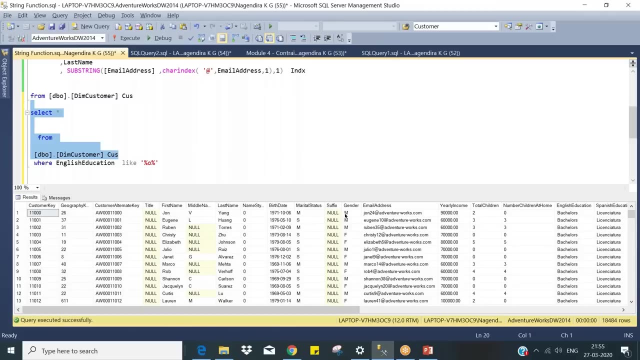 so I'm going to show you how to use the function like, like condition that we use. okay, yesterday we saw about all- I mean yesterday, our previous classes. I mean unconditioned, let's say, like I have a male gender and who is having a salary of 8,000, and what about when I have a male, or he can be a married or unmarried. 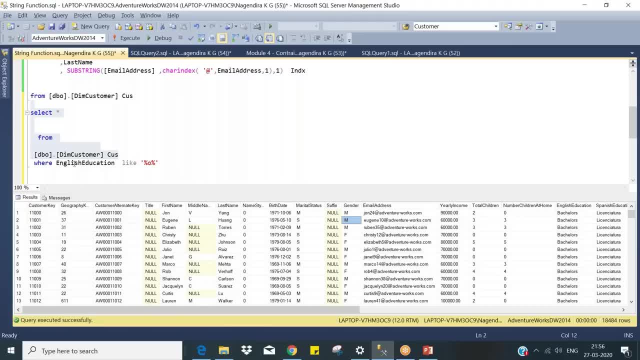 you should use R condition condition also. so whatever functions you use- and and or you- you understand the difference between under all right. if say like M and S, so it should be M equal to yes and the M and S should be there in this, both the columns. and if you say M R S here, M and R S means it will pick. 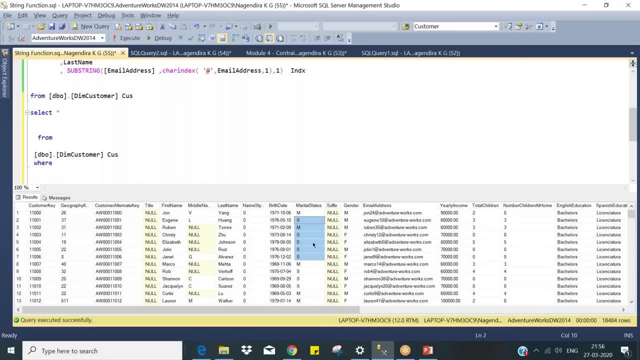 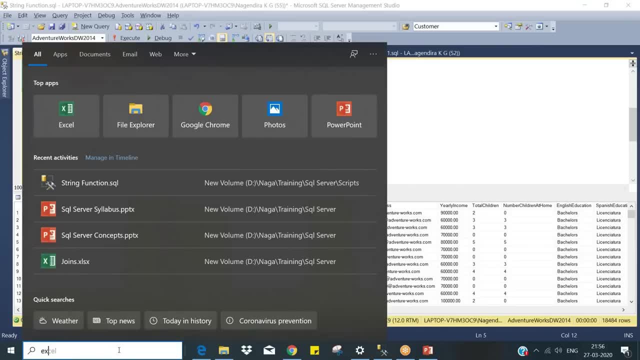 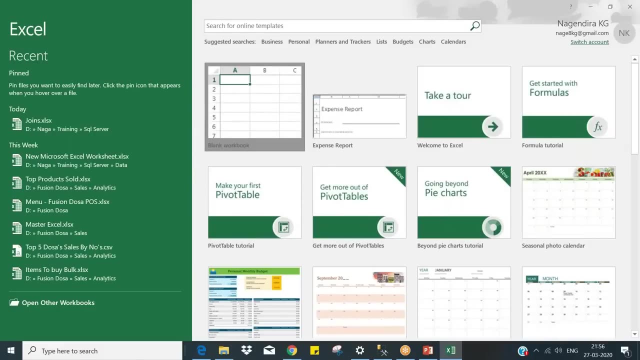 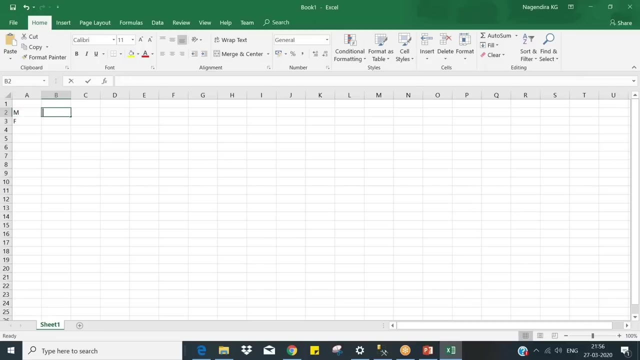 up all the M's here, all the ss here. in this case let me take excel, the difference between and and or- I don't think you need to work both on this. let's say male-female here and use have yes and T values, so the possible combination of x, y and z to have the amongst values, carrying out, for example, the give or take analysis. 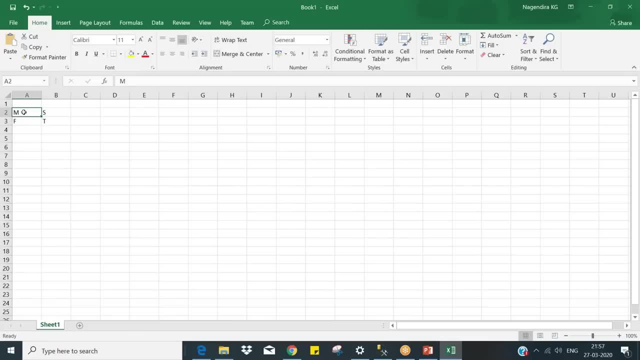 of these two is nothing, but you are. I will repeat this guy twice: okay here also. yes, also T and T okay. so unconditioned means I say like M and S. only this row is returned when I say M are yes, okay here. it's a gender. it says: 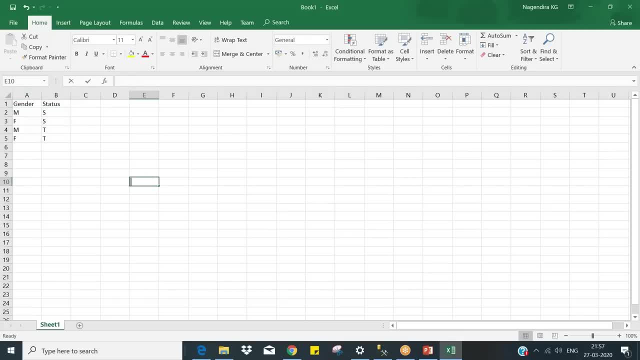 like status. you consider status. when I say gender and gender equal to M and status equal to yes, then this will return only this row, okay, M and S, and means it should match. this also should match if I say, like M or yes, gender equal to M. so this will return this record because 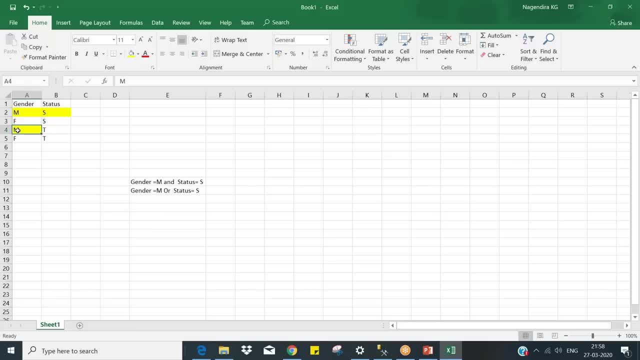 of this is true and this will return this record, because this is true, then it comes with it. checks status is yes and obviously, if this is true, because of this reason and this reason, and this will also return this record, so it will return one, two, three records. so this is the difference between R and N. so you need 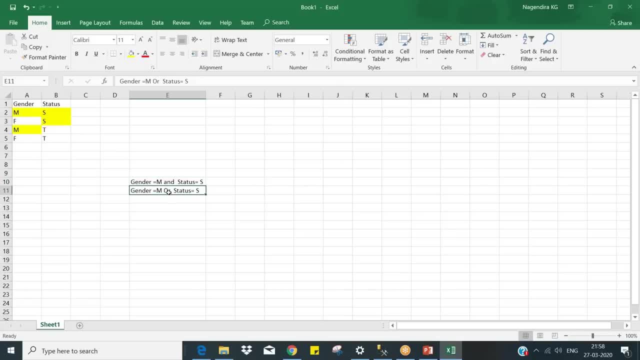 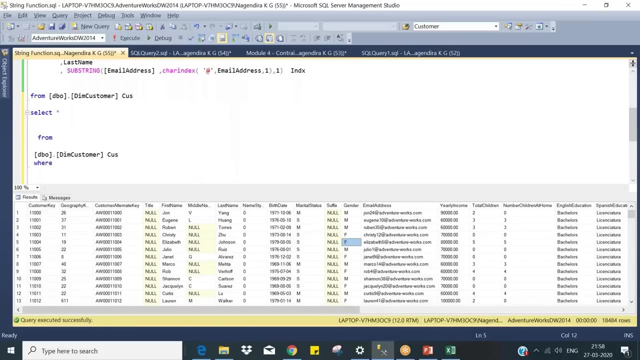 to be very careful while choosing and condition and our condition. okay, so for each column it will keep on adding a true or false based on that. either one of the true, then it will go. it's a generic. I mean you, we have studied in some trigonometry or mathematics. it's mathematics rules. okay, I hope you got. 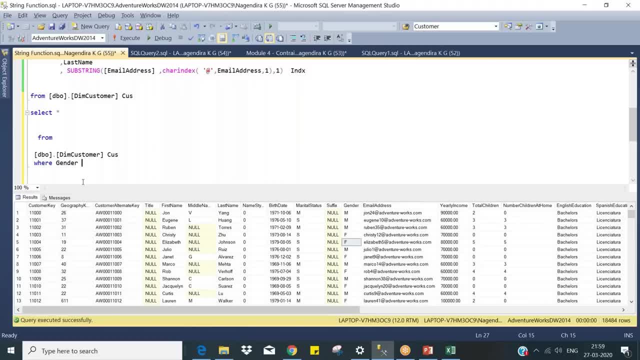 the point. let us try one equal to jam. I'll put our Malaysian status equal to yes. so this brought me both M and yes. see, now you see like here i have brought efforts away because this becomes true. this is: yeah, i want male gender only, but this for this condition it becomes true, and for this also true. and if i say and 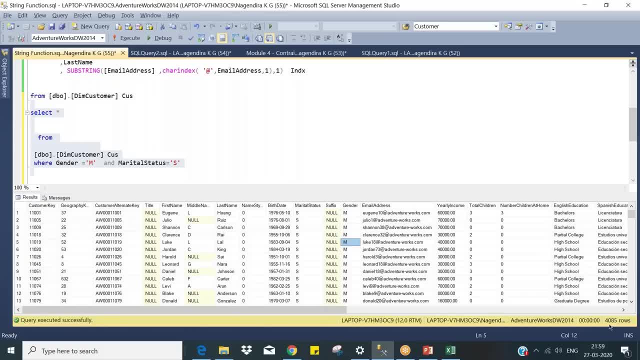 so all the records, the records drastically increase four, zero, eight, five. okay, got the point this. so this is the crucial thing: where, in that condition you can have multiple com combination, you always go for and rr equal to and any greater symbol. even you can have this functions care index of these functions. you say like what it will return. 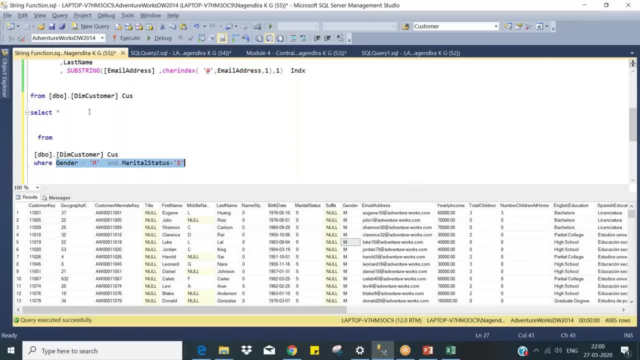 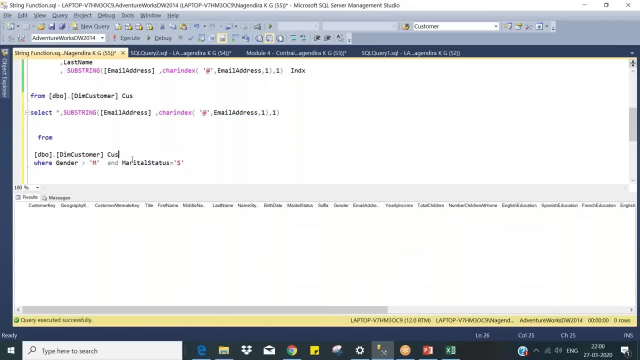 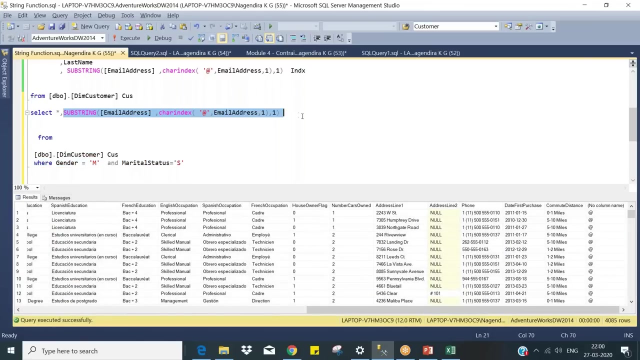 it will return at right. so you say like, uh see, see, guys, what i'm trying to say is why? so here you have a trade, same function also i can have. i mean, you can write a function also over here. let it be like this: and i want whatever character having art. if you say like, you find some other characters, that character. 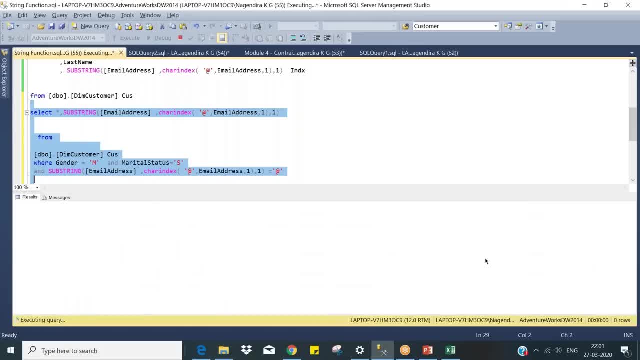 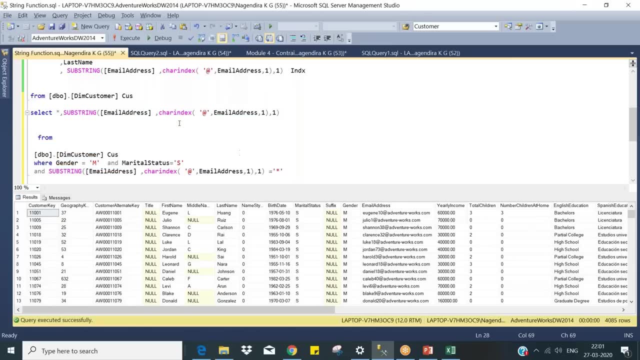 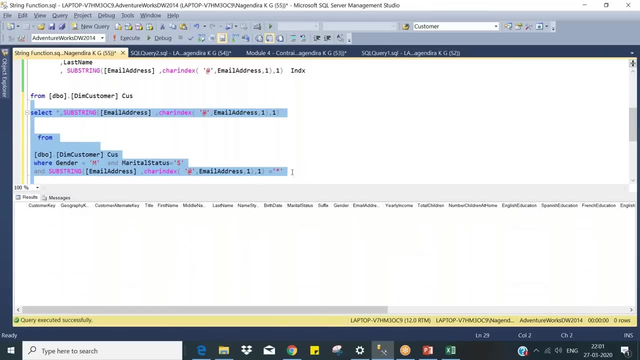 alone you want. then you can get so same: four, zero, eight, five. if i change the symbol to something else like star r8, star output, it will not return any of my record, okay, so it's like how the character is how you execute each row. it will go and check this condition is passed. this condition is. 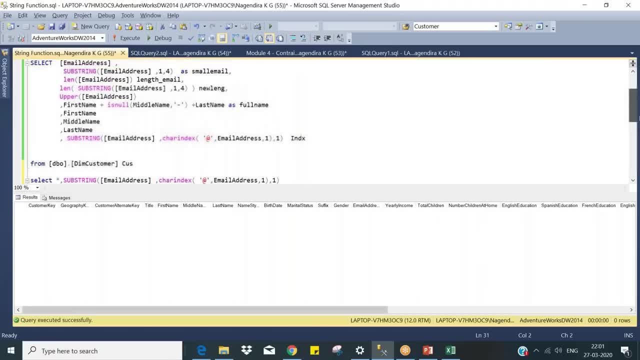 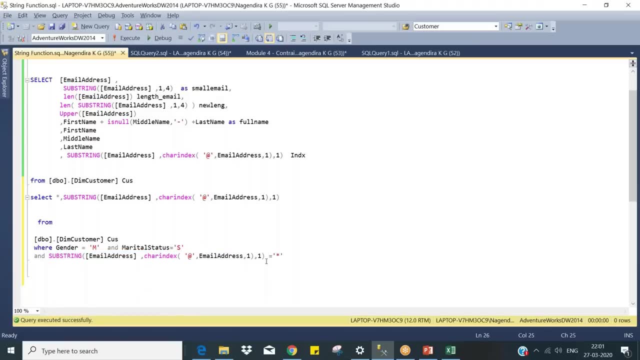 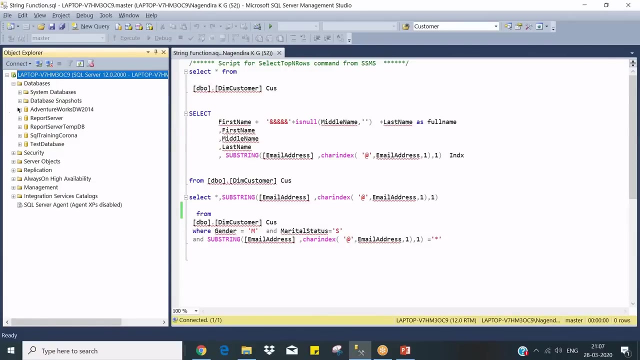 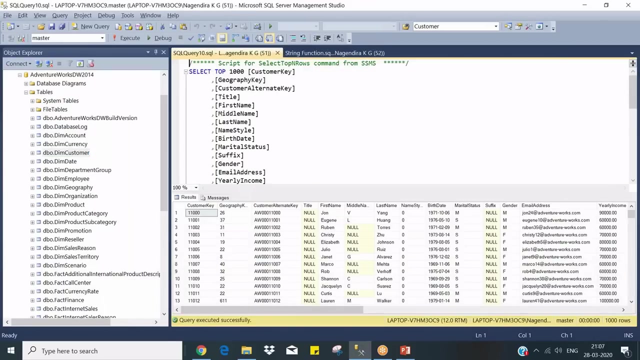 passed and, after returning, whether this condition is passed. so either you can use the functions in select class or in the back class, it doesn't matter. okay, guys, with this i'll stop here. everything. so we have a customer information and, as i said, if we need to get some information, we 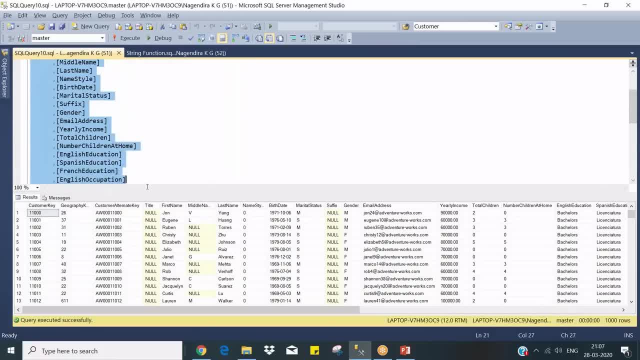 always need to work on select queries, that is, dql queries. so, based on the requirement, people will ask different queries and using our select statement, using var condition, we'll filter the records. we will use different condition and or combination to get the results. so we saw about these operators equal to. 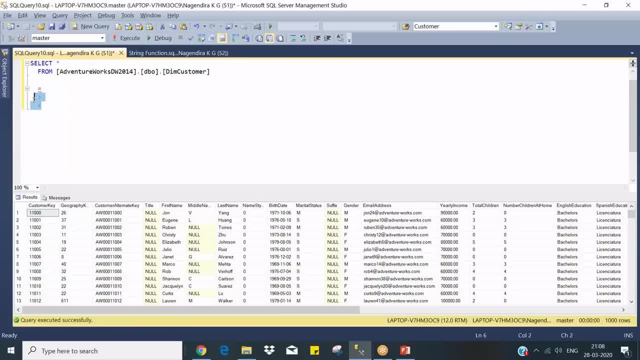 greater than less than. these things are used in numerical values: greater than 100. less than 100 are greater than or equal to like this, less than or equal to like this, and there is some cases you need to filter with a range like date of birth: whoever born between 1970 till 1980s. 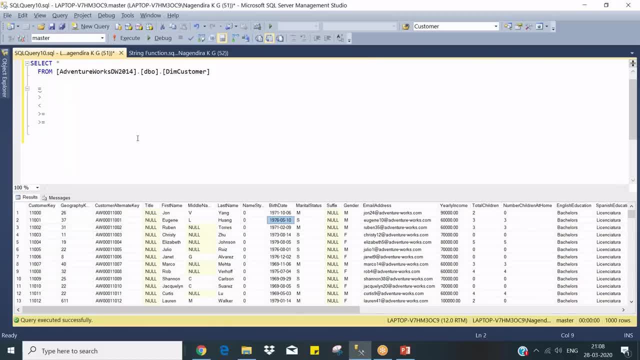 so you need to get the between the range. okay, so for that cases you used between is the keyword or operator vc. so let me have that query where now the scenario is: you need to get the list of customers who has born between 1970s till 1980. okay, so for that case you can write different. 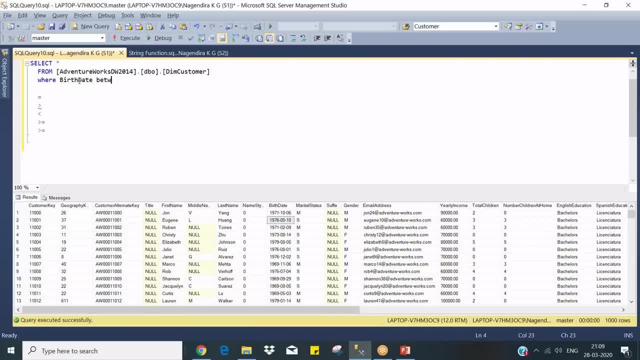 one of the easiest way is like writing but date between. you need to mention two dates: 2000, sorry, 1970, zero one, zero one then. and so if you use between then, you need to use, and obviously so 19, uh, what you need, both the dates are included. okay, so you need to write 1980. 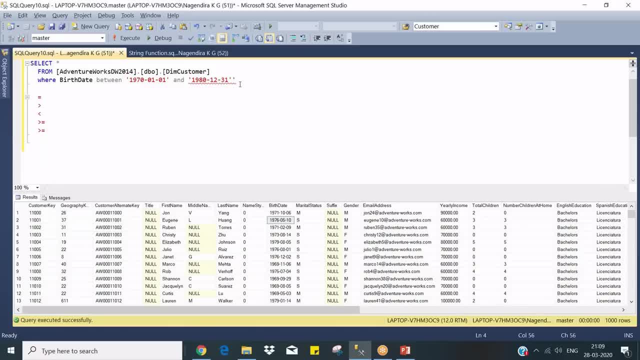 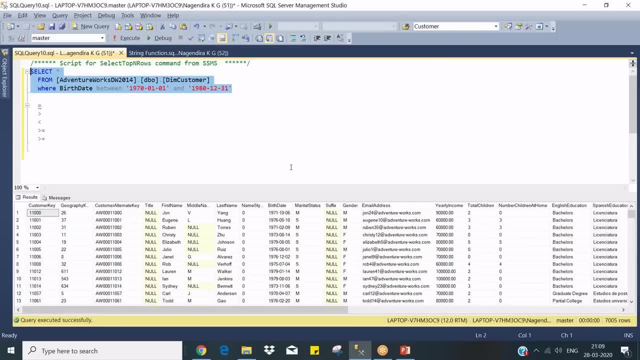 to a 31, so this data is included. this data is included now when you use this one. so there are seven thousand five customers who has born between this decade 70s. okay, you can see quickly: 79, 79, 75, those things. okay, only it's between this range, see even 80 april. 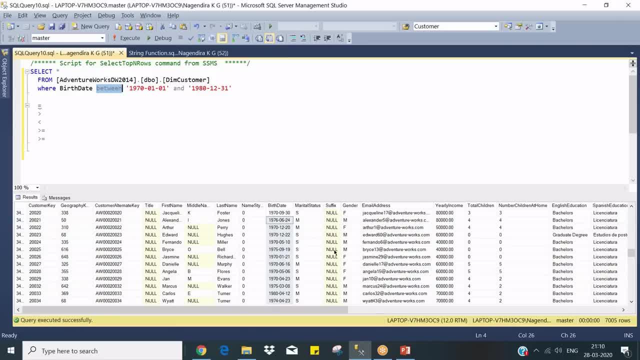 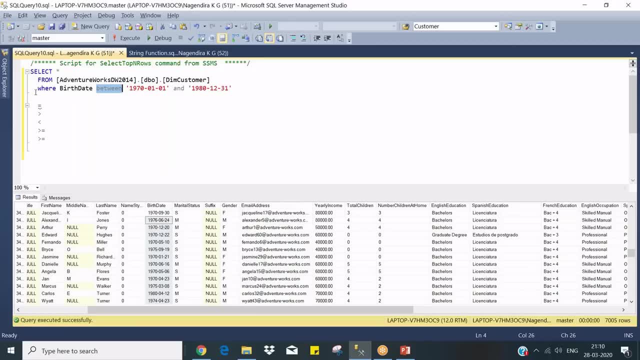 so this is the about between keyword or operator. now there are certain things, like earlier, we used to query using a equal to operator that filters only one particular case, like: if i want only the bachelor's customer, or as a bachelor, then english education equal to crab crab. 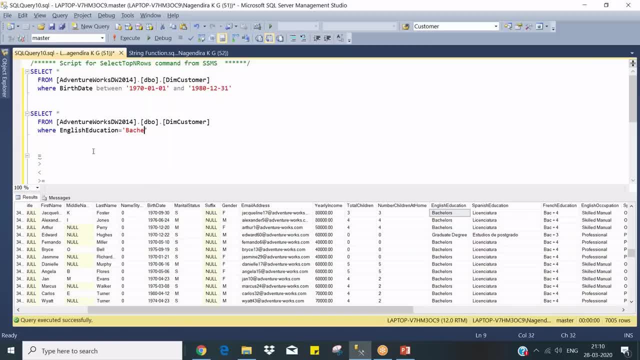 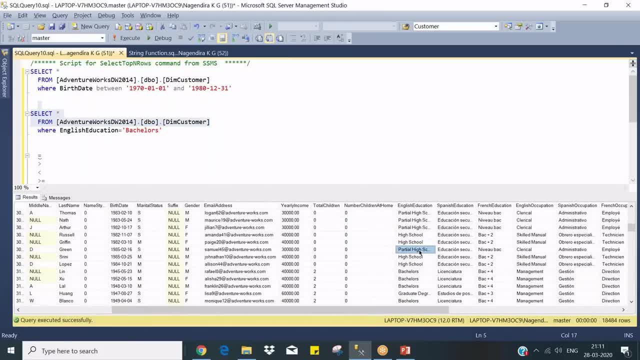 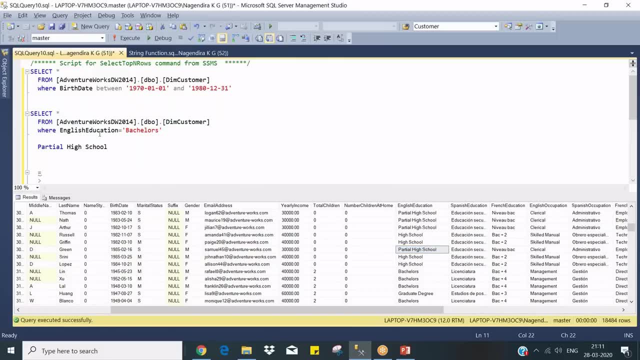 bachelors as well, as i need something like who did the partial highest secondary? so i need both the cases. so in this case there are different ways to write. either you can use our condition where english education equal to bachelors are again see the see the syntax guys. so you cannot put english educational batches or the value. so once 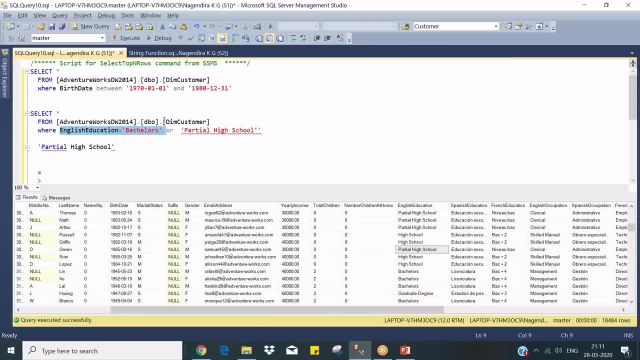 you are done with the single column and value. column and value. you are done with your one condition. then another condition: you need to specify the column name again. so english education equal to okay. so this will give me both. so if i run this one, it gives me five thousand. 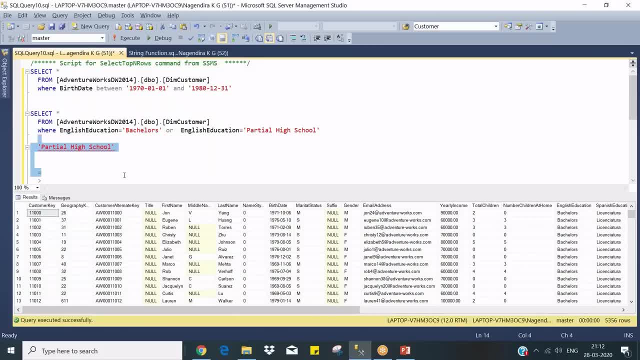 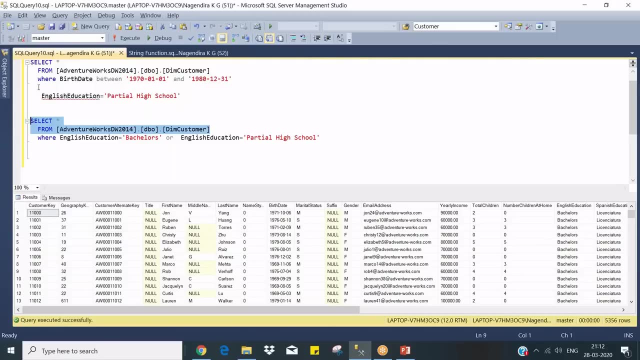 five three, five six. so let me put in another way. yeah, can we put both in a list rather than giving yeah, that is what i'm going to do next. so if you keep writing like this, i'm saying the count, i'm trying to take the count. 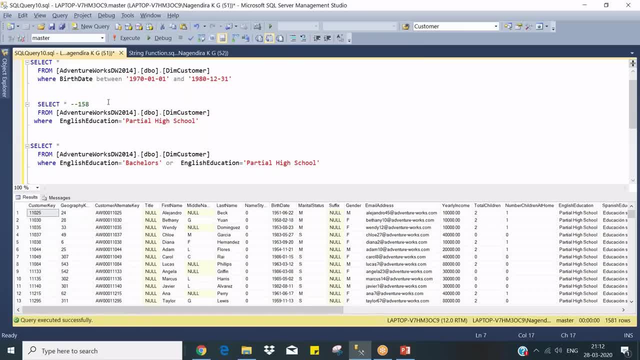 so that it it gives you the proper output: one eight one. five eight one. so this partial high school is one five eight one. you can see the record counts here: one five eight one. now i'm running only the bachelors. i'm not running the partial high school, so bachelors. 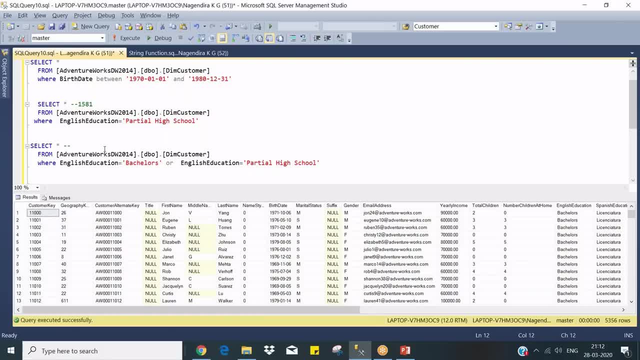 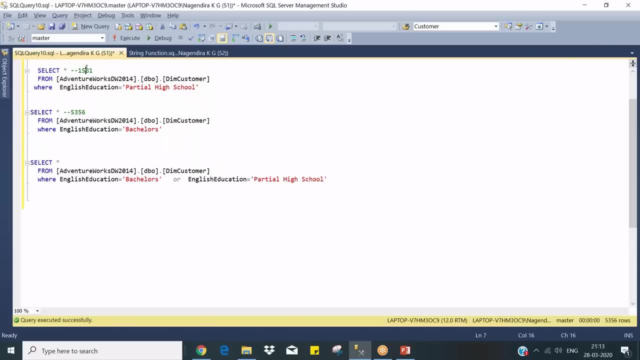 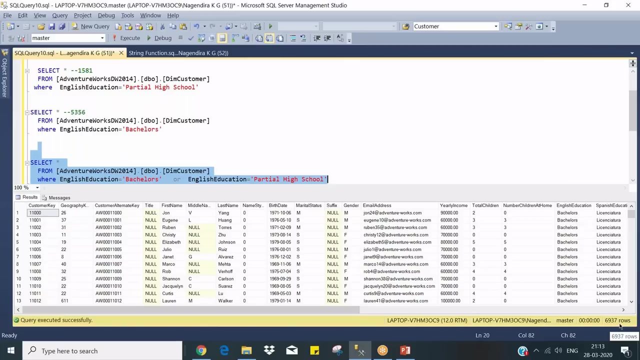 is five, three, five, six. five, three, five, six. okay, so let me copy this guy and put it here. so now i am putting both cases. so it is addition of these two: one, five, eight, one and five, three, five, six. if you put r, so it should return me something around six, nine, three, seven. so this is the correct results, okay. 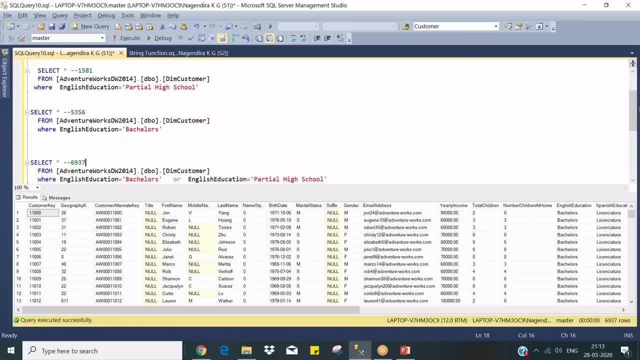 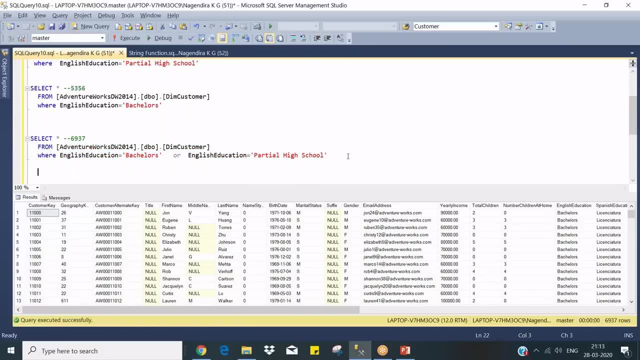 six, nine, three, seven. so we have different ways. that is varun highlighted. this is one way of writing. then what happens if my list keep on increasing? like i have a 10 members in that list, i need to put it in, filter it out. okay, so for that, instead of putting like this, i can put it here in: 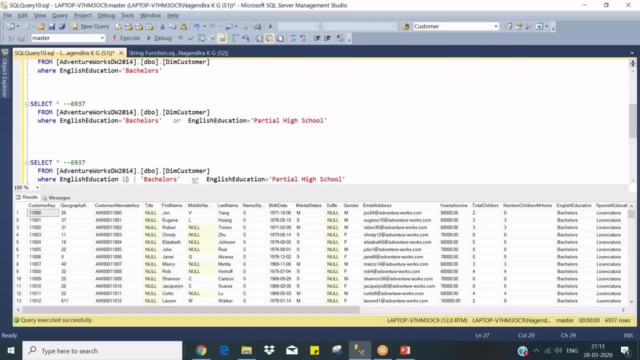 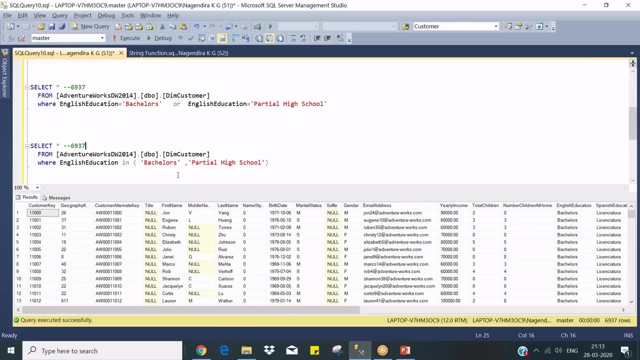 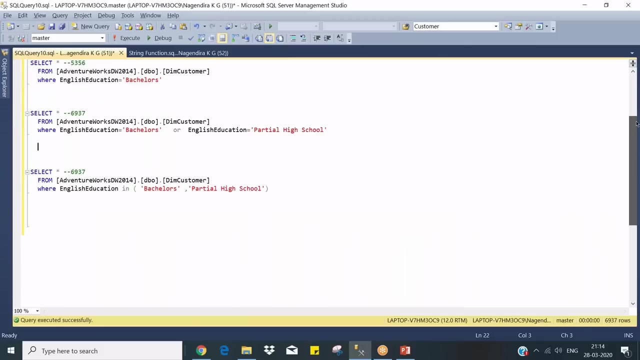 in condition. so the list here. it is not a list, so it is like in condition. you can put multiple values over here. it will return multiple values. so this query, this query will return same. so this has written six nine three, seven. you see here this one, also written six nine three, seven. six nine three, seven. so now to summarize: so we have a. 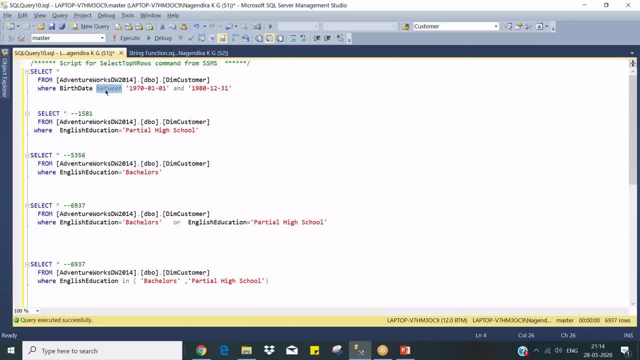 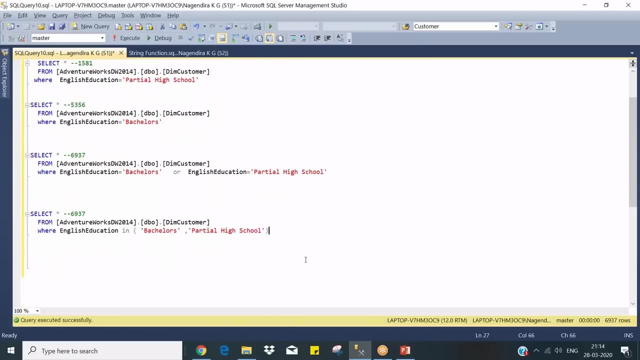 between operator to filter out using a range, and we have a between operator to filter out using a range and we have in condition to filter a list, list of values. okay, now, the same thing i can write in another format. uh, maybe in select statement. also, we can use in a sub query what i'm trying. 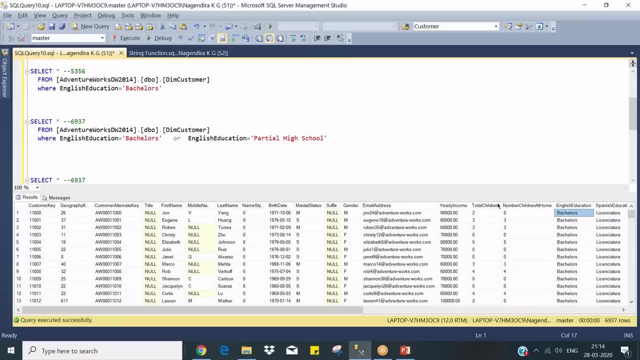 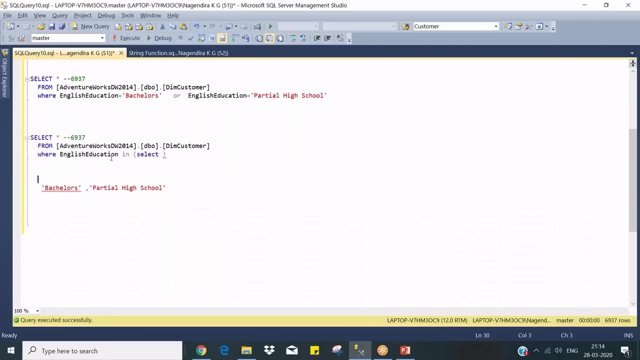 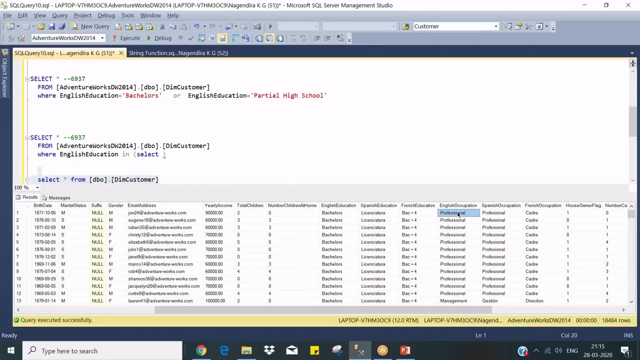 to say is: yeah, this, uh, assume you have a one query that returns these two distinct values you can have. you can have a select class inside this one also. that's what i'm saying. so for that, let me prepare that query first, so that it should be a class, that is at least a class type, and then i can use a class that is. 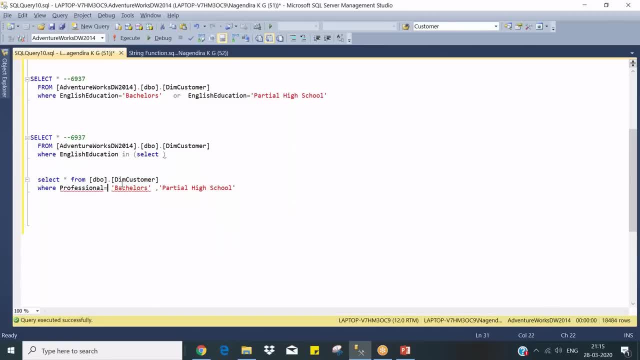 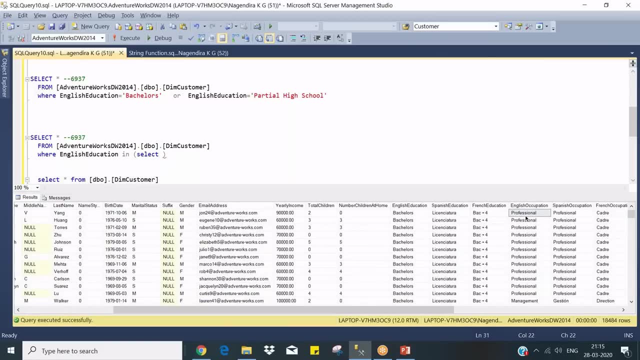 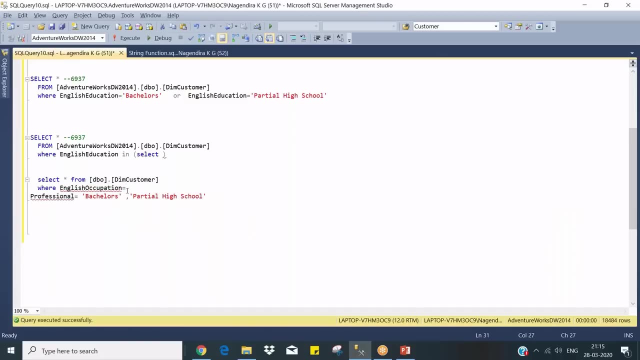 a class type. so i'm going to write a class type inside this and i'm going to put there a class type in this one. that is a class type and, based on this, i'm going to put it in framework. i don't want to put any class in it, so i'm going to put it in the same box. so i'm going to put there. 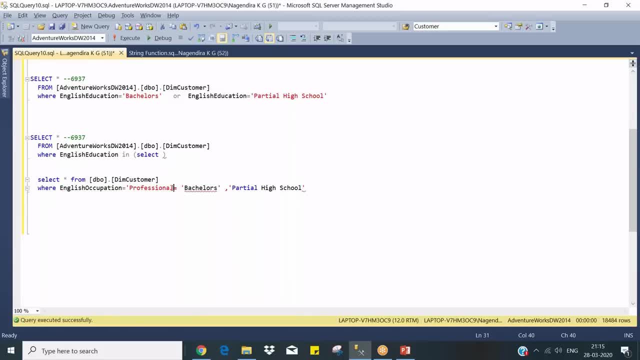 See, let us see what are the distinct values we are getting in English: education for the occupation equal to profession. So we get. so all the professionals have did all the five categories Okay, And even you can mention this one here. I'm just moving it forward so that, um, I mean to what's right. 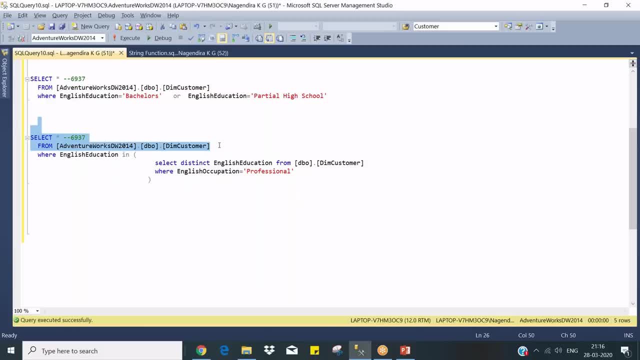 Okay, So see the query. So this will return my customers and it says like whoever did the English education and English education In this will this should return list of only those values in this education. I mean some values, or this should return only single column. 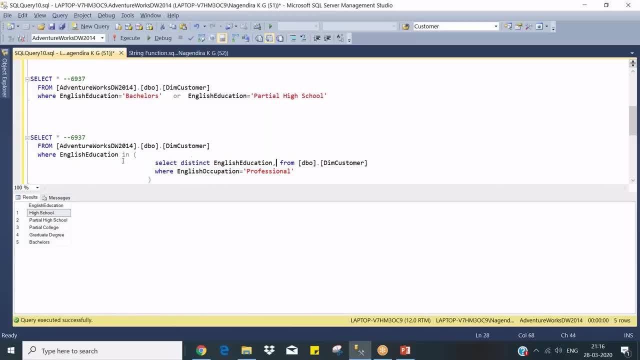 They should not return multiple columns. If I say like: uh, English occupation, that will throw me at: oh, this is nothing but your sub queries. Only one expression can be specified in the select list when the sub query is not introduced with exist. 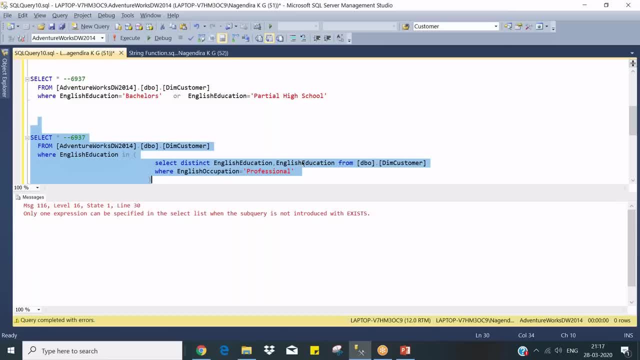 Forget about this. It says like only one column It is expecting. Okay, If you specify multiple columns, it will throw error. So basically, either you can specify it in a list of values or you can specify a query. Okay, That will return list of values so that it will automatically picks up. 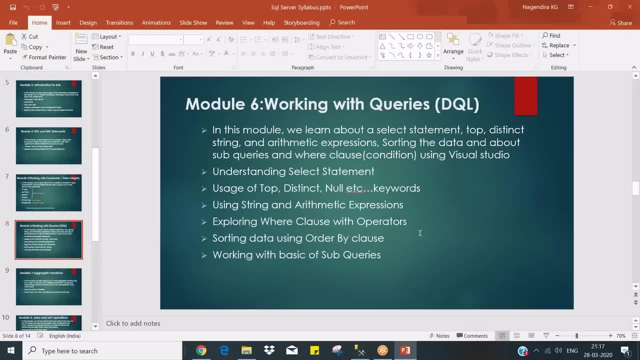 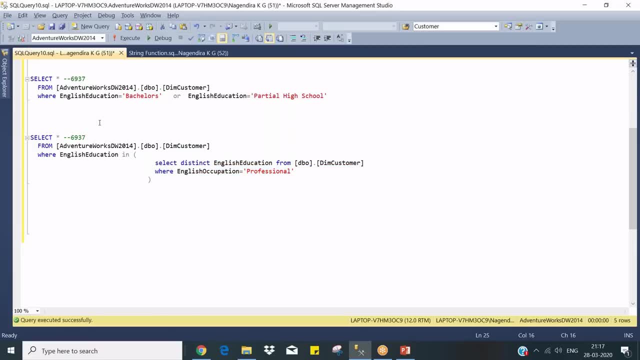 You got it. So that is what working with basic sub queries. It's as simple as that. You got it, guys, Okay, So I hope you are. you are in the room. I am your host, Rahil. Thank you very much. 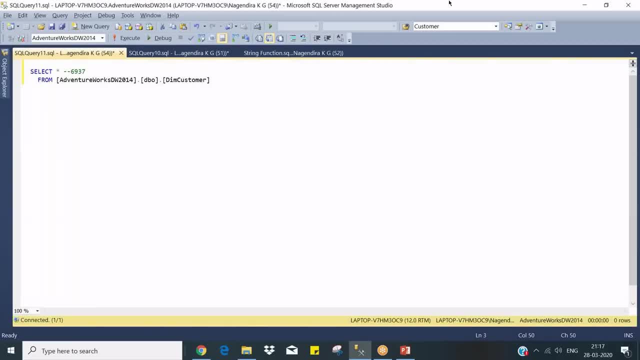 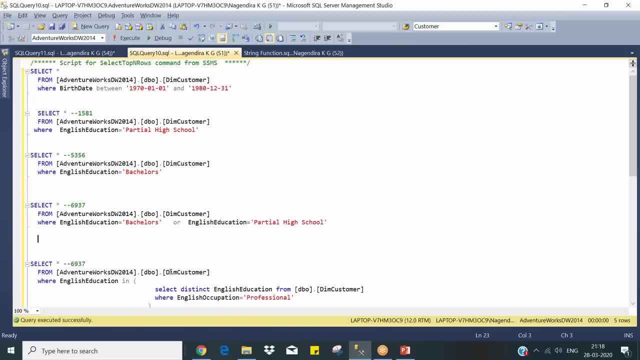 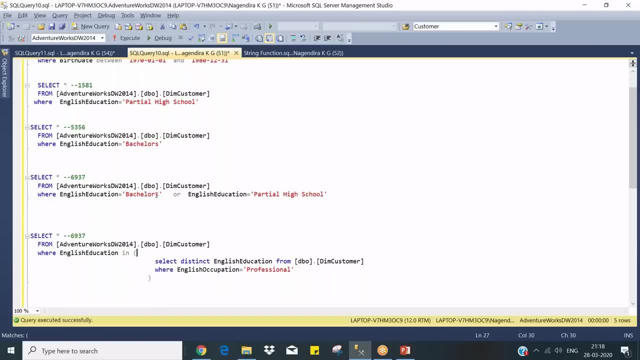 Bye, Bye, Bye, Bye in operator when to use so in operator to filter list of values. you see like you cannot have r condition here, so you might have thought like: instead of r, i used in condition, so in condition is used, so this and this will return same. if you have a single values that you, whatever values you. 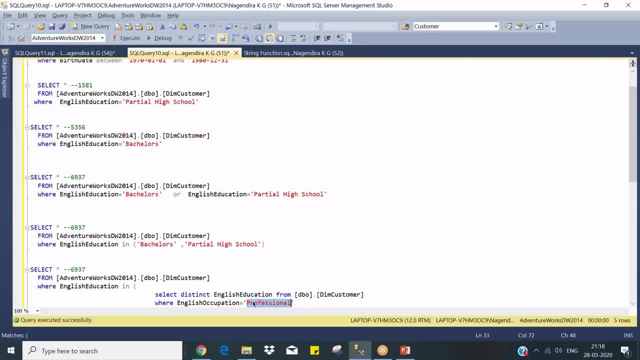 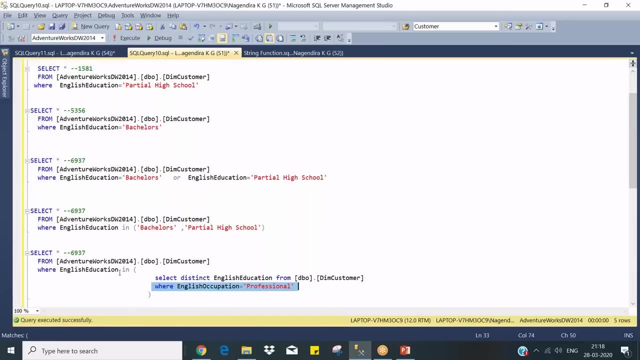 know you can put it like this, but in this you don't know what are the list of values. it is going to return english education, but this value, whatever it is going to return, it depends upon the another subquery, this query result based on the filters. so in that case it will be very useful. 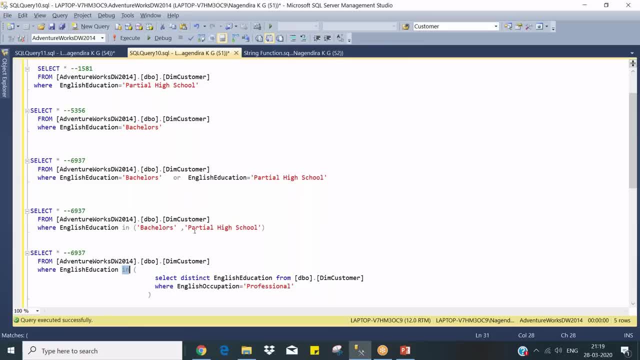 so you cannot compare these two, so when to use? so if you don't know the prediction of output, then you go for this statement in statement. if you know the exact values, you can keep adding the r and whatever the values you have. so it's the way you have to query. 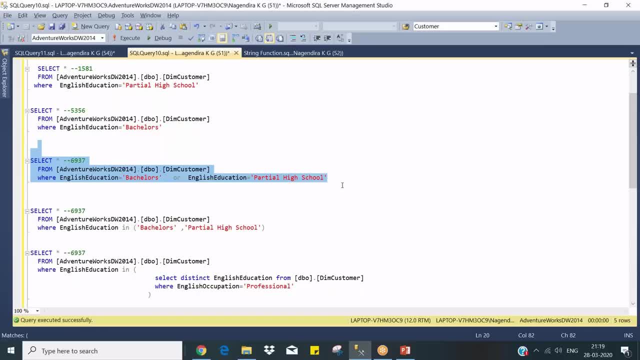 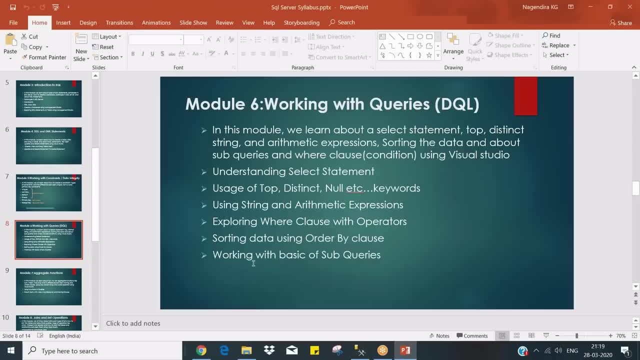 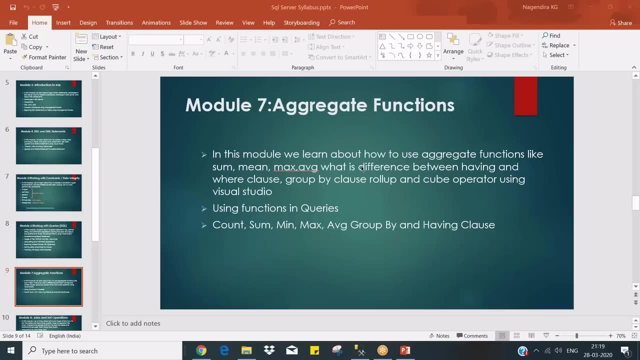 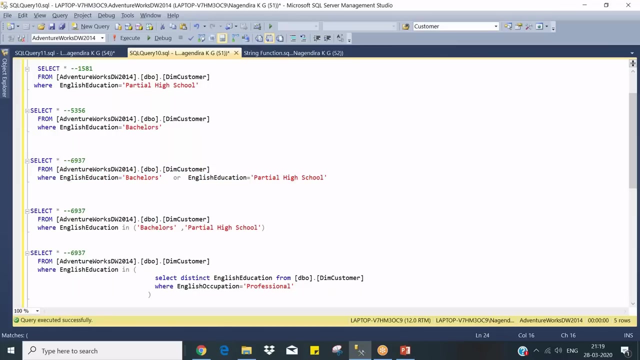 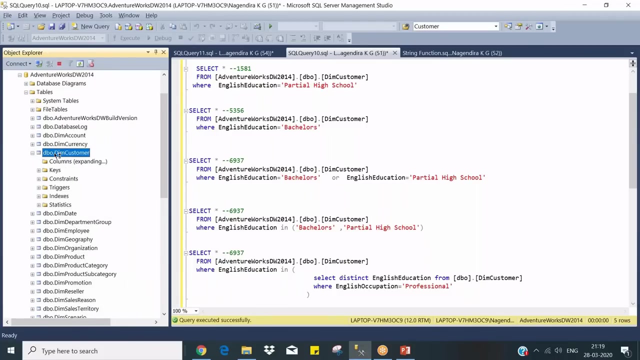 you need to know when to use this such a queries. okay, so with this note, uh, we stop operators. let's move on to our next topic: aggregation functions. okay, so, any idea, guys, when, when we use this aggregation functions? any idea, no, so, uh, let me ask this question. so how many of you used pivot tables in excel? pivot table. 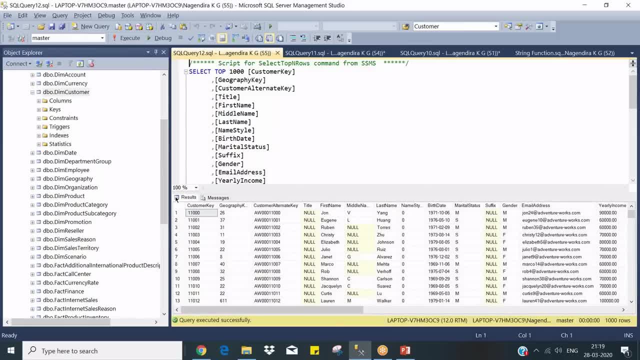 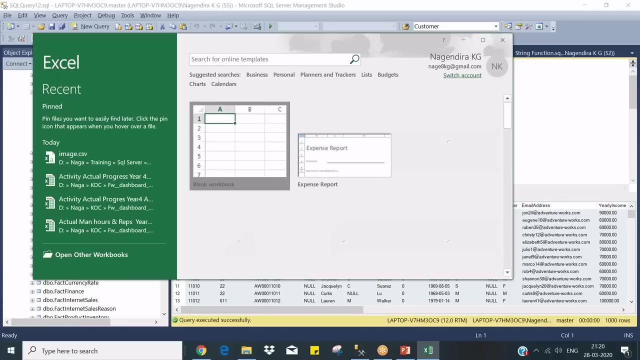 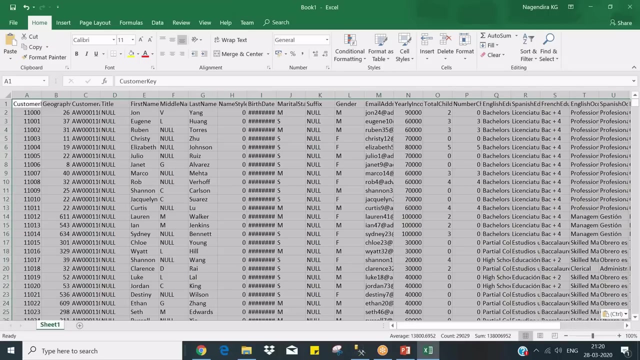 any idea? no idea, hello. so what is it's used for? we can sort out the data according, right. it's like it's a number of data we can like. we can have the whatever we need in the pivot table. it's like, uh, okay, getting the whatever data we need in short form. not such in the short form. 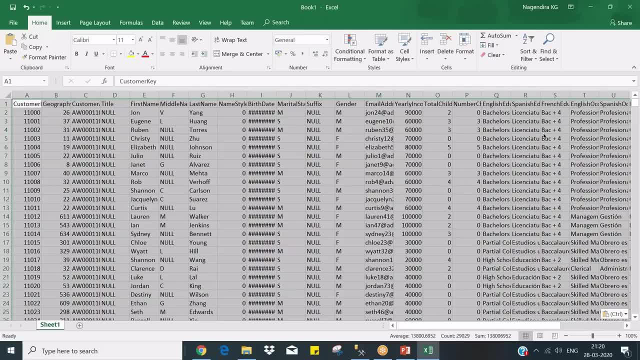 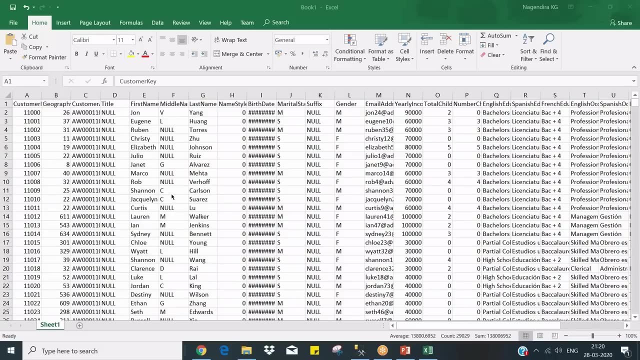 see are. you guys know about pivot table but you are not coming. actual point. the thing is: let me explain to you guys. so forget about those things. thanks for your answers, and so i copied the customer data once again here. i'm going to do a pivot now. 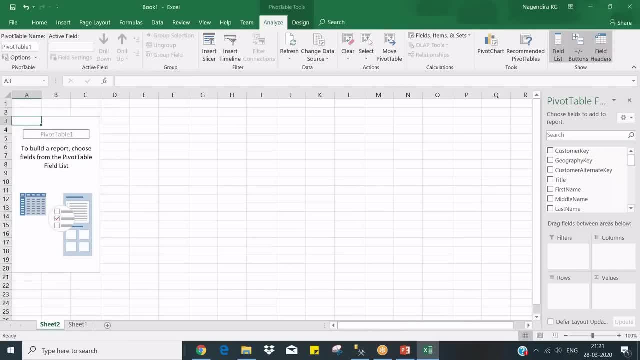 the idea behind the pivot table is like: you want to see the data in aggregated manner. see, as a company executive, our managers. they want to see the data at the higher level. say, for example, you are running some supermarket, so at the end of the day, each day, you want to see the total sales and you are having different shops. 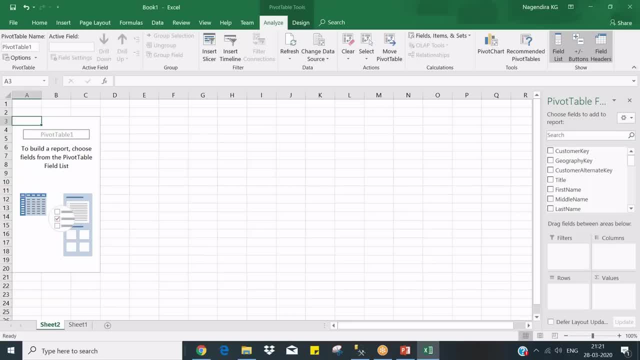 say, for example, three shops, so you need to know how. what is the sales of these three shops all together in a single day? so aggregate level, you know, no need to see in detail each time. okay, at the given shot in a single day you want to say: what is my total sales, correct? so these are nothing but your aggregates. 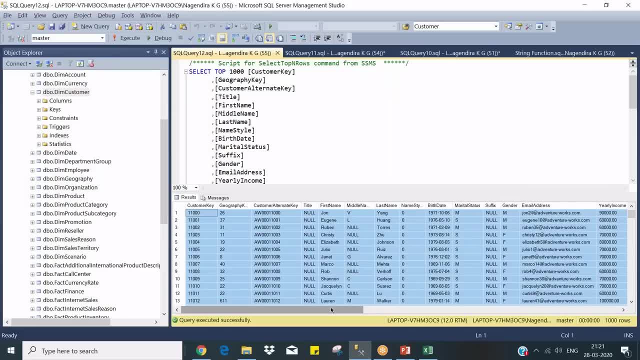 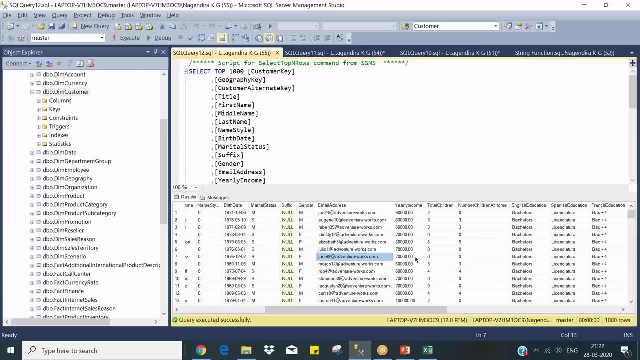 total sum, so nothing. but if you see here as you, this is your customer data, I want to see what is the salary, total income, okay, total early income of all the back-end customers, okay. so I want to see what is my total income and this is an. 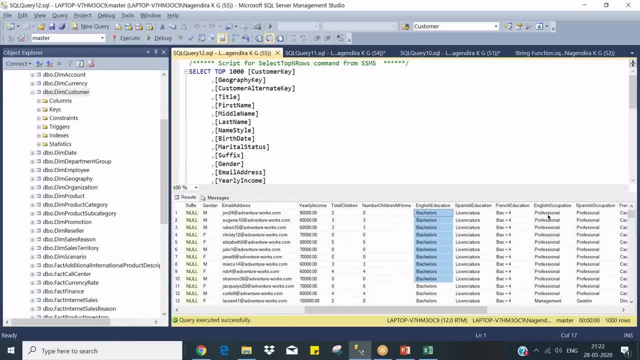 I want to see what is the total income of the professionals in my customers, or management students in my customers. total income, okay. so are how much they are spending how. what is the salary? okay, I assume these are some kind of employees instead of customer. you forget about the customer perspective. we'll stick to this salary perspective. this is the. 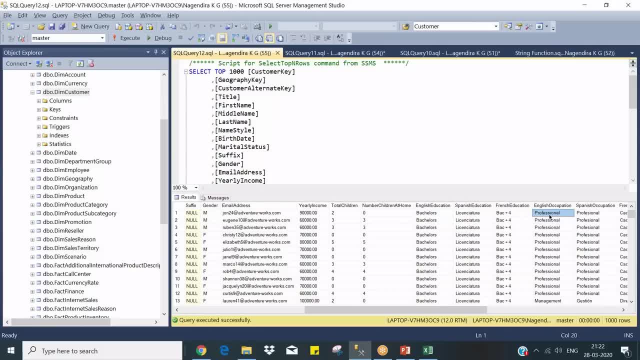 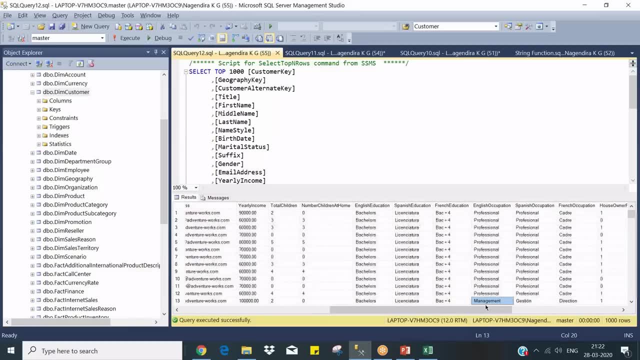 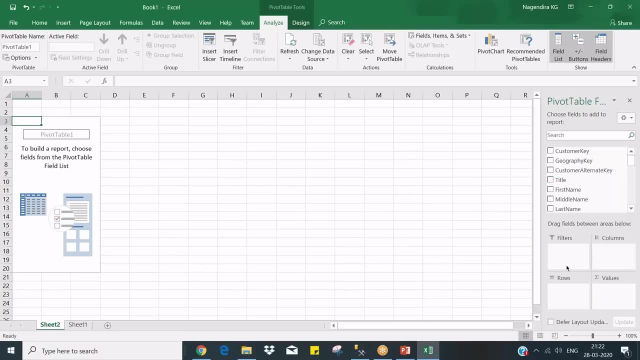 employee information. so employees role is profession and he did. he's a management profession and he did some cater or education like that. okay, now I want to analyze how much I am spending for a profession, something like that- so I have a base data here. let me search for a. 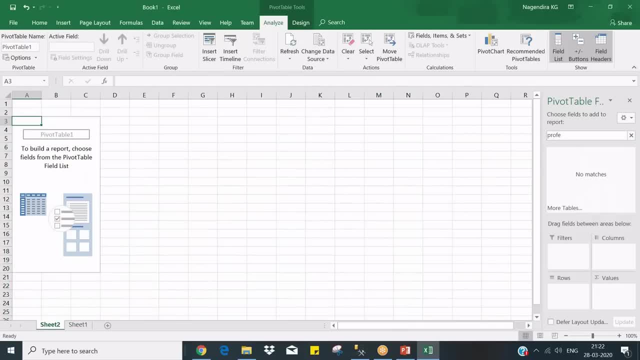 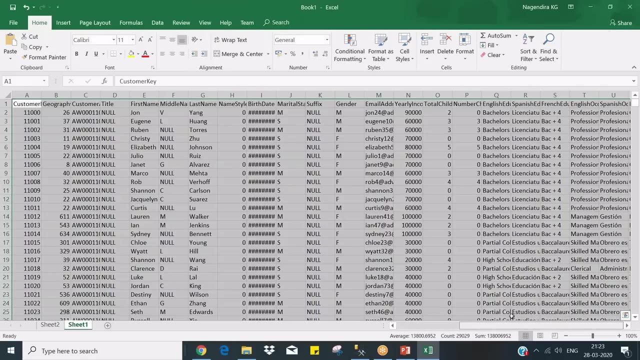 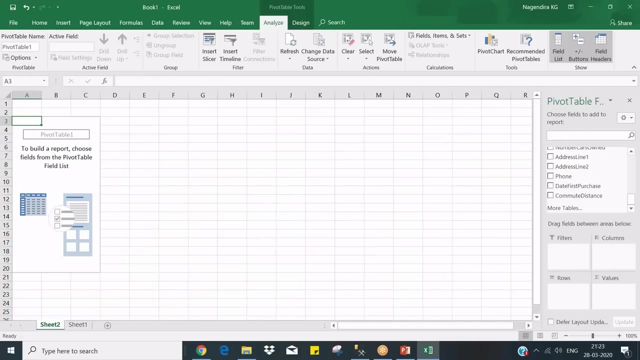 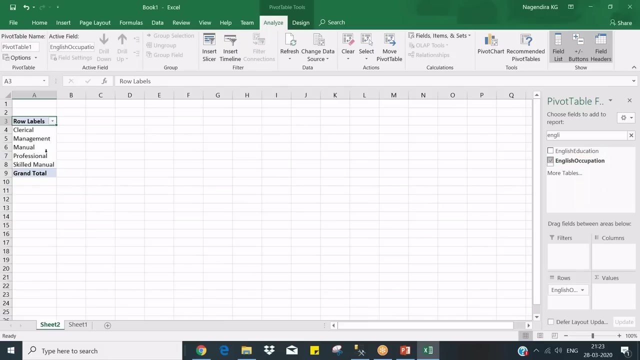 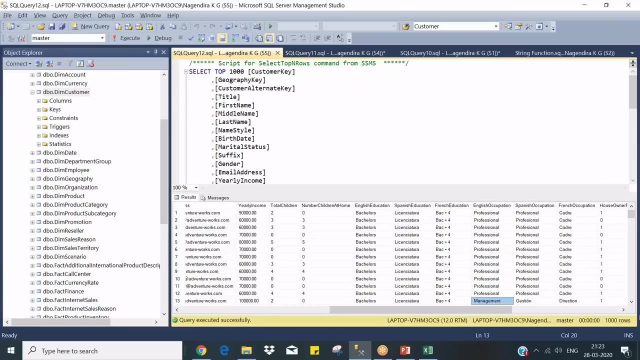 profession one. it starts with English occupation. okay, see when I put it, it's not sorting actually. okay, someone said it's a sorting, it's not actually, it's like grouping. so what are the distinct values it have against which? what you want to see? I want to see the salary. what is the? 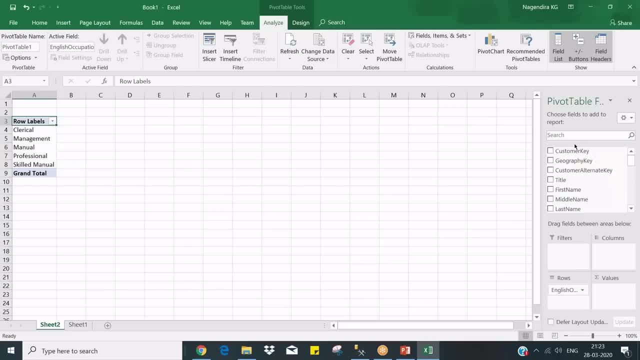 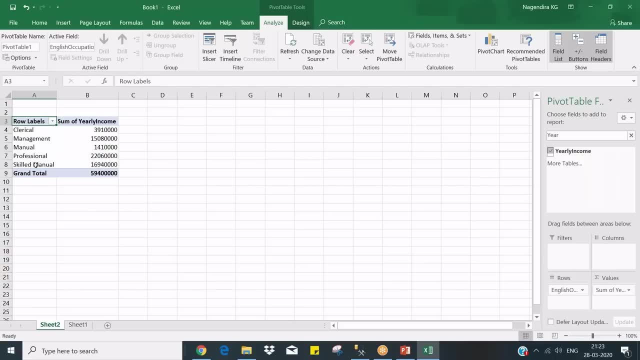 salary column, here yearly income. so if you see here total yearly income I'm spending for an employee, for who is a profession, this is my total yearly income. skilled manual: this is my total income. I mean total. I'm paying for the skilled manuals and whoever is in management for them. I'm paying this. 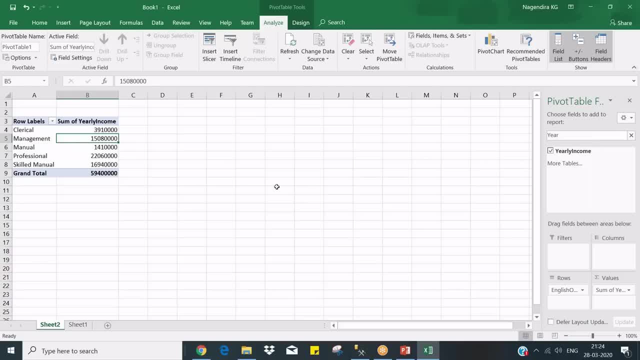 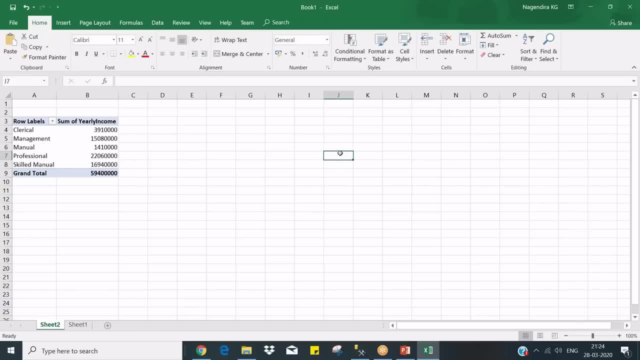 much. this is the yearly income of it. so you are aggregating the data. assume you have four employees. someone is getting twenty thousand, thirty thousand, fifty thousand. you add twenty thirty fifty and another guy twenty. so two twenties, thirty fifty, with which will be like 110, okay, twenty thousand. 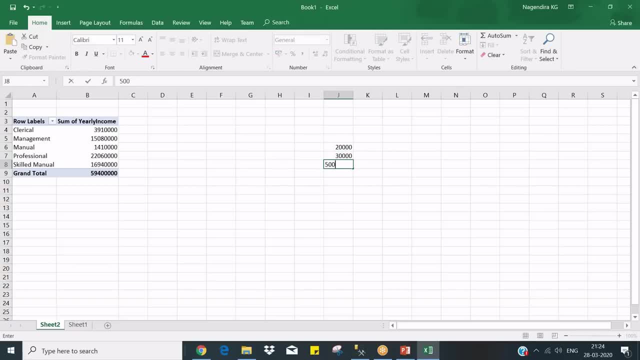 thirty thousand and you are paying forty thousand, fifty thousand, twenty thousand. so these are your three employees. so what is your total employee expense? it's like one lakh, one like ten thousand. so if you see here, one like twenty thousand. so my calculation is so poor. so one like twenty thousand I am spending for my employee salary now, as you. 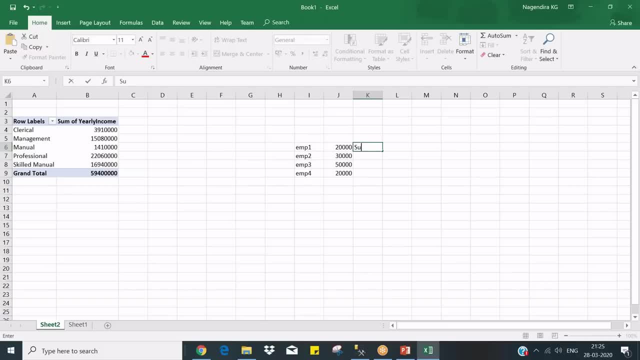 guys. two guys are your supervisor. okay, these two guys as supervisors and these two waves are cash here as you make that, okay. so if I want to see how much I'm spending, for I cash here, I will sum these two. if I want to spend how I mean, I want to analyze these two, which is fifty, so it's like: 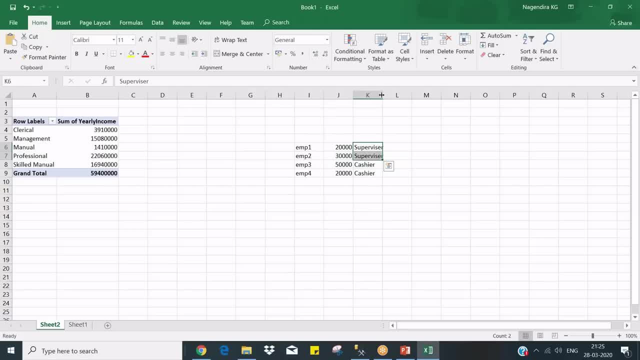 grouping of certain values, certain columns, and how can it split if it's a team, ick opens here we pour a bucket, so easily I can вид suited to twenty five, so it's like grouping of certain values, so columns and two in it, so there's two. 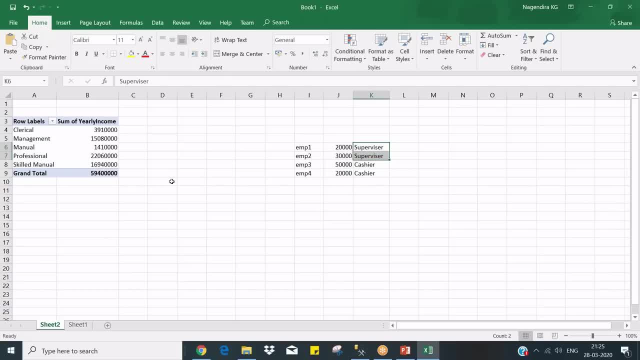 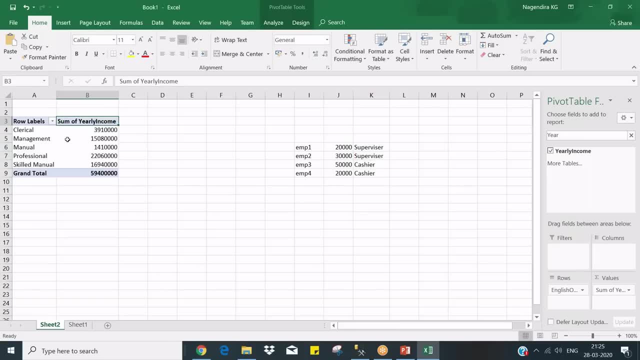 and you want to see the summarized results of it. This is what your pivot table does. This is the main purpose of your pivot table, So what operation it does here some instead of that, I can go and do the other. aggregation value: See summarize value field. 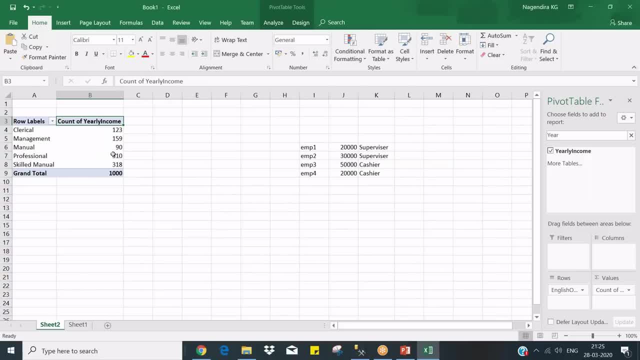 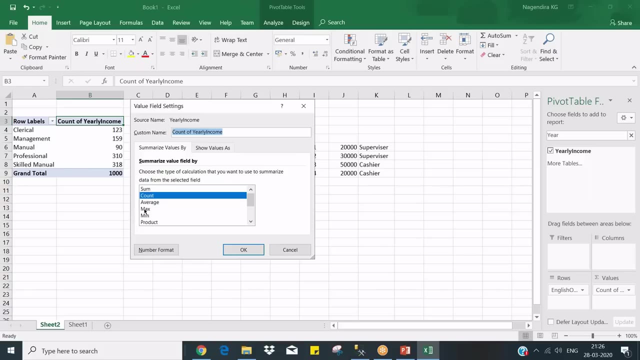 I can go and check how many persons count. if I put count, It will give me the count of employees. in clerical. There are 123 employees in management, 159 employees in manual, 90. So it just says aggregate values And I want whoever is getting maximum salary. 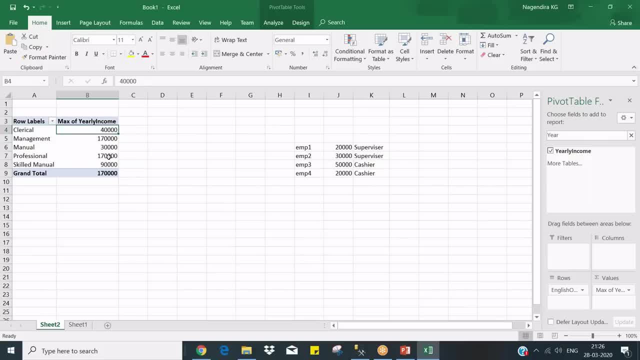 In clerical I'm getting. I mean, someone is getting 40,000.. He is the maximum. let us go and check how this is correct or not. Okay, let's do some research. I mean not a research, Just filter it out. 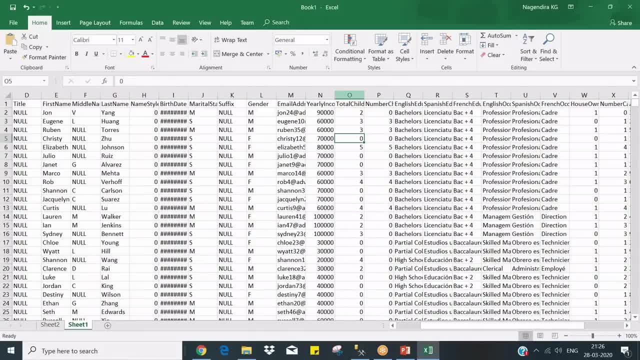 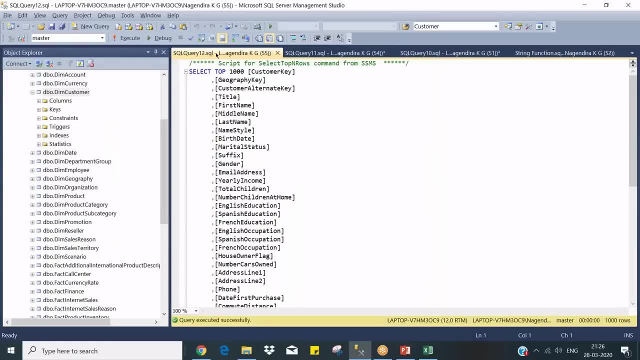 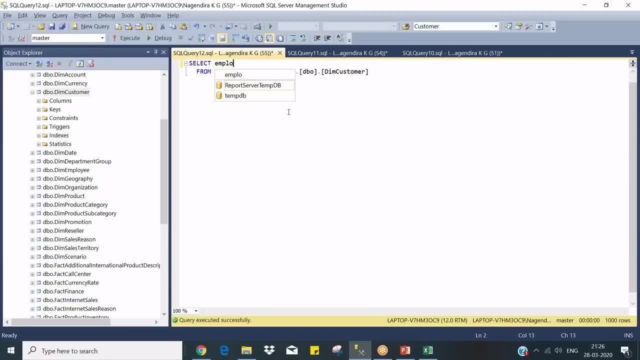 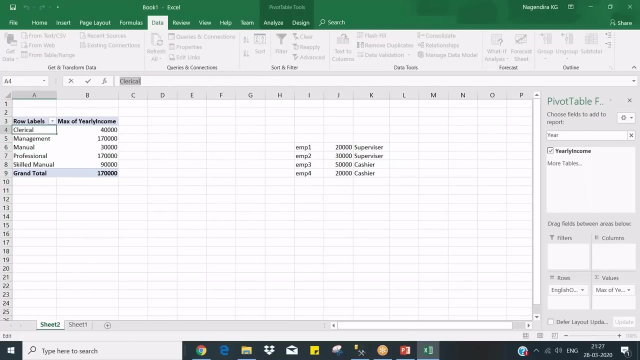 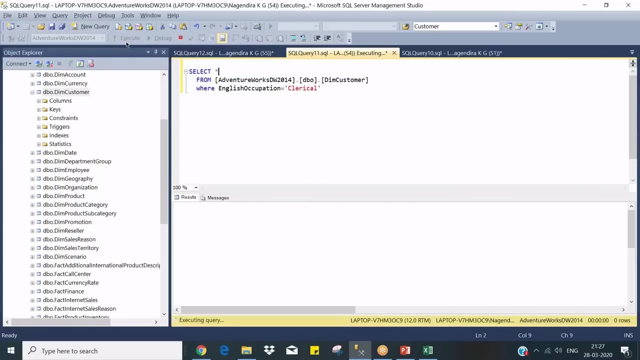 So I will go here. Okay, let's filter. Okay, I will go and query it. Employee. Hey, come on. What is the column name In English? occupation, English occupation. English occupation equal to clerical. Okay, I'll just. 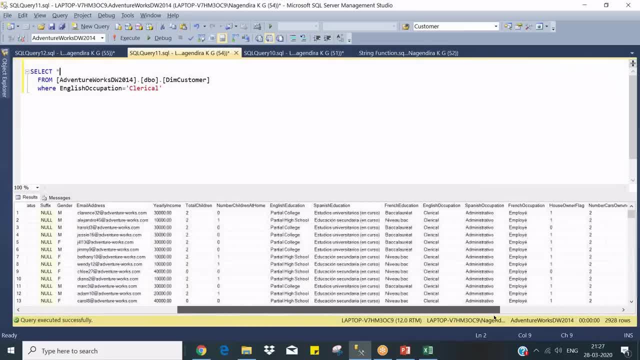 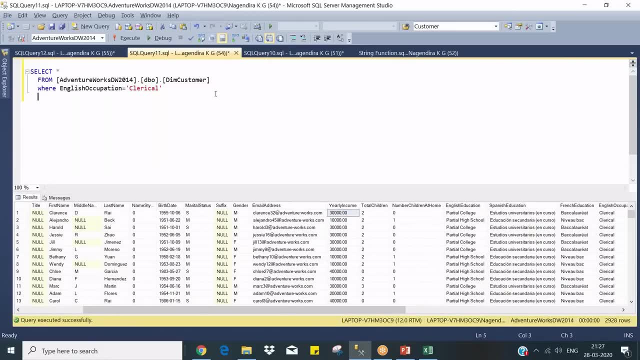 I filtered the data clerical and I will try to. I'm saying the maximum Salary in clerical is 40,000, whether it's true or not. How can I find I can put like this order by Yearly income: descending: ascending, descending. 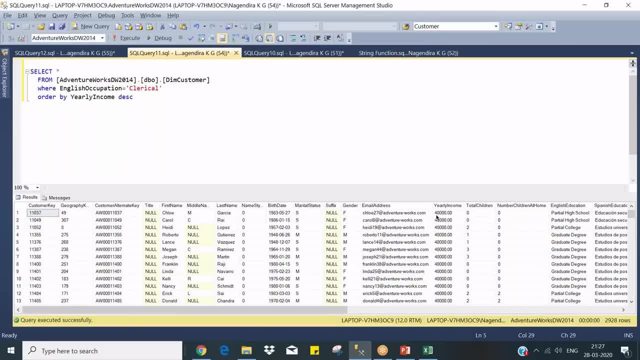 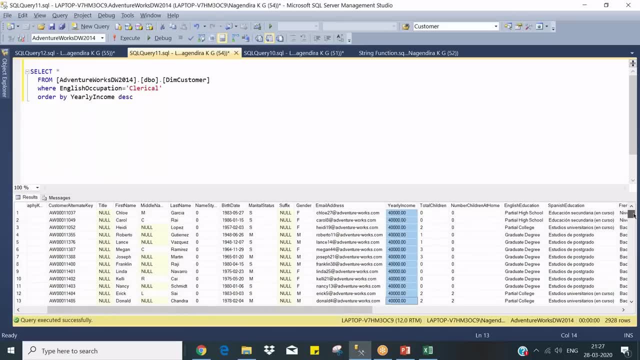 There you go, So 40.. So there are a lot of people who get 40.. So it doesn't give me a ranking basis, which is whichever is maximum in that column. Now for clerical, it will give me 40.. 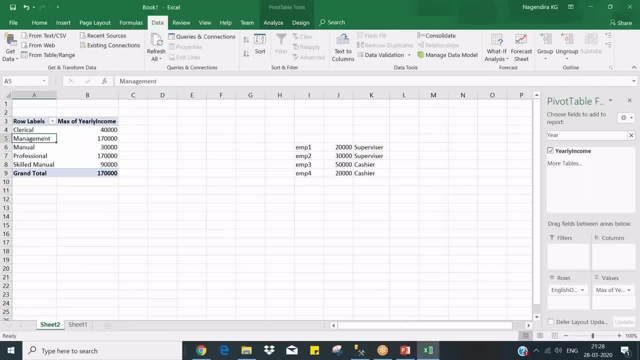 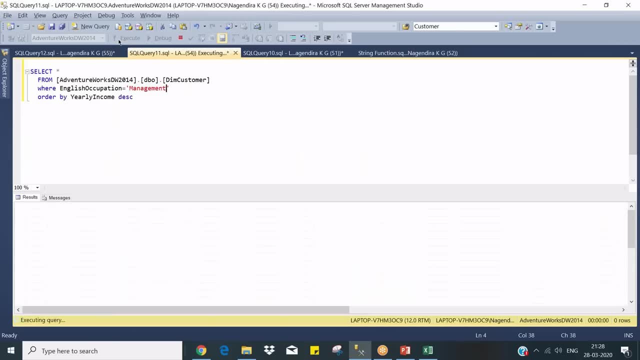 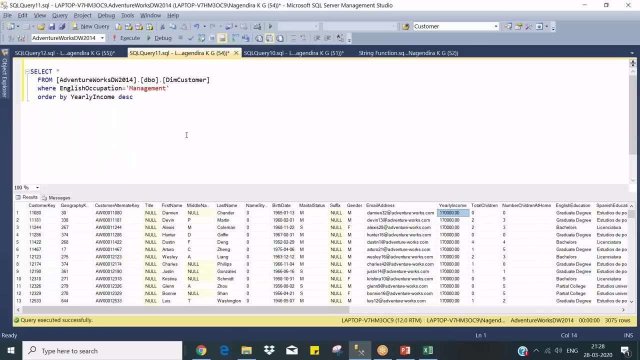 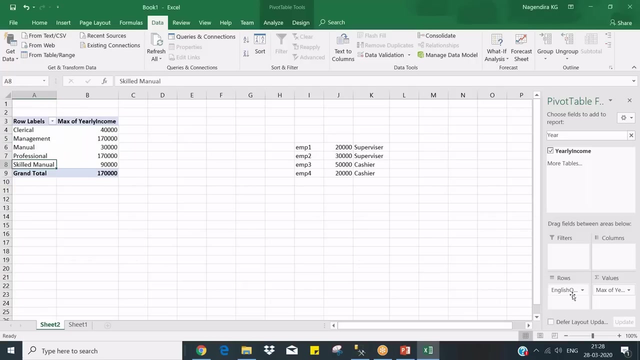 That is what you got- 40 here. So let me change it to management 177. that is what you are getting here. Okay, and now I will slightly change the query, like I will remove this guy. See now what happens. I put Max and remove this guy. 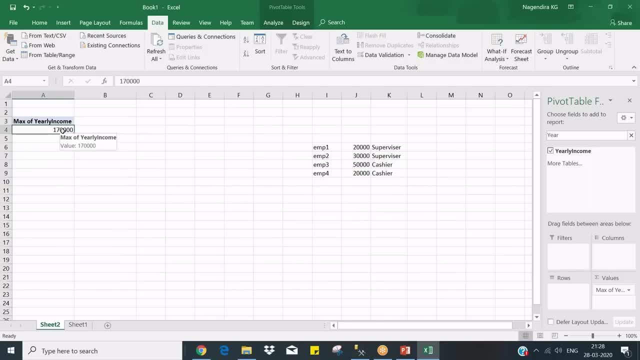 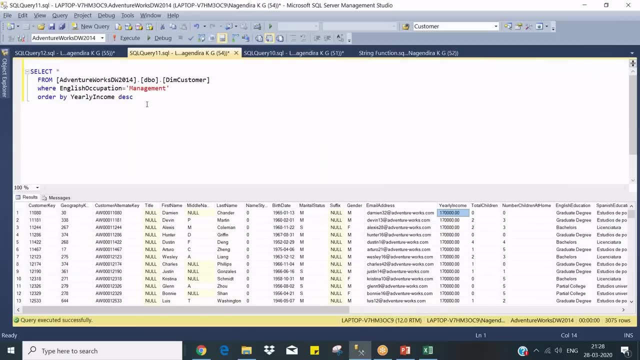 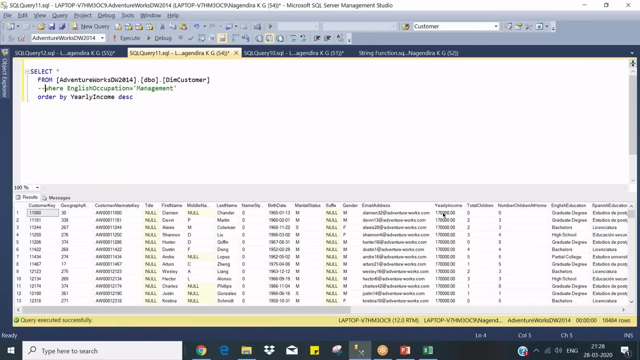 So what happens? it will pick me who. this is the guy who is getting the maximum salary across entire department, irrespective of the department. So let us see, without this, where condition this is what it's happening. So this is the maximum salary. You got it, guys. 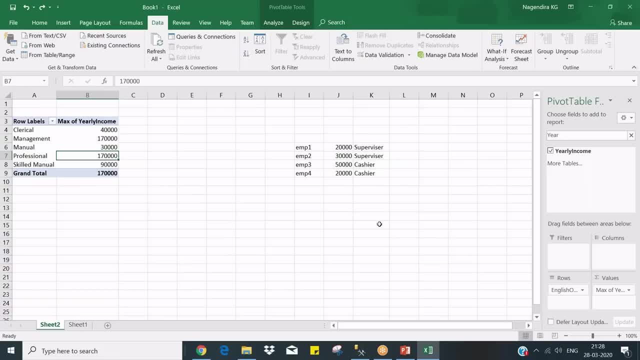 So these two guys are getting maximum salary. So basically, a pivot table will give you the aggregated results, The high-level information to group based on particular column, and you need to do what aggregations you want to perform. So, basic level of aggregation: some average minimum, maximum count. 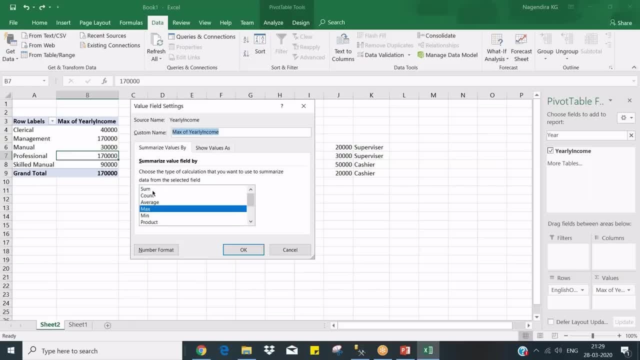 These are the five aggregation functions. You can perform some count, average, minimum acts. Okay, These and all belong to Excel. So in a, In a scale, we will perform these three. So all these things are conventional one. Whatever you see in Excel, that will be applicable layer. 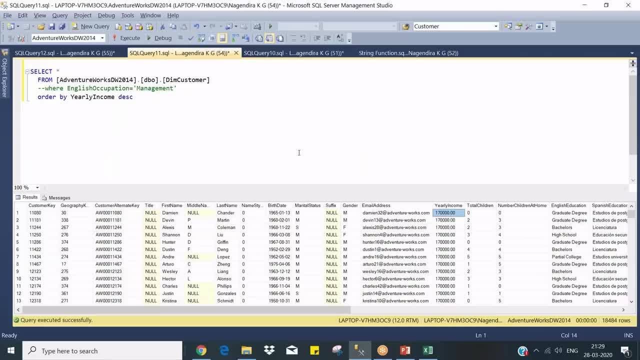 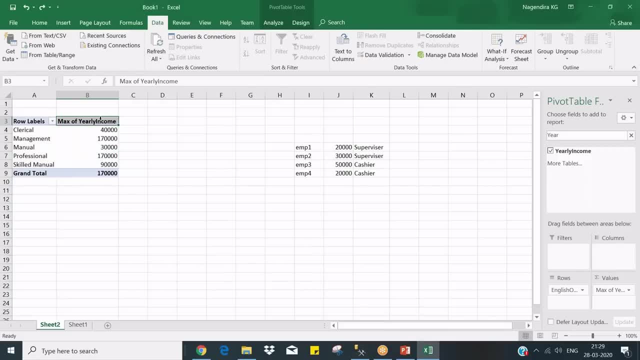 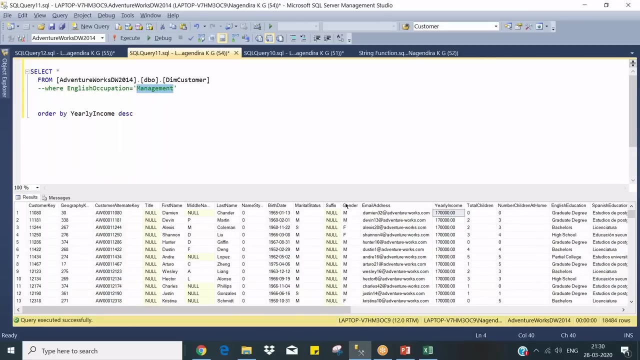 How you work in SQL. that's, we are going to see So same results. I want to get it now here, What I'm seeing here. So just choose value field, some becomes same results. I'm going to get it now. So now, instead of filtering to management, all those things. 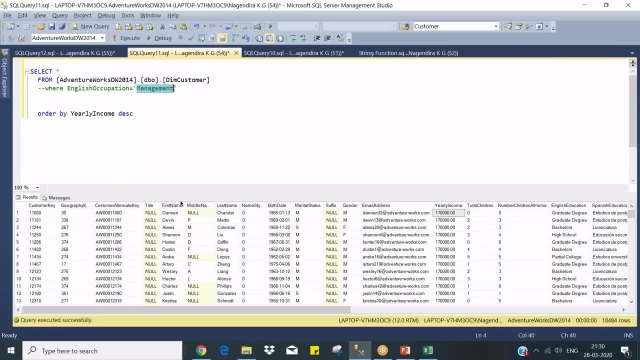 So if I filter through one particular category it will give me all the results. I cannot analyze using the 5000 records or 6000 records. Just I want to use group by group by what column? English occupation, that you need to specify the column name. 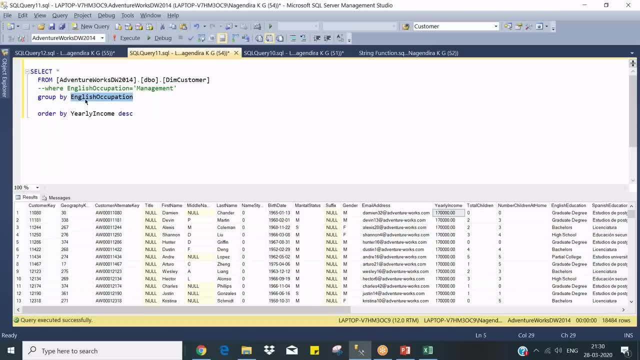 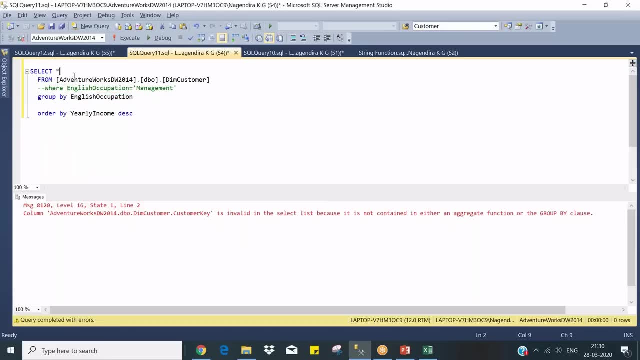 Okay, and whatever column name you are specifying here in the group by, you need to put it in the select statement. Okay, If the star won't work out, if you see I can put it like this will throw me error. if I put like this, then fine, then okay. now this is incomplete. what aggregation I want to perform? 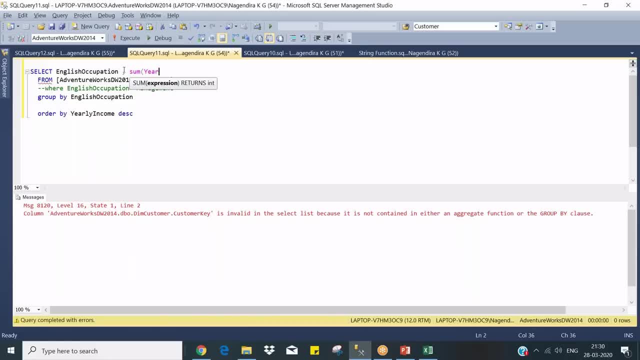 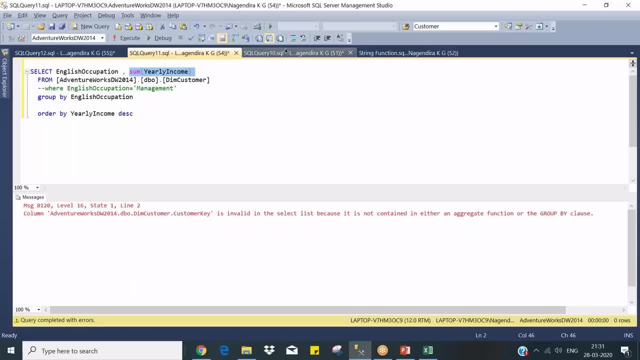 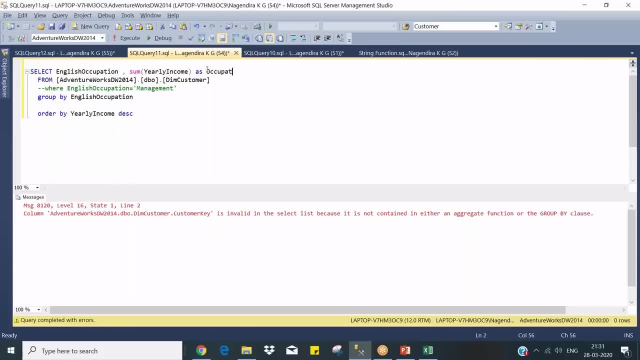 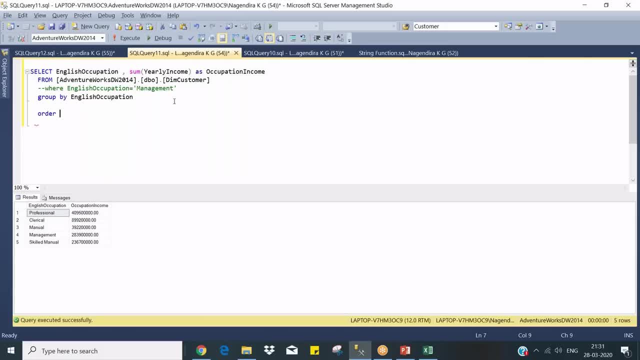 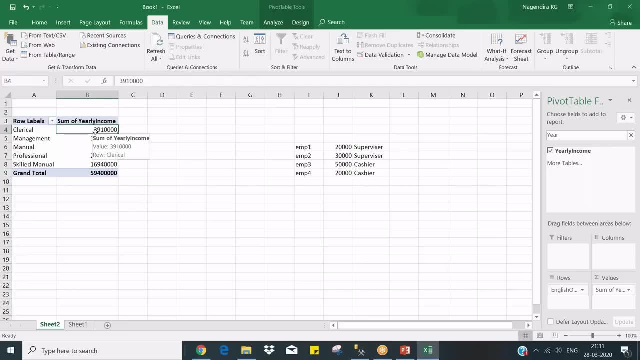 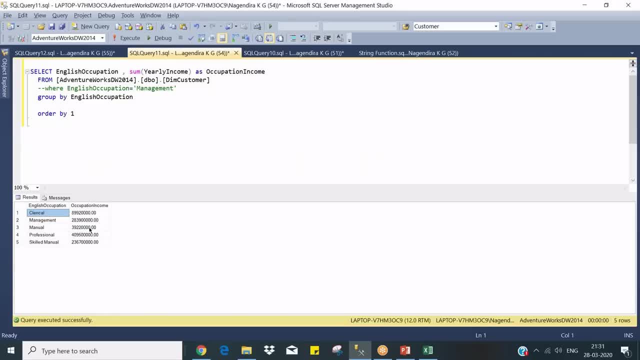 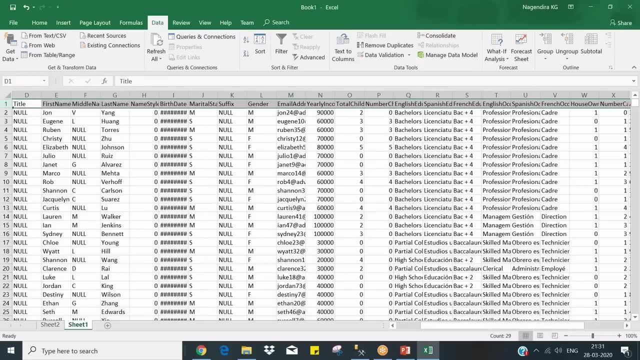 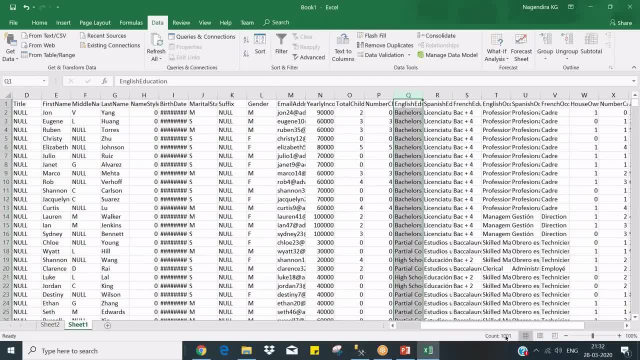 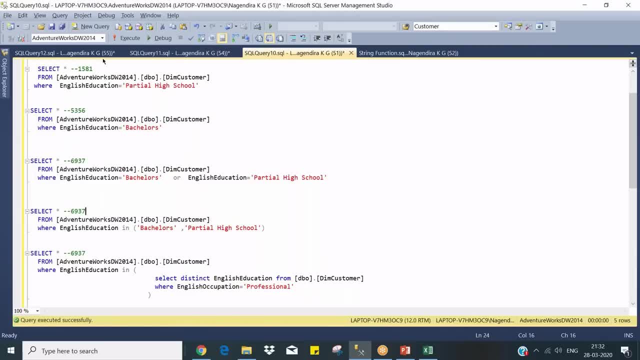 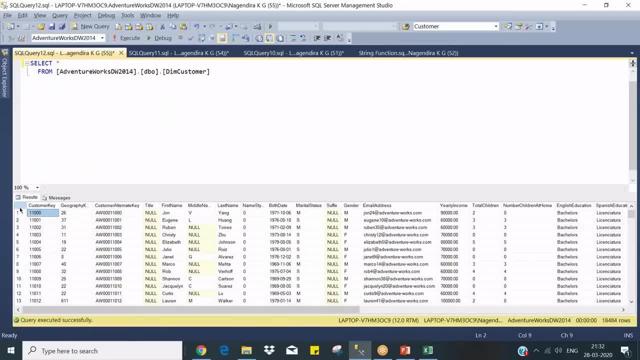 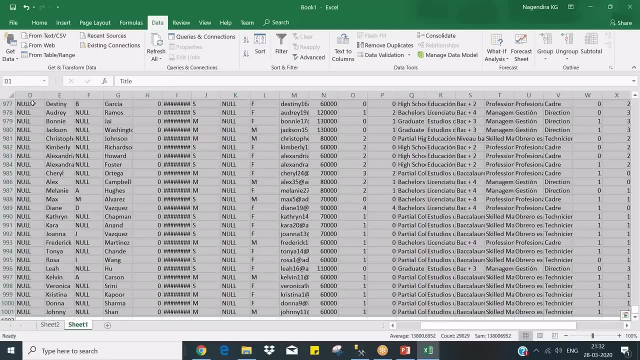 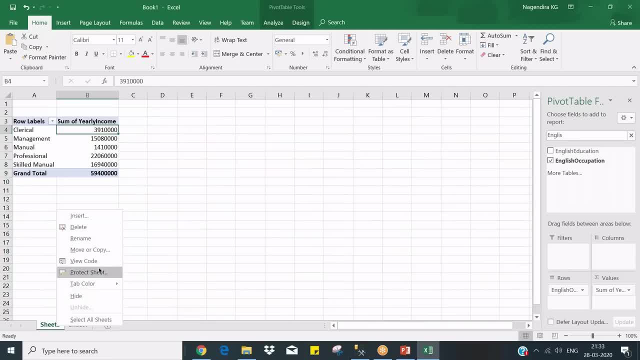 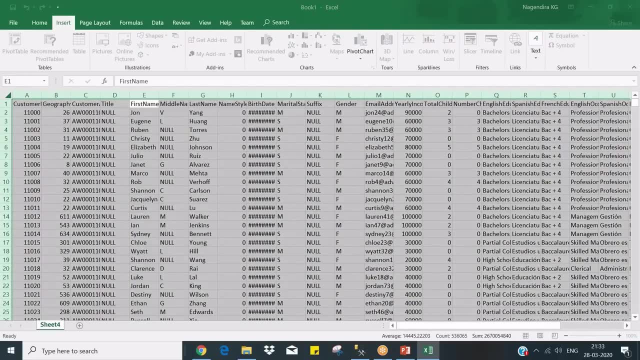 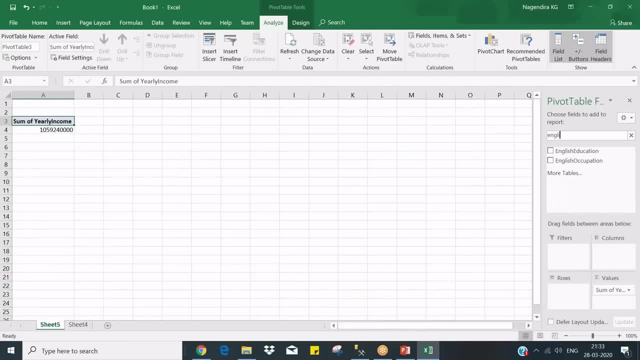 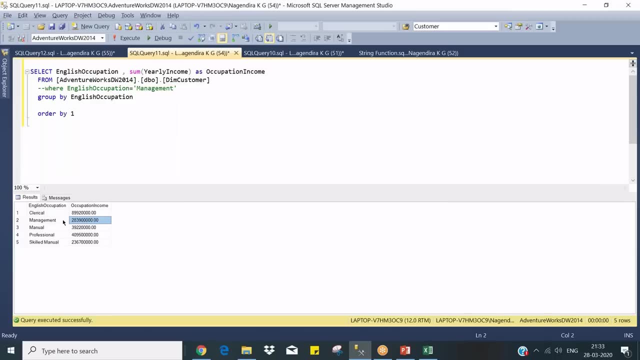 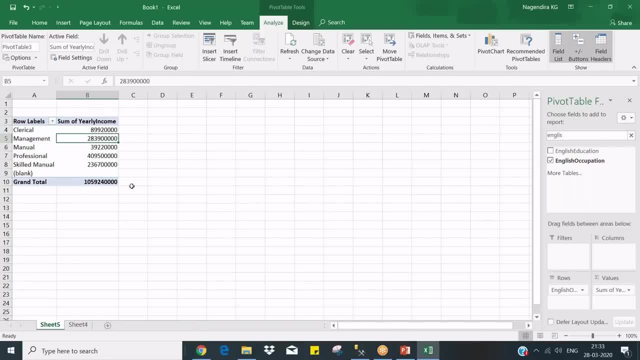 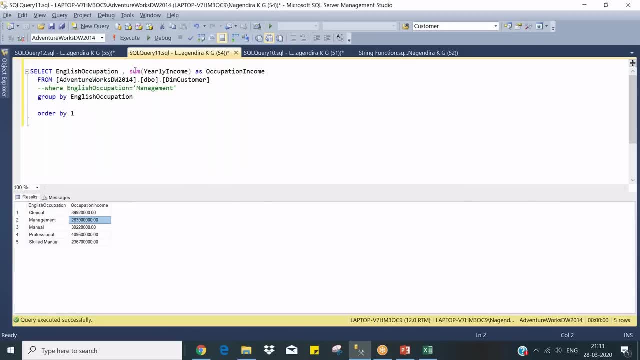 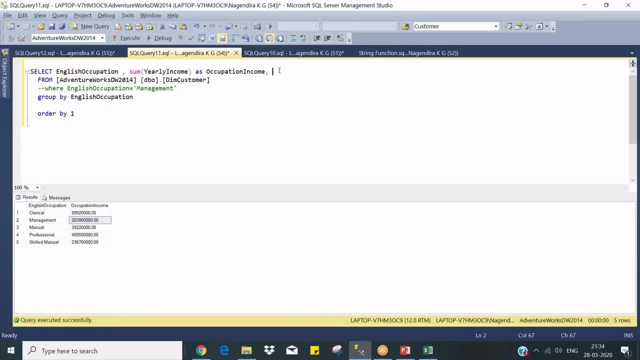 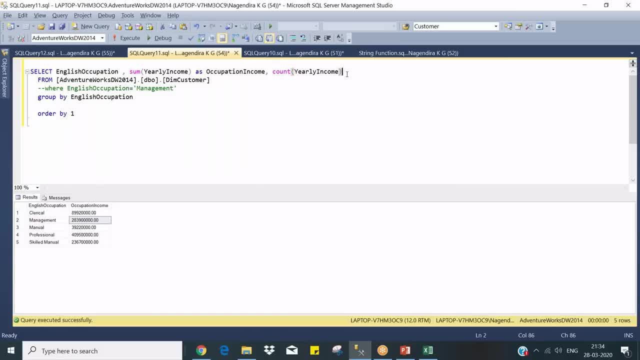 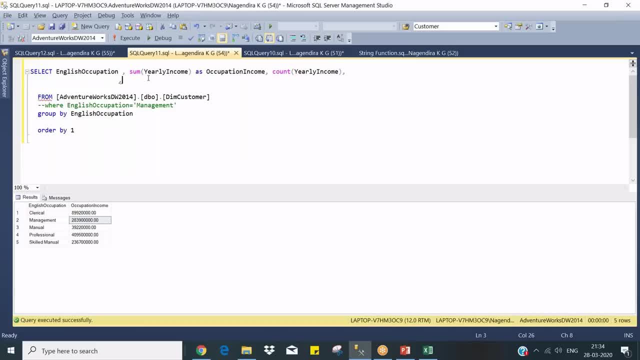 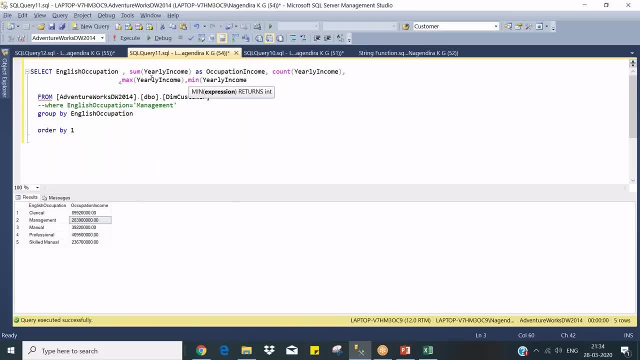 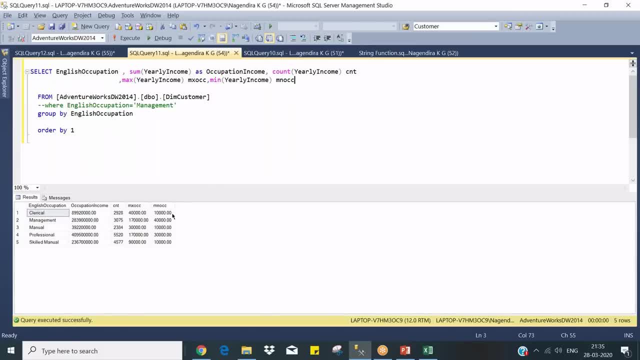 And in clerical someone is getting 40,000. Someone is getting 10,000.. So as an aggregated level I can see in a single report as summarized report here. Okay, So basically this group is very essential part when you take reports. 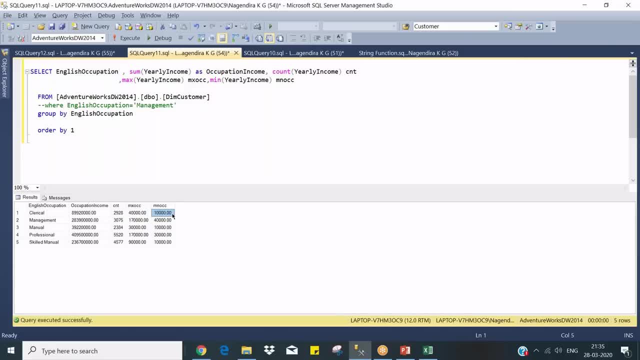 Now, This is fine. So what about, like now, based on the computer results from this, I want to filter certain things, like whoever is getting maximum salary In any of this group. the salary greater than 30,000, okay, or 50,000, say, for example, 50,000,. some scenarios will come. 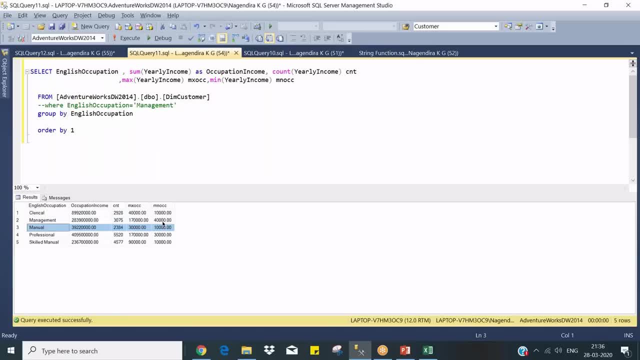 You just choose The maximum salary And from that whoever is getting the 50,000, filter those groups alone. okay, like that scenario will come. So here you can't use the VAR condition over here where salary maximum said they're asking only the maximum salary is greater than 50,000.. 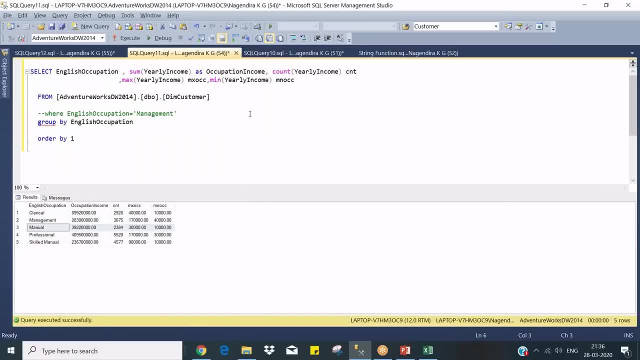 Okay, So after computation you want to filter means you need to have having. If you're just trying to figure out, like, what's the minimum salary of that person, Okay, So the minimum salary is that of 180,000, okay. 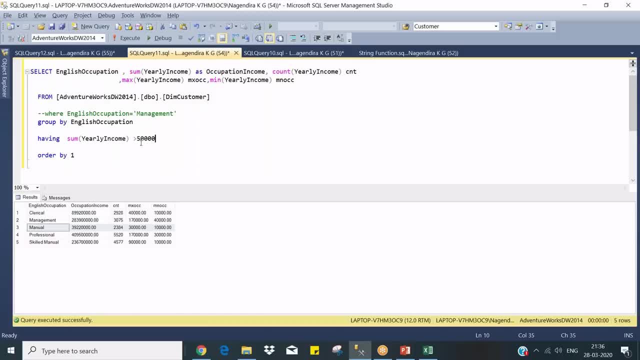 So the minimum salary for the person is 100,000.. And the minimum salary for the person is nine, So you're actually getting a minimum wage of 8,000.. Okay, So the minimum salary is almost the same. Now the minimum salary is $1,000. 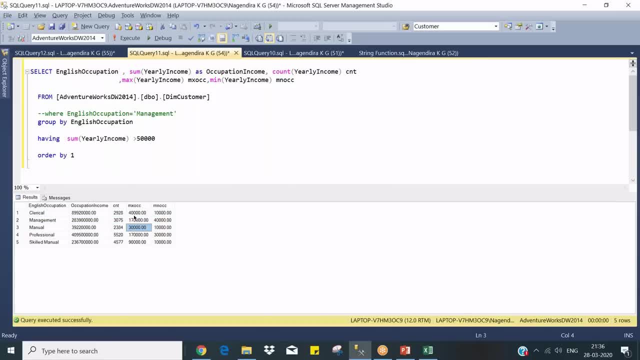 How much is that? That's a net minimum salary. So That's more than that. That's more than that. Yeah, this condition: failure. because of this rule, the salary, or the maximum salary, should be greater than fifty thousand, so these two will be neglected. 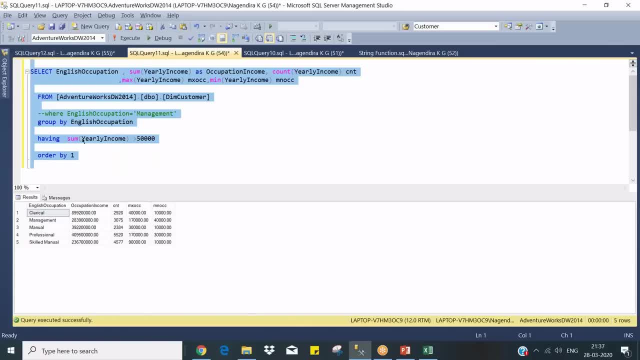 oh, am i wrong? okay, sorry, this is not a yearly, see yearly say. i put having some of yearly income. sum of yearly income is this column which is greater than fifty thousand. so only come. i need to put this condition, that is max of yearly income. so you need to choose appropriate function now. filter it out, okay. 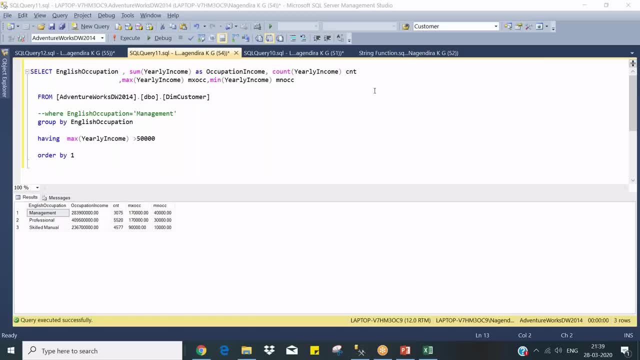 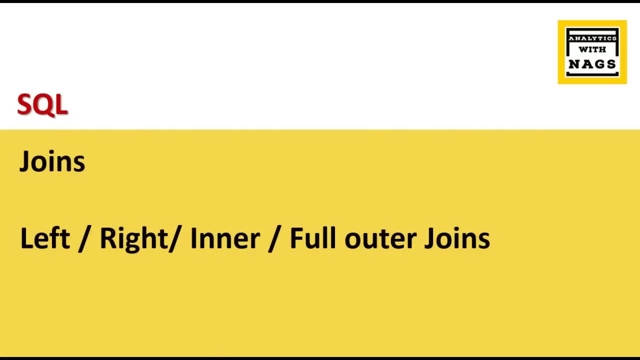 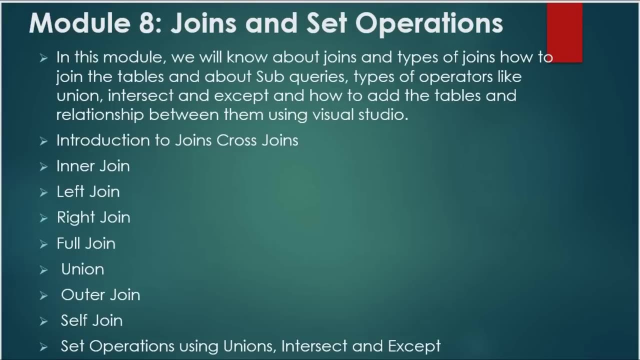 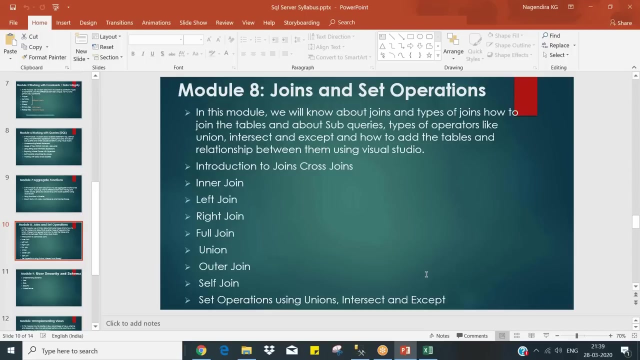 any confusion here. now i'm going to start a interesting part, guys, about the joints. okay, but now i'm going to start a interesting part, guys, joins. okay, when you go for join, join is nothing, but you join two tables. so when you will go for it, no one says okay, fine, let me, when you want to compare data. 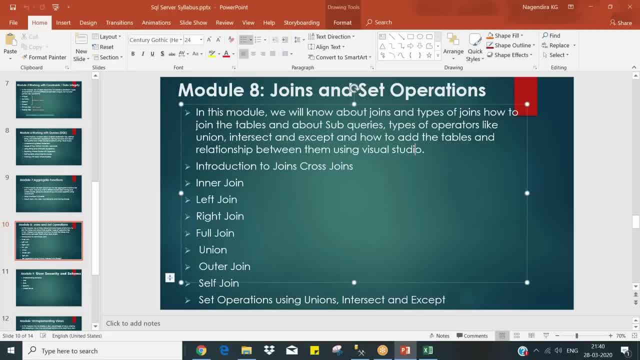 with one table and on both tables, between both, not only comparison. there might be a situation we need to compare. uh, basically, yeah, one at a time to retrieve the data. also, we need to, uh, we need to use the joints right with the common column name. from that we can. yes, 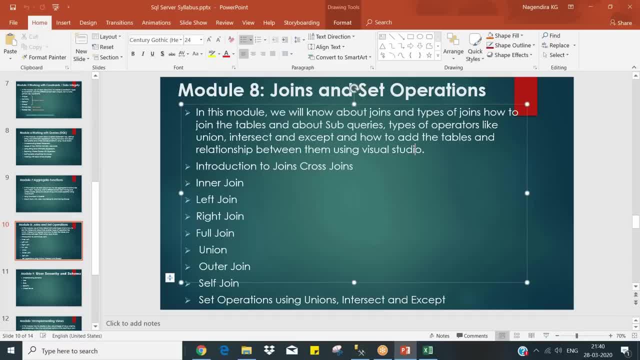 combine, so the table and get the data. yeah, you, we saw about primary key and foreign key, so in that case you need to get, uh, the product information, the purchase. you remember the customer constraint or customer master and customer purchase. so in order to retrieve, so you need. 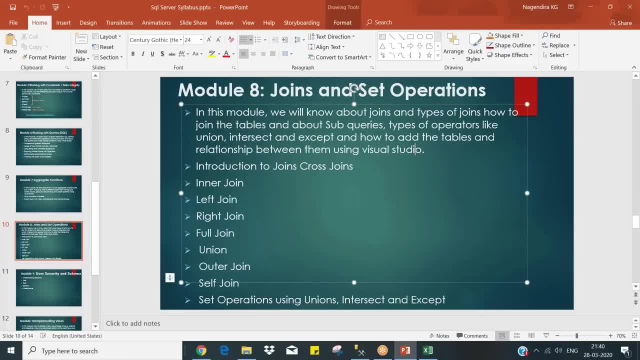 some information from other tables, you need to join. okay, this is the thumb rule. so, in after joining, you want to apply some condition, as um pravin highlighted? yes, you need to do it, that is fine. so, basically, join is required because you need to get information from another table. 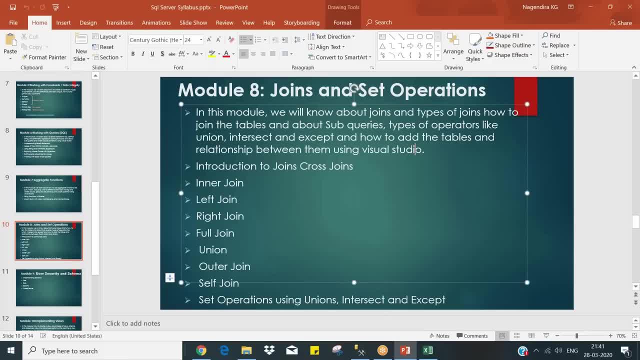 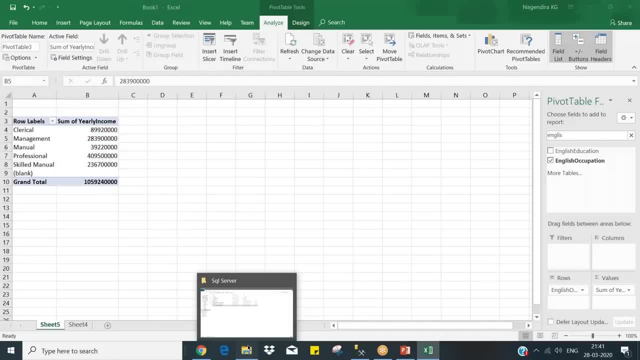 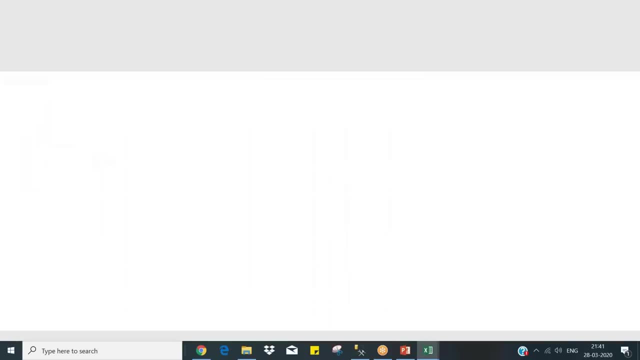 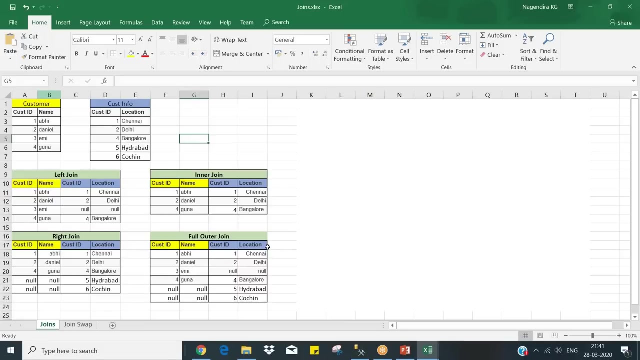 that is why you are joining. that is the thing, as simple as that. okay, yes, with this note, let me open um joints search. alright, let me see. okay, our content is accepted here. so, uh, i want, uh location information for the customers. that's why i need to join in this table to get. 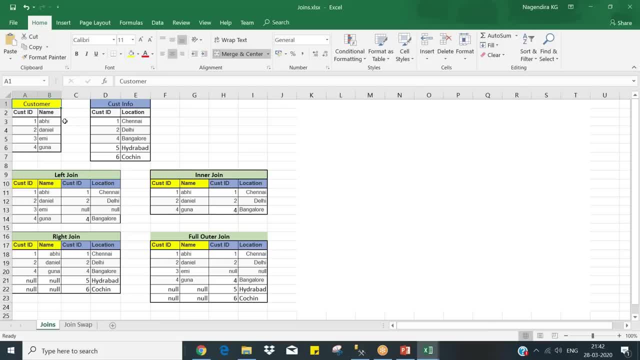 the customer location. now what is left join, inner join, right join, full auto join- let us see in this picture. so left join means i use this one as the base table and this is my right table, so this will include all the records- okay, all the records from the left hand side table, then whatever is matching. 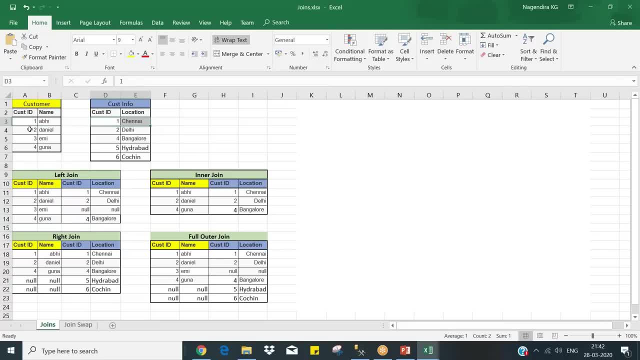 that is for one is from chennai, for two is from delhi, for three there is no matching records, so the result set is null. and for four you have bangalore. fine, what about these two guys- i mean five and six, since it is left- join. this will include only all the records from the left hand side table. it will ignore what. 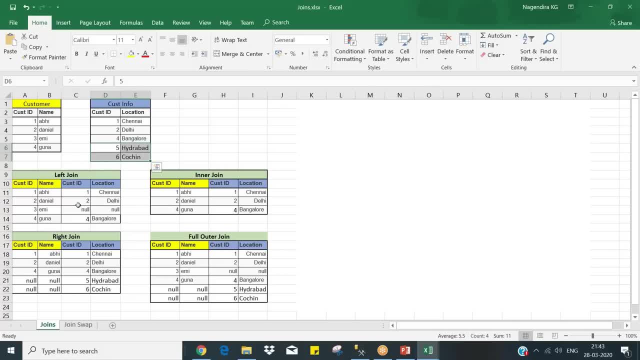 are the extra records in your right hand side table. it doesn't matter to it. so this is your left join will perform okay. and in a join or e join, people will say like when you do yeah, do we classify which one is left join? yeah, see, now you try to understand. uh, left join inner. 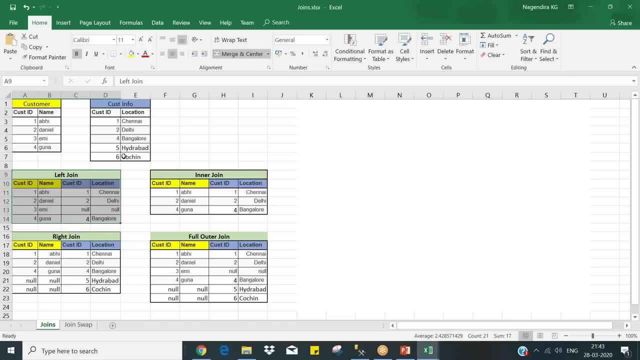 join, right join and, uh, we need to use appropriately, when you understand the left join, right gen and inner join. okay, then you need to query. while querying, you will decide which time to use: whether it should be you we need to use inner join, whether we need to use left join, that you 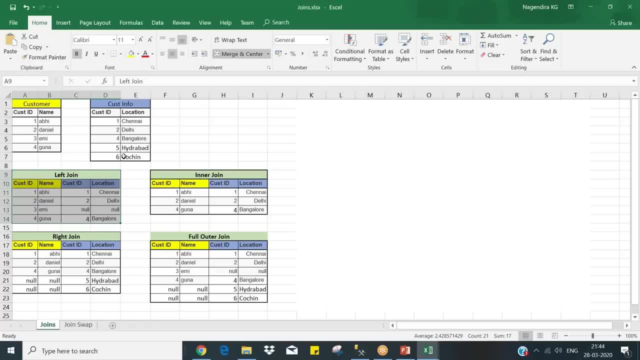 will decide. okay, okay, but if now i you try to understand what is left join, what is in a join, what is right join for now, then while uh querying, we will see you will understand when to use this one. okay, okay, here is note in a joint. so in a joint, like it should match both the sides, the record should. 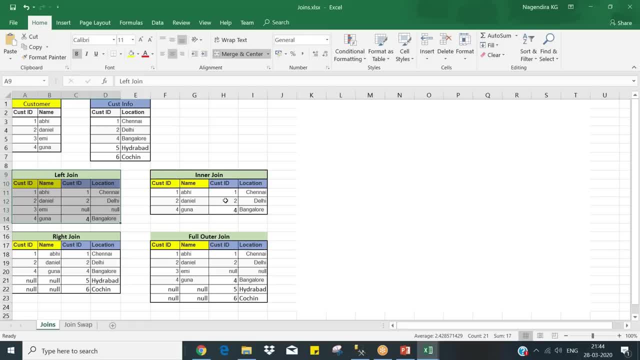 exist on both the sides, so that data will come here. you see, like, for one it is there, for two it is there, and for three there is no record exist here, so it will skip this record itself. okay, now for four, you have bangalore, so this is your record. so these two columns from this table and these two columns. 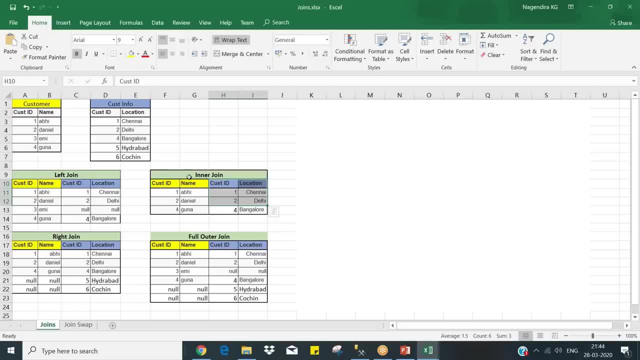 from this table i mean this two column from this trip. so this is your inner join. so both tables should match right join. like i said, it will include all the records from your right hand side table and matching records from your left table. that is for one, two and four, only five and six there. 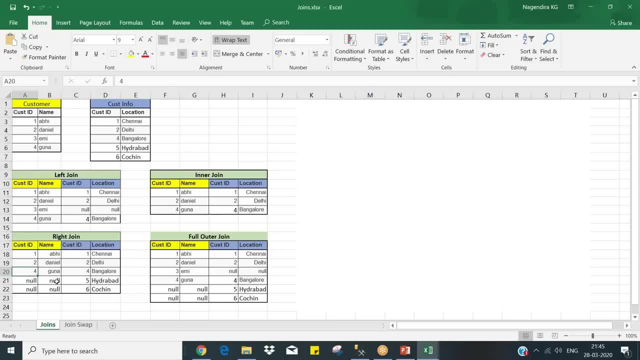 is no records here, so it will populate null. there is no for three. me is script here, since it's a right join. right join means it will include all the records, only matching records from left table. this is your right join. then a scenario like full outer joint, full level join, which includes both: whatever in your left hand. 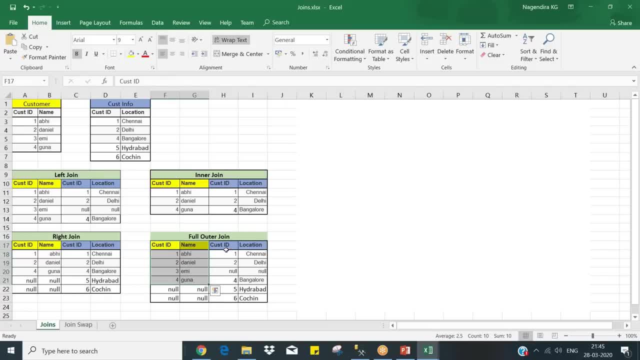 side table, everything. four records and whatever you need to use in your left hand side table, your right hand side table by records. so if it is not matching it will throw. i mean it will have null values for this. it is having not matching left, so it will have null values. this is your. 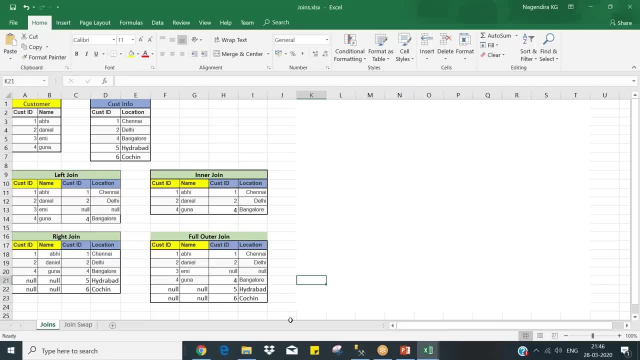 full loader chain. this is about joins guys. any questions in this? it's clear now, hello, you can explain the full outer join. yes, so repeat full loader join or repeat all the things. all i do not understand anything. oh, who is this? i mean pk from web one and pravin pravin. okay, okay, fine. 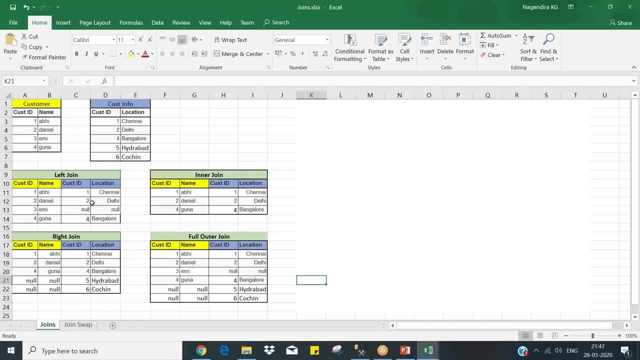 you change the name? okay, fine, first i'll explain the full order join and i will explain, uh, the other things once again. so full order, join. so, basically, as i said, forget about these thing, guys. okay, forget about this, i can't hide it. hold on, okay, okay. 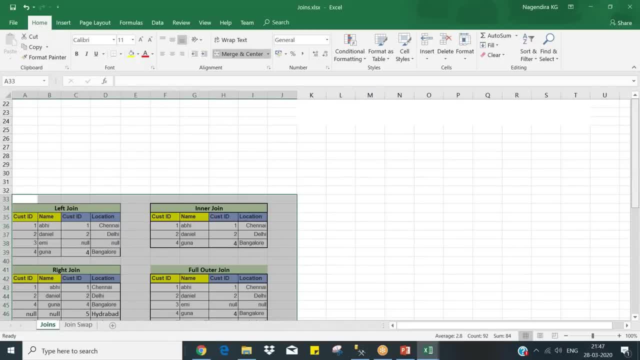 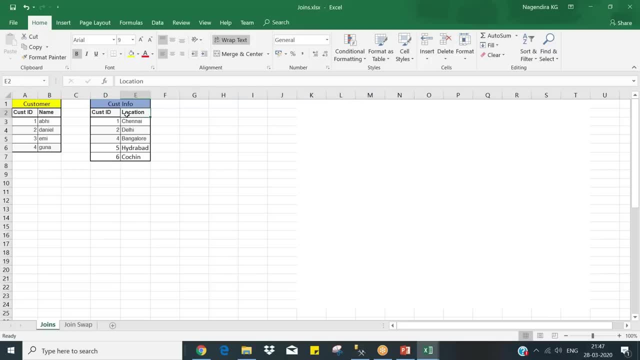 hide it here. okay, now you see, this is your tables, okay, customer and customer info. so now you tell me what is the location of guna. location of guna. hello guys, you can unmute one at a time. bangalore, bangalore, bangalore, bangalore, bangalore. 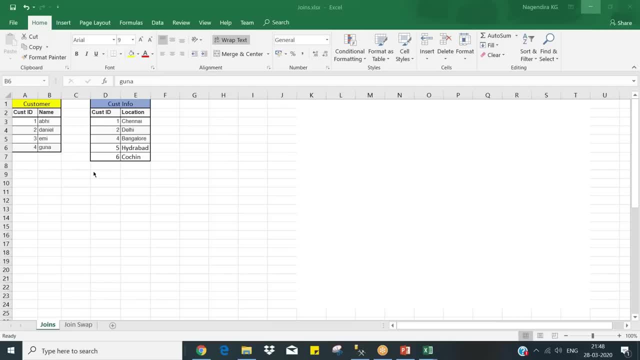 canada, canada, canada, canada, canada, california- no location. phary, Jorge, ch الد här, ch الد- 200 نفع based on the match. if they don't have a location, then they have a null. so basically now, sorry, Bangalore for him, Chennai for him Delhi. okay, this is what you are expecting for. 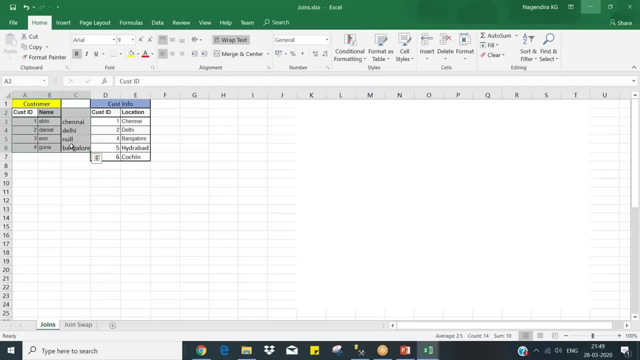 a join. as I said, join is required only when you need to get information from some other table. now I need a location information, so I will go and pick it up and i will fetch it as a result. now, how to do that. you can do multiple joints. okay, what happens? 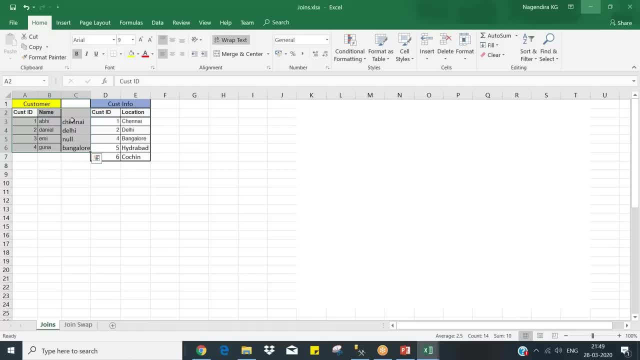 i need all the employees, i mean all the customers. okay, only having a location. i mean to say, if the- if he contains null values, don't show him, then i need to use the inner join. what inner join will do? it will go and check here. if it is there, these two guys will come. 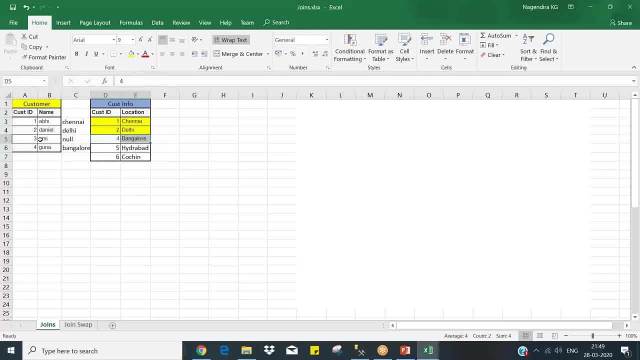 and this guy will also come. i mean to say these two guys will come and this guy will come because he doesn't have a location. okay, so you skip the record. if there is no matching record, you need to save the location, so you skip. if the question is like that, if the request is, i need those customers. who is? 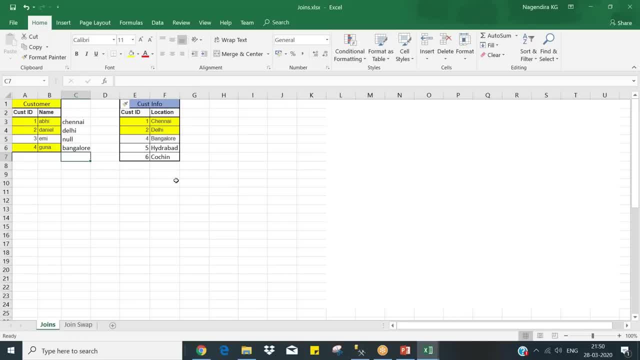 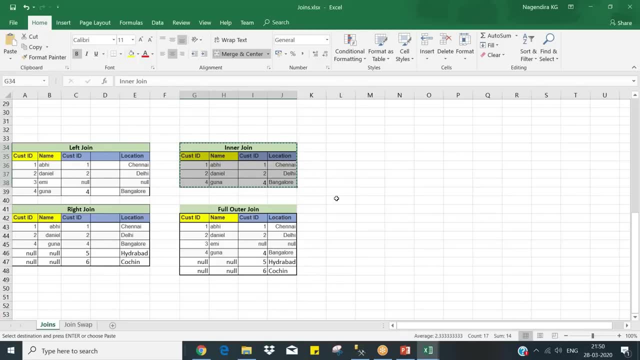 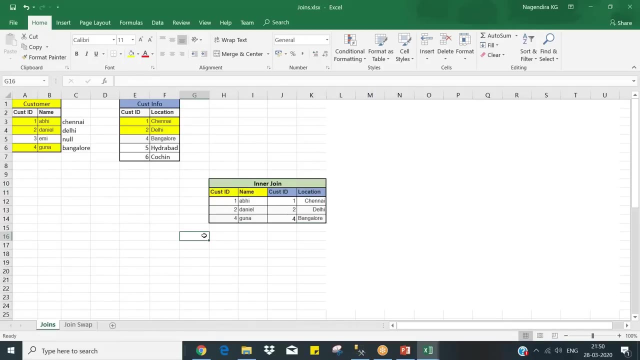 having a location. okay, then you need to do in a join. what is the inner join here? if you see, now i bring the inner join first. okay, so in a join, as expected. one, abby chennai, two, daniel delhi, guna bangalore. so these three records asking when i ask, i need only the customers. 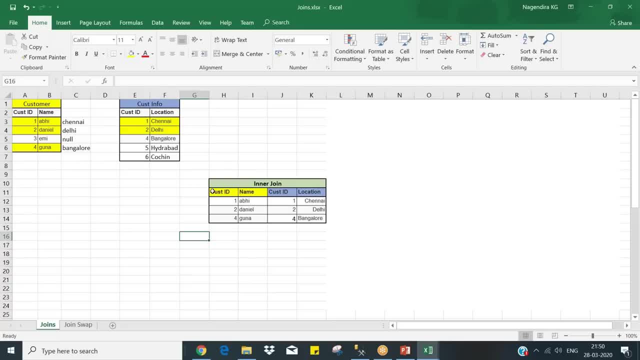 having a location, so then you need to perform inner join. okay, now people ask a question like i need all the customers, whether, if they have a location, bring them, if they don't have location, show them a null or default in something else, whatever they can ask. okay, i need all the customers. 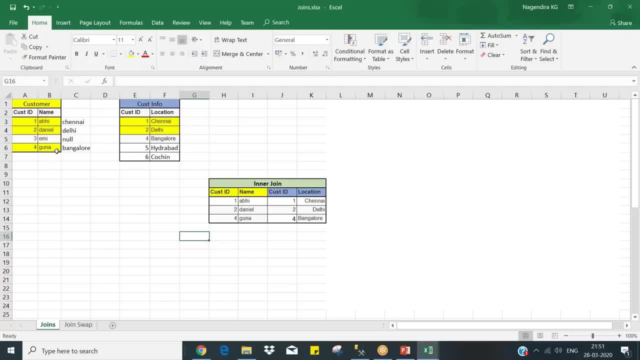 need all the customers, but if they have a location, bring them. if they don't have, show me none. okay, if the question is like this, then I will show all the guys and, along with the location. if it doesn't have, it will show none. then I need to use left join. 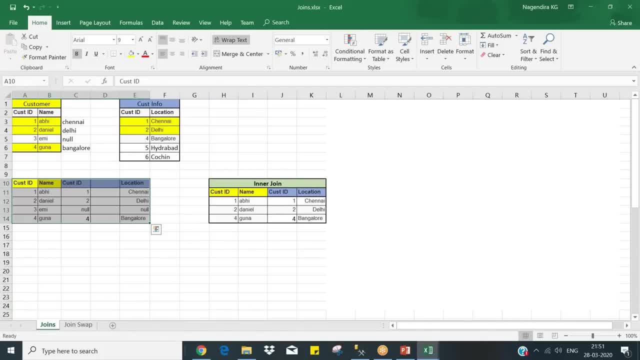 you. so what happened here? I brought all the customers. okay, whatever here I introduced, I brought all the customers. then, whose location is here and customer location is null for me, but I need to have all the customers. I should not lose my customer information because not having a location. 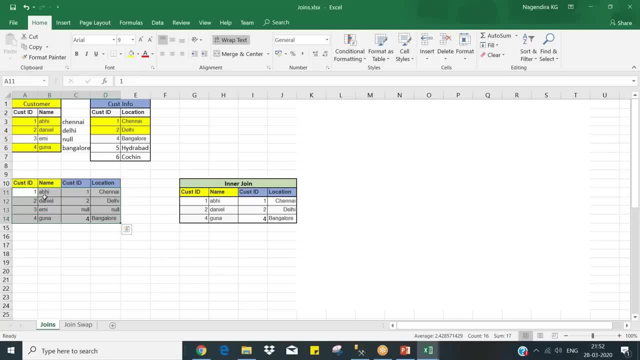 I need to count. if I count, this is my query output. if I count this one, it will give me proper customer count for count. if I count this one, I will skip the customer count. I will show only the three count. but it is which is not correct. but if the question is like that, then you need to use inner join, it is. 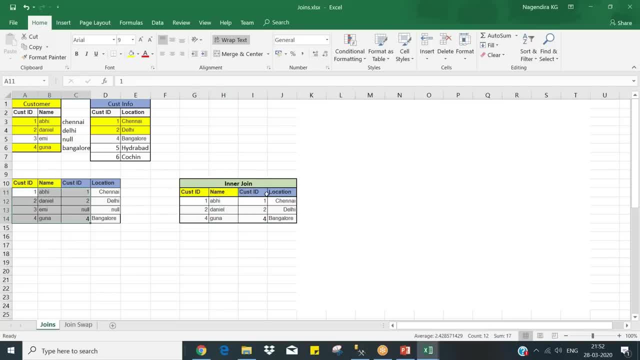 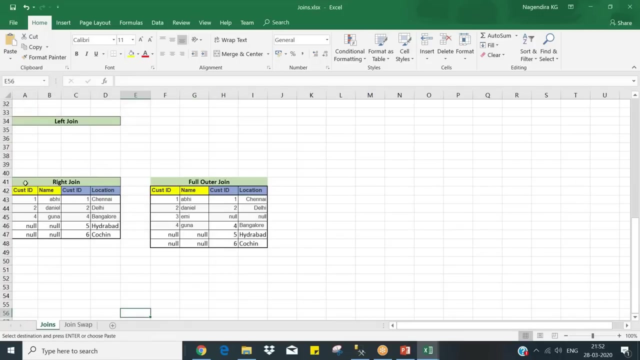 always safer to use left join. but, based on this situation, you need to choose between the joins. either you need to use inner join or let it join. okay, okay guys. now I'm clear. Kevin, there are too many detours. then all we can decide, the way we can use left join. 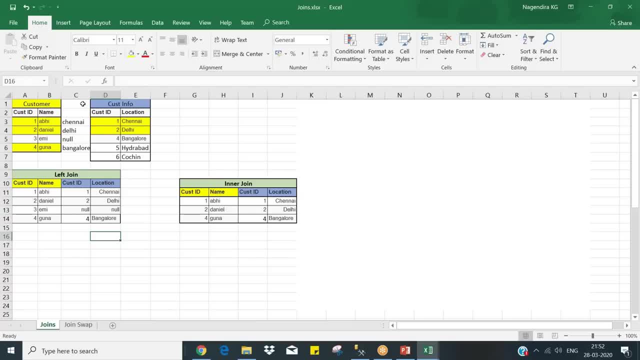 because some customer using data switch, choose the any anywhere but which I can use, and clickонец. then now we can decide the left join or not because some customer ready the location if there are too many data. if there are too many data, then all we can is a way we can use left join or not, the li escuch. we can choose which is the left join or not because some customer ready location we can use, but besides which we can choose our wherever host we can use over here in this go we also choose a daily SEO choice option. 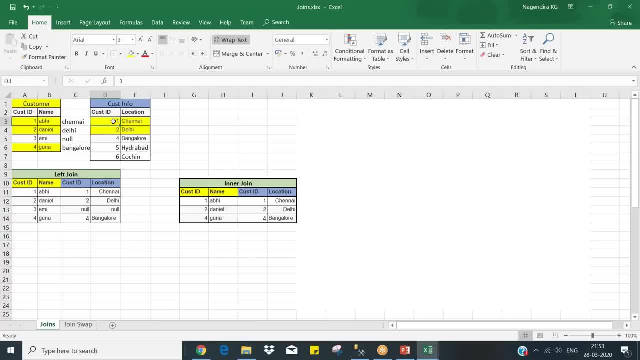 doesn't matter. see, data doesn't. you are saying, uh, here you want too many data or multiple records, or too many data means, which you mean multiple columns. no, no, the left join the customer id3 has emi and location is null. so yeah, uh, we're not sure. 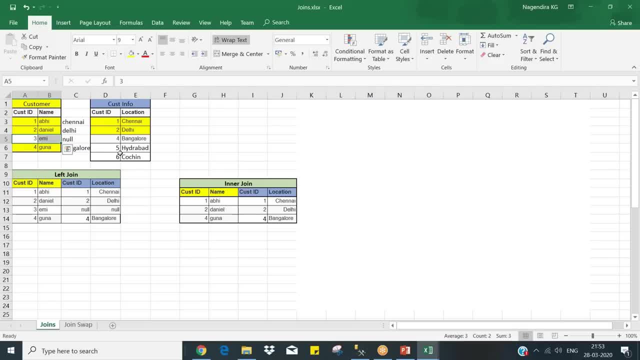 whatever the data is having null. so no, no, no, data is not null. see, data is not null. there is no data at all. see, simple as that, deepak. they are asking: i need locations for all customers where you are storing your location. you are storing it here, so what you do? you go. 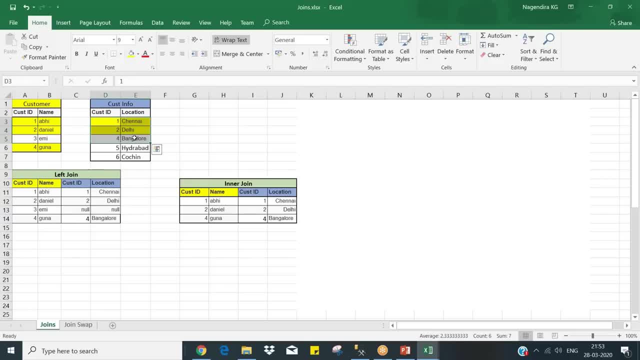 here and pick up all the locations based on the join, but the location for me is not there. it can be a scenario like emi does not provided you the location. she has given only her name. she didn't provide her location. that is fine. it is a valid business case based on your database design. 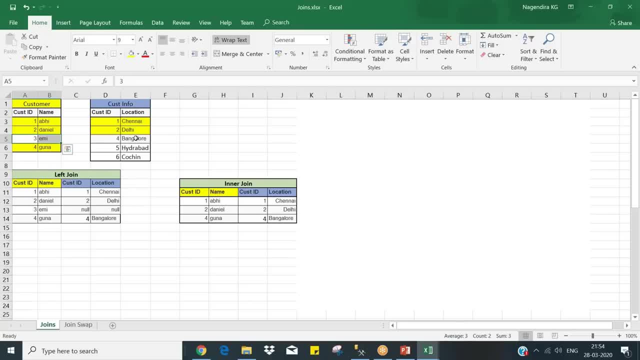 she refused to give her location, so there won't be entry here. so she didn't provide you the location, okay. so, uh, what's your question in this? okay, yeah? yeah, that is one. so it is not mandatory that you need to have a location or something. it's based on the business in it. this table can be anything. for simple understanding of this, this is: 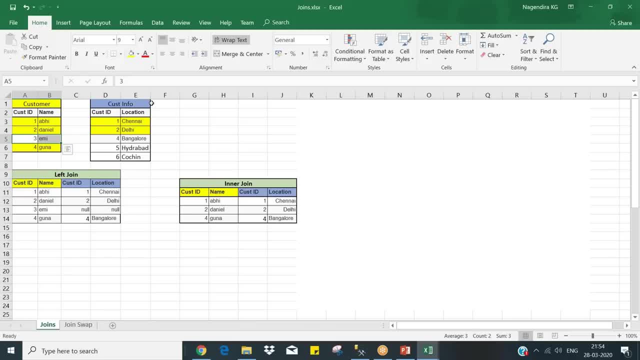 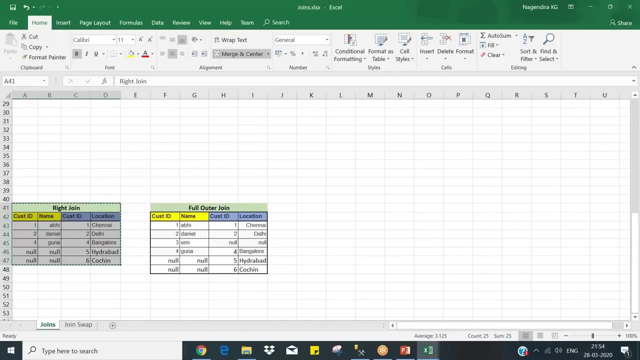 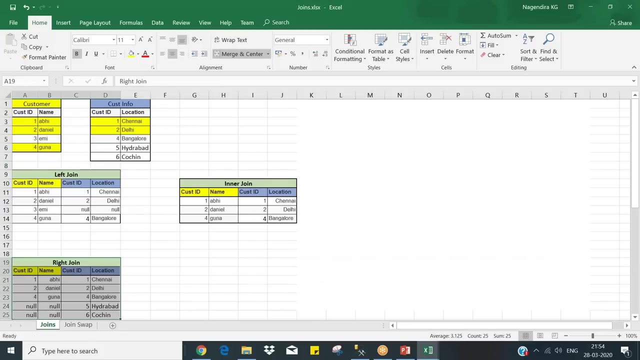 the thumb rule used for any complex uh joints. i mean complex tables also. okay, fine, so right, join is same as like that. yes, following the those of which we have seen in d ata. any of those are on d api, right, let us go ahead and add c繼續. 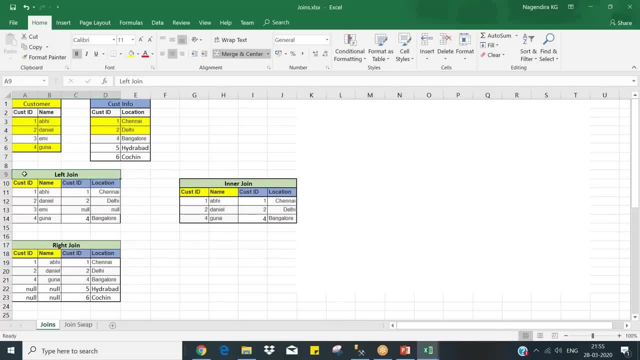 go ahead and add note. as i said, go for joint. that is the thumb rule usually for joints. okay, you use left joint or inner joint and right join is typical case. it's good to know like you need all the locations to be there and whichever customers. you map something like this. you got the point. it is vice versa. okay, if you have. 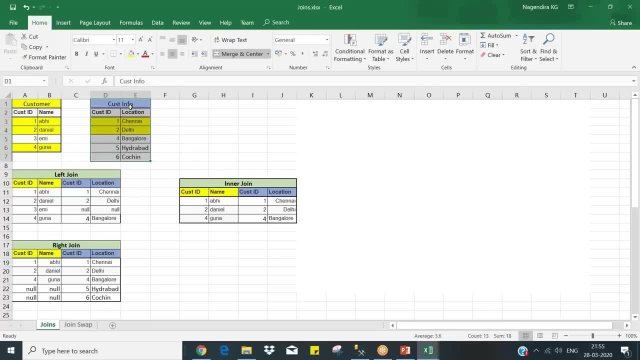 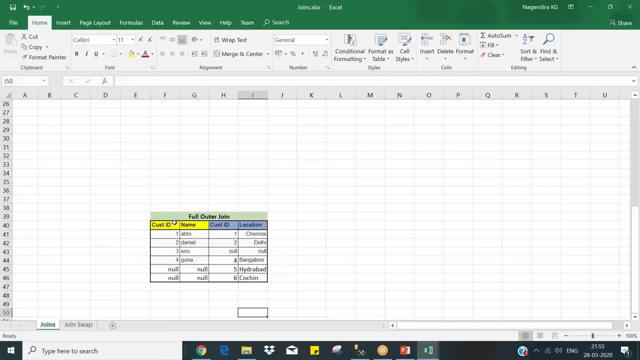 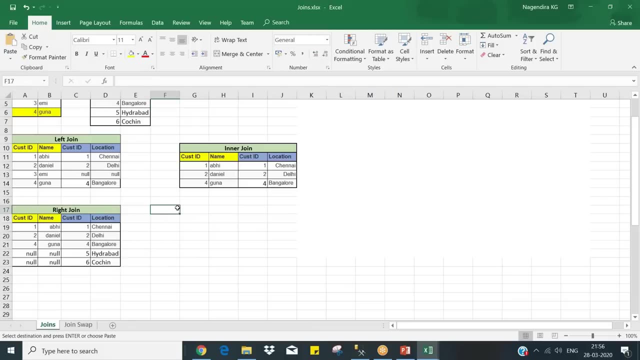 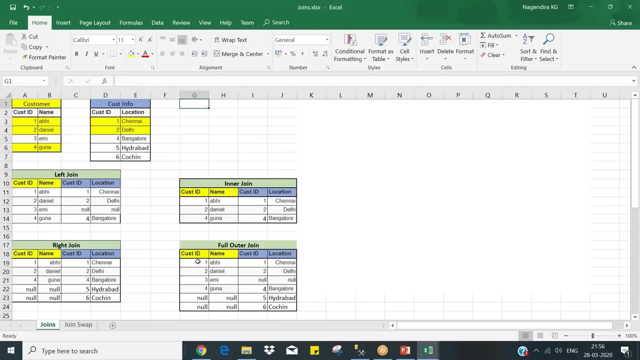 this guy. here i mean this swap. if you use this one as a left table, then this is nothing but your left joint. let me explain that later now. already you got confused, so i don't want to confuse again. full outer join on our contrast. you will have both the information, all the elements in your 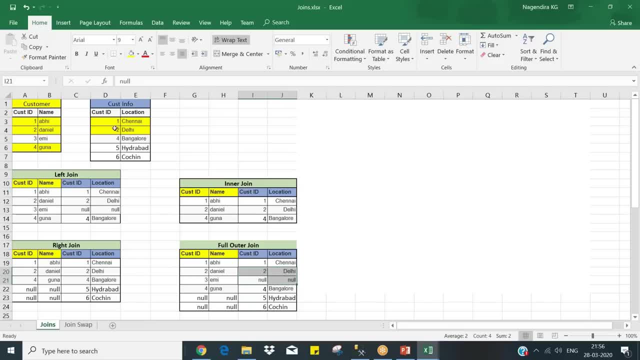 left-hand side table will be there. whatever matching it will come, and whatever you have here- i mean right hand side table- everything will be, uh, displayed, i mean in your query and with your null values. whatever matching in the left side, that is your full outer choice. this is the case, guys. okay, let us try to query it with our 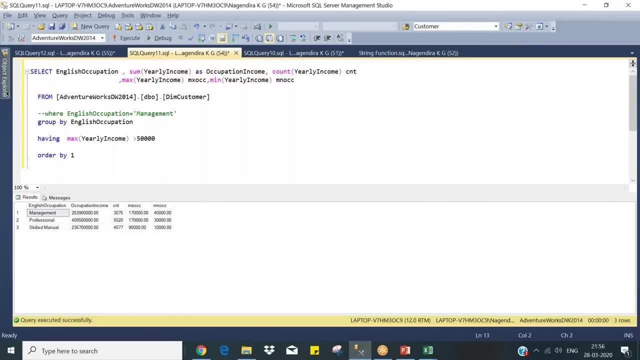 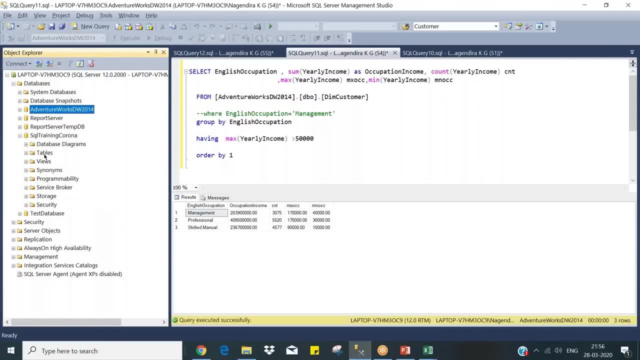 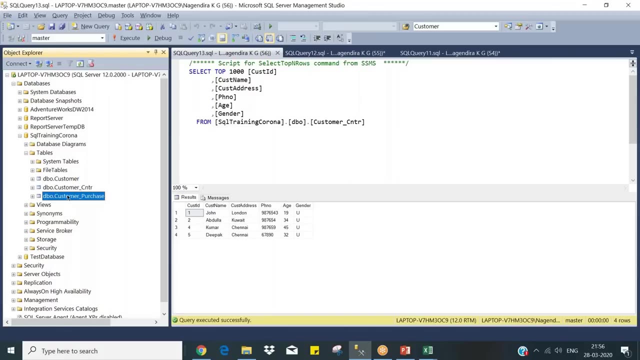 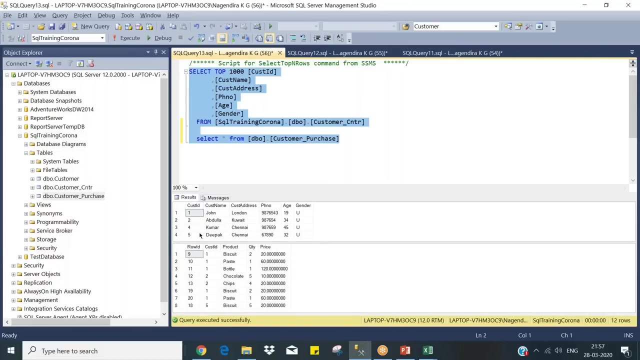 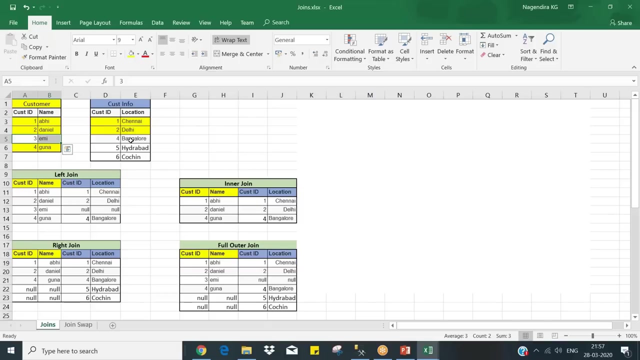 customer and customer constraint purchase table, how it works. so here again we have two piece of information: whether we have created um, i think we have created uh, this one, right? what happened? so primary key, foreign key, right? yeah, all right, we don't have any uh since c. this scenario will not happen for me. okay, you have entry. there won't be any cases this. 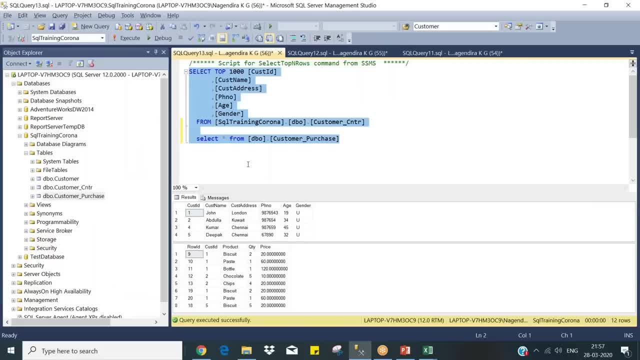 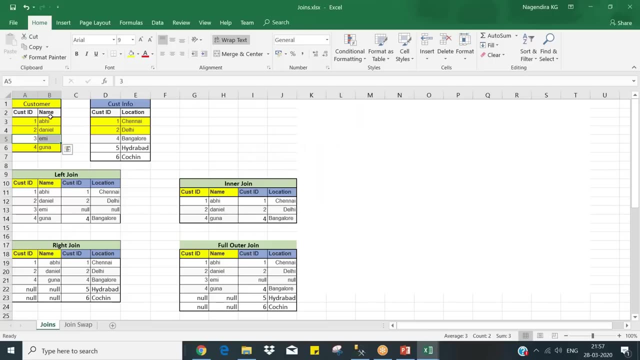 is fine, this is fine, absolutely fine, yeah, uh, okay, what i'm trying to say is for four, there is no entry. okay, when we do the left join, now i will say, like how to do all these things? i want what are the items. now, you see, guys, i explain only with one example for a, b, i want only the location, okay. 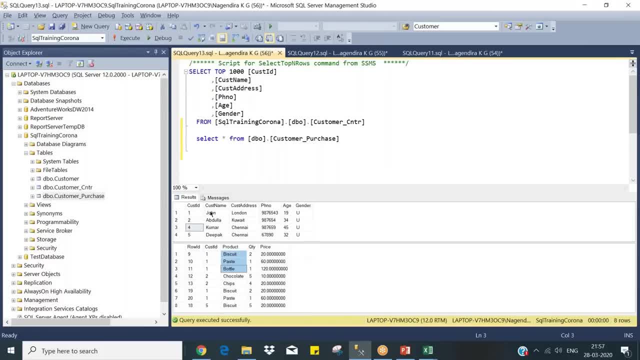 here i want. what are the things he purchased? john purchase biscuit paste bottle. so i need customer id. john. it will repeat three times. now let me show that. select star from left join. see now i take this particular customer master or customer constraint as my base table. base table, okay, and i'm using it as a left hand side table. left join with. 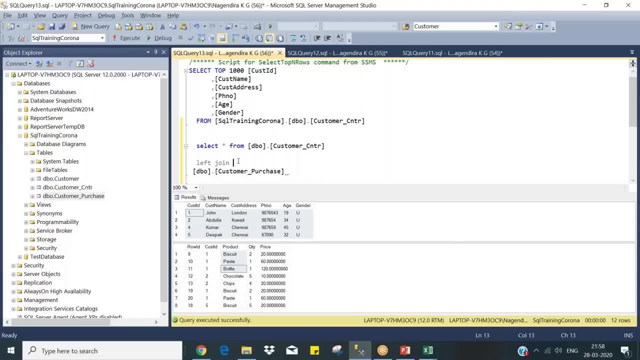 customer purchase table. okay, as i said, i can give uh ally's name. to make it otherwise, i need to use the three name convention schema name, table name and column name to join. okay, instead i will give a alice name as master and this one is transaction. they'll join on. okay, this is the syntax. so this is my first table. 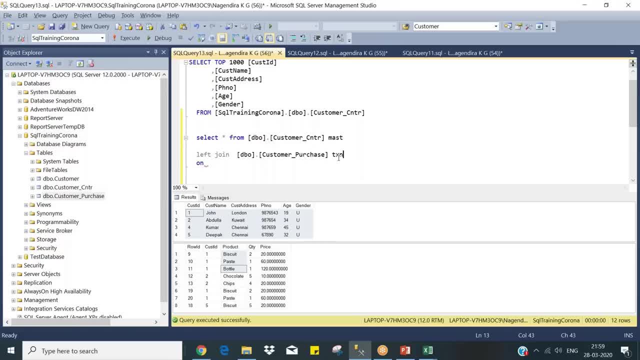 left to join with the right hand side table. i'm giving my um alice name based on what i want to join from: master table customer id and in transaction table again a customer id. okay, now see, always a result of a join is again a table. so you have a table here separately. you. 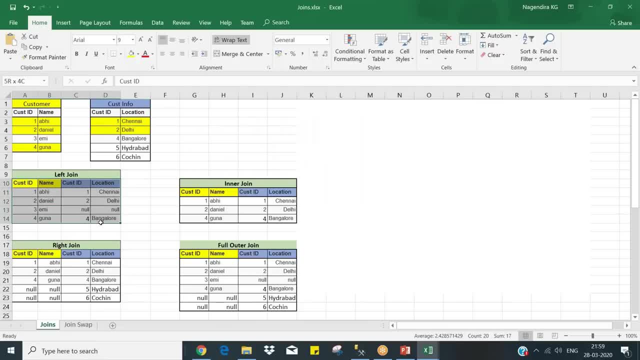 have a symbol in separately. that is why i put a combined together. once you have a join here, both the tables will combine. once you'll link these two, both tables will combine and give you another table. so from here you can do any var condition. i want only delhi means, so i want only the delhi customers. then do the join, then filter. 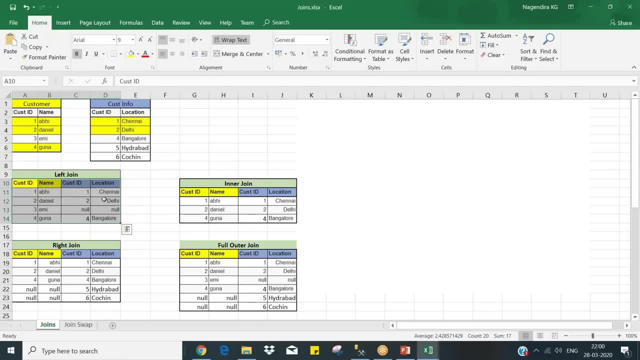 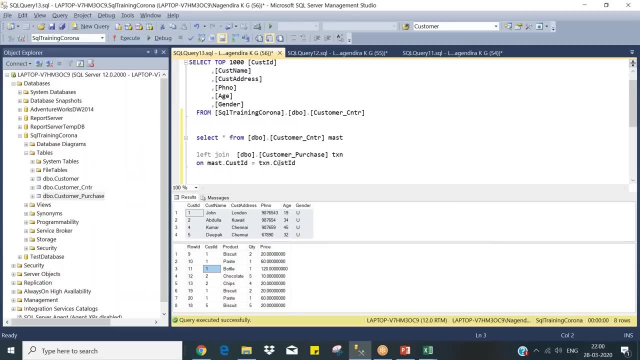 with delhi, so it will first evaluate this result, then it will filter only this guy. this is how it works. now let's see that one now. uh, when i do this- so from here the columns are conflicting- i mean, i'm going to basically just go in here and there, and then i'm going to specify this one here and here. 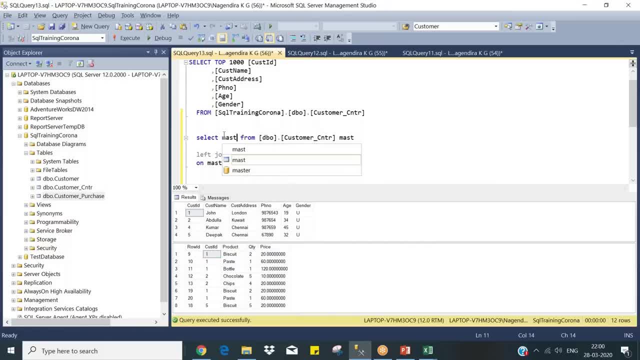 also customer id. here also customer id. you need to specify which column to specify here in order: master dot customer id. i want master dot customer name, comma here. this is enough. i want, uh, these two guys- i mean here customer id and customer name- and whatever he purchased- biscuit paste and bottle. that is what i want. 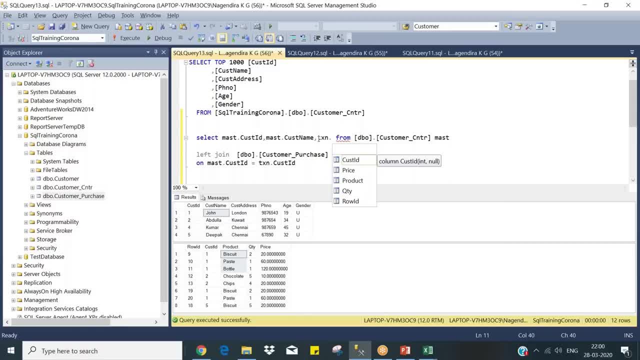 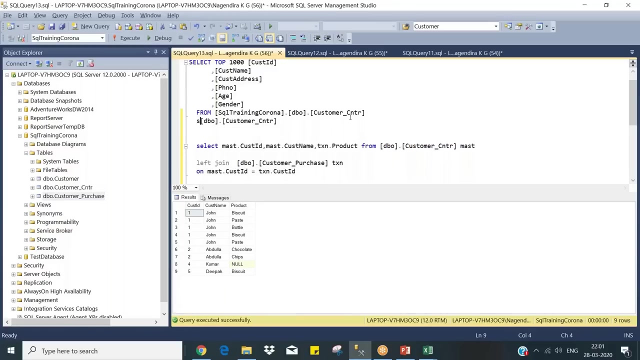 where that data exists: transaction dot product. that's all. so i want these guys. that's all you are done live join customer id and whatever columns you want, you get it here. so john has got multiple things. let's see why. yeah, he has purchased once again in bottom and we have entered another two records. so totally, 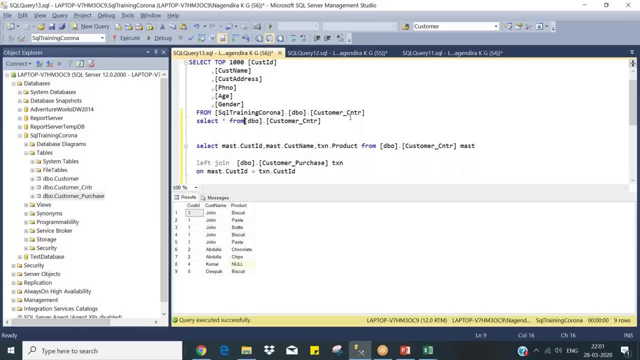 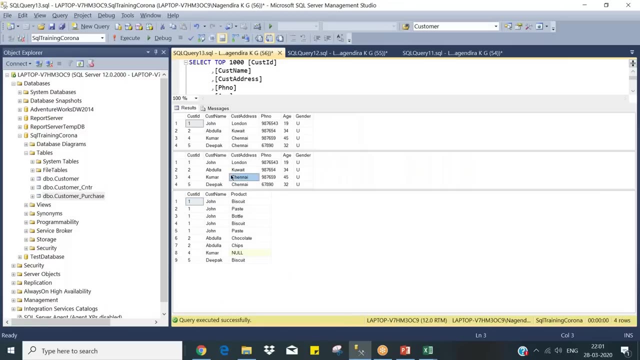 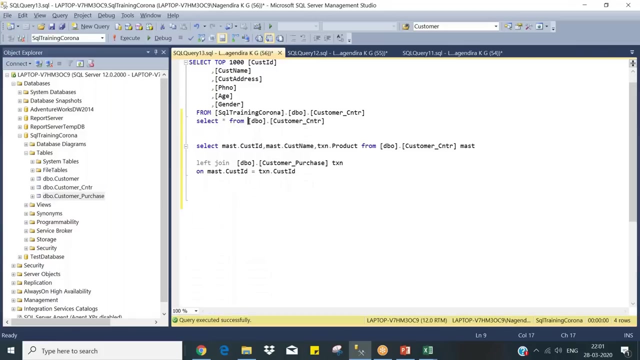 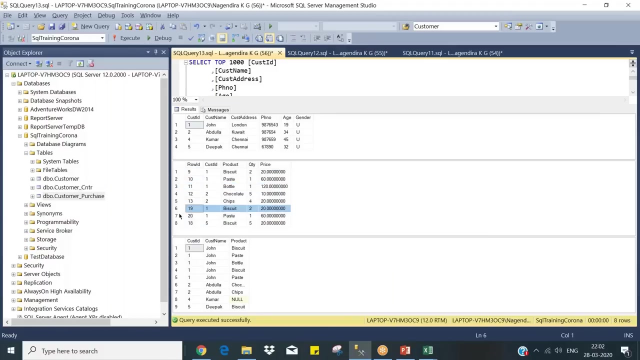 he has got four or five purchases. let us see all three together, then you get a good idea. sorry, sorry, yeah. so here you see the three records for john and another two records over here. so for john, biscuit paste portal, these three records. then biscuit pissed, again these three records. 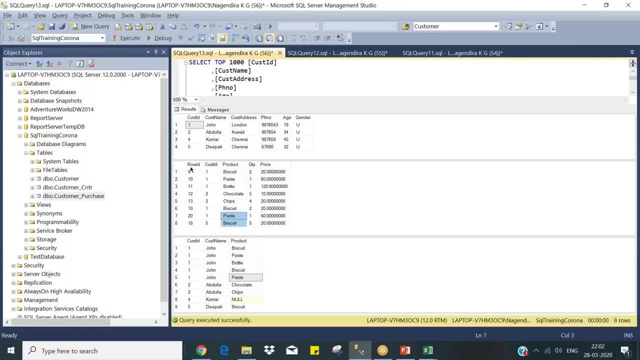 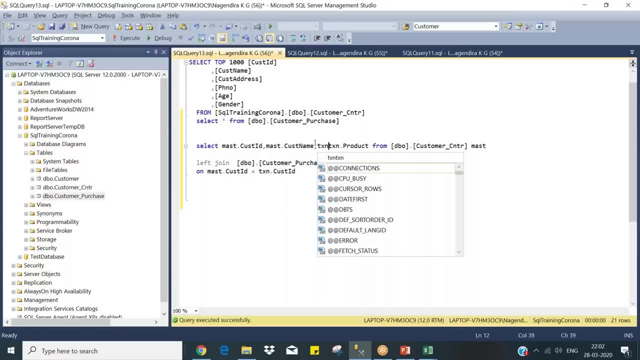 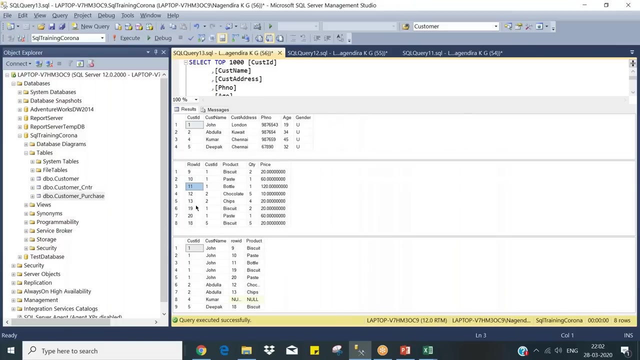 records. Instead of that, to distinguish what is this, What is this record, You need to have this row ID to clarify Transaction. Okay, You see here for John, this 9,, 10,, 11, you are 19,, 20,, 19,, 20.. So John has purchased these things. Now you've got the entire thing. 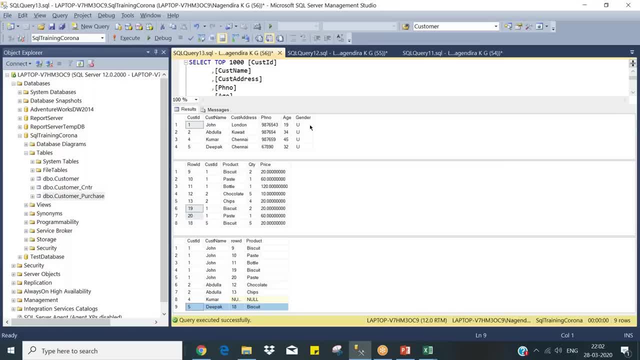 Abdullah chocolate biscuits. Now in this you have a left joint which says, like I included all the records, all the customers. So I got one, two, four and five, whatever the matching records, in my transaction table, right-hand side table, all the matching. 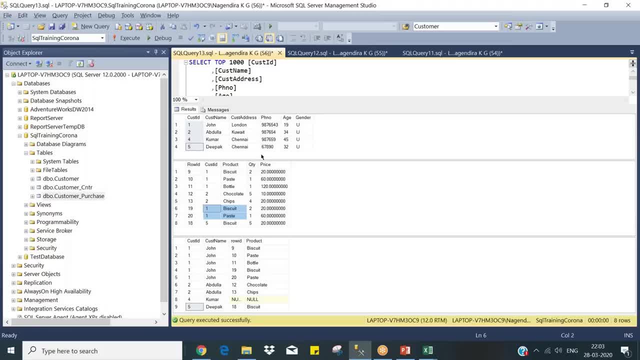 records For this guy. it will be repeated. So I it is not a duplicate. You cannot say it's a duplicate. It is actual typical requirement. because what are the purchases made by John? John has purchased biscuit paste, bottle biscuit paste again, And based on this transaction. 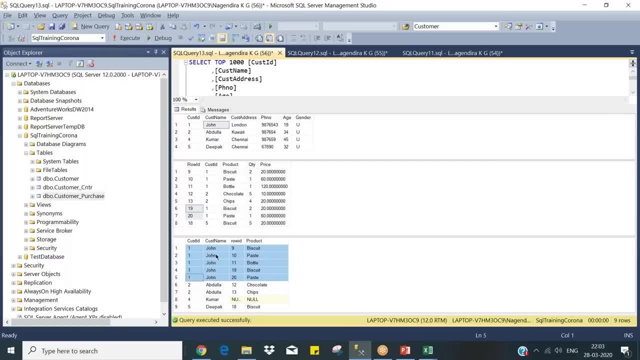 ID. I have brought everything. This is not. you say it as a duplicate. This is actual thing. The purchase flow: Okay, This is the purchase of the bill. You consider like that- Now you see the null record here- Why He is a customer but he didn't have any purchase. 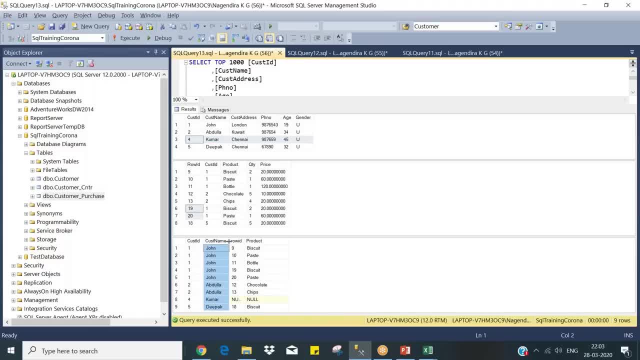 record over here. That is why you don't find any records in this table, So it turns to be null. This is your left joint, So which includes all the matching records. Now, in case I do the inner joint, what it will do? whatever is matched, those things only it. 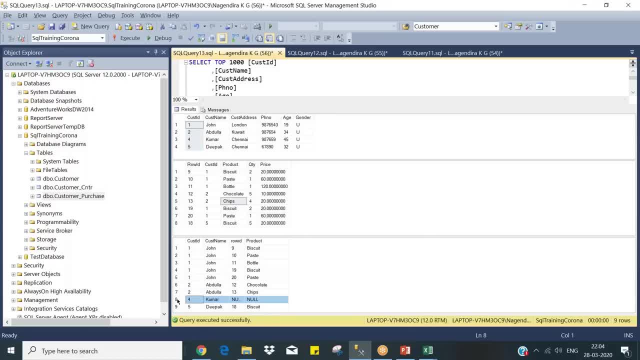 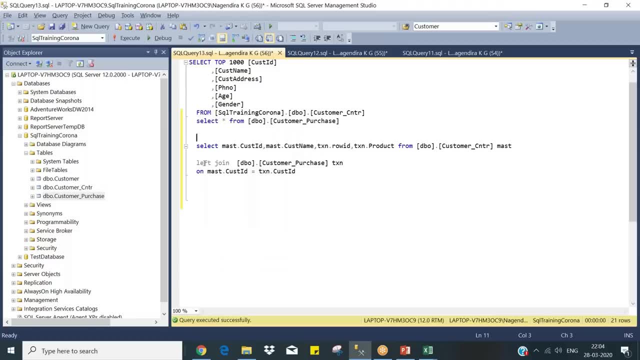 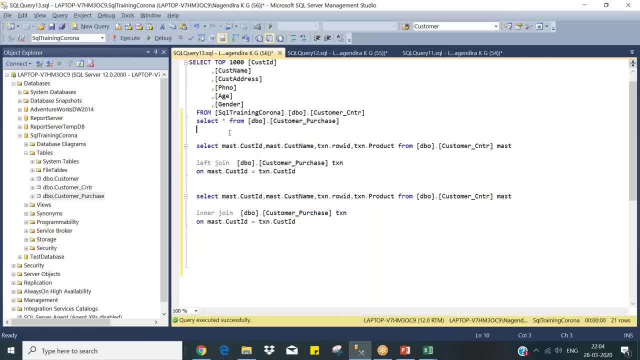 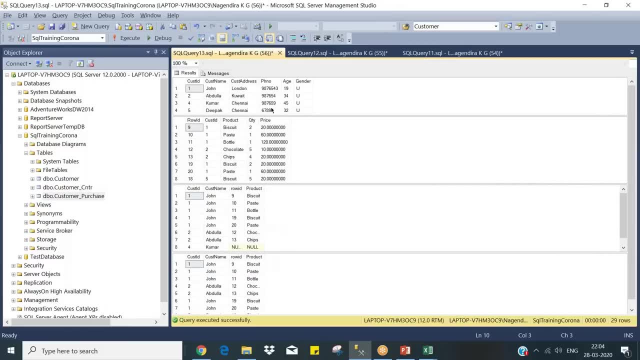 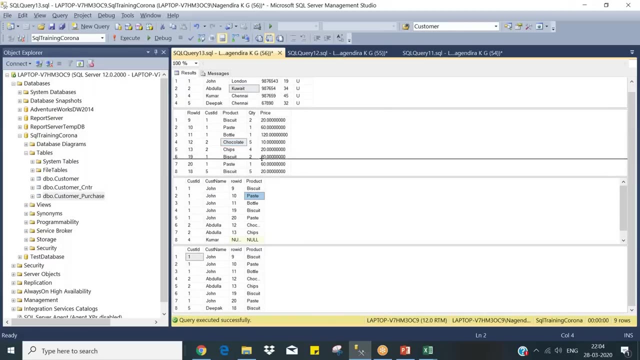 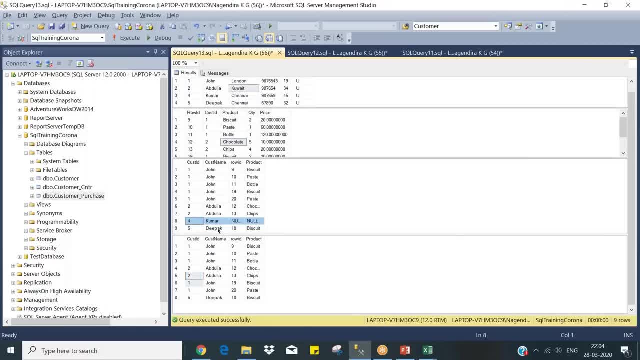 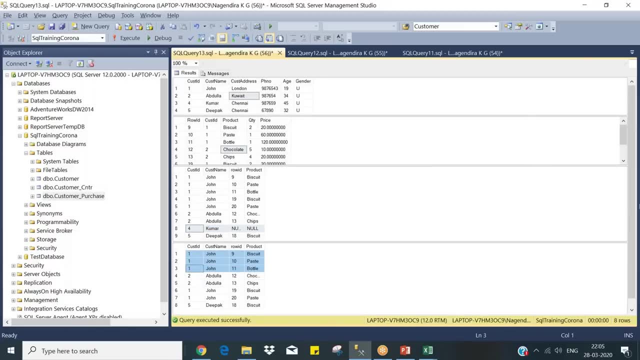 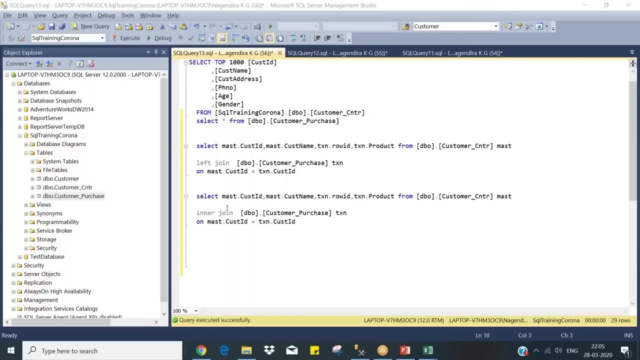 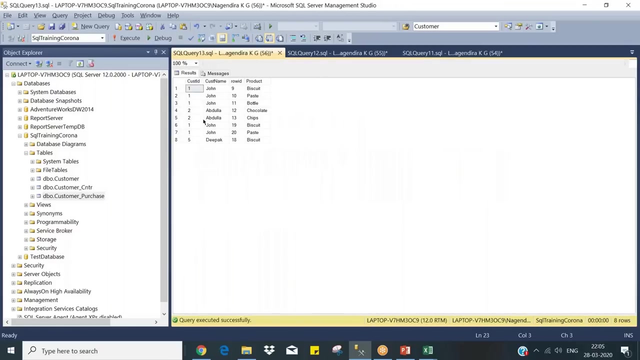 you see only eight records. the fourth record got missed. okay, this is your inner join. so this is the purpose of join this. hello there. and you say, right, join here. same result. it will include all the records. whatever this match, you will get all the records. and since I imposed 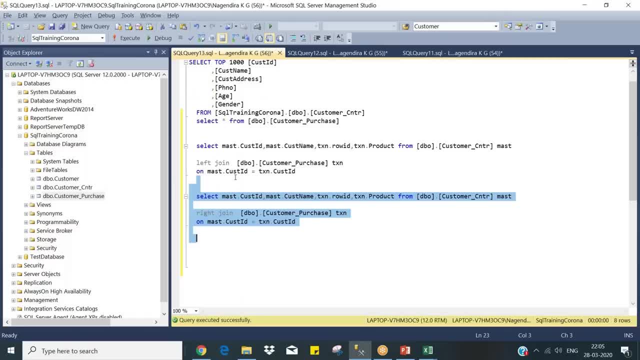 foreign key constraint. you cannot have a record without having that case. okay, that is why you don't find anything else, but it will have a matching case here. you focus on left join and in a joint. that's more than enough. don't confuse with other joints, but it's good to know. any clarification required, guys, joins is 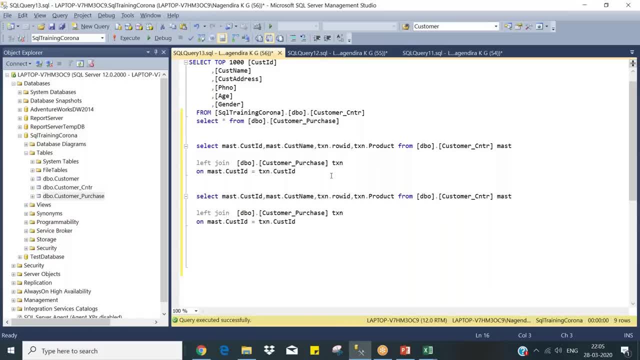 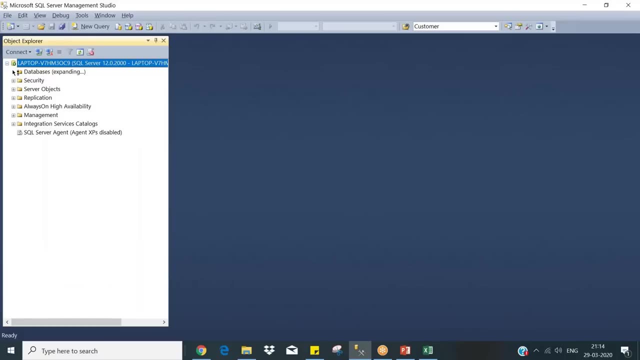 fine, you got it very clear. until you practice you it will, it will be really difficult to understand. you need to figure it out. oh, this is what it is. okay, you need to ensure that one. now let's take one table. we're just having multiple joints so that we can go. 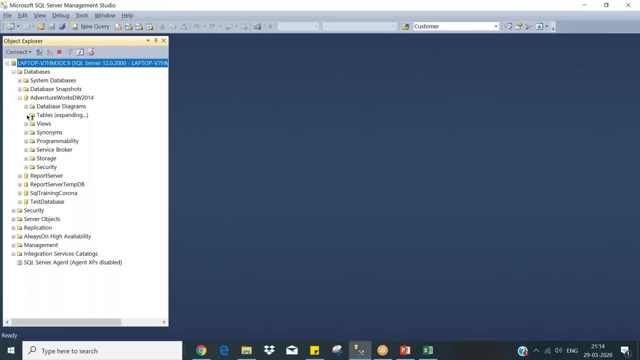 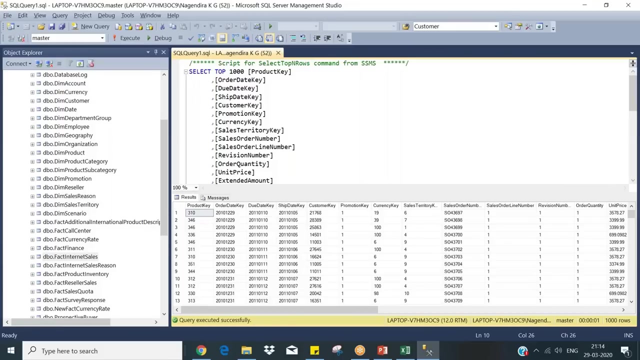 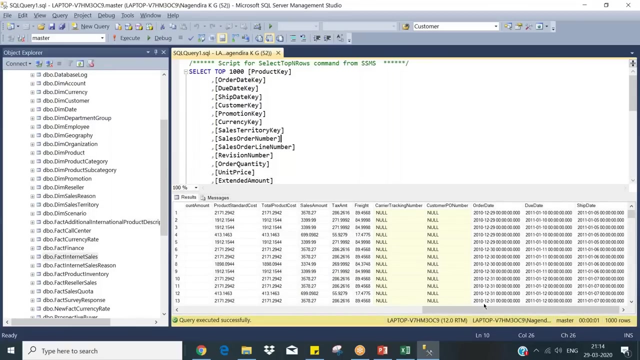 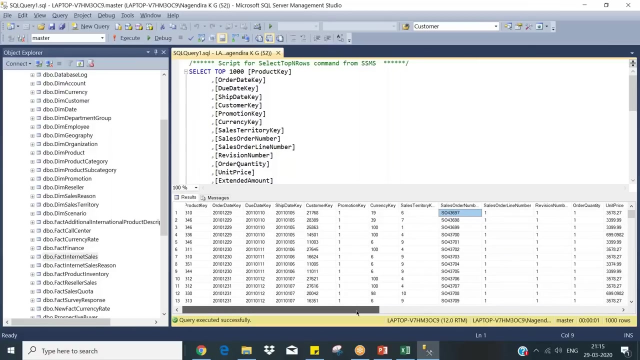 forward for that. I need some table here. you beண. okay, here we go. so this one is set down, okay, however, close a bottom. it is kind of right here and now. let's test you brandум. you have order number, then you have a unit price- how much it is, and order. 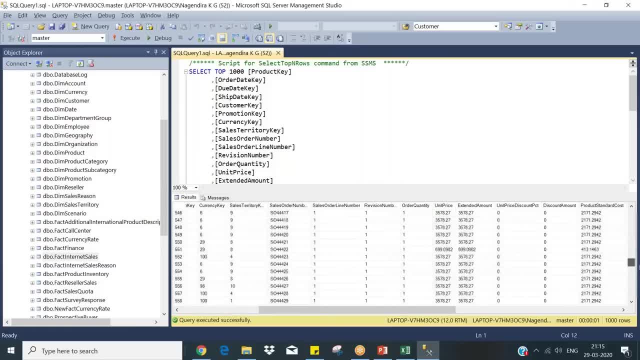 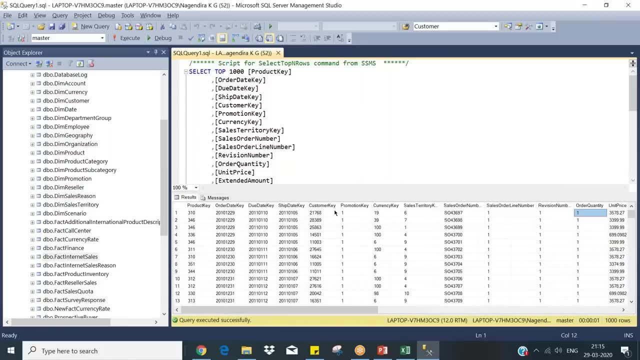 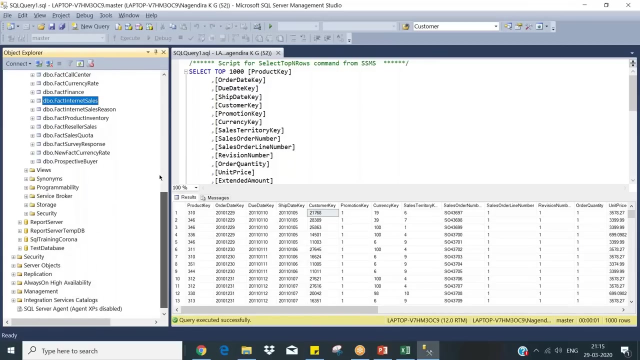 quantity. quantity is one, two or three, something like that. okay, then what is the product? everything, now, this is typically which is a customer as a as we created primary. find me we already discussed that one. now, you see, here I will go to our table first, then I will show you how it looks like: the keys. 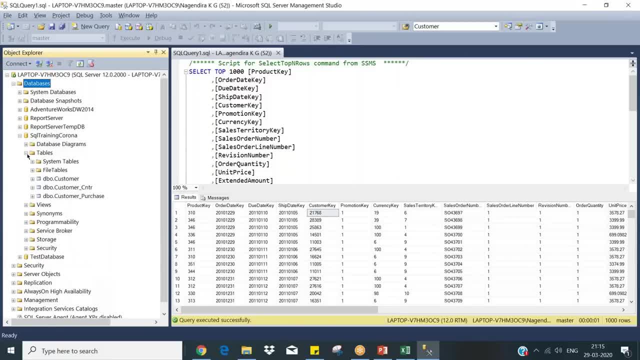 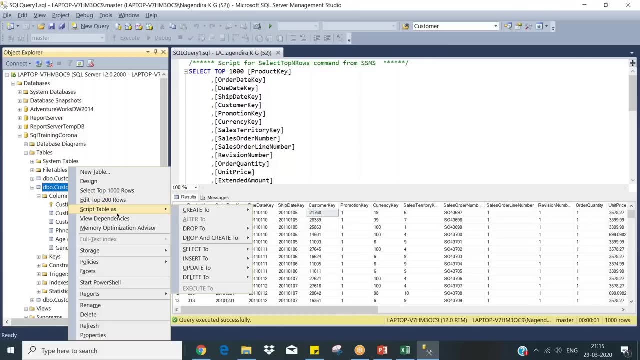 what we have created. so customer concern is our master table. the primary key will look as a golden color. okay, golden color key. this is your primary key. if you guys forgot about the syntax, I mean the structure definition of it, just have a look, right click, everything is right. 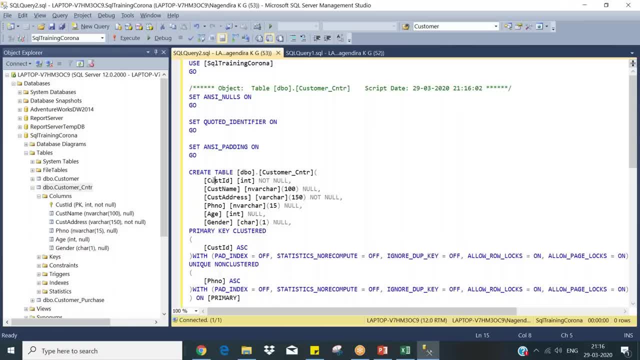 clear click and you see new. so this is the structure customer ID I created here. so it will create like this: if you the proper definition: primary key, cluster custard customer ID. okay, this is your primary key customer ID. now I have created foreign key. foreign key will look in a silver. okay, silver color. 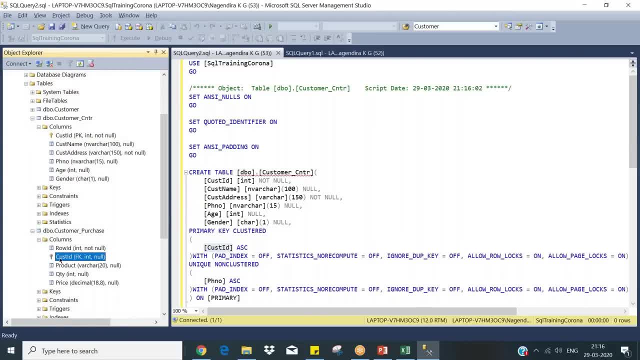 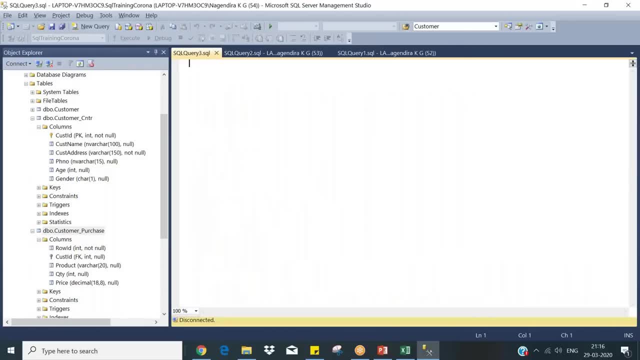 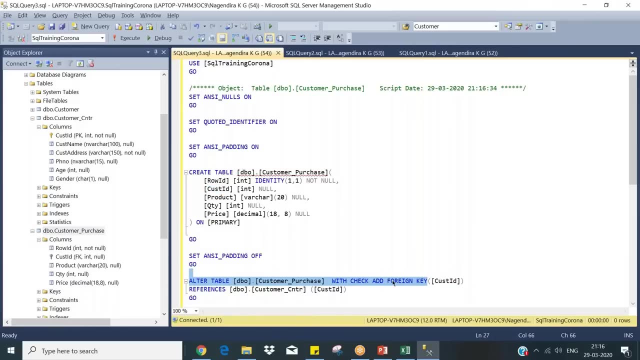 primary key: golden color. foreign key: silver color. this is your primary you you check at what is it. can you see IC? the remaining key for services is the key number being private key is the product ID. is the initial message. if I dont, I don't have this data right. you can call my service now. 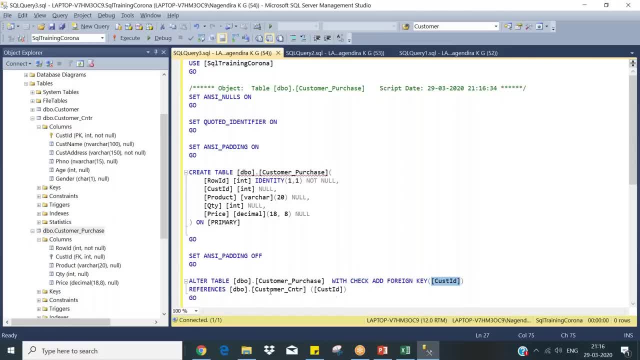 but turn off this list once. so if you have left home and you are not able to do so until it neues gonna and then you look at both versus similar sorts of differences between the materials and then that tells you what kind of product authentication is down on the customer table using listing. 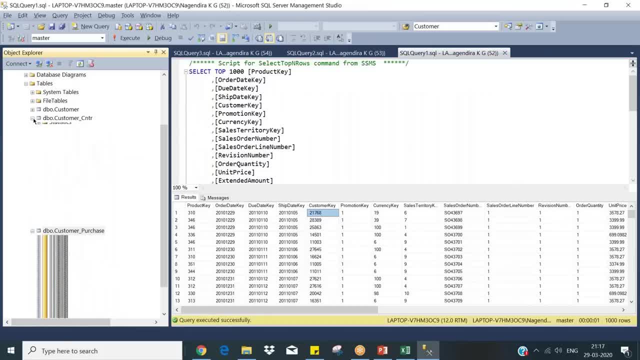 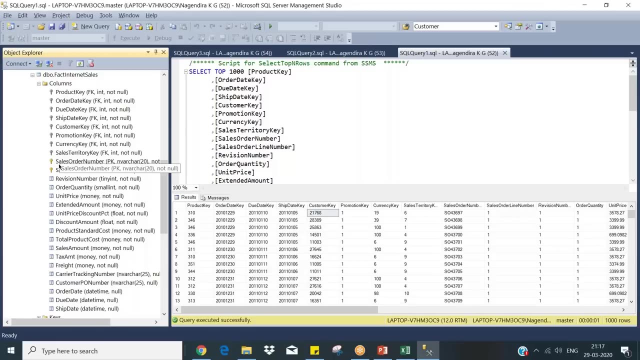 For example here to explain the joins, I want to take internet sales fact. internet sales This table has, this indicates the silver key, indicates a foreign key And these two combination will make you. we already discussed primary key can be a combination of columns. 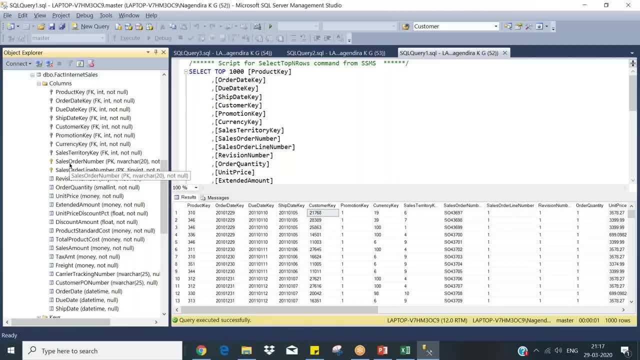 So these two indicates your primary PLT. see guys, you have uh. from the column name itself You can uh identify sales order number. Okay, People will have a lot of number of bill number and each bill We have a line number. If I go to supermarket, I be which? 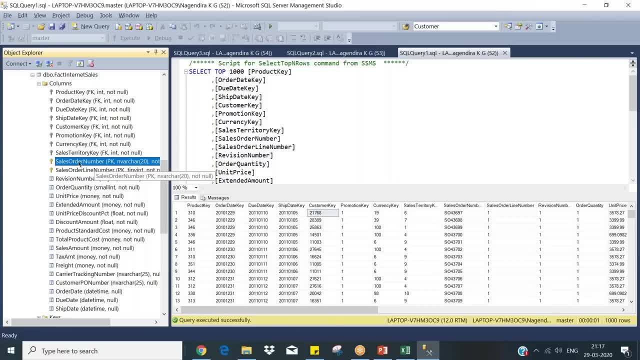 is at least 10 items. So uh say, for example, number one: 20, bill number 1 to 10 items. So bill number 120.. So Bill 12, Sleep number one, Number three: 20 food items. So who is wearing therices? 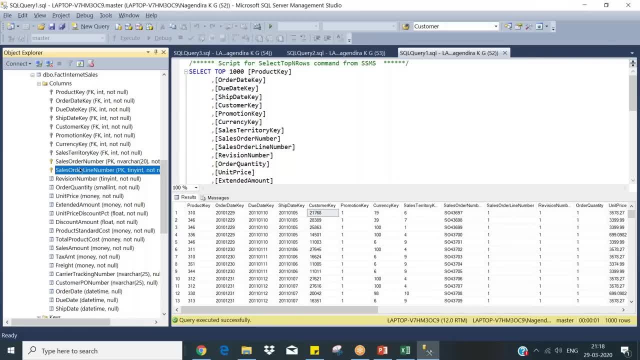 120 will be repeating here. so that's why i add line number also. line number will be all those 10 items will be unique. so you have both the things together to make it unique. that is why you have a primary key. so this is your fact: internet sales and you, as we defined earlier. 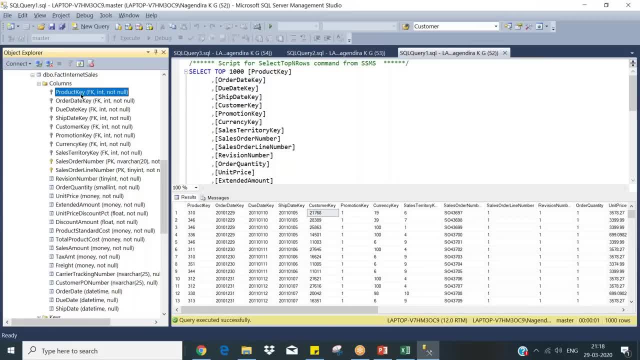 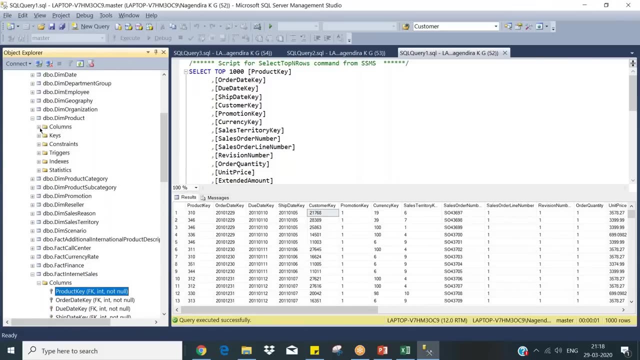 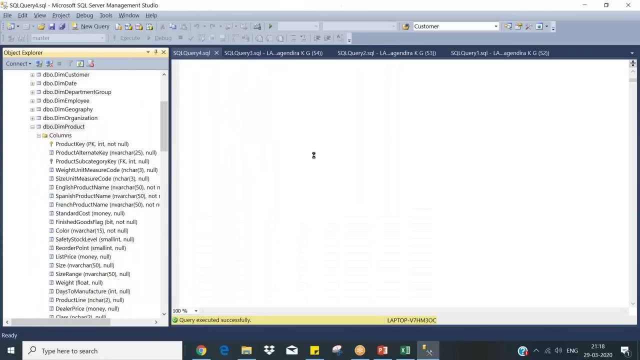 what is the purpose of foreign key? you have a product information stored in your master table- product master- so you no need to repeat those information again here. so just refer the product key into a sales transaction so all other information can be fetched from here. so product key is the primary key here. so these are the product information i have. 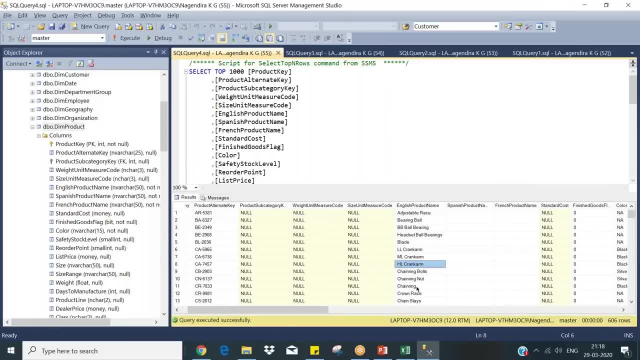 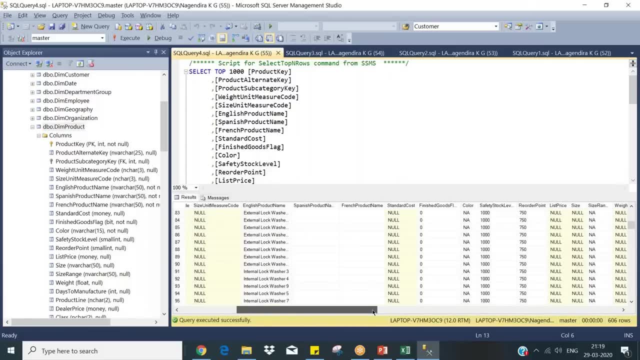 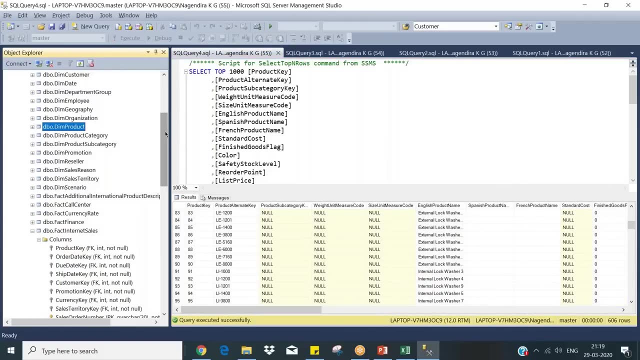 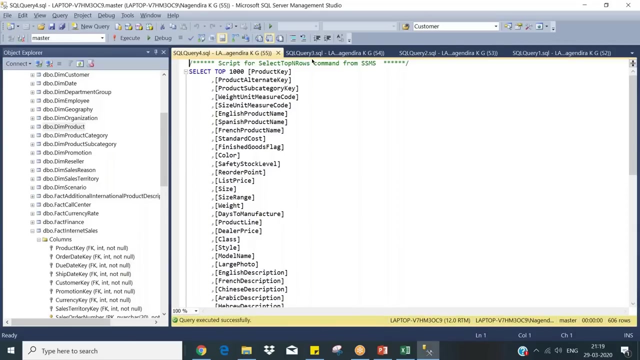 what is the product name? yeah, here, adjustable rays, channing ground rays, something like that. okay, everything will be here. okay, guys, now i have a product product sub category. where is that product under the sub category key? why it's not okay, fine, okay, now the question. uh, based on the different question, we'll try. 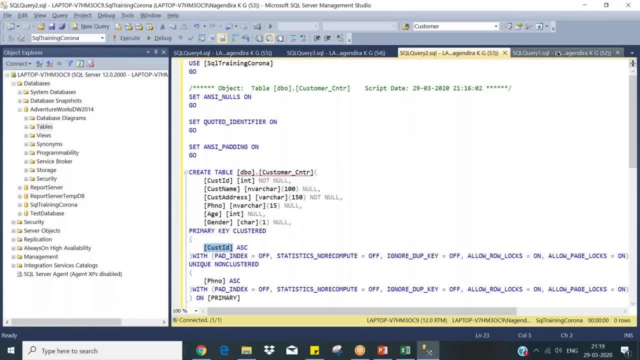 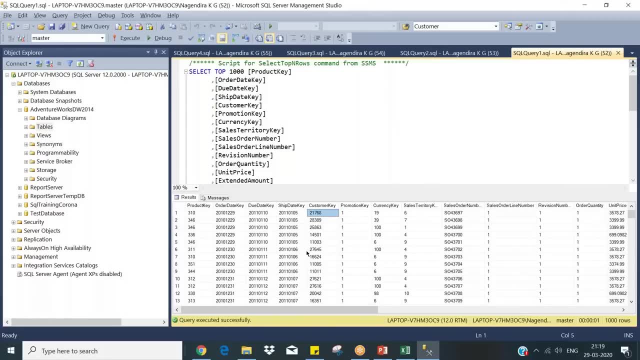 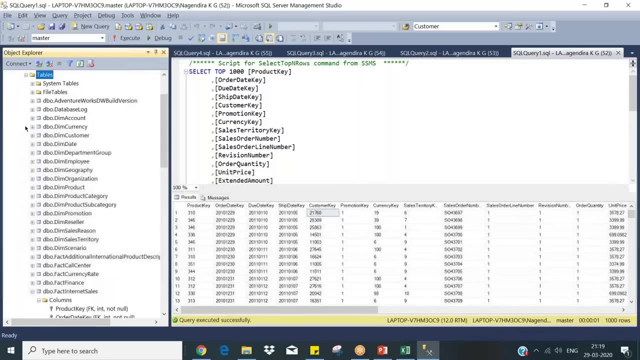 to answer using our skill joints. now. i just explained the table structure. now let's have some uh questions. that needs to be answered. okay, now i have this sales transaction. i have a customer, let's go for a customer. let's see some field here. okay, i need um. 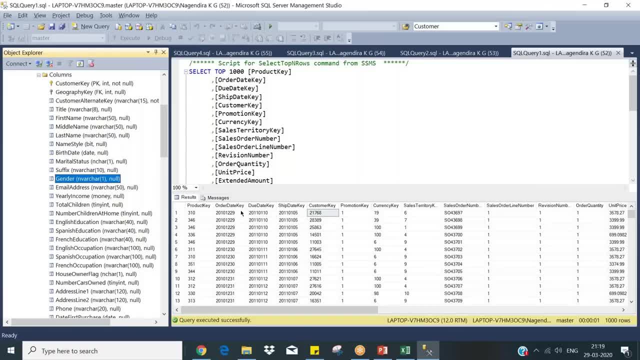 male customers who have purchased over 1970s- people section. i have like 2020- 16- 70 period. whatever period we have, the sales date is like 2010, so we will consider the 2010 date in 2010 december. i need those customer names. this is the. 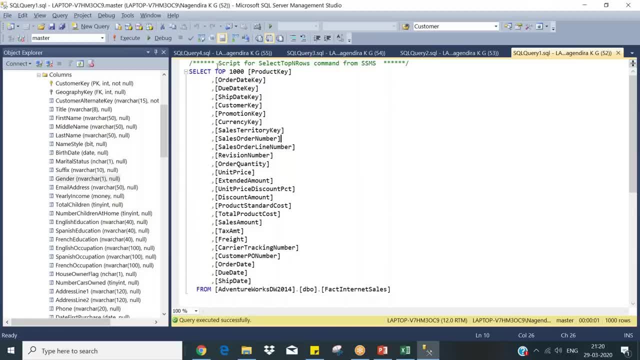 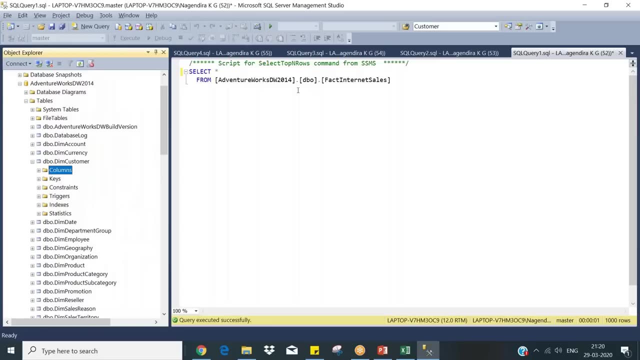 first question. what you need to do now. you need to identify what are the different labels you going to work on. i need customer name, correct. so either are you connected to the store or you we are now going to. I can use, but the question is says: like I need a customer name during over. 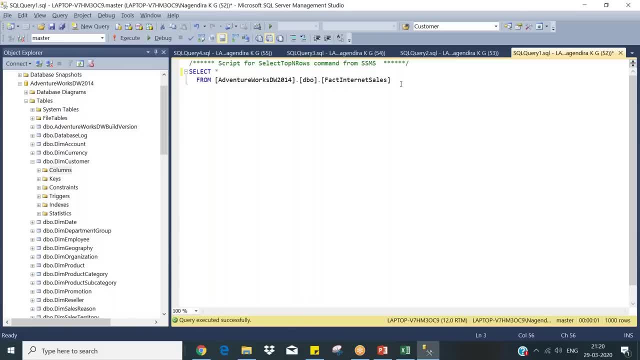 purchase December 2010. now in this you tell me, guys, what are the tables involved. one is fact: internet says another customer now in this, which one to use left join and which one to use right. I need these two tables now. I given up to any guess. 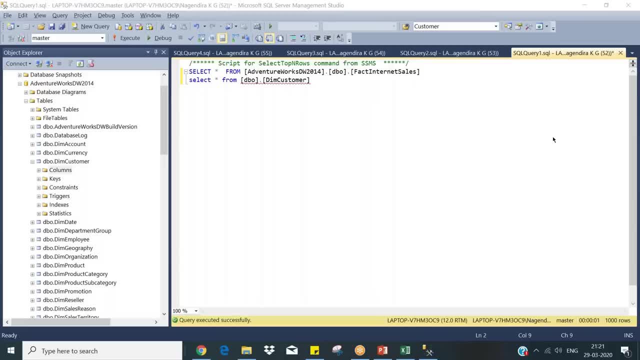 no, it's there, just guess. you have only two options: which one you will use left, which one to use right? I need list of customer name you need to use right, right? no, no, I'm asking, I need stuff. customers during December 2010. that's all simple as that. okay, you, I need to tell me which one I 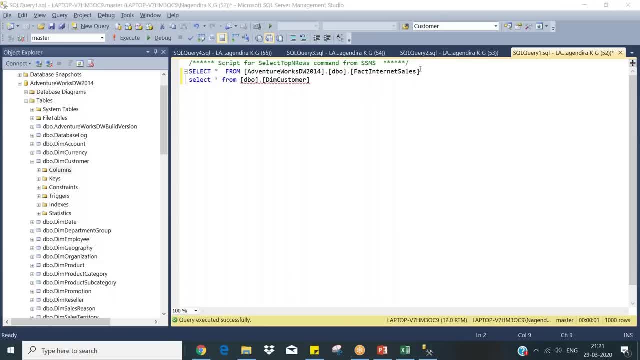 need to use. I need to use join because the condition says if they ask only the customer list of names, I need a list of customer names. then I will only this table. okay, but they asked me over purchase during December 2010. they ask only the customer name. I will get. 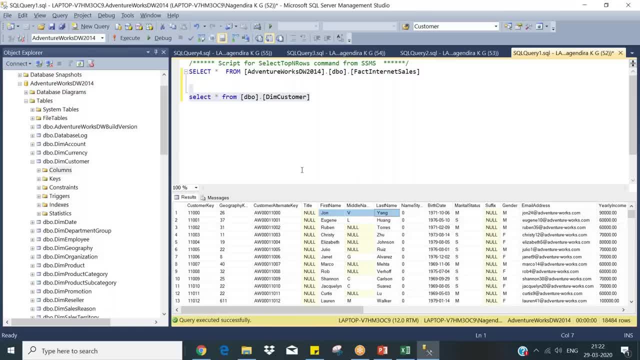 the distinct values of this name. that's fine, only one table is enough. but they asked me who over purchased during December 2010 that during December 2010 available, in fact, internet sales. so I am asking: I need to use a joint here. I need to join the inner, join left. 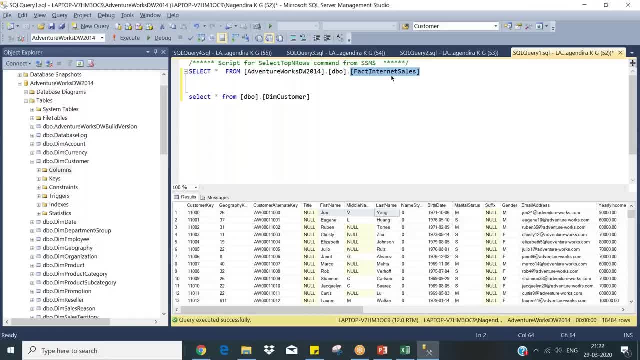 join and if it is a left join, which one I need to use first, whether I need to use dim customer table in that and in a joint like this, are you I need I need to use like this option, one, option to option one or option to option. 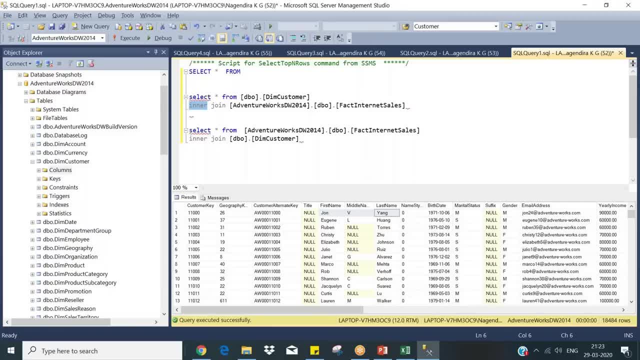 2 & 1 are same. if I use gonna join, so you, canане, is either of the cases. if we use in join, the problem comes only with the left job. you need to understand the difference. forget about now. I will go for option tool, as I highlighted, because he worked most on these problems, so so I need to. 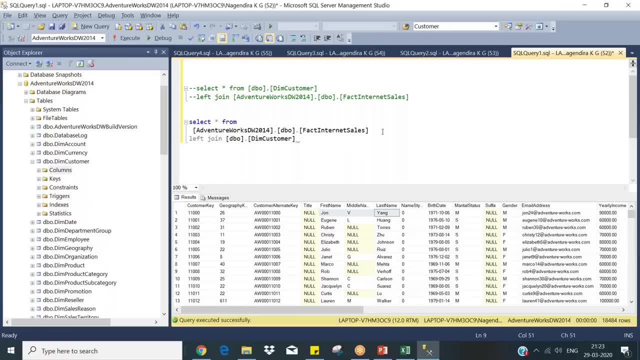 filter the dates. so first of all, fact, internet sales. I will keep it as intersection and this one as customer and I use, so this will include all the records from this table. so first our account of records here. this will be little confusing for you guys, will you like this? so the total count is 60,000. 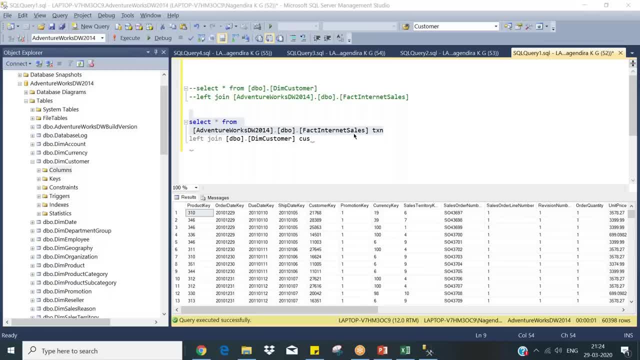 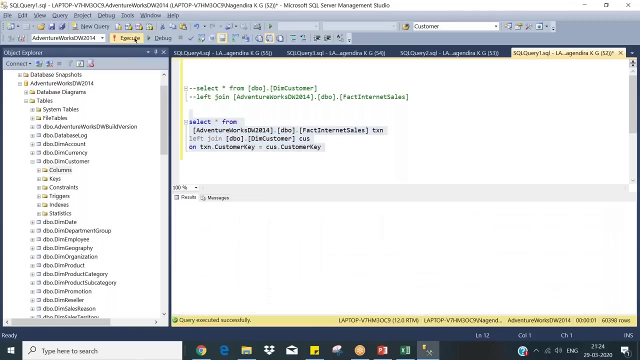 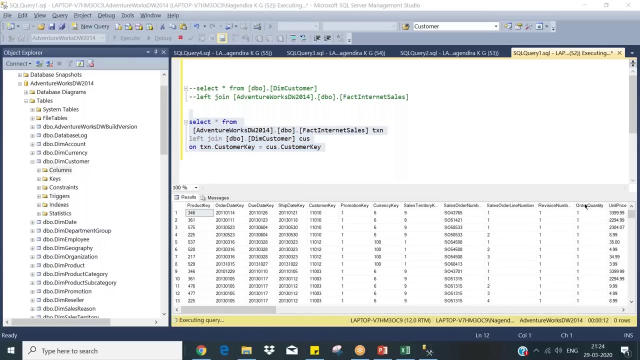 390. this includes all the records from the this one table. now they've joined on transaction. that customer key, equal to customers. that customer key again. when I select star, you look at the count: 60,000 398. let's take some time, okay again: 60,000 390. this is fine, so. 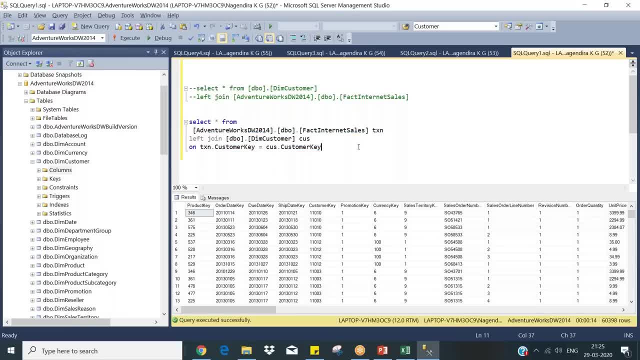 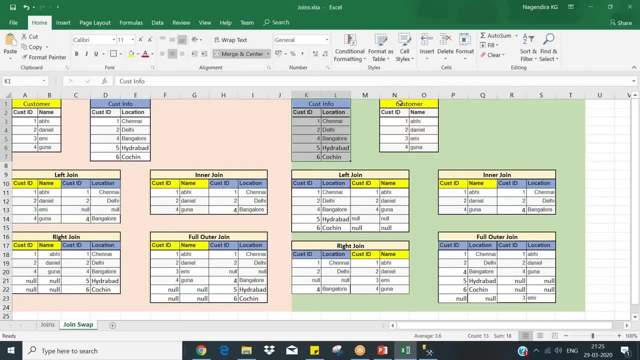 that is no duplication. now you have joined both the tables. what will be now? what is happening here? like you consider, this is your transaction table and this is your customer table. so you were trying to make sure that your current to do the left join now. so this is your output you have got. so is there any increase in the? 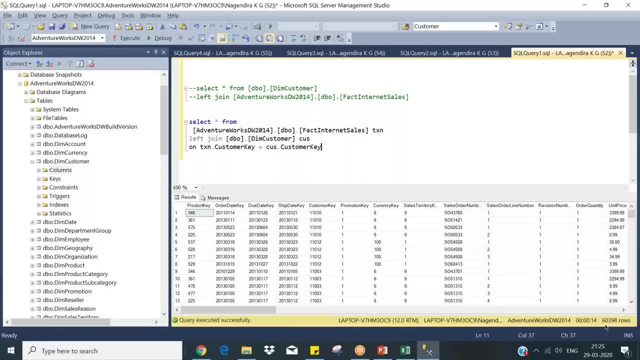 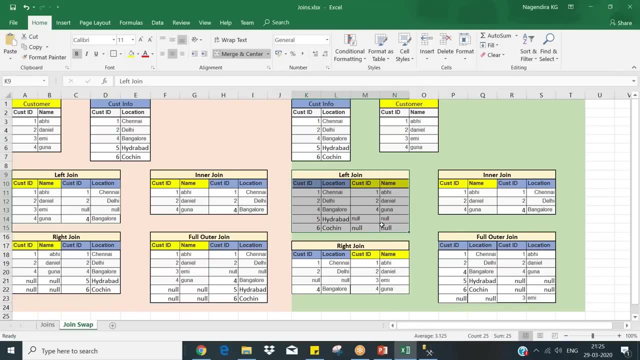 data. it is same because you have six records. you have got all the six records since you use left join. so i'm trying to plan with the small examples. if you work with the large data, it is same. now what happened? you combine these two table data like this: so once you make a join, 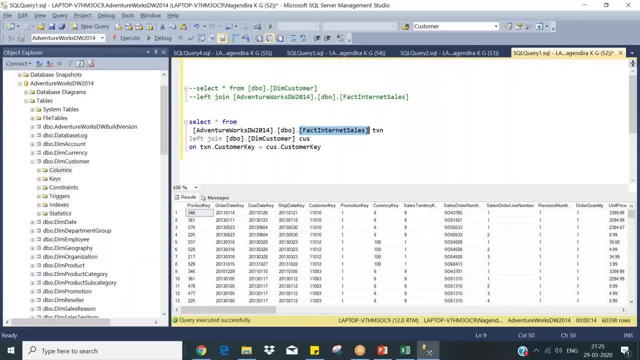 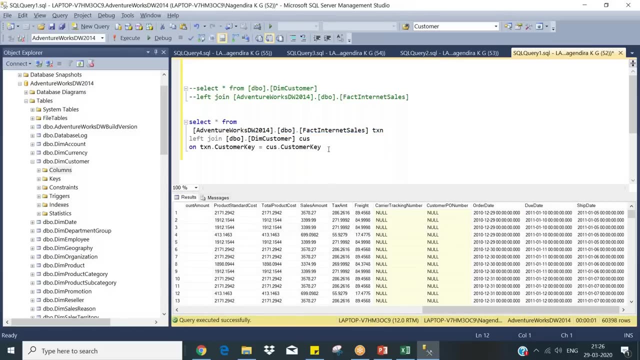 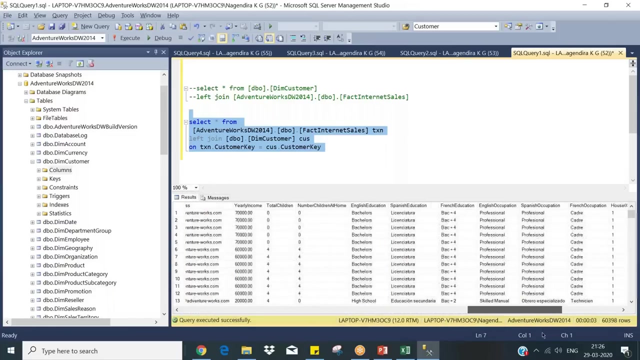 this star indicates all the columns from your internet sales, all the columns from dim customer has combined here. so if you see here what is the last column, only i'm selecting the fact: internet sales. ship date is your last column. if i select along with this, you see after ship date, where is that guy? 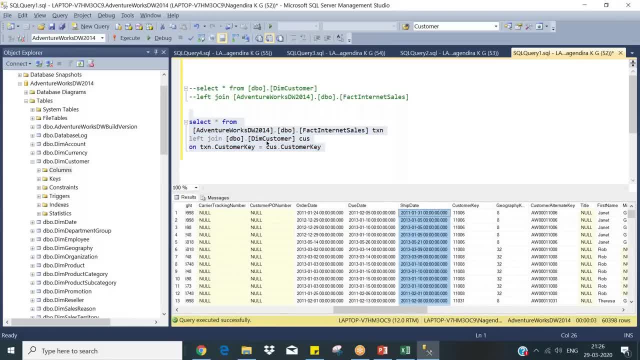 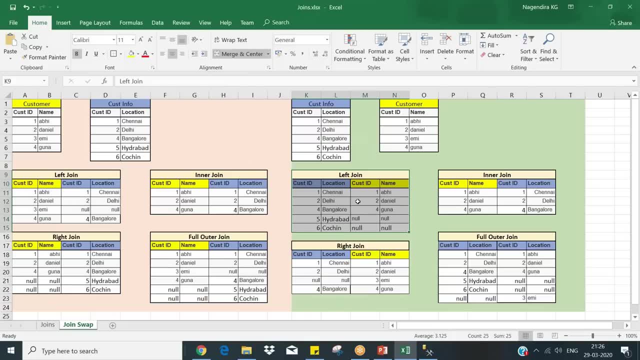 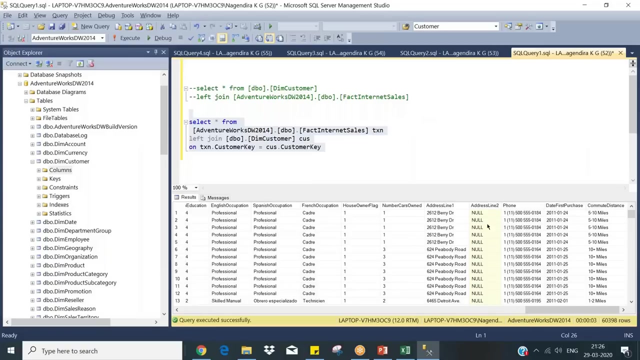 yeah, after ship date the customer key started. customer key is from dim customer table. okay, so this is your output. now, whichever has a map that will have a mapping record. if some customer information is missing in the master, you will have null records. here it is. this is not the null you need to. you should not look at null means. 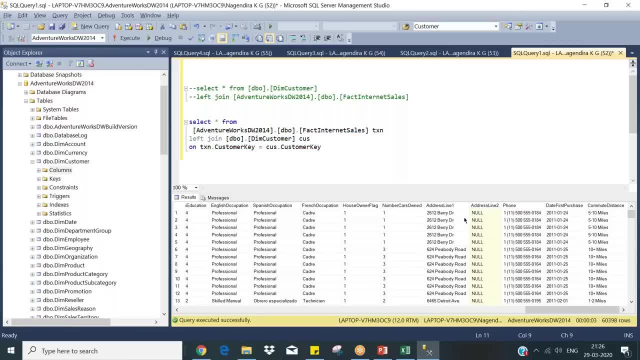 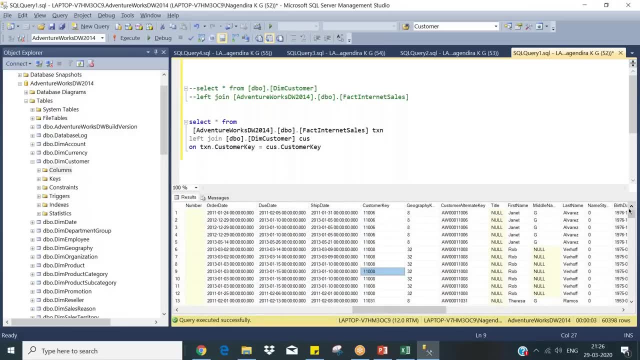 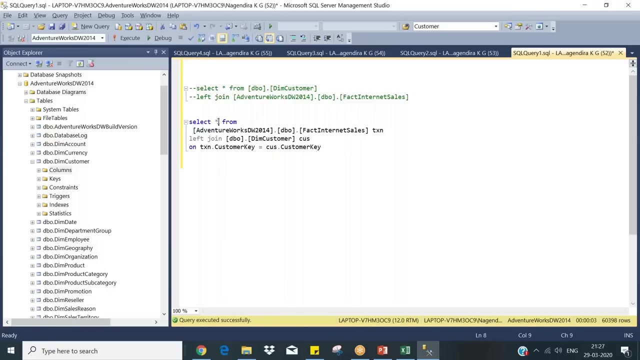 this null always. whatever you are joining with this column, customer key should not be null, okay, okay, there is no null columns because all the customers exist here. forget about that. okay, guys, now back to our question. now i need only the name, where the name exists: customer dot. let's make it simple as like first name alone. then. 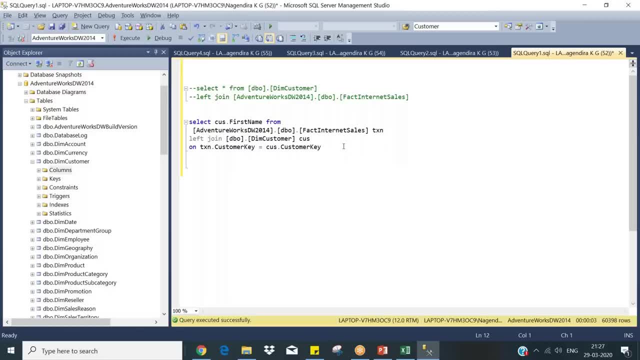 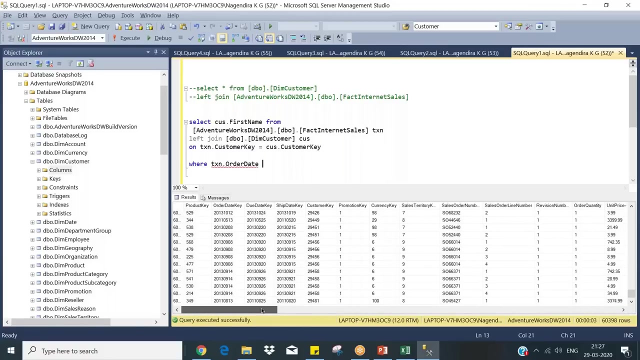 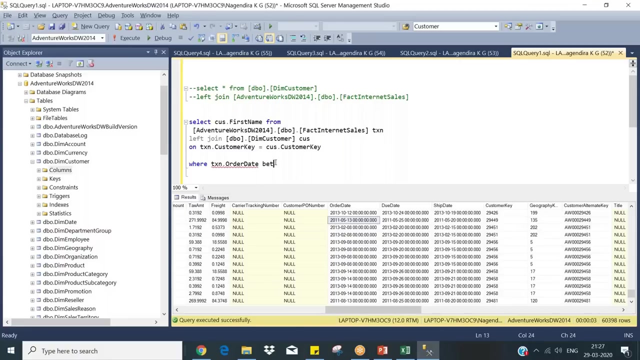 this is your requirement, then i didn't filter it, so i need to filter where transaction dot, sales date or order date or date. uh, i will use some other function as well. okay, here, order date. okay, order date equal to, or. i can use between two thousand two zero one. 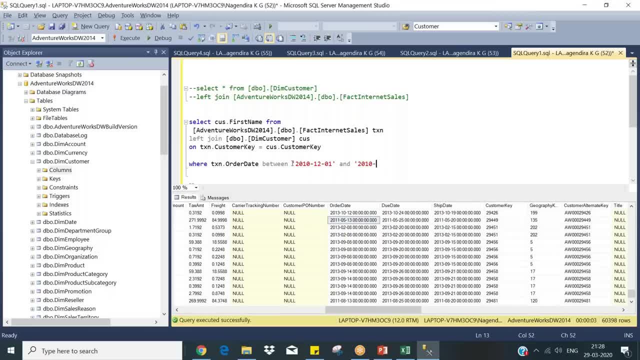 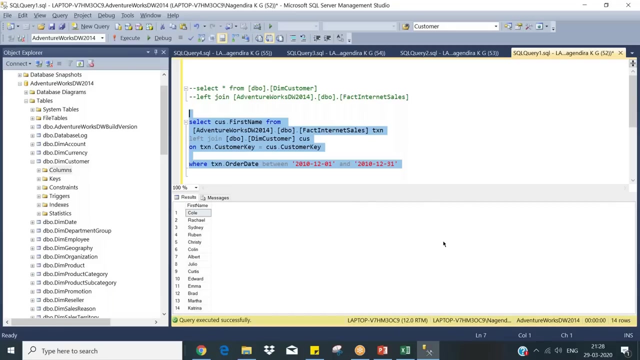 and 2010 to 31. okay, this answered. so any list of customers was brought the items during december 2010. so only 14 customers okay, has brought the items during this month. this is same, like the corona who. whoever came from immigration, they will find a query like this only so after some period. whoever, 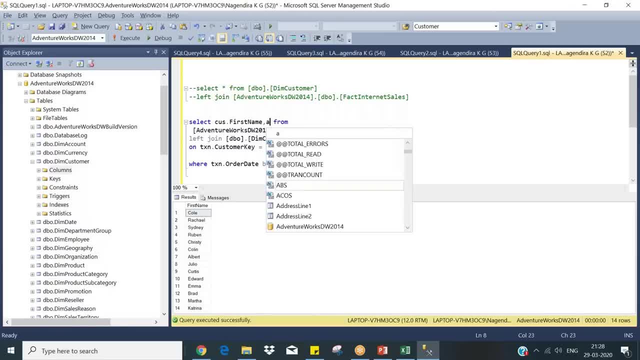 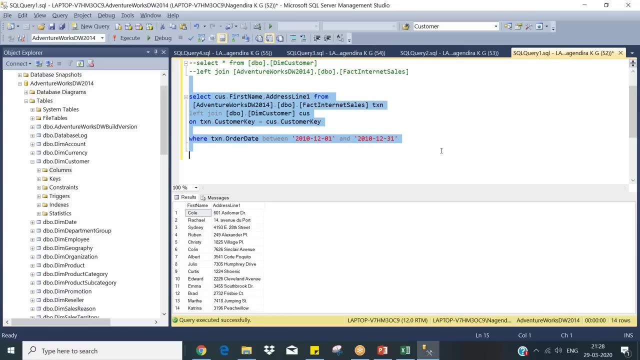 came and along with their address i want. so just put address address line one so they will come and choose a question admitted, Posted after having. that's all okay. this is how you will inquire programmers based on different periods, whatever period you want. you will have to answer government in the while condition. so basically, we started the selection. 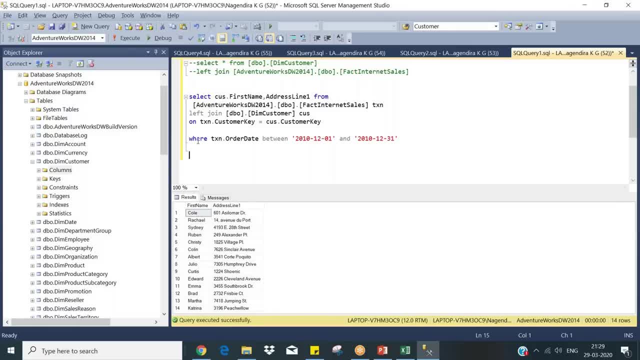 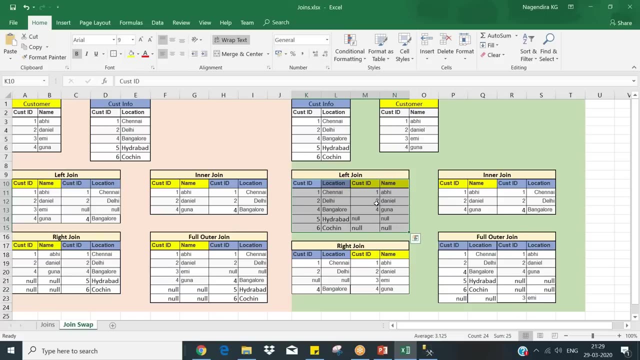 the last year with where condition in a single table don't confuse with the condition with joints. when you add volumes to us, once you have a joint do output is nothing but another common, another new table, new table. so from this you are going to query, that's all okay. 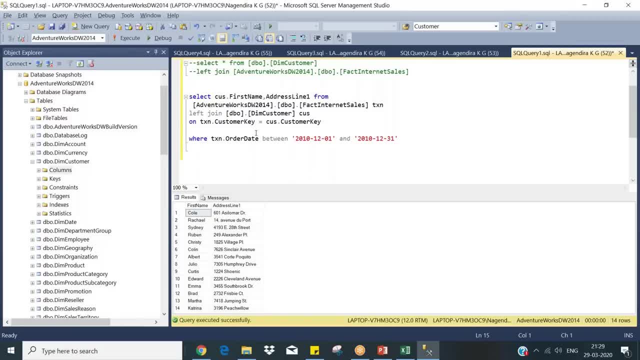 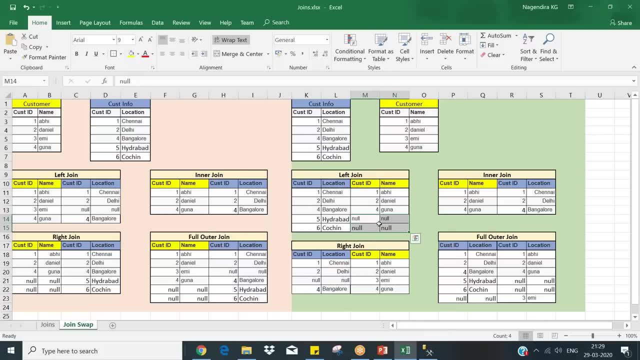 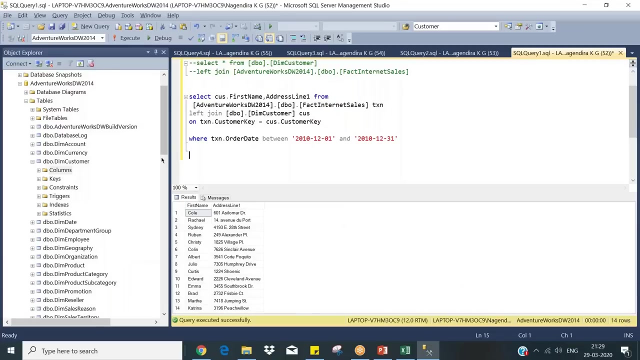 i hope i'm clear, guys. now let us see um this example. okay, like i want to filter out when i do a live join, i want to filter out whoever whose customer information is missing in this thing. okay, you can do it in multiple ways. i can do it in a live join, but try to do that. 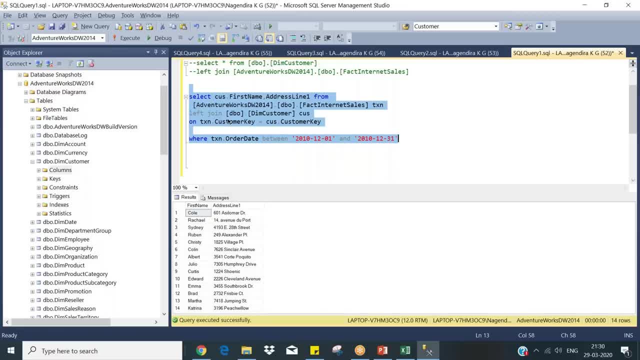 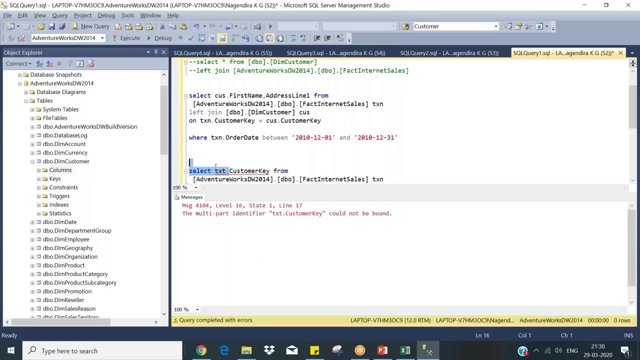 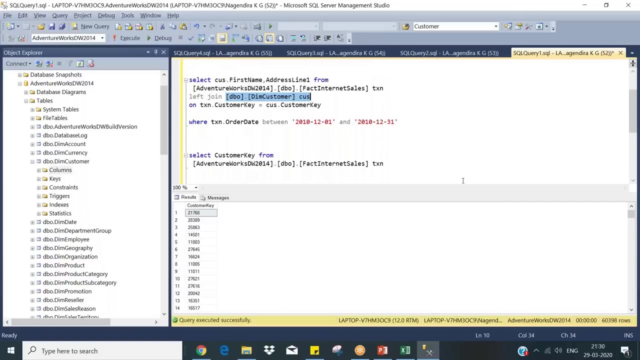 let us take a simple case. customer key whatever: six, zero, three, nine, eight, all the customers. oh, this is the transaction count. what I'm trying to check is whether all customers exist here or not. that's what I want to check. I want to delete one particular customer key from this record. let us take this. 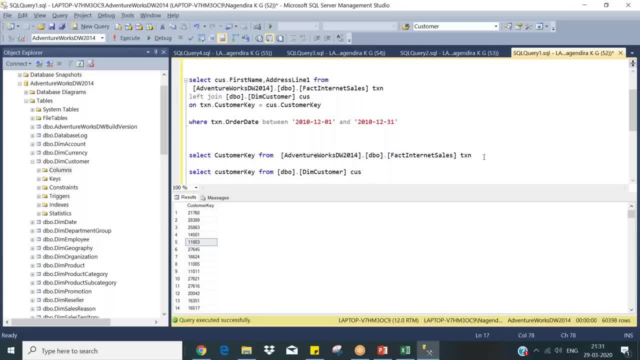 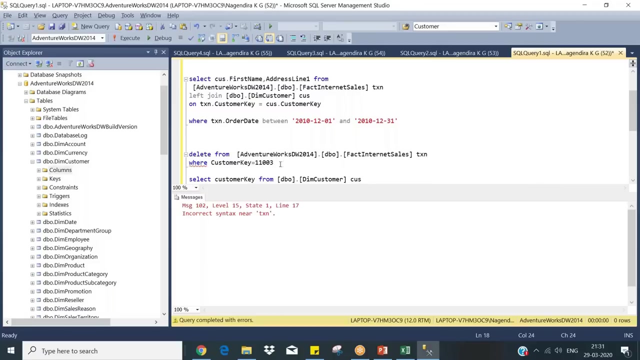 guy delete from this table the customer key equal to this. what happened? incorrect syntax, near I think it is not to play. see, it says that I'm rooted with the reference constrain I. there is some other direction. reference constraint fact: internal sales. I'm sure. maybe give me a minute. I'm trying to give you a scenario where you can understand very 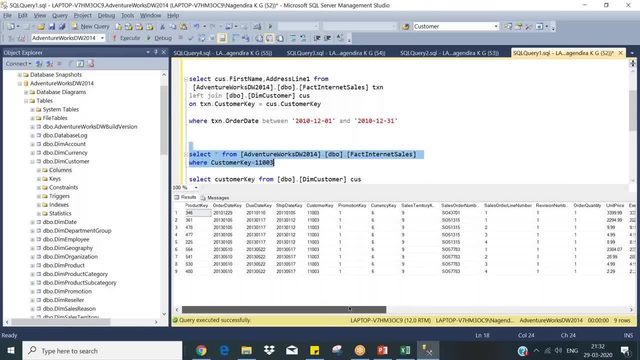 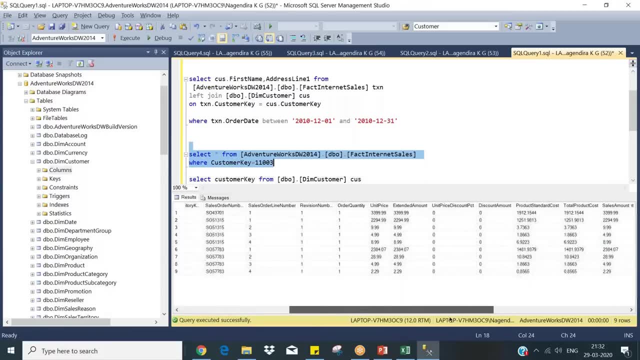 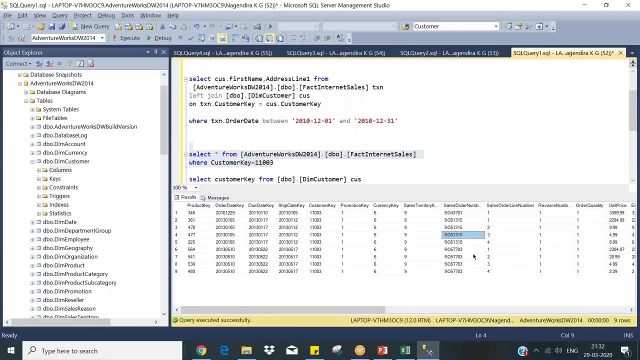 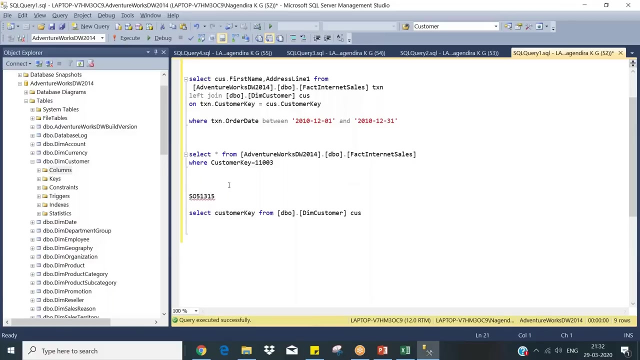 better. let us delete this by delete customer key. what reference constraints those? not sure. okay, let me delete this. if I'm not able to delete, I don't want to fix this one right now. let us focus on something from this table. I'm going to leave my 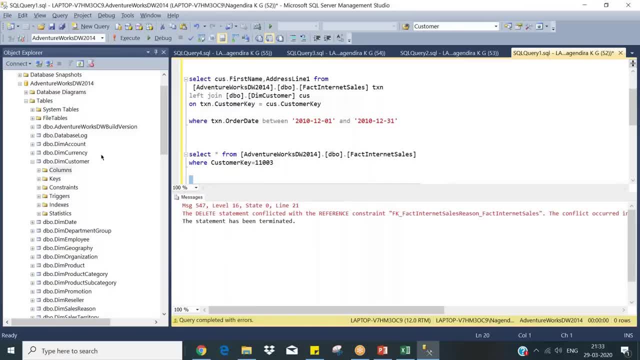 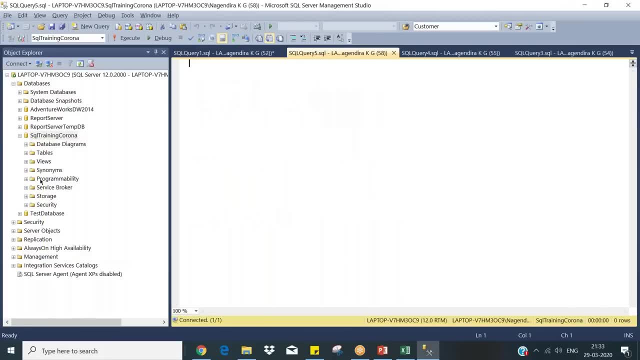 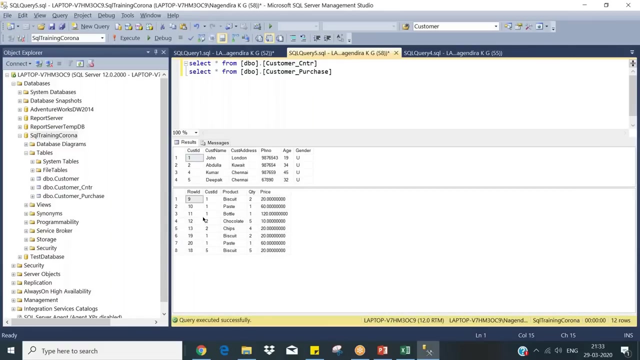 field default and I'm going to delete this by delete. there is a 2015, so I want you to understand the joints as much as possible then. only it's clearly record. okay, now you see here guys. so one, two, one, five and we have four is missing here. so when I do a inner, 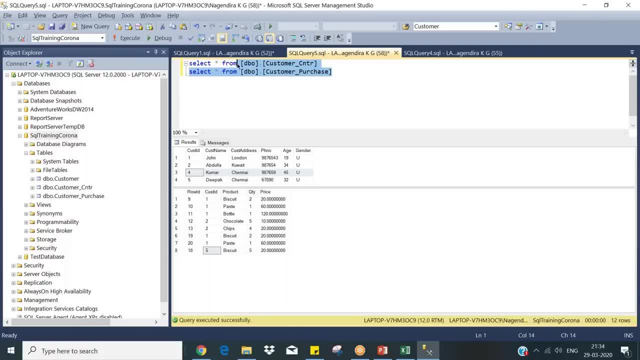 join select star from you know. join customer purchase. I'll you key. I will keep the alliance name as a for time being. I will put a and b: a dot cluster id equal to b dot cluster id. so what I want actually, I want only a dot cluster id. 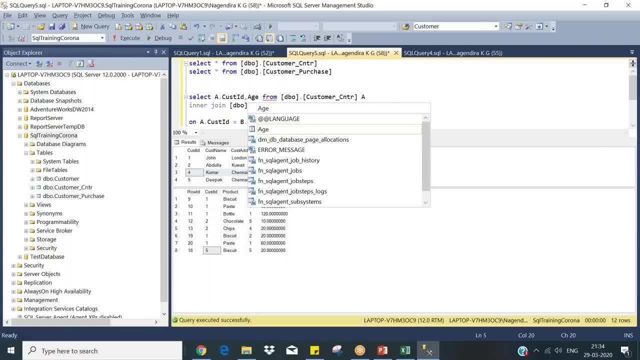 and I want h. yes, one more time. yeah, alias is nothing but your alternate name. you can get alias name in your particular column. see when I the you need to instructor this joint, this column. I mean from this table, this particular column, customer ID. when I used I need to explicitly specify like this, the big table name. so once you 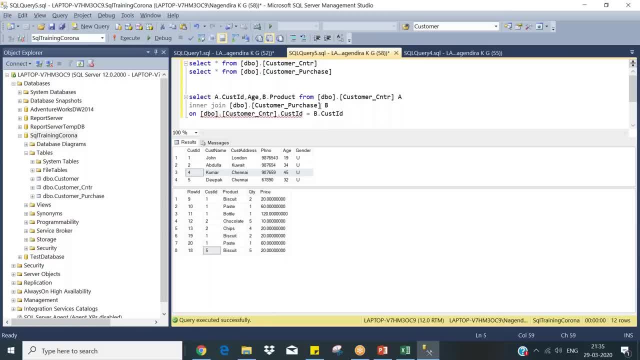 give the alias name. once you start giving the alias name, then you can refer using that alias name instead of giving this table name. just I'll put a dot for prayer in. we are calling chintu, right, so same thing applies uh. going forward, we will refer chintu uh instead of. 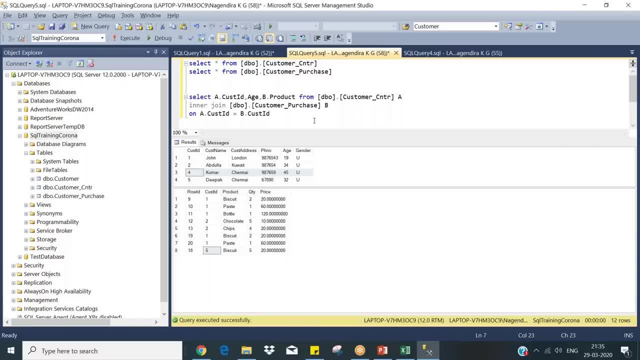 calling him pravin. same thing: alias name, short name like that. i mean not a short name, it is like uh. alias name like nickname, like nickname, exactly so nickname, uh. in technically it is like alias. okay, so you are keeping a and for this b, going forward, i can refer using a wherever i say a. 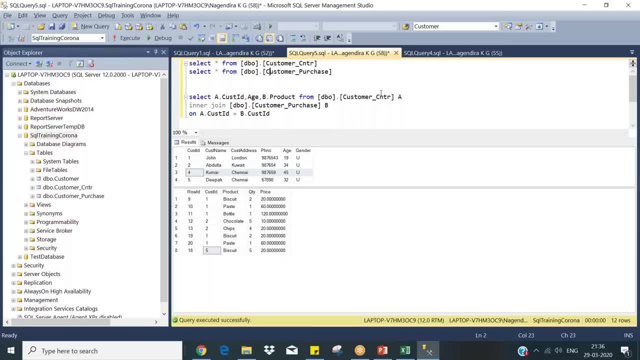 in this query only, okay, not, uh, other queries, only in this query. the scope is within this query, so it had customer id b, that customer id. so b indicates this table, a indicates this tip. okay. now, what i'm trying to say is: so it will skip the fifth record. i mean, uh, that four. 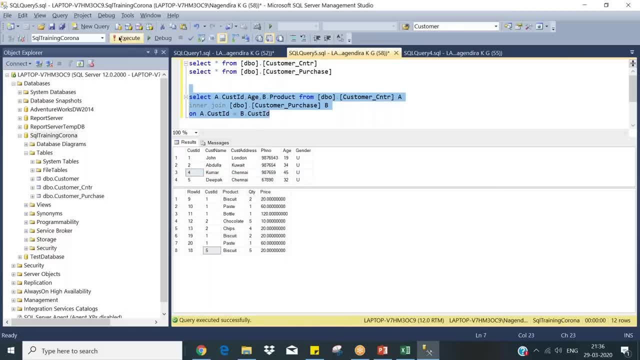 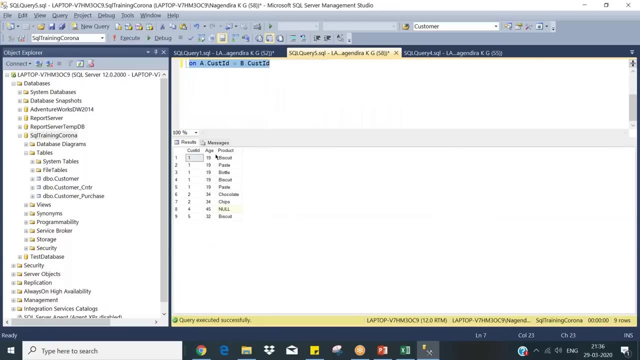 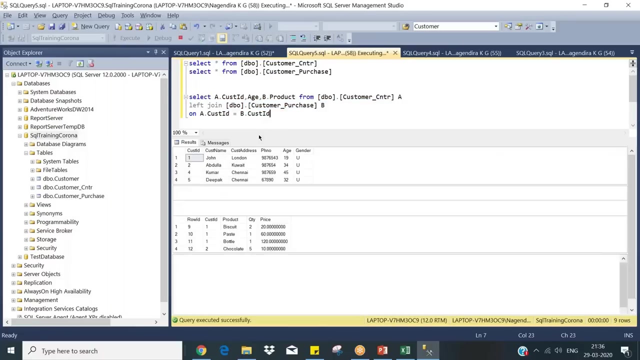 whom are, since the customer id does not exist. you now, what i want you to see here is, when i do the left join, what happens sometimes? there is some cases, so this is the i will. if you see the output like this, you can't get it. so always run along with your base tables and the result i mean. 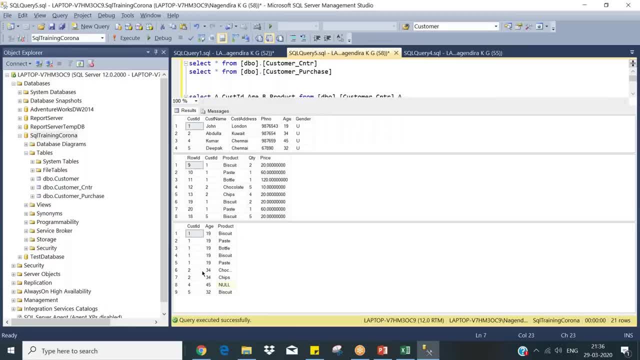 the query. so this is your base table a and b and you are using a left join, so it includes all the records here left. all the records, in the sense all the members. then, if you it can, the right side table. it contains multiple records. it is repeated, okay, so if i have a row id, then you. 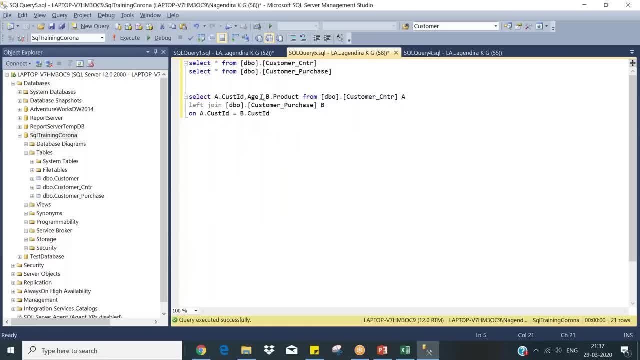 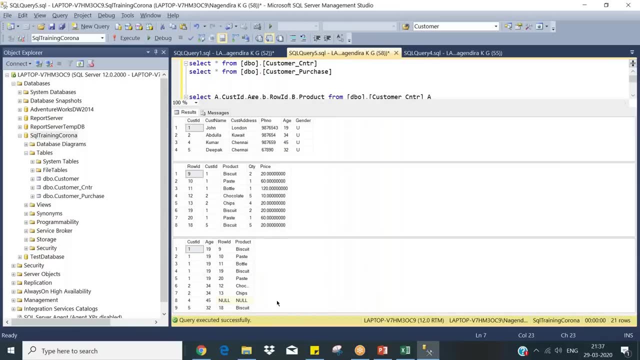 will understand b dot row id. so b dot row id is nothing. but you have distinct records here: uh, 1911, 1920, 1911, 1920 for customer id. now there is some cases like we have a customer and people will ask: whoever doesn't purchase at all? we have customers or we have one product. 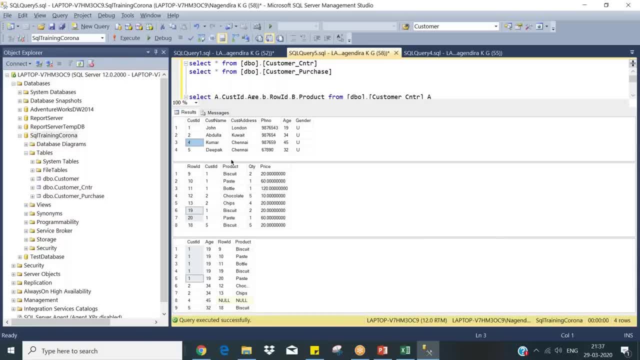 that doesn't sold in our list, okay, something like that. you consider this as a product and this is your transaction. then there will be some cases like you. there people will ask: whichever has not sold at all, then this is the case. so this particular product, okay, our customer who has not. 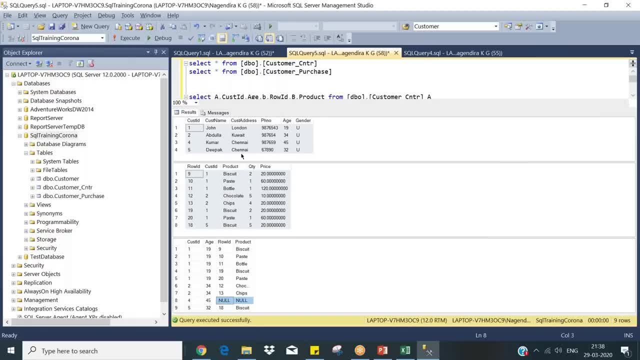 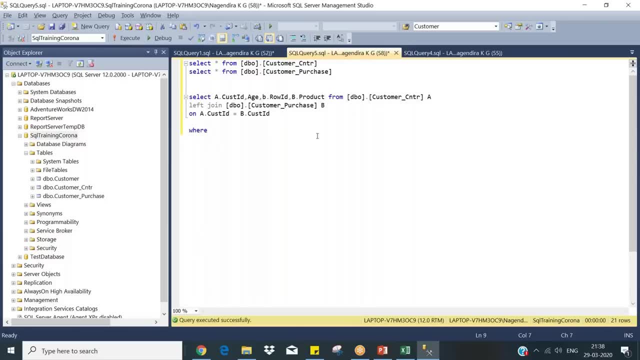 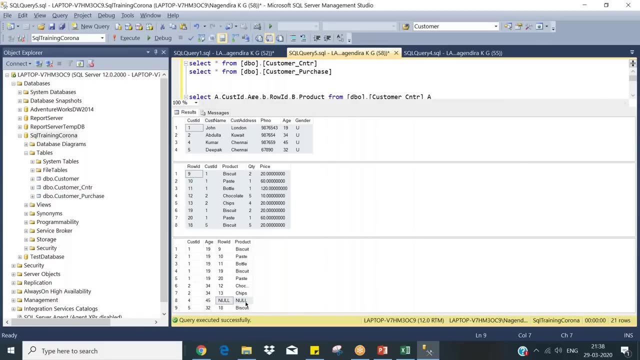 purchased at all, but he is a our customer, then how to filter it. so you got the result here. then what you need to do: just put where where this column exists- row id, right row id or product anything, any column you need to specify. so these two columns are from b table. 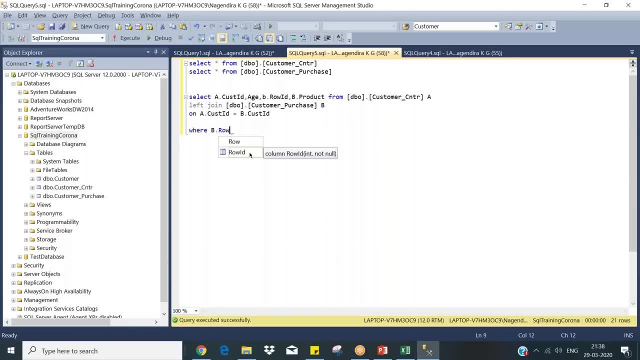 so you put b dot row. id is null because var condition we have seen about equal to greater than less than or less than equal to, between, like in all those things. okay, so for, in order to filter and null value, you cannot specify equal to null. this will not work, because if you Nutter this way, in Russia. if you say we are going to see a Mode between действительно, no value is like the value b dot, Women and so on and so on, feel so we're seeing, uh, the less than less than equal to between between, like in all those things. okay, so for an, whatever the Then is where you define. Lake gets equal. does it rode that meaning? or better, you present the only kind or not? Soeste Re Она. we can't specify equal often. 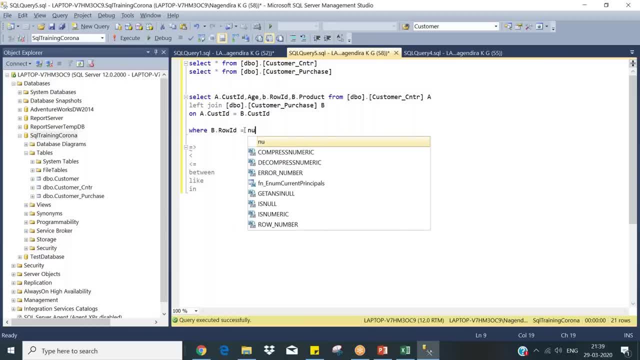 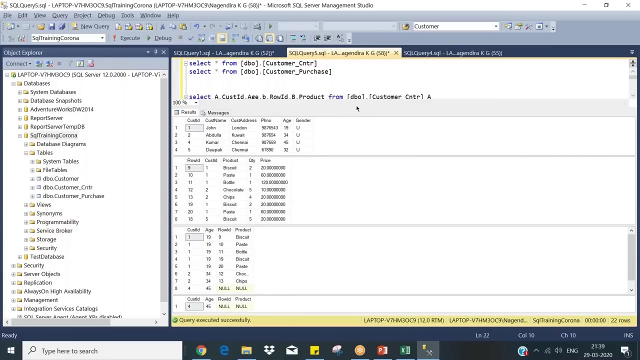 out. this is not. this will return false. only so for null values to filter is null. okay, now you see, I will have that condition. I will have all the outputs together. so when you select, you can comment it out. now you see the output case. so this is your first table. second table: when I do the left, join it. 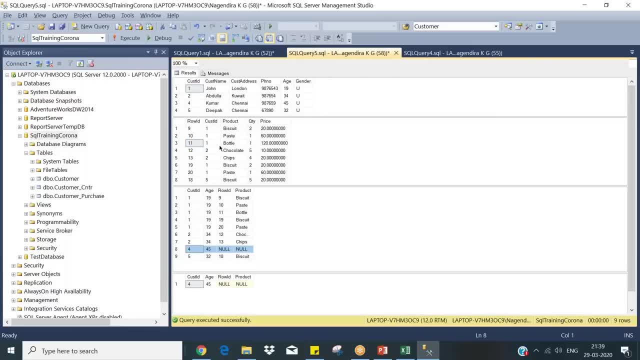 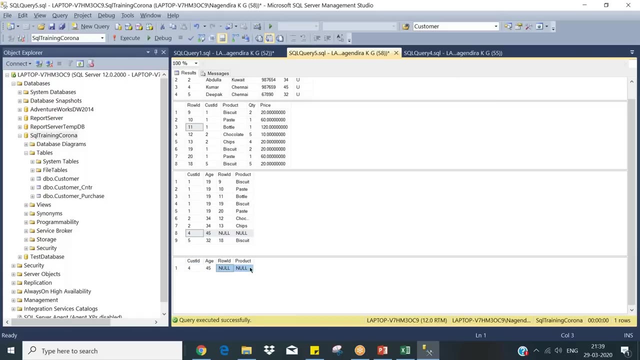 includes all the products from the left table and whatever appeared then. the next query I approved. this is like whichever customer who doesn't purchase at all, so we can get the results like this. okay, so this is how they will try to analyze and business will ask lot. 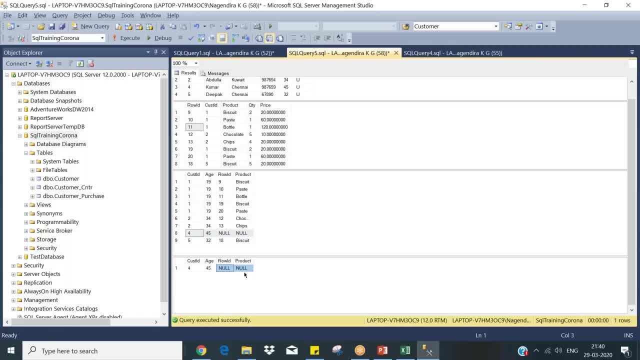 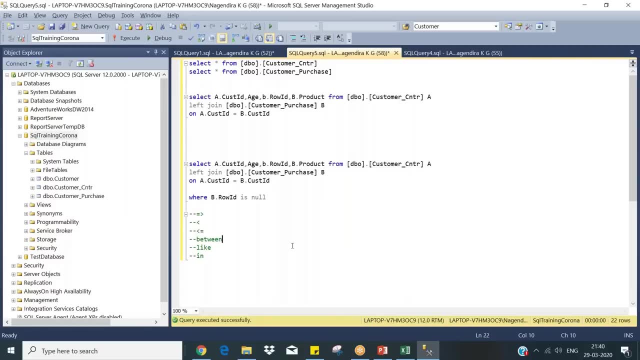 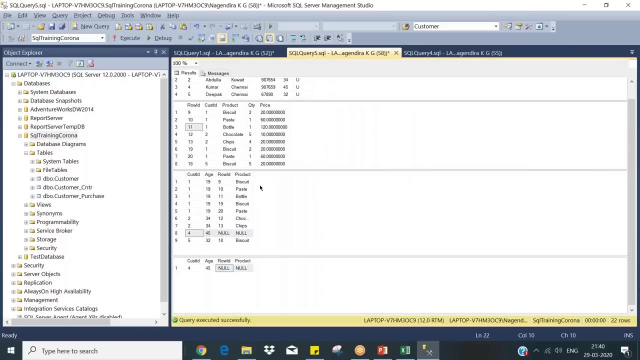 of questions. most of them are questions. so these kind of stuffs you keep it ready, these queries, you will run that one, you will get that queries answered. okay, this is the main important thing. so you just know you. you just not use the joints only for joining. as I said, joints is. 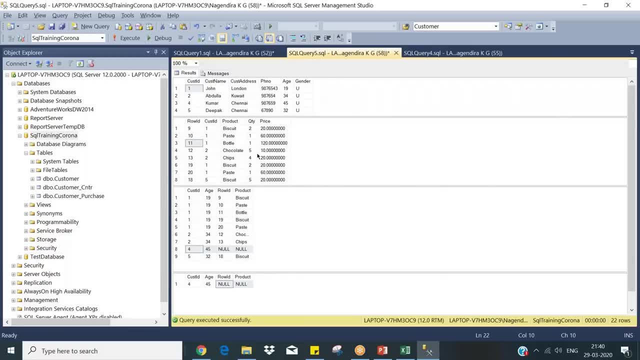 used for looking information in another table. that is absolutely correct. but in this case you are looking information for another table that is not exist- the doesn't purchase- then you need to look up. then only you know that he doesn't purchase. so obviously you are looking up information, then only you know that is. 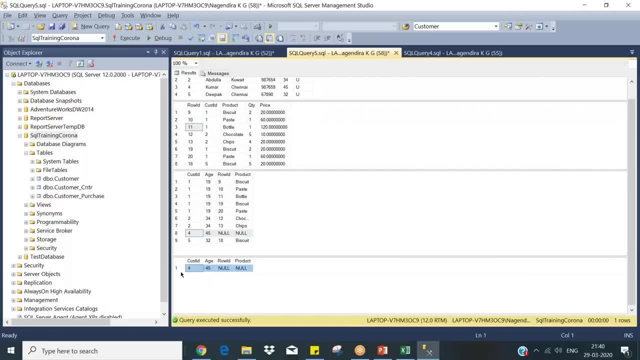 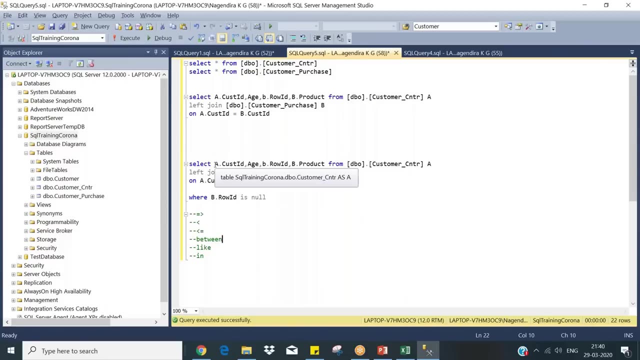 not purchased. so you got this answer okay. yes, this is what very important when you use joints, when to use values. so there is no thumb rule like which one to use, which table to use as left or right. it depends upon the scenario. let me show you guys. so now you have count of records for records now, and this one: 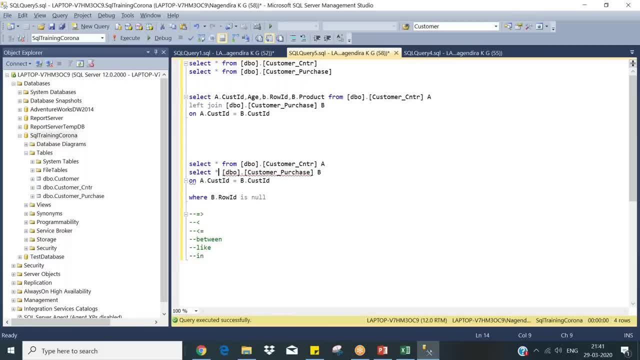 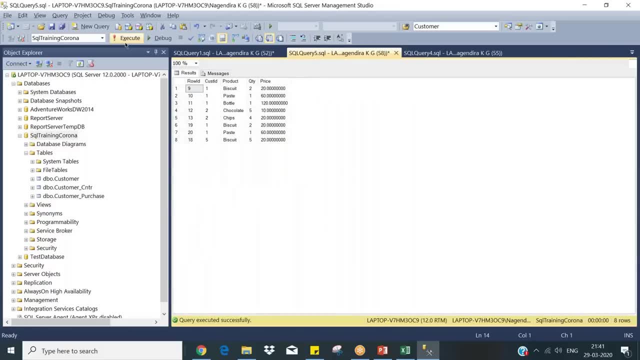 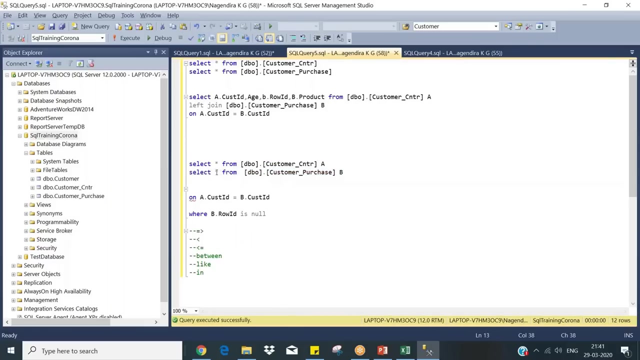 how something around eight or ten records, eight records. okay. so when you run together four and eight, so when you use this one with this you are increasing the records. okay, when you use in a joint, I mean this one will totally you will get maximum of eight records. how come? 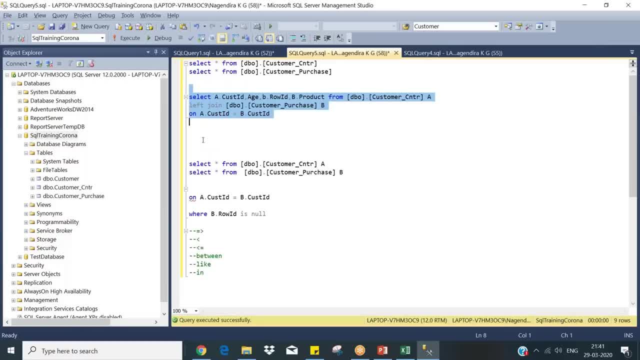 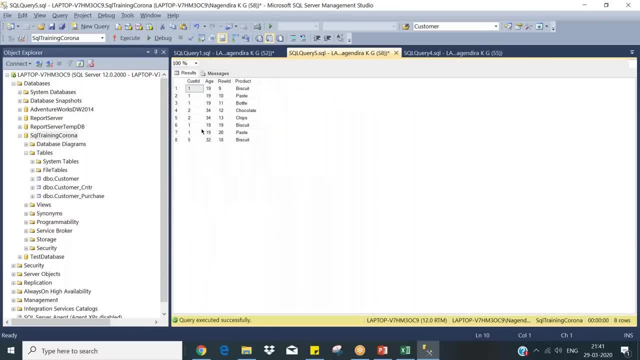 it's nine. okay, this one has left joint, it included, all okay. so in a joint always will have only the matching records. okay, left joint will give you different results. so there is no count. you cannot make based on the data value only. you are saying the it. now it increased to nine records. how? 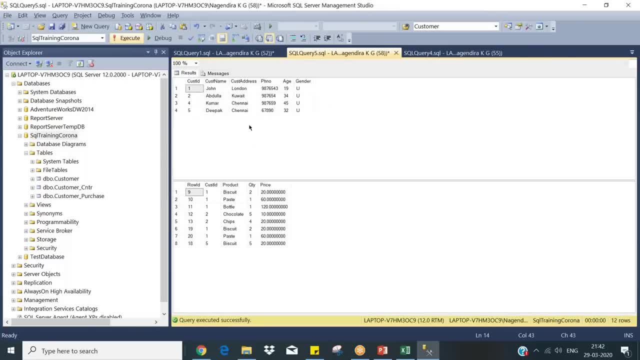 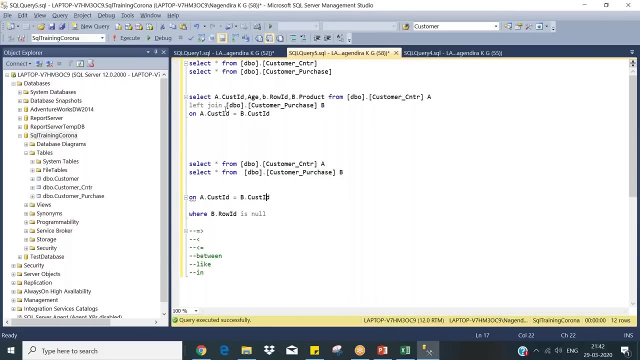 many records you have in a table. that doesn't decide you how many records you will get. there is no duplication, nothing. you can say: this contains eight, so final is it should be eight, not like that. okay, okay, no, no. the point i want to make here is, you see, 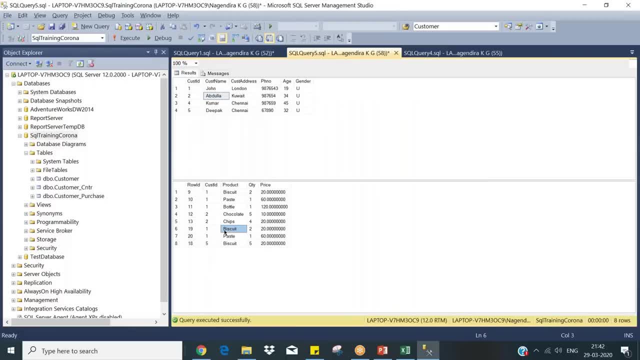 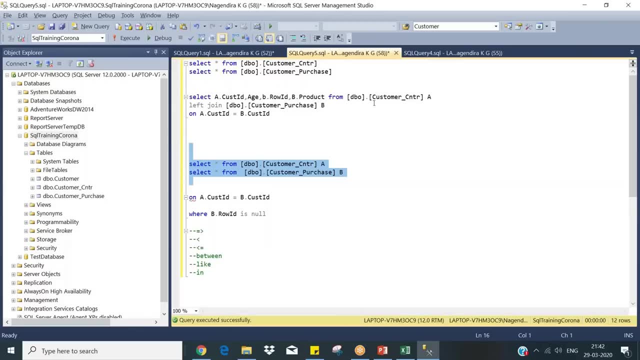 like here four records, here eight records. but when you use this one as your base table, okay, you will get always eight records. so here i will swap this guy, the customer purchase, or here why, as i swapped, it becomes a table and this guy will become b table. 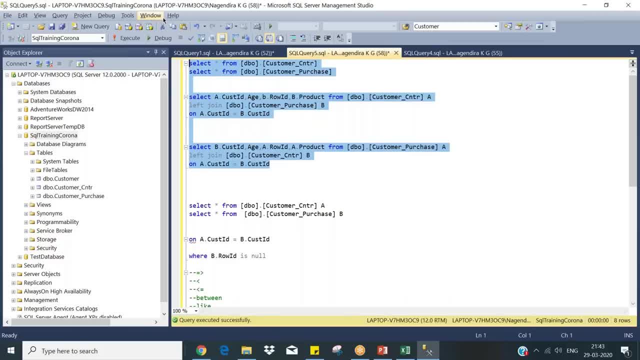 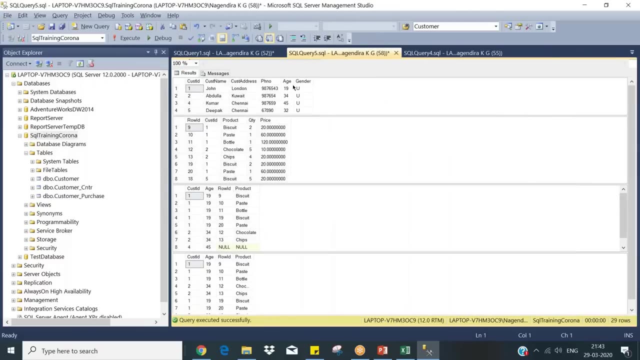 okay, now you see the difference between these two. when i, when you use a customer control as a base table, customer purchase second table and customer purchase base table and customer control in the second table, i mean left. now see the results. this contains four. this contain eight. so your customer control when? 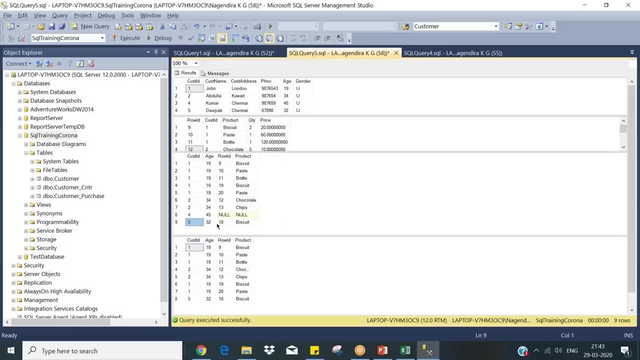 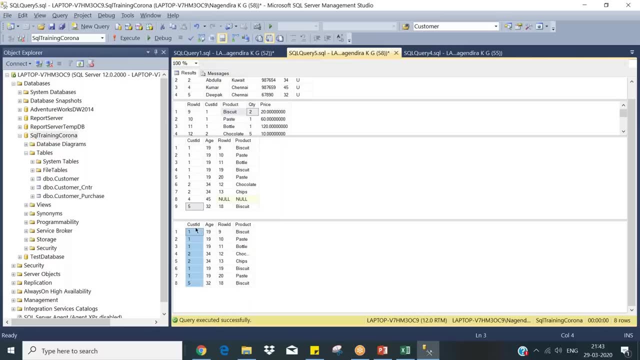 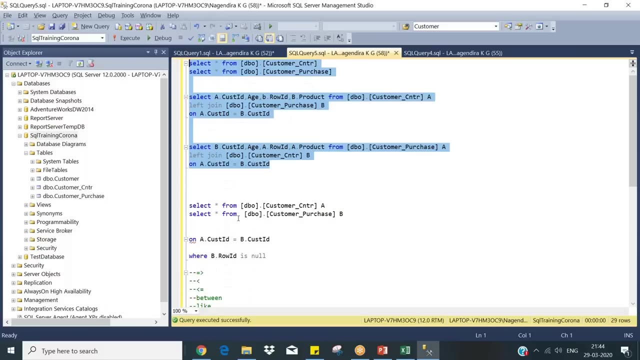 you use as a base table, it gives me nine records. but when you use customer purchase as your base table, it gives me eight records because it uses a left join. it all includes all the records. records in the sense all the values. it should include all the values. that values is based on this particular joining column. so eight records. 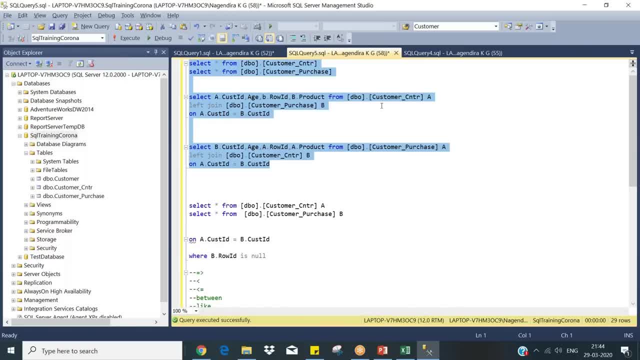 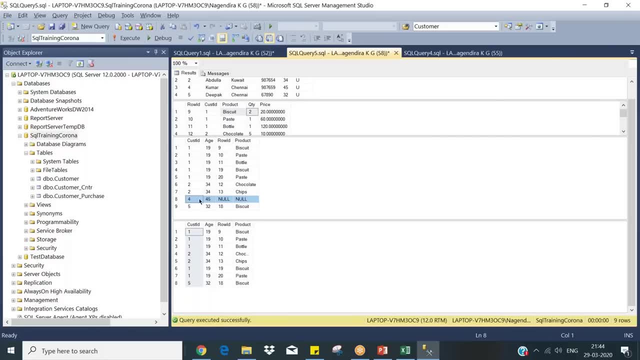 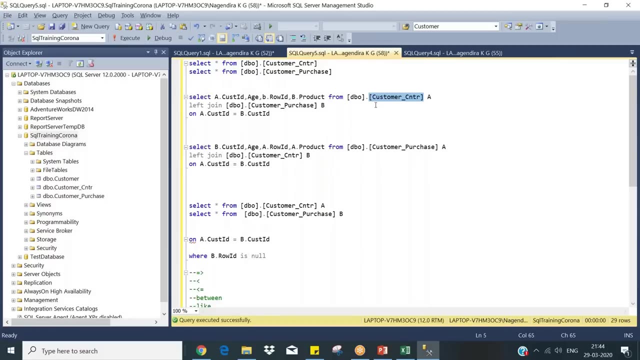 and this one, since it included all the unique values from your customer control, that is four. this guy also included. that is why one extra record is coming in this customer control when you use customer control as your base table. okay guys, i think uh taken more time in joints since. 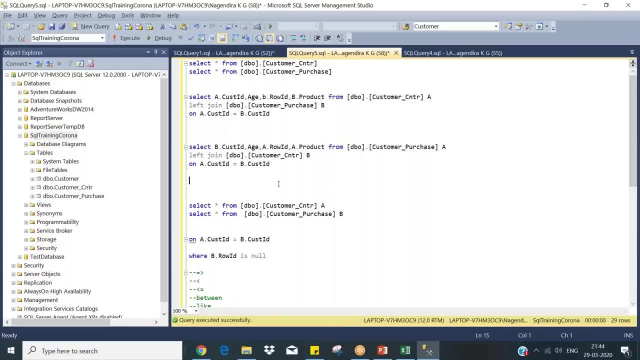 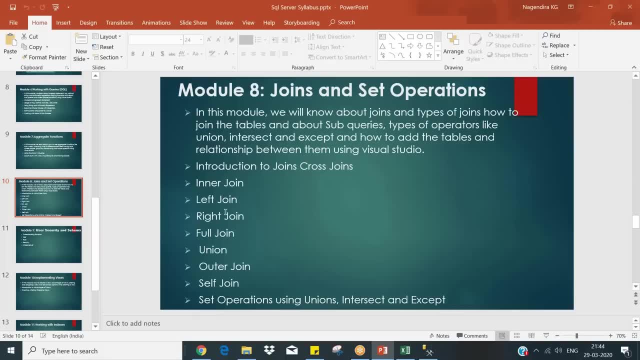 this is very important concept in any skill. once you have familiar with joints, then you are done. you are expert in a skill. so this. so left and right doesn't matter, you use use instead of using right. you can use left and right. so you can use left and right. so you can use left and. 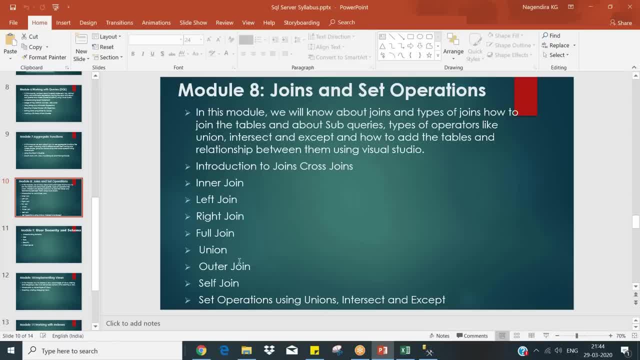 join. you swap the tables and use: okay, full join. we already seen. uh, we have a one more join called a self-join. all these things are recovered. full join, union, outer joins, outer join is nothing but left of the giant, right of the gen, but it's self-join. 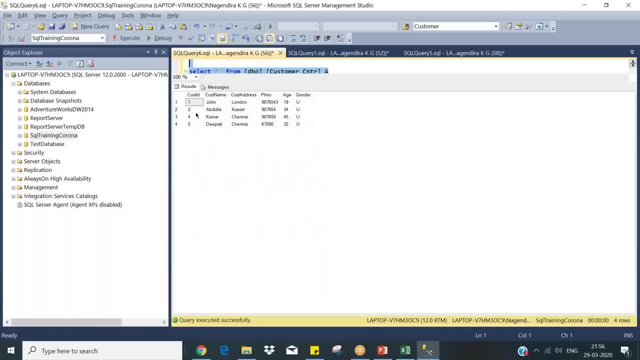 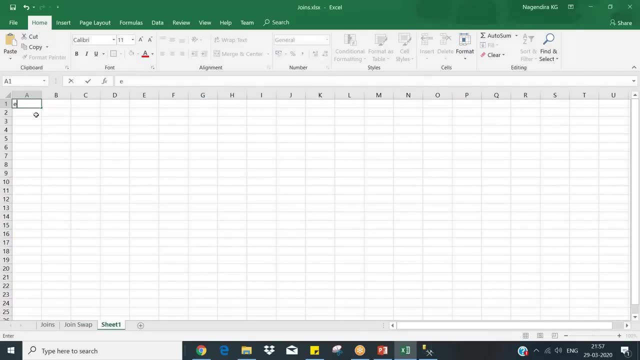 any idea. so self-join is nothing, but you join the same table again for some purpose, okay. usually it will be like: um, you have, uh, i will go to excel when you will use employee id. you have name, i have a manager id. okay, this is again uh important interview question in cts 101: 102, 103, 104. 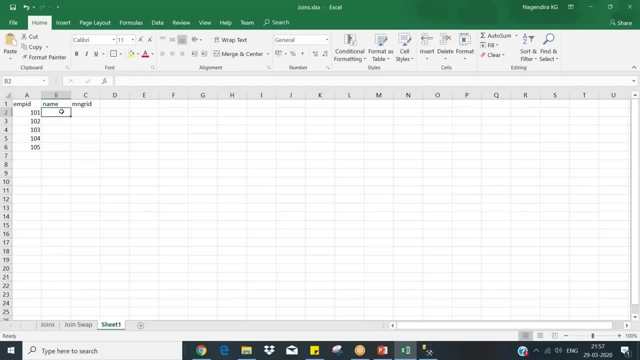 104, 105.. okay, these are employee names. assume like that: uh, c, each employee has a id and manager id is nothing but b is uh manager. i mean b's manager is a. if it is null, he is a manager, which means that this producer is. you need another um project manager, which means that the project manager is. you need a manager, which means that there is noidade. so we see as usual in the case of an offering unit, each employee has a manager id as an銷 juga, y tube and all things agreed. in this case, we will use a manager id as a manager id, just because using any empty cit with DK B 그렇죠. 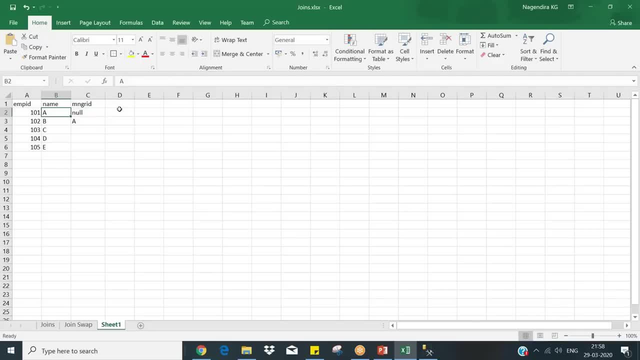 the topmost. no one has above him, maybe he is the CEO, something like that. so again, yeah, it can be a, C, hmm B. okay, so if the data maintained like this, so what it indicates is like: so these two information, it's easy to understand. so 101 is employee ID, his name is ABCD, and the same information, the manager ID. okay. 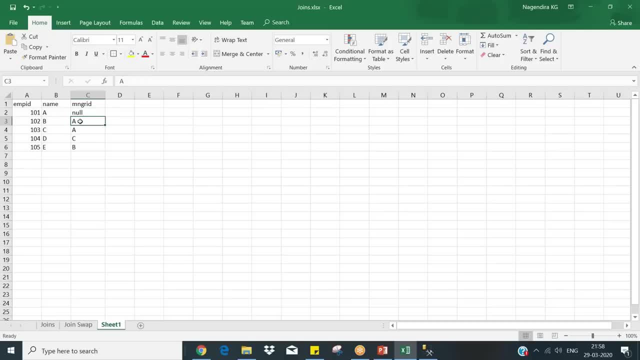 manager ID is nothing, but maybe name. ensured I need to use ID right. so it should be 101, and here it should be again 101. here it should be like 103, here it should be 102. okay, so manager ID means so far be a is the. 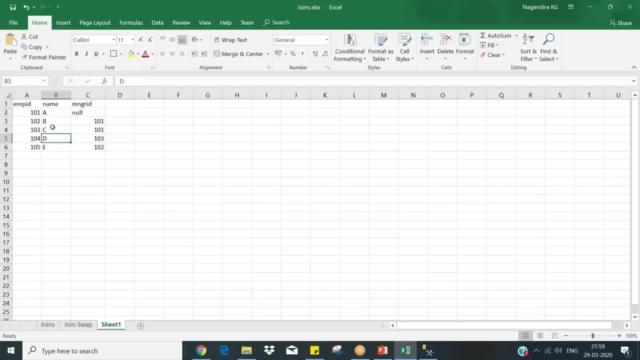 manager for C is the manager for D. C is the manager for E. B is a manager. in this case, I want name of manager. I mean I want this result like this name and manager name: okay, so he doesn't have a manager. and for B, it is nothing but a here. so yeah, and for 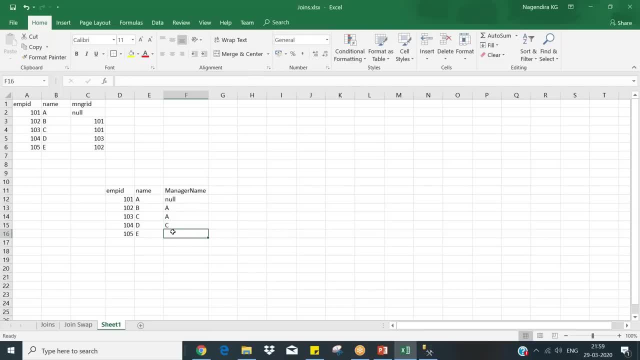 D it is C and for E it is B. you got it, guys, so this should be the result. how you will get this result? you need to do the join of same table again. okay, I mean I, you need to use the lift join of. you will use select star from employee left. 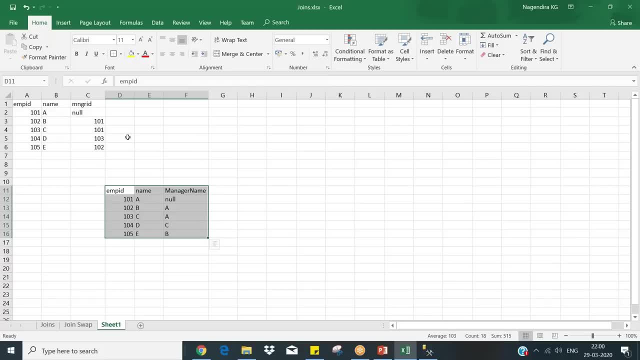 join with selection from employee again and you will give a different alice name. then you will get this results. okay, let me have a, let me insert this record. okay, then I will try to quote it in you. you got this guy this output rate. this is why there is what they are expected output. you need an employee ID name and 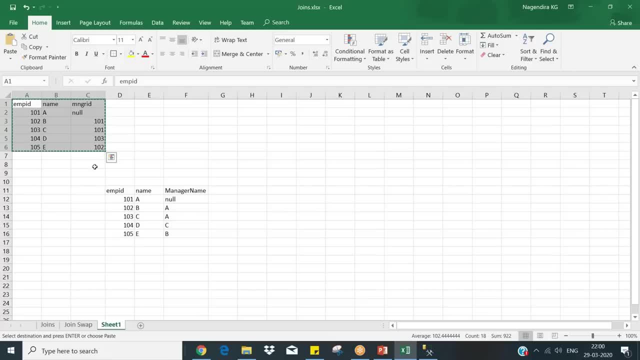 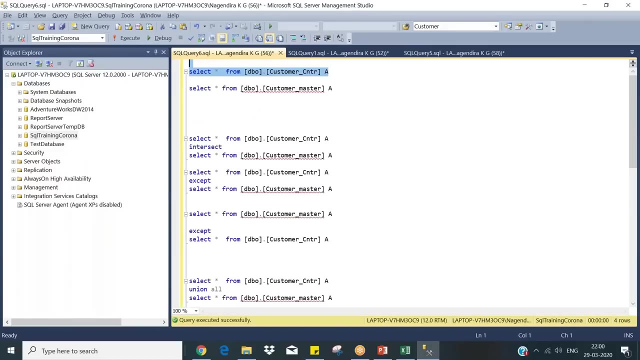 manager name. but you have idea. so you need to do this self-join of the same table to get the respective description. that is why you know there is a concept called self-join. so this is the scenario. it is not only you should have a manager id, self id, there can. 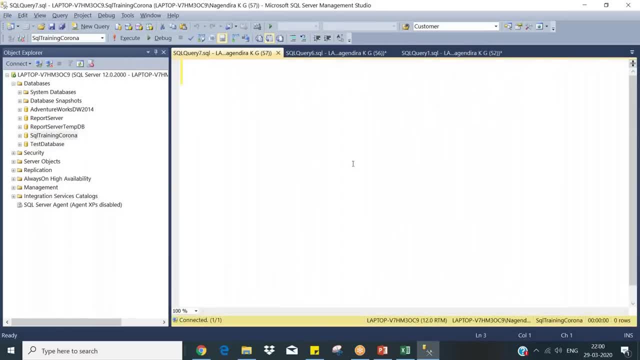 be a chance as any other column you want to create. i mean you need to fetch so that the same information available in the same table. so you will do the self-join. it's a time now, okay, i'll try to create in five minutes. okay, uh, create table employee. any doubt guys in this? 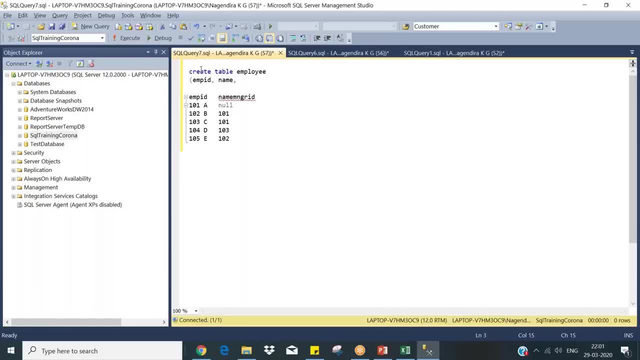 by id name and manager id. sorry, i didn't specify the data type- integer- where care of 10- and manager id- again integer. okay, i created, then insert values. i'm going to do some trick here. i don't think the trick will work. okay, it's working. 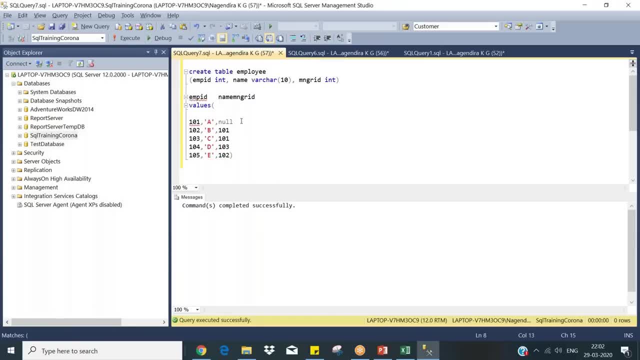 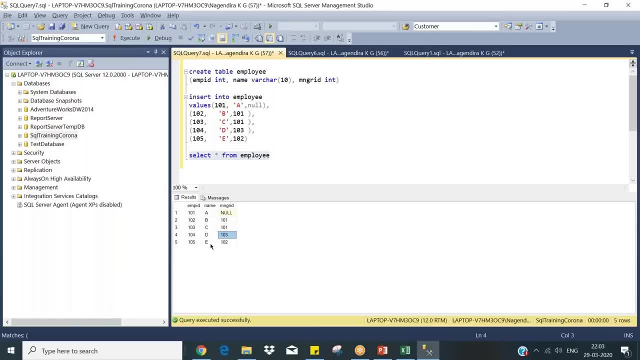 for C, I need to get a here. for D, I need to get C here. for E, I need to get B here. that is the output I want. now. this is the only table I have, so how to do that? so consider this as a table as left join. so now you see, this should be my output. 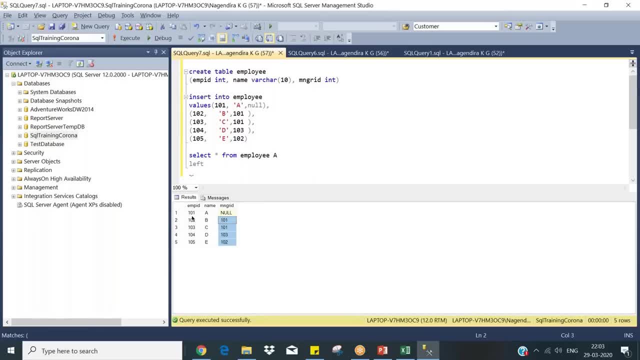 column for this guy only. I need ABCD. I don't want anything with this. so from this base table identified: this is my a table. okay, left, join again with employee table. what I want from the a table you don't do the manager ID, then join on a dot manager. 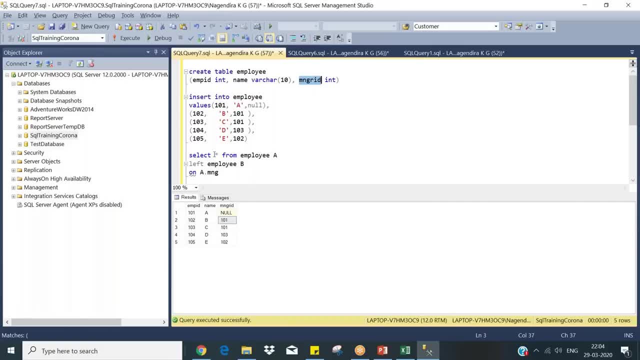 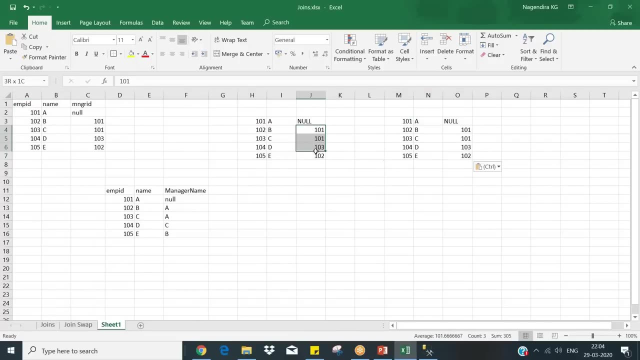 ID and from the a table. okay, what? what it does is basically, if you do the join, you have a table and have a B table. so from a table you take this call a manager ID, you join with B table this column, so obviously you will get a BCD. 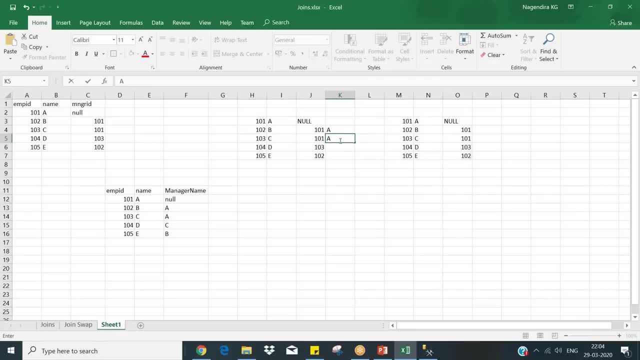 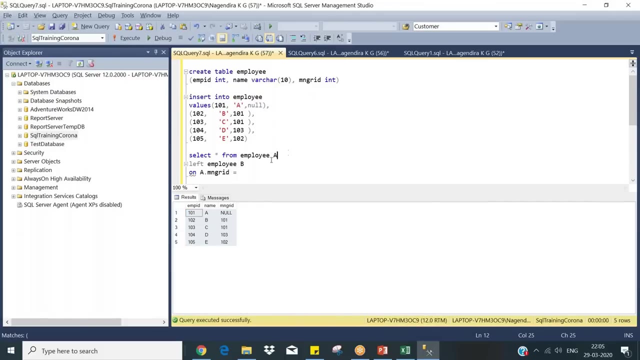 against here? yay, yay, c and B. so this is your a table and that is first table, left, left table and this is your B table. that is what I am putting. a and B, okay, so a, that managers HAngers' ID, B dot and employee ID. okay, you see a dot, start first. you see the. 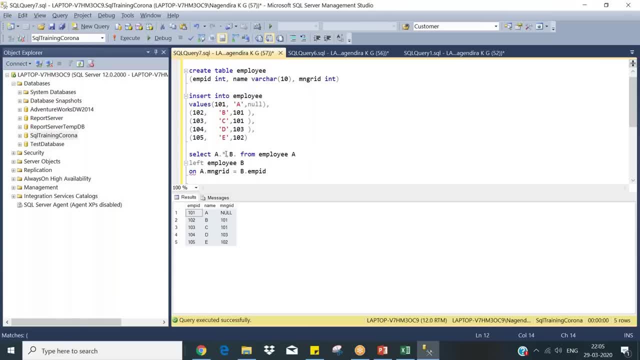 output. then you will get the manager. that way. I left and I join and I am on the get to know. be that star correct, right, live, join. I put only lift left join on this right now, you see. so these three columns from a table and these three. 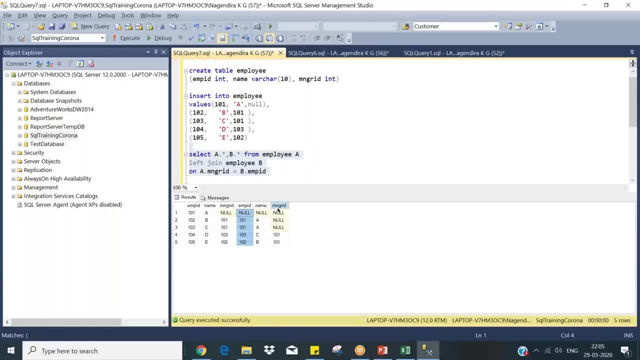 columns as, as I indicated before, join will give you a table format. whatever you use the left table for that, it will add some more columns based on the join you used. left join link. there is no 101. I mean for him null. so there is no records for 101. so it had these two records repeated here. this is again this. 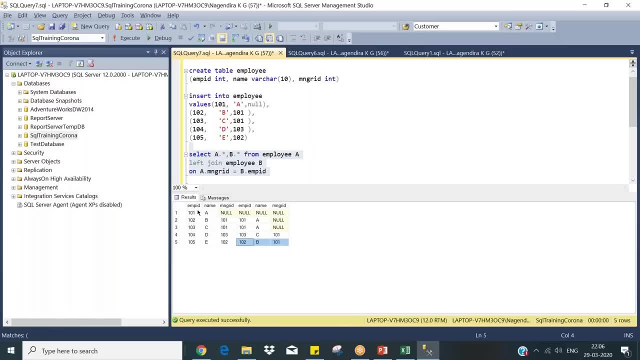 is again now what you want. so you see guys here: employee name, manager ID, again employee name, manager ID. so this name, you are giving allies a name as manager name, that's all. so let it be a manager ID here. I want output be that name. make it as manager name. so this is like giving 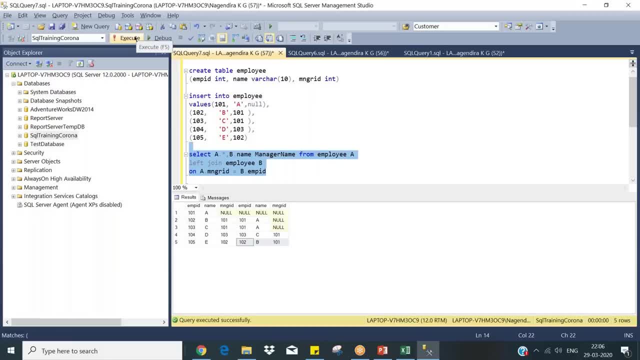 allies making it as manager name. you see the source data. then only you can understand better. so understand it, guys. for be employer, be 101 is a manager whose name is J. say a 103 for D 1 or 3. 1 or 3 name is see, so see for II. 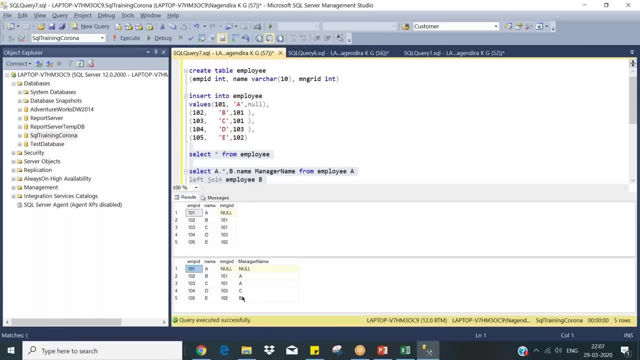 one or two. one or two is B be here. so you got a manager name, okay. yes, so your crucial part in understanding SQL is understanding your joints. if you are familiar with this class, I mean if you are confident in this class, live, join in a joint. forget about right, John, stop it later. this conference will now be: 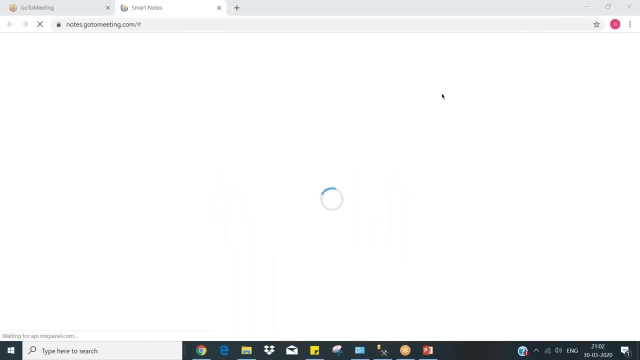 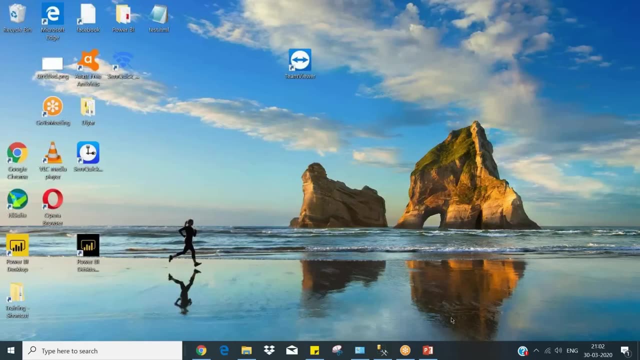 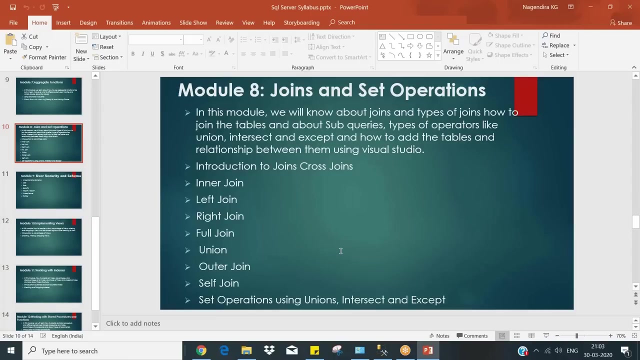 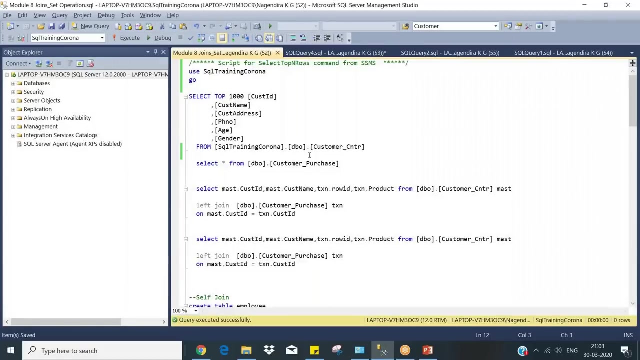 recorded. so I just want to have a couple of minutes again in joints because people have always have a confusion and only if you know joints then you can say you are expert in escape. so yesterday we saw about left joints I mean. I mean we need to use joint for the purpose of, in order to get 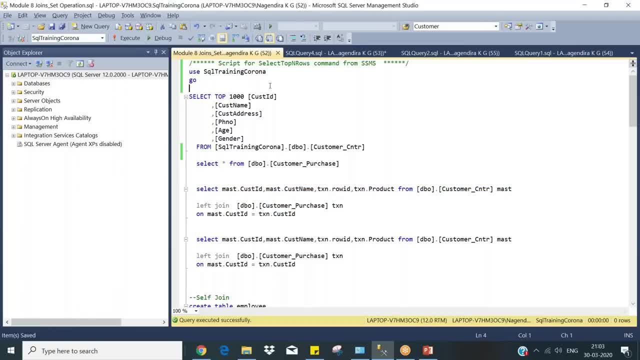 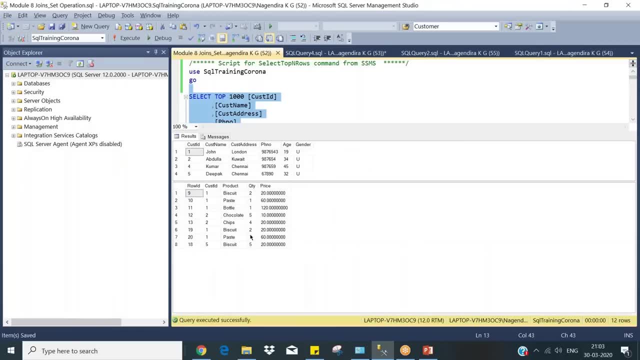 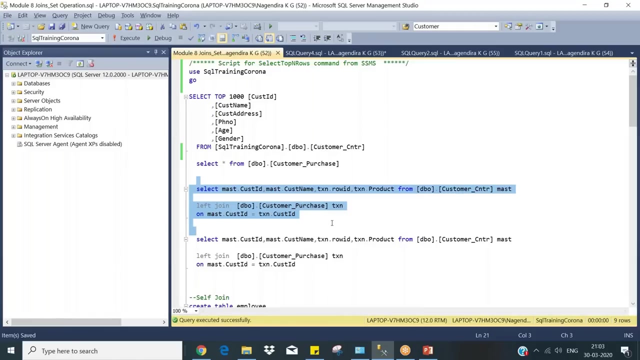 information from some other table. so refresh session up. so you've got two tables. now you are doing a left run here to get the related information, this product, whatever he purchased. so is there any rules like how many tables we need to join? so we got here a transaction table. fact: internet says: 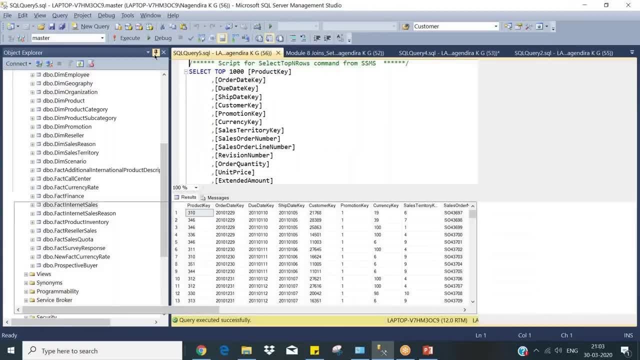 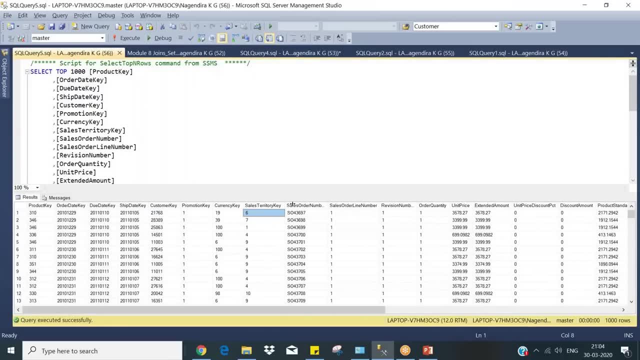 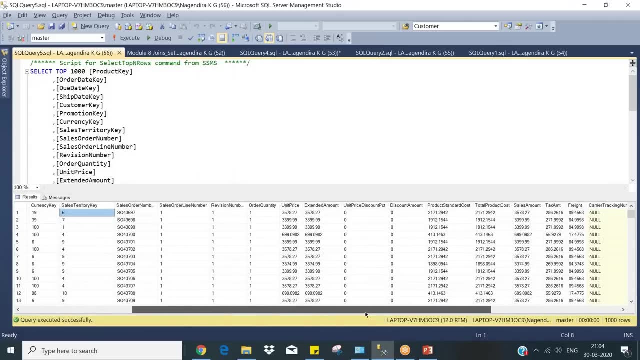 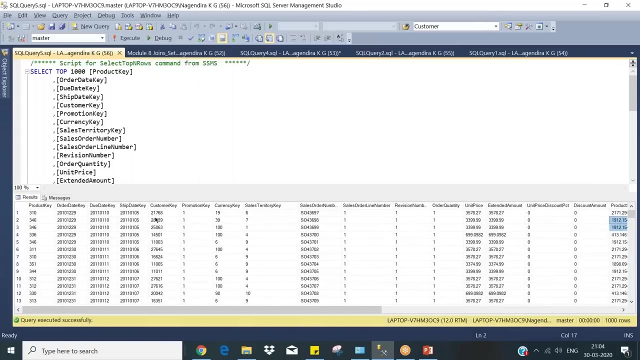 okay, this guy contains all the references like customer key and what is the sales territory? key territory is nothing but your region. so this guy has got only the references. the values are available here. so say, for example, I want to get, I want to know this customer, what are the products he brought and in which? 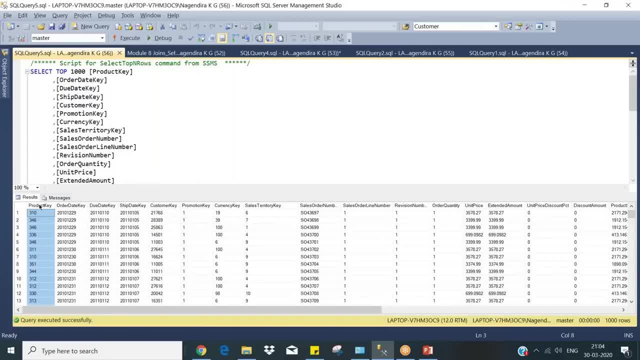 location he has brought. okay, so this column, this column and this column. so, in order to get this particular customer name and what are the products he has brought and what is this location, physical location, he has brought, there are, to get this one, I need to join three. 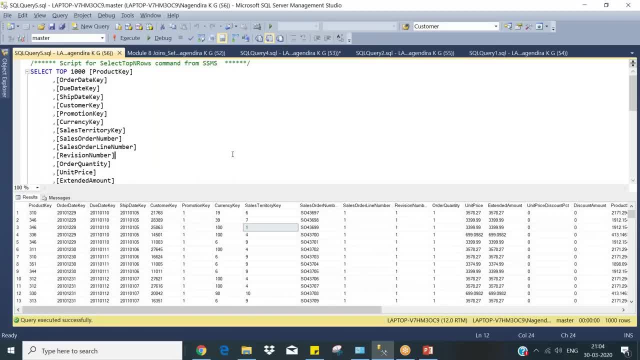 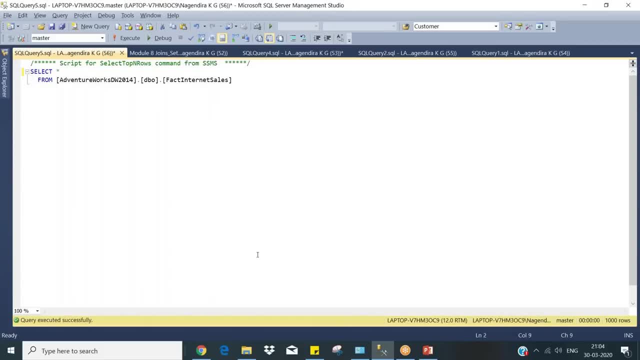 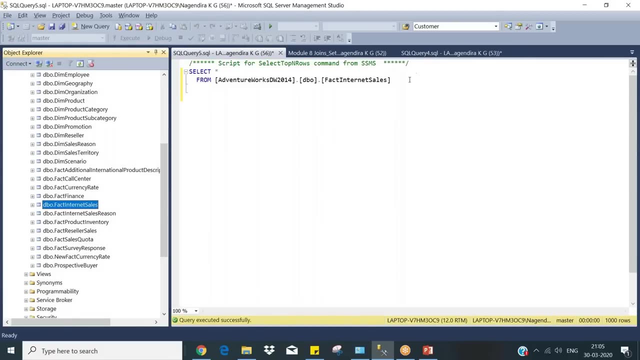 tables to get this information, okay. so how to do that? so obviously we will select all those tables here, will list down all those tables. so this is the first table. as I said, I want a customer, I want product, I want sales. I want product, I want sales. 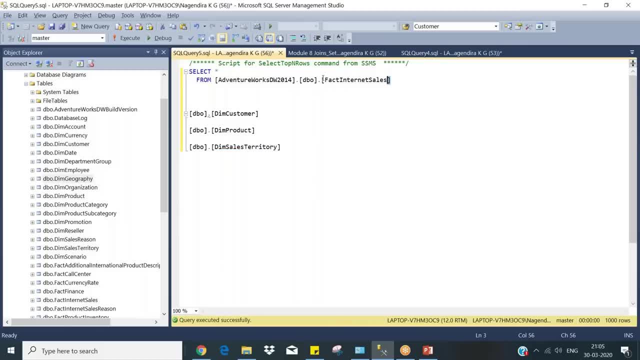 stay. Okay, start from. so usually, in our two sense, that is not Esperanza. here is A column: which job says it's worth a hundred, but this sentence says it will be created Hey, star from. so usually in order to sense the data. everybody knows this thing is dare to. 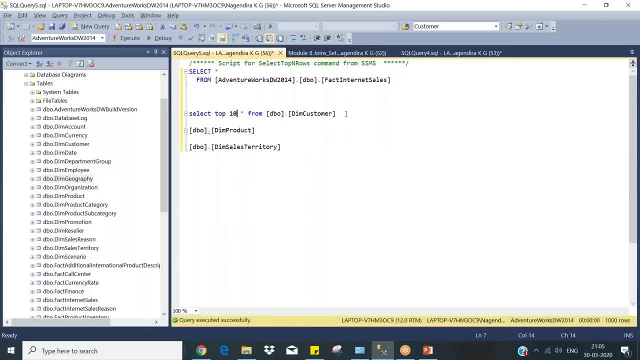 want a identity. did not get the RT, I want a customer. okay. so sometimes there are have often Any other voice excursions here. we want just one right, if any, and other reason mean what data it contains. so just put select top 10 rows, a top two rows for now, to get what are the 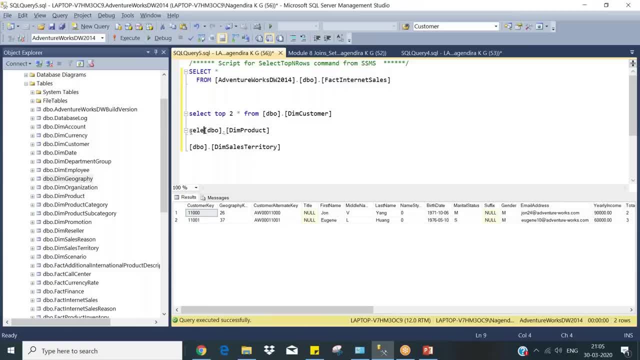 information we need. so people will ask: i want a customer information and what products he has brought and from which location. like this only people will ask: you need to see what information we can provide. some cases it will be specific. they will provide exact column names: what they. 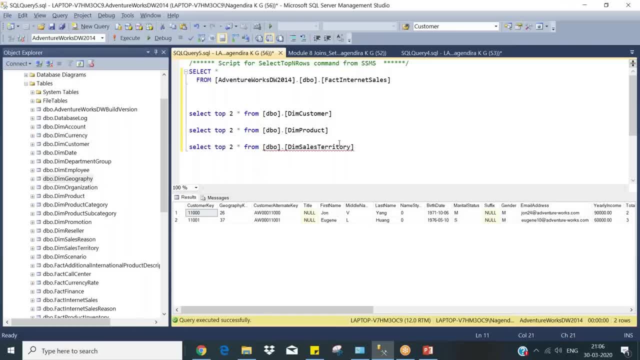 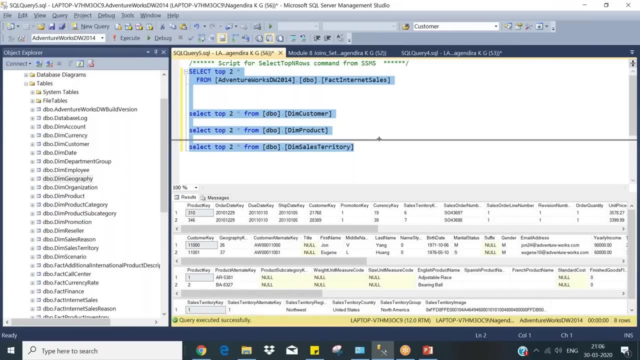 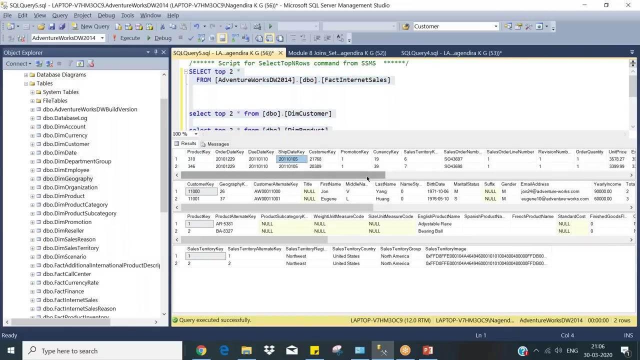 want. i need customer name, i need customer location and i need this product category, something like that. in some cases, they won't provide anything. you need to grasp all the information, okay, so this is what you have in this table. so this is your transaction table: the customer product and what. what is the purchase price of it? and 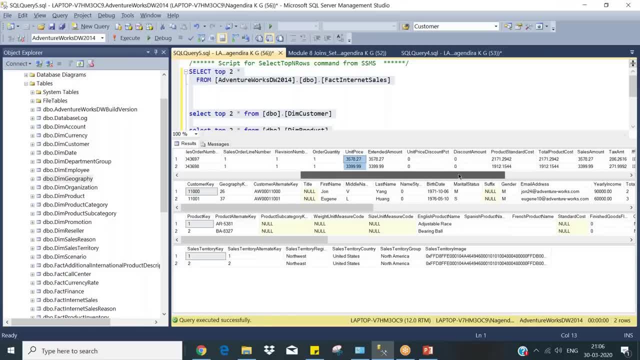 uh, is there any discount amount, discount price, percentage, product standard cost. all those things are available here. and when it got ordered, when it goes shipped, all this information is present here. this is your transaction. then this is your customer information. customer information: have a name, birth date, email address. what is this income? all those things then. product product code is: 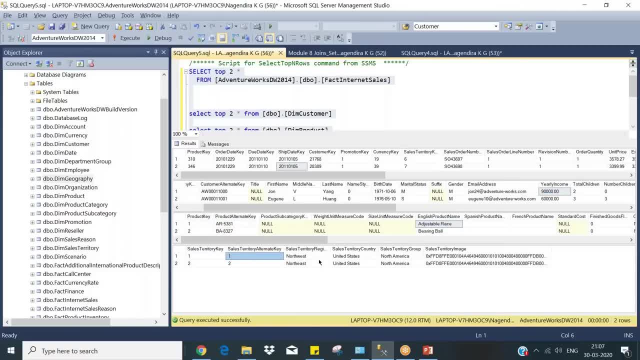 there. what is the description of it? then, sales territory: it contains the country name and group. let us, uh, have our in our report. we will have a customer name and his email address. then from product i need a product name and from region i will have a country. so these are the things i need from this transaction for this customer. okay. 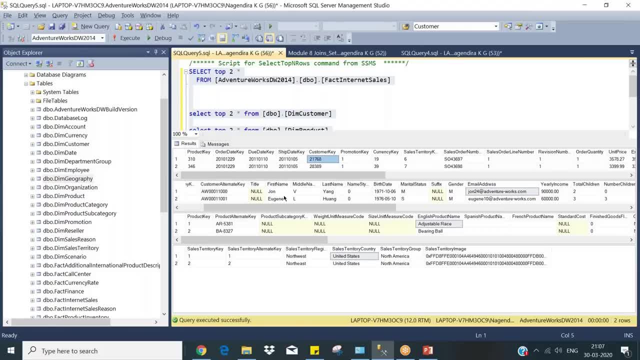 first of all, if, if the if the people ask, like for john v young, i need um all those information. or they can ask from united states who are the customers from, uh, this particular product, adjustable race, who are not as broad. so if they ask like this, you need to join all this possible. 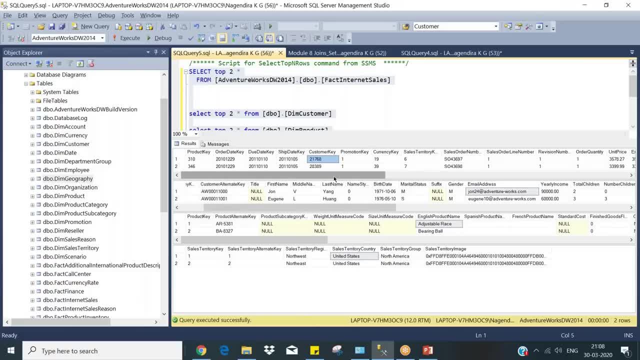 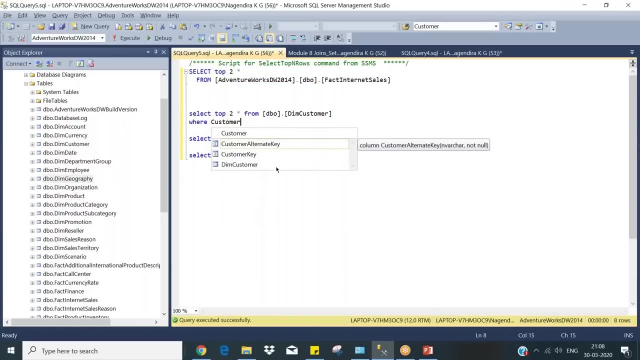 company. you need to ensure that. so back to our question. so for this customer 21768, they will not be able to open the client. they will ask like 21768. maybe we need to find for one particular customer what is the 21968 where customer key equal to. 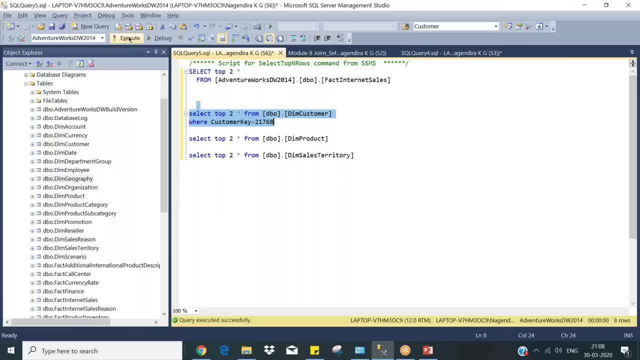 you can put it in quotes or integer. i mean, if it's integer, no need to put so. people will ask, like for cole air watson, can you give me all this list? okay, something like this. they will ask a question like this, so let us do it in a query. so first of all, i need to have this table. 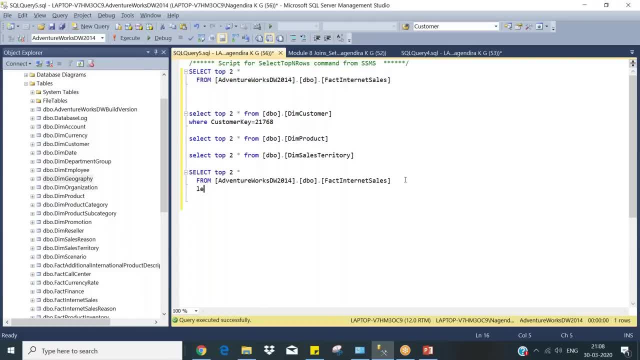 then let me join. there can be any order. there is no specific order here because i want all the transactions first, so i will put all the transactions will be included. then i do the left join of customer. so first i will put fact, internet sales, i will put fct for customer. 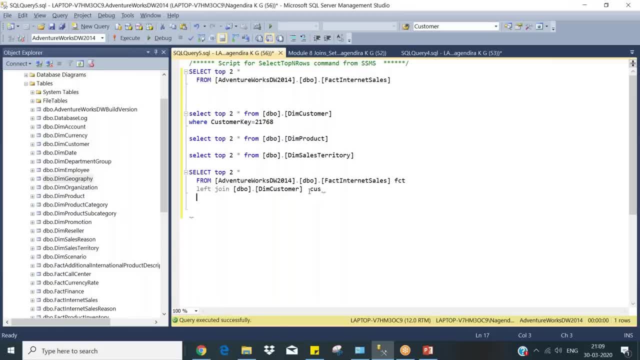 i will put cus so i hope you remember what is this. this is alia's name. let's join on fact. sorry, fct dot. customer key, customer key. customer key, dot. customer key. now what this will result i i will get a transaction details after doing this join. 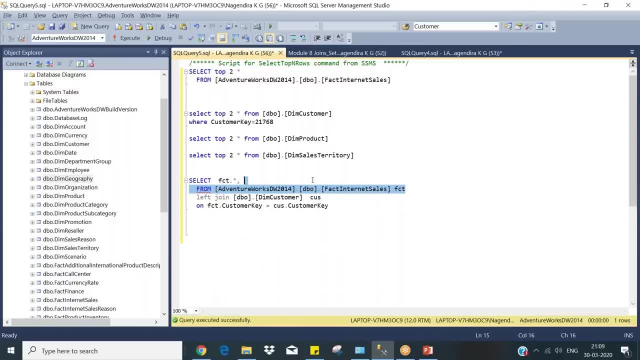 my output will be another new table that will have all the columns in the fact: internet sales and what are the customer attributes of it. so customer dot. let's start. maybe i will put the customer information first: first name, middle name, last name. okay, let's keep it like this. so when i select this one, 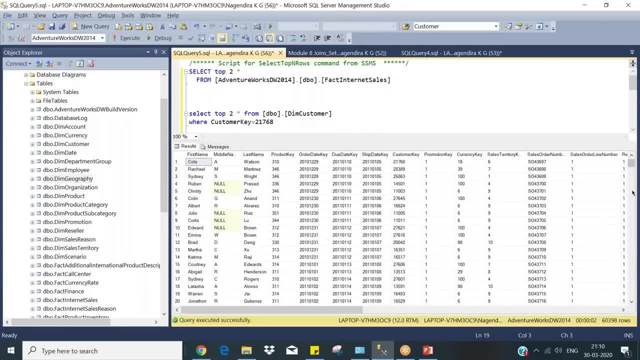 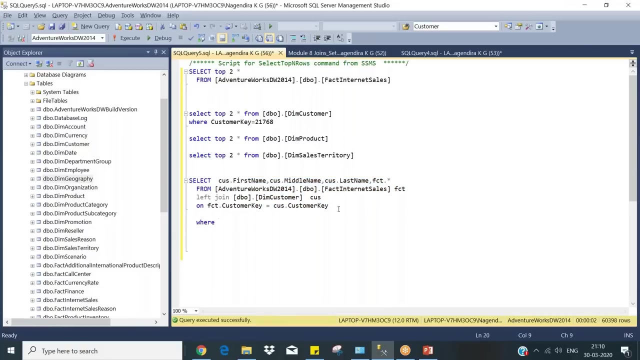 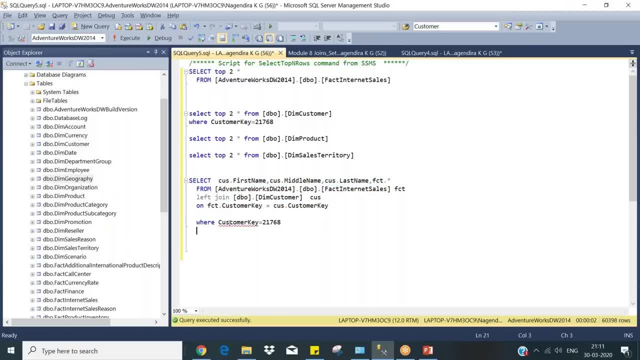 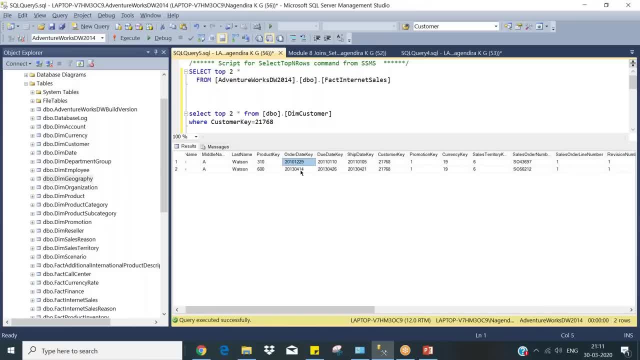 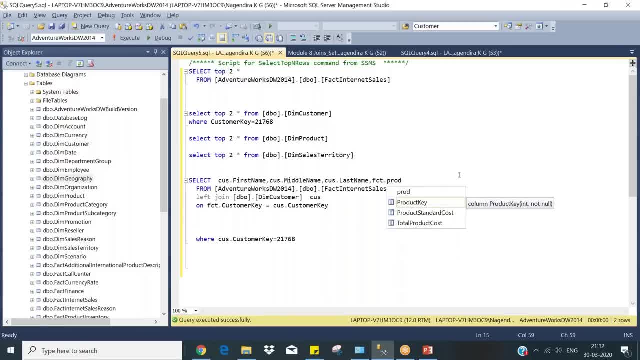 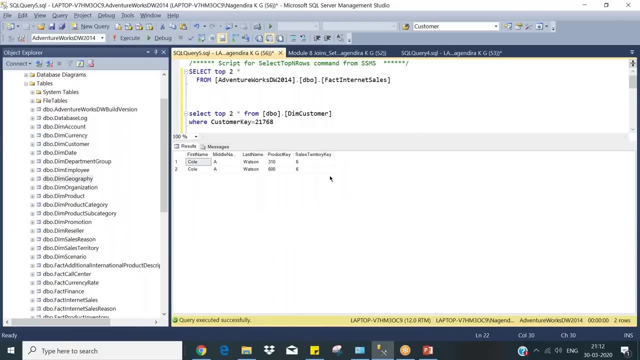 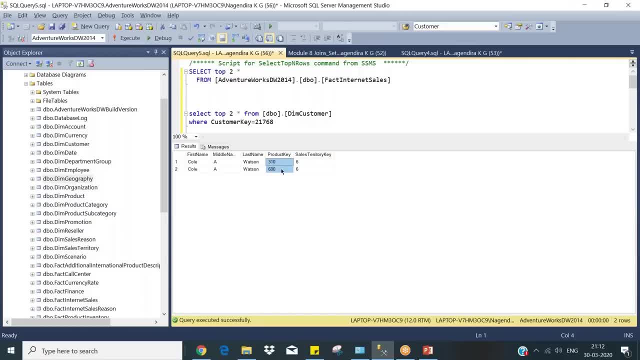 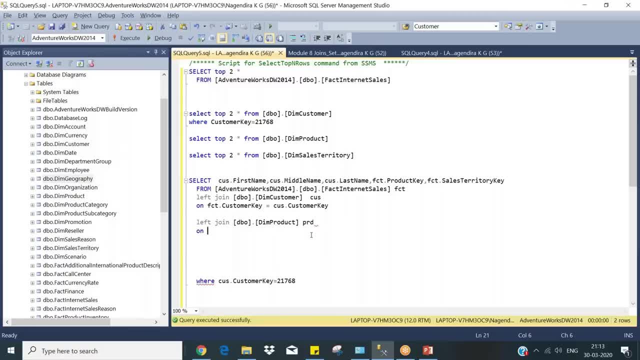 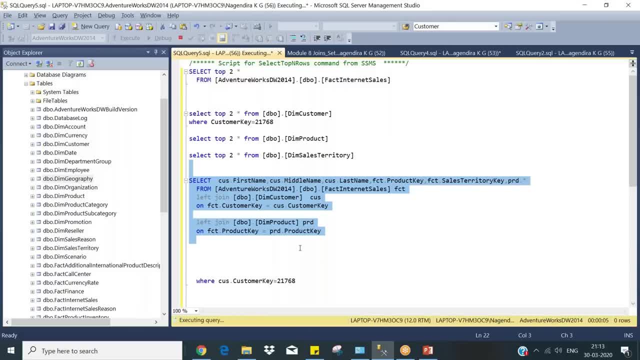 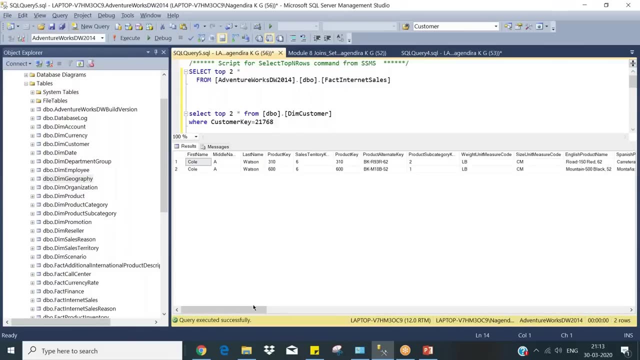 Oh, sorry, See, I have to filter. I mean, I use, I need to use where condition. Okay, Now you see, for this product key. this is a till, this it's from fact table. After joining, you got for three, 10 and 600 product. What is its attributes? You got it in a table. 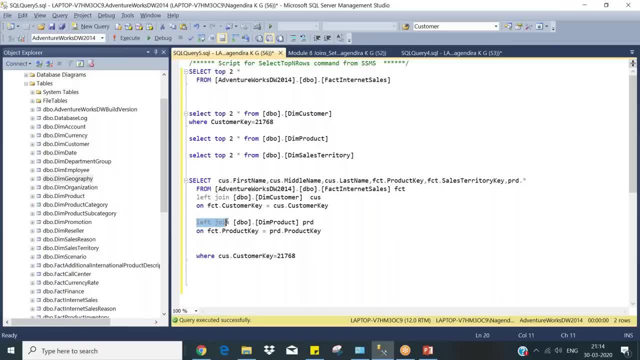 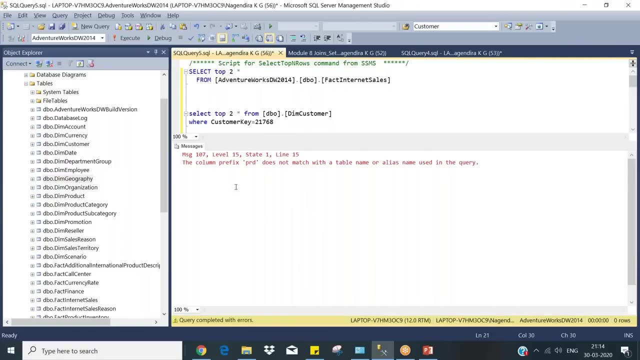 This is your left join, See left join here. We'll take all the inputs from here. Okay, All the inputs. What is the output of this, too? I mean, when you have a condition here, okay, You need to have a condition. What happened? Okay? 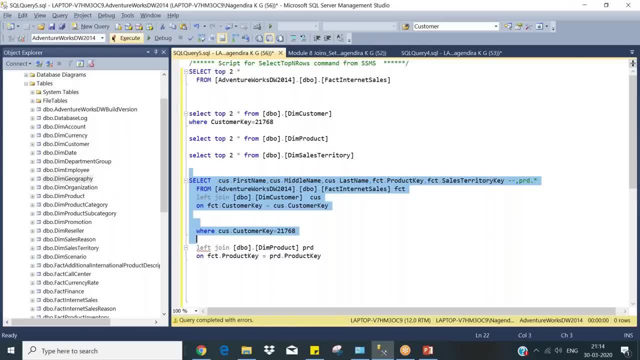 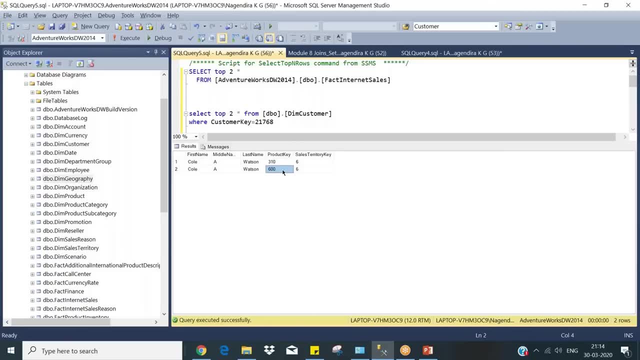 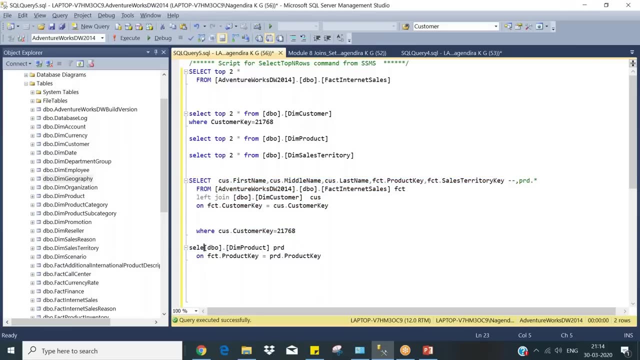 This table doesn't include it. now, See, that is the purpose of your left join. So this is your output. Okay, For these two products. Okay, What is my data? So you can have multiple data here. in your left table You have only two records, but in your right table, right. 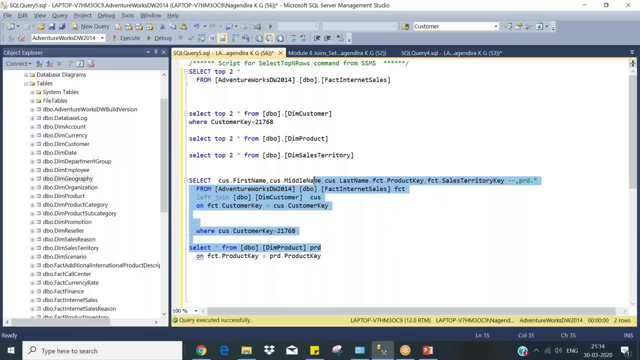 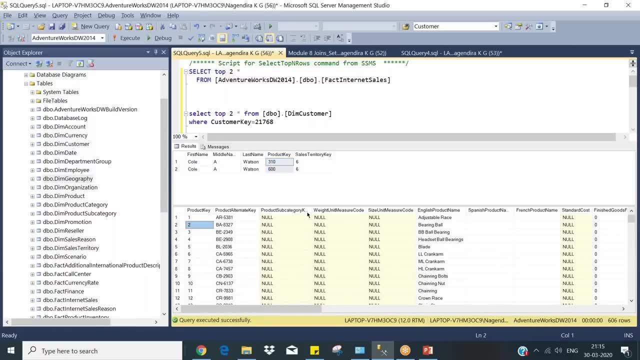 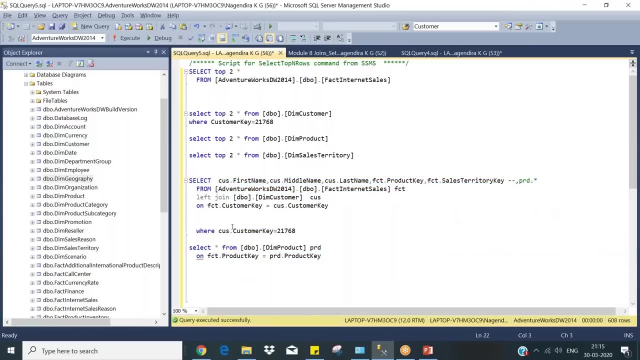 table is nothing but your product table. You have only two records. in your right table You have 600 records. It doesn't matter. Once you do the join, Okay, It will give you the results. This is your condition. See, without. 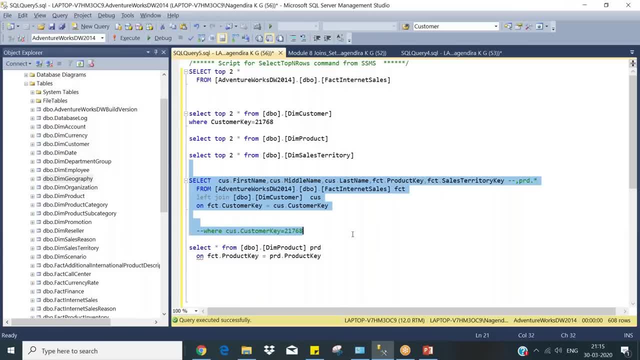 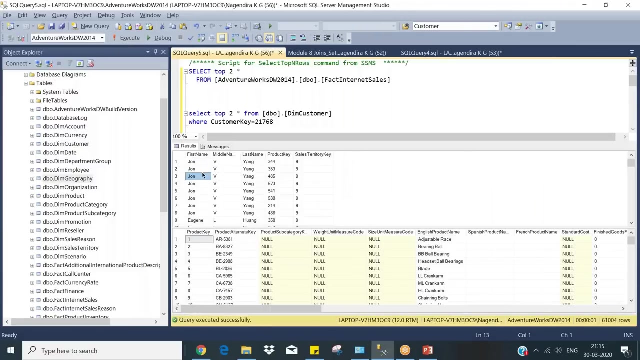 this condition. it does for all the records, I mean all the 60,000 records for this fact table. this condition filters it. If you see, if I put this condition here, you got. my point I'm trying to convey is typically this first query is giving me 60,000 records, all the records where 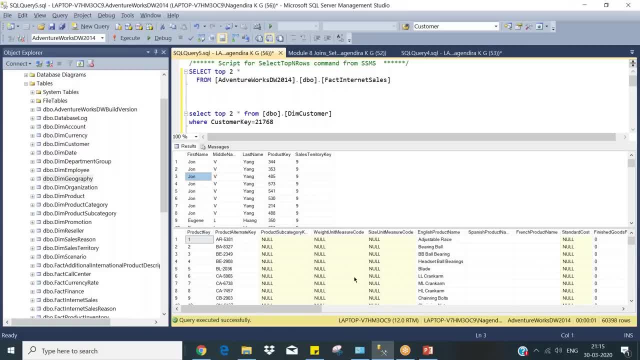 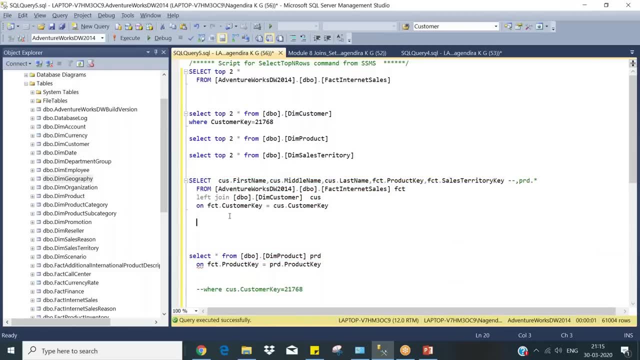 condition is filtering for only John and the second product table. if I join without where condition, it is returning for all the 60,000 records. when you use this where condition, it is filtering only customer key, that is what it is happening. left join. okay, now obviously you need. 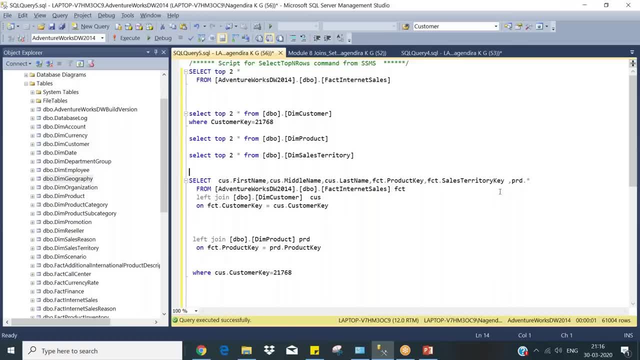 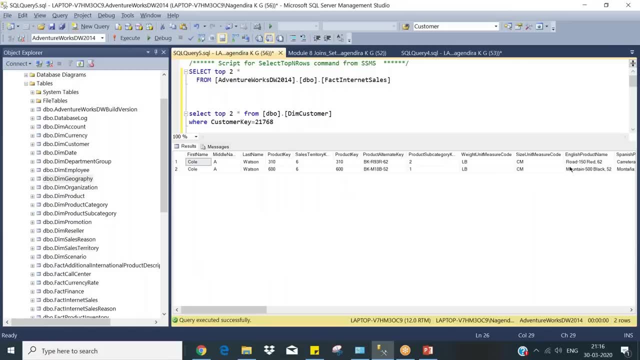 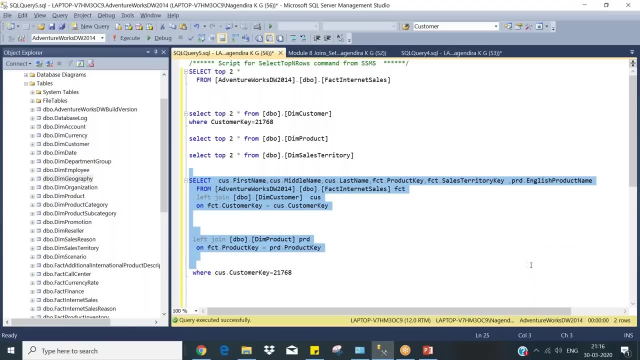 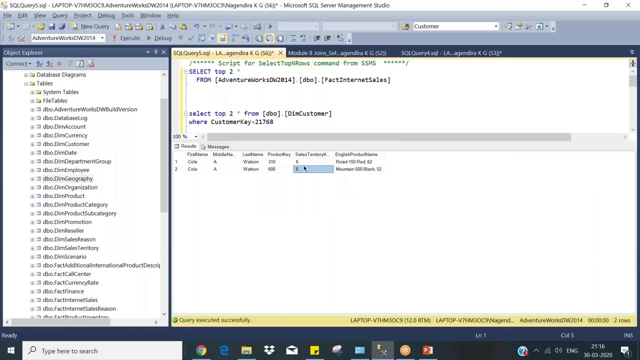 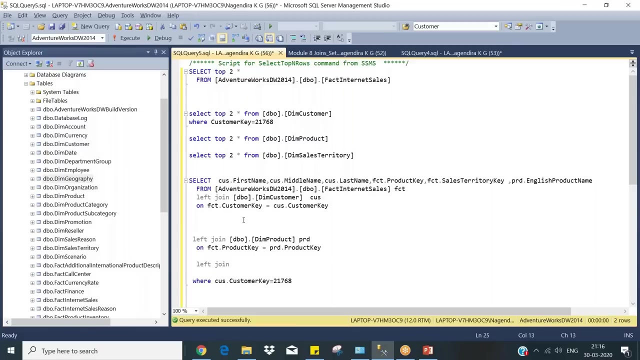 to have this guy. now I got product information. I don't want anything else except the product English name. so just keep product English name. again. you run now this is fine. so what about the territory key? territory key is six. again you need to do. let's join. data key is in this table on FCT dot. 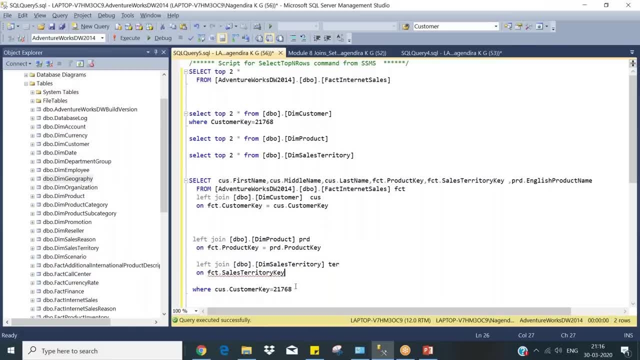 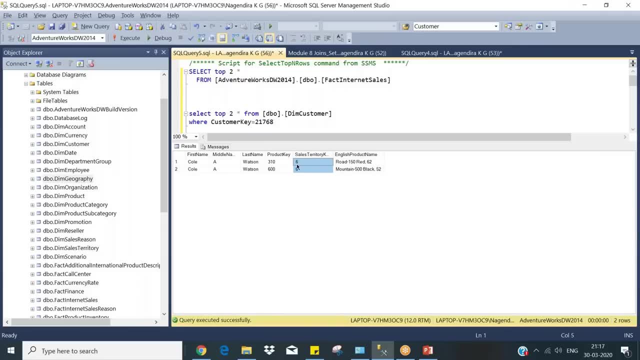 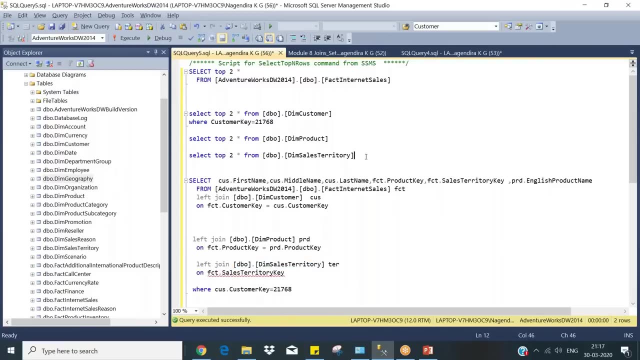 sales territory key. see. let us go one step back, since static key is six. so in this record, instead of six, what values you need? you need the country. what is the value for sales territory key is equal to see. six will see that one sales territory key equal to six. 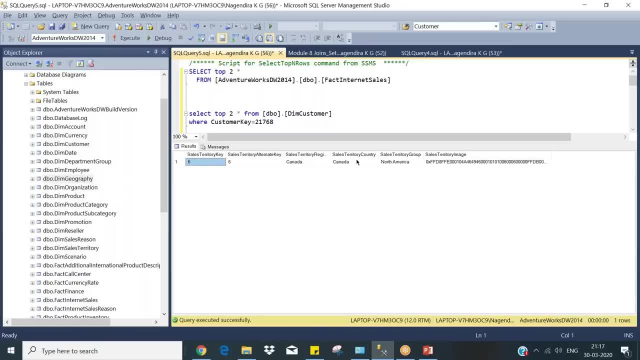 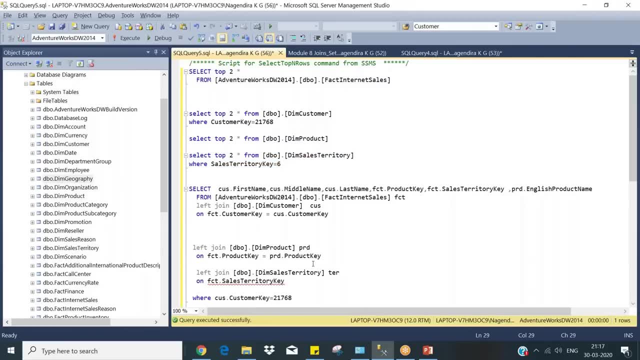 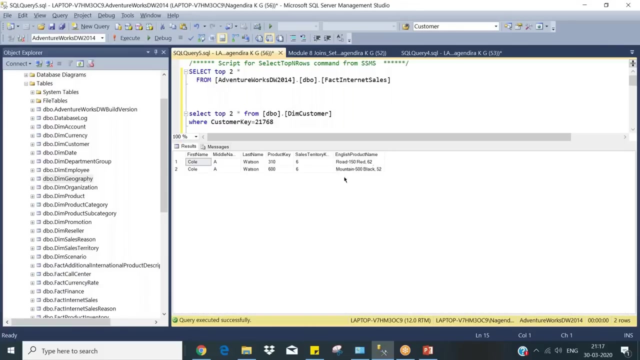 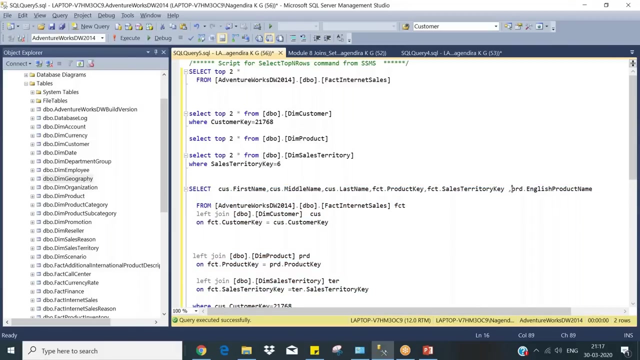 so sales territory key is six. what is the country name? Canada? okay, Canada. I am expecting in this output you, since territory key now I didn't see once you join it it will not obviously come. you need to say select what columns you need. okay, you need to explicitly specify. 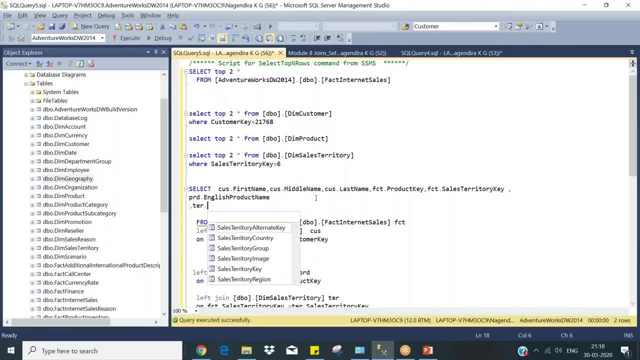 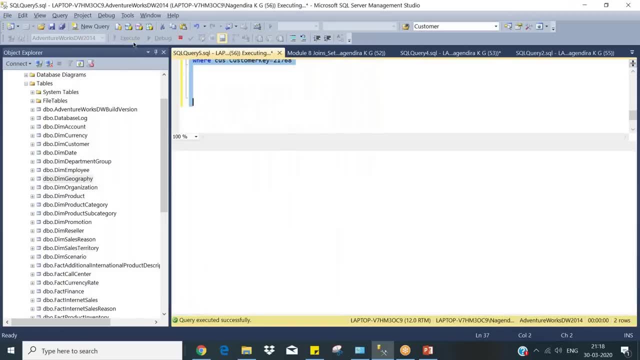 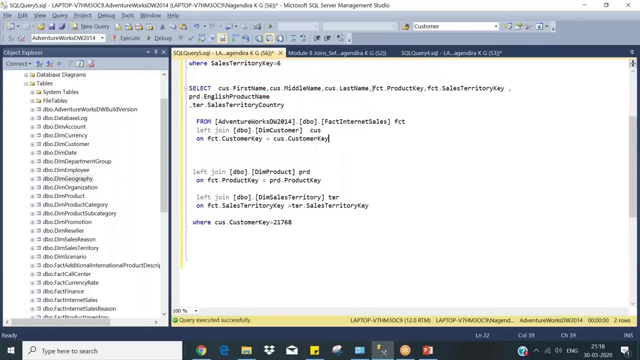 but internally it has created another table with those columns country. now you need to query like this: so now you got canada here, so you use this product keys as a joining column. once you got the desired output, you can remove those keys. keys doesn't have any meaningful information. 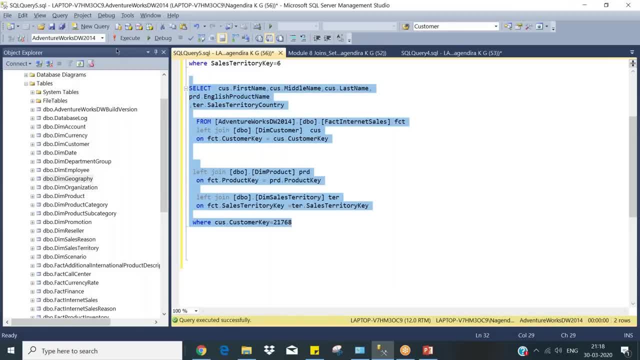 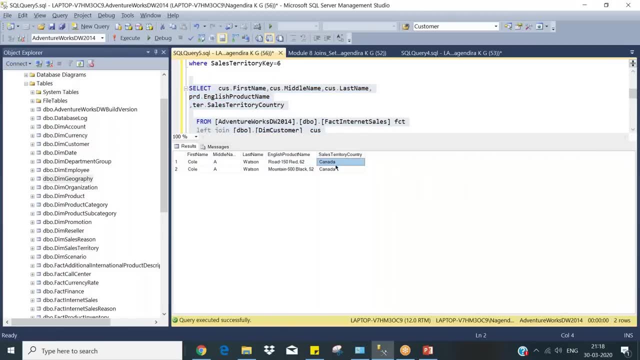 okay, now this is your final output. if they ask for cole watson, he has purchased these two products. he from the location canada. this is your output. so joints: there is no restriction that number of joints you can make. it's not only two tables from a single table, whatever columns it refers. 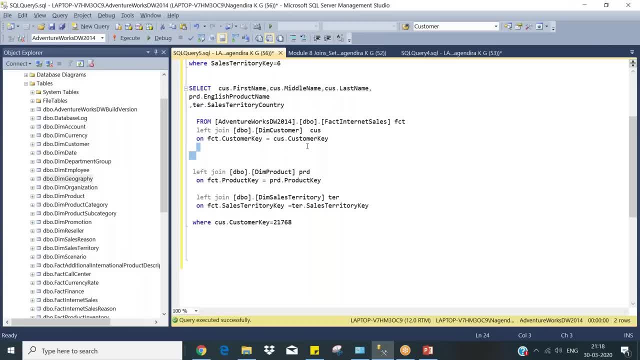 you need to get the missing information in another table. i mean, if the information is missing in the same table, it is in available in another table. you find the link, then you use appropriate joints. see this condition: from here factcustomer key, customercustomer key and from here factproduct key in dim productproduct key. 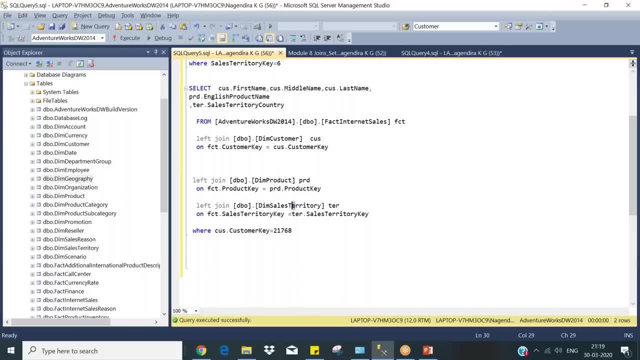 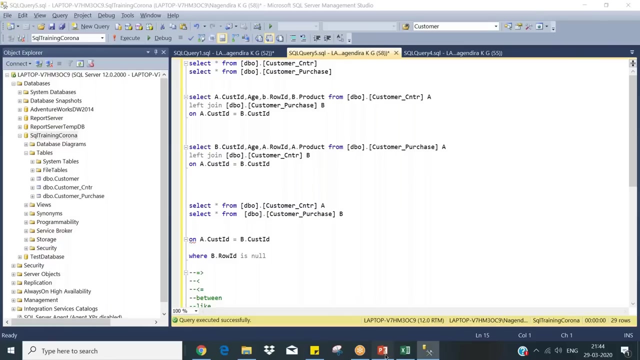 from here you have a sales territory key and dim sales territory key. this is again a simple example for using multiple tables in a joints. okay, any doubts guys? okay, great important concept in any skill. once you have familiar with joints, then you are done, you are expert in a skill. so this is a left hand. 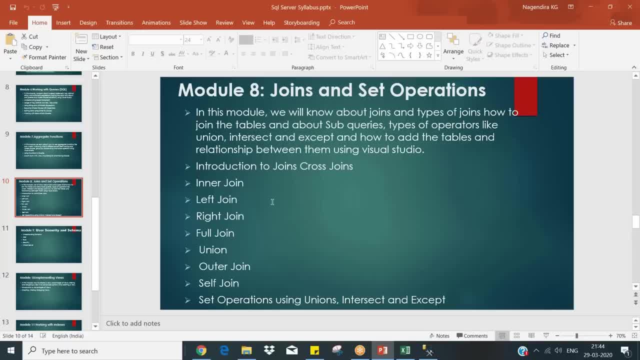 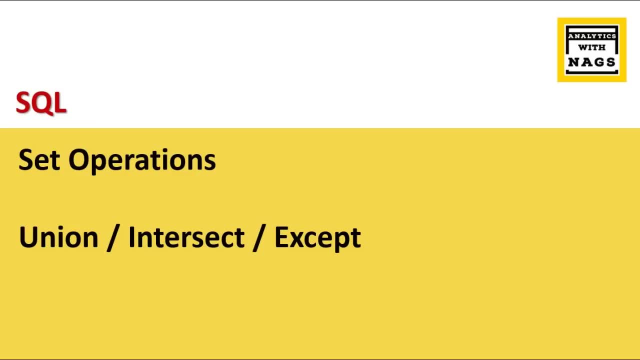 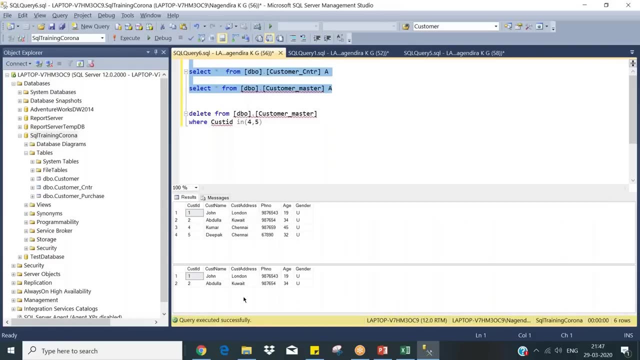 right, doesn't matter. you use use instead of using right, joint. you swap the tables and use: okay, full join, we already seen, then we'll see something. and self join, union, all those things, okay, okay, guys. now you see, uh, customer one and two, john abdullah, all those things. now i want to combine the results of these two, okay, uh. 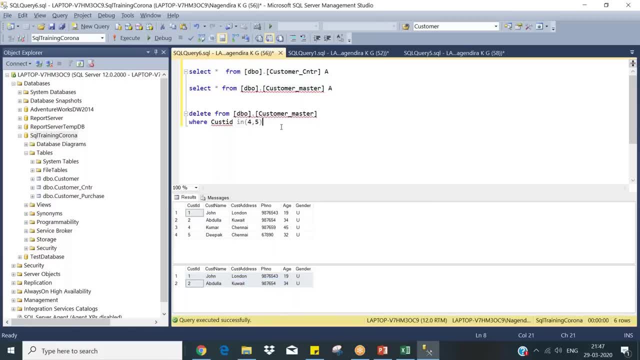 instead of this i will have another record inserted, insert into on the query, maybe quickly i will do the things. so i'm not specifying the column name here, i mean, instead i will directly put the values. so i i taught you about values. instead, you can also have a select one. 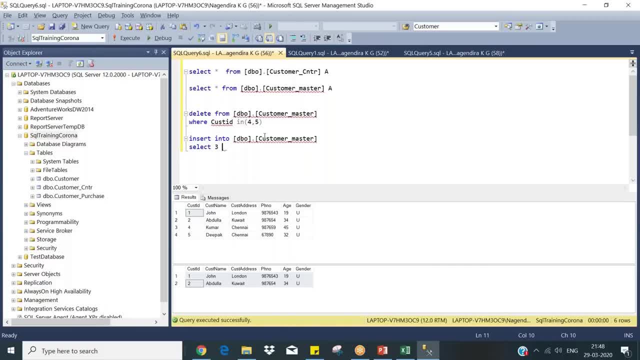 comma. instead of one i'd say three, another landlord you can specify like this also: okay, now what i'm trying to do is, like you got uh customer information, uh in two tables, uh, table one and table two. this kind of scenarios will come. you have multiple branches, some people will have a branches wise. 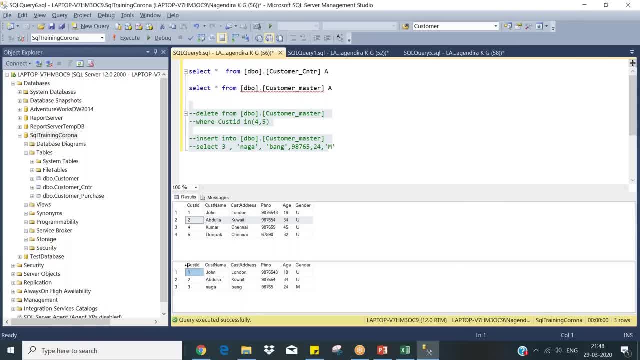 information they, if their application is legacy system, they use- uh, i mean, they have information scattered in different places. at the end they want to match informations. okay, now i want to call the information system, so i will just do a little bit of a plug and fly that way in just a second. 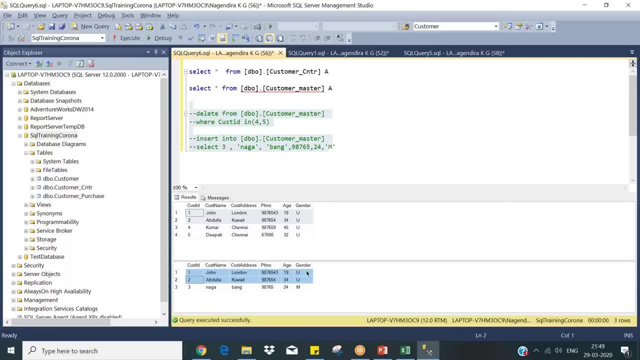 so the way i'm showing you guys is just a quick way to how to combine and see both the customers and that can be chances like i have a duplication also, these two customers over here, these two customers over here, but i want a unique. values are just first of all, we will see. 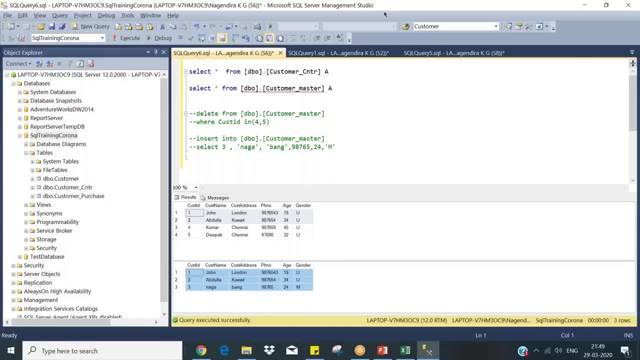 how to combine these two results so you cannot do the join. join means this information: okay, this information will come to your right side as an attachment to the existing records. it it will again pick you a table. okay, result set. but it is a attribute. it becomes attribute of this particular. 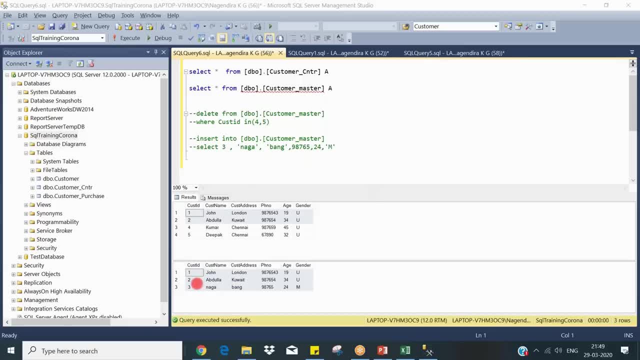 column if you do the join. but when i want to get the same results as one, two, four, five and it should result as three, i mean concatenate the results. i i want to add a row, i don't want to add a column, extra column. okay, for that you need to use set operations like union, union, all, so let. 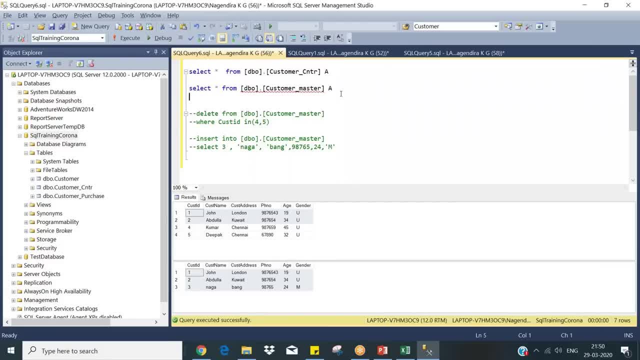 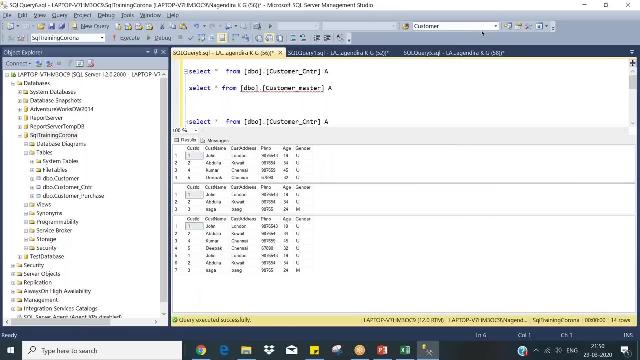 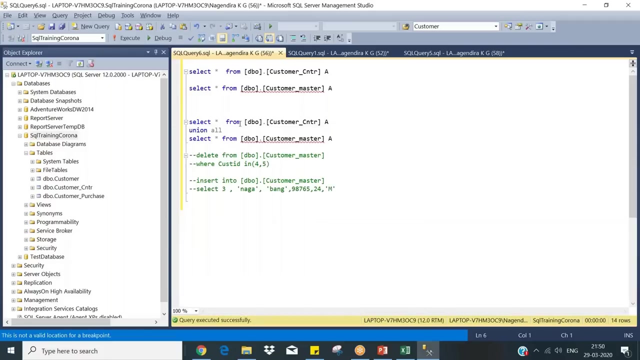 us do union all. so you need to execute as a whole. then only you will get exact output, expected output. so what is the result, guys? so you have a table and this is your table two. the combined results is nothing, but you match the records rows- okay, not as a column- and again this will result you a new table. so this is your union all operation. 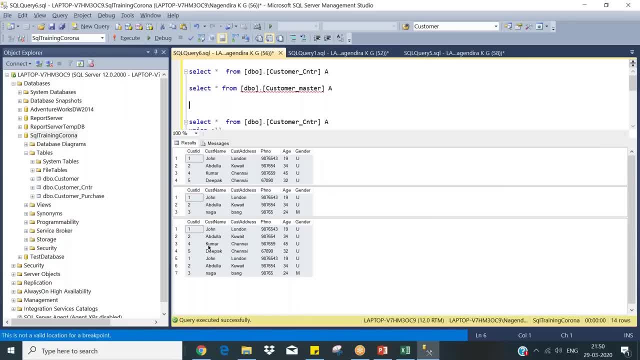 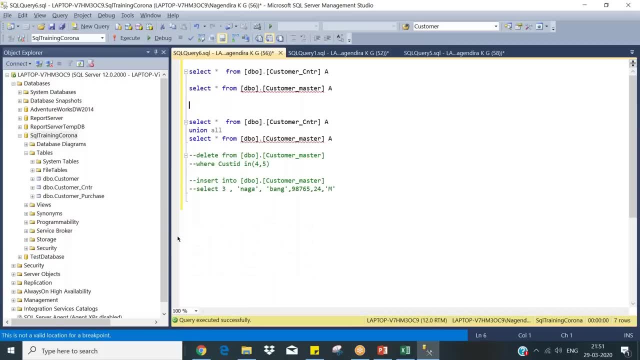 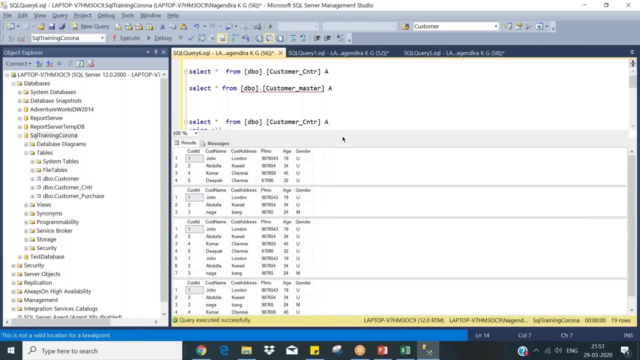 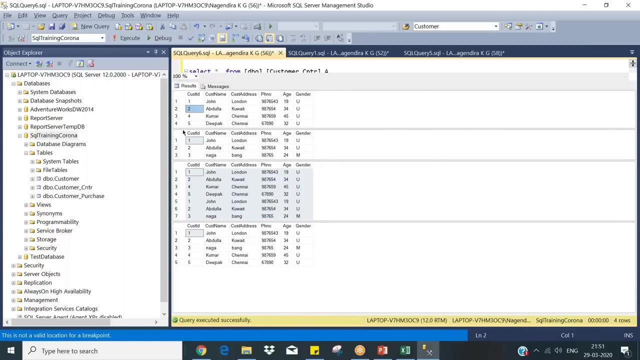 okay, and there are some cases like i don't want the duplicates. so this five and six and one and two is exact duplicates. in that case, i don't want duplicate means just you do the union, remove this all, condition that will give me the unique values. now you see, this is union, all it combined: three plus four plus three, seven records, so seven and. 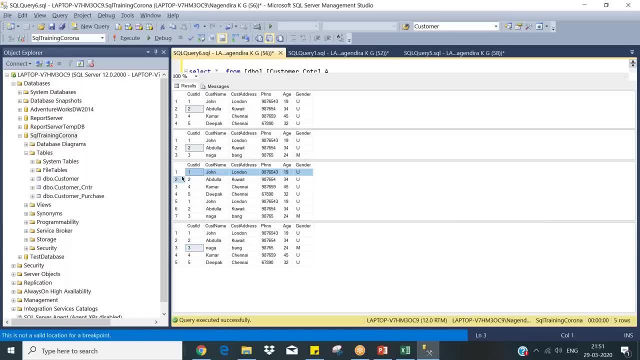 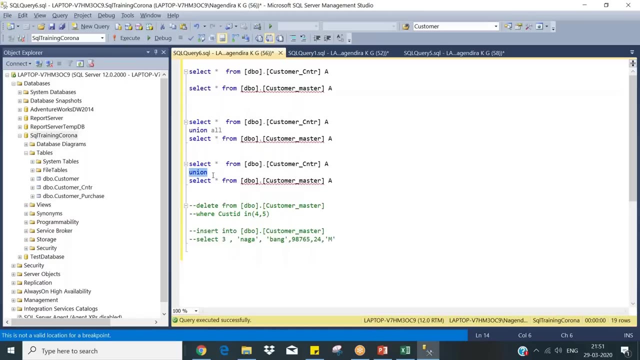 union. what happened? it skipped the duplicate and i want duplicate. so i have to duplicate the duplicate. duplicates one, two, one, two here. it skipped it and it gave me only the unique records. so how it skipped all those things this union will take. the union program is written, i mean. 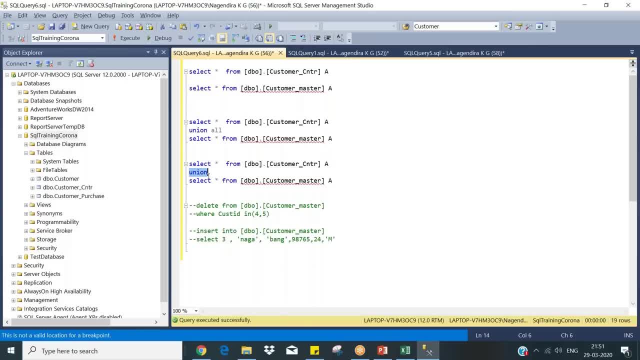 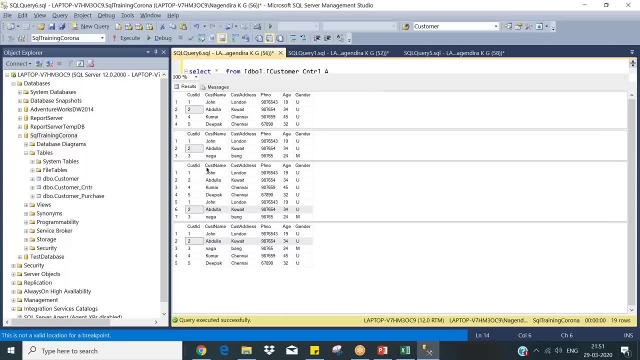 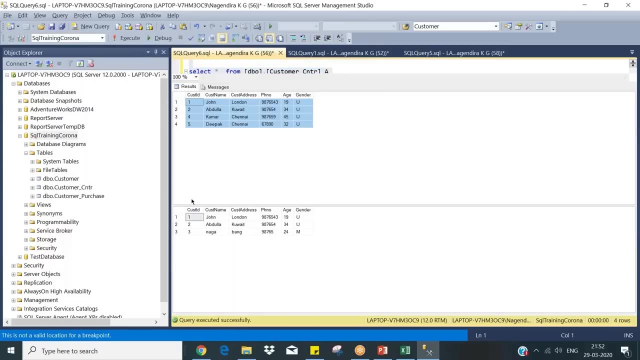 this program is already written. so this is your union and union all, and there are some cases like you have a customer here and you have customer over here. i want to identify those are not exist in b table, so i want four and five. okay, in that case. 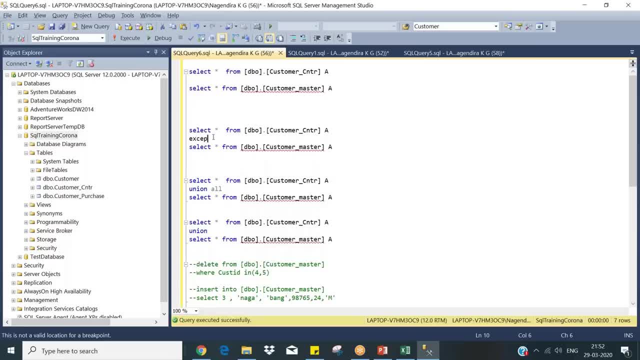 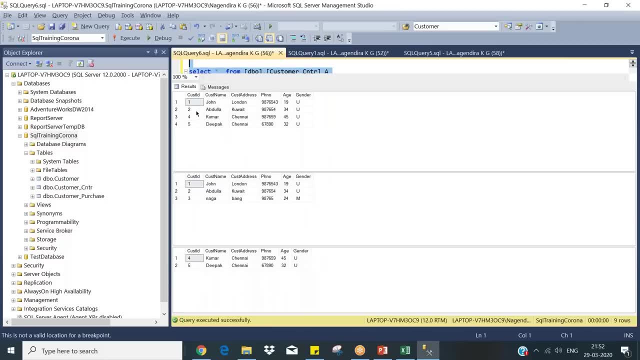 take to this guy. i'll just put accept. so what happens from the table one, i? i will compare with table two. i want those who are not existing table two, so i got four and five and if you do the vice versa, so one, and i mean to say i want, uh, those. 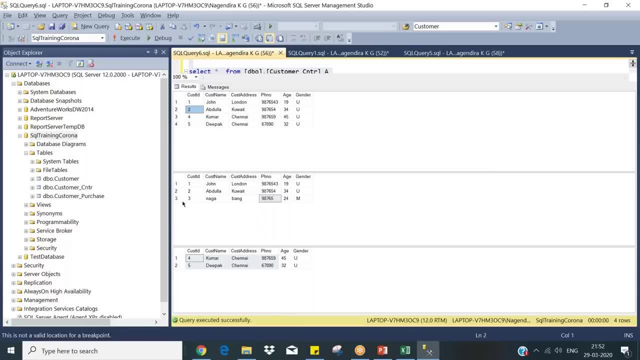 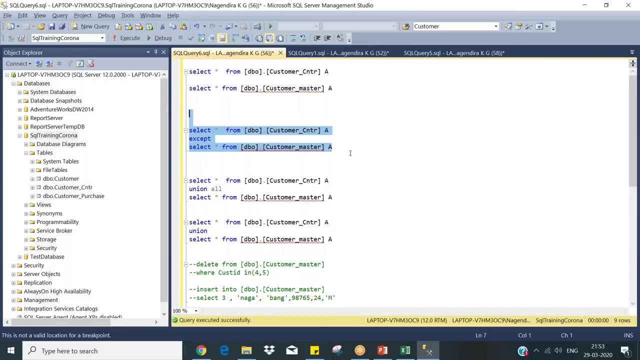 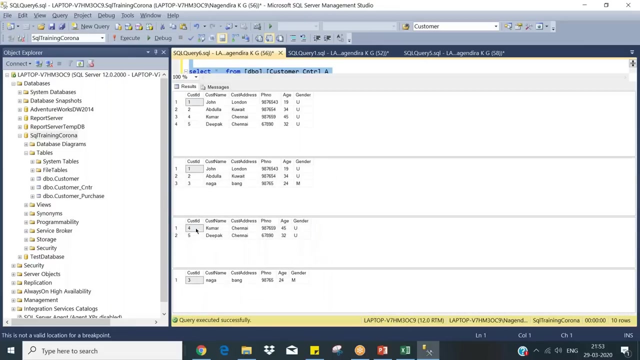 who are does not exist from table one. i mean table. what i'm saying is: i will use, i want this result from table two. i want the customer who does not exist in table one. then just stop the table and i'll run together. so first result is: uh. 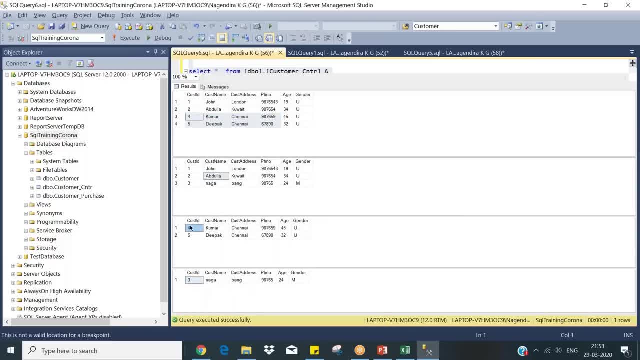 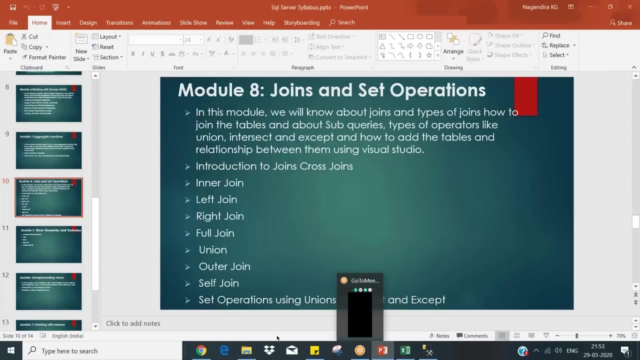 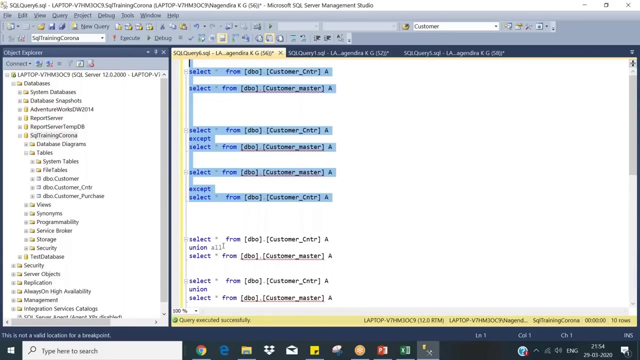 one except table two. second result: i mean this result is nothing but four and five. and the next query: I have written table to accept table one. so this resulted me three. now got you guys Union intersect, except yeah, intersected in, tell you. so now we saw about Union, Union all, Union all. 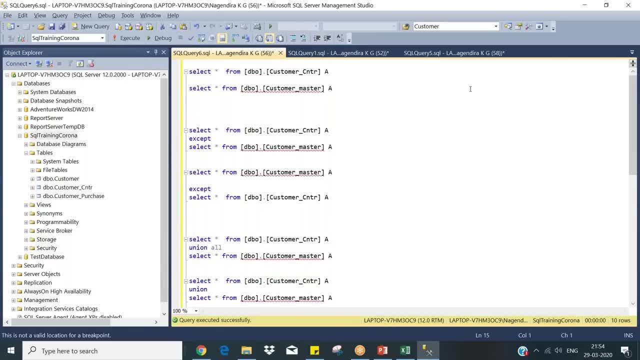 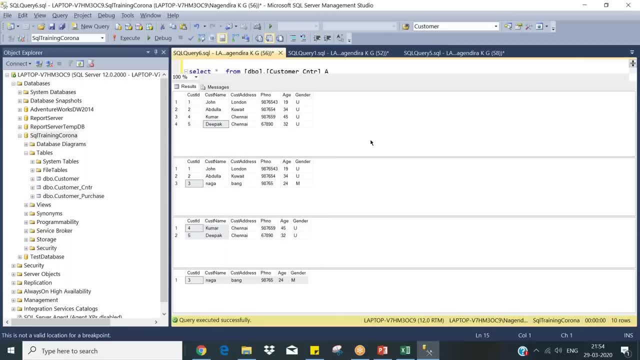 Union and except that is something like: so it's like a set operation. as you already understand, about set operation, you have a circle here, you have a circle over here. then, in between, what is a common factor? in between same thing or whatever, we have a set operation. that is what it's happening. 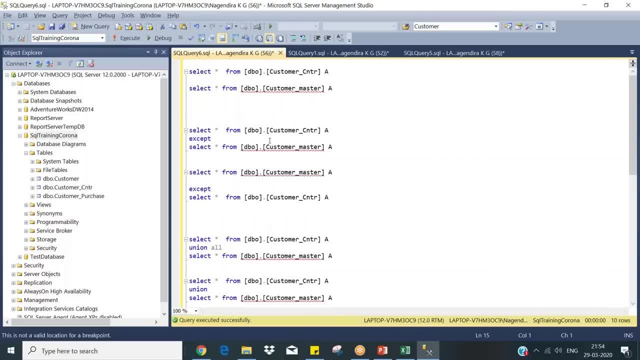 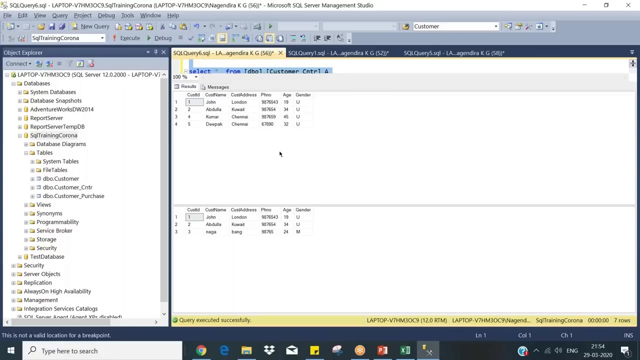 in a scale how you approach it in table level. now, final thing is like: intersect, intersect. any guesses you what it will do? without I will not execute. intersect what is intersect will do? hello, I'm asking because you guys are watching, are you guys are listening or not? so intersect, any idea guys? 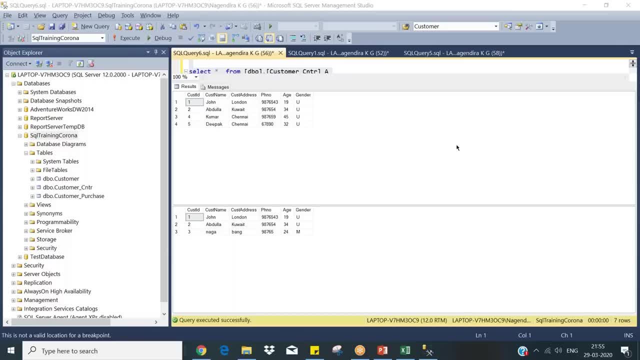 no, I don't no idea. you can do that. we can do it here. as to if we did it as I was asked, yes and I think okay. so hold, we need to find somehow. we need to find a common item, what we need, if you may, to meal objects, and this doesn't really go the same you are expecting, so for a for people who? 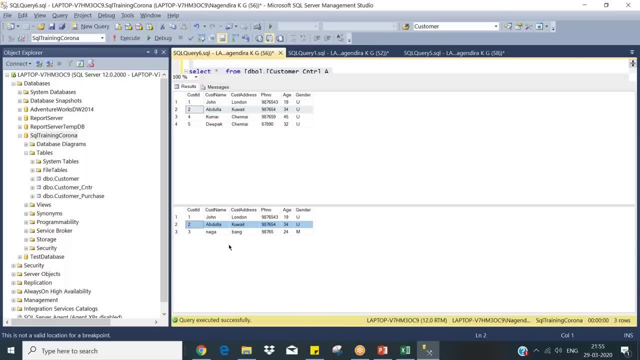 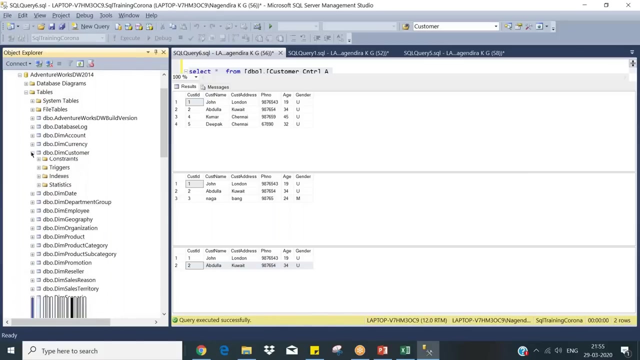 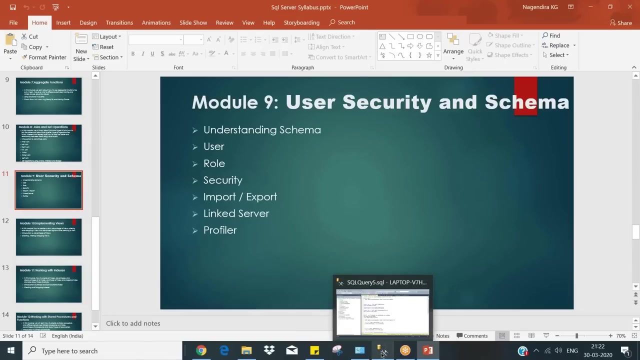 do not necessarily stare at something that is weird like this and do not be- and we need to- about in a few moments. you can just do that. okay, ever before, okay, okay, okay. So the one and two is your result. Okay, This is your intersect, Okay, So let us spot sometime. 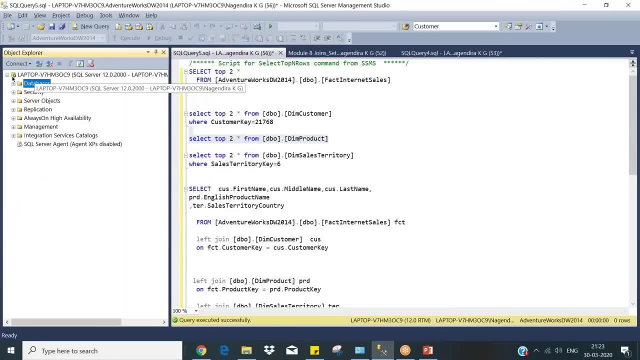 querying. Let us focus on some security aspects of it. Okay, Now, that is something like always. if we see here, this is table, What about this? guys? We have something like before that some object is there, some reference is there. This is nothing but a schema. So schema definition is like: 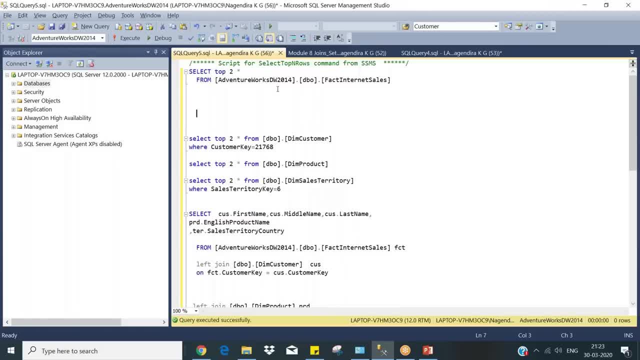 it's like container or a grouping of objects. Okay, So you create a schema. say, for example, you create a database for a college and your college has multiple departments and you want to store attendance for each department separately, or you want to categorize. 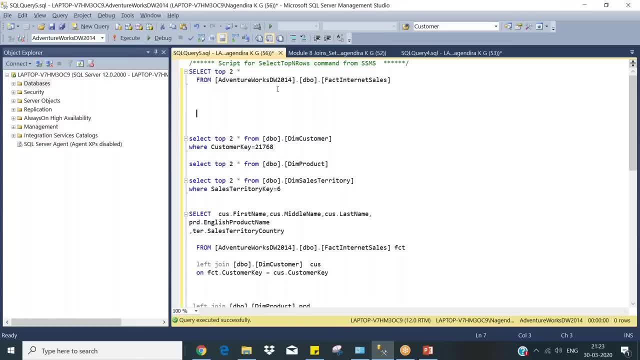 database tables based on the departments. So you create schema for each department And you will add three tables in one department or schema. You add 10 tables in another department or schema based on the organization structure. Okay, You will segregate the groups underneath. 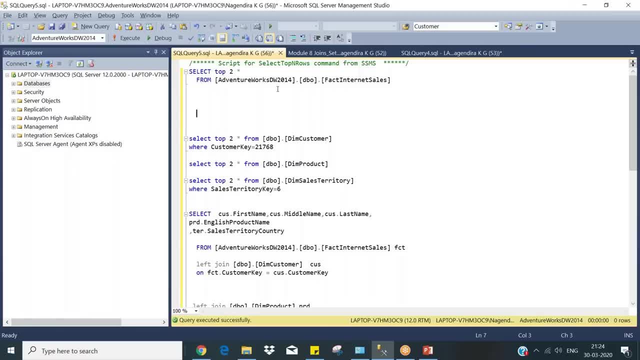 You will create the tables. So that is what a schema is. Schema is nothing, but you are acting as a container to refer the tables. So how to create it? So it comes under security. No, it comes under database schema. Yes, So under the database you have. this is your database security and schemas. 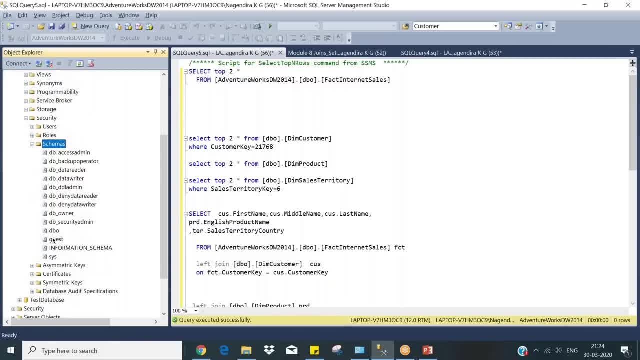 if you see here, by default you have these many schemas. Okay, DBO, So all objects you few, and on the one hand is the schema and schemas and on the other hand is the interface. So you can, can ask me. so always, I should have a schema. yes, by default. if you are not. 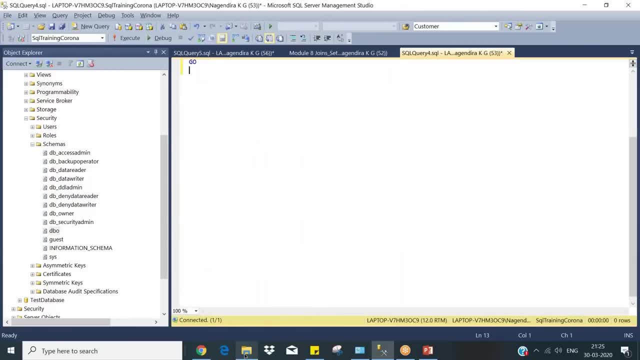 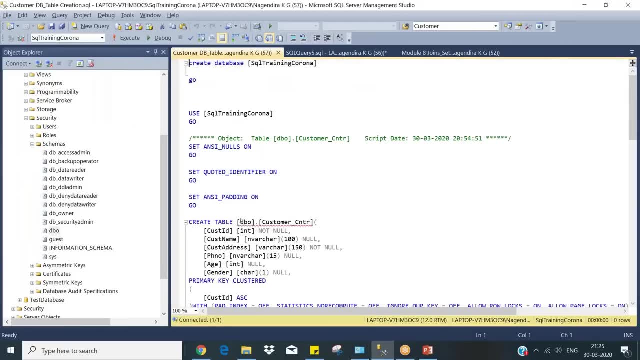 specifying a schema. if you see our earlier examples of creation of scripts, just now created some DB table scripts so we didn't specify anything like this. okay, now I have saved from the database. even if you are not specifying all the tables, by default it will go and sit in your schema. so always it follows. 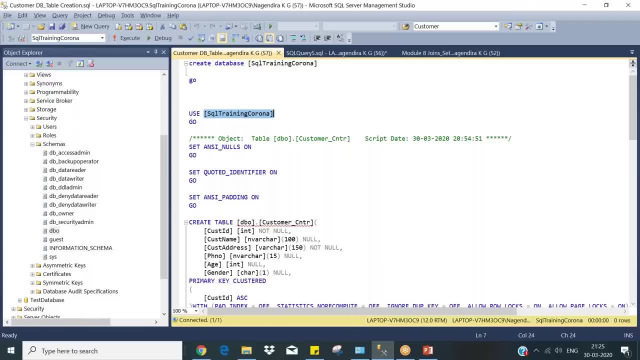 three naming convention. one is your database name. if, if you want to refer your table, you need to refer using three naming convention. that is your database name, schema and table name. okay, this is the order now how to create your user defined schemas. so if you are not specifying schema, then it will show in. 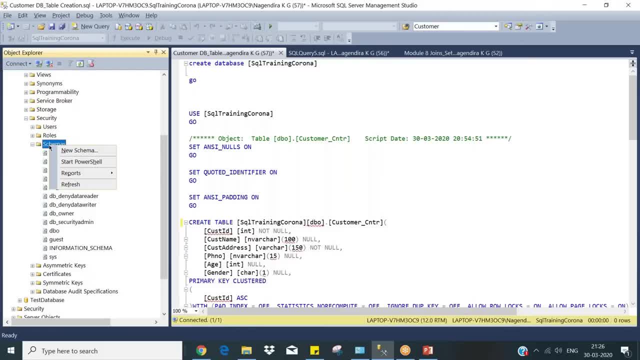 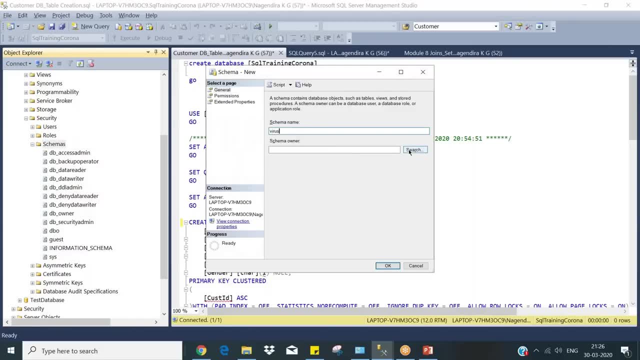 DBO and you can create your own schema. you can create your own schema. and you can create your own schema. and you can create your own schema and you can say, for example, this is Corona, I will create. say, for example, this is Corona, I will create. say, for example, this is Corona, I will create a schema as virus. okay, schema owner. 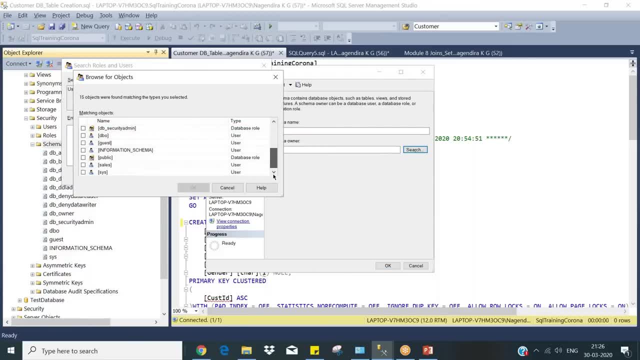 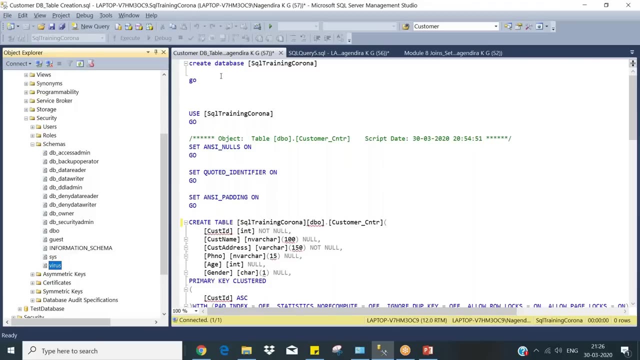 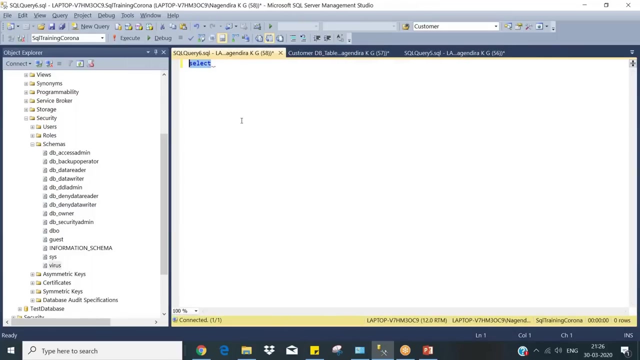 not sure whom to add. let us have the security admin of war, okay. so I have a schema called virus. okay, if we want to create a schema called virus. okay, if we want to create a schema called virus. okay, if we want to create a table and this create table virus, that customer. so 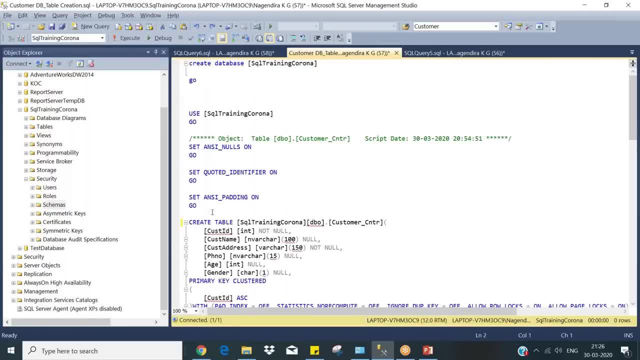 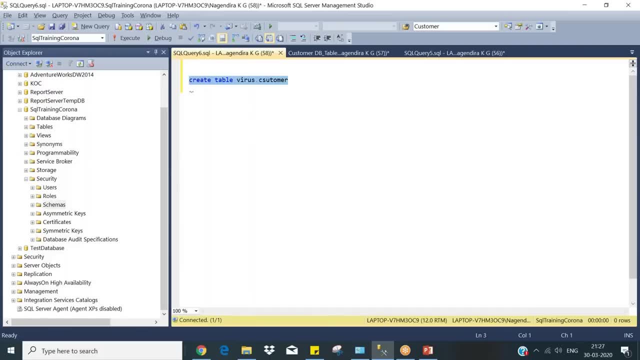 table virus that customer. so table virus that customer. so here you already have a script, right, I can take. here you already have a script, right, I can take. here you already have a script, right, I can take the same script, the same script, the same script instead of DBO. I can create it like in another schema, so you can have a same. 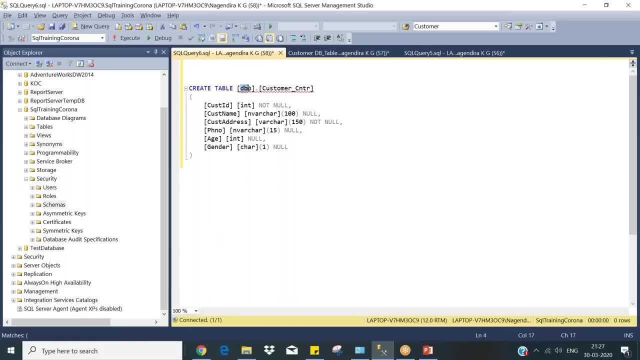 instead of DBO. I can create it like in another schema, so you can have a same instead of DBO. I can create it like in another schema, so you can have a same table name. okay, why is okay, let me run this one so. table name: okay. why is okay, let me run this one so. 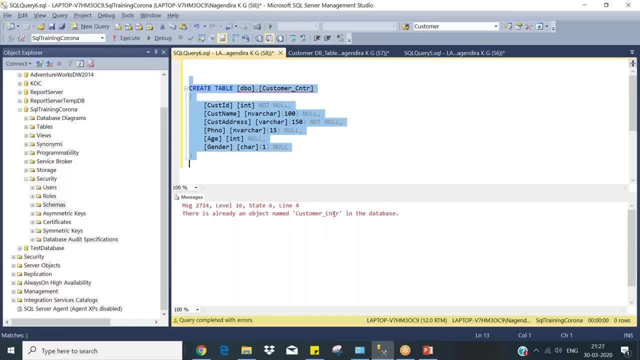 table name. okay, why is okay, let me run this one. so when I run this one it will. when I run this one it will. when I run this one, it will say that is already object name. customer say that is already object name. customer say that is already object name. customer control in the database. okay, when you. 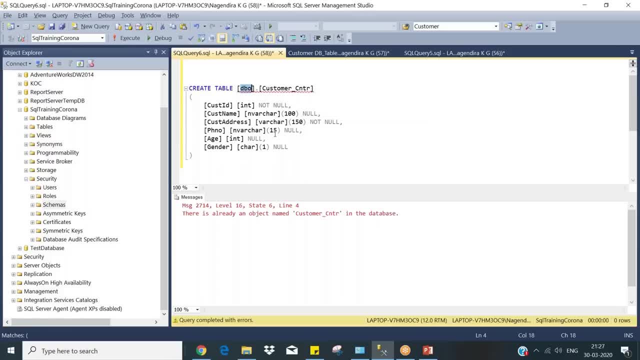 control in the database. okay, when you control in the database. okay, when you have the same object in the same schema. have the same object in the same schema. have the same object in the same schema. it will throw error, but you can create. it will throw error, but you can create. 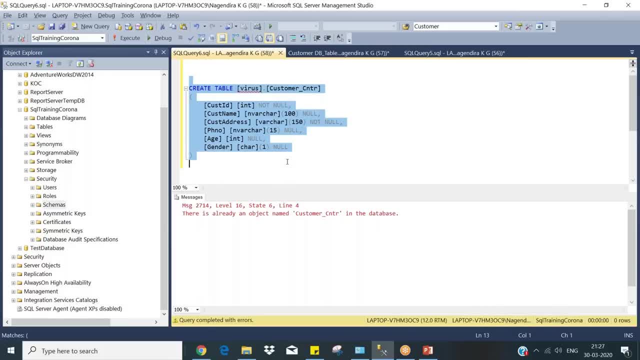 it will throw error, but you can create virus that customer table. I hope you can virus that customer table. I hope you can virus that customer table. I hope you can create courtesy. yes, it does so. if you create courtesy, yes, it does so. if you create courtesy, yes, it does so. if you see here in the tables, now go and check. 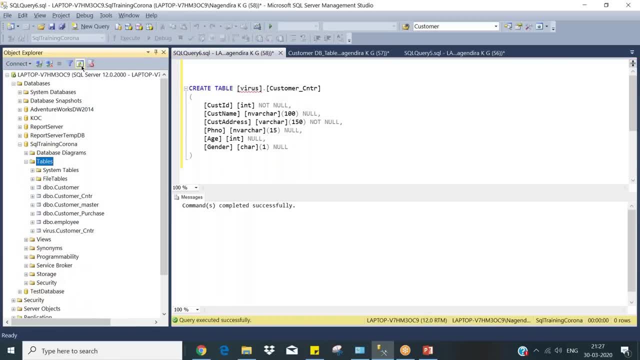 see here in the tables: now go and check. see here in the tables: now go and check it here. refresh it, so DBO, our customer, it here. refresh it so DBO, our customer, it here. refresh it so DBO, our customer, DBO, DBO, DBO. now I have created another. 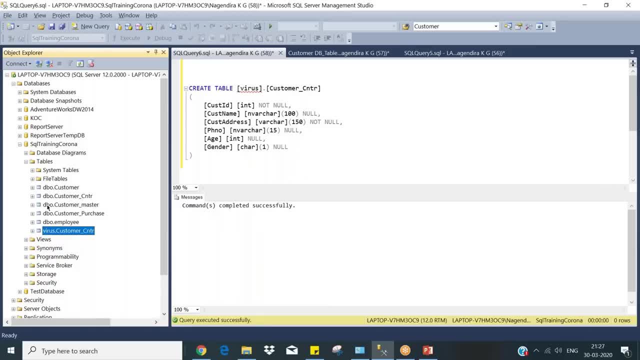 DBO, DBO, DBO. now I have created another DBO, DBO, DBO. now I have created another schema: customer that customer constraint schema. customer that customer constraint schema. customer that customer constraint. with the same name. so, as I said, this can. with the same name. so, as I said, this can. 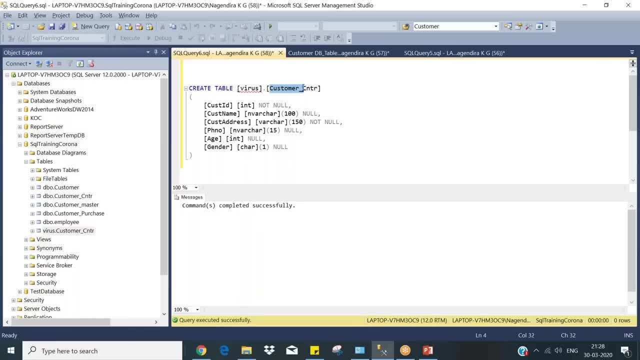 with the same name. so, as I said, this can be one department DBO and virus can be be one department. DBO and virus can be be one department. DBO and virus can be another department customer. I can say another department customer. I can say another department customer. I can say where is that severity? I want to track. 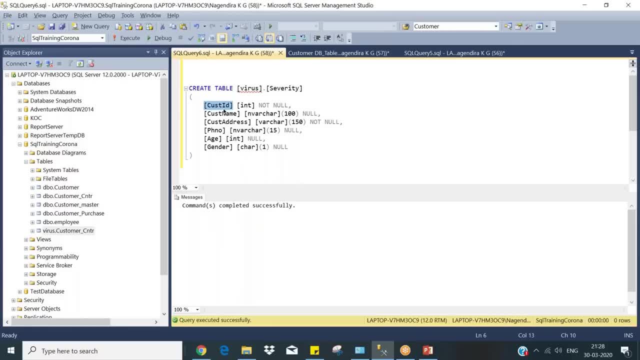 where is that severity I want to track? where is that severity I want to track? why does severity? how many? what is the? why does severity how many? what is the? why does severity? how many? what is the level, or something like that level, level, level, or something like that level level. 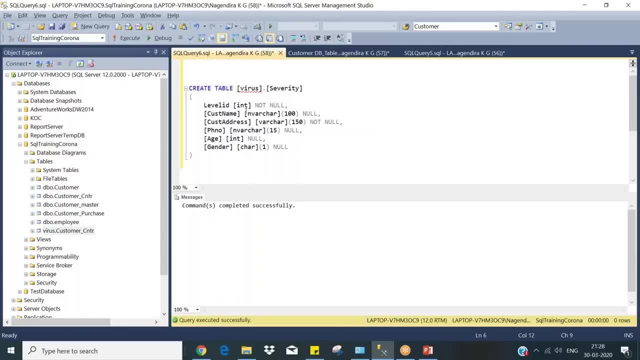 level or something like that. level level, ID level ID is integer. I will say just ID level ID is integer. I will say just ID level ID is integer. I will say just like a level name or stage, like a level name or stage, like a level name or stage or stage. 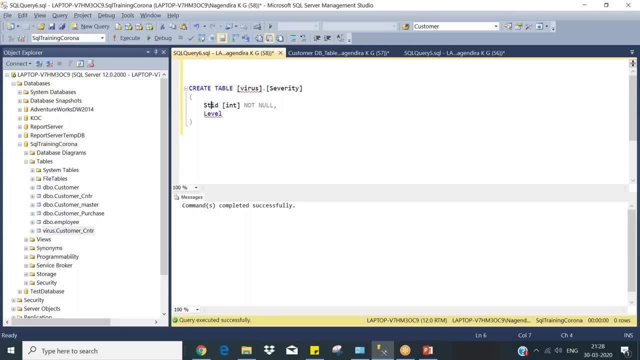 or stage one, stage two. this is, I'll say one, stage two. this is, I'll say one, stage two. this is, I'll say, stage ID stage description. now we are in stage stage ID stage description. now we are in stage stage ID stage description. now we are in stage 2 in India. so like that, I'm saying: 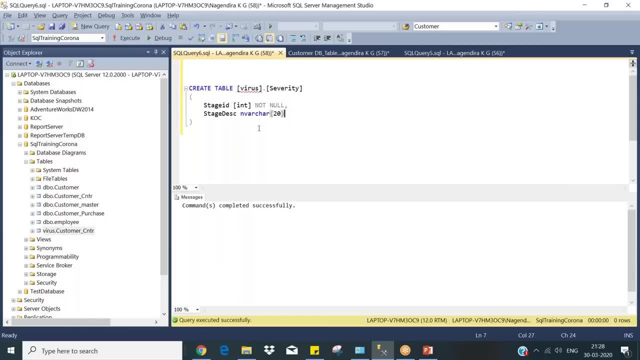 2 in India. so like that, I'm saying 2 in India. so like that, I'm saying so: stage 1, stage 2. what is stage 2 means so stage 1, stage 2. what is stage 2 means so stage 1, stage 2. what is stage 2 means those, say those information I can. 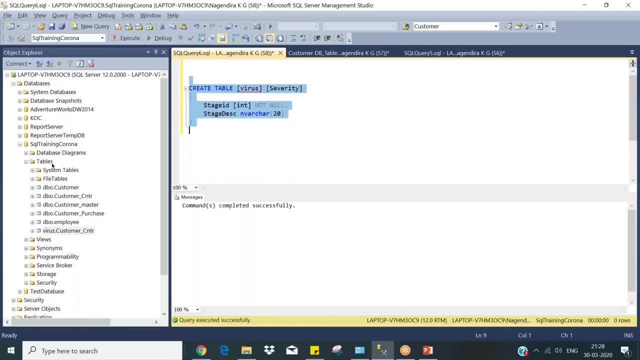 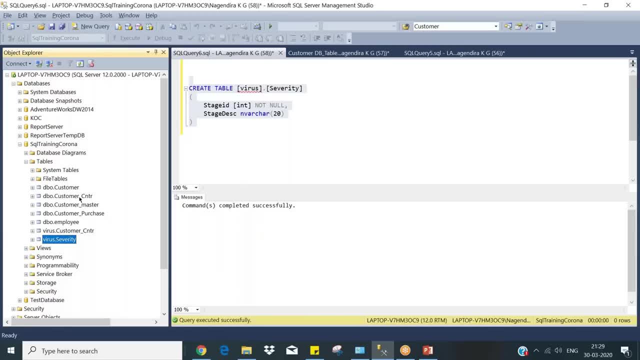 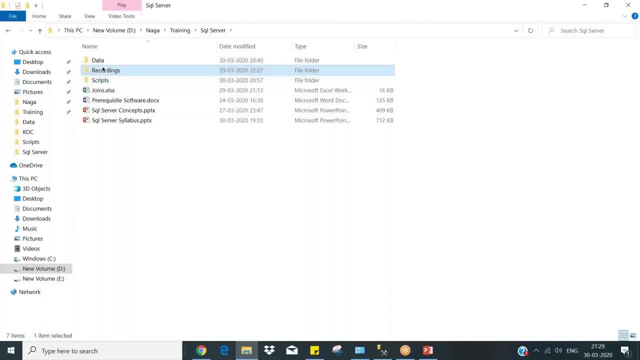 the tables organize matter. similarly, how you maintain in a folders like here I. how you maintain in a folders like here I. how you maintain in a folders like here I maintain. this is my recording, this is my maintain, this is my recording, this is my maintain, this is my recording, this is my data. this is my script under the. 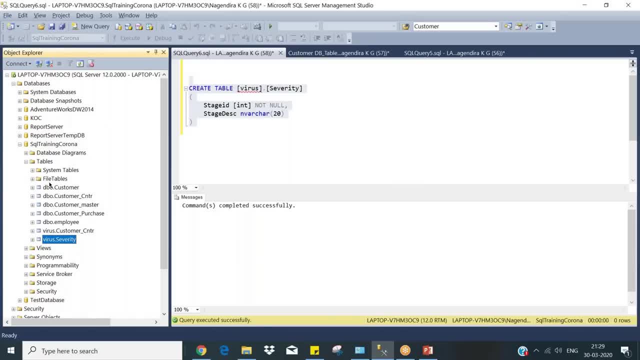 data. this is my script under the data. this is my script under the database. you have tables, but you have database. you have tables, but you have database. you have tables, but you have everything in same schema. you need to everything in same schema. you need to everything in same schema. you need to organize as a folder. so consider you, you. 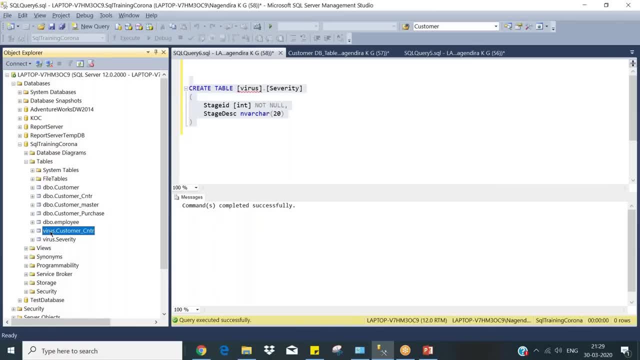 organize as a folder, so consider you. you organize as a folder, so consider you. you can refer it as a folder, or it can be a can refer it as a folder, or it can be a can refer it as a folder, or it can be a group, something like that. okay, so. 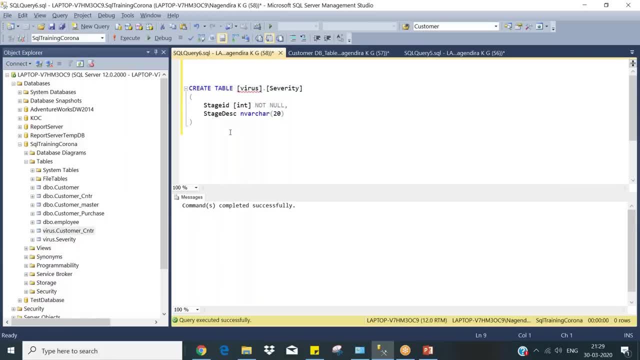 group something like that. okay, so group something like that, okay. so schemas in database perspective. it is a schemas in database perspective. it is a schemas in database perspective. it is a schema. so all other operations same, just schema. so all other operations same, just schema. so all other operations same, just is a schema. okay, you can insert, delete. 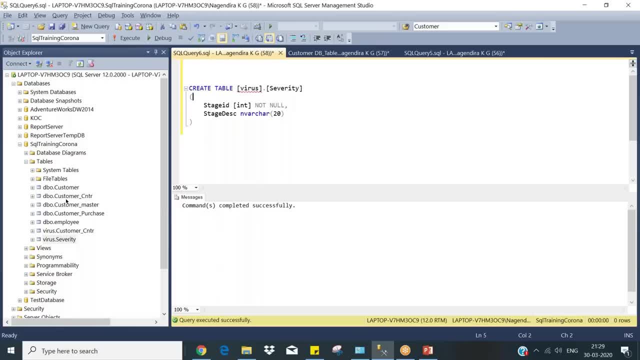 is a schema, okay, you can insert. delete is a schema. okay, you can insert. delete all those things with these schema name, all those things with these schema name, all those things with these schema name. but if you, what happens if I say for? but if you, what happens if I say for? 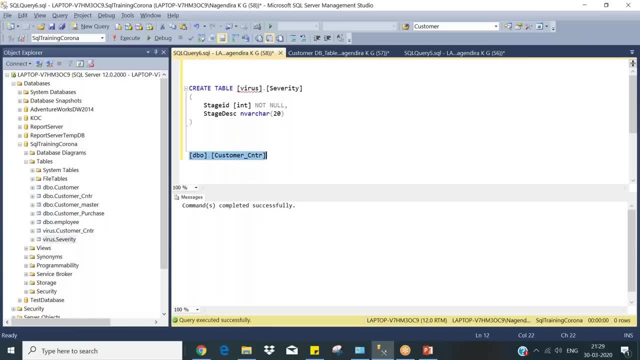 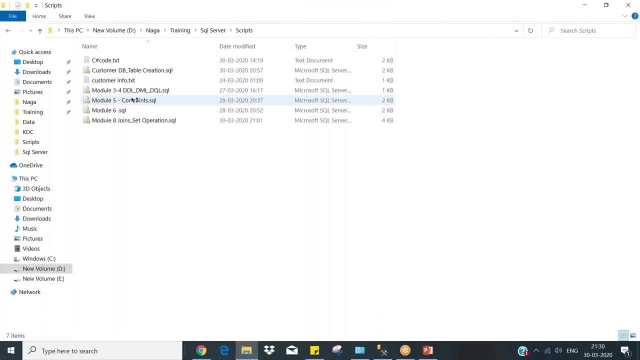 but if you, what happens? if I say, for example, when I try to insert without a example, when I try to insert without a example, when I try to insert without a schema, insert into scripts here. so schema insert into scripts here. so schema insert into scripts here. so without a schema, obviously it will go. 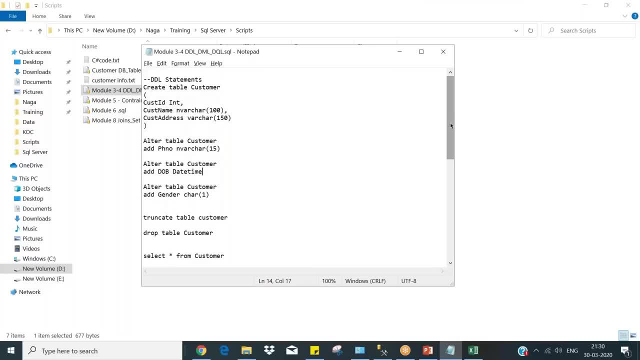 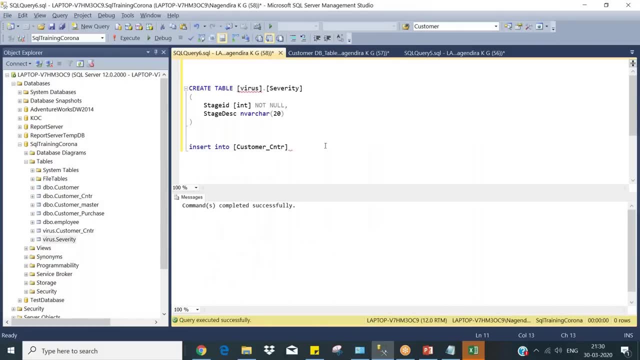 without a schema. obviously it will go without a schema. obviously it will go and insert in your default schema and insert in your default schema and insert in your default schema default data. I don't think it will have a lot of. I don't think it will have a lot of. 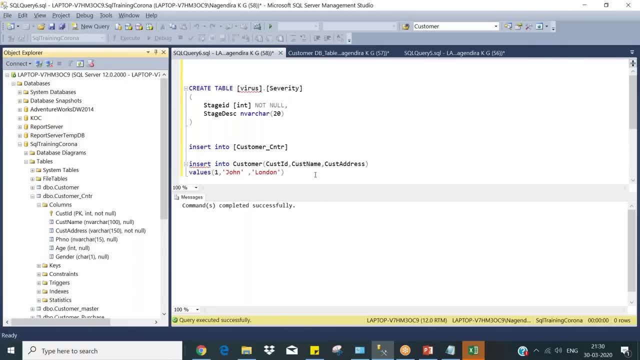 I don't think it will have a lot of numbers we have added already. okay, so I numbers we have added already. okay, so I numbers we have added already. okay, so I can insert it now. I didn't mention the can insert it now. I didn't mention the. 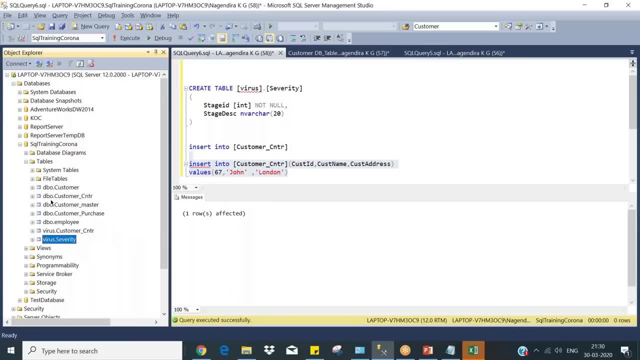 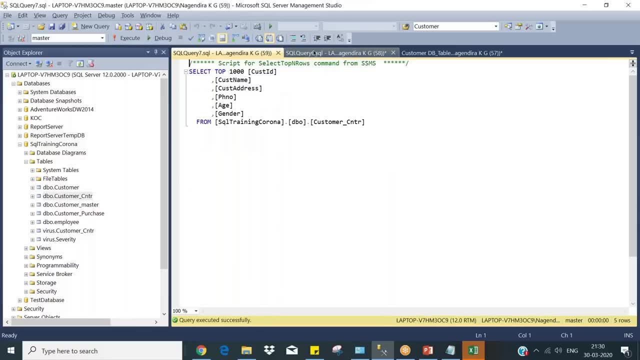 can insert it. now. I didn't mention the schema now which table it got inserted. schema now which table it got inserted. schema now which table it got inserted. it got inserted into this: 67 John London. it got inserted into this 67 John London. it got inserted into this 67 John London. okay, if I want to. 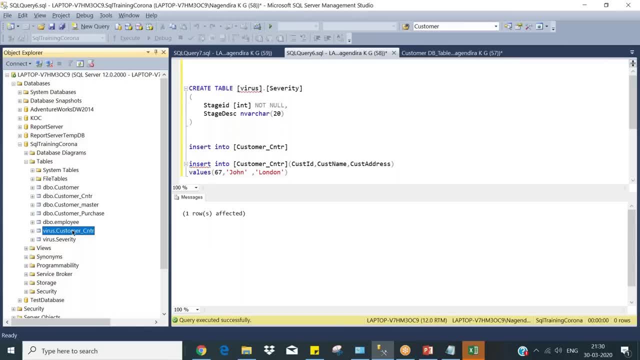 okay if I want to, okay, if I want to mention explicitly in this table: I want mention explicitly in this table. I want mention explicitly in this table I want to insert. now you select the virus table to insert. now you select the virus table to insert. now you select the virus table. there is no entry, I'm going to insert it. 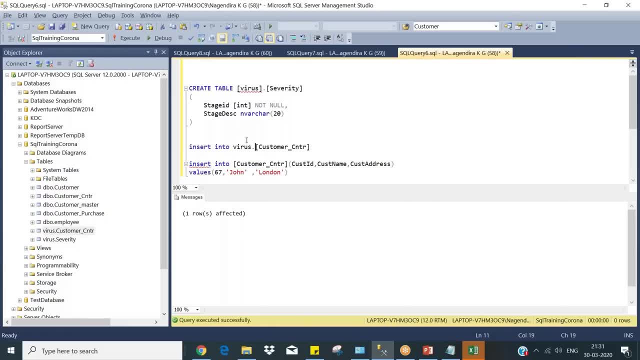 there is no entry, I'm going to insert it. there is no entry. I'm going to insert it now. you need to specify: where is that now? you need to specify: where is that now? you need to specify: where is that? sorry, where is that now? I check the. 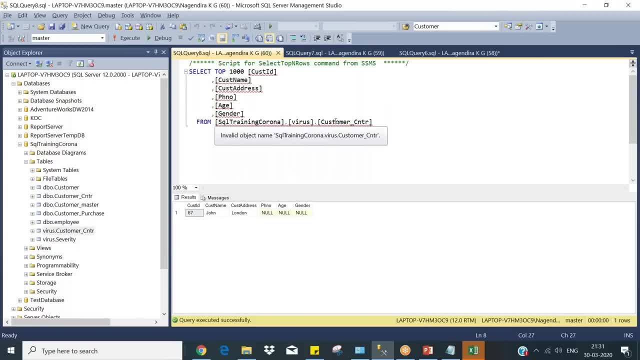 sorry, where is that now? I check the sorry. where is that now? I check the virus table. now you got that entry. so virus table. now you got that entry. so virus table. now you got that entry. so it's same as any other table. it's same as any other table. 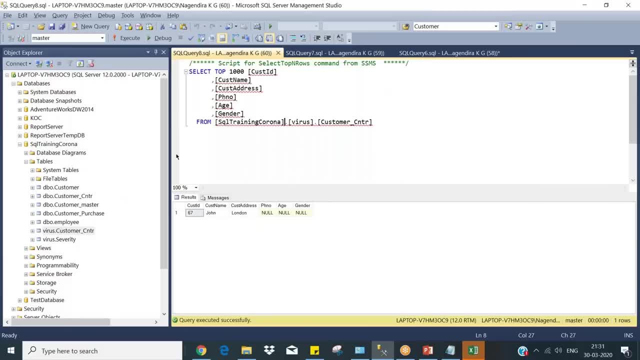 it's same as any other table, so I'm not going to. there is no difference, so I'm not going to. there is no difference, so I'm not going to. there is no difference in if you have a schema in same table. in if you have a schema in same table. 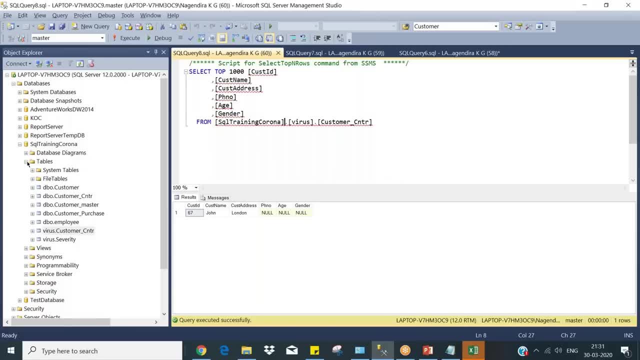 in. if you have a schema in same table, nothing is going to differ. just you need. nothing is going to differ. just you need. nothing is going to differ. just you need to specify the schema name. okay, this is to specify the schema name. okay, this is to specify the schema name. okay, this is one thing I want to tell you now another: 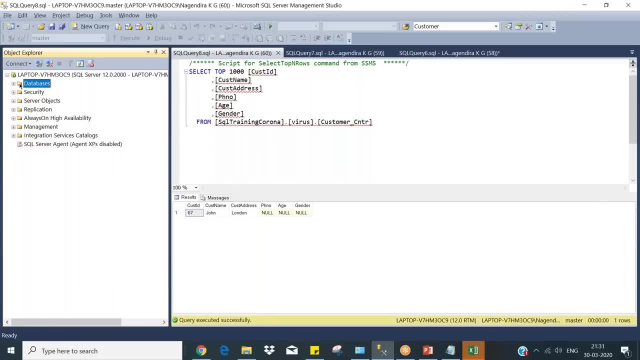 one thing I want to tell you now. another one thing I want to tell you now. another important aspect is like you want to. important aspect is like you want to. important aspect is like you want to secure the tables. I want to give access. secure the tables, I want to give access. 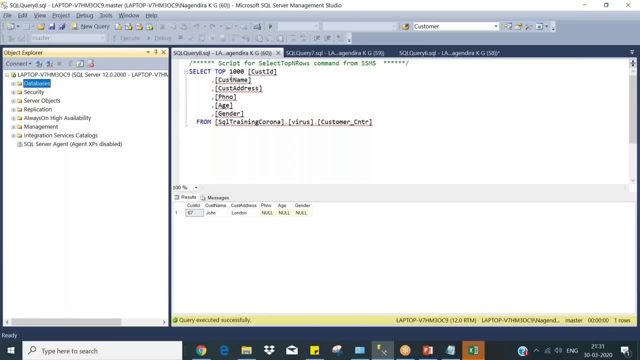 secure the tables I want to give access to only certain people who are logs in, to only certain people who are logs in, to only certain people who are logs in. say, for example, I have to give access. say, for example, I have to give access. say, for example, I have to give access only to certain tables, dim account. 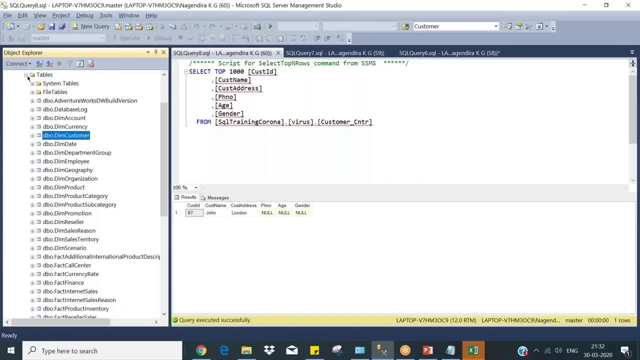 only to certain tables. dim account: only to certain tables. dim account. currency and customers. okay, only these currency and customers. okay, only these currency and customers. okay, only these three tables. I want to give access to three tables. I want to give access to three tables. I want to give access to some users. how to do that? that I need to. 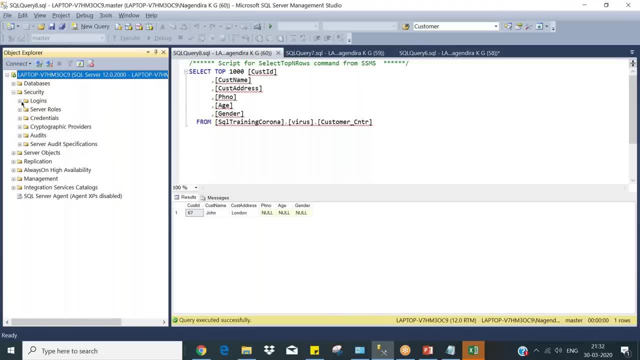 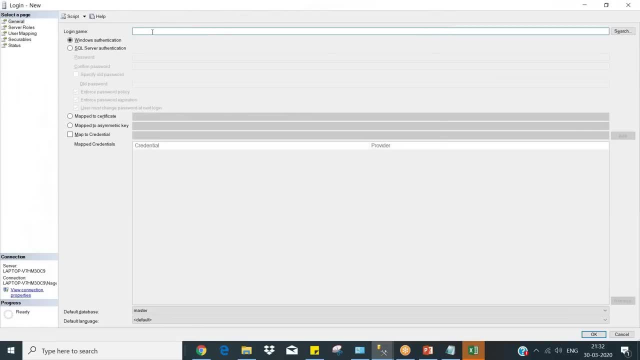 some users how to do that that I need to some users how to do that that I need to have a login created. have a login created. have a login created. okay, okay, okay, okay, so, so, so you log in and he's something like account. you log in and he's something like account. 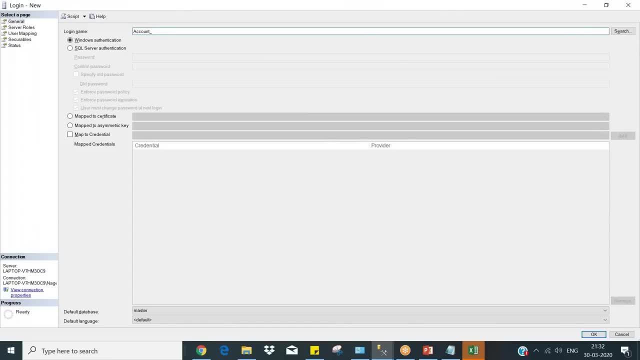 you log in and he's something like account accounts accounts manager: our accounts accounts accounts manager: our accounts accounts accounts manager. our accounts team lead accounts team lead accounts team lead. okay, accounts team lead kind of role. I okay. accounts team lead kind of role. I okay, accounts team lead kind of role I want to give you must SQL authentication. 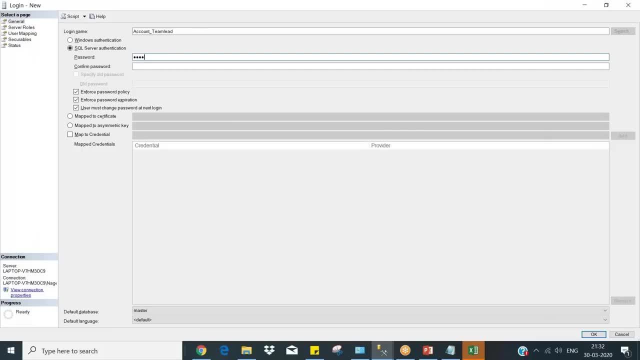 want to give you must SQL authentication. want to give you must SQL authentication? so SQL authentication. I give some so SQL authentication. I give some so SQL authentication. I give some password, password, password, keep it secret. okay, I don't want the keep it secret. okay, I don't want the. 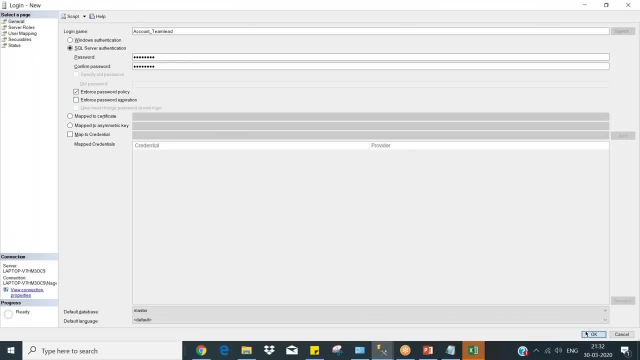 keep it secret. okay, I don't want the password expirations. so just creating a password expirations. so just creating a password expirations. so just creating a login here now. fine account team lead is login here now. fine account team lead is login here now. fine account team lead is your login. so you need to create a login. 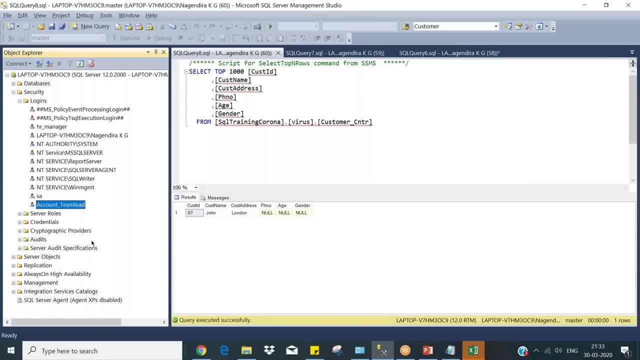 your login, so you need to create a login. your login, so you need to create a login. this is to this. using this account only. this is to this. using this account only. this is to this. using this account only I can login into my server. this is your. 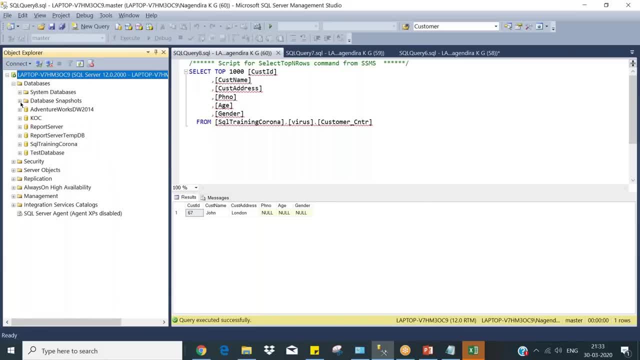 I can login into my server. this is your. I can login into my server. this is your server. okay, now I need to go to database server. okay, now I need to go to database server. okay, now I need to go to database in this database. yeah, I need to create a. 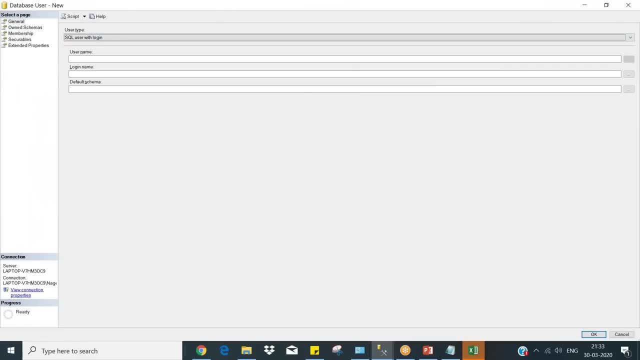 in this database. yeah, I need to create a in this database. yeah, I need to create a user user. user username can be same as login, so a username can be same as login. so a username can be same as login. so a skill user with login. okay, username can. 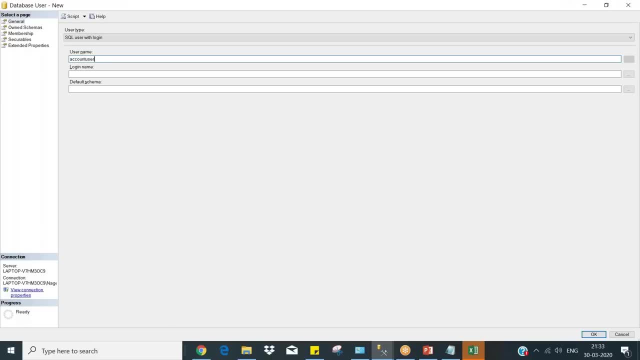 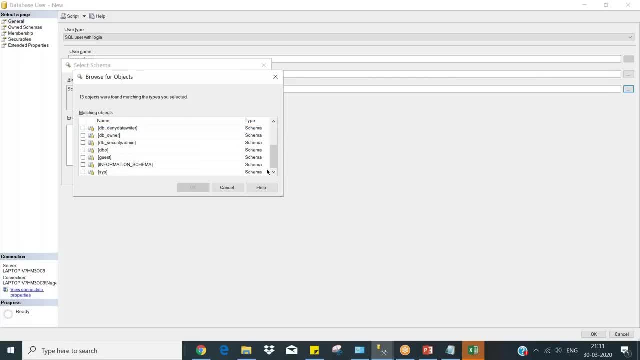 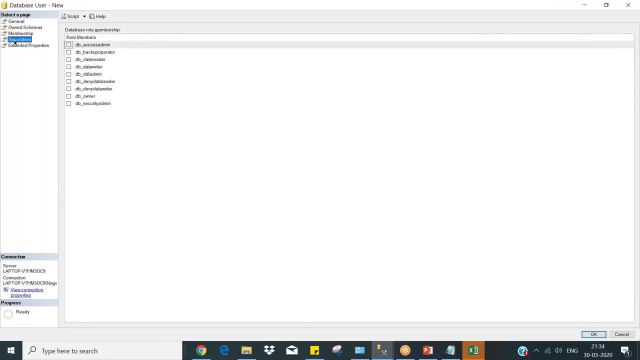 account stimulate okay. and for him, what are account stimulate okay. and for him, what are? the access I want to give hold on no. the access I want to give hold on no. the access I want to give hold on no own schemas is not secure of its okay. 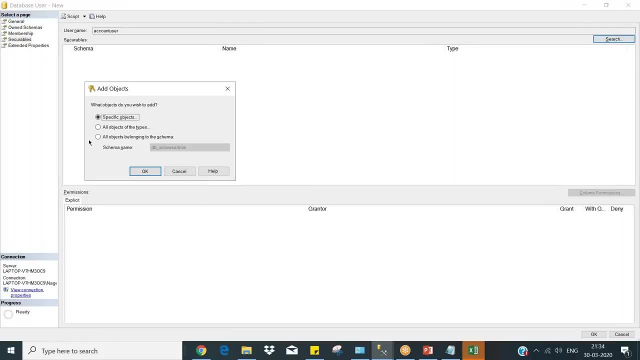 own schemas is not secure of its okay own schemas is not secure of its okay insecure of us. you need to add specific insecure of us. you need to add specific insecure of us. you need to add specific objects. as I said, I want to give those objects. as I said, I want to give those. 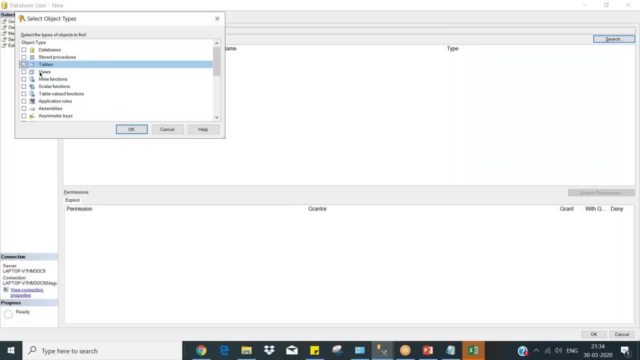 objects. as I said, I want to give those objects only tables, objects only tables, tables only tables. objects, only tables, tables, only tables. you can give any of them only three. you can give any of them only three. you can give any of them only three. tables are used, whatever you want to give. 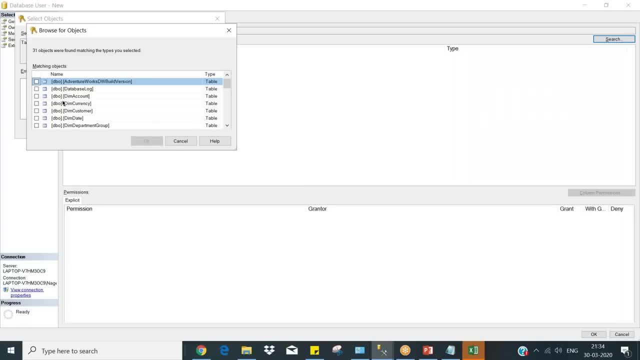 tables are used whatever you want to give. tables are used whatever you want to give. so you choose tables, then browse as I. so you choose tables, then browse as I. so you choose tables, then browse as I said I want to give, say, for example, three. said I want to give, say, for example, three. 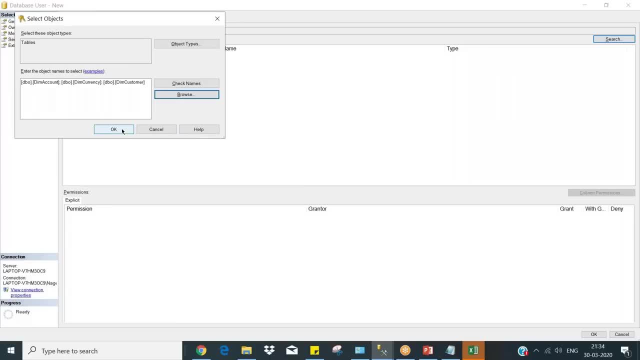 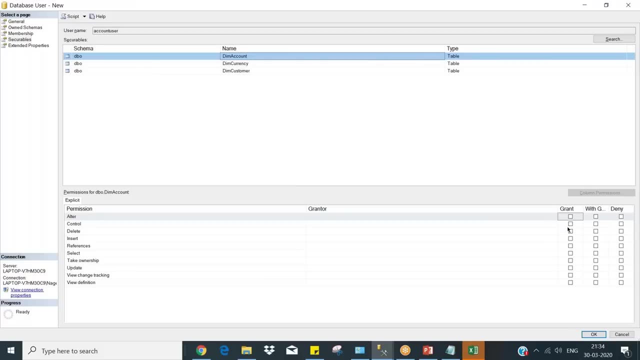 said I want to give, say, for example, three tables, three tables. and then press ok, tables, three tables. and then press ok, tables, three tables. and then press ok, then what access you want, I want to. then what access you want. I want to. then what access you want. I want to select access, I want only select, okay. 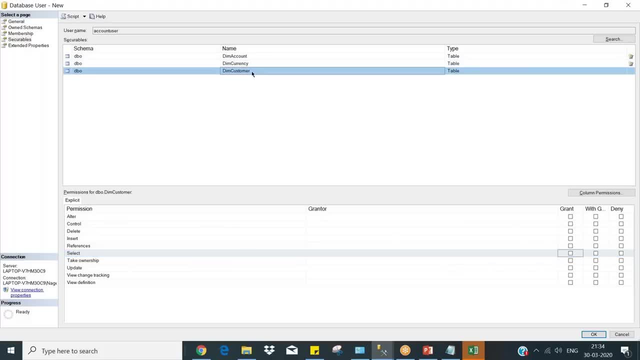 select access. I want only select. okay, select access. I want only select. okay, let us see, only select these three. let us see, only select these three. let us see, only select these three tables. I'm giving only select, that's tables. I'm giving only select that's. 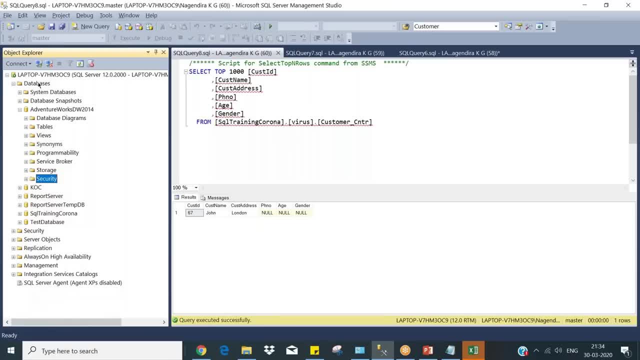 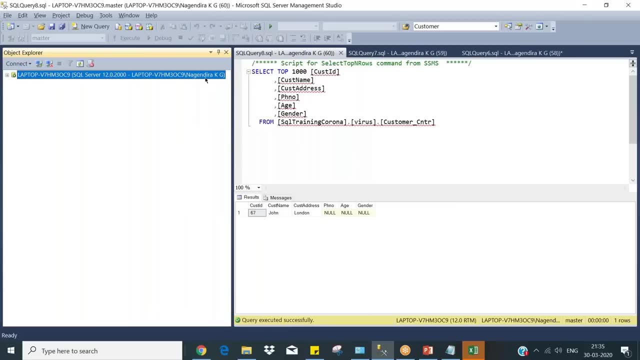 tables. I'm giving only select, that's all okay. all okay, all okay, I can't use it. let us login using see. I can't use it. let us login using see. I can't use it. let us login using see. this login is using my admin access. I'm 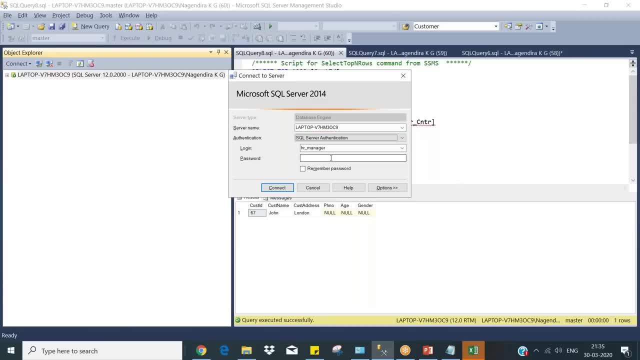 this login is using my admin access. I'm. this login is using my admin access. I'm going to connect using the. the newly going to connect using the. the newly going to connect using the. the newly created login. that is account created login. that is account created login. that is account underscore. team lead: team leader team. 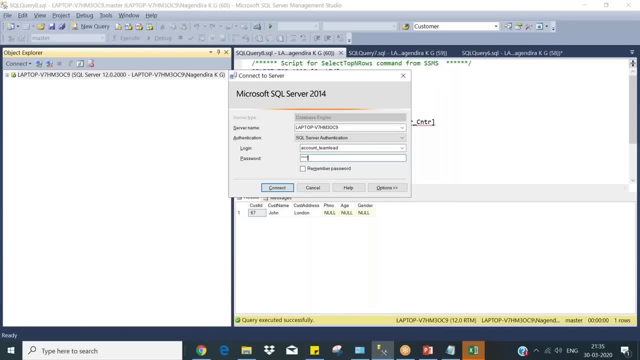 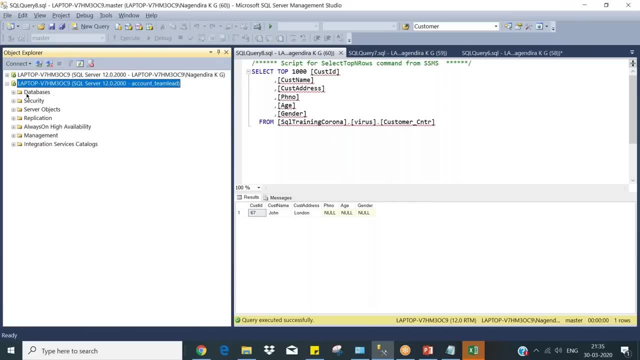 underscore: team lead team leader- team underscore- team lead team leader- team leader. I forgot the name. let us see good leader. I forgot the name. let us see good leader. I forgot the name. let us see good. so here's the login logged in: now you. so here's the login logged in: now you. 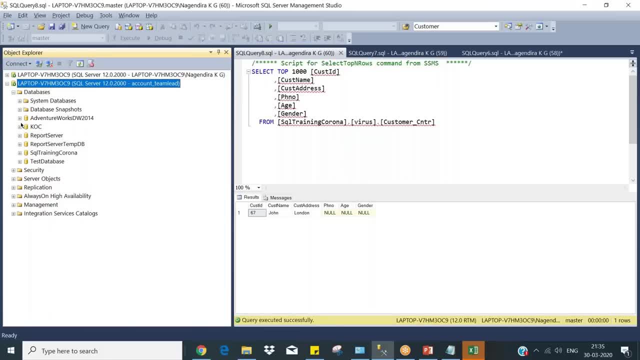 so here's the login logged in now. you can see: you can still see the database. can see. you can still see the database. can see, you can still see the database. I need to fix that one now, but when I? I need to fix that one now, but when I. 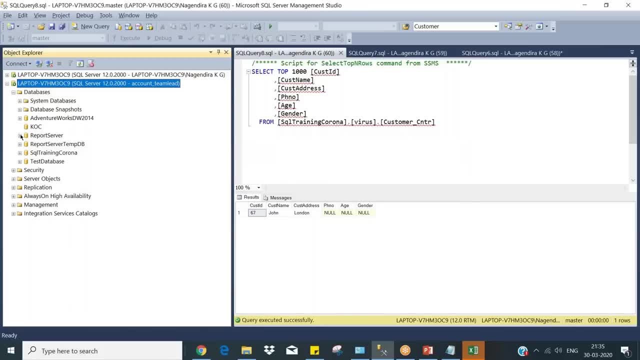 I need to fix that one now. but when I try to expand the other database, it try to expand the other database. it try to expand the other database. it doesn't have access. it tries to expand- doesn't have access. it tries to expand- doesn't have access. it tries to expand it. the account team lead: okay, but when? 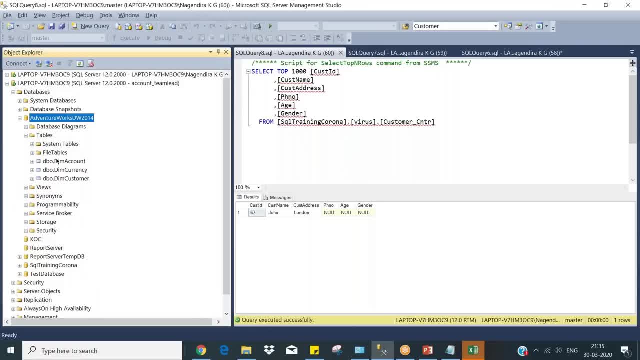 it the account team lead, okay. but when it the account team lead, okay. but when he tries to expand this one, I have given he tries to expand this one, I have given. he tries to expand this one, I have given the rights he can see only that these. 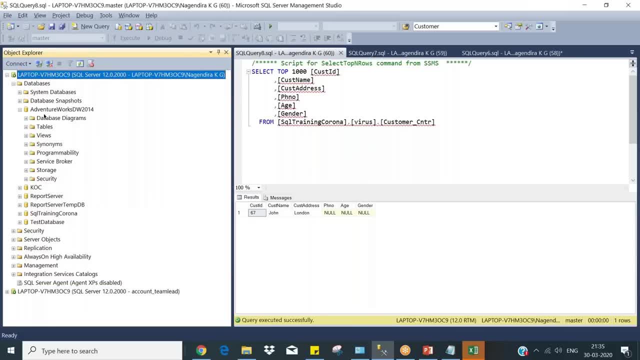 the rights. he can see only that. these the rights. he can see only that. these three tables. this account is my admin. three tables. this account is my admin. three tables. this account is my admin account. I can see all the tables in this account. I can see all the tables in this. 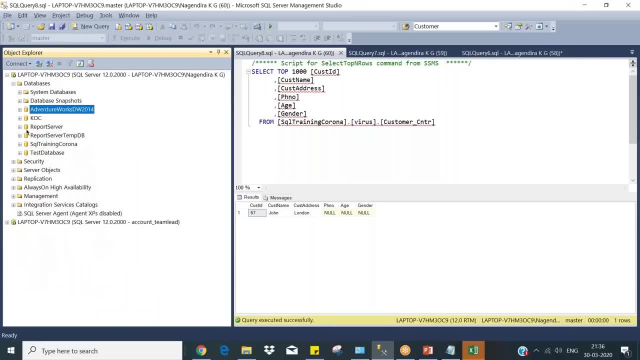 account. I can see all the tables in this adventure works. but using this I mean adventure works. but using this I mean adventure works. but using this I mean for account team lead. he can see only the for account team lead. he can see only the for account team lead. he can see only the three tables, and even he can 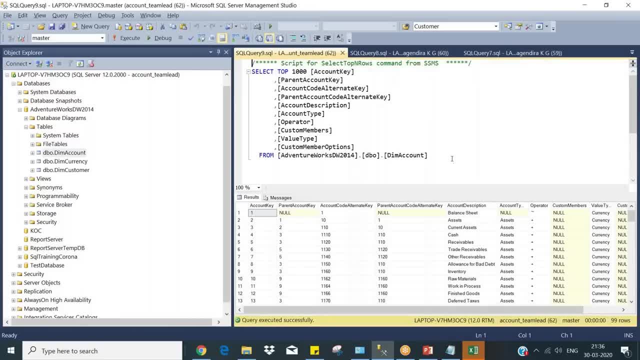 three tables and even he can three tables, and even he can only select the tables. he can select the only select the tables. he can select the only select the tables. he can select the tables when he tries to insert or delete tables. when he tries to insert or delete, 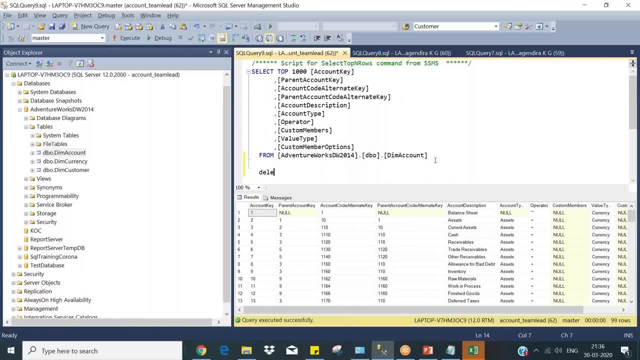 tables. when he tries to insert or delete the record, it will throw him. let us try the record, it will throw him. let us try the record, it will throw him. let us try that. one. delete from dim account. see that one. delete from dim account. see that one. delete from dim account. see, guys, one, you, once you are querying it is. 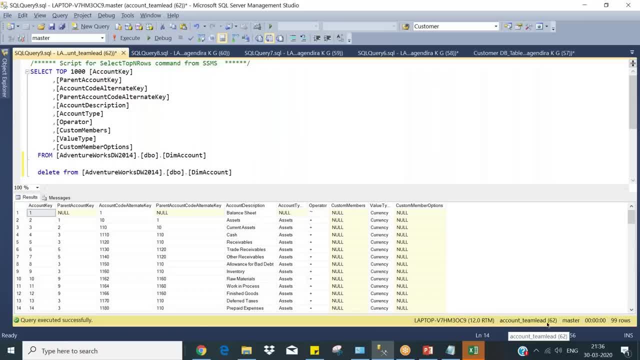 guys one you once you are querying it is guys one you once you are querying it is taking the here. you can see the user taking the here. you can see the user taking the here. you can see the user name: who has executing these queries. name: who has executing these queries? 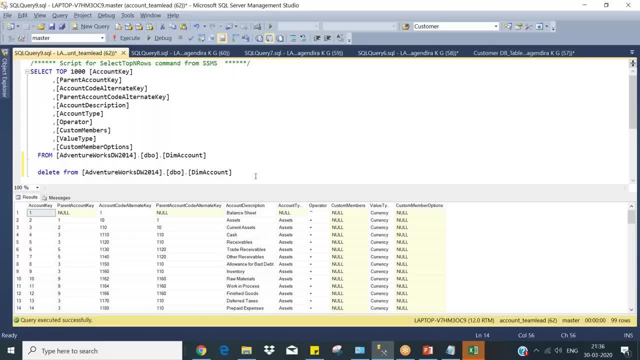 name: who has executing these queries? okay, so those things also is taken into. okay, so those things also is taken into. okay, so those things also is taken into account. it's just not running the query account. it's just not running the query account. it's just not running the query. who is running all those things? so when 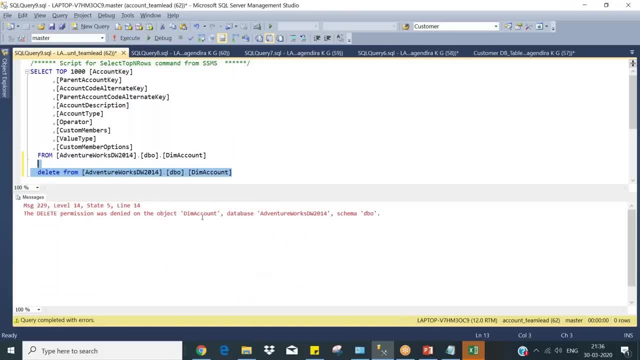 who is running all those things? so when, who is running all those things? so when you try to delete it, delete permission- you try to delete it. delete permission, you try to delete it. delete permission was denied on the object schema- okay, he. was denied on the object schema- okay he. 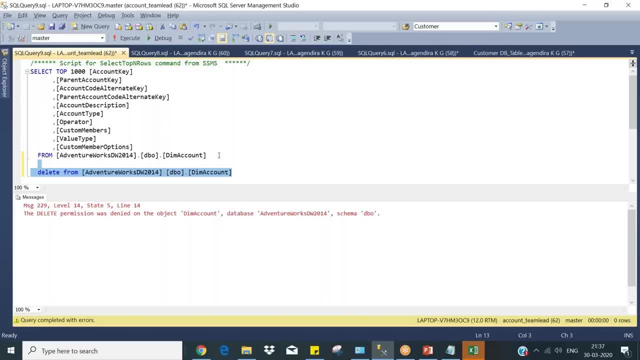 was denied on the object schema. okay, he doesn't have access to delete the doesn't have access to delete the doesn't have access to delete the records. he has only have access to records. he has only have access to records. he has only have access to select the records. so this level of this 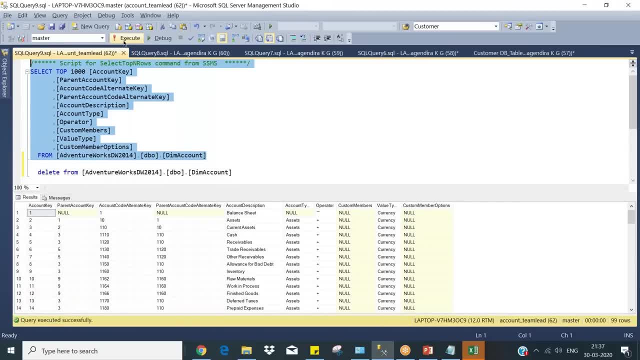 select the records. so this level of this select the records, so this level of this granular level of access control, you granular level of access control, you granular level of access control, you are providing, are providing, are providing so that any banking applications like, so that any banking applications like 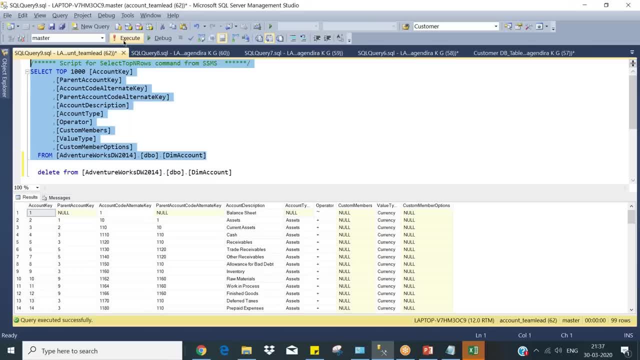 so that any banking applications, like crucial applications correct. so you crucial applications correct. so you crucial applications correct. so you cannot update your balance. someone cannot update your balance. someone cannot update your balance. someone balance. so people will have only access balance. so people will have only access balance. so people will have only access to read. 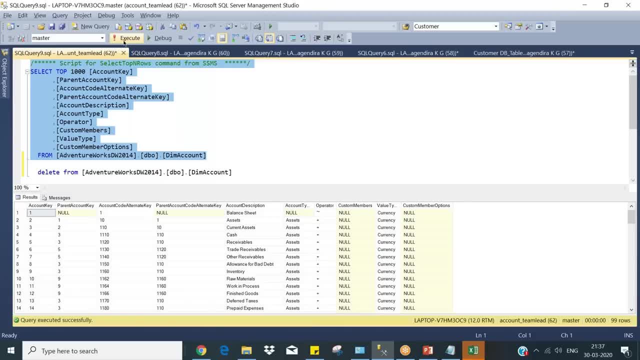 to read, to read. only very crucial people will have access. only very crucial people will have access. only very crucial people will have access to updation, to updation, to updation or correction- sometimes we need to- or correction. sometimes we need to. or correction, sometimes we need to manually correct the name or update the. 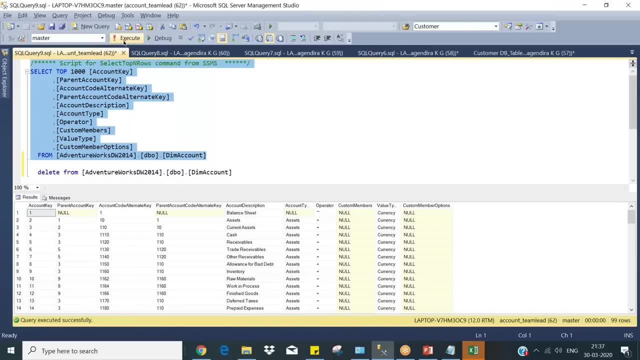 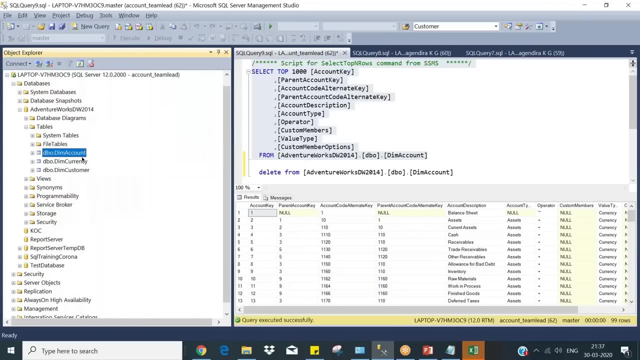 manually correct the name or update the user information. so this is what they implement: the security, so these kind of things. you cannot impose it in a file system earlier conventional file system. this is very important things to consider. okay, i hope i'm clear, guys. so you imagine whatever other roles you can. 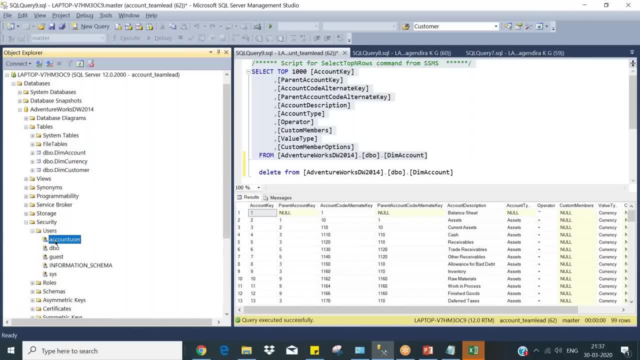 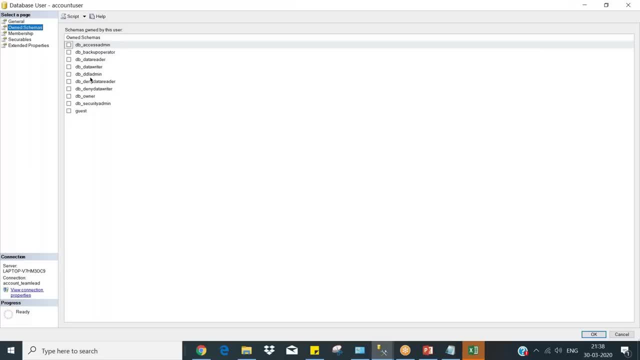 create. let's see that one, like each thing over here, as defined schemas, has its own. i mean to say ddl use. we saw about ddl right. so if you give ddl admin, he can able to create the tables, he can able to alter the column definition, those kind of roles. so these roles are predefined by 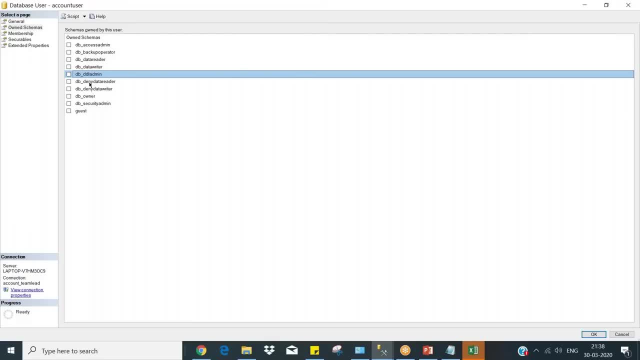 sql server. so some like uh deny data reader or deny data writer, so you cannot insert or update. right means it's not only insert, insert, update. so these are different access or roles already created by uh sql server. db owner means he has access to all. i mean db owner can create or modify all the sql uh task he can do. 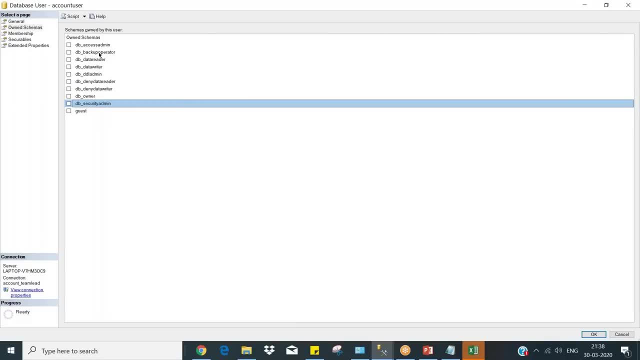 but he is not a system admin, security admin. there are certain things even i'm not sure what are the things. these things are dba activities as a developer, which is good to know. just uh, to highlight some something. if you find like i don't have access, what to do? so you should. 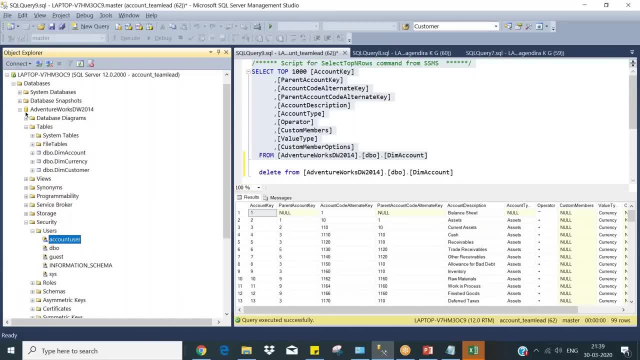 know they have restricted your access. okay, this is about schemas, users and security. so i hope you guys know about your roles. roles are nothing but again, a group you give some roles of. i mean in you create a role and same security. whatever security restrictions you want to have, you give it for. 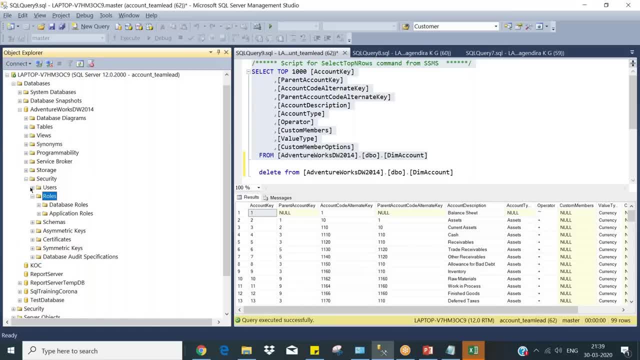 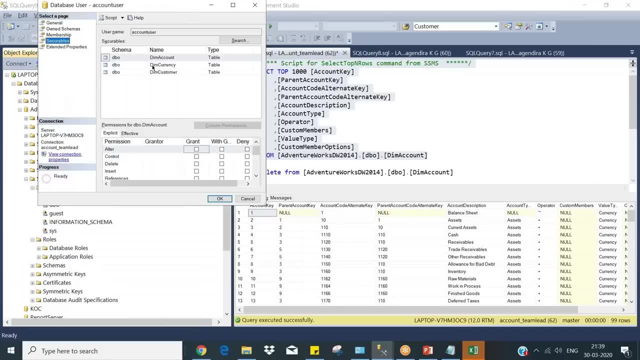 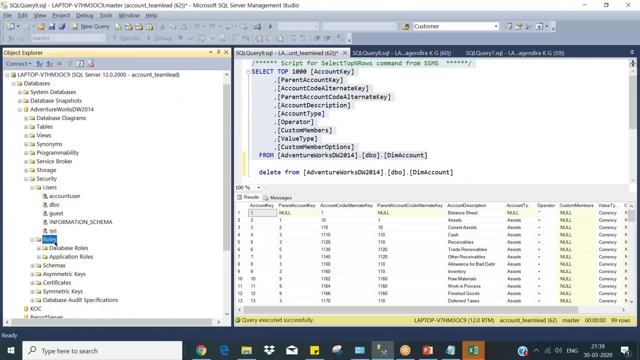 role, then you map those users, because if you create a user for each user, you need to give this security restriction, this table, this table instead, if you create a role, you can give whatever access objects you need to provide it in a role. just map 10 users into that role. it's again like a grouping. 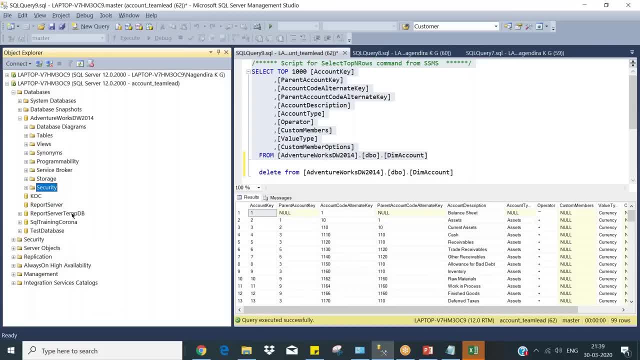 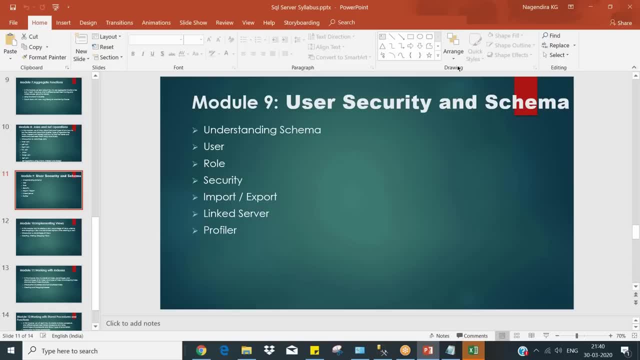 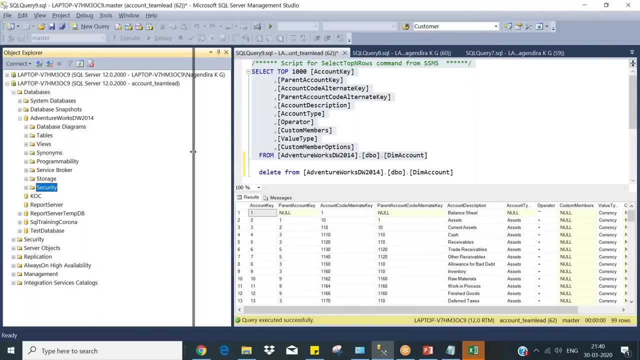 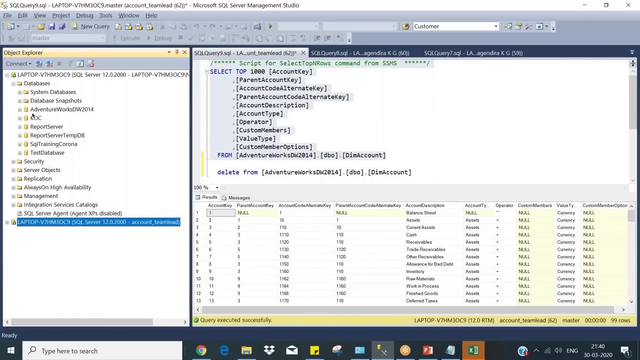 role based security. okay, so with this note, then, what i want to cover is import, export. when we start the session, someone asked me whether we can import data from excel into database. yes, we can do. that is what i'm going to show, but for now, what i'm trying to do is like, uh, there is. 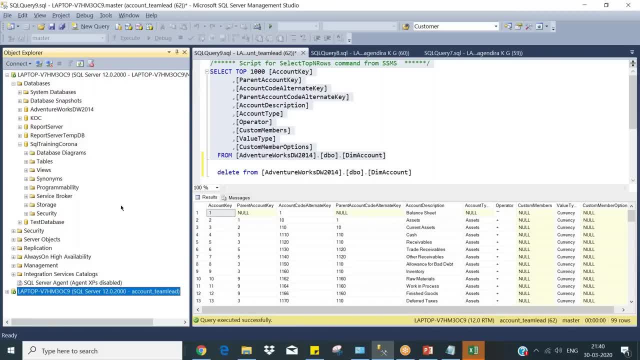 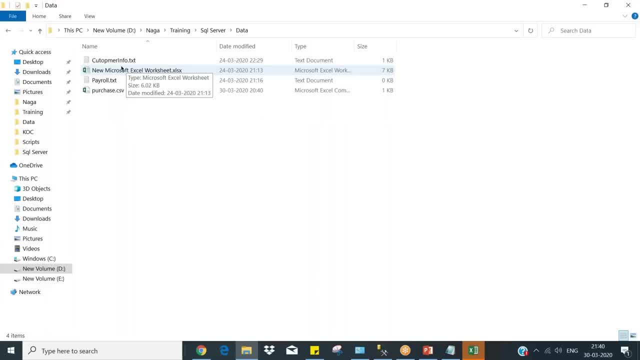 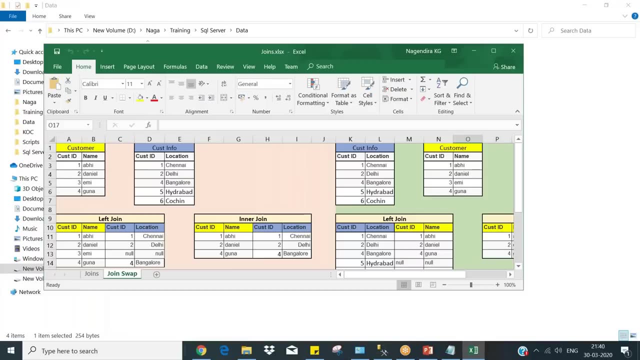 a issue in excel. so i'm going to show you what i'm trying to do is like: uh, there is a issue in excel importing an excel in my laptop. for time being i will import- um, no dot csv file. so i've created already a purchase csv file here. let us have a look. it is nothing but our customer purchase table. 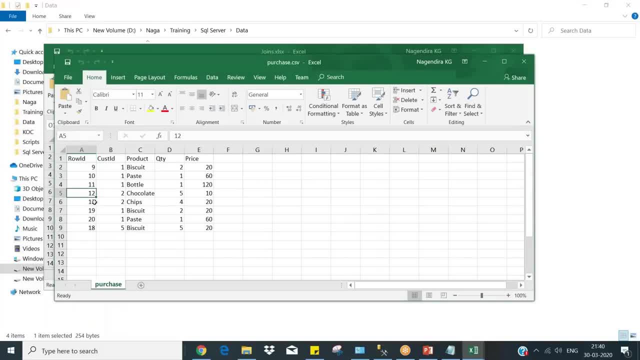 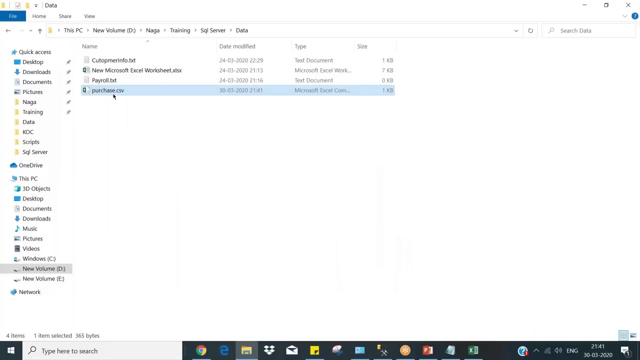 only so same thing. maybe i will replicate some data to have a huge records. so this contains um, almost 25 records. okay, 19, 18 records, including the 18 records excluding the header. okay, so this purchase csv file or excel file. if the procedure is same- how to import into a database- it can be. 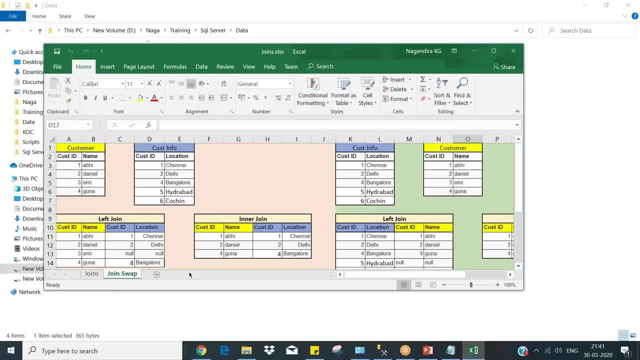 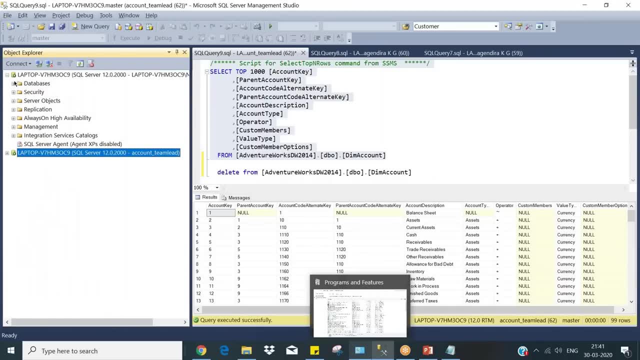 a huge file, 1gb file or whatever can be the thing. it should be in a table format. how to do that? so you have a database. choose where you want to import um. here you already have a customer purchase. let us do it in viruscustomer purchase, okay. so click on the database. right click, okay. right click on the. 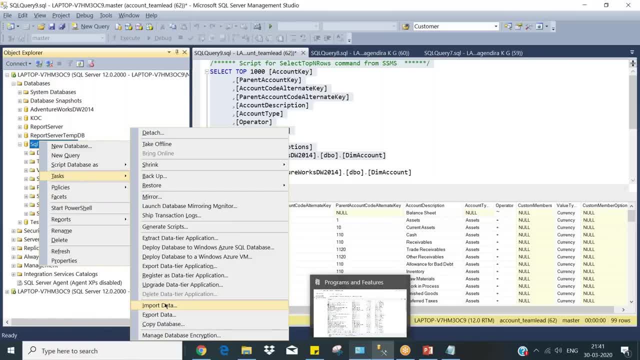 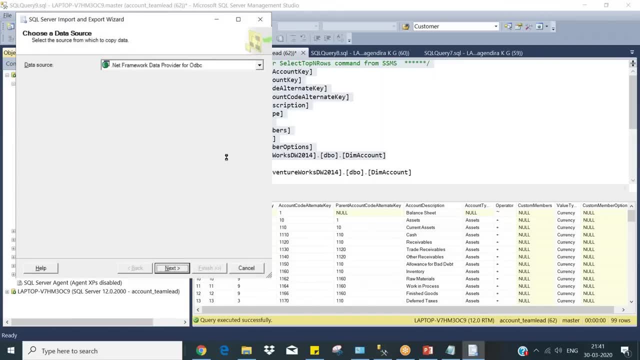 database. you have a task, then import data and click on next. next, everything is uh simple, guys. microsoft has done very good gi for you. you don't need to do any coding, all those steps, just choose, then your job is simple. choose this, guys, and screen server data. 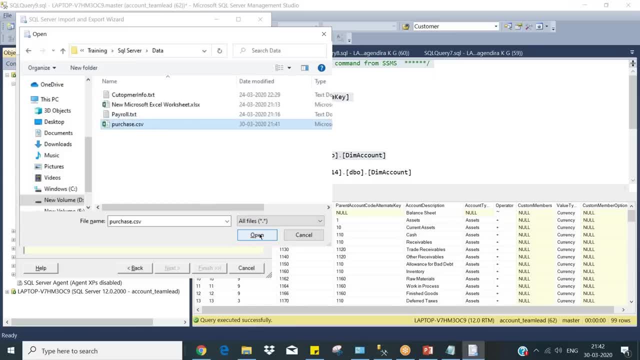 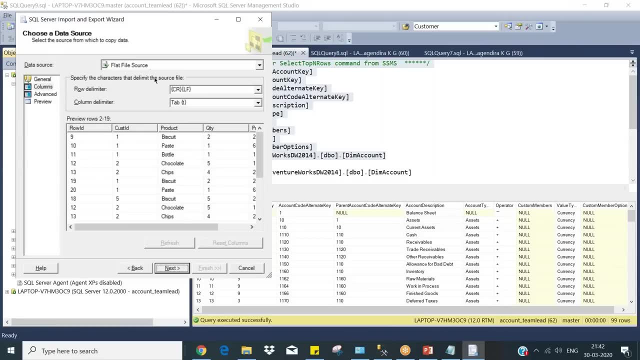 choose all files, purchase just csv. okay, so this is what you have. okay, one single license. now this is your flat file, once you choose that csv it. so you are already understand about the row delimiters and column really Sharp。」. column delimiter: what was there in the csv file is like csv. csv means comma. it will be comma, comma. 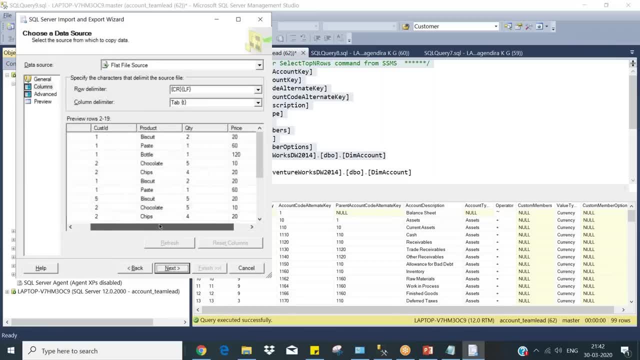 comma separated, so tabs or commas, usually it will take and it has created the new table for you. this is the structure: row id: customer. you remember i copied and pasted multiple times, so 19.. it showed you the preview. okay, so this is your source file, just showing you a preview this. 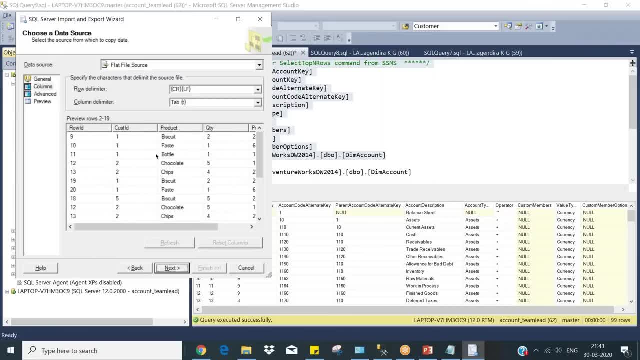 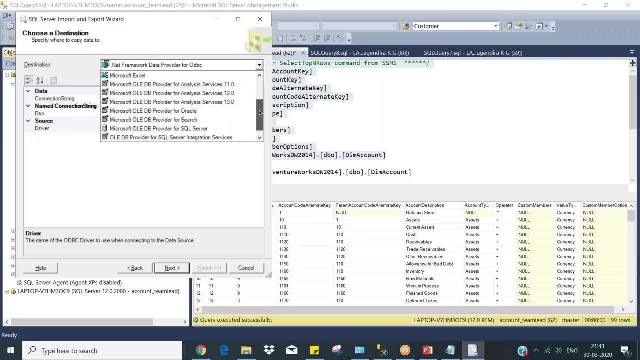 is what you're going to get, because there will be some issues sometimes you need you can fix it. this column might come here, this model might went there, so just ensuring it's correct. now, what is your target? target is my database, microsoft oldb provider for sql server and this is my server name. 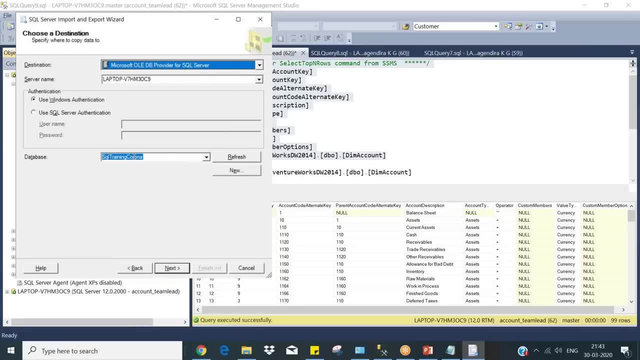 you, i can go for windows authentication, since i choose the database already and right click from there so it is showing me the correct database. then you click on next, so it suggests us some name based on the file name. okay, i don't want this name, just go and. 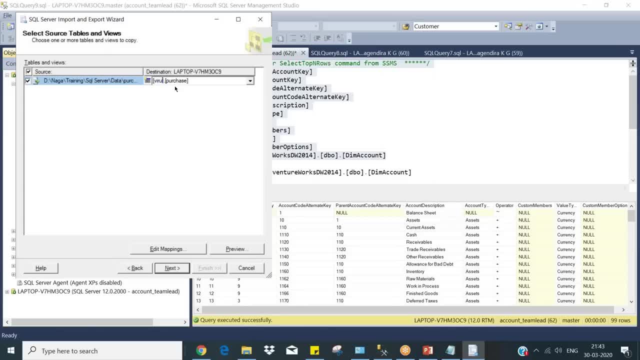 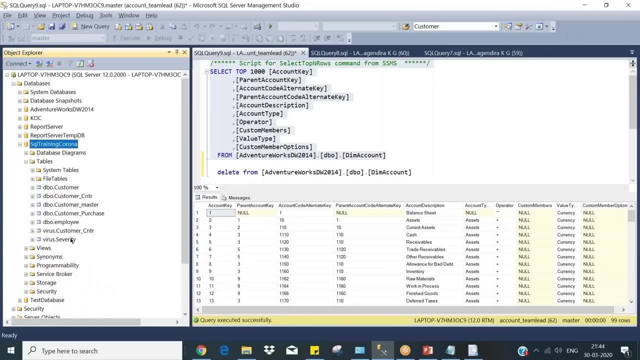 do it in purchase, now virus, or the schema, and purchase, import and name it as input. so now we don't have any tables. you know this point, guys. okay, i mean, uh, what i'm trying to say is here: i don't have any target table. so either you can have a table created by you manually so that you 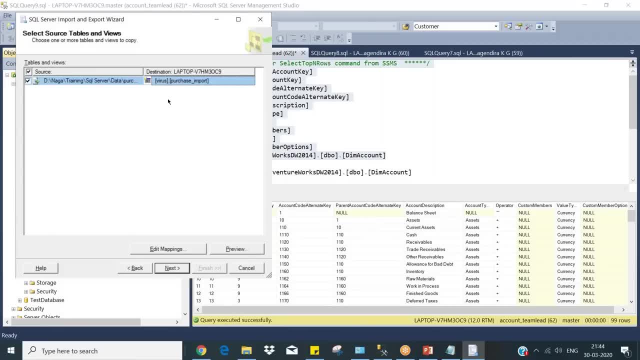 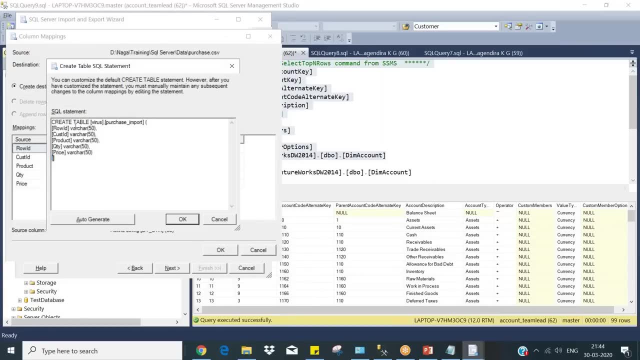 can map, otherwise this will create you a table for you. okay, now you can see the edit mappings here. edit sql here. so this is the structure it's going to create. where is that? purchase import row, id, customer id, product quantity, price based on the metadata you didn't. 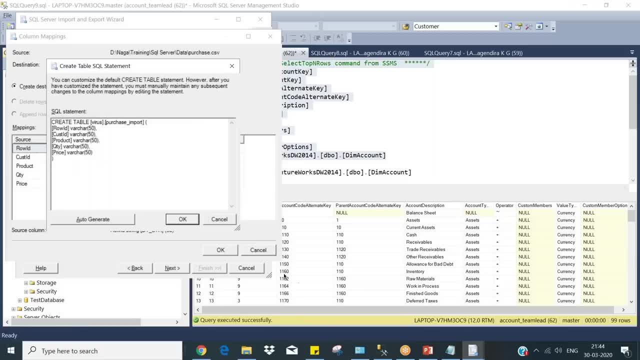 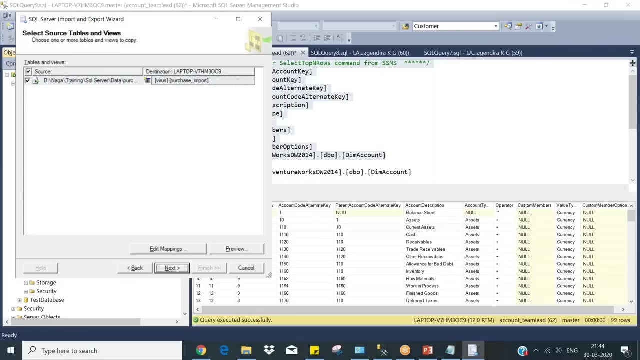 provide anything there. see, it will sense the data. so how it created the data type? you didn't provide anything, so it by default it created with worker worker, worker of 50, 50, 50. okay, you, If you have data in file or excel, just import. 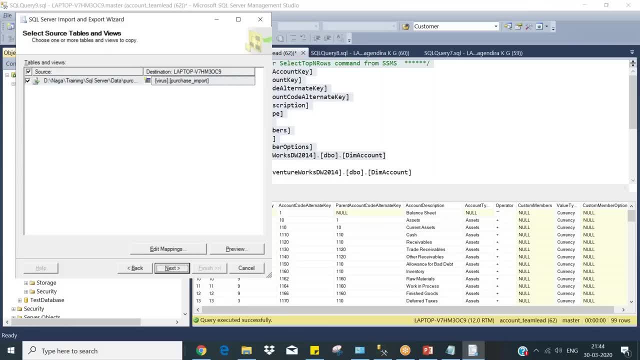 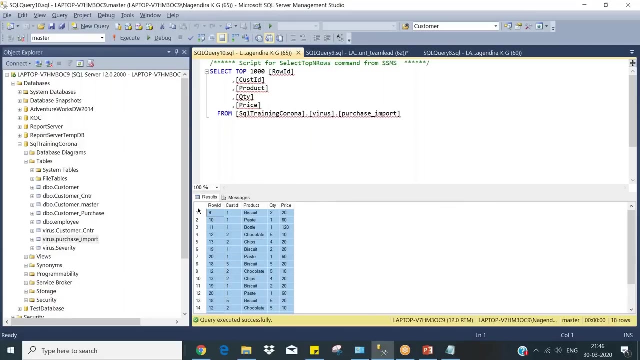 it. That will be very simple. Any doubts in this case, guys? Nagendran, if we have a live database in office when we import those data, do we restrict that It not be done by everybody? No, that is what I am saying. 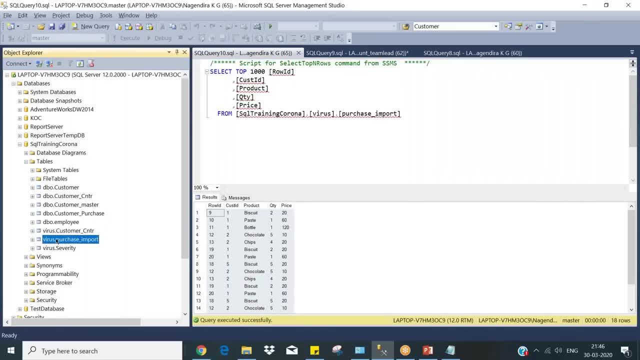 Districting is one part. You imported, you created a physical table As an admin. you should have access to it. Now you can restrict. this is the table you can restrict to some users, So not all users can log in and take the data. 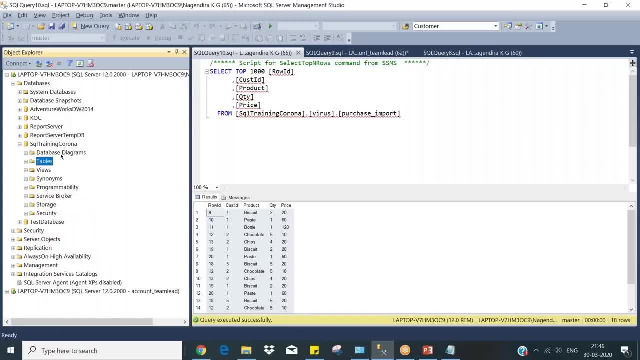 That's what I told in the previous point. You can create read access only to this and you do not show this table at all. You don't give rights to read or write anything. So those users have that right only can see it. 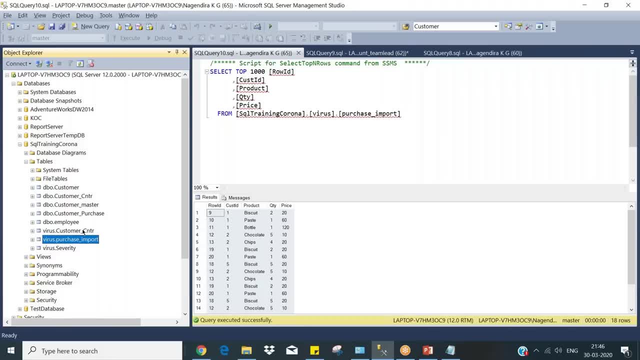 If the users have the data in excel, if they are adding importing, will they do, or we can restrict the importing the data to be done only with the respective users? No, you are saying who can import the data? Correct, Right. 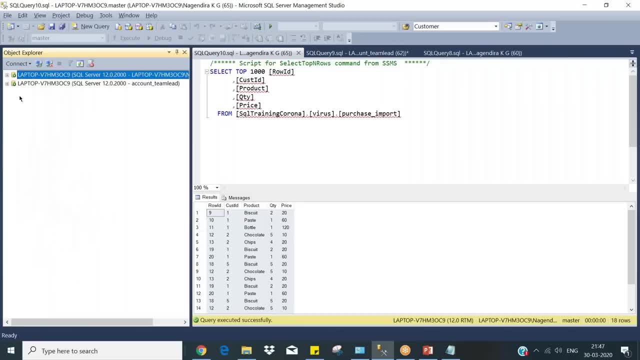 So it's again: whoever has access. So it's again: whoever has access, Correct Right. So it's again whoever has access. Let us try with this guy. He don't have import access, I think, Because you said the security and all. 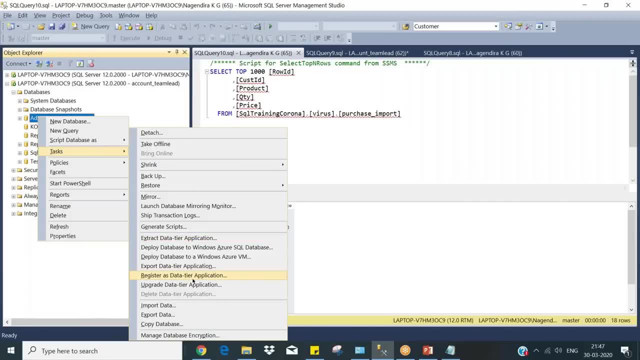 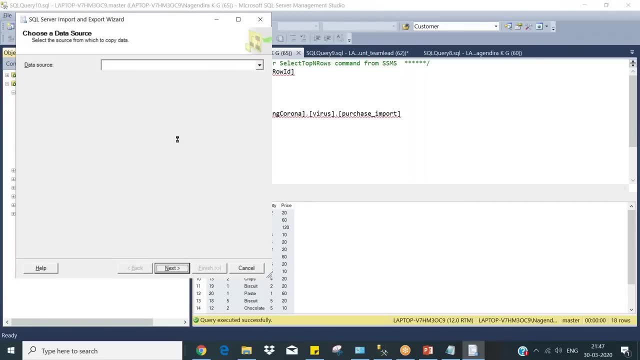 Right option he don't have, So you cannot write or create a table at all. So using him I can't do. let us try quickly. He can't do it, It will throw error for him. Okay, Nope, I answered. 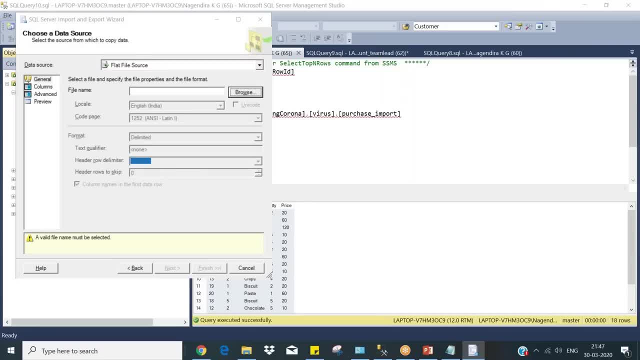 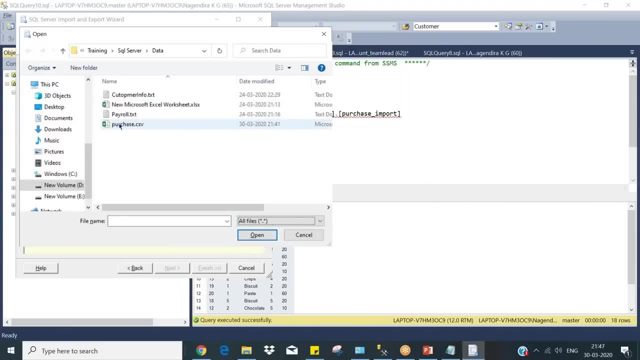 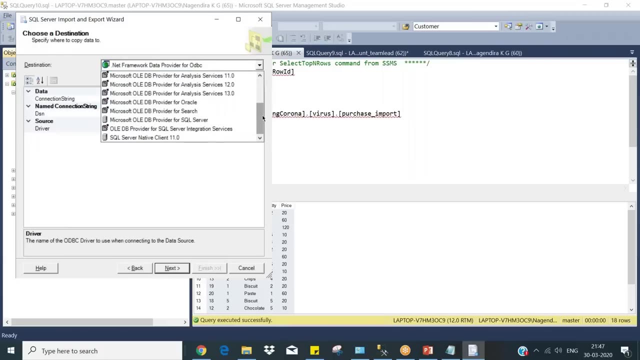 Let us quickly check what happens for him. I'm using another user. Okay, Okay, Let us try it. Okay, Okay, This one is open. Yes, Oh, I see, Let us read him a message. I see, I see. 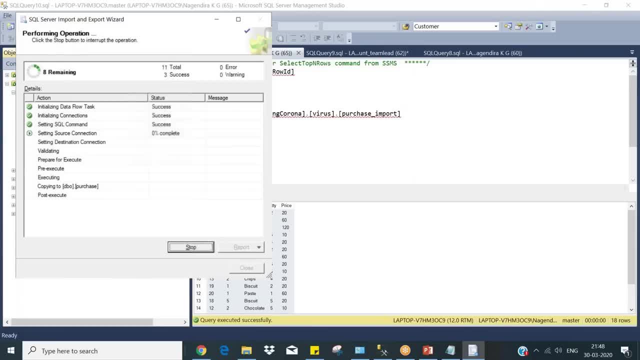 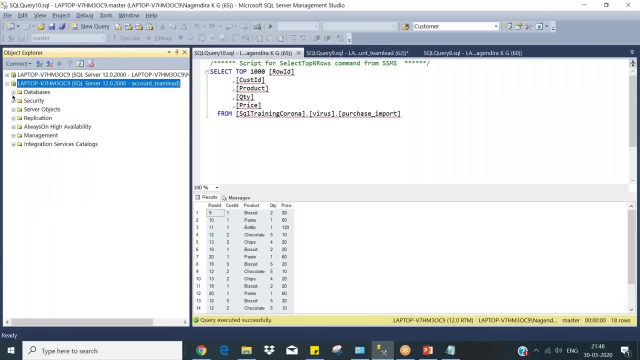 Let us read him a message: Oh okay, Okay, But we have to do it this way, Like before. This is it? Okay, Okay, Okay, All right, Yes, Okay, There were no error for that. We can wait to make changes. 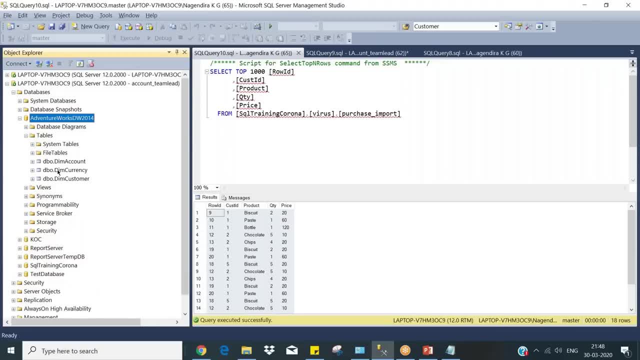 All right, So let us do it. Oh, okay, Okay, but it has written somewhere else. maybe it created from something else, not here. so the rights i've created has not given him a right to see the table you still see here. uh, it has created a table here, but he can see that in adventure works he has created, he can see. 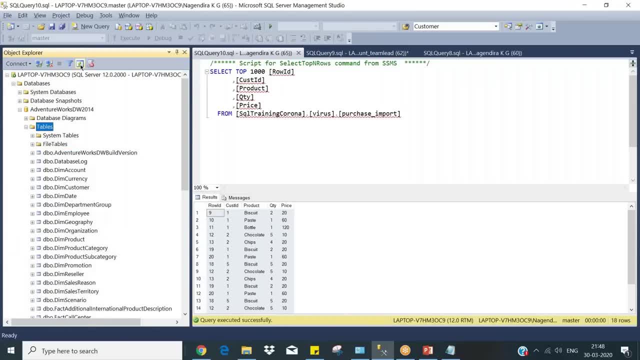 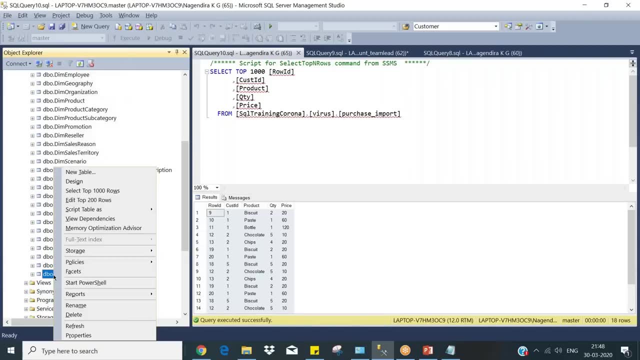 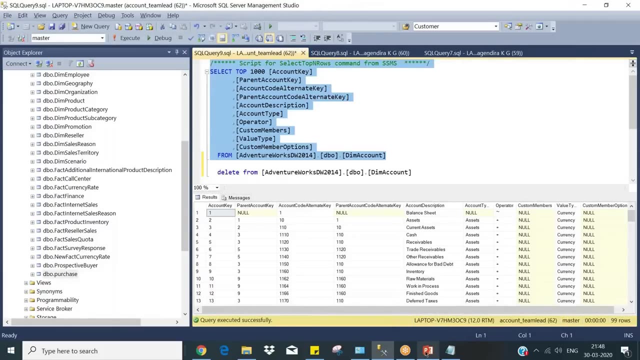 this one that that is doable. uh, to answer your question simply, it is stupid. see, you got a purchase table here. so, yeah, that is based on the security rates. okay, uh, this is one thing, then, linked server. i especially put here to make you to understand what is link service. yeah, 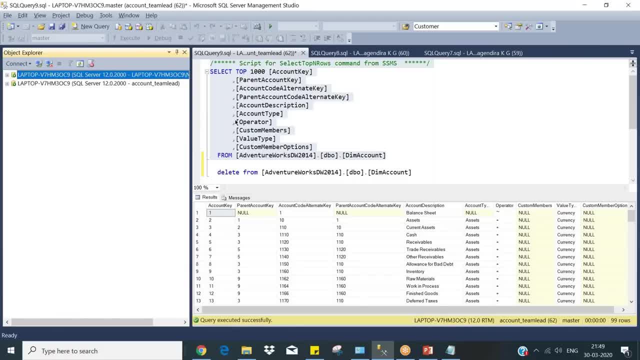 import the data. will this also include the column name? or because it's inside whatever we have in, including excel, according to which it's split into a column, wise, so the column names will it choose? yeah, see it. that is a built-in functionality. so, column names, you have given us a. 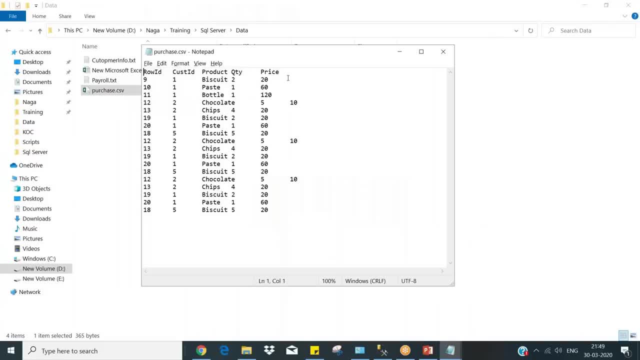 top order in the top. okay, you should have a top column and you will specify like first column as a row, i mean first row as a column name. some options will be there to specify so this and the tab delimited. here you have tab delimited. that is picked up automatically. you can even correct it sometimes. 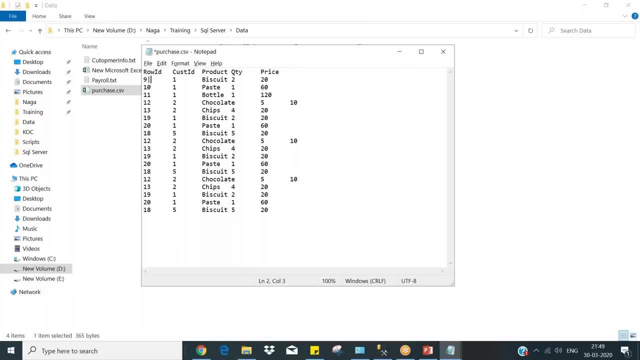 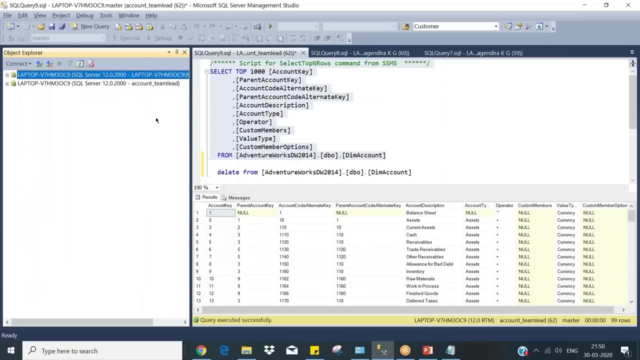 it will be like this, or sometimes the separator will be like this, so you need to specify that one. okay is okay, so based on your data, you can edit it. so this is about your import and linked server i have created because- see linked server concept is very 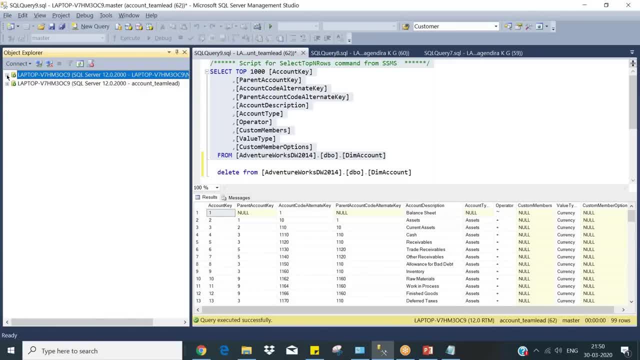 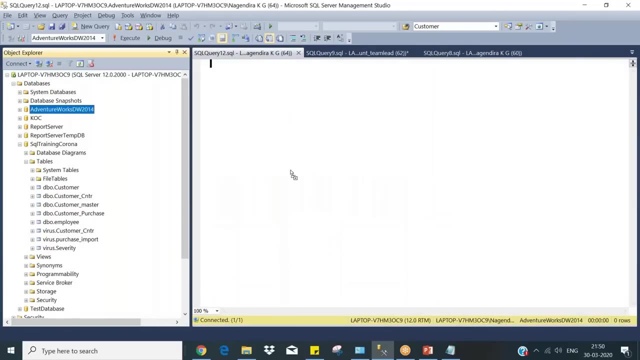 simple. you have a server here, you have a database. you can talk with different databases. between this, i mean in the same server. i can query a table from here. in this database, like here, i have a select star. see here i have adventure works database. i'm querying the. 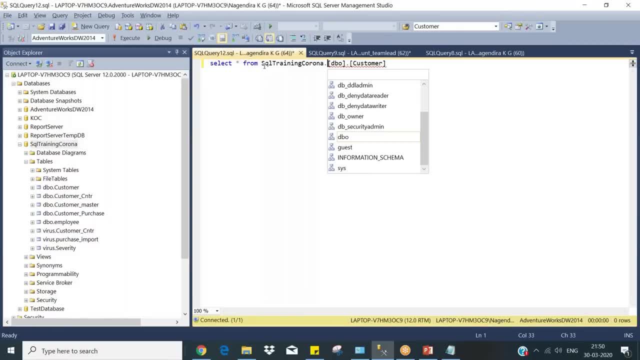 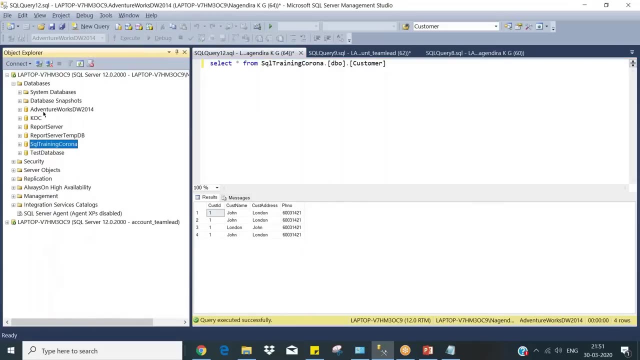 table in another database. okay, so i can query using three naming convention: database name, schema name and table name. and what about if you have a database or table to be accessed from different server? say, for example, you have a server, i mean deepak has installed the his own system, i mean sql server. that is, as i said, the dbms. sql server is a dbms he has in. 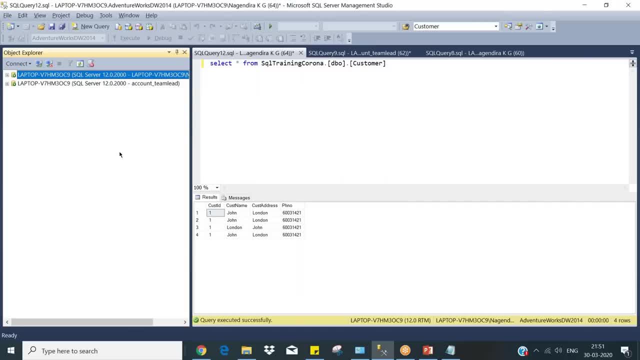 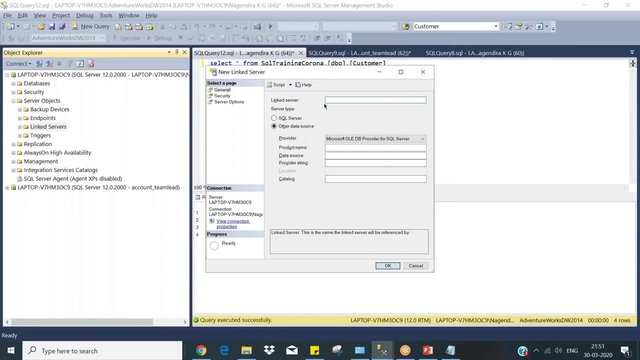 his laptop. i am having this table. i want to combine a table from deepak's laptop into my laptop. i want to create icon. i want to see it. so what i will do is- so this is again some rare cases. you will create a new linked server. i will give the deepak's server name and both should talk. 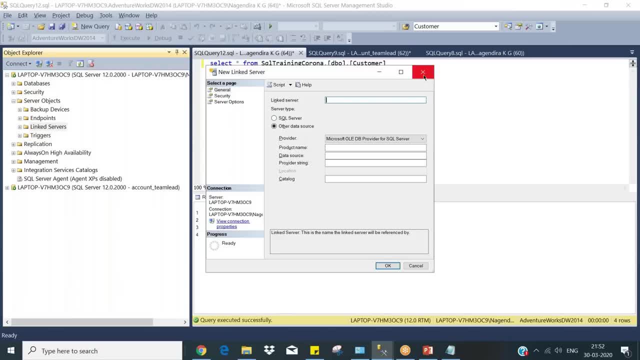 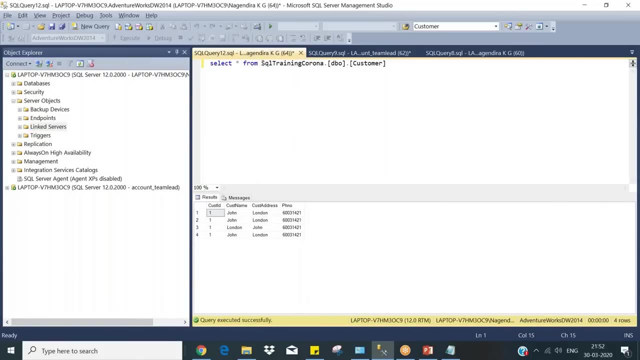 okay, there should not be any firewall or other issue. so your system should enable to read my system to accept the server request. so those things you can mention it here: server name. then it's like again you can use instead of this database name you also have another dot, like you have a link- server name. 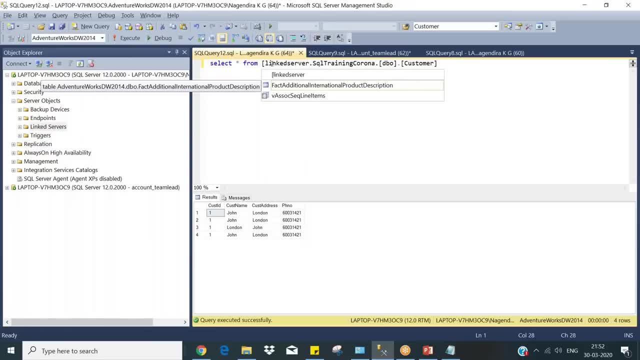 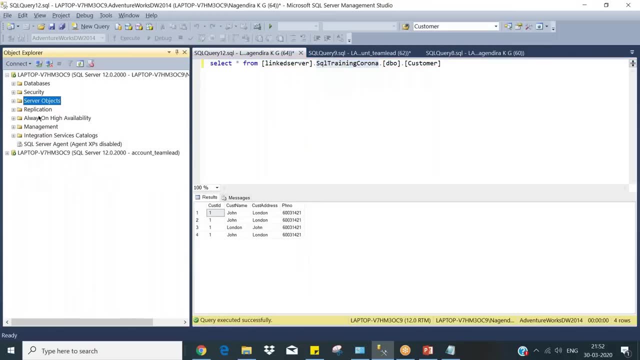 i don't have another server here. i can't talk to the book server. so link server name dot the database. you got it right. so just a link server is nothing. but you have a database in another servers you want to access in your environment. you need to create. 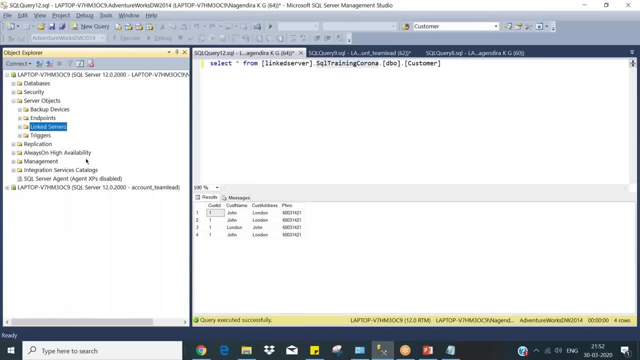 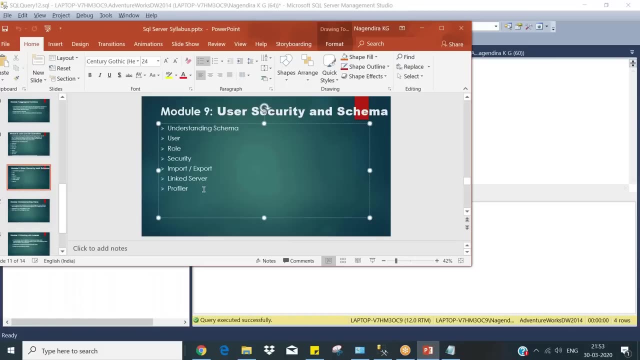 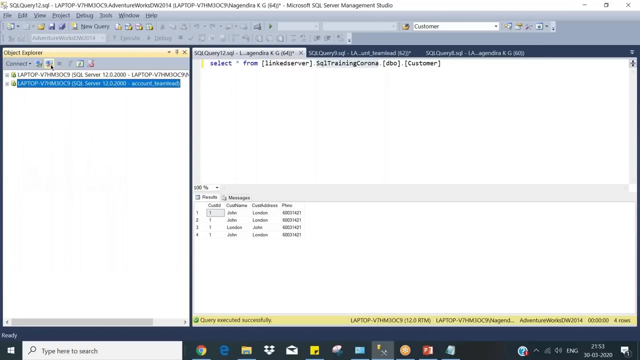 a linked server. okay, then only you can able to access it. this is what. okay, so this is about your link server. then one important aspect i want to cover is like a profiler. it's very crucial guys. most of them won't use a very important concept to learn. so what is a profiler? so profiler is a. 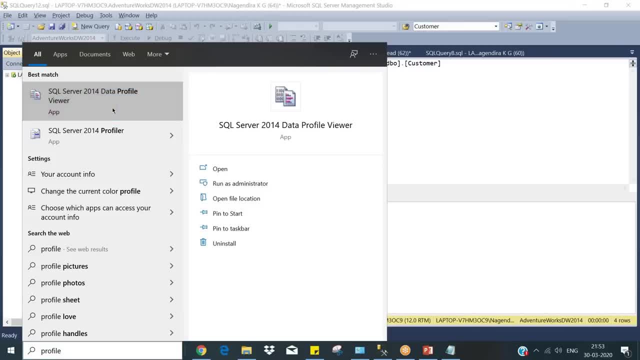 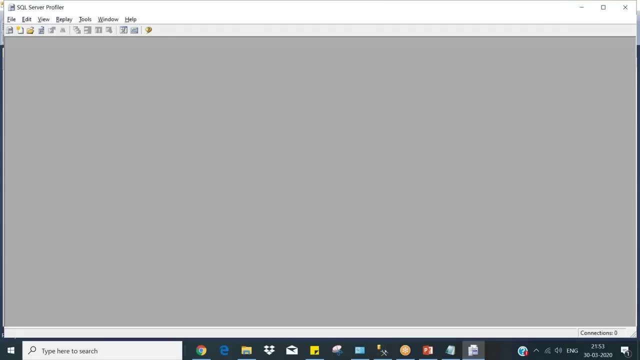 separate tool, data profiler. now, it's not a data profiler, it's your sql server profiler, sql server profile. so what it will do is like, as the name indicates, is the part of dbms and it will give all your activities inside the dbms. you see, like in the windows profiler. 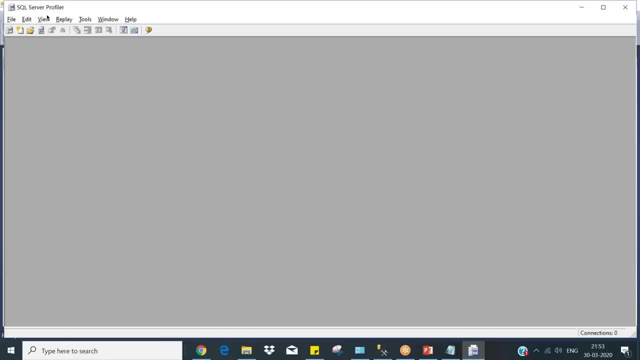 you have logs: whoever logs in, whoever logs out and what activities you did. you created a table and you created a file. you watched a movie, some windows player has went- those logs will be tracked. similarly, if you run your profiler- only if you run it- okay, all the activities happen in the 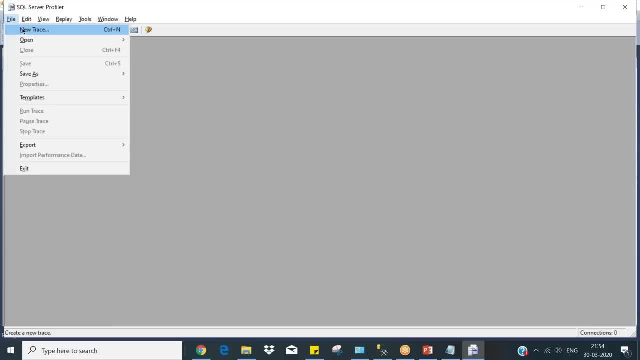 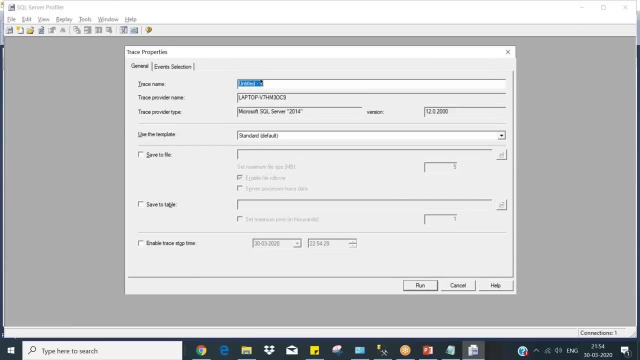 database will be logged here so you can see the things. so, whoever has deleted some records you have deleted, which user has deleted, which user has modified, so that you can easily track, you can identify that person. so what are what is this thing track? so, basically, for all purpose, it will be using exactly. 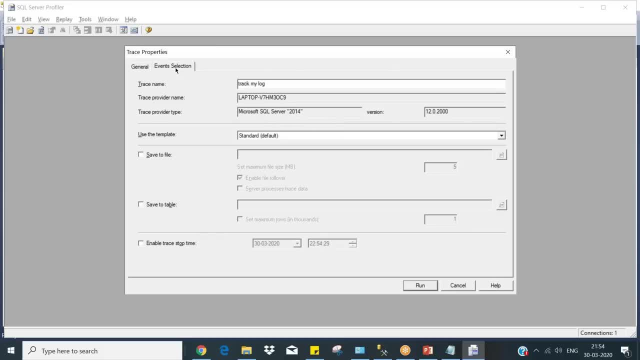 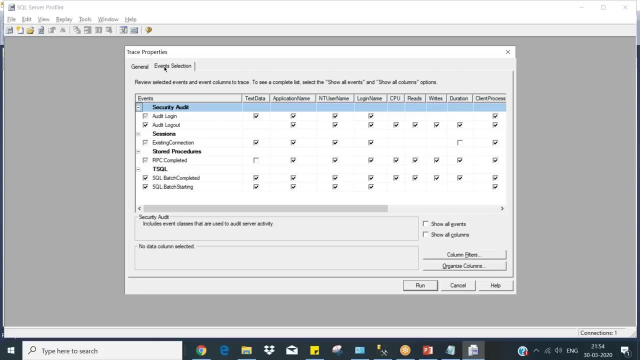 all purpose. so events: yeah, go ahead for that. they're separate um application reserve sql server profiler. yeah, yeah, yeah, so it. you see, if you enable it, it will log. but you can see what is happening here. what core is? it is five, the runtime. when you hit some applications, what code is it came from the client application, what? 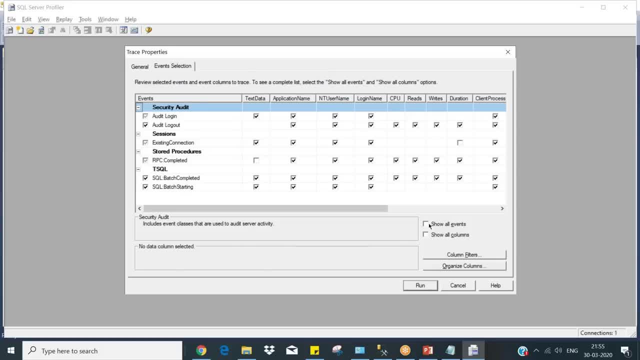 code is. it has written the results. those things will come here. so just, you need to see all the events in database level, all those things. let us see what important here is. think database, let's see, uh, okay, i will choose all columns, all uh things. let's keep it like this, okay now. 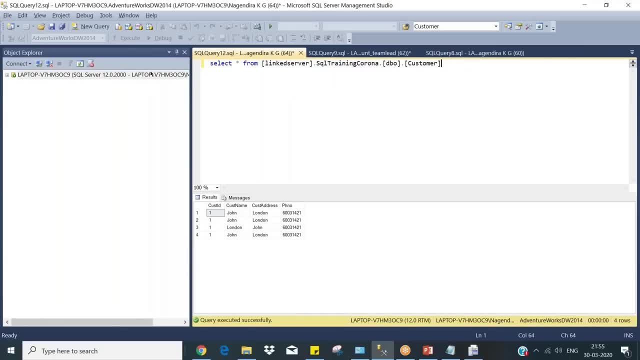 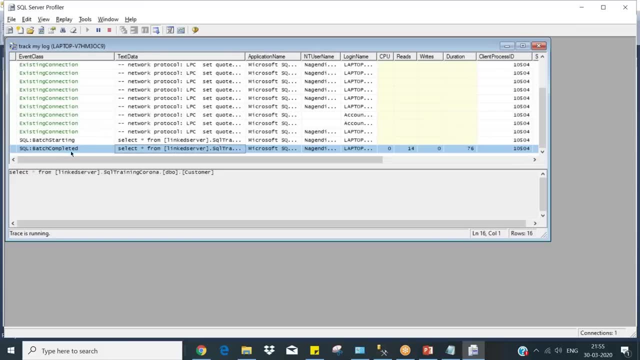 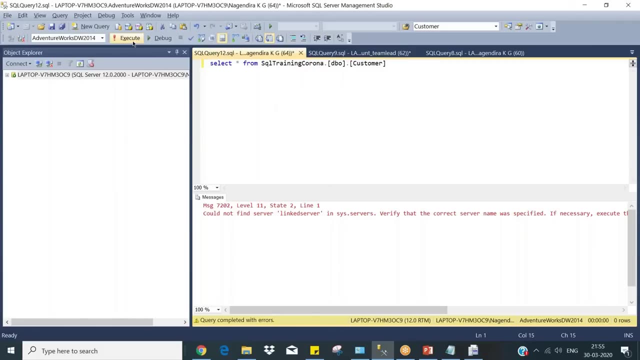 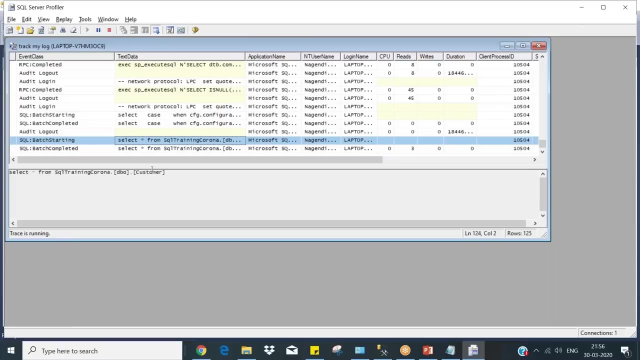 you have everything over here. just i run this query so that will be available over here. so i have run that query. sql batch completed. select start from link server. since this doesn't have any link server, so i throw it there now i run that query. you see here, without that, uh links, it has written. so what queries are. 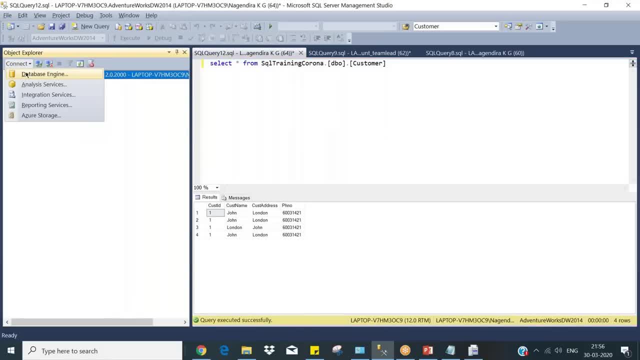 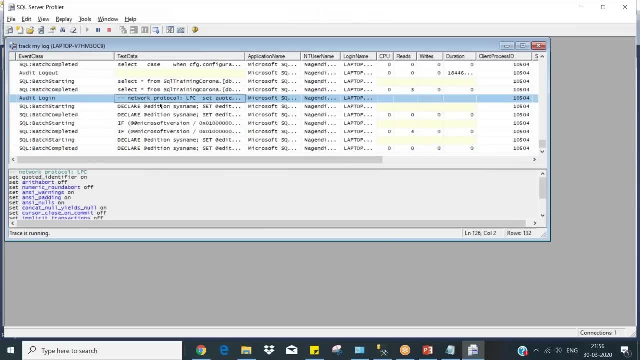 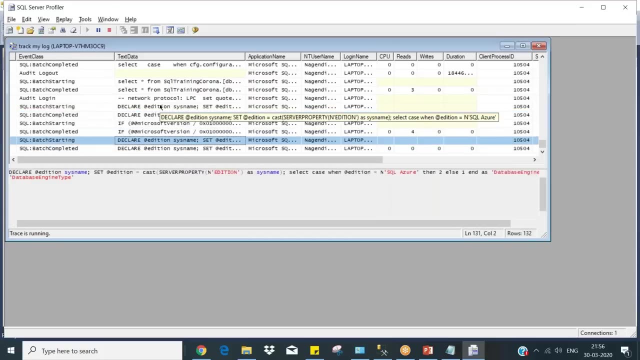 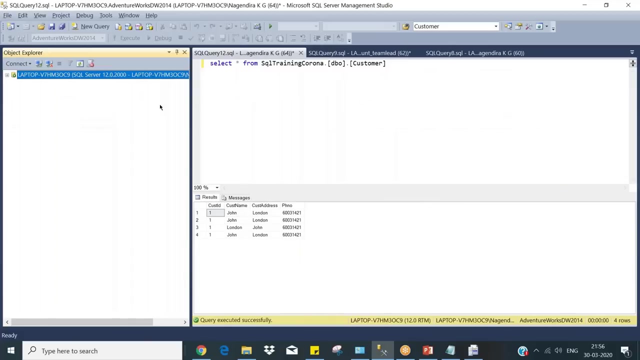 keep on firing whoever logs in. if i log in, the activity also will be tracked system admin addition. what is all those things who are logged in? adm connection edition. so this is the events which will tell you who started the fez client and what they expect if they want to share with you to see whether or not they. 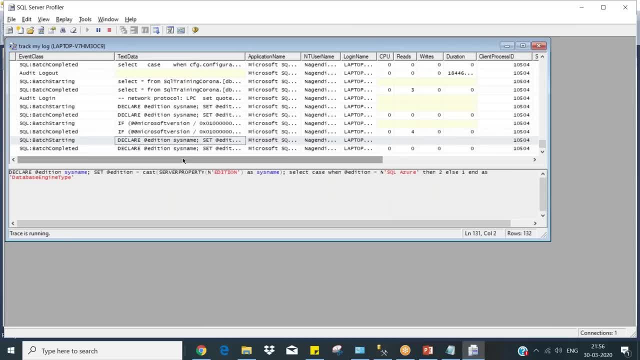 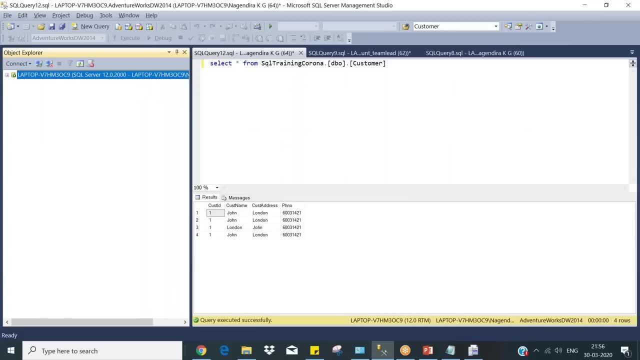 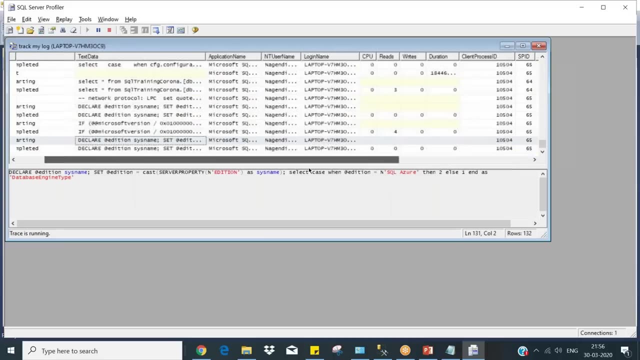 are going to be like in the Church service: bancho. um, something is going wrong. someone has goes and deleted, and which user has deleted. it will keep track. so login name, who has logged in, who has done the changes? we can Push-It so people can't say i have deleted, no, i don't know who did that. 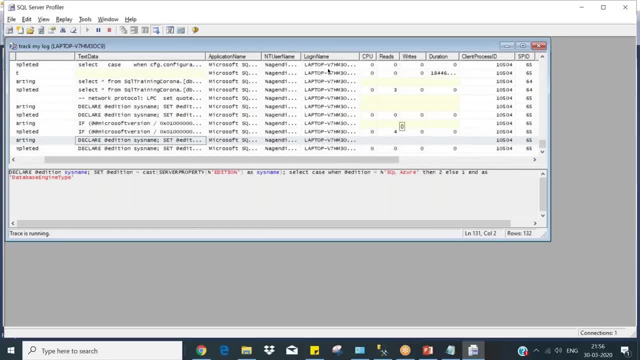 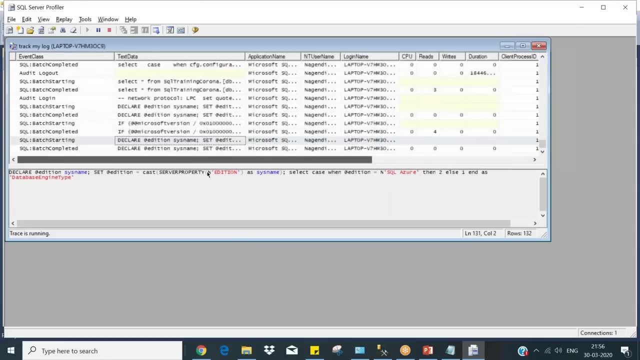 so this is very important tool to identify. okay, so people will say: don't share your logins, all those things. right, this is because of this. someone has logged in in your user and deleted. that will become a very tedious problem. so this is main purpose. so I hope I always tell to Rahil we need a profiler because they ask some. 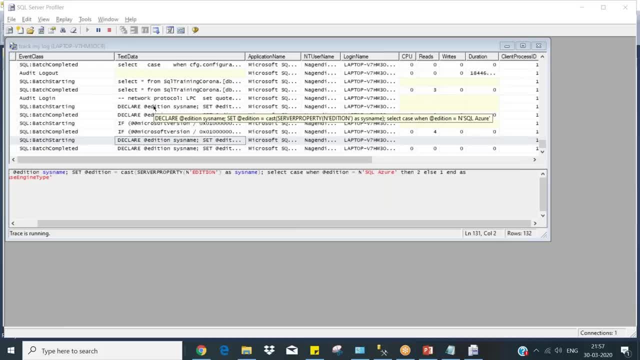 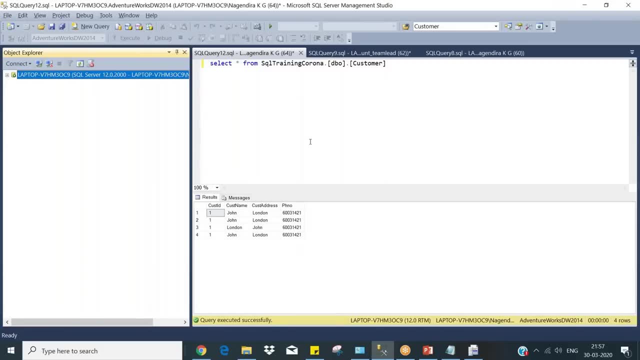 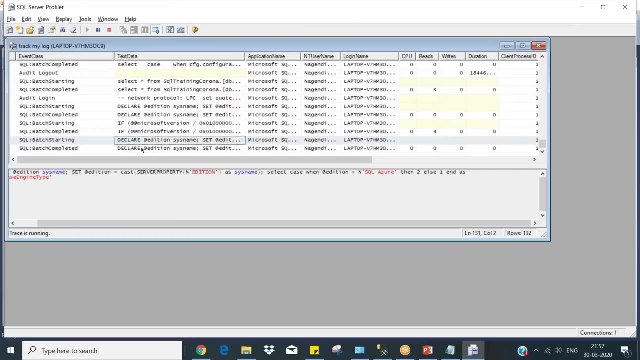 application. so all these commands, whatever commands coming from the applications, front-end applications, your client. so, since it's a client, my application also will be a client. my web, it can be a web page, it can be windows forms. anything will fire a query. whatever queries it fires, it will be. 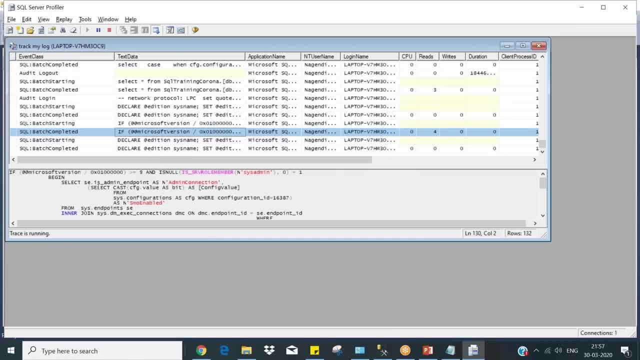 captured here so we can see what as what I mean what queries it is firing. based on that, we can easily point out which table it is referring to. I will be don't know what tables it is referring, so I can see from this profiler what tables it's referring. so I can see it's system configurations. 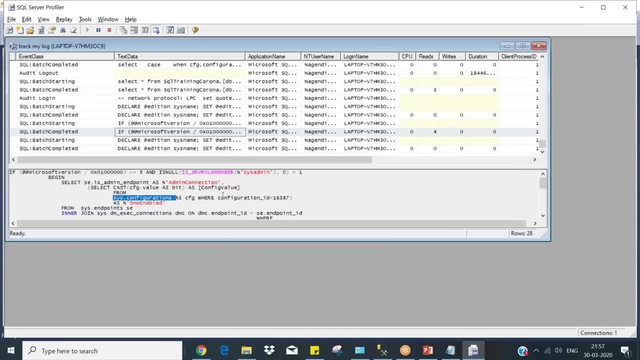 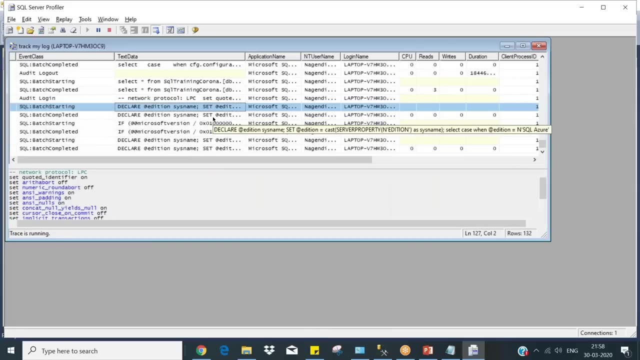 it's referring my username so I can go and check in that table. so it is as simple as that. when you have a profiler in place, we can easily find what tables. so it is used for troubleshooting, basically, and also it's used for to know the whoever logged in. which data is the query is: 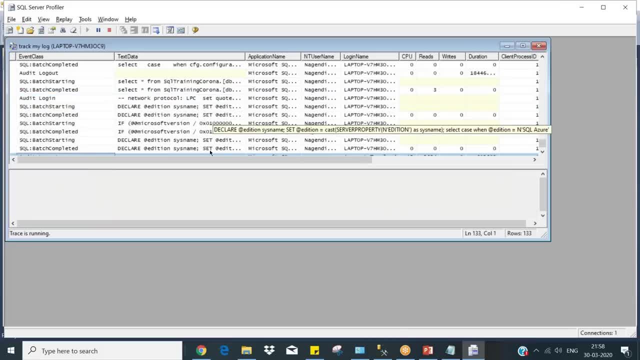 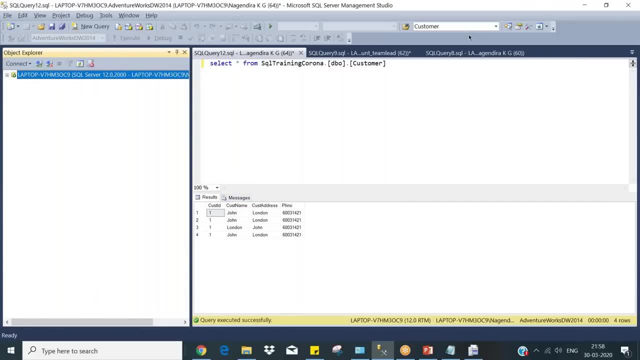 firing. what queries are firing frequently? those things will be tracked. this is one of the main important any questions in this skill profiler. okay, one last thing. I want to show it to you. so I have something like this: I want to take a backup, or once I have taken a backup, I want to restore the database. what I need to do? go here, restore. 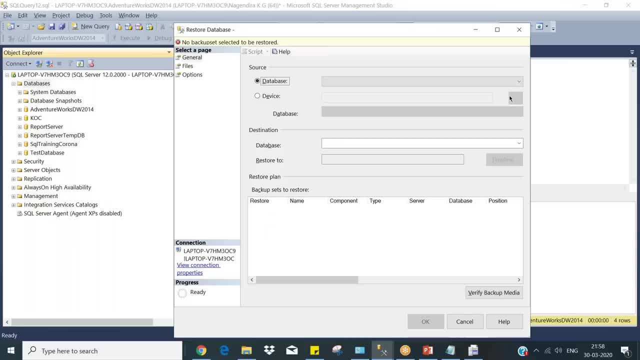 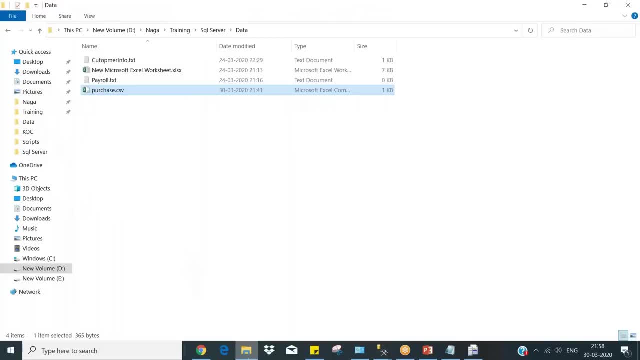 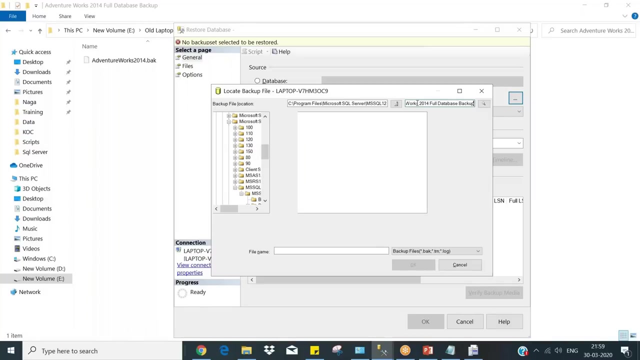 database already taken a backup of it. so from device, if it's stored and add something over here, so of course when she works, so these database files will be stored in stored. when you take a backup of a database it will show that back be a key so it will be stored once you. 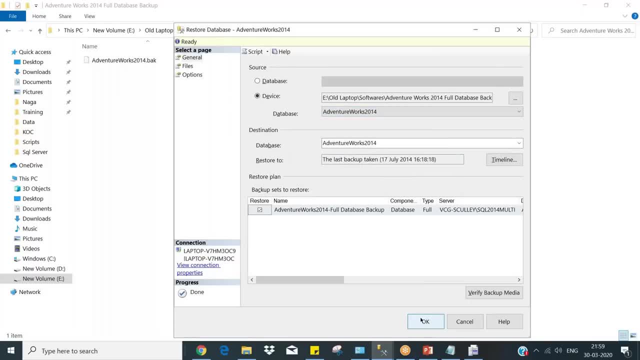 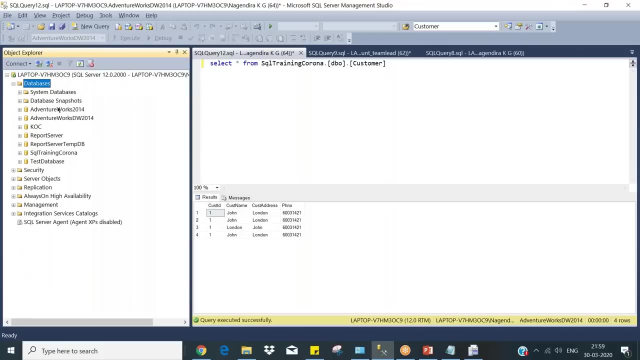 choose that one. that's okay. then press ok. database restored successfully. so earlier we have DW. now you have another database here which is nothing but works- 2014. the tables are entirely different. here, you see, with the schema: human resource, person, person, entity, all those things okay, and taking a backup of database is so simple. 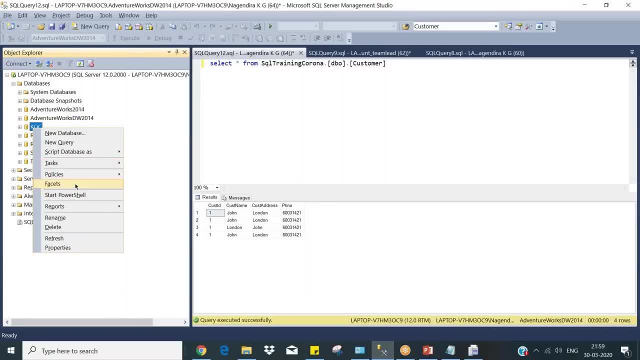 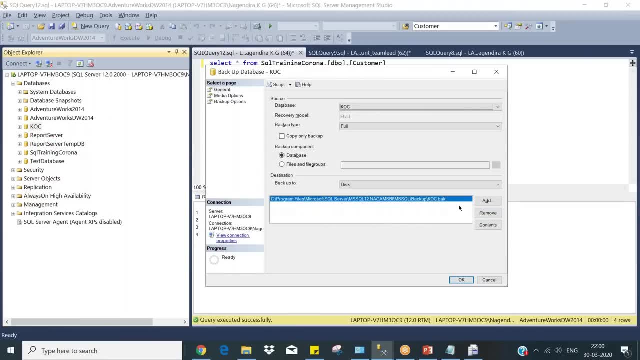 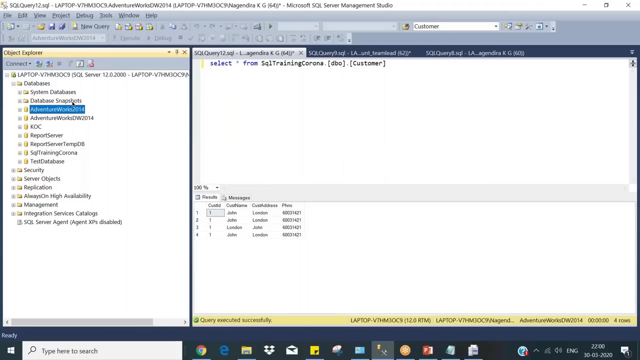 right click task back up. that's all okay. just choose the path. let it be in same path. just press ok. that's all okay. once you want to restore, right click and create. so this database does not exist earlier, so usually you can go and check. I want to not be a k files to work on, so 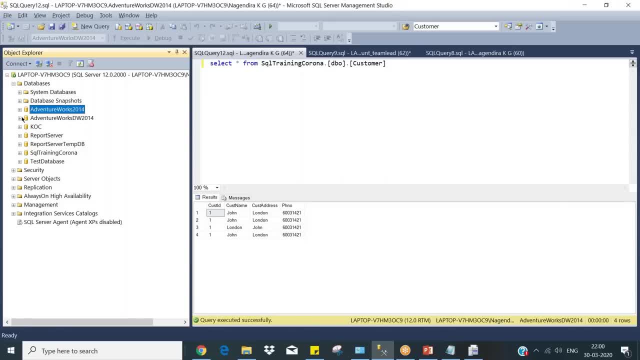 just go and check. I want to not be a k files to work on, so just go and check. I want to not be a k files to work on, so just download it, then import it. it is as simple as that. you no need to create tables, all those. 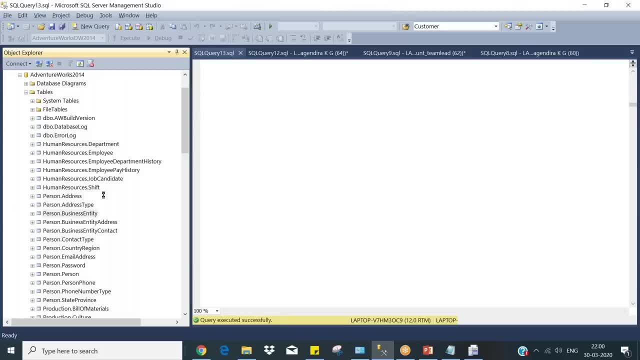 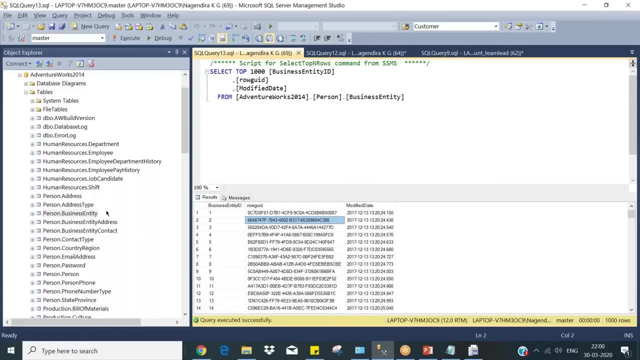 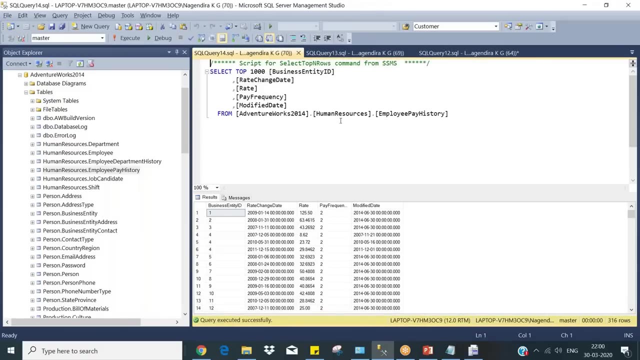 things, the tables, everything. it is not only the schemas, or I mean one of the structure, it will also have a data. once you take a backup, it will also have the data. all the data is not there. okay, okay, guys, one time I've completed anything in this session, any class. 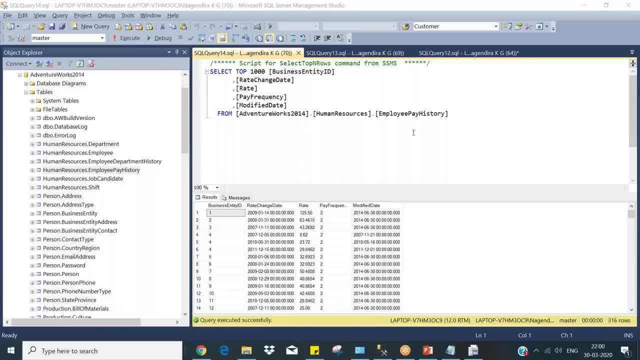 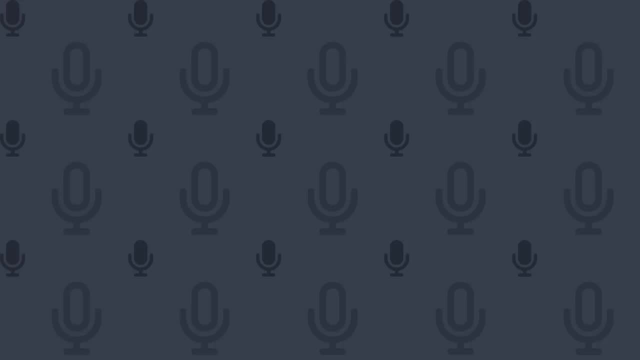 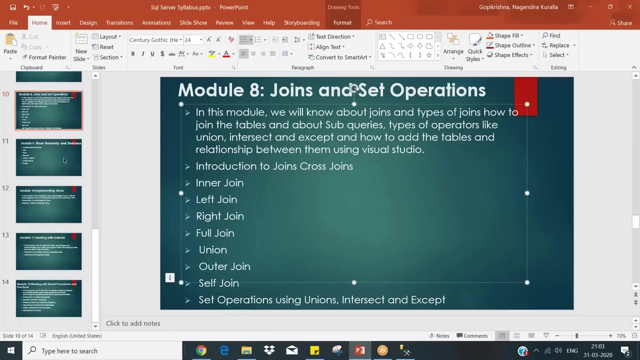 okay, guys, one time I've completed anything in this session, any class. okay, that's good, let's stop it today. this conference will now be recorded. okay, guys, one time I've completed anything in this session, any class. so let's let's have a quick overview of the management of Brave hè. 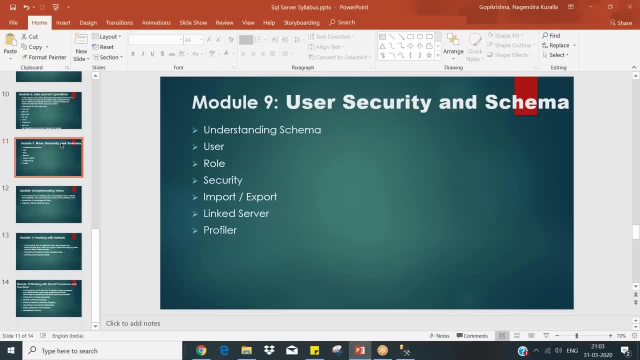 so let's let's have a quick overview of the management, of the management of Brave hè you. what we have discussed yesterday, so yesterday we saw about schemas, and schemas is nothing but group of grouping of tables that is used for your giving security rights. so only those people's. 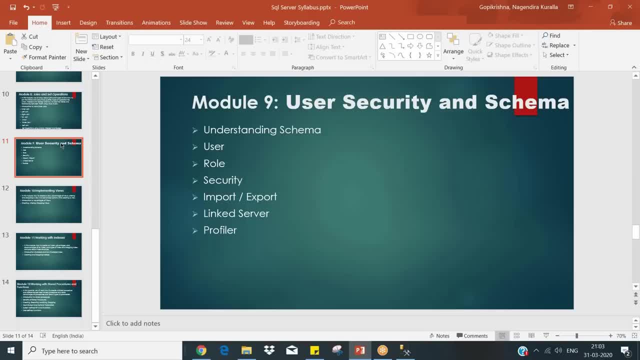 having pertaining to certain departments they can access and there is a main purpose and we have created some users and role-based security, how to do that and the purpose of security. so yesterday we saw about giving one particular user giving only the three tables, having a select access. when we try to delete it, it doesn't allow him since he, the user, has only select access. 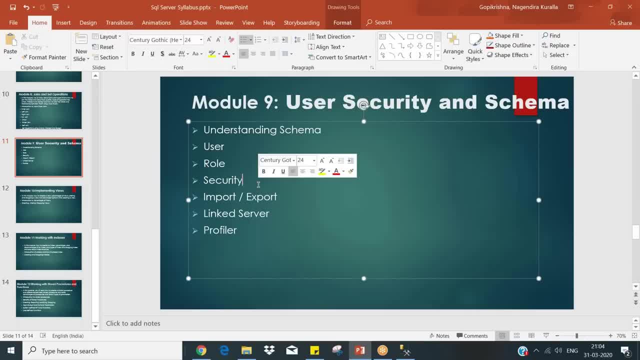 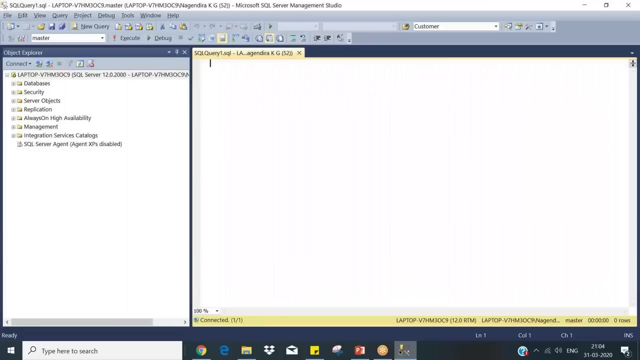 so these kind of things we can't do it in file management system. that is where we there is a main advantage of going for a database management system. that point we have highlighted and we just imported one of the file. export is same operation. you see here: hello, who joined Deepak? okay, so hello. 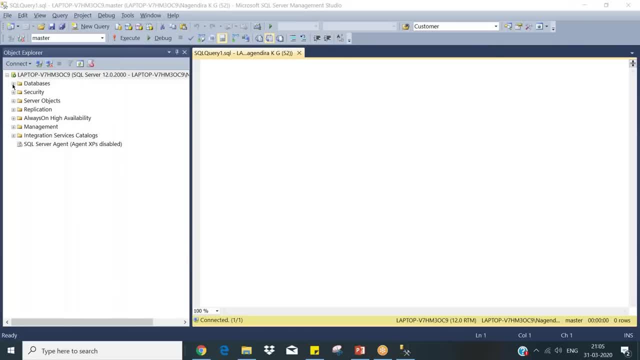 just we are discussing about what we have saw yesterday. so we just saw what import of our table and how we need to do an export. you see some data over here. you joined some queries and you got some table information here. so this query can be a simple query, as like this: select star from table. 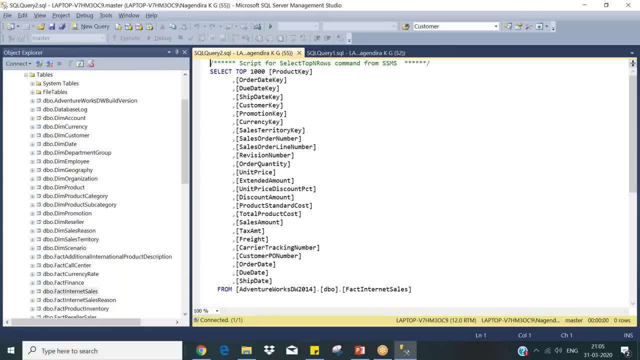 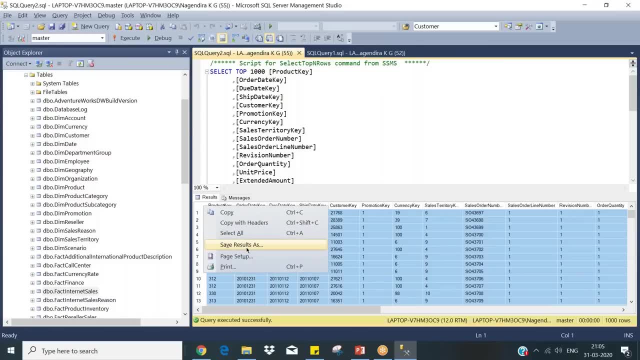 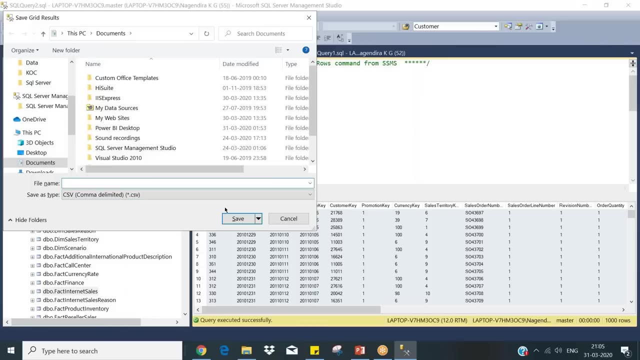 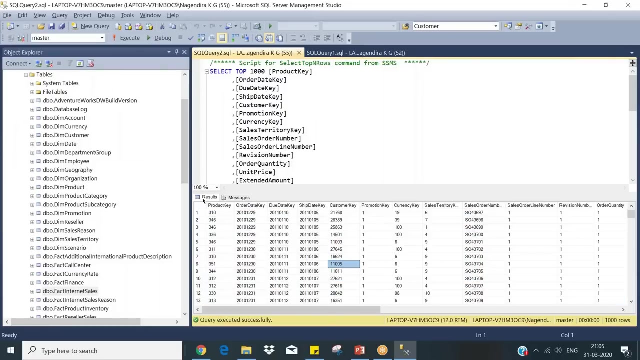 or whatever queries you have did yesterday or previous days using multiple times. this is your output. assume like that. then you can save these results. as there is not a just an export, see this will also give you the results that saved in a csv file, comma separated file. so just returning. 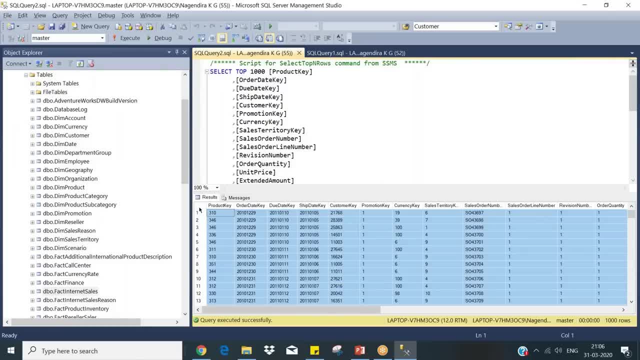 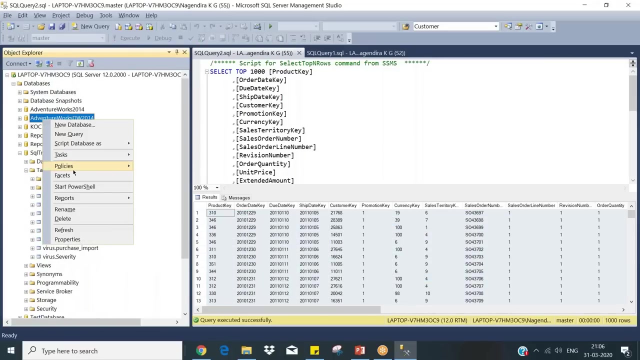 this result and click on this uh corner, left top corner, then you can right click it, you can save the results. so this is kind of export. but this is not the actual export. this will give you only the one file. if you want to export multiple files, how to do that? so click on the database task. so these many tasks you can do- backup, restore, 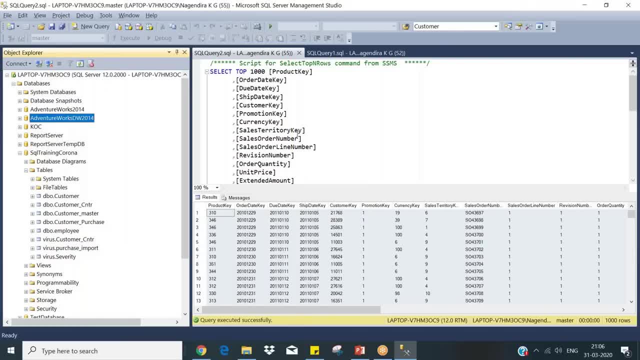 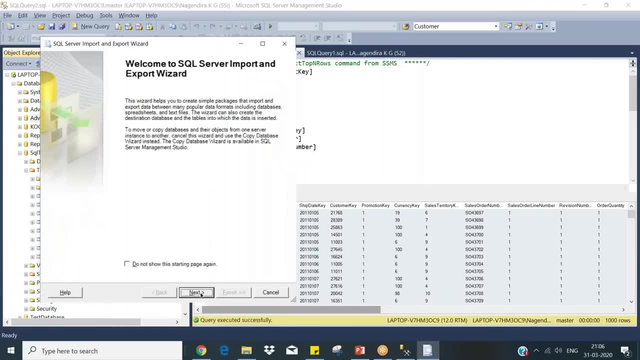 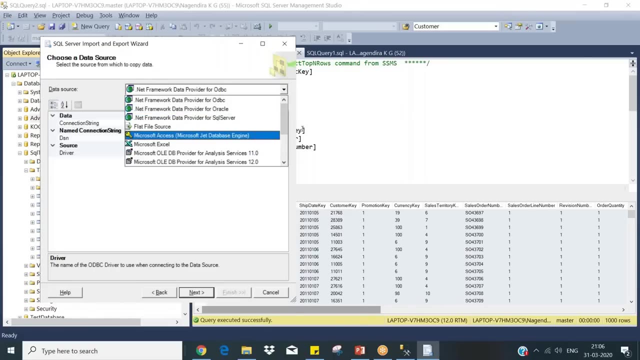 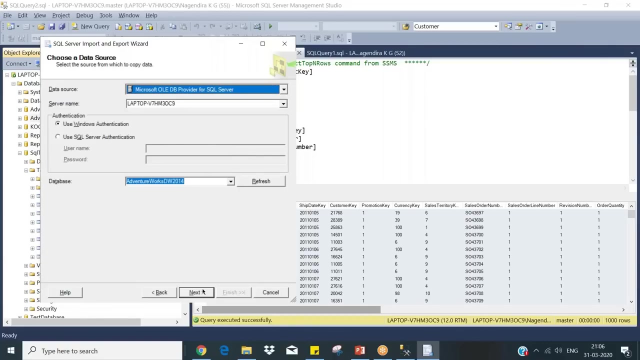 measuring all of the steps. so export data. similarly, we saw yesterday about uh- import data. so let us have export. choose a data source again. data source is our SQL server only. so same server. this is the database, and choose what you want where to export. I will export it to a flat file. 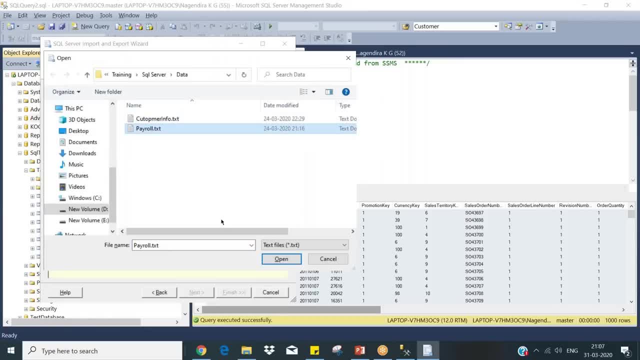 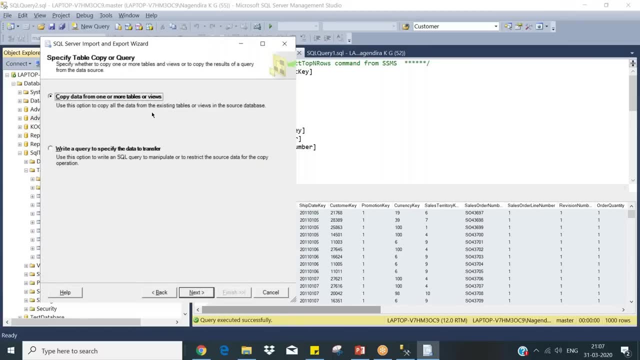 I need to choose file over here. let me choose payrolltxt, whatever next. copy data from one or more tables have used. okay, so I can copy multiple data table into one file or I can create one file per table, something like that. those things you can specify here. so this is my source table. 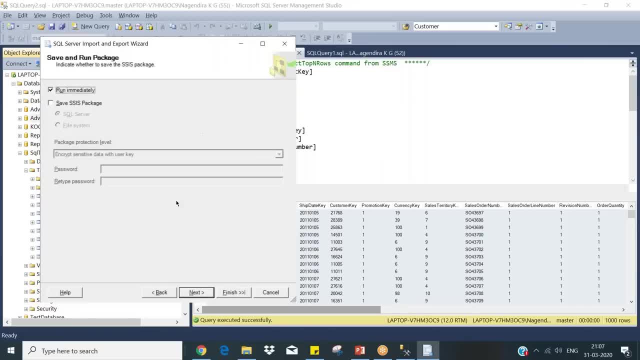 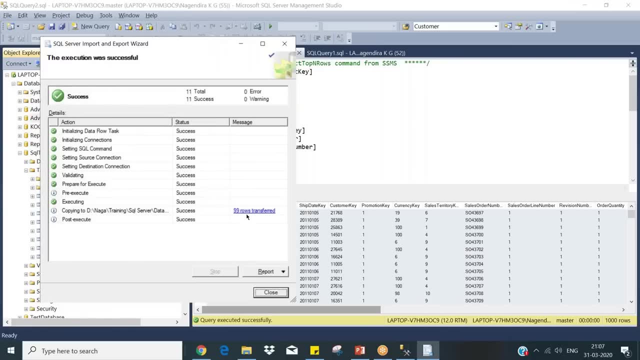 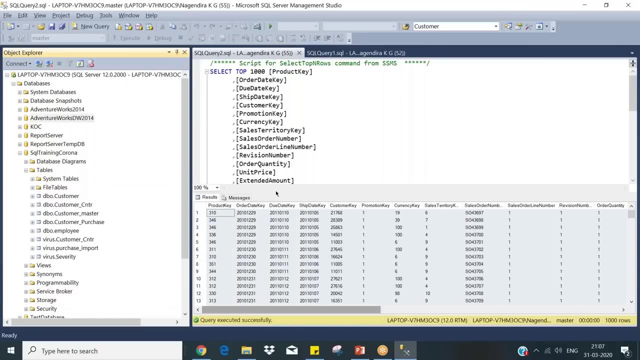 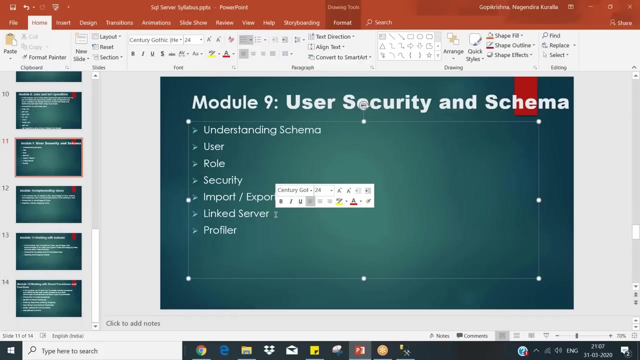 account table, then immediately. so same thing will happen: the purchase or those file will return some records, okay, so this is the kind of exporting your table. then we discussed about link server. as we do not have another server in place, we can't able to, uh, practically see how it works. 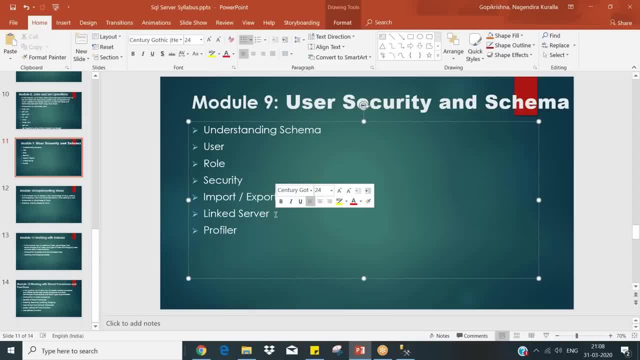 so it's as i said earlier. we need to refer the link, server and database name, follow the schema name and table name. so, in order to access the table and the profiler is a tool used to track keyword changes or whatever changes you do. all the events will be captured there. it's used for it, okay. 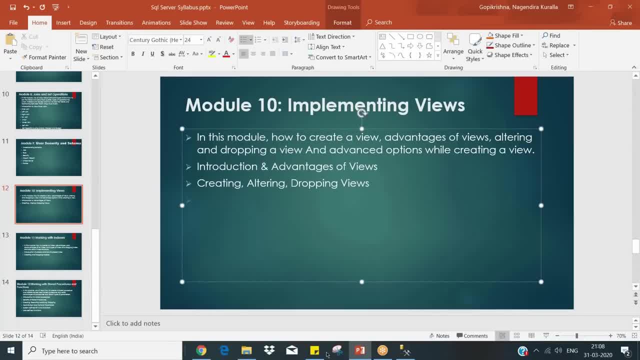 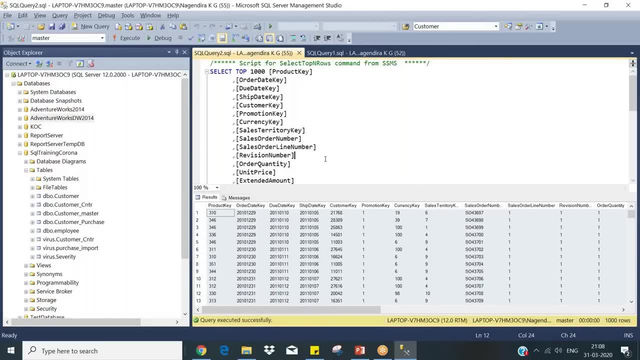 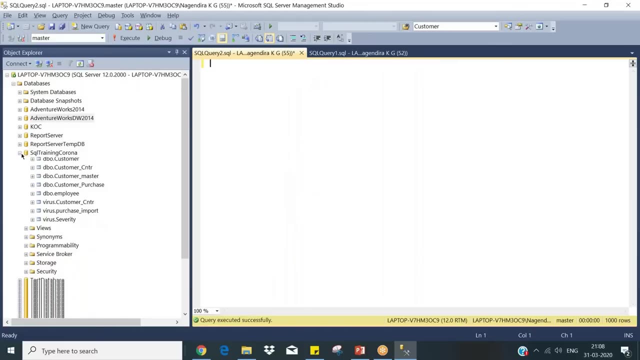 okay, view what it is used for. any idea, anyone aware of it? hello, obviously, yes, so can you tell these people so that they can understand? i have to collect the data from multiple tables. okay, it will view. yeah, okay, great. so what is the purpose of it when you create multiple tables, when you want the data from multiple 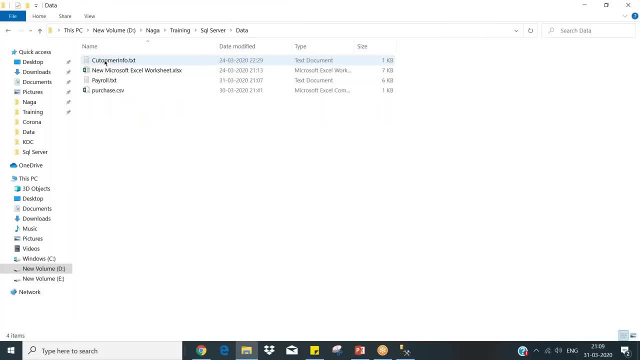 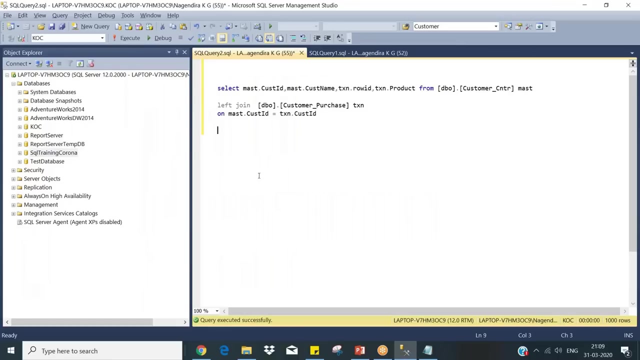 tables. you will always query it. i mean, um, yesterday query i'm trying to take- let's take this joints example. okay, so this is the table we have taken yesterday, so this contains a joint. okay, so when you want to have a join, multiple tables, okay, we need to use. 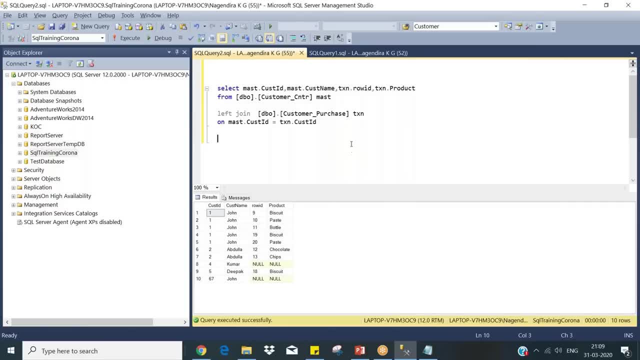 left, join in the join, whatever can be. so, um rahil, i will ask one question. so if we have a one table, do we not no need to create a view? let's come again. i mean you said like if we want to join multiple tables, then you need to create a. 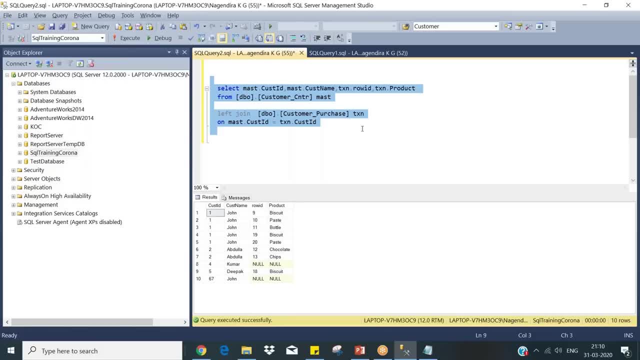 view. so what about if i have only one table? even with that, i can create a view or not? yeah, you can create a view with one table option. yeah. so basically, it doesn't matter you how many tables you want to have. basically you want to store this query in the database object. that is the main. 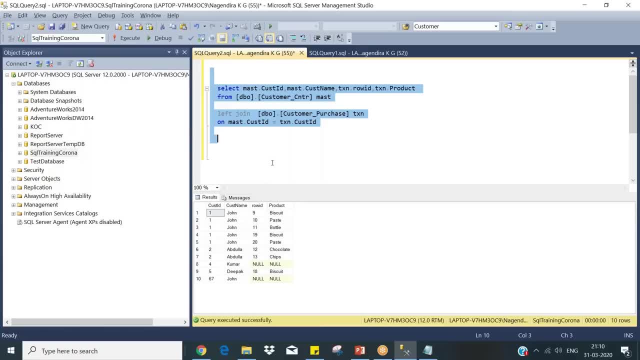 purpose. so a view definition says: like: it's a virtual table. now you can see like this is the result when you execute this query. so you can see like this is the result when you execute this query, whatever you see here. so this result is not stored, whereas this query can be stored. 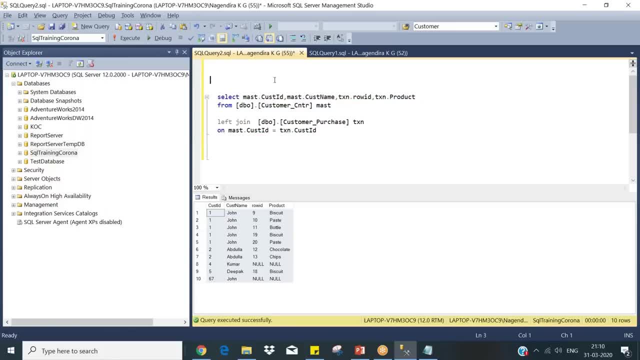 somewhere in uh database. so that is the purpose of creating a view: create view, view name. view name is like customer product purchase. okay, so you always end up with having this kind of queries frequently. okay, you need to join multiple tables and if you forgot this query somewhere, then it becomes very complex. so what you need to do is whatever query. 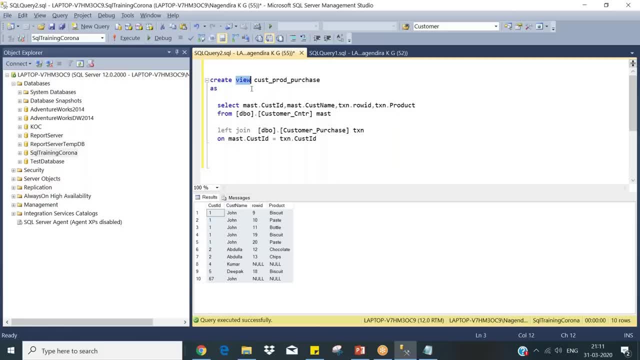 result you want to have. you write that query and put it in a view. so this will create a virtual table. let me show it to you guys. so when you select this query, you are getting these four columns and with 10 rows. so when you create a view with this query, what it will do is: 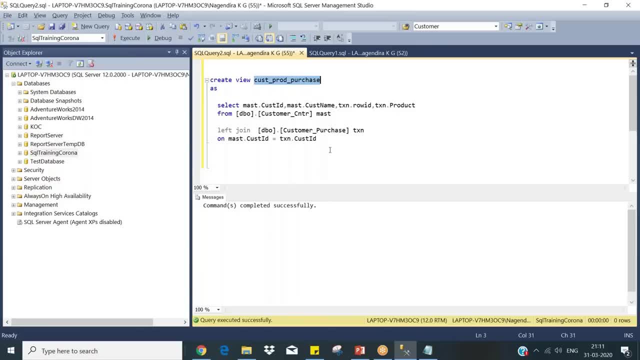 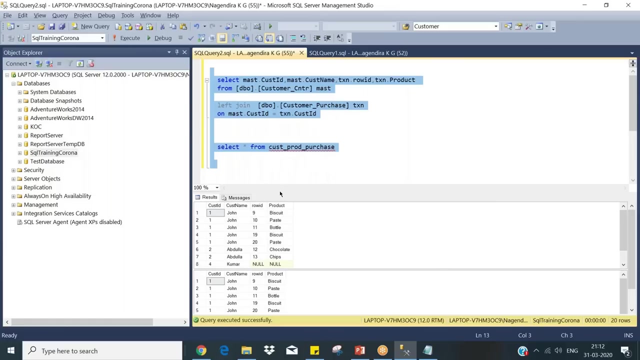 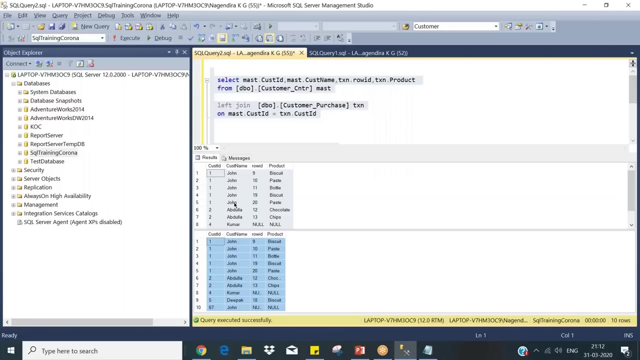 instead of selecting this particular statement, i can select this particular view. select star from this one. okay, so you see the difference, even from here and the very background of your words. ok, you can see that your query is in a view've put the point somewhere, it'sçe. 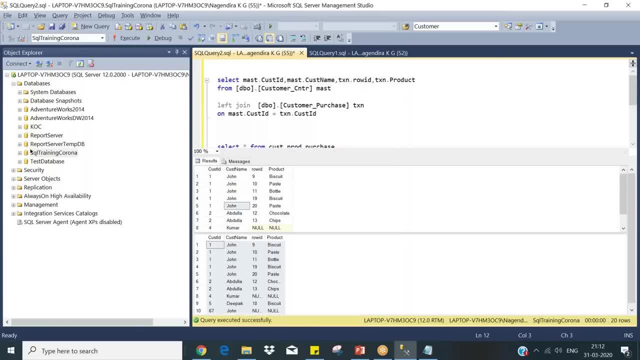 go that you would give any bitten loam you can on. may be. something like this is posed by bastante. so view won't store the data, it will store only the query. that is the main purpose of view. let me show it to you. so here it is the query. i mean. the view is stored here. customer. 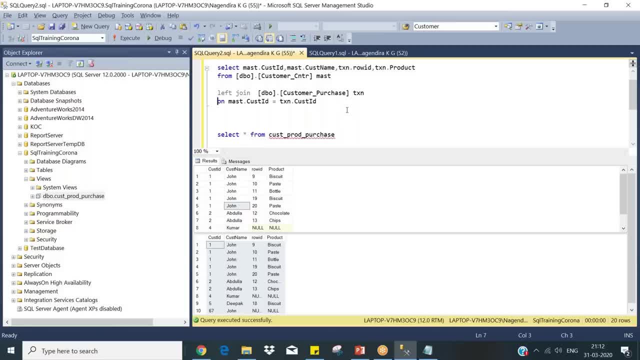 product purchase. so, as rahil pointed out, in order to have multiple joints, okay, so people will forget, or they use different joints sometimes once you use left joiner in engine. so this query will be stored. and if you use only one table, okay, and you use some war conditions. 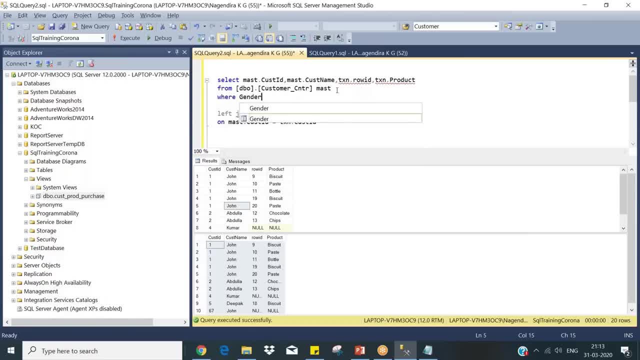 where gender equal to male are kind of. i want to have some constraints to be defined. someone has some question? okay, okay, so commonly used queries where we every time we will run again on a daily basis or some time, so those queries, if we can save it, it will be easy to retrieve. yeah, yeah, so there. 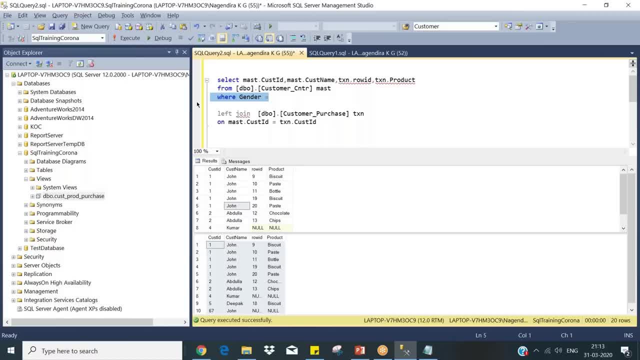 are multiple purpose, so it is not. you cannot store those queries, whatever you regularly use for that. even this is used for a security purpose as well. the views: the thing is like: instead of giving access to the you cannot, I mean you can give access to the views, okay. so, as we discussed, 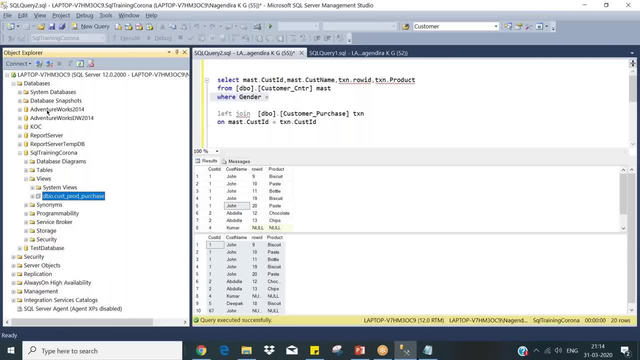 yesterday giving object level security only the what objects you need to do? only a three tables are given for HR manager role or someone has a different user name so you can give access to the views, so he cannot able to do any operations in the view. only a deletion insertion can happen in the table. do is? 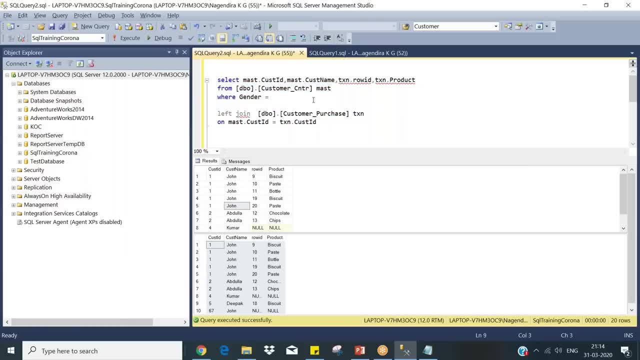 just a query. so that is main purpose of it. it is not only the common, that is also one of the purpose. but you say like you use a hundred to I mean 10 to 15 copies. usually you cannot store it as a view, just the query will be having. 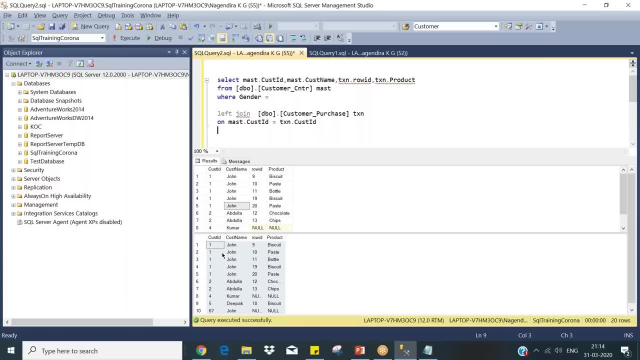 written some useful information always like this. so I want customer product information. then you store it okay and that is main purpose. then you have something like security, security purpose. instead of providing a table access, you give access to the view. that is a too important purpose of creating a view. so, in the view, what you 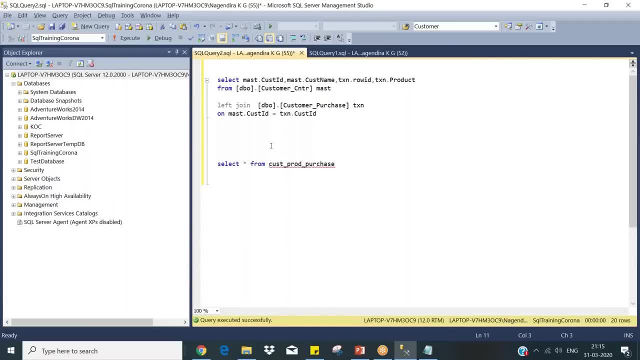 can do, whether you can do a delete or insert. as I said in the table, you can do a delete or insert. as I said in the table, you can do a delete or insert. as I said earlier, it will create one with a virtual table. you can have only the. 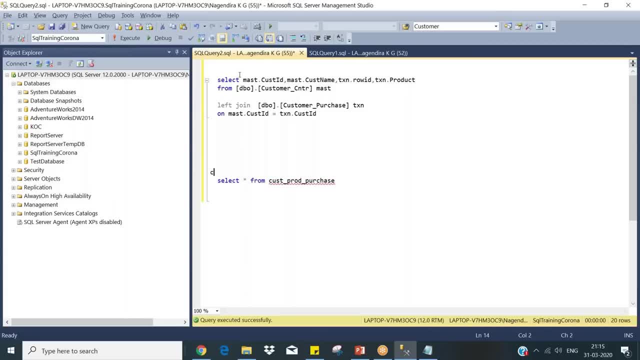 but I mean a selection inside the view. so what about out of a class, create view, customer purchase. this is the customer purchase and you can see the view. that is, I have a customer purchase, select stuff even you can create like this, so this is used for encapsulation, come some kind of? 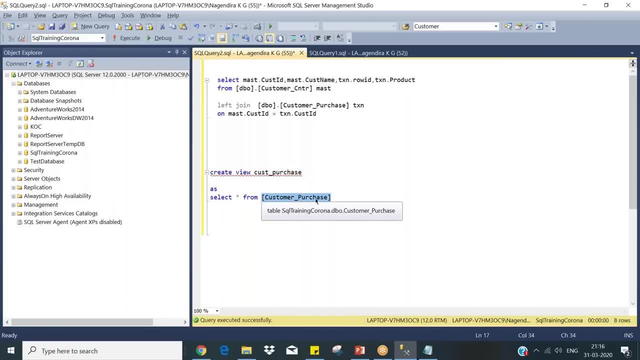 concept: like you have a customer table, customer purpose, and you don't want to expose this table name. instead, you want to clear access to customer purchase. so you are. this is used to hide the base table information. there are multiple purpose for creating a view. so when I create a view, 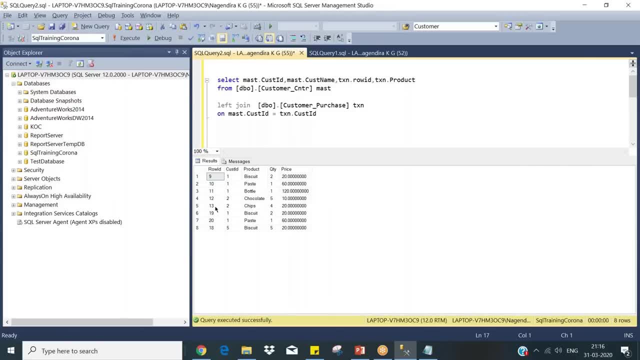 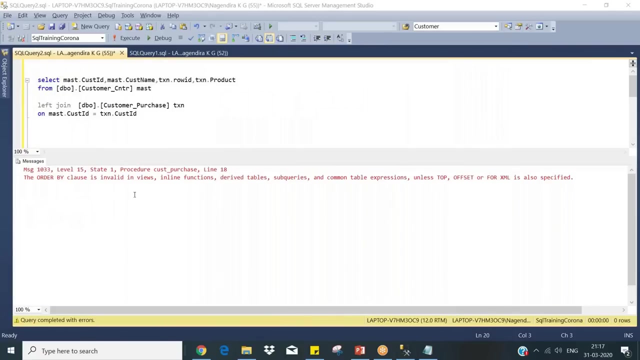 like this only with this table information: select star from based on order. I think it should not allow order by row ID. I don't think it will create. see, this is another very important thing: you cannot specify order by class. inside the views inline function there are tables of. 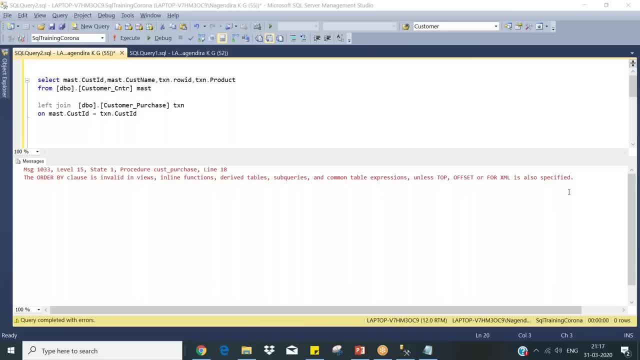 queries, all those things, common table expressions, all other stuff's, because it will show one in the result, whatever order it is fetching. you cannot specify it here, but once you create the view, okay, then you can specify the order select. I will comment it out so that you can understand. so let's start. 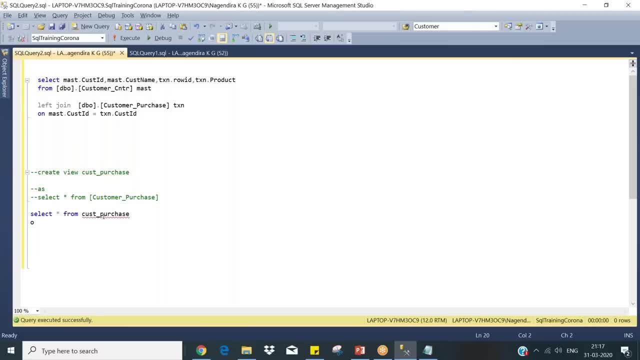 from. I'm selecting from the view. okay, then I can specify the order by row ID. this is simple. I mean, it is as usual. you can specify the order by: okay, because it is storing one day the structure. okay, it will not store what order you need to. 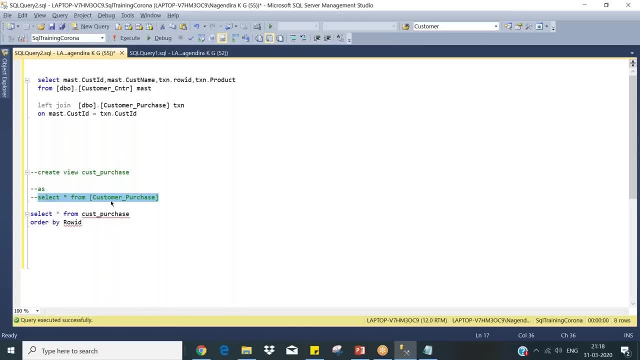 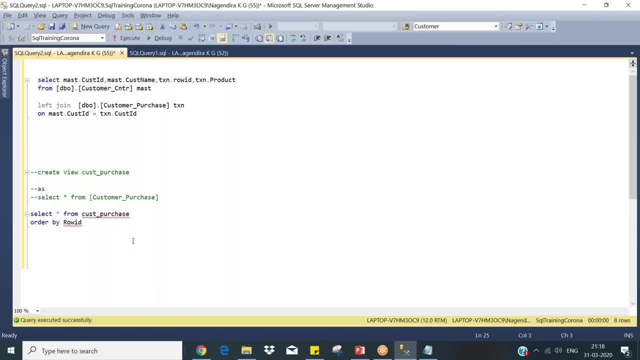 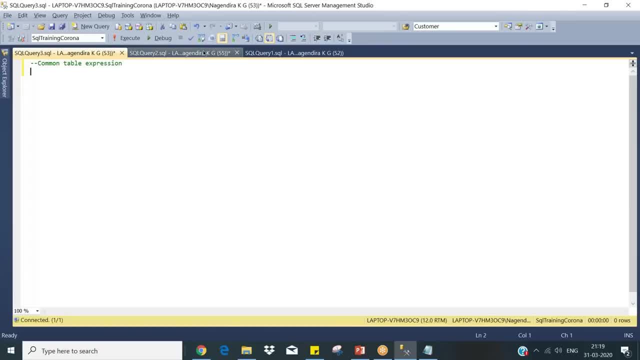 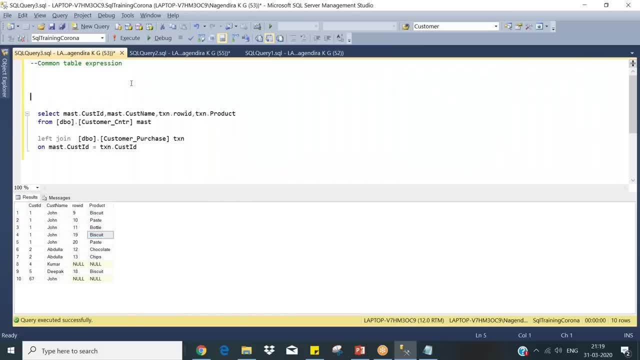 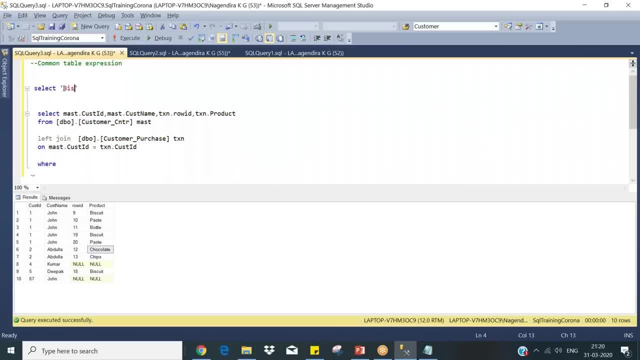 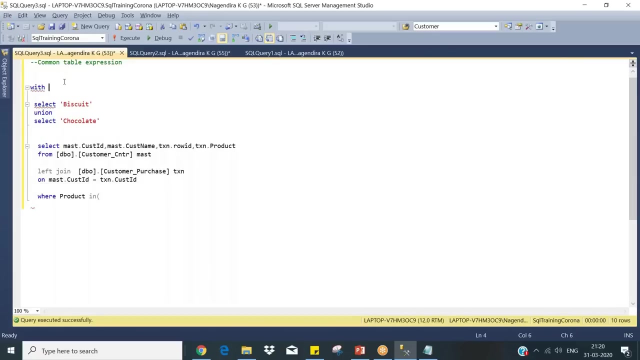 like this. assume you, you need to create some temporary table and those results. you need to filter it over here. okay, where product in with them: product as: so this is a way to create some temporary results. okay, select star from see: see here, if i select this statement, it will throw me error because, whereas when you create 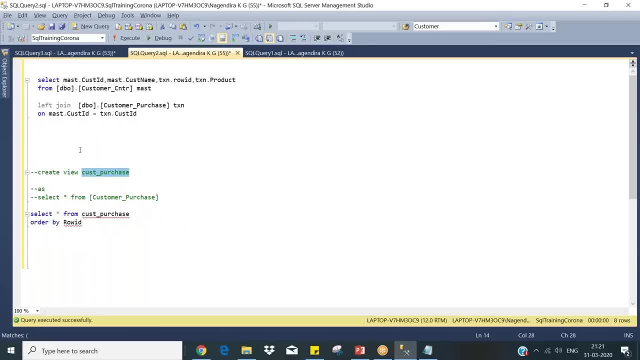 a view. after creation of the view: this is object created in the database. i can able to go and select it. okay, without choosing that. one creation is like: your object is created, the metadata is created, but it's a common table expression. i have this one here. okay, even i do like this. 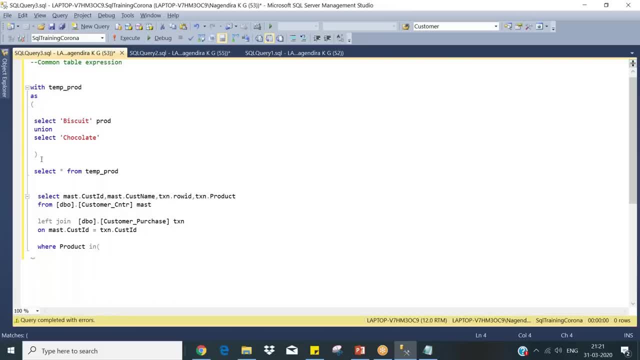 okay, it will throw error because it should have. the width statement should follow with the select statement. you see, here i need to select both with and select statement. the width should followed by a- i mean the select here- statement. okay, so this is the thing, like um, i have created some temporary results. i want to 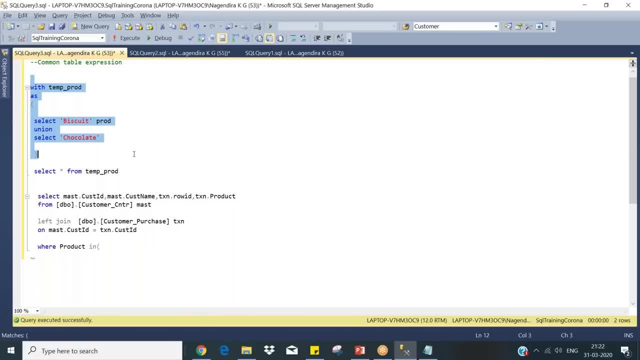 store it. so this is nothing but your common table expression, which will hold some temporary results. this can have any table information. okay, for simplicity, i have created two rows and which is having only one column product. okay, so this result, what i am going to do. this should be. 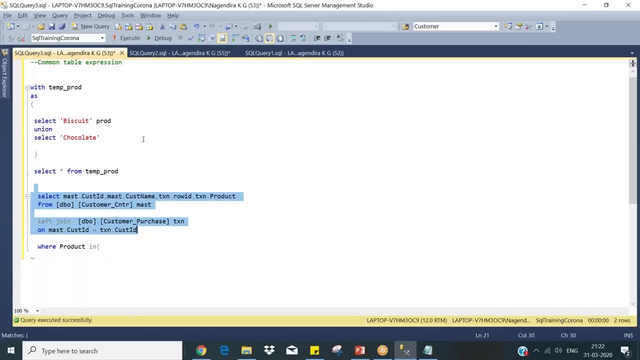 acting as a filters. in this particular table, i want biscuit and chocolates, so select product in. you guys know about uh temporary tables, i mean uh sub queries, select broad from this table. so so N, i need to command it. once i select this, i need to command it. as i said, this scope of this table, this common table expression, is within the next select statement. so i should not use this select statement. i need to use this select statement. i got over purchased biscuits and chocolates. okay, this, this column. i mean uh, this, you can mention it here also. 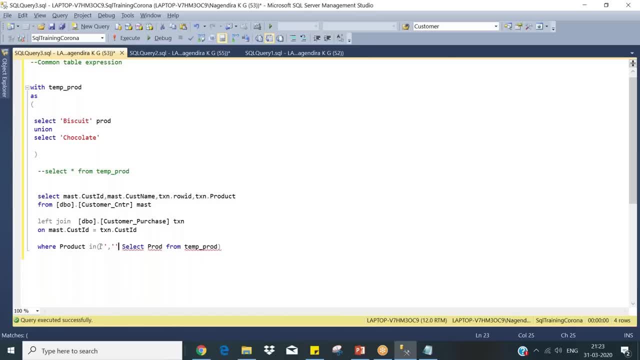 this column. i mean this: you can mention it here also: okay, biscuits and chocolates, something like that. but assume you have- uh, you don't know how many records it's going to fetch. whatever query it's going to fetch here, you remember some queries like whoever has this degree and the employees, whoever has this designation. 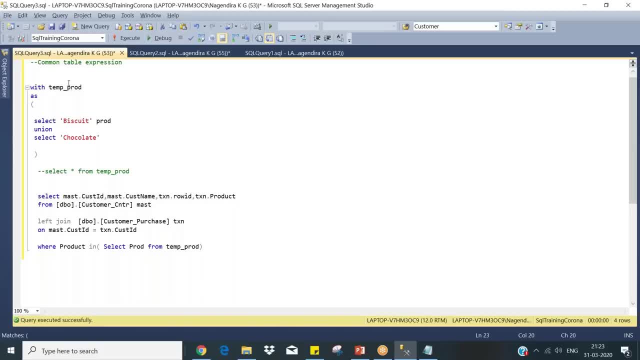 those employees should be filtered, something like that. so in those cases, if we don't predict the account have a discrete values, the result set will be based on the conditions over here. in those cases you can use such a common table expression. okay, so a view and common table. 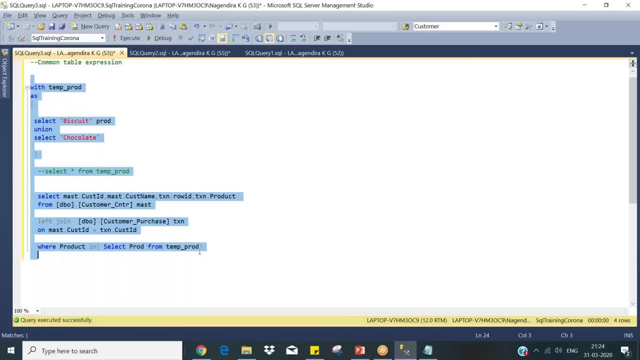 expression is different. this will exist only with this query if i use the same table reference after the select statement. if i run along after the select statement, this will not execute. invalid object name: temp: broad. okay, so that is the scope: scope. you understand, i think, the scope statement. 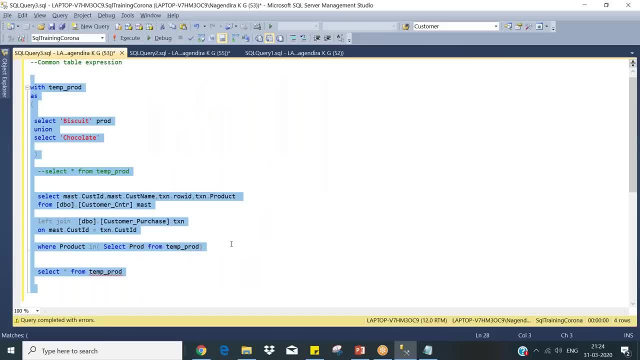 scope of any statement, how long it will exist, whether it's a global or it will last for the session, all those things. someone has a question. this is yuri. union is uh will combine both the select statement, right data, uh union. you include right select biscuit prod union. so this union will combine both the right queries. yes, yes, yes, get the. 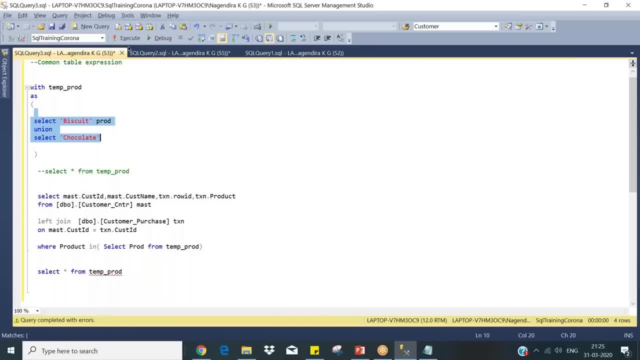 data. yes, yes, yes, it will uh append the rows, amend the rows. this is row one, this row two. maybe you for confusion, i'll put it as id: yesterday, i think, union and all i taken last session. so so this is uh first and second. forget about the union part. 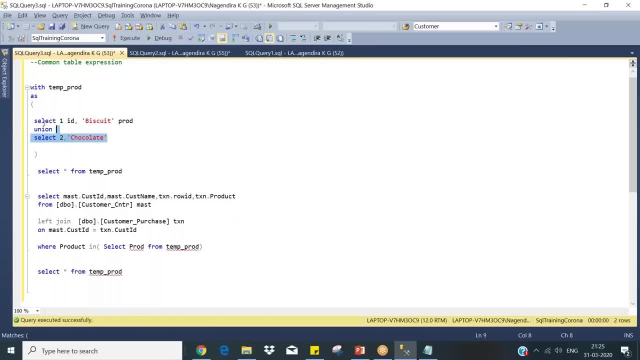 just uh. i mean, uh, you, you still have a contribution with union, how it works. no, no, just uh. okay, now the focus should be on the common table expression. this is a with okay, the view definition. you just try to compare it with a view and a common table expression. view is permanently stood in. the database. that is common table instruction. the scope is kind of tested and if there is no common table expression, which you never need to if your systemSo марina does really well because if there is a common person in the service pages in the database and you in the practice, if possible. but if you could shift to last table expression, the view detail fx. 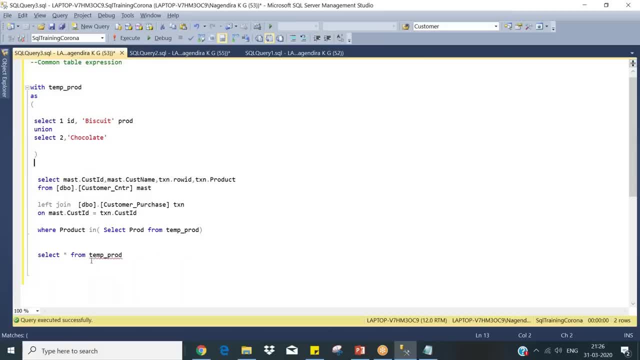 is within the next select statement. even if you use here, this won't work, but whereas if it is a view, you can create it as a view. if i change this one as a view now you have seen like this: result: you got result for this query. you got error for this select statement. 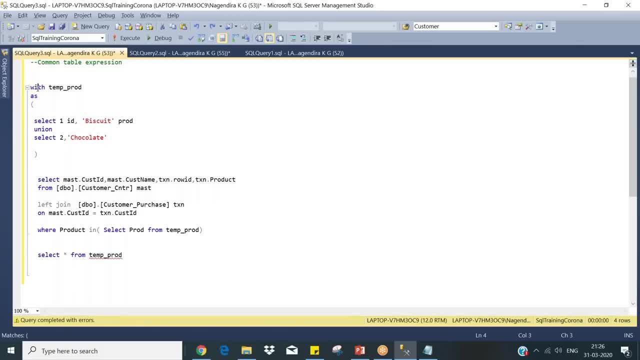 and error over here. okay, what happens if i create it as a view? create view. okay, even you can do like this view. first you need to create. you cannot take you along with this. just execute with that. two select statements. now you got the output. okay, this is the main purpose. when to use, when not to use. 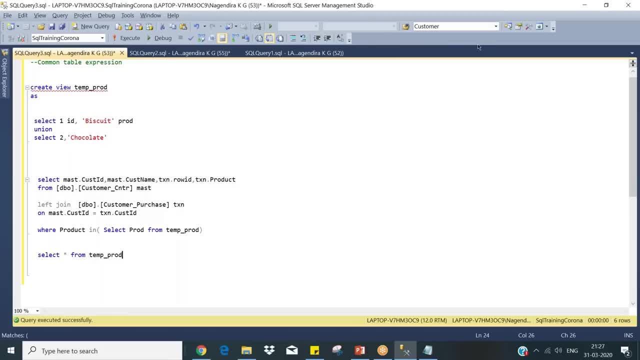 okay, now there is something like common table expression, similar to that. you have something like temp tables, temp tables. okay, there are two types, i think. for now, i think you can stick to two: uh, hash table, hash table, has table is nothing but local temp table and hash dash table is nothing but a global temp table. 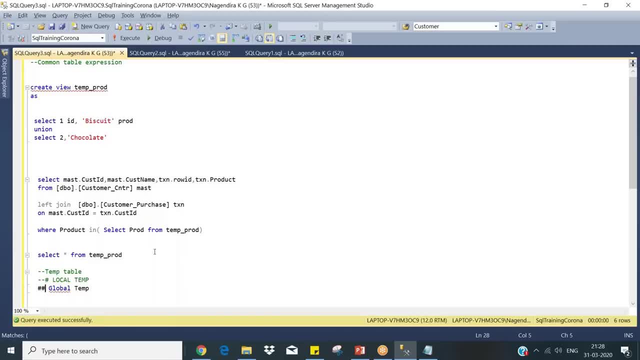 global temp. so what is those? so all these things, guys? uh, the temp table purpose is: the table purpose is to store your results temporarily and when, while the purpose of the table is met, then you can drop the tables. that is the main purpose. so till now we have seen like this can: 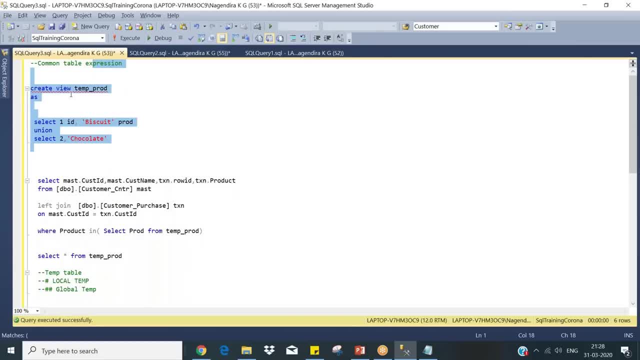 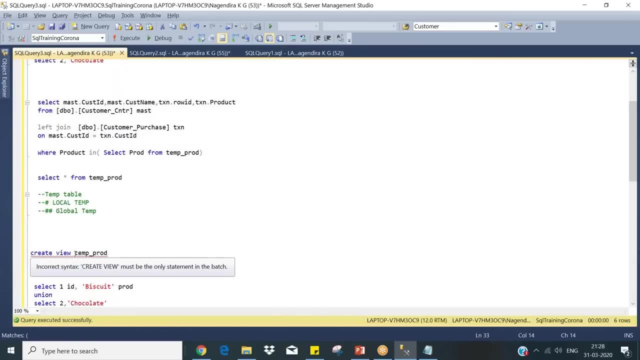 be stored in a view. this can be stored in a cte. now i'm going to store this result in temp table, so let's look at the table. so now, if we see that i can store the results of the table, so let's go to the list and i have a table. 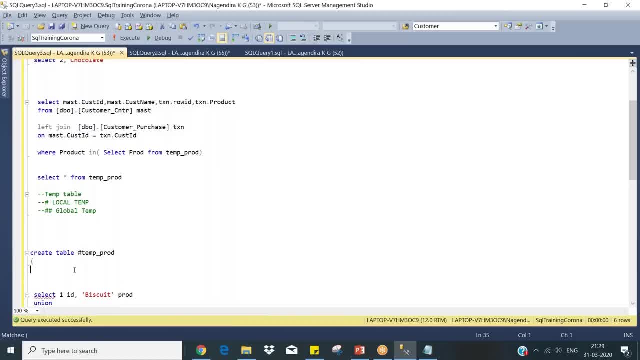 so let's see if i can store the results of the table. so ID and you say product integer. save a care of one thing, okay, I can. I am going to create another table and say global temp product and prefix with hash hash. so this is the one. now let us insert these two records. 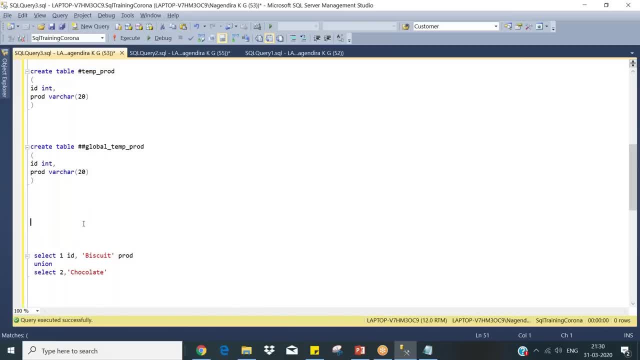 so this is the one. now let us insert these two records. so this is the one. now let us insert these two records. have a template table insert into? okay, it is as simple as that. let us insert for global table as well. okay, okay, okay, okay, okay, okay. 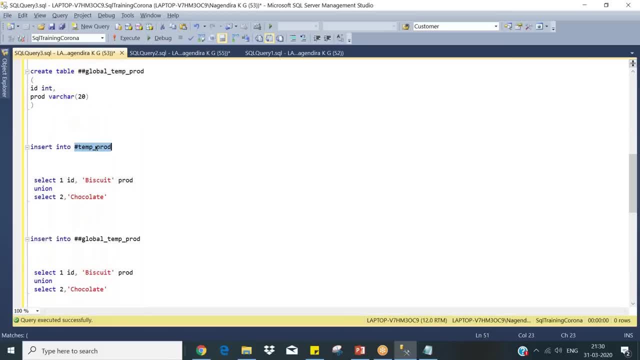 so what is the difference? why? when to use when you should not use global, when to use local, those things I will explain shortly. you both have data, okay, here. now I will take this guy, this local temporary table, and put it in a new session. there is see, whatever you create a new query here, okay, that will. 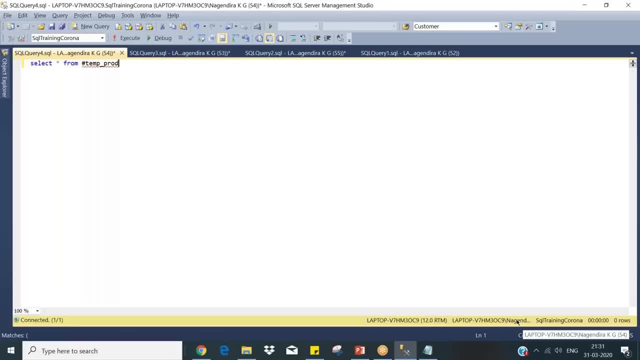 have ID. if you can see at right end bottom when I highlight there is a number after my name- 54- then over here it is 53. this is nothing but 53, 54 and all session IDs. okay, so you have created this local temporary variable in session 53. you cannot go and access this temporary table. 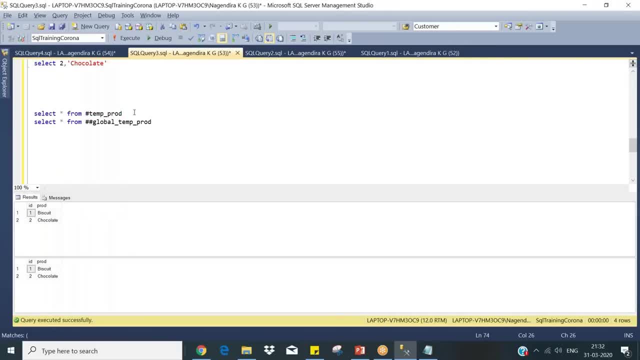 in another session but you can access within the same session. so the scope of local temporary variable is within same session, whereas hashes table I created here in session 53 I can go and access in a new session. okay, so this temporary table and global temporary table once. 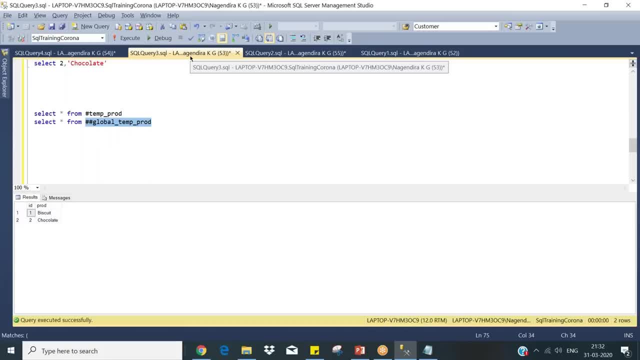 you drop wherever you are created. once you close this guy- okay this session- then these temporary tables will be dropped automatically so I can drop it manually. also drop table like this table. so the all other operations are tearing a table or whatever operations you performed in the table. those operations you can do it in this table. 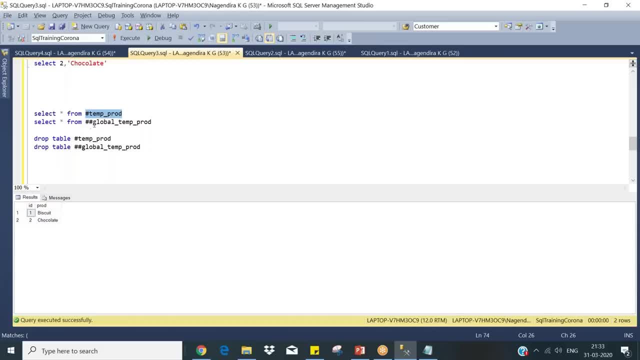 the only purpose is to store your results temporarily, okay, and sometimes you can send some data to a table and you can store it in the table, okay, so sometimes you can send some data to a table and you can store it in the table. so where you will use? okay, basically, let me answer this question. so, basically, you have next. next i'm. 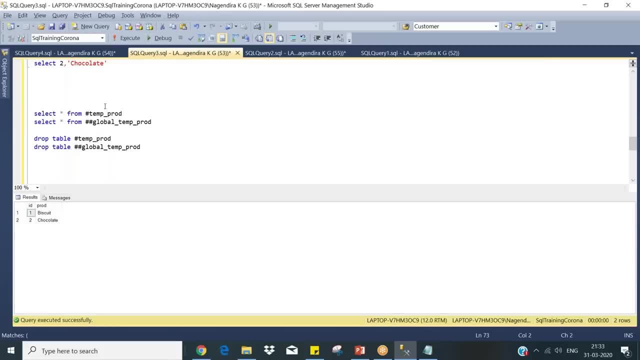 going to talk about the stored procedure, where you keep calling one procedure from another procedure and sometimes what happens, based on different applications, you you call some data called in one session should be accessed in another session, okay, and in the in those cases, and that results should be stored temporarily. so in those cases you will use global and some cases like within. 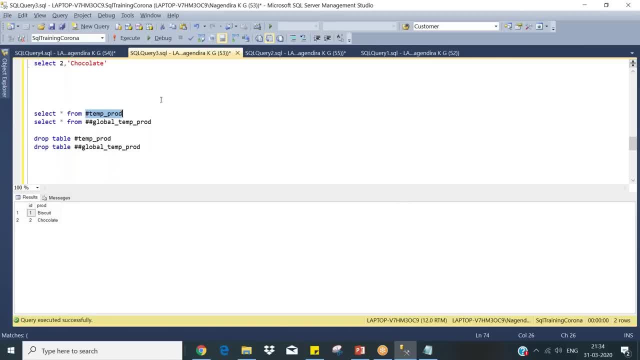 the procedure or within the execution of the batch. okay, all these things. when I go and execute as a whole query, it is called batch running. when I run, the batch starts from go, when you have a go statement, from this go statement, whatever statements you execute, it is as a batch okay. 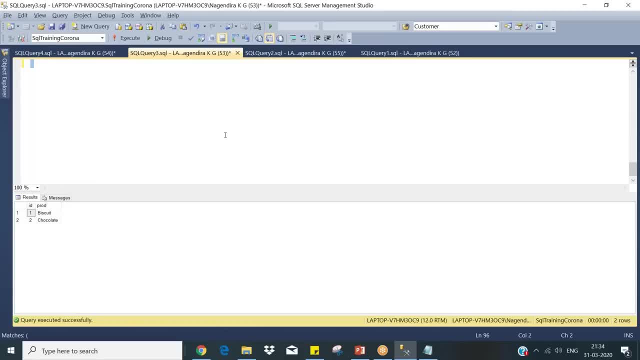 in procedures you use go statement, so within that go statement it's running as a batch that will create one session. so you have scope. should exist within that batch our session, then you will use local variable and your data should reside for other sessions. I mean, you will use local variable and your data should reside for other sessions. I mean 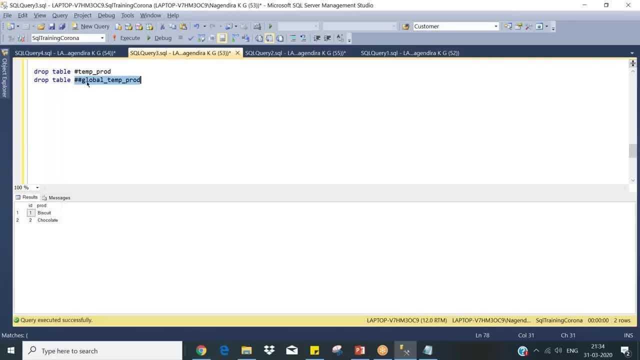 should be available for other sessions, then you need to use global temporary. should be available for other sessions, then you need to use global temporary wave. mostly we will use this one because our logics is not so that complex, so this wave. mostly we will use this one because our logics is not so that complex, so this. 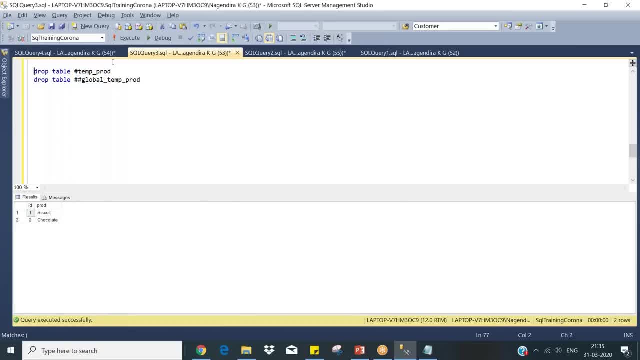 is good to know and what is the purpose of common table expression that is used is good to know and what is the purpose of common table expression that is used to store small results. basically, there is a memory logic behind all these three: to store small results. basically, there is a memory logic behind all these three. 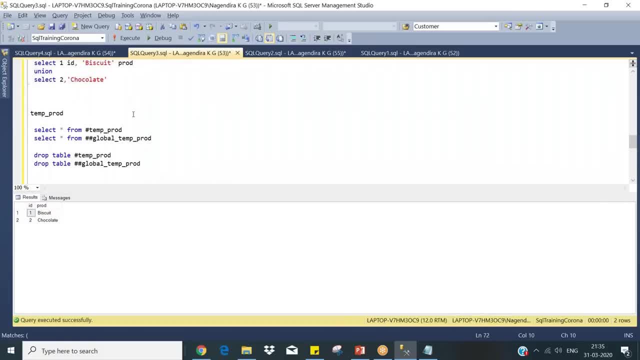 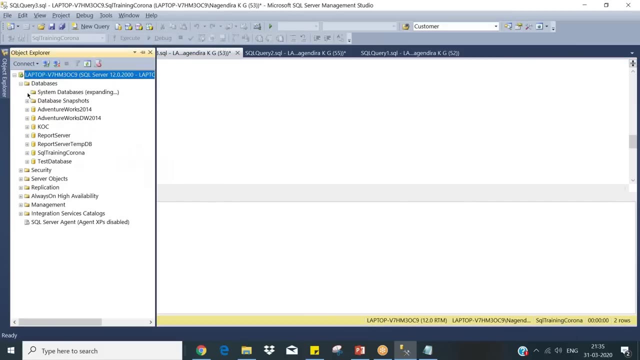 local, global and this is your city. okay, there are some memory requirements. this temporary product and temporary tables. there are some memory requirements. this temporary product and temporary tables is stored in your system databases- stem DBs. I think it will have somewhere over. is stored in your system databases- stem DBs. I think it will have somewhere over. 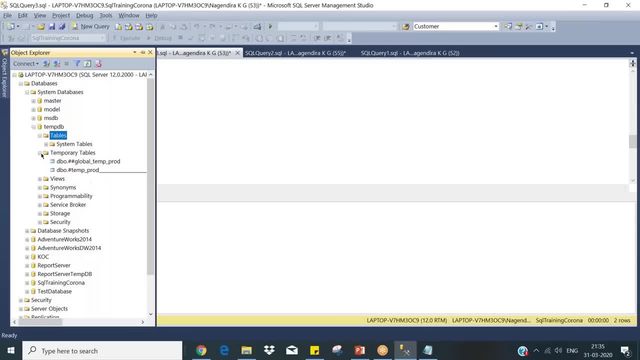 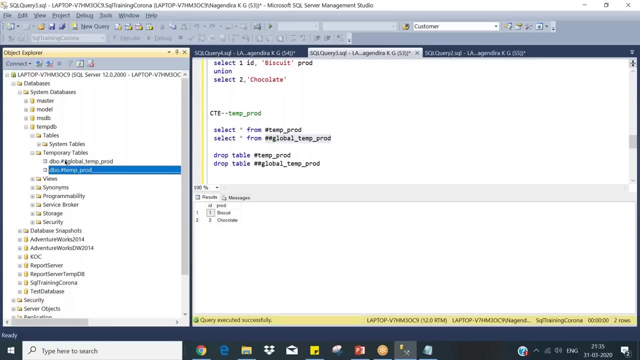 here, uh, temporary tables, see global temp prod. global temp prod. so it will be stored in your, as i mentioned earlier. what are the system database? you have a master model, msdb, temp db. so when you create a temp db here, it will create a temporary tables here. so physically physical. 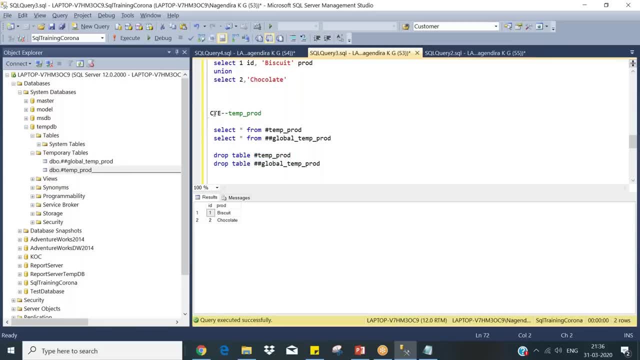 table is created okay, whereas in cte you don't create a physical table anywhere in the database. that is the main difference. so you might ask why i need to use temporary tables. instead, i can show the results in cte within the scope, so usually if the volume is huge, that requires some storage. 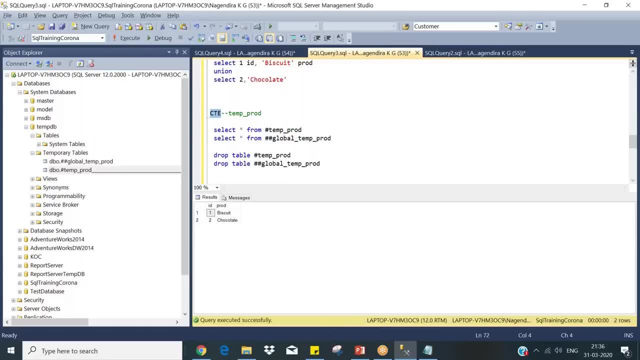 go for local temporary variable. otherwise if you run it on the cte it will be stored in ram. so whichever doesn't be stored in a database physically, these things will be stored in ram. so better avoid it. your system performance will reduce. say, for example, if you are storing more than one million record, don't. 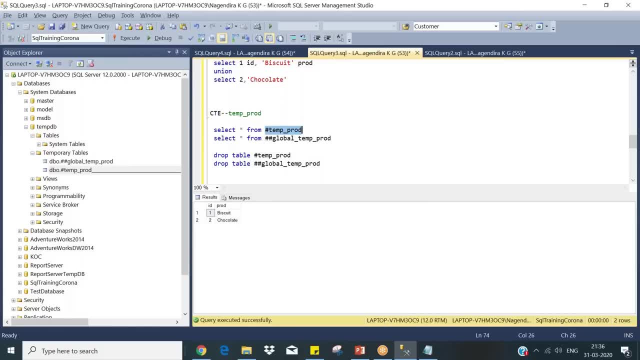 go for ct. instead, you should show for temporary tables. such cases you need to take a call based on that, okay, and if your temporary table should be accessed by different sessions, go for global temporary tables. all right guys, any doubts in this? no, okay, fine, let me proceed to stored procedure. 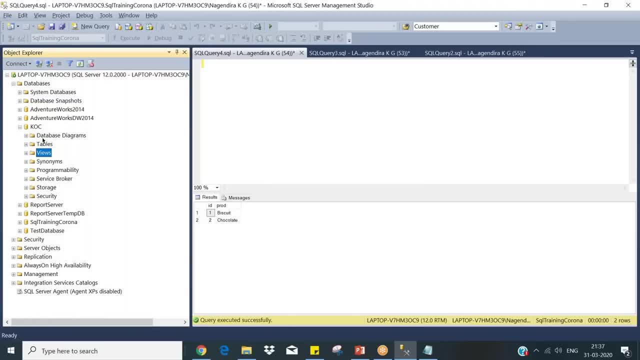 so we've seen about these tables, views, the purpose of views, your all your predefined queries and used for security purposes as well. now let's go little on programming part, like the stored procedures and functions, all those things. let's start with the stored procedure first. so, similarly, you have your queries written. 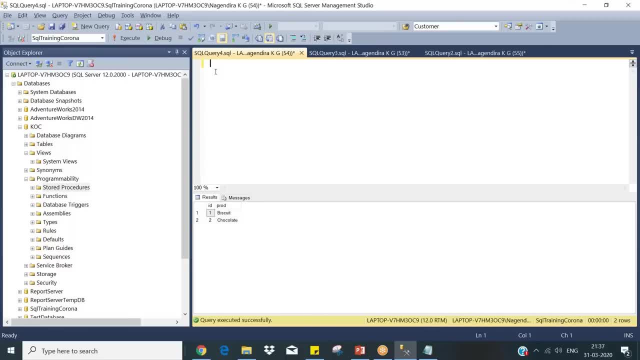 okay, in the views you have only select statement. what happens when i have some uh data querying or data manipulation language? i need to frequently update one particular record: customer information. okay, whenever i receive in the forms you have like, as we discussed earlier how the data will get into a database from. 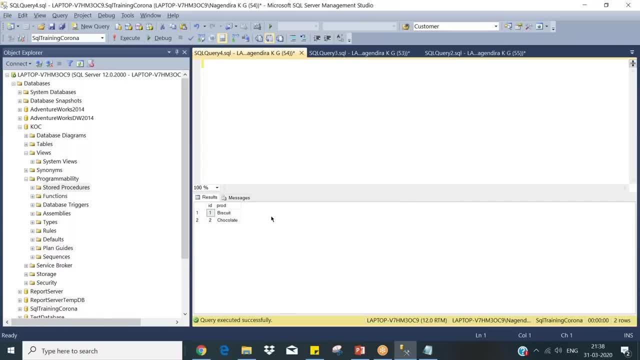 business perspective. you have forms in front end. they create a customer, they press button, insert, or i mean submit. you will get insert into statement, into the table. similarly, sometimes, like when i want to do change in my customer information. so what we need to do, we need to do the update correct. so 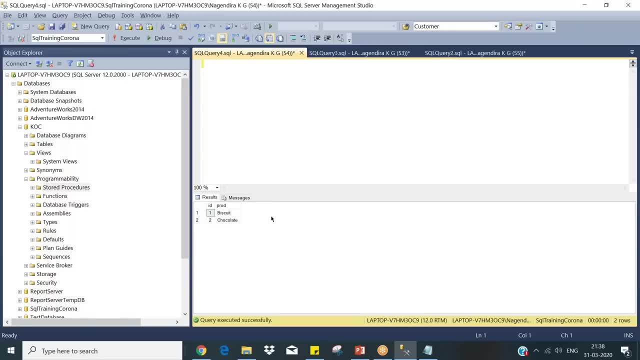 update each time. you cannot run one code. i mean, uh, that stupid. i mean that piece of code is by default. what you need to pass during the data check and update means that, and when you can do it in the state, you do not have to give a update after the data check is done. 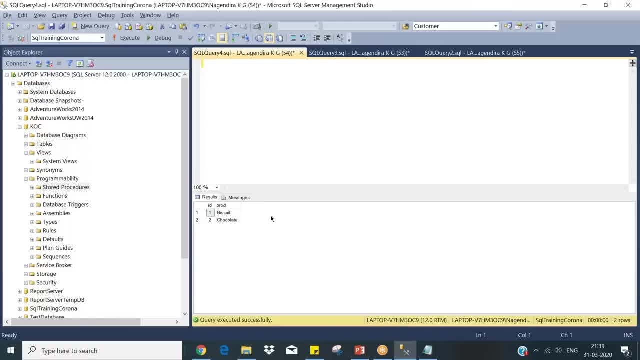 that piece of code is, by default, what you need to pass. usually people will update a phone number, people will update address. so what information you need to update phone number or address based on what you need to update customer id. so this is a predefined structure and i'm going to repeat for n number of customers. if i write a code once, basing 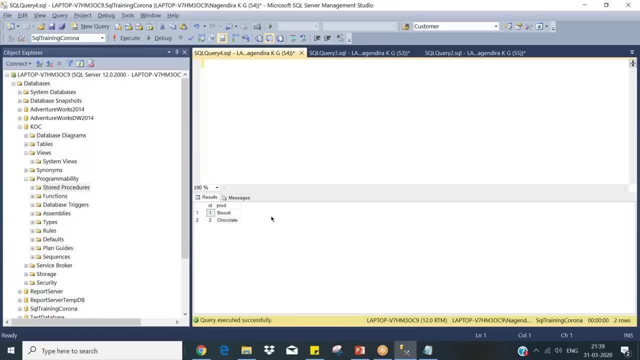 passing parameters, then customer information will be updated just passing a parameter. so these kind of scenarios, you create that code in a procedure. okay, that is what the one of the main purpose. you go for a procedure, repeated task. you want to do that code to be executed every time some operation happens. then you go for a procedure. let's have the same uh. 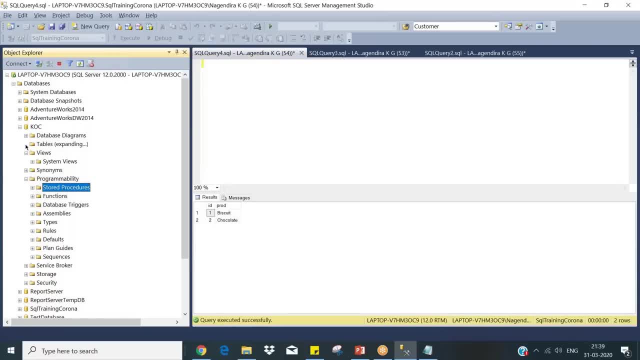 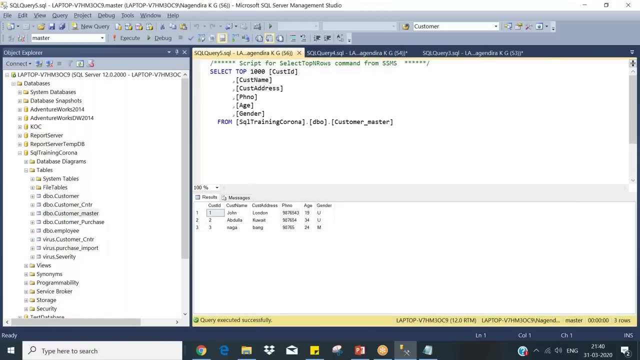 example, now i'm going to update uh customer information, sql training, corona, customer master. okay, here what i'm going to do: i give a customer id, okay, i i will pass customer address and phone number, okay, when i change any of this information, my information should get updated. so how to update? usually, 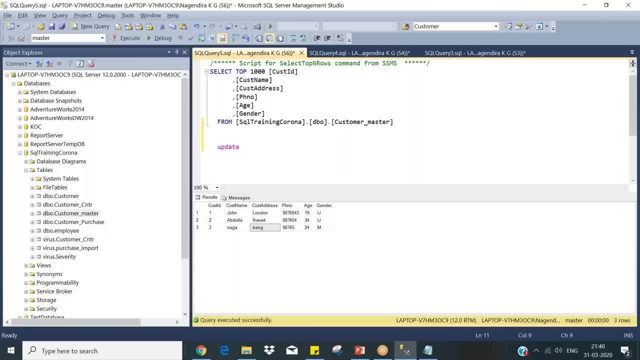 we write update query right. update customer master, set customer address. for simplicity, i will go for a customer address update. for now, okay, and we can focus on another parameter later. customer address: i will say like: um, i have bangalore. i moved to chennai where customer id equal to three, so what it does, it does like for uh naga, you update the. 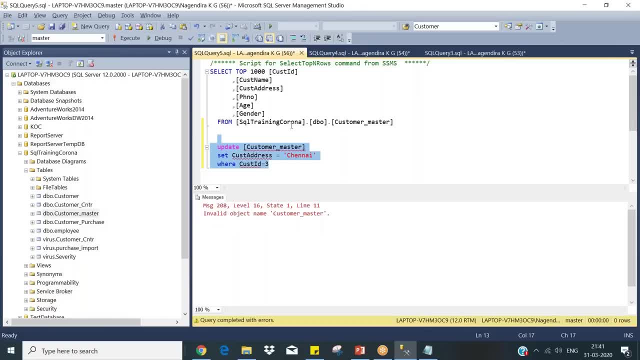 customer address to chennai. let us try that. for example, i moved to bangalore. i reached it on bangalore. i received a phone call from the inside why i am not in a correct database. okay, this is the thing now. you see the same information now from naga. it's moved to chennai. 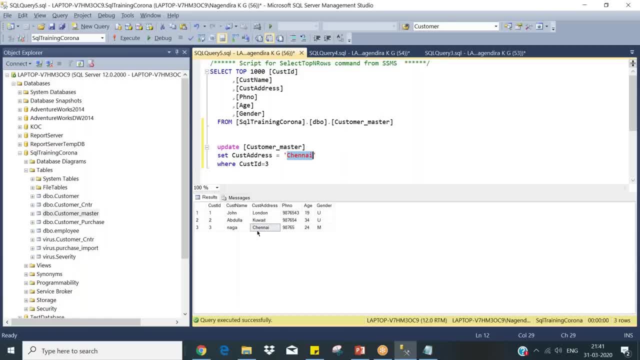 now you got it right. earlier it was bangalore, now you are moving to bangalore. so why did you update your work page? you actually want to go to bangalore. you are in bangalore. in you updated to chennai now. now this is a repeated task. people will keep updating the location phone. 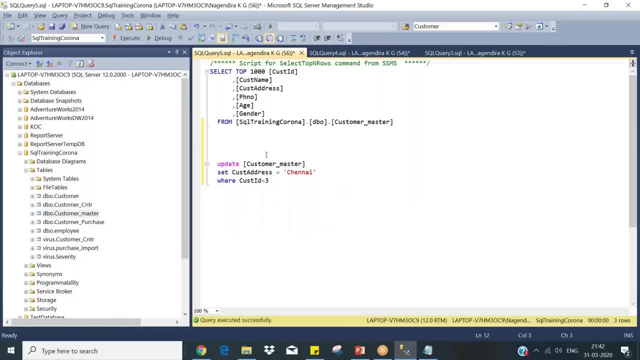 number, all those things. so this is the statement i want to execute each time when there is an update: okay. so such a scenario is what i will do: create procedure, procedure, customer update- okay, and the procedure- if you can have any without any parameters- also okay. if you keep like this. 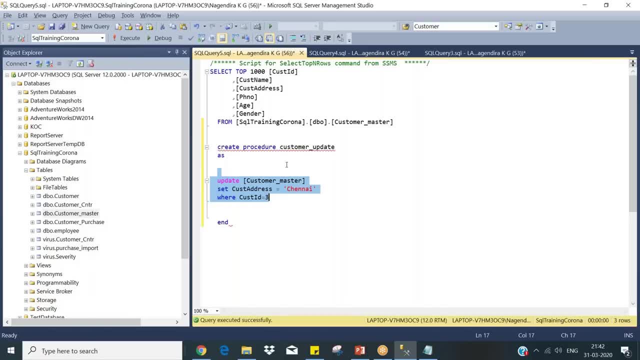 it doesn't get any information about the customer or what values to update. so you need to create a parameter here at customer id. okay, so remember the symbol that indicates a viewer variable. okay, at customer id comma at address you need to define um, the data type of. obviously, okay, what is the data type of? master? 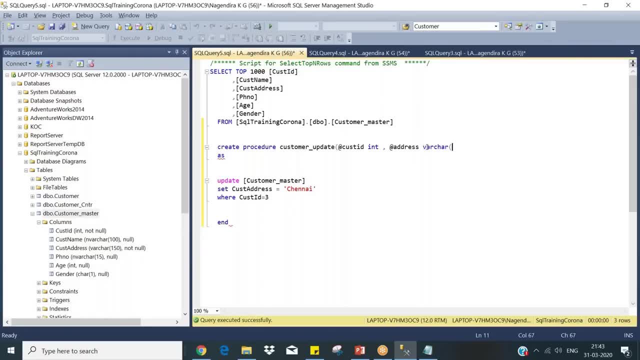 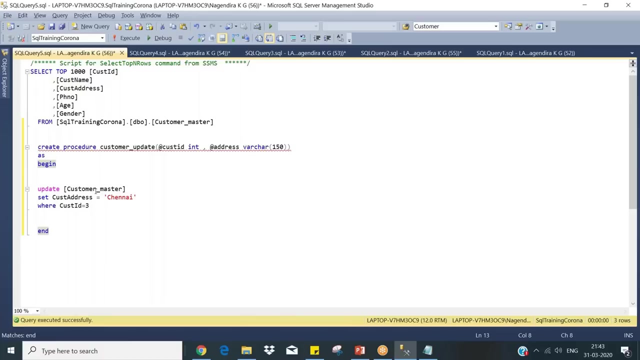 and worker keep same as whatever you mentioned. okay, so the procedure, create procedure, procedure name with parameters. then begin, okay, begin should be the thing, then end, okay, guys. so now i have given these two things now here, then okay. next is question: whatever values are getting it over here should be updated here. okay, that is. 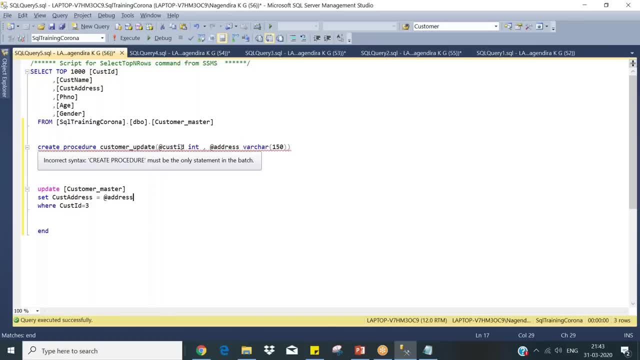 what- replacing the hardcoded value with whatever you pass. got it guys. so this is, yeah, see if i have a hardcoded value here. okay, let us see. like the main purpose of creating these wasnt centered on the icon. these are the values that are needed in order to get them. it might be called hardcoded values and how it is that. okay, well, i have said so in the other things. again, those the two. they are increasing tasks i have, so these are going to do that because i have. otherwise, if you pass whatever they are missing, you will receive that. if you anyren to no, i Cos 2 will have the 거야 error. so mostly worked on this one in localization setting. this is how we did so. okay, so what? you哀 sorry, can i add something else to it? okay, what would you do to free you that? you got it guys. 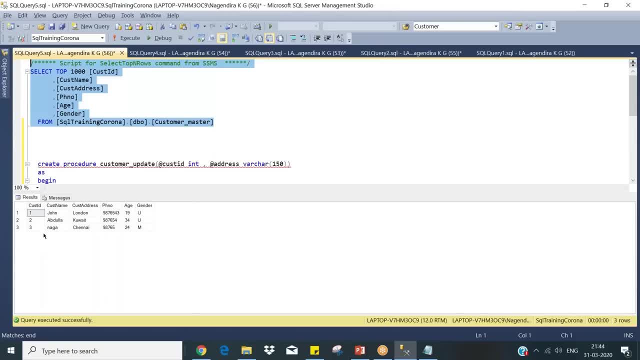 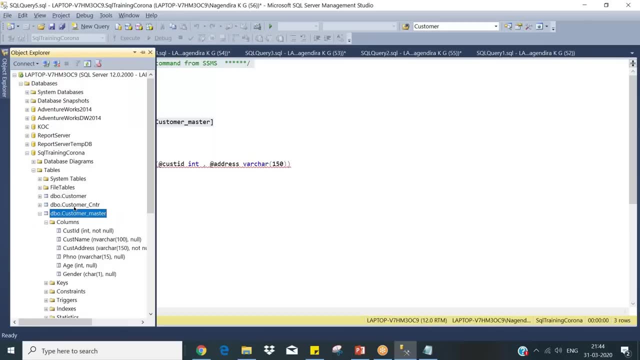 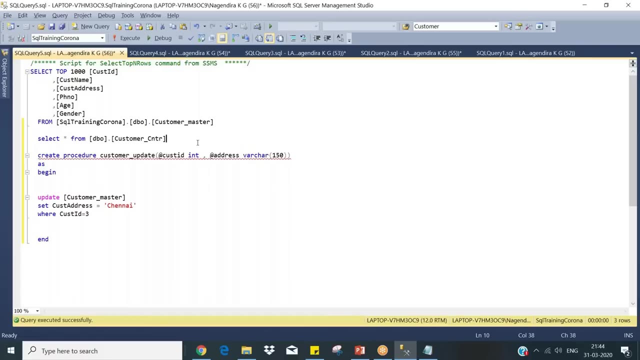 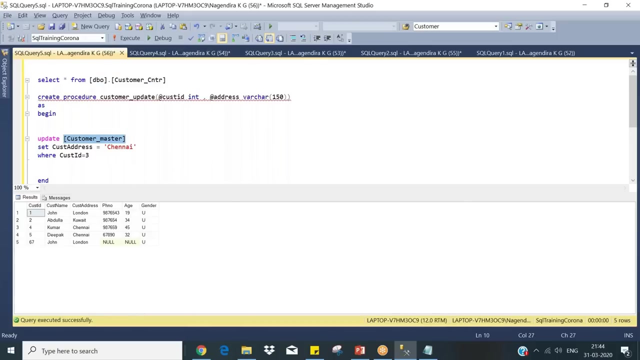 a procedure is like: there are number of customers over here. okay, maybe I will take. someone has huge data, six to seven records. okay, here you have five records. this is for better. I'll take this. David, see, you assume you have. we have a customer data. you have thousands of ten thousands of customers, okay. so basically, we want to update the phone. 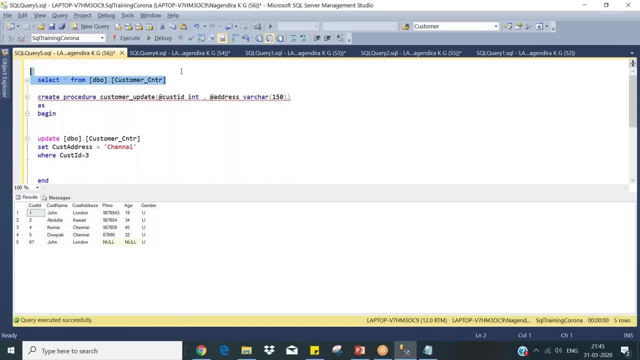 number, customer address frequently. so how you will do it: people enter in the screen in the GUI front end, then you capture those value. whatever you want to modify, you will capture that value and for you whom you want to apply for that particular customer. so obviously in a customer. 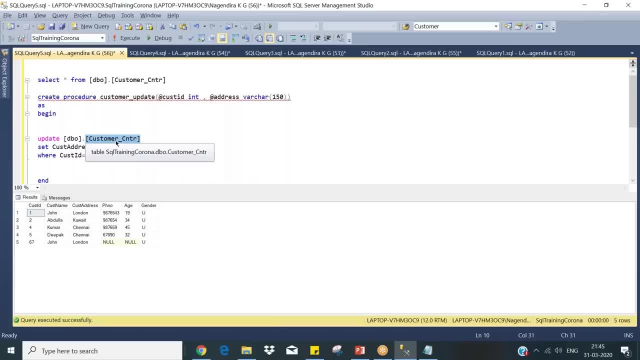 table only you want to apply. so you need to get these two information: what information you need to update. that is, for now it's an address and for whom you want to update, for whom is customer id. so these two things are very crucial things that you need to capture from the input system. okay, 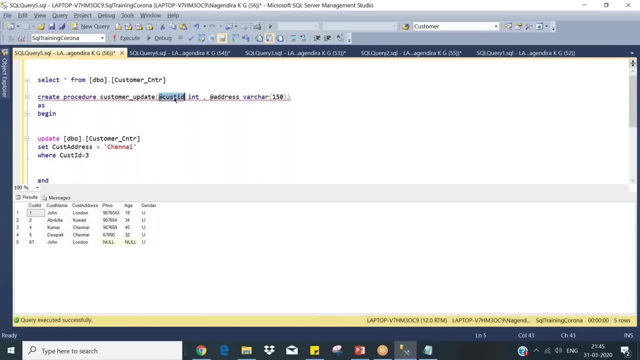 that will update it. okay, based on that only, we will update. so earlier what I did here is for customer id three. when I want to update, for now there is no three. when I want to update for Kumar, now he is in Chennai, when I want to, he is changed to Bangalore. I need to write Bangalore, so assume like you. 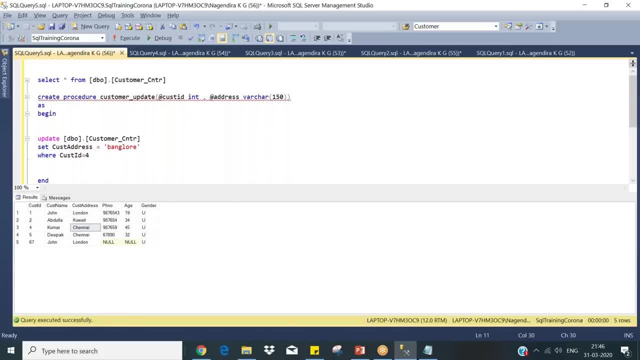 keep on storing this information. what you want to update, then you are not going to update it manually, should not do it, because you have 10 000 customers. you cannot have it one by one. okay, instead, what we are doing, we have written a procedure, programmatic approach, where you get those information. customer. 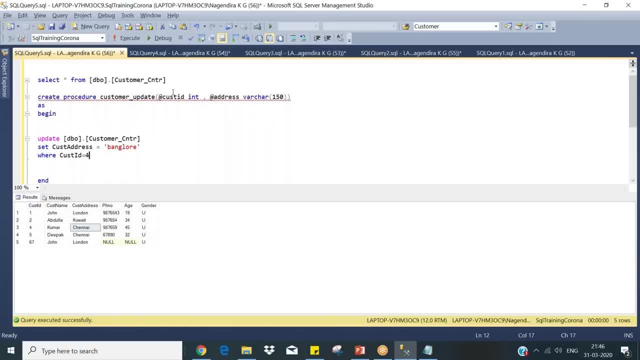 id and address and in this place you replace those values instead of four. see now. first i will update for kumar. i will update to bangalore. so how i can do it programmatically i will pass four and bangalore here. okay, in this customer id in bangalore. so this should update me. 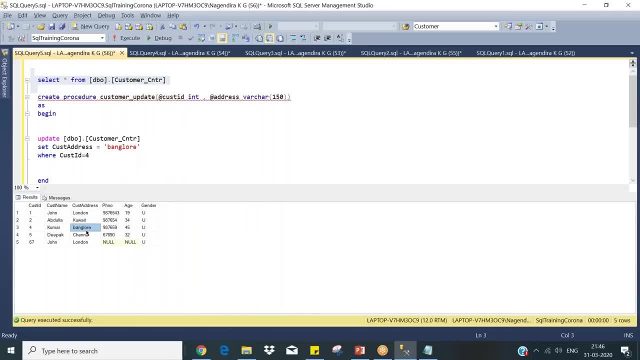 that bangalore information. now you see he already changed to bangalore. now i say he moved to delhi, kumar moved to delhi. so i i should not make it dynamically. sure, in order to make it dynamically for any customer i change, i should not hard code it. so just replace these two values the hardcoded values. 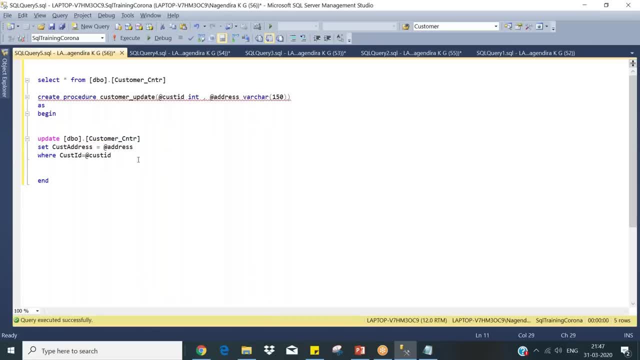 wherever you wish and whatever values you are getting as input, you put it here. now i create this procedure. okay, now you see the value here. now: one, two, three, one, two, four, five, seven. now i want to update deepak from chennai to delhi. i can use this procedure. 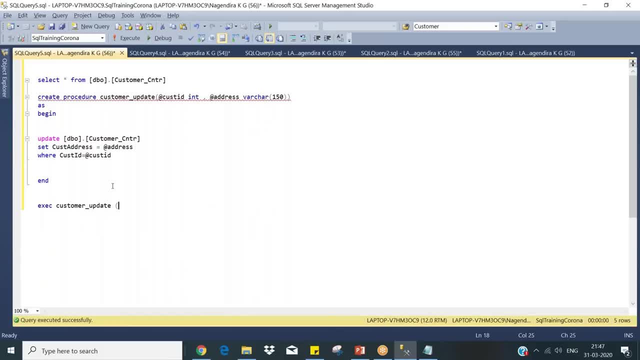 execute. you give a values, like you need to give the value five comma. deepak: i want to change him to delhi. now i'm not running the update scriptment, i am running this procedure now done so. you see, deepak was in chennai. now he got updated to delhi. 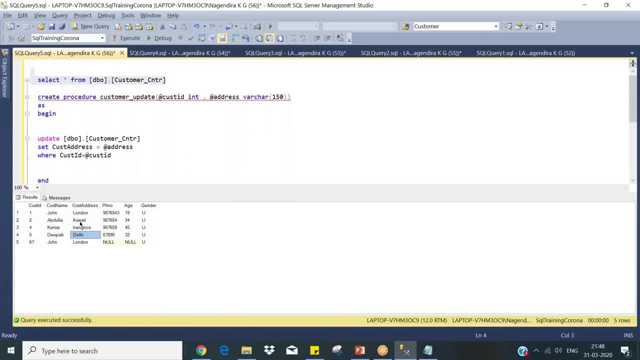 now, you want to do it for abdullah? he's in kuwait. i will move him to delhi. abdullah is two. i will move him to somewhere else. i will say: africa. you see, guys, abdullah is in kuwait. i'm just passing it here. but 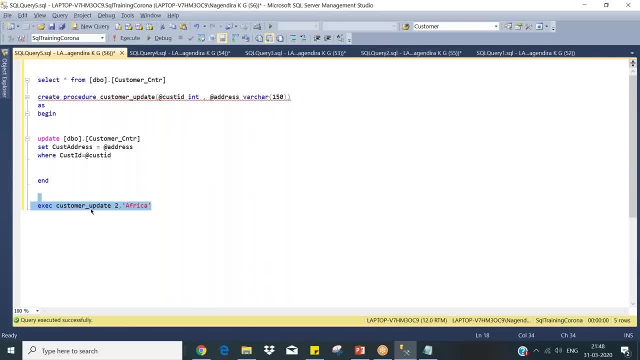 how it get. uh, this is not referring any table. i'm just calling this procedure to africa, the logic, whatever i've written here that updates the Abdullah to Africa. You got it, guys. Any doubts? So this is, this is how you need to create. 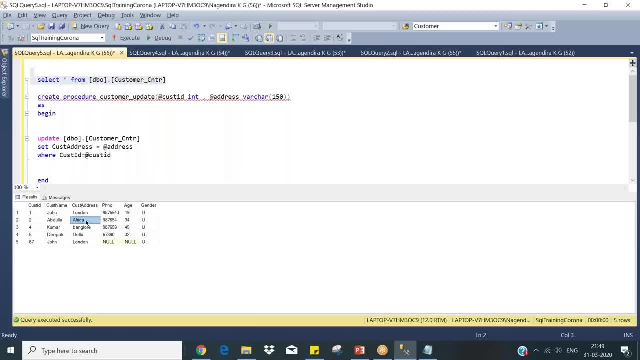 This is the main purpose. You go for a procedure, any kind of operations that will perform your data manipulation: language updates, deletes, inserts, regular inserts. So into a table those things. you store it in a procedure. So all applications, your Windows forms, Web. 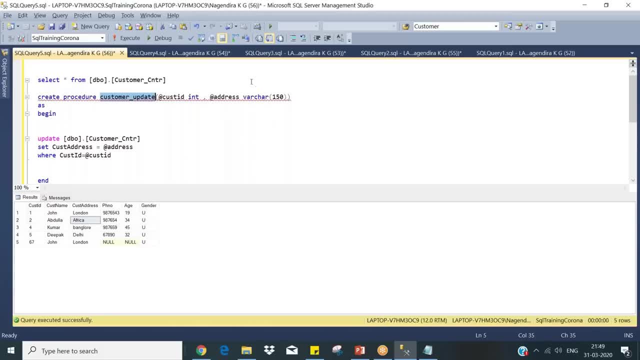 forms will access to this procedure. They will pass their parameters, like customer idea or customer name, whatever the key attribute that will pass in this parameters. So they will capture it here. Then it will be passed here. This is the thing, guys, so you can do. 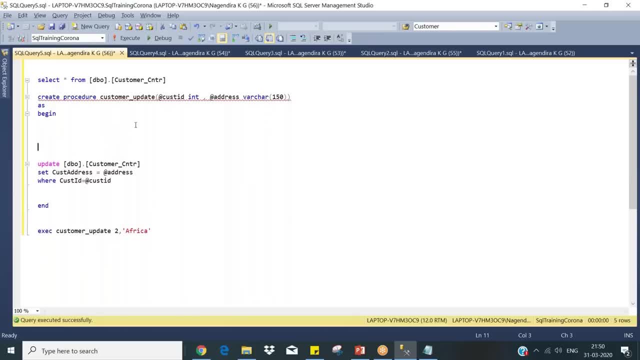 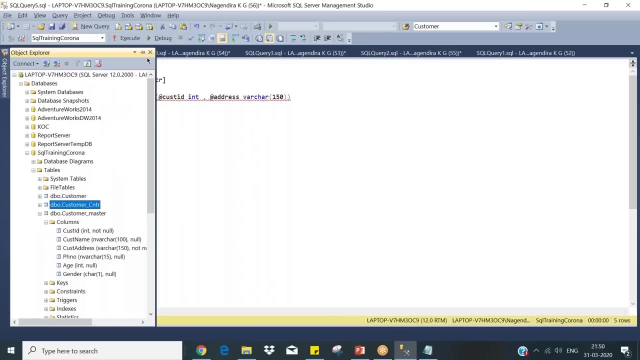 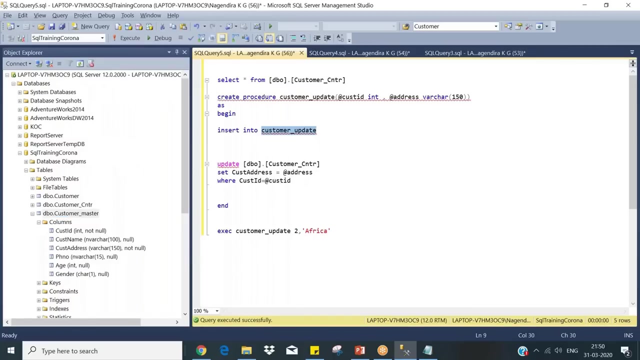 any operations here Even can use the same statement here for logging also, so it is not only one statement. insert into customer master. I'm passing here I can do a log, so multiple statements you can do. insert into select what are the columns? only a name is not. 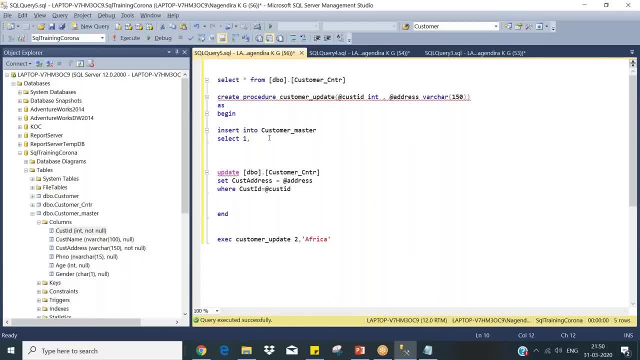 the one is that no, so I have only this information here. one I mean customer ID comma and this. so how? so now I have created the procedure earlier. now I'm changing some logic incentives. this is the logic change. earlier I had only update, so now I'm changing little logic. so it's. 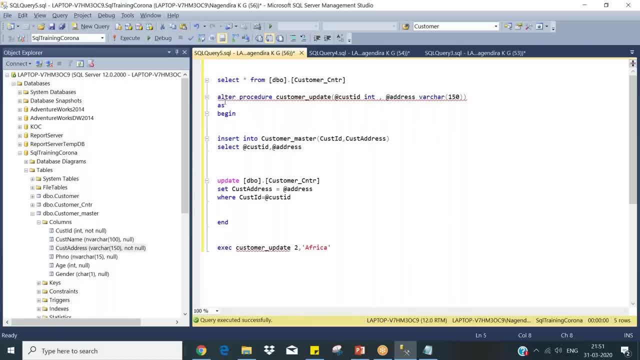 the command is as usual. you are changing the structure, just create a new and change the create to alter. alter procedure, procedure name: same thing, just use this one now. you see, i have two tables now: select star from customer control, customer master. okay, now i got these two tables. now i will say for john 67: i'm changing him to london, to. 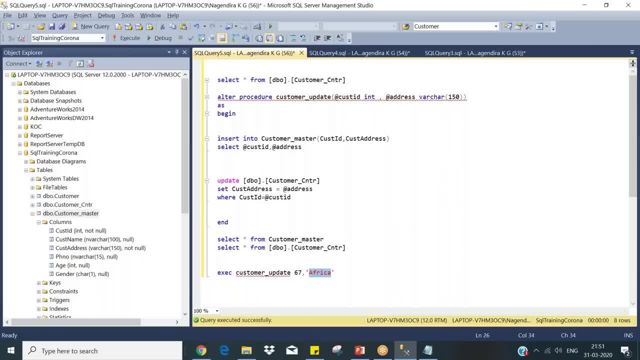 67. first, i pass 67 to london to. i'll say uae. now what happens earlier? whatever we did changes. there is no entry here now. i made a logic to insert entry into customer master as well. customer master: only two columns will be inserted: id and address. there won't be any names. okay, just for your understanding, it's. 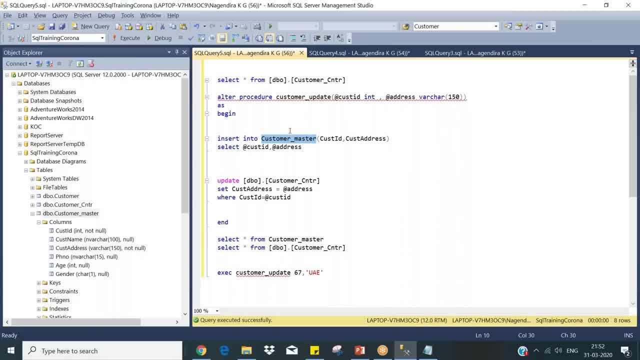 not a proper way, but still so. for 67 uae will be inserted first, then for john uae will be available here. that is the expected output. let us execute this. you see one row affected. one row affected inside. what rows affected? it will be replicated in your result set. now select the data. 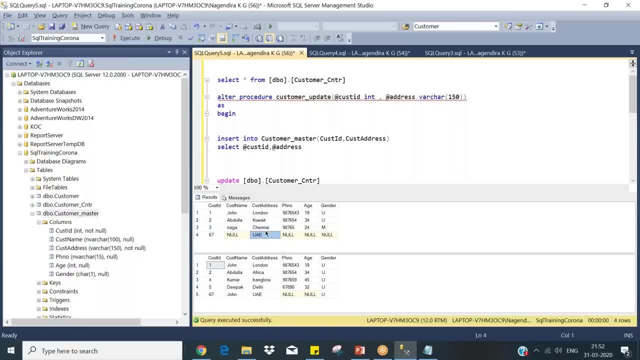 so now you see here another entry in customer master table 67, uae, and for john, we have changed to. the address is changed, okay. so this is the thing, guys, uh about uh procedure. it's a very simple as that and something like we can have a set no count, set row count on something. 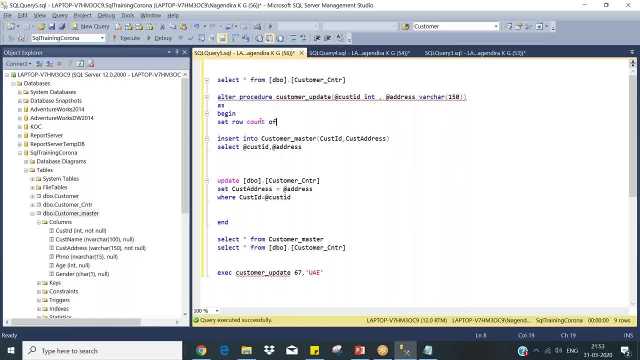 row count on off. there is some function that will say like no count or something. this is the. this is useful. like no count of no count on. so this is useful when you have. so there is a cast involved when you run this query. i mean earlier, you see, like row counts on. i mean one rows affected, one rows affected. message was: 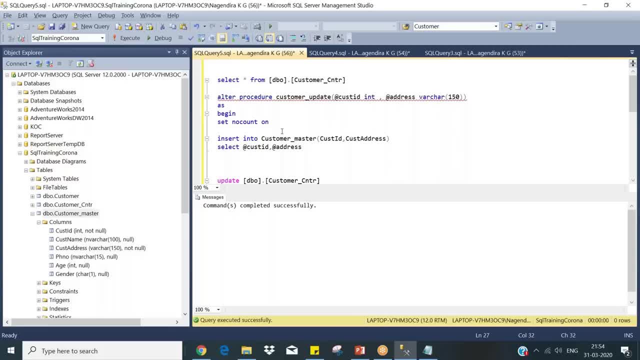 displaying. so this is useful. this itself will take some time. so this is: people say like: this is one of the performance improvement factor. so in order to avoid the such messages, you say like: does it no count on off something like that? okay, just for your understanding, i'll mention 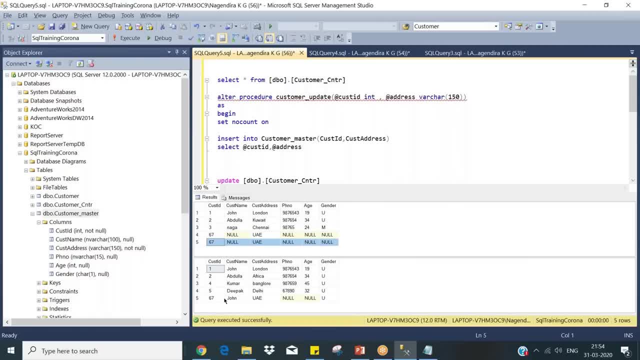 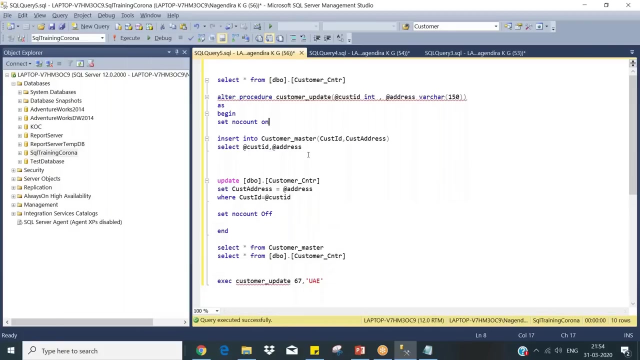 okay. so when i executed again, so another entity was there. there is no changes in your data here. so this is about your procedure. guys. any doubts in this? procedures: views, hello, hello, let me explain this again. this, uh, yeah, so when i have this one remote, you see like halter procedure, like this: when i update uae, you get rows affected. rows affected. 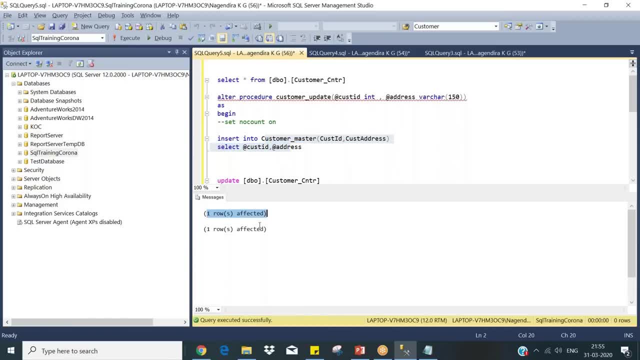 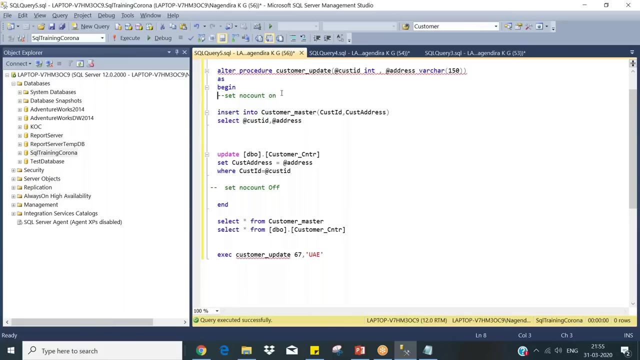 based on the insert statement: here this message is displayed. based on the update statement: here the second message is displayed. sometimes what happens? to avoid there will be number of statements here, you keep on executing, so that will have a lot of messages like this. so to avoid these messages to be displayed, you need to enable this option. okay, so I'm altering again. now you try. 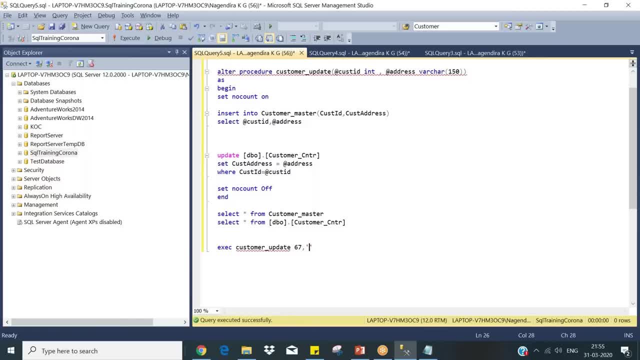 to run this guy woman. I will make him to woman. so sorry, now, you. now. you see, like I said, omen, there is no messages now. one rose affected. one rose affected, you got it. yeah, that is a main purpose. okay, so this is the thing. and similarly, 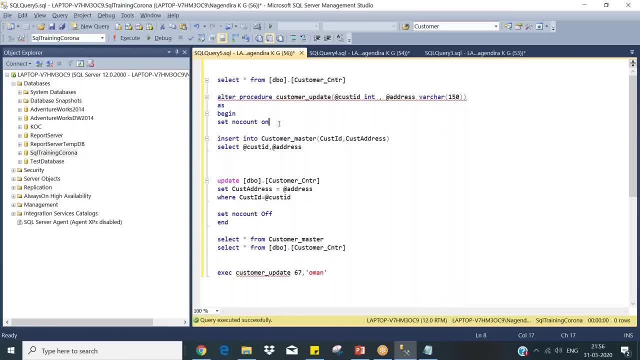 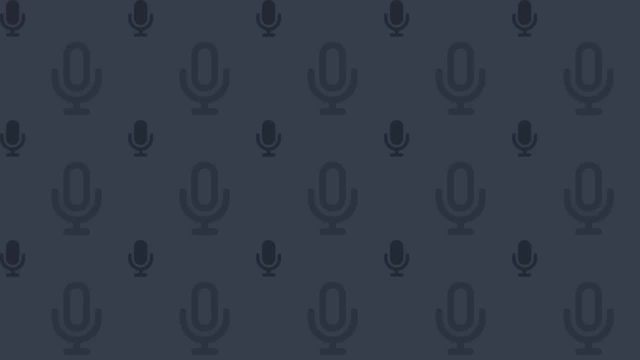 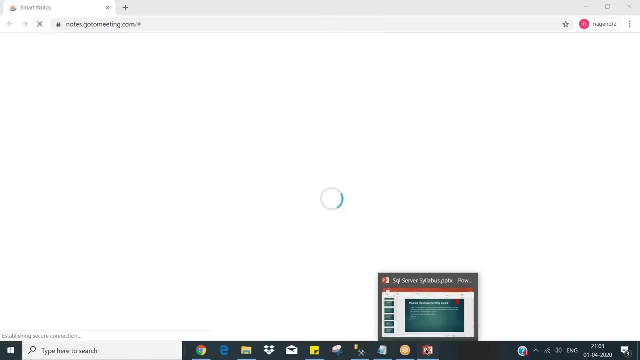 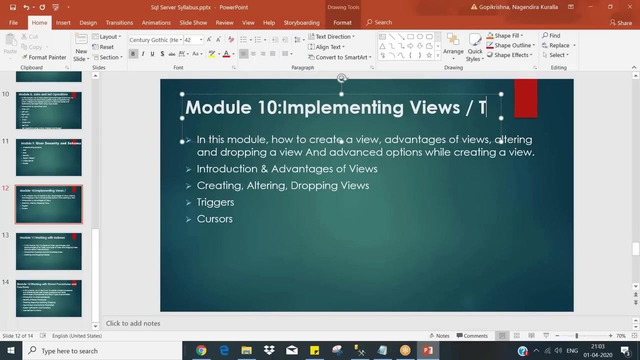 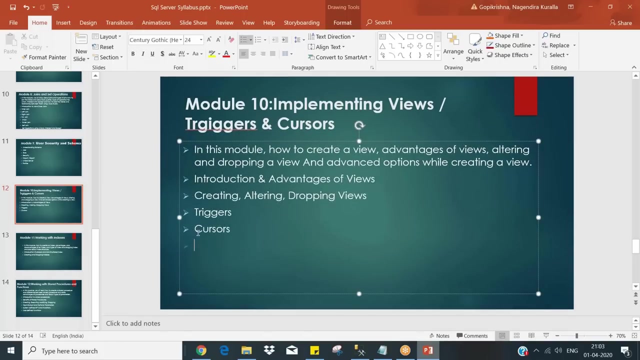 you have one last thing about today's session. we have a procedure, we have something like functions. this conference will now be recorded. so I read some more points here. it was only abuse and usual triggers and verses. okay, fine, so I I'm jumping between the topics. I'm not going in this flow. I mean, yesterday we saw 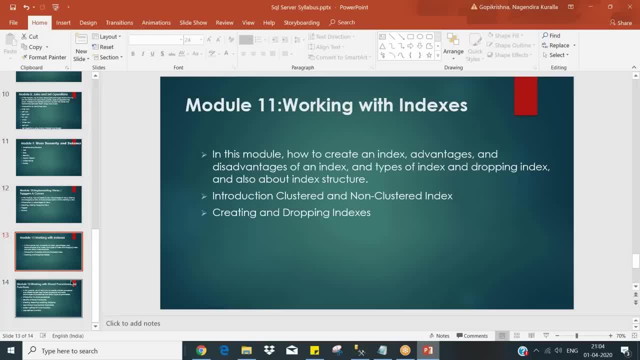 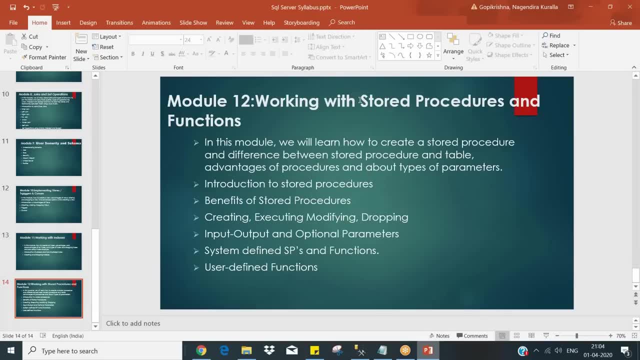 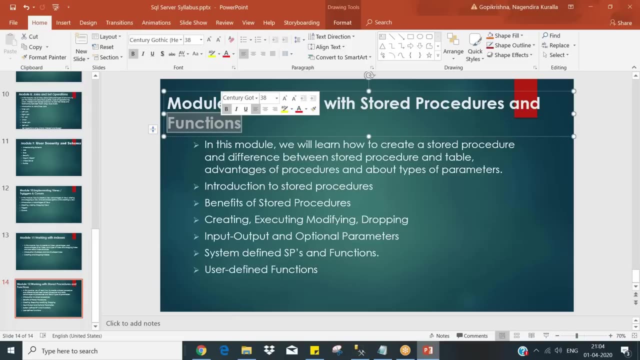 about you use then the order over here I need to revamp, so forget about that. so we start working on stroke procedures and functions. so yesterday we saw about short bridges and cover some more in that, and today we will start with the functions. okay, and moreover, what are the difference between functions and stroke? 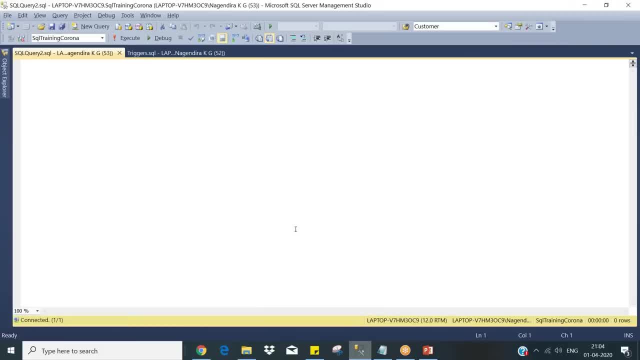 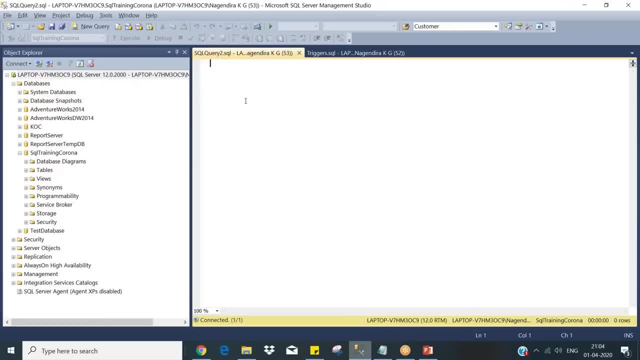 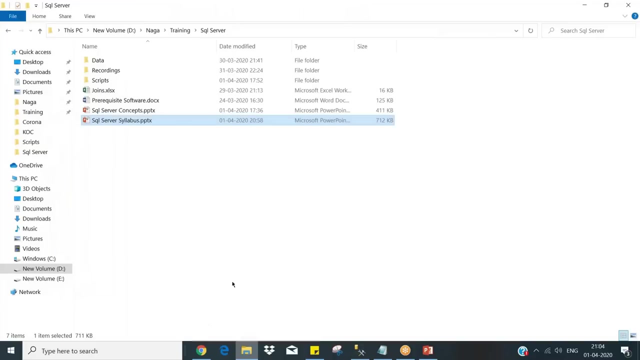 procedures. that we will see. once I create some function example, then we'll go for it. okay, so functions. it is again a same kind of thing. yesterday we created a stored procedure and store procedure. what it will do. it will do the update. let me check whether I showed that script. 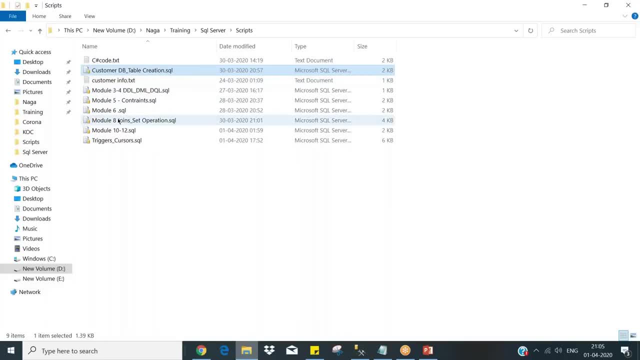 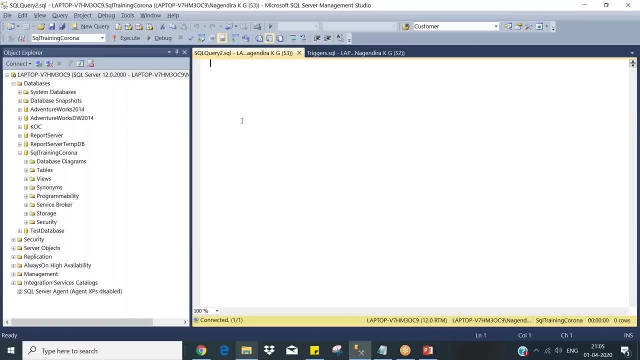 triggers, functions, operations- no, I think I don't have that one, it's 30. first of us and some other McGregor didn't say okay. so yesterday we saw what structure that you do to update, that will get two parameters. no need to worry, we already have this one here: customer update. so why I said these? 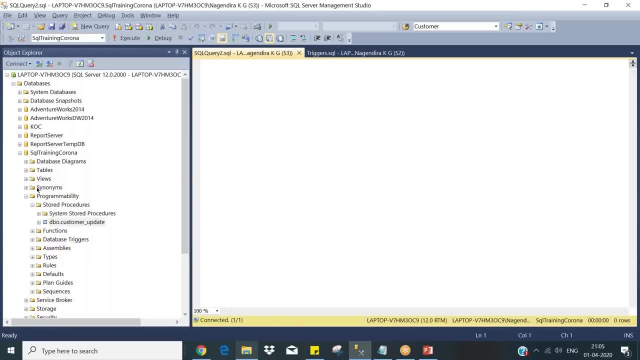 are the objects. so your table is your object, your view is our object. you see here, these are the physical structure. it will create it. so tables and we have created views, those things are created as an object here. then you have a store position. this is also an object. 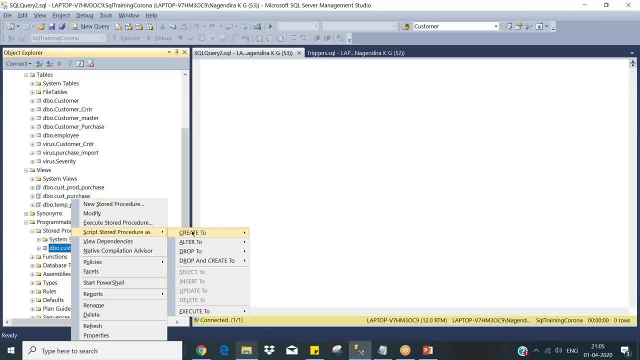 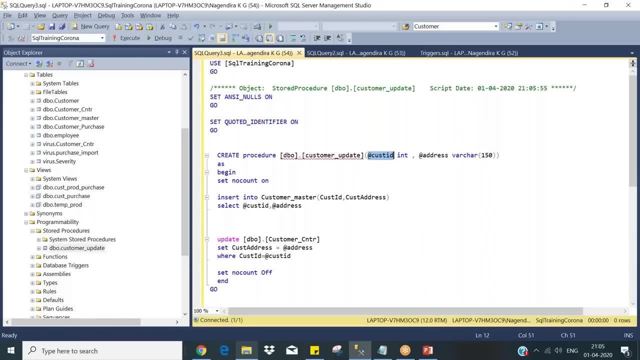 so these are the things it has created. now you can see the script over here. so what it does: it gives two parameters, one is customer id and address. then it does its job. just it will insert into a table and update the address, both the things. it will do, so like this: 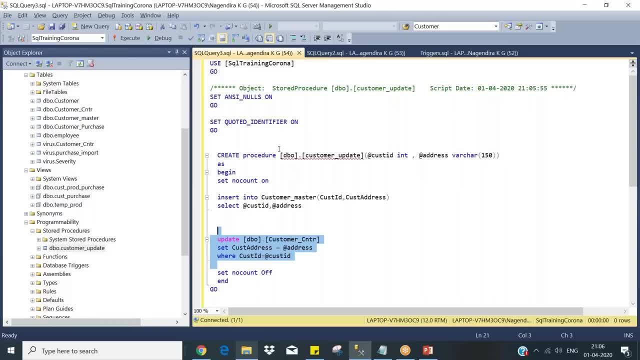 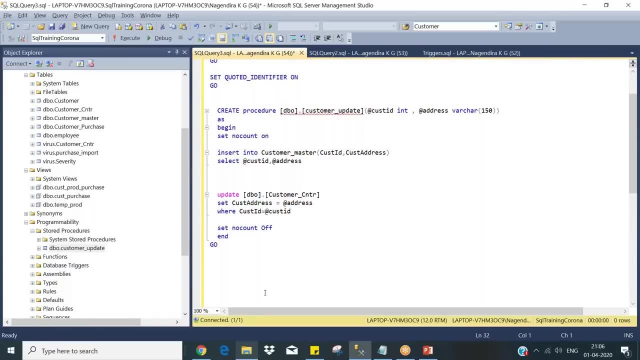 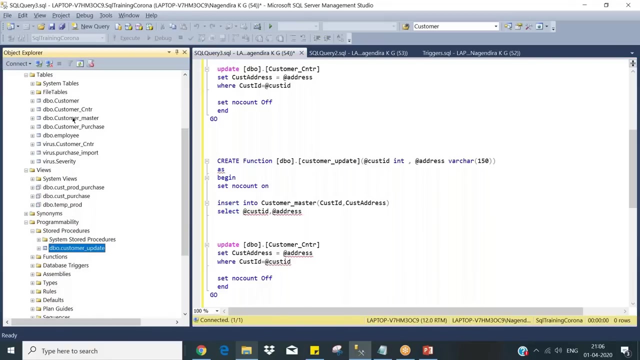 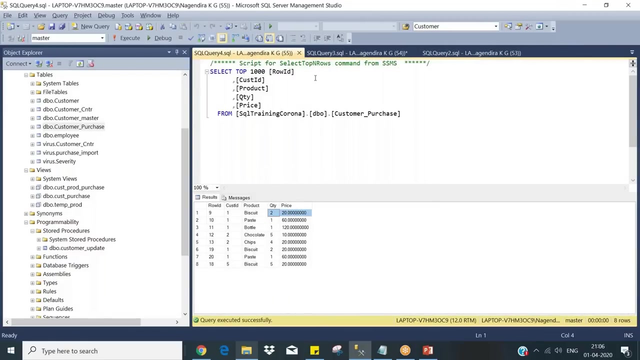 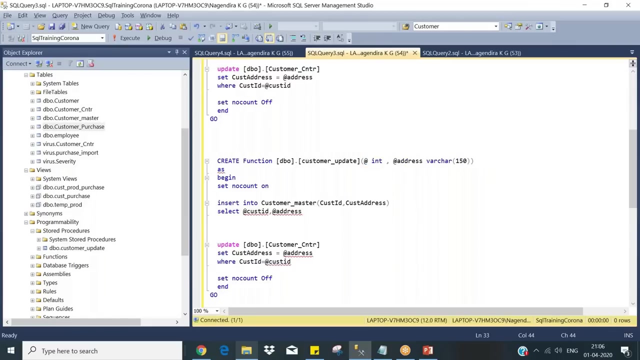 operations. if you want to perform, you use procedures, whereas functions create function. okay, let me take some table here. customer master or customer purchase, just want to see what it's taking? okay, price into quantity, perfect, i'll take. uh, at quantity at price. let me見 the other value. 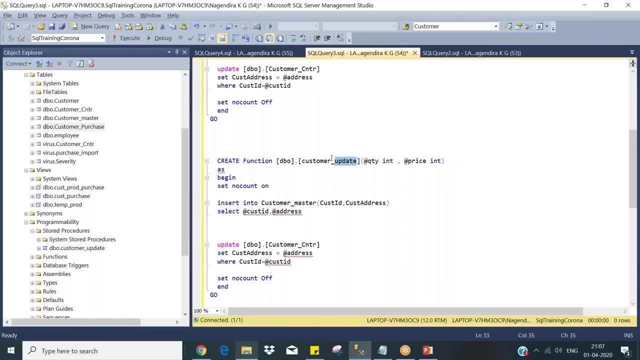 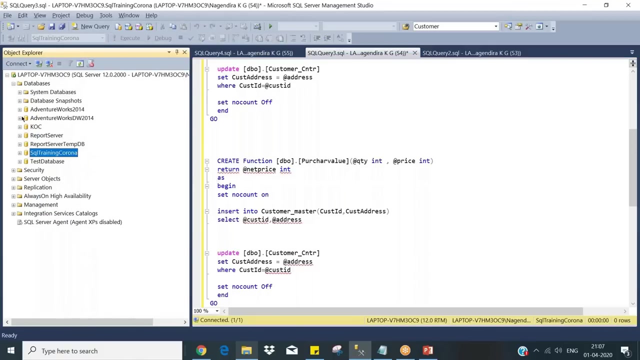 and this is. i pulled out that, and i know that the value above price, it's nothing but value. okay, here the value is also perfect. therefore, when i look at the table, here is value and from here you can see that value is taking two parameters, something like that. okay, this is the syntax of it. i just found something over here. give me a minute. 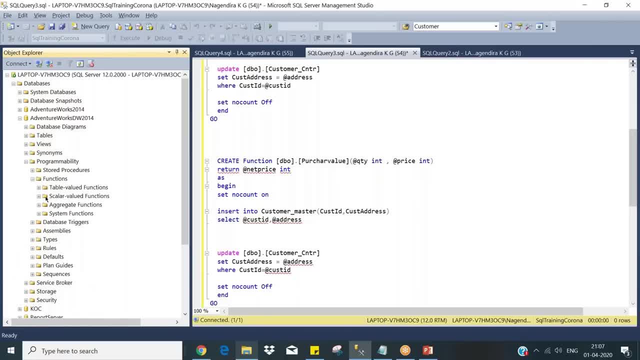 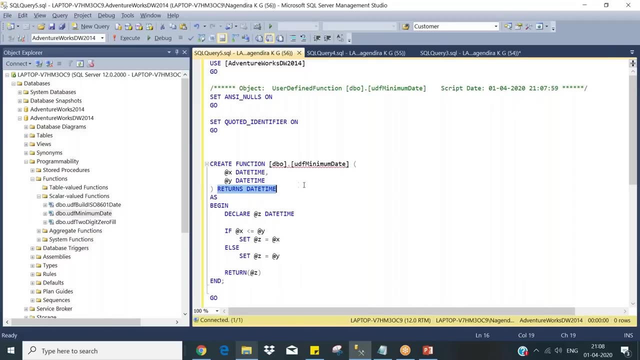 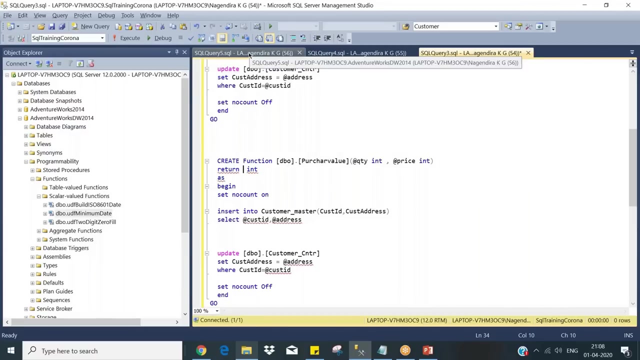 functions: table valued function. scale of a rate function: see: basically, a function should return a value over here. if you see a create function that will take parameters, that should return a value: okay, returns date time. maybe we will say written in teacher: okay as begin. declare: okay, fine. 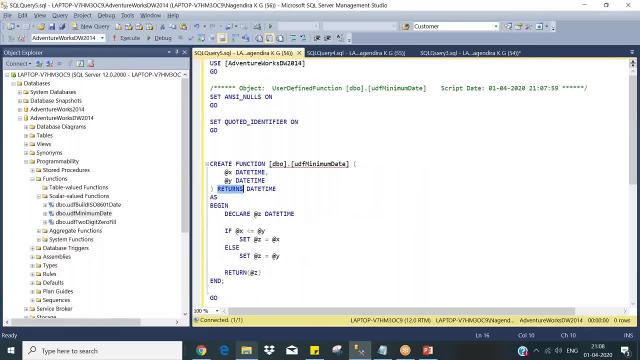 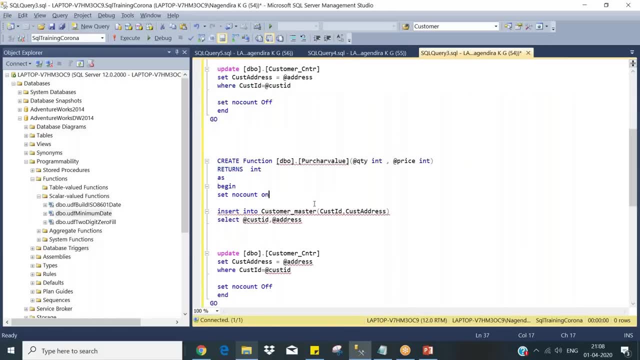 it should say returns. i'll take the syntax from references: returns, integer. okay, that is a problem here. you don't see anything. so what it does is see similar to a programming language. you can declare a variable- i hope everyone familiar with c or what basic languages you can declare a variable. 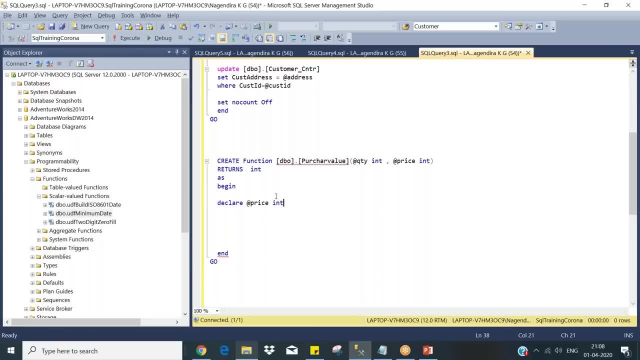 price: okay and declare a variable price: okay, write it as integer. then what you can do is set. you need to. if you want to assign value to this variable, you can say like set: okay, set price equal to quantity into, or i will say: net price, quantity into price. 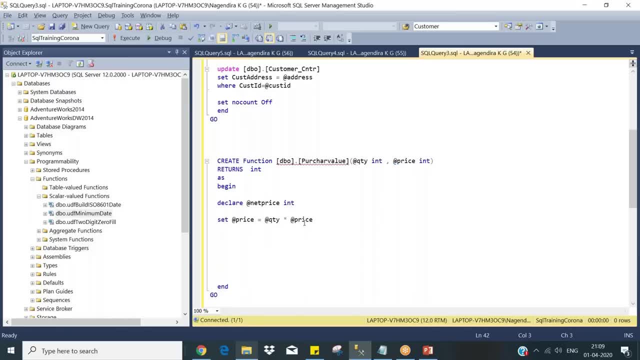 this is as simple as that. okay, then, what it will ask to do? one second: it calculates, just return me the value, return net price. this is simple programming. okay, that you understand this one. it gets two input variable once, quantity and price. it will multiply and return the results. if you give two and three here, it will return six. so this is what. 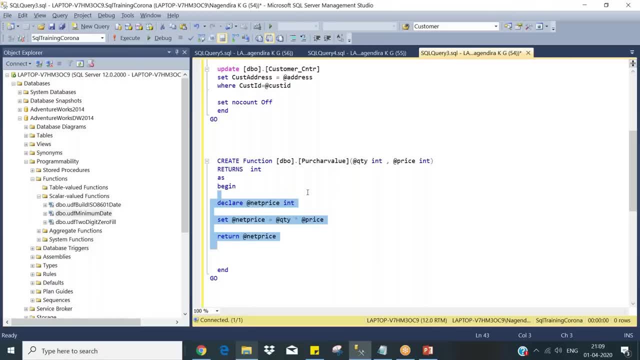 you return a program- or i hope everyone has written some programs. if not, this is the way you have to write, so you need to store these results in some place. that is the variable i have created here. this is the way to create your variable. declare is a statement. to create a. 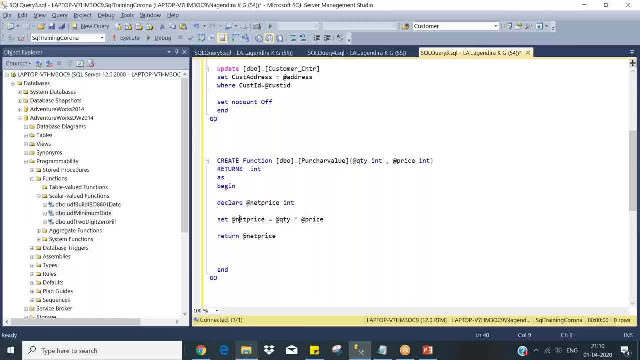 variable that will hold temporary results. so i'm setting the value- i mean the calculation of this will be stored in net price- and i'm returning this value over here. okay, this is the definition of your function. then i'll just execute it. okay, then, how to call them? 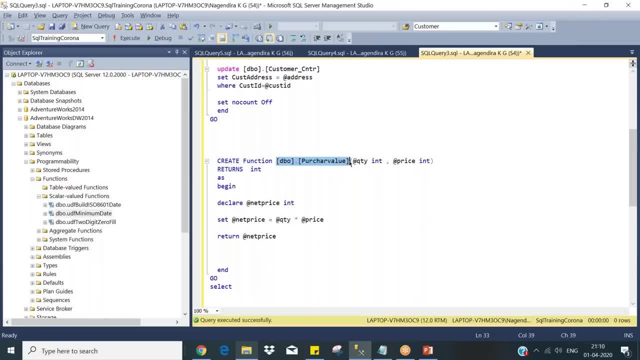 so i can use select of purchase value and i need to specify two comma, something like that. so i hope everyone knows the multiplication. just i will execute: 2 into 9 is 18.. i'm getting this value okay. so what is the main difference? over here is like: so you, you guys understand right, these kind of 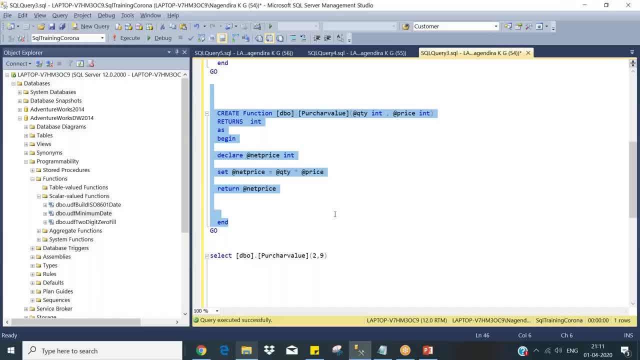 calculations you will create, okay, and you can use this function to compute some values. it is as simple as that. you just imagine you are finding the uh tan theta. i mean some average values are. you are passing some calculations like average for that month, any calculations you can do over. 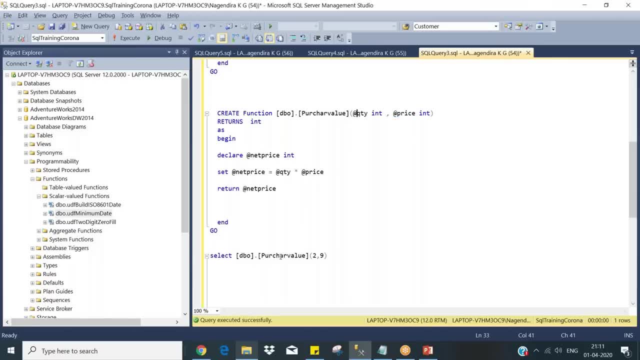 here. okay. so in this situation you're getting the first one over here and then you pass that value, two input values, then you can execute. you can pass those two values here, then you get the results over here. okay, this is your function: net price. i think even you can execute like you cannot execute. 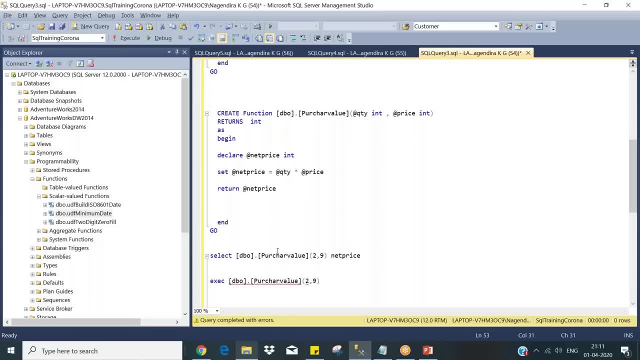 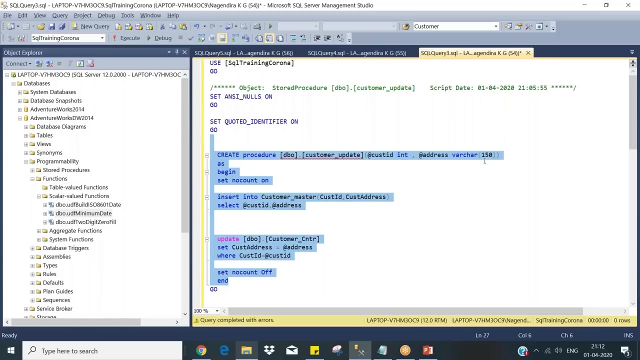 a function like this. let me check that one. you cannot execute a function, okay. you can select a function like this, only okay. so that is the main difference between your uh store procedure and functions. what i'm trying to say is you have here a create procedure over here, okay, create procedure, procedure name. 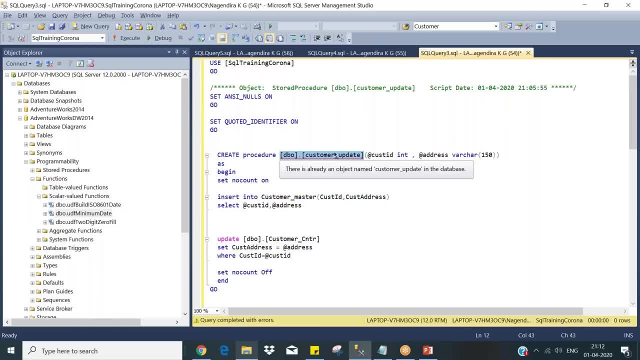 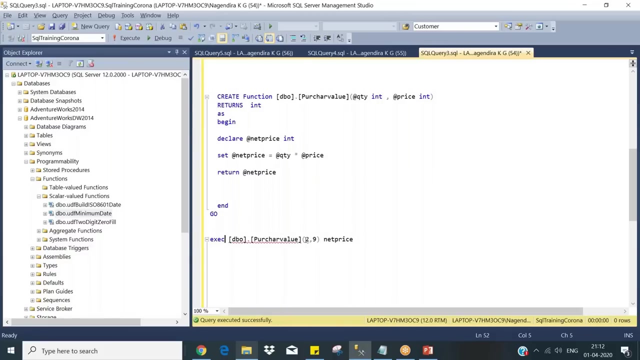 and in order to do a call to this procedure, you use execute procedure name. you pass some id three comma, some bangalore or chennai, whatever, like this: you will pass, you will. you are executing without parameter, i think. okay, now you got the value. similarly here, i think you can do it. let me check that one: execute. 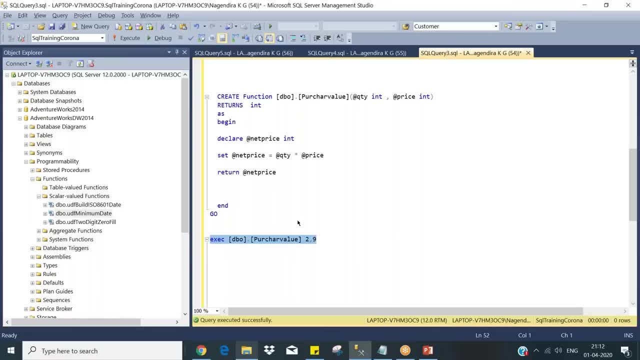 will not work here. okay, this is executing, but you are not getting the result. in order to get the result, you need to put it like this: select. you no need to use the select. if you select, then this is enough. you can get that value in the select statement. 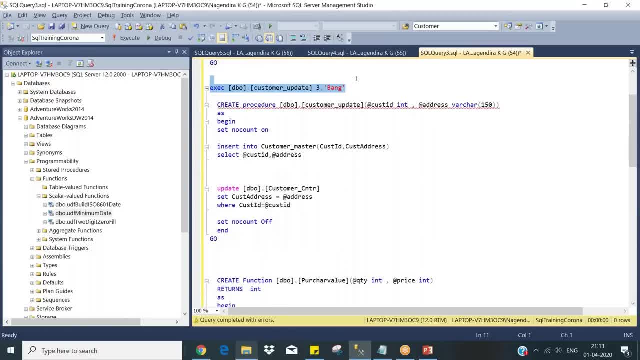 i'll use both the guys together. so in order to get the values, you need to use select statement to run the query. now this is the value. i'm passing it over here. two comma nine. what happens if i run this function for a table? you can do that by passing this function. so here i found one data. 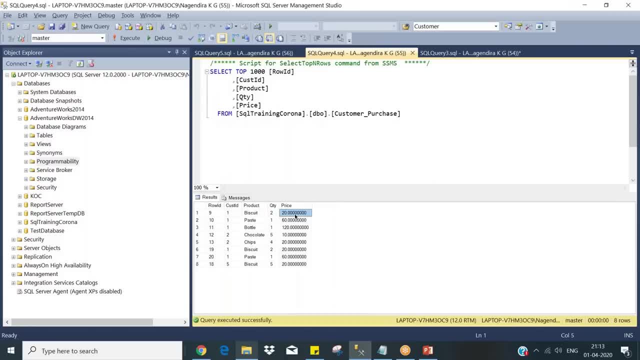 this table. i want to multiply this quantity into price. i want the result 40 to be displayed in a new column. this i want to do programmatically. i don't want to write the code. even i can write like this: the same thing: quantity into price. okay, this i can do it. 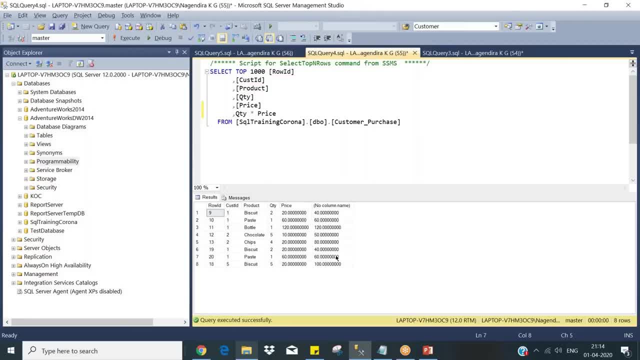 here itself. i'll get the results. i got this result: 40, 60, something like that. instead of that in this place i can call that function passing quantity comma price. that will calculate this: 40, 60, 70.. let us show. let me show that one what i'm trying to say. 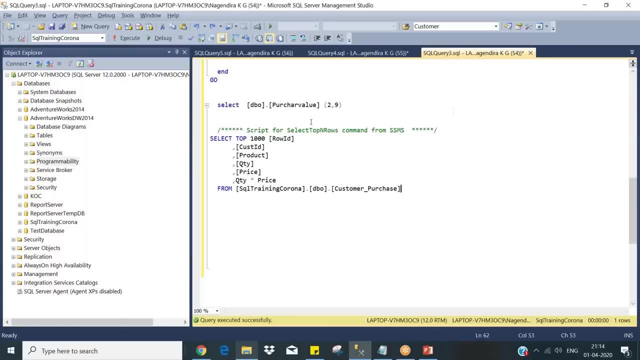 so this is a table and i'm having the without function thought function. i'm using this function. i'm calling this function. okay, here you see, in the select statement, i'm calling this function. this is the function name: purchase value. and then now i'm going to give the political function Ellie. 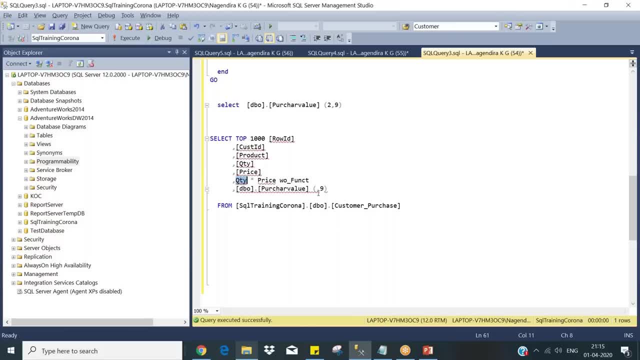 instead of 2 comma 9. i need to pass this quantity here, this price over here. so 2 comma 9 gave me 18. so this one and this one should return me the same using function. so this is without function. this is using a function. both return me a same. 5 into 10 is 50. 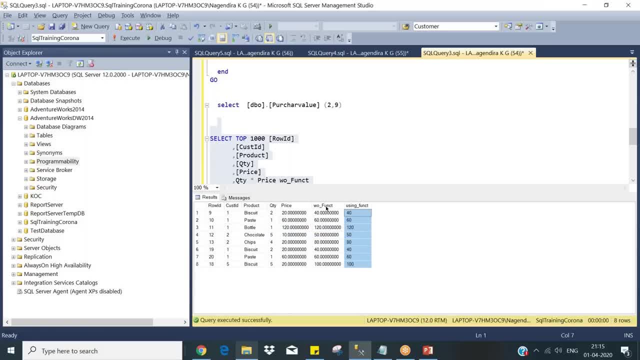 5 into 10, 50. so using a function, this returns. this is without a function in the direct column, so i have written it like this, because some calculations you cannot do it in a simple calculation like this. okay, some calculations. you will pass these two values and in your logic you compute a lot of. 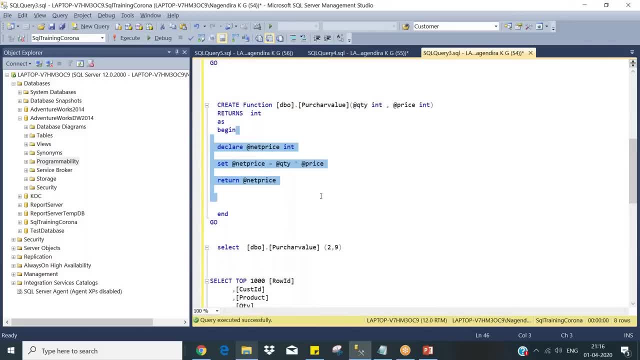 things over here. you write hundreds of codes over here, then final results should be passed to this column based on the two input values. so such a things you go for. function and the main difference. now you got about what is the function used for and the stored procedure. also, you can do it. 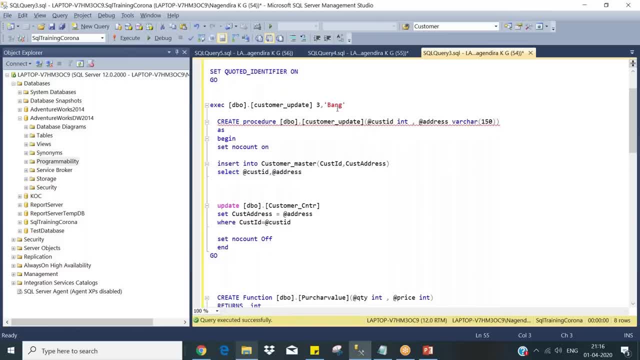 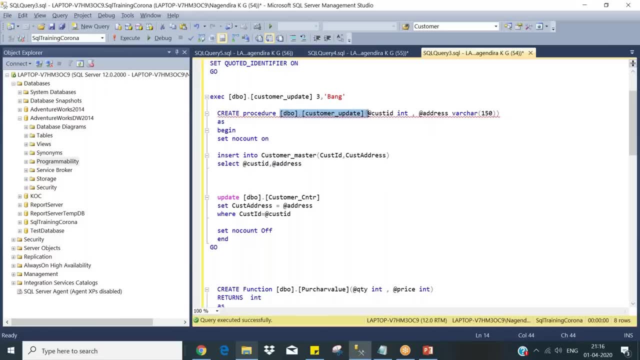 the same way, but you cannot use it in the select statement. the stored procedure, you cannot use it in the select statement. say for example: what i'm trying to say is: so, since i said, like i can pass parameters here, so this customer id and address also i can pass right. 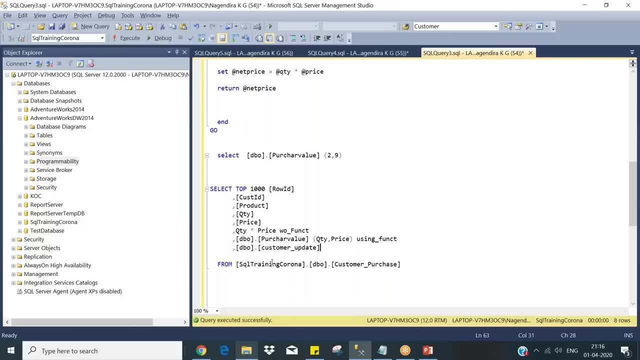 you might have asked. so this is the stored procedure. customer update, since the stored procedure requires execute statement explicitly mentioned. okay, you cannot have a select statement and the execute statement over here, so you cannot use a stored procedure in your, uh, select statement. okay, that is the thing, but whereas you can have your function, 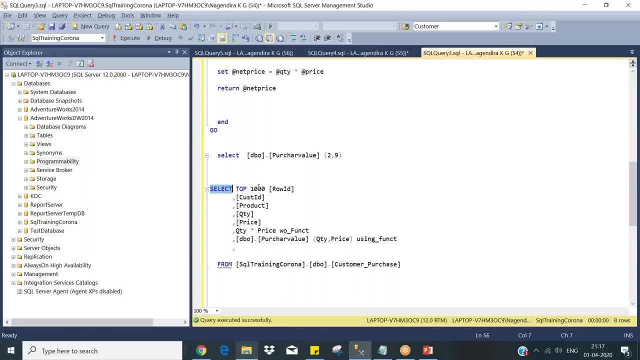 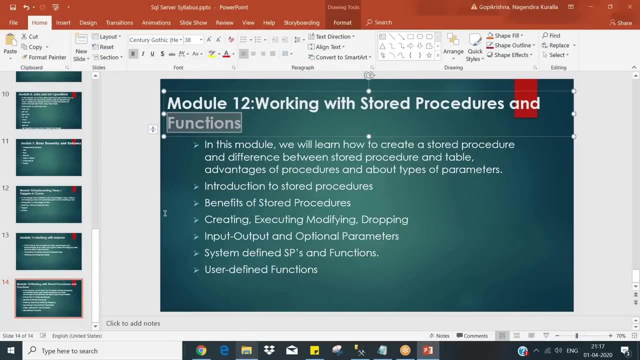 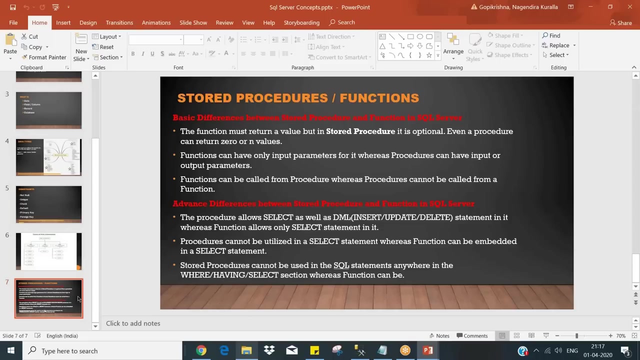 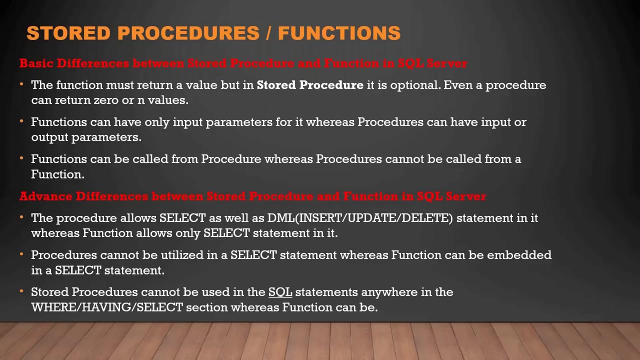 in your select statement that will execute for each row. i hope i am clear with this. let me show you base difference between these two. so stored procedures and functions. the difference is this: the basic difference: and the function must return a value, but stored procedure it is an optional. 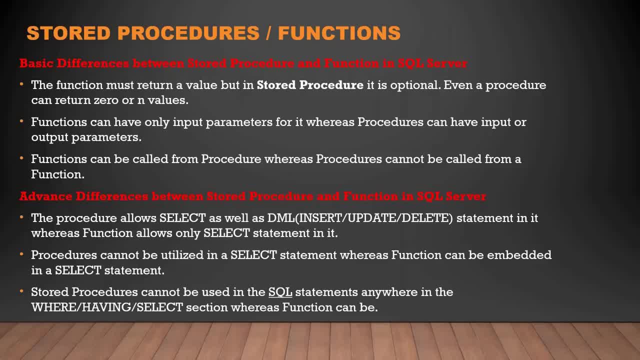 so this is the core difference between your function and a stored procedure. you remember our stored procedure. that was inserted and updated. so if you have stored procedure, you will have a stored procedure right now. that did not return any value written in the sense you give some input that will return that value. 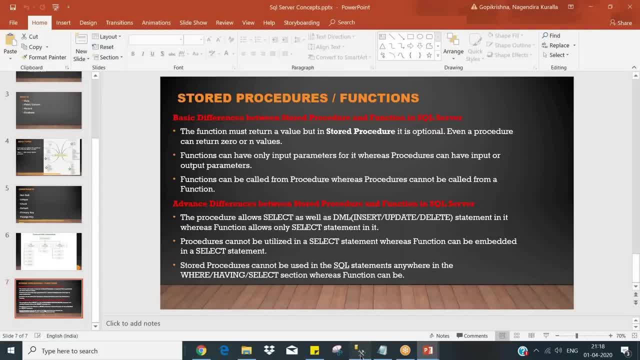 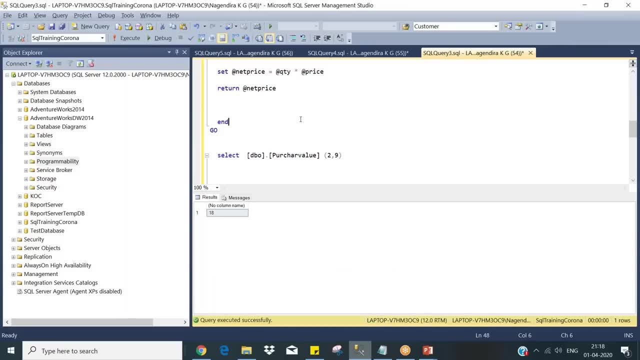 and you store it, whereas that function you gave these two inputs, it returned you a value called 18. when you execute this procedure, that does not return any value. this does not return any value, just it has. it has done his operation, whatever you do, okay, if you want some operations to. 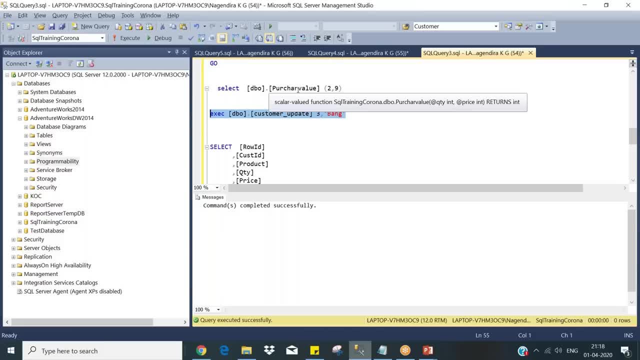 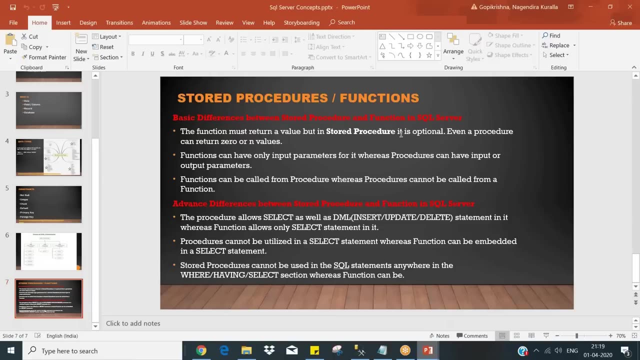 return some value. by default. you go for function. okay, then store procedure can also return a value. it is not mandatory, like it should not return it's they said like it's an optional. okay, but short pressure, it is an optional, but when you want something to return a value. 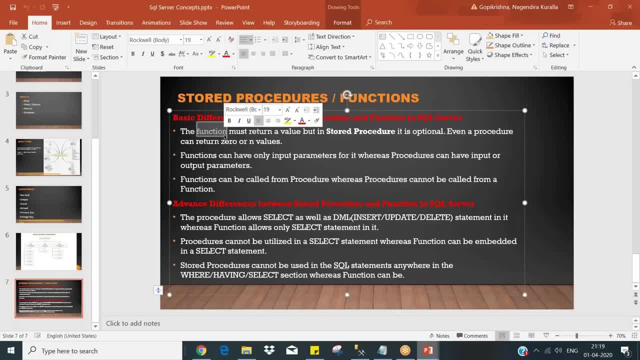 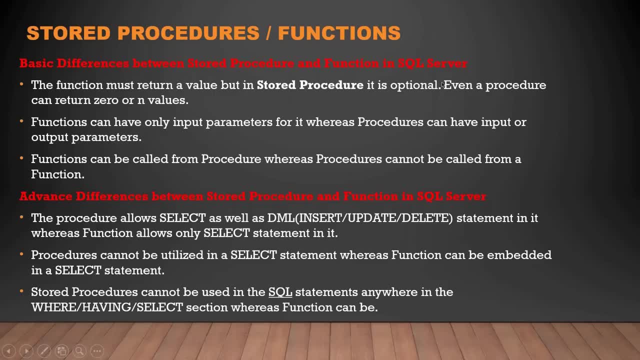 you can do it like this: if you want it to be returned, then you go for a function. okay, so that is what they mentioned, even as procedure store procedure can return zero or n values, that is any that can return values. that is a core difference, okay. next point is: function can have only. 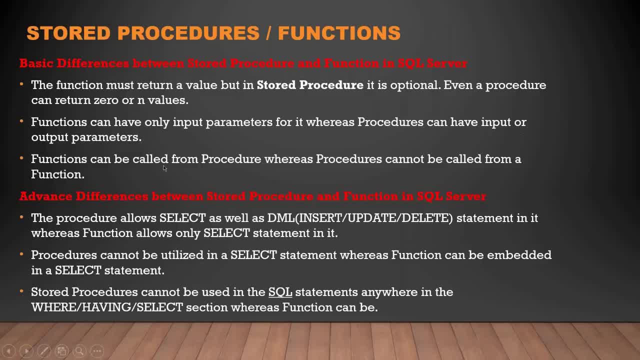 input parameters for its, whereas approaches can have input or output parameters, so it is same. i mean more or less. so function should have input parameters, can have only input parameters. only input parameters means whatever you pass and procedures instead of written value they say it has output parameters. 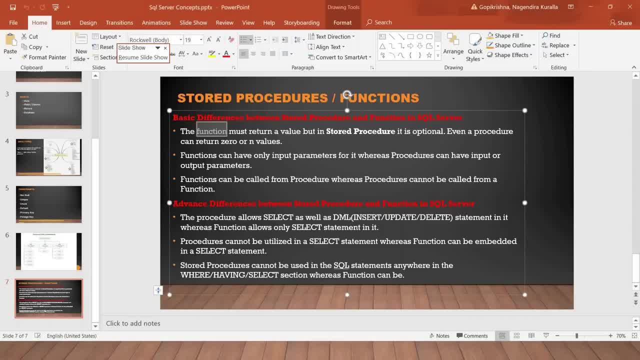 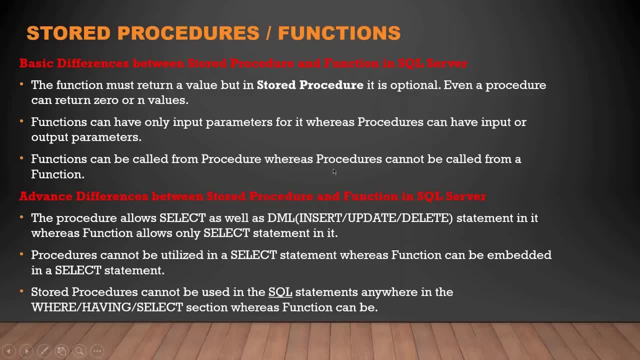 okay, the parameters matters. whatever you pass here, you can specify. i will tell you later. functions can be called from a procedure, whereas the procedures cannot be called from a function can be called from a procedure, so it is like some people will have a comment from here to the, there to the. 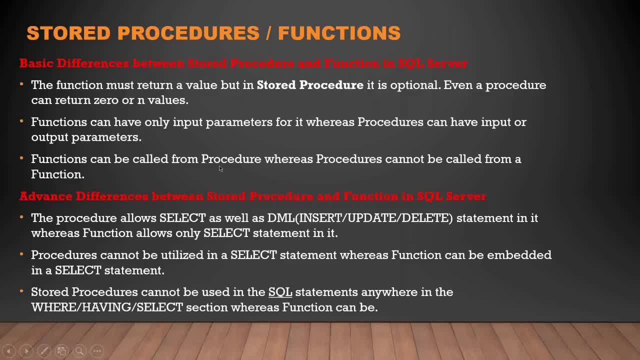 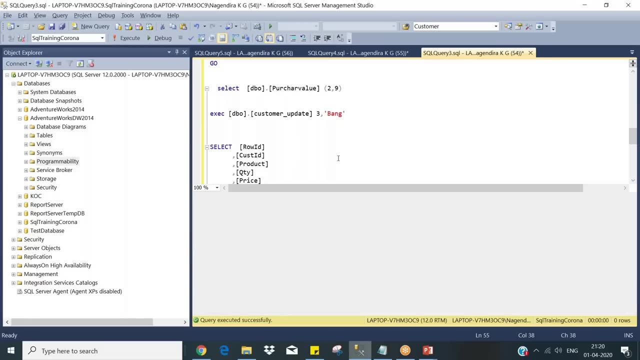 it is not possible. vice versa, it's not possible meaning like: inside a procedure, okay, inside a procedure you can call the function, but from a function you cannot call a procedure. that is what it mentioned. let us have that one, these two points, clarified and just altering this procedure create. 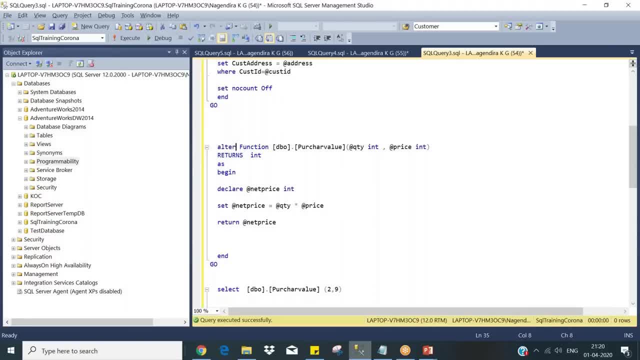 function, function name: i'm saying alter. so, as you know, guys, this d, d, dl operation applicable. alter means you are modifying something, alter mean you are modifying something. what they are saying is: i have this function. if i say, like, i want to call something inside this function, i'm calling this procedure, okay. 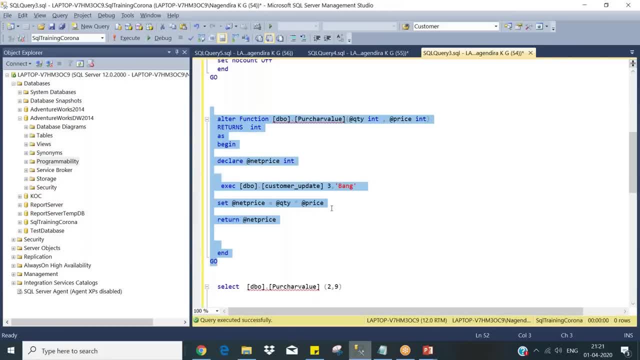 okay, now it see that i have this function. so i putting its name on visitors. see it has compiled. compiled means this code is saved. but when you run this one, only functions and some extended short bridges can be executed from within a function. so it says like only functions can be executed. another function you can call. 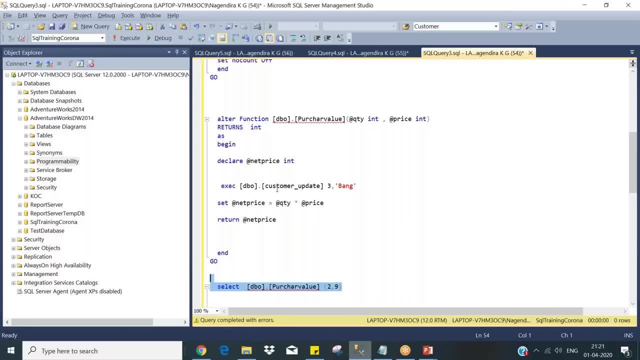 you cannot call a store procedure inside your function. okay, in such a cases you should avoid it. basically, guys, people will confuse where which one i want to use. i want to use function or stored procedure. when you want to call us another stored procedure inside your code, then you go for store procedure. so store procedure can call another store procedure. 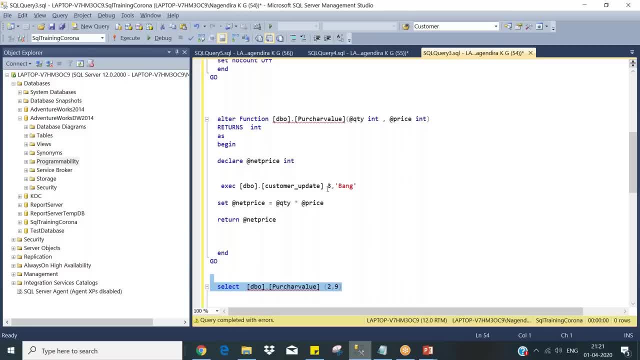 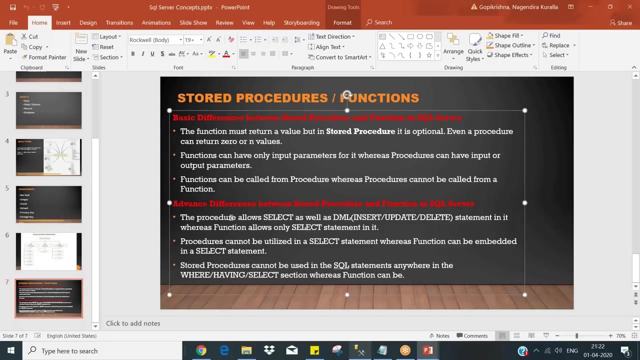 fine, but you want to do some simple calculations, such a kind of things, or any other complex calculation that returns a value, single value or multi-value, whatever. then you go for function. so this is the simplest way to understand about functions and store procedures and the other things are there. procedures allows the stored procedure. see, people always say: 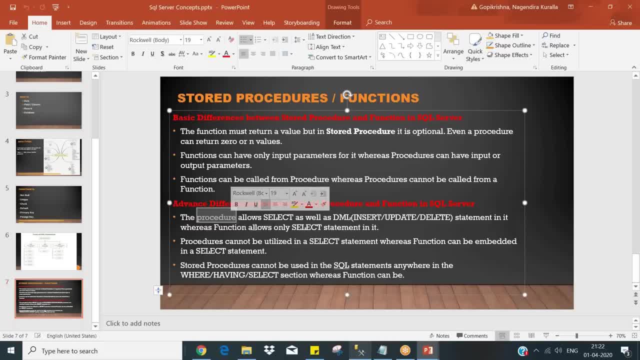 procedures. in a skill world they will not say: with the short procedure, it's procedure procedure allows dml, insert, update, delete, whereas function allows only select statement. okay, these are the things you need to consider: what to choose, whether you go for stored procedure or function. if you want to do insert, 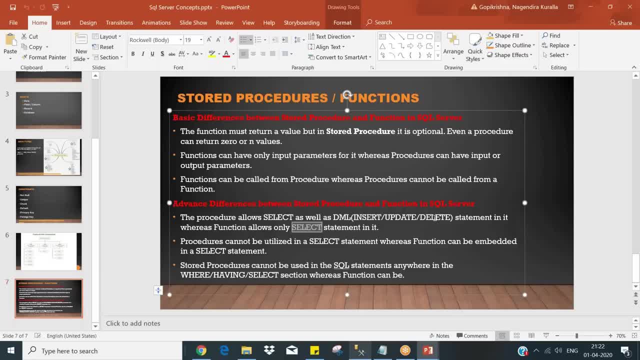 delete update inside that, so always you need to go for stored procedure. this is the point i highlighted. procedures cannot be utilized in a select statement. we cannot call a procedure in a select statement, as we did before, the price into quantity, whereas functions can be embedded in a select statement. so they use some technical words, don't confuse. in the select statement you. 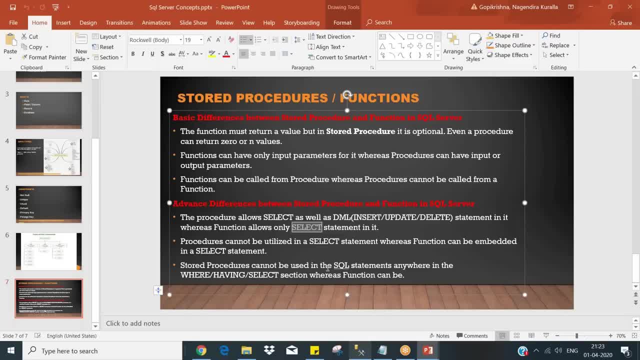 can call a function, then short bridges cannot be used in a skill statements. it's simply either in a skill or select. both are same and functions can be used. since it's used in select, you can use it in a bad condition whatever place. okay, these are the things you just keep it for your. 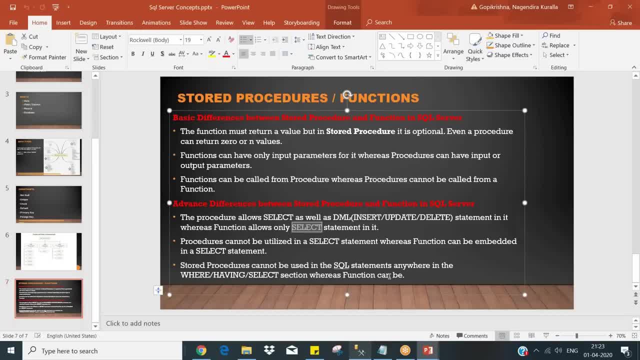 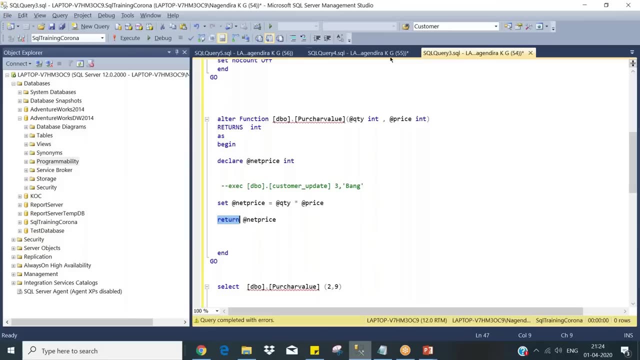 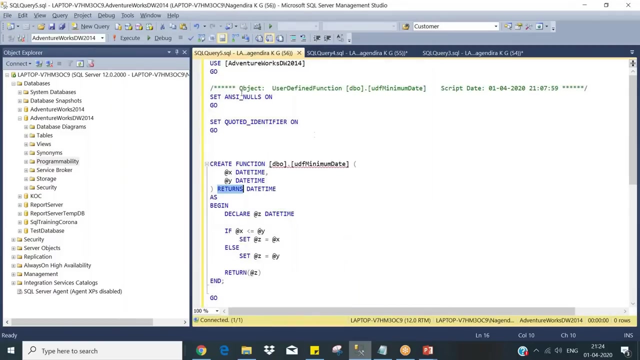 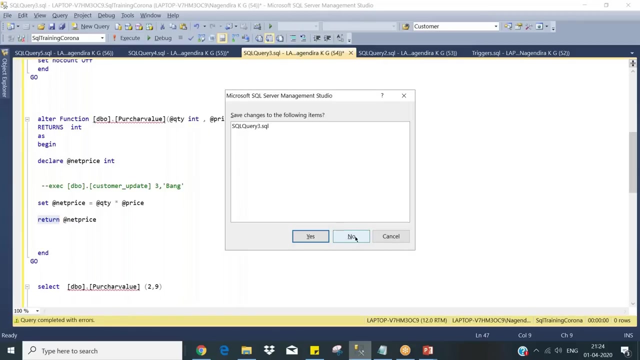 reference, I will. anyway, I'm going to share this presentation- one least syllabus I have shared- and keep updating this slide. so, once it is done tomorrow or day after tomorrow, and share this, both the things, along with the recordings. now I'm going to another session. I mean another topic: triggers and causes. so 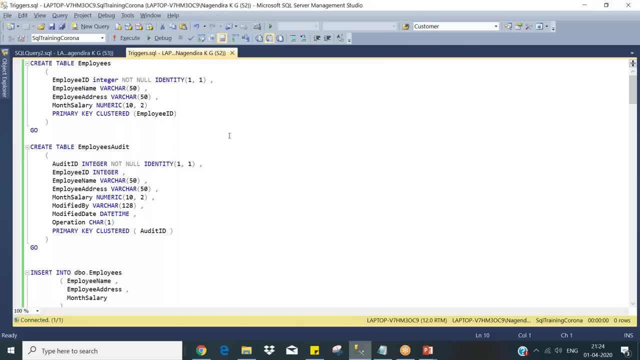 before heading to explaining about triggers, technically, let me tell you when you you want to use triggers, when you want to use causes, okay, so triggers. as the name indicates, it will trigger something, some other operation, if something has happened and it should initiate some other operation. so this is what a trigger is. this is one you use: trigger. 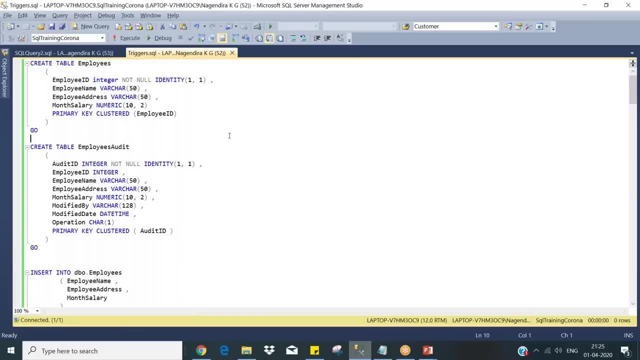 so, for example, when I want to create product- okay, and I want to intimate this to my manager- or any new request comes, I want to intimate to someone else. so assume there is new product entered, then that will insert into a product information. then what it? we have to inform this like it has to send. 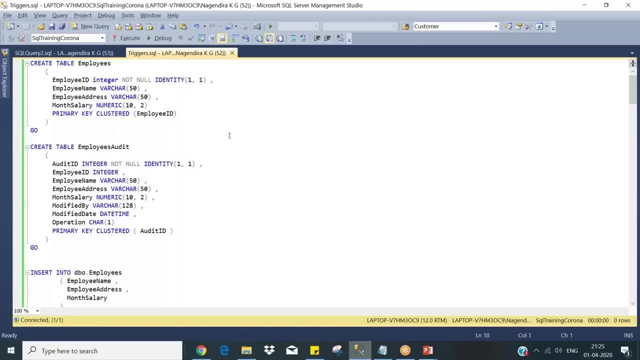 some email or text message from the user that has already been used and which is the URL in the article information, then what it will have to inform is like it has to send some email to a manager, or it has to insert in the log table, or it has to uh, intimate some other operations. 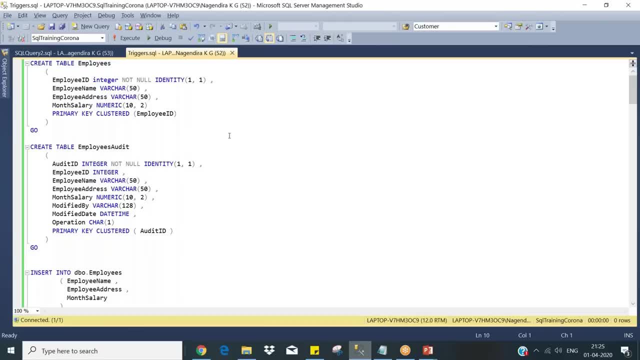 trigger some other operations. so these kind of things, how will you do? you cannot keep on monitoring these things like once the product got inserted, what has to be done, something has to happen automatically once some operations happen. so these cases you create a trigger and say that what has happened, what should happen, whether some insert should happen or 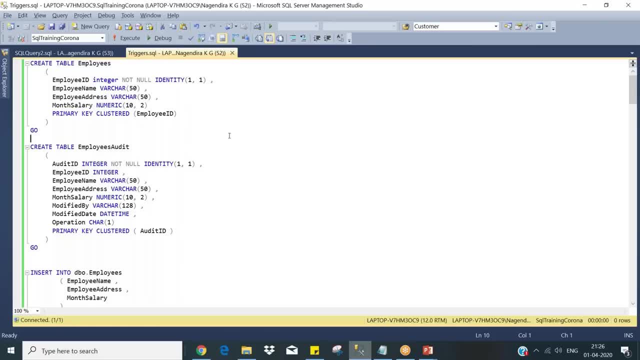 some select is happening or delete is happening in a table or object. someone has logged in, so those kind of things. something has happened, what should happen that you need to mention in the code. so this is what uh trigger is. okay. let us discuss uh later about the cursors. 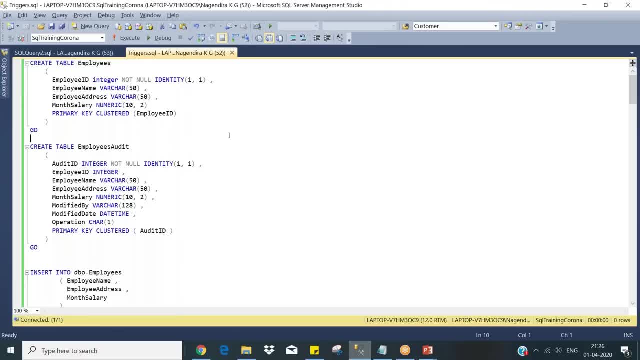 with this note. let us focus on trigger example technically. so what i'm going to do, and let me explain that. first, i'm going to create an employee and employee edit, as i said so in this example, whenever a insert happen in this employee table, or not only insert, insert or delete. 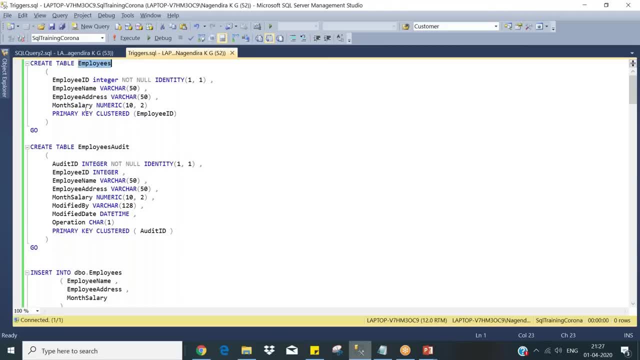 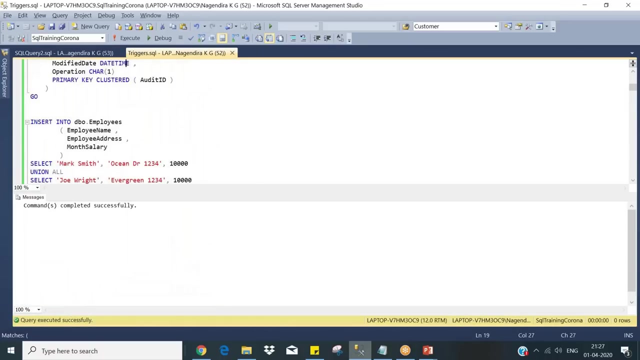 or update happens in this employee table, that should insert automatically in this table. so this is a simple example i'm going to explain. so let us have this table employees employee added, then i'm i'm inserting into employees, okay. so this is the definition of the trigger. let's go one by one. 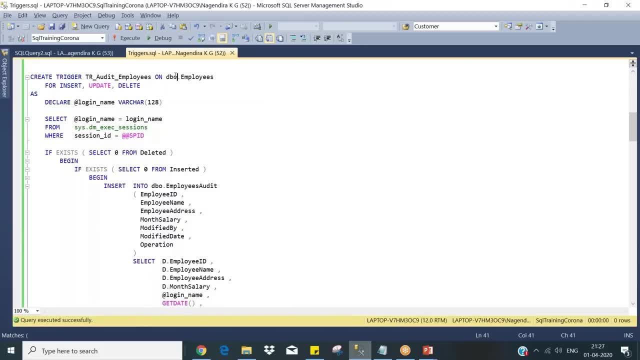 line by line. so the definition of trigger is says like that. similarly, how you create a procedure views- it is syntax is somewhat similar. in procedure you say: create procedure procedure name, create view view name. that is, create what object you are going to create. then object name. similarly. 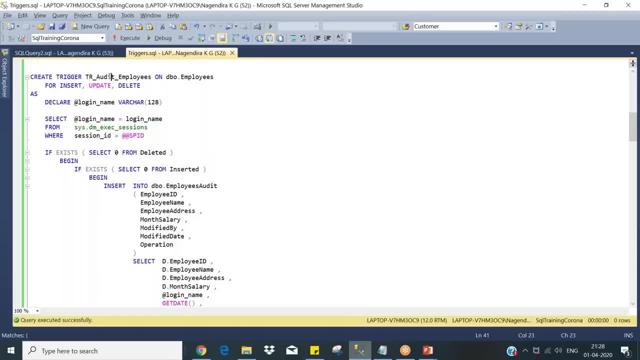 here: create trigger trigger. name that trigger on which table? as i said, i want to insert into a whatever operations happened in employee, it should trigger some other operation. so i'm creating a trigger on this table and for what? for these operations: insert, update and delete. so if these 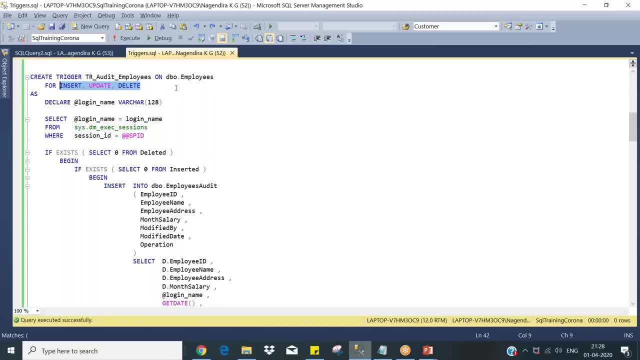 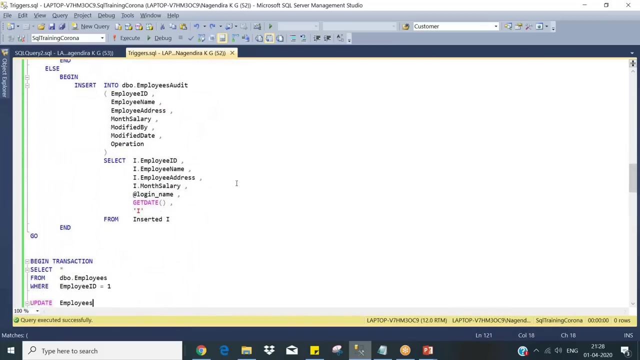 three operation happens. i want to initiate a trigger and that trigger what it has to do. it has to do this logic, what it is doing, this is inserting into employee audit. just as simple as that. okay, let me create this definition of this. so this is the definition of the trigger. before that, i want to explain another. 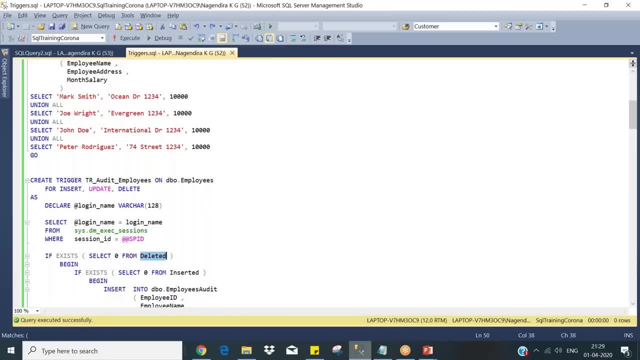 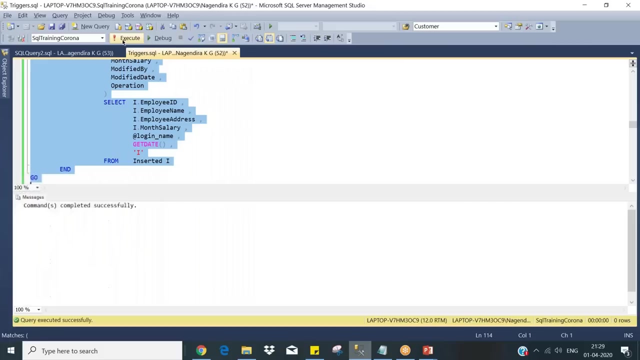 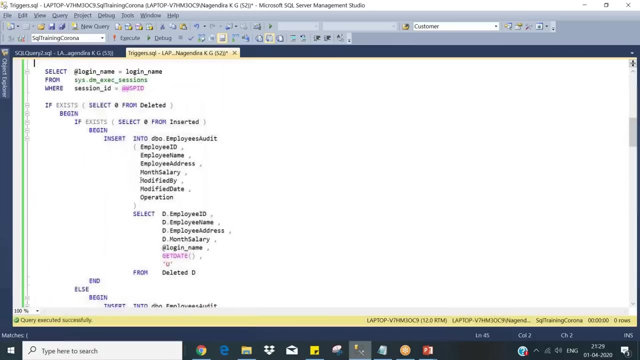 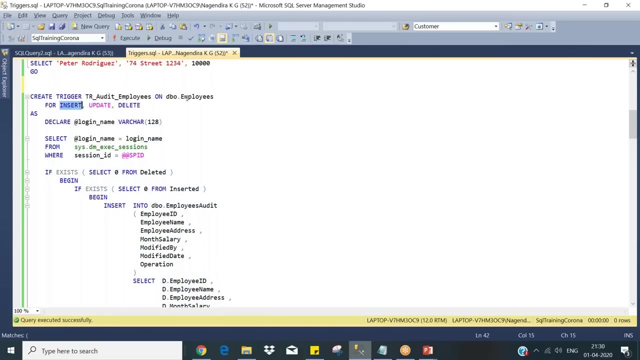 table. so um, okay guys, so now this is the definition of viewer trigger. so so we have seen the top part, two lines. if something happens, this operation happens in this table, then do this operation. if something happens in this table, then do this operation. let me quickly explain what is happening. so it is just getting the login names. 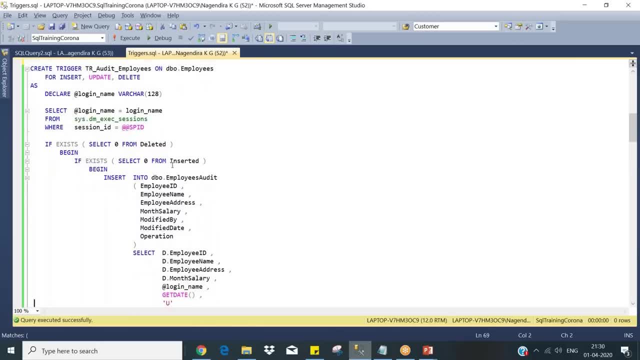 all those things. then see there is some concept like deleted, inserted of this table. basically, when you do insert in this table employees, debut dot, employees- okay, and what has happening here is it is not getting from the employees information. let us path these two, this deleted command, this one insertion, okay. 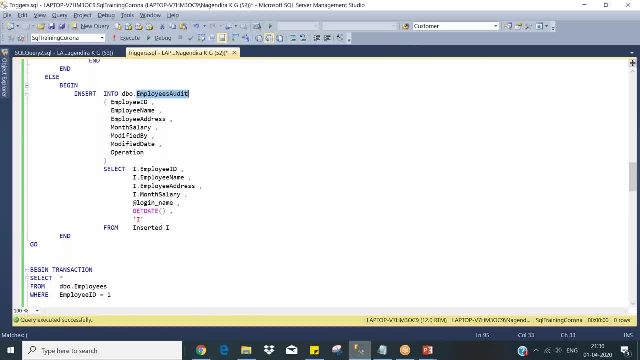 it is not picking up from the employees table and inserting into audit. instead, there is something like inserted- okay, what is this called so in SQL? basically, during the transaction happening, once you do insert into any table or any other operation, there is a temporary table. it is created. 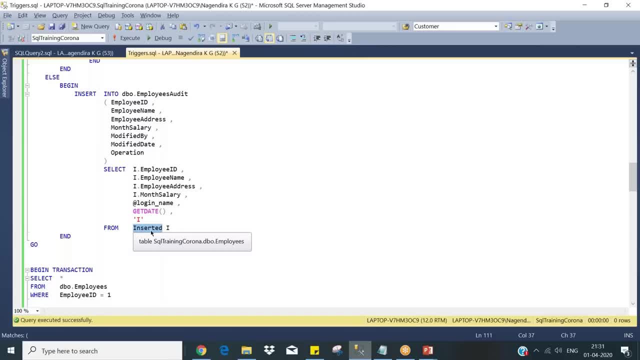 okay, a virtual or it is a physical table, during that time only. this will have that value once you have inserted, so this will have the value at that time. so, using that value when it is inserted, you are inserting into this employee's audit table. okay, this is the one insert into employee. 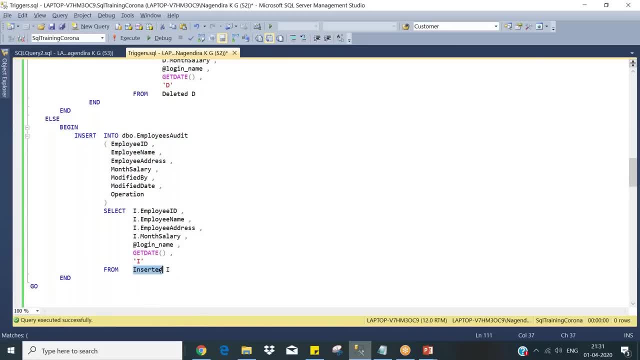 table where inserted: okay. similarly, if there is any delete or update happens, that will be stored in your deleted table. so from that you are inserting into audit table. if you have a delete, then you are getting that value deleted, okay, and inserting into audit value. so basically, we are getting, we are not getting. 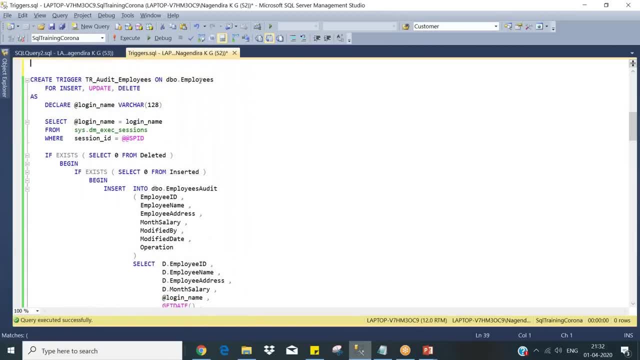 the data from the base table there is from employees, because you can ask, once you delete the record that is gone, how you will get that data and you will store it in a temporary table or audit table. you are running one query: delete into this table once you deleted. that's all that. 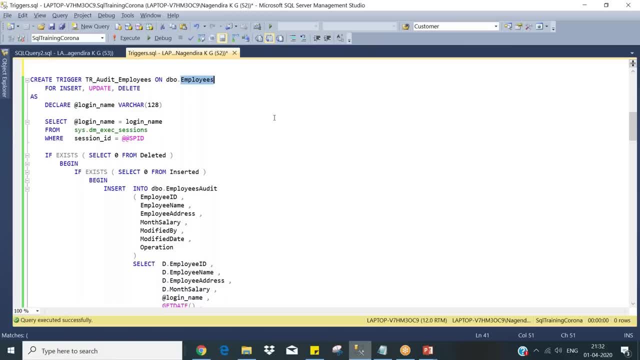 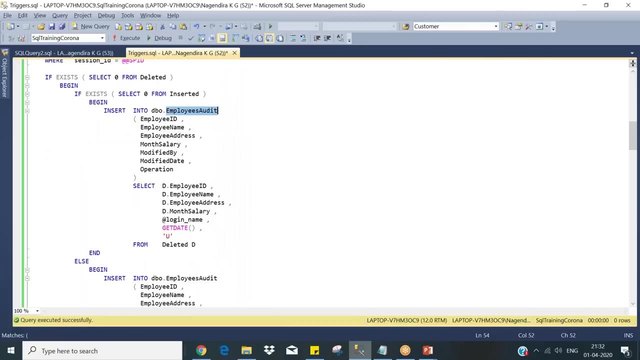 is gone, then you need to store it into your audit table. so before deletion, you need to copy and delete. this is the one way. instead, you can use this kind of temporary tables. okay, that is internally stored. use that one to for audit purpose. let us have a look with an example. okay, so i have created the trigger. that explains. 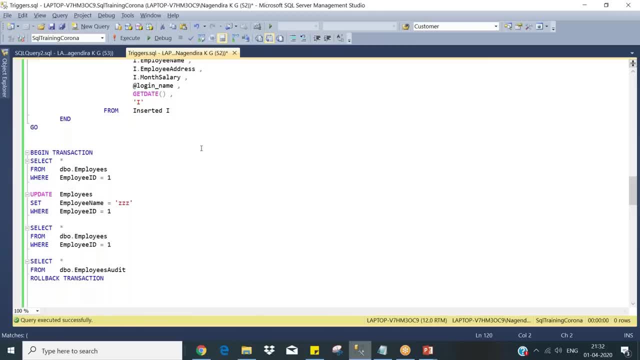 it will insert into audit table, irrespective of whatever operations you do. so now let us see what is there here. i have four records, four records and one record here what I'm doing. first of all, I'm doing a update, so it's rollback in transaction. okay, let me explain that one also. okay, 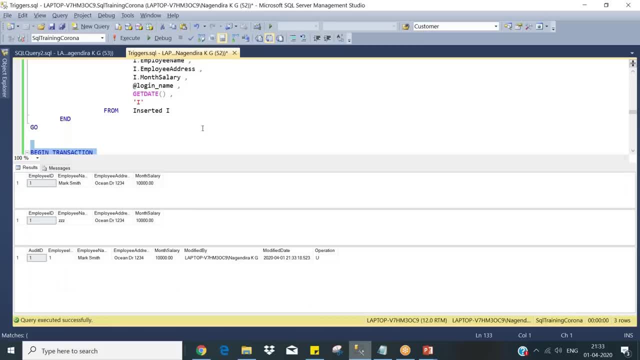 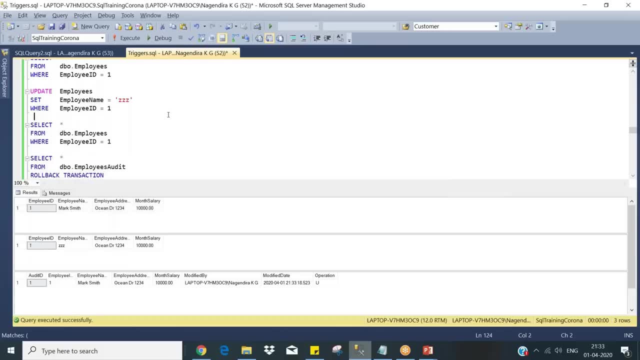 yes, now you see here what is happened. you see the query first. so first select statement: this treatment is written one: mark Smith. then I am updating the mark Smith. see the data here before updation: Mark Smith. what I am updating employee name am playing. name is Mark Smith, I am. 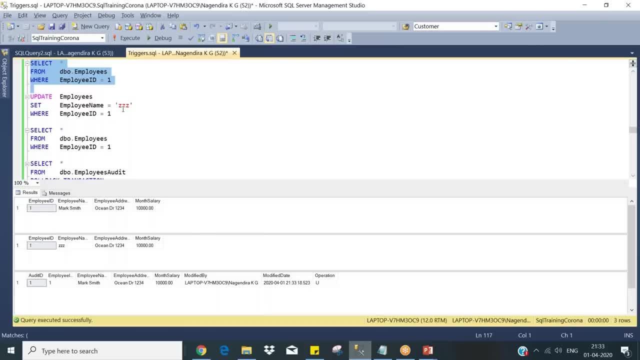 updating employee name and we need to check that. this mark Smith. I am updating. updating the employee smith to triple z. this is the one. okay, then i am selecting this record. i mean updation won't give you any record. this result, okay, this result has given you. 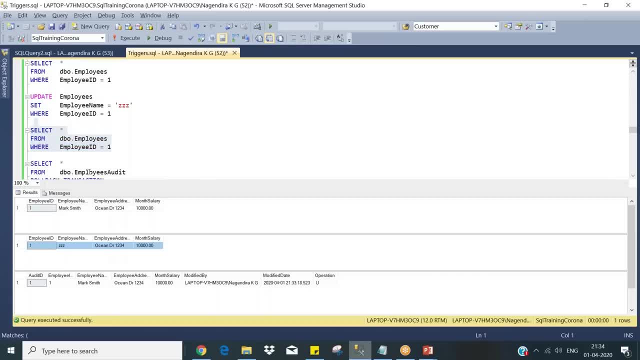 i mean this select statement has given you this result. then i'm selecting from the employee audit table. i didn't do anything in the employee audit table because earlier you see only one. four records i have created for mark smith. i'll change it to triple z. what has inserted here? 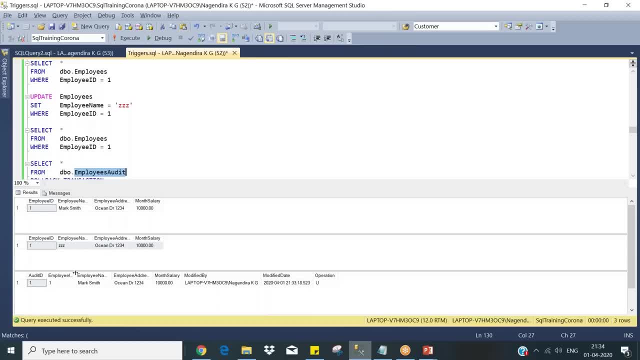 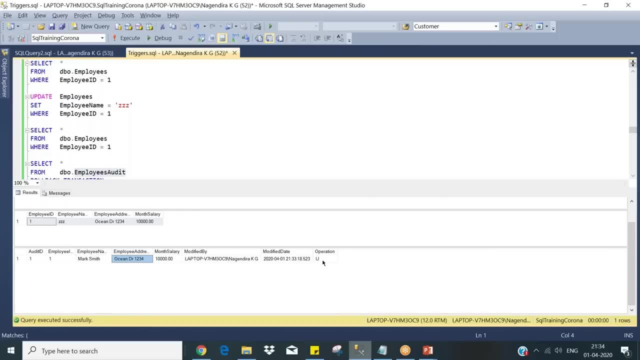 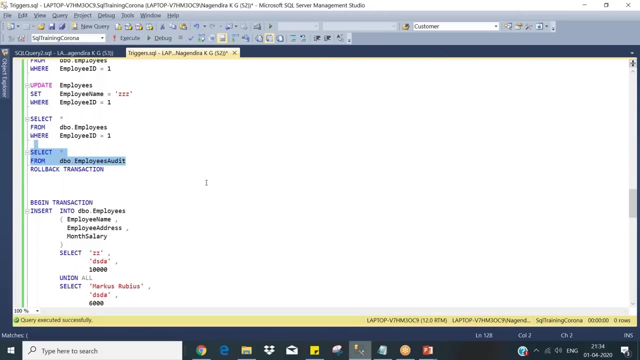 audit id1. employee id1: mark smith. mark smith was the old value and i did a update. okay, mark smith was updated. this is the thing next i'm going to do. see the magic guys here. i didn't say about transaction. let me explain that one along with this. see, if i do along with 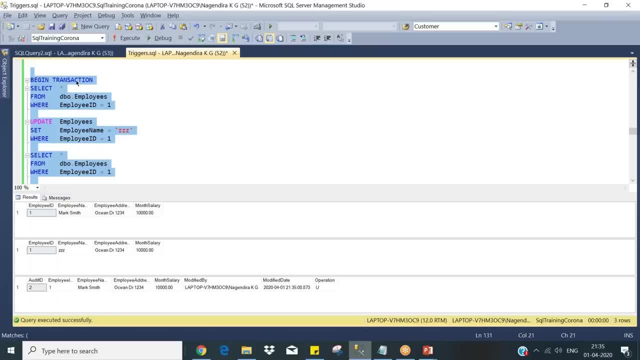 all other stuffs like this. this begin transaction will make you to have the batch execution, whatever statement followed by this begin transaction, which run in a full batch, where the data interests of the transaction within the words Nah, take인데. will be setup. so the transaction is. scratch is open, so the transaction will be started. 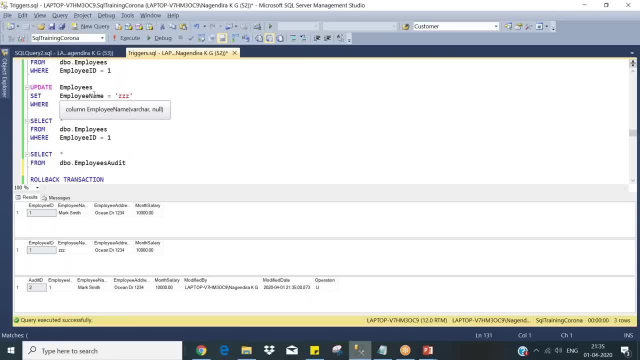 then each one has no words. so after this transaction you say commit here, then only all operations, whatever it performed, will be updated in the respective tables. now you see, like we executed this command, i mean, uh, along with the begin transaction, end transaction. so, mark smith, what i'm trying to say is: 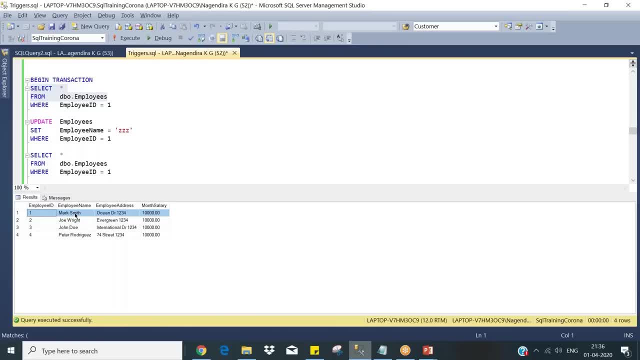 one. we saw like he has got updated triple z. okay, why it is not being updated here in this employees table? because we have rolled back the transaction, so all these things are rolled back. it will not happen in the actual table once i say commit, okay, whatever operations. so when i run update here, see when i do only the 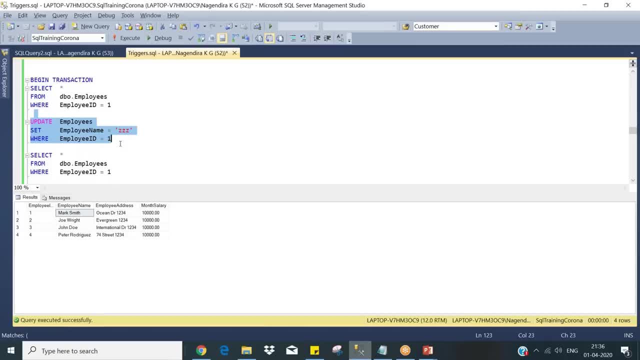 selection of this query alone, i mean, uh, update alone, it will auto commit. there is no begin transaction, no end transaction, commit a rollback transaction. so this is another important factor here. so what i'm trying to convey is like: now, instead of roll backing, i will update this guy for one. i'm going to run begin. 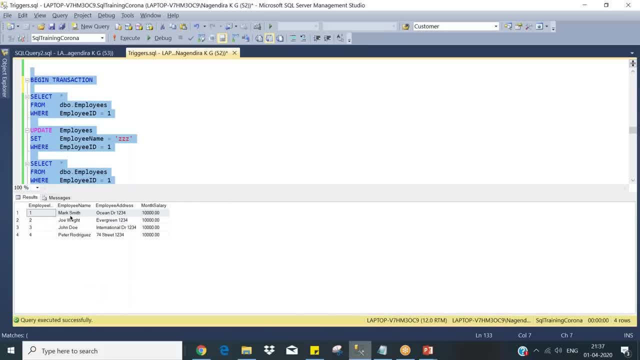 transaction to commit, then this time, when i execute this employee for one, it will update it to two triple, is it okay? now, again, it is saying the same. now, you see, is it? that is for uh, instead of mark smith? you have triple, is it now? so? rollback transaction is like whatever you. 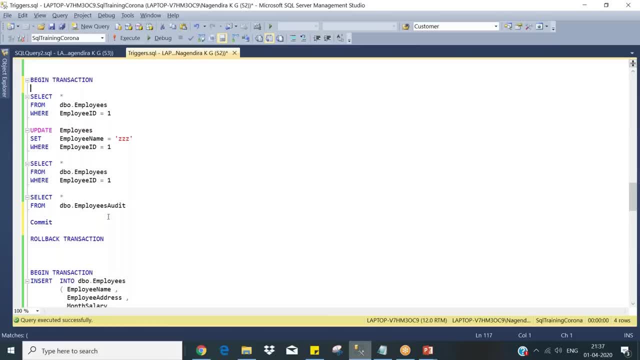 have a code between begin transaction and this transaction, all the statements will be rolled back. that will be nullified, it will be, uh, ignored all those comments. okay, that is the main purpose of rollback transaction. oh and again, when you roll back, you need to doing: uh, including the table name right: employees audit. 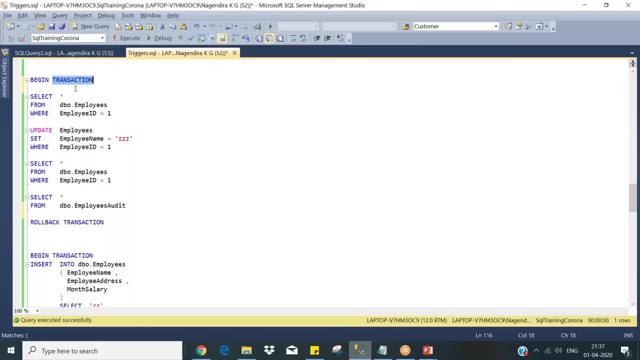 no, no, no see. rollback means begin transaction. so it says rollback means all this operation, irrespective of the tables or whatever operations you do, everything will be stored until you say rollback or commit. you say commit, all the things will be committed. it is not for the table. transaction means batch, irrespective of the tables or 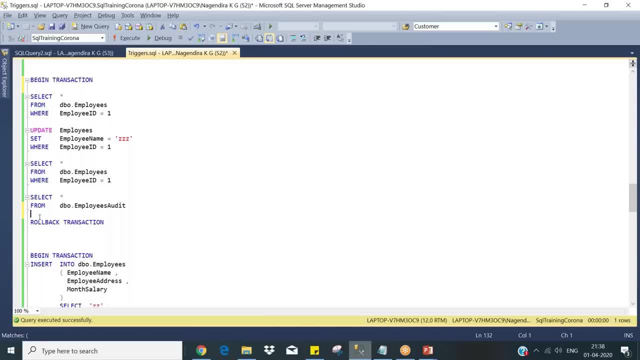 procedures, what you call okay, okay. so when i begin, see, whenever, see, i have doubt. when you say rollback transaction, will this rollback only for whatever we have done today or any any time within this code? it's not for today. begin transaction. you're saying from here to till this previous transfer, if you do update here, that will not be rolled back. 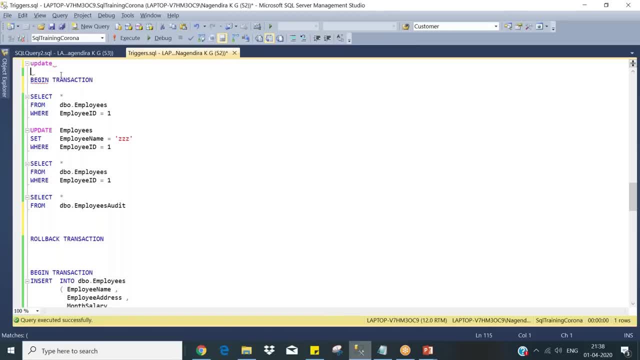 if you say here, if you put some update here, that will not be rolled back, you need to execute as a batch, like this: if you execute within this, it will, it will update or it will roll back, okay, okay. yeah, this is what i said: batch. you run it as a batch, so all the usually in uh stored. 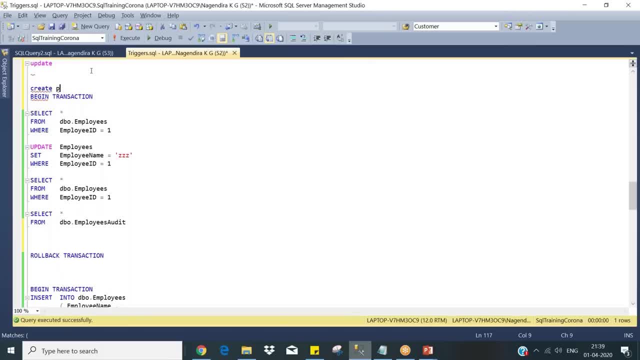 procedure. they will write like this: create procedure, begin transaction, end transaction. begin should be at the beginning and roll back or end should be. if some failure happens, they will go back to the beginning and they will call it as a rollback transaction. if something, everything goes smooth, then they will commit it. so these three statements is very important. if everything, 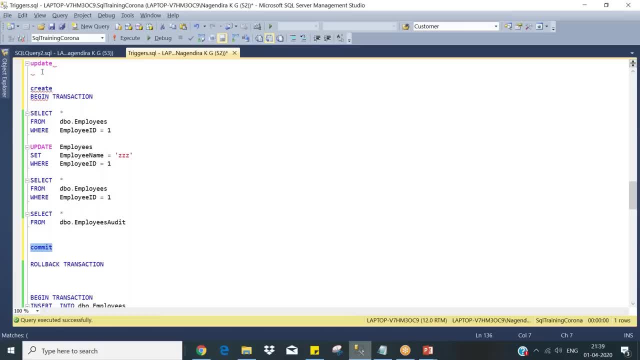 is good, then commit it. if something goes wrong, roll back it. okay, forget about that. uh, let me update again. maybe look at directly. let me check this next point. i see the model is max with okay. okay now. so you got it right, guys. so now you see again the audit table. now i did. 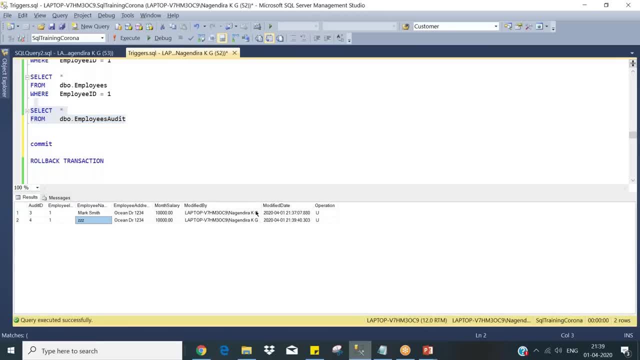 many times. okay, these are two times. i did and it logs me modified who user because who has done that. that is why it is getting in the first of your trigger, first line, or a few lines of the trigger. now, here, what i'm doing, i am making just a change, so i am selecting the trigger again now. so that we are going to use this for today because we have made the change here. so now i am designing that a little bit, and now i am going to make the change a little bit. and now here, what i am doing, i am making a shift, i am working on a code now just making a change here so that you just 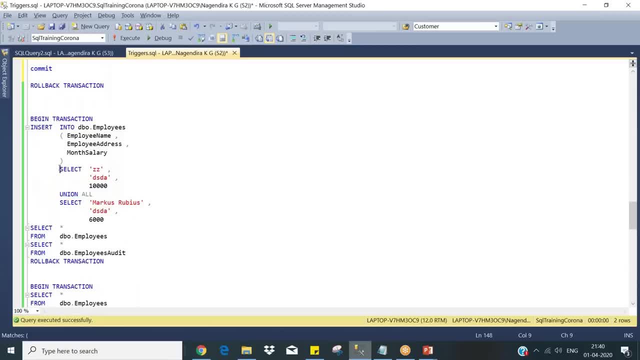 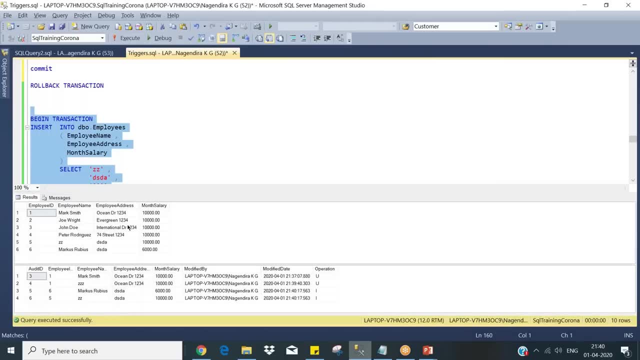 I'm trying to insert. see again Union, all all these things people are using again. here I'm doing the rollback, let me check. so here what I'm doing- I inserted these two records- is that is that Marcus Rebius? and here it is trying to insert. 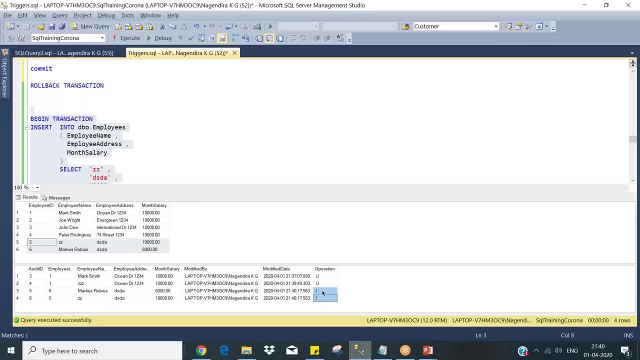 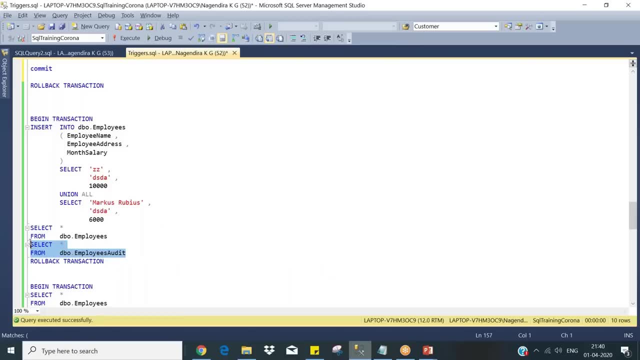 in the audit. also, I'm getting the operation. what operation I did? I'm not doing anything here, but it automatically does some job. you have only two records. since it is rollback, those two records are gone. okay, guys, so this is the load triggers. I hope you got it. you no need to do something certain. 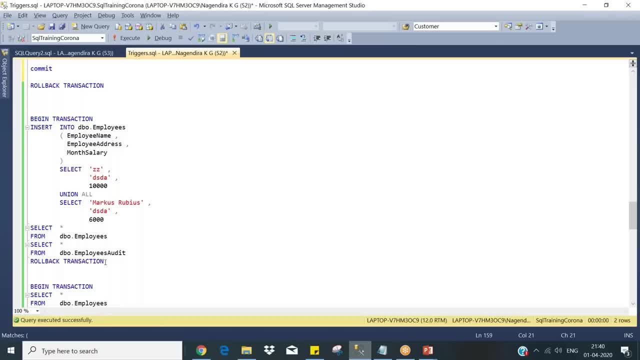 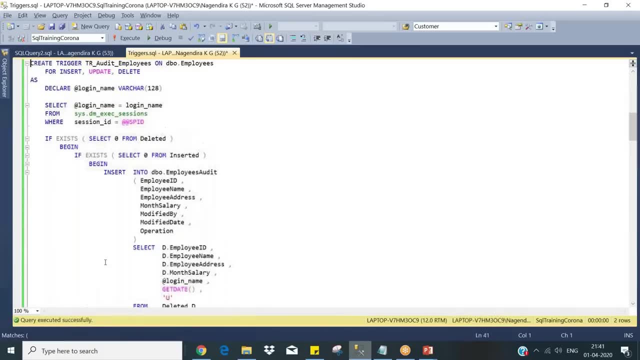 things that should trigger some other operation. what it should, it has to do. that has defined in your trigger logic. so I need to initiate trigger on this table for these operations: insert, delete, update or select also okay. and what it has to do it will do: insert or 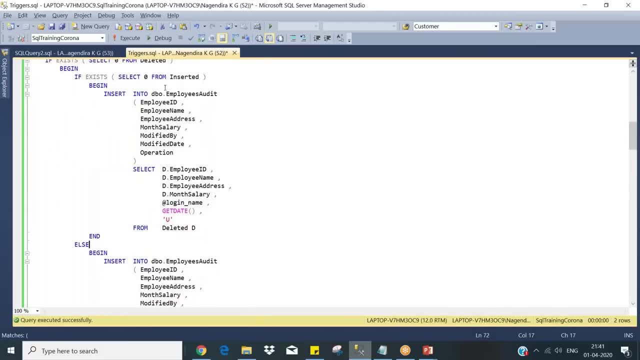 delete into based on the logics. so this: I have spent some temporary tables. it will keep based on the insertion happened. so using that, it is inserting into another table. so this is your trigger. here you can send us, as usually will send the emails. that is why I know I'm. 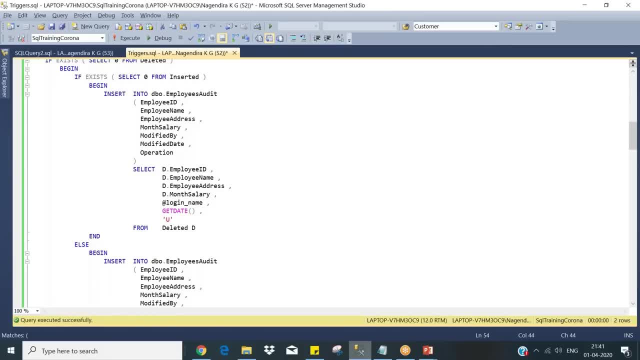 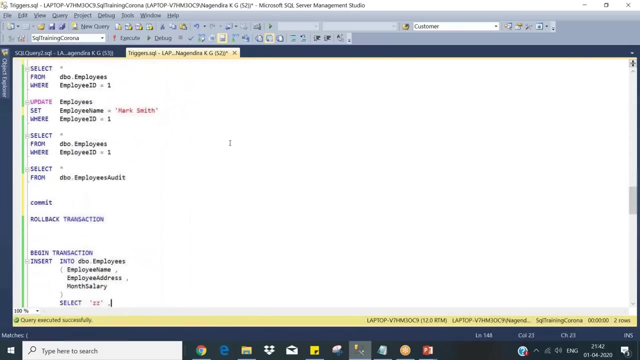 pointed out. if something happens, say, for example, someone has deposited huge amount, then you can write some logic there, in that you can send emails to your managers, alerts, all those things. okay, for those purposes we will use triggers. okay, with this note, it's more on to causes. so just now we discussed about triggers. 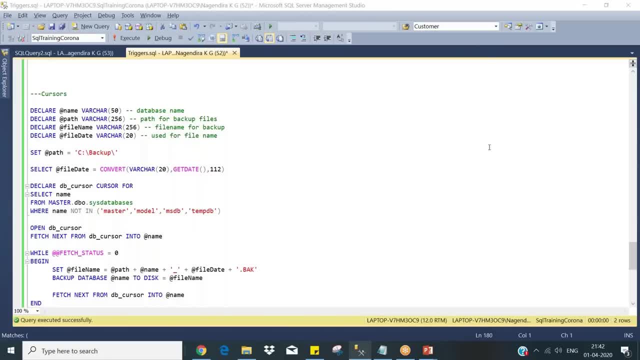 that's one. two causes curses when we use. so there are certain cases like all these operations, select statement or functions are stored procedures and these things you are running as a set operation. set operation means for a table, okay, for a entire row. you are selecting, entire column, you are selecting as a set operation. 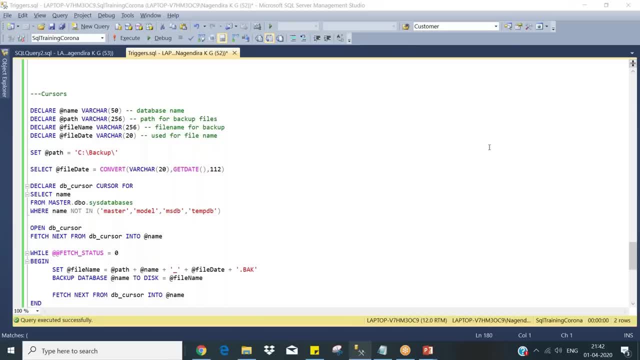 but what happens? i want some operations to be performed for each row, one by one, like looping. okay, you basically it's kind of a looping operation. okay, those kind of stuffs. you go for causes, so causes. if you have a 10 000 records in your table, you want to loop. 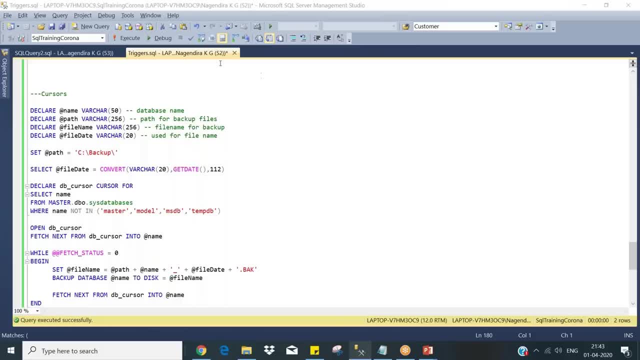 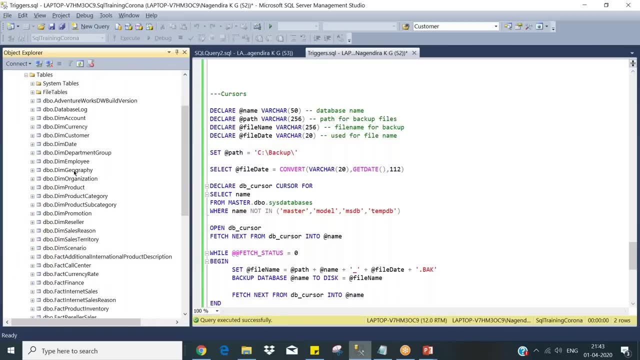 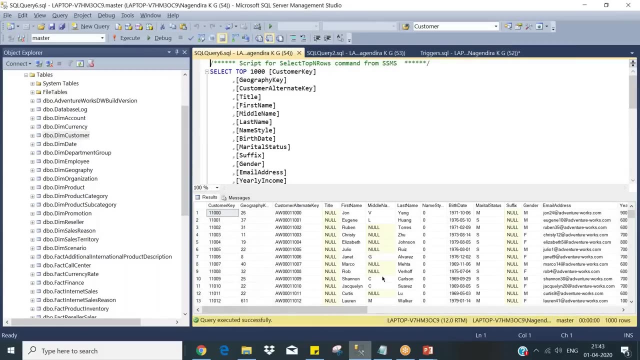 through all the 10 000 records to do some operation. let us give one example so say, for example: uh, like today's corona case, like these are the guys who has identified as having a corona. and i want to identify for each customer, whom, whomever he has met, those kind of 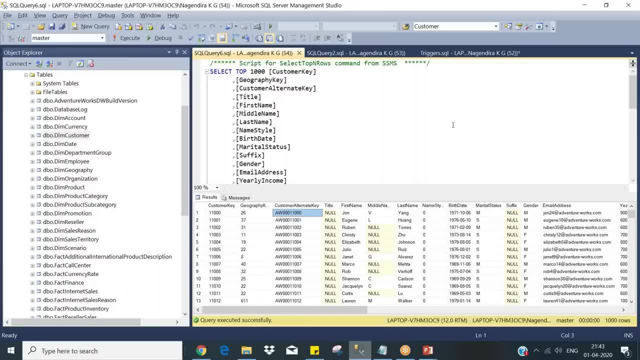 steps: okay, so i want to identify for each customer whomever he has met. those kind of steps- okay, that information, you have it in some other table, so you need to pass this guy- okay, in some other table and you need to fetch those information, whomever he met, something like that, okay, so each. 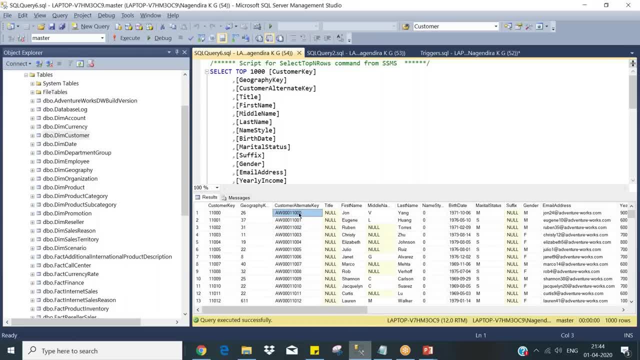 row, each customer you need to pass. this will be acting as a parameter and for each row you are finding something else, and this procedure should run for multiple values, row by row operations. it's like a looping. that looping can be anything. it can be a thousand rows or 10 000 rows. 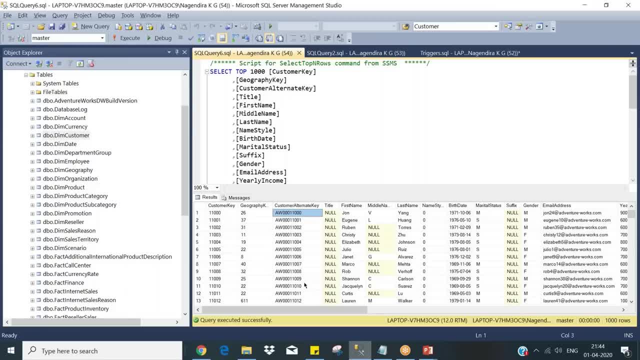 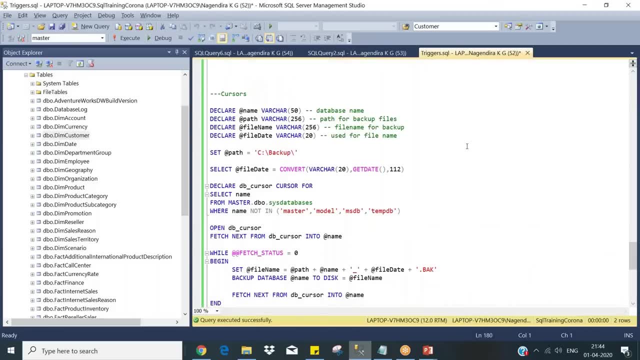 such kind of operations if you want to perform, then you go for courses. let's have a quick look at an example, then you will understand much better. so here, what, uh, they're doing is like in this example. they're taking um backup. okay, we are going to call it back up, okay. 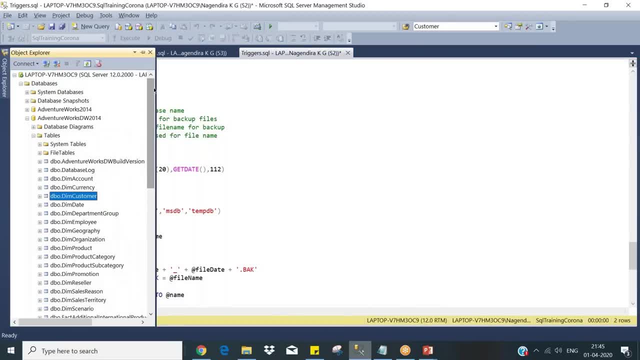 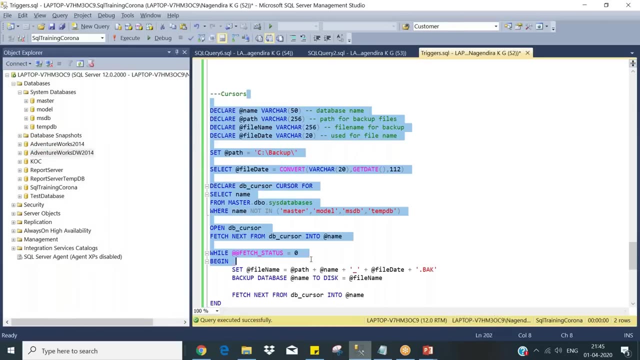 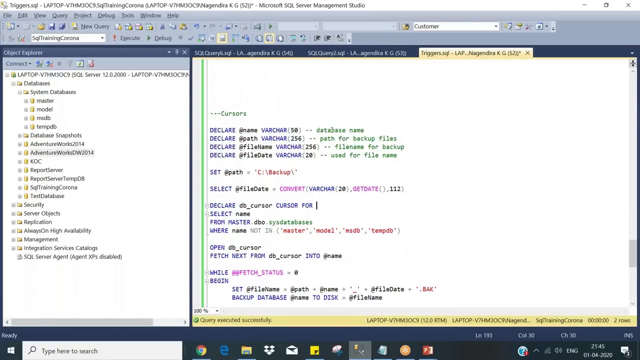 to take a backup of the system databases over here automatically. you have four databases back up. okay, I mean these things to be taken automatically when I run this code, single piece of code that will take my backup automatically. that is the main purpose. let us see the code so here. so these are the variables as I 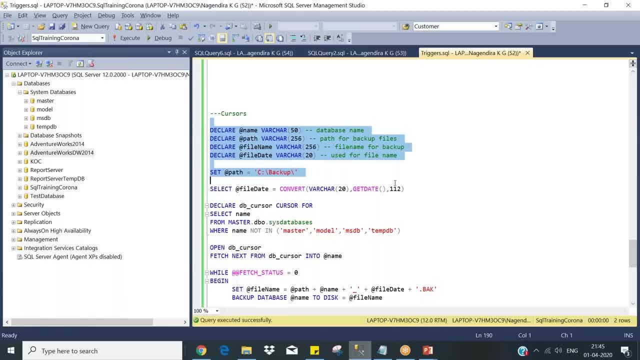 said before, these are the variables to store some temporary results. okay, and code for a cursor starts from here. so cursor, declare cursor. okay, I mean here it follows the name before you. it's like a variable only guys. so declare cause of name. here you see. declare variable name and data type. so similarly, declare cause your name and. 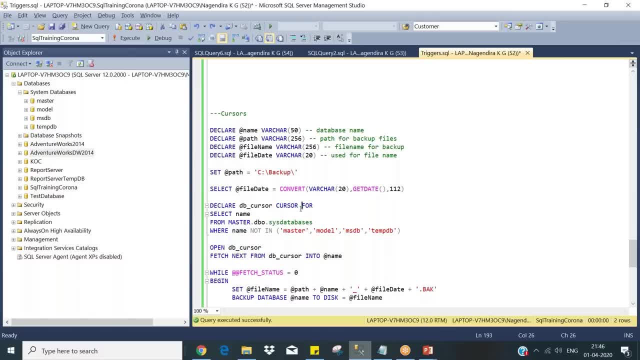 your cursor is a keyword for. for see, these are the things it will have as a list, like if you have multiple values, or in my. in our previous example I quoted all the values that are in the list and if you have multiple values in the list, you can give you the list beginning form. so first long line tentar is你们. 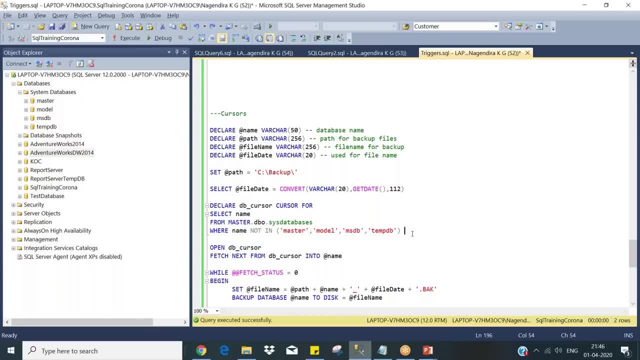 all the customers you want to loop. so that list you need to keep it here. your query should return whom to loop or what to loop. thousand records and thousand customers, those customer list. it should written here: okay, so that information is stored in your cursor. then what you are doing, then you are. 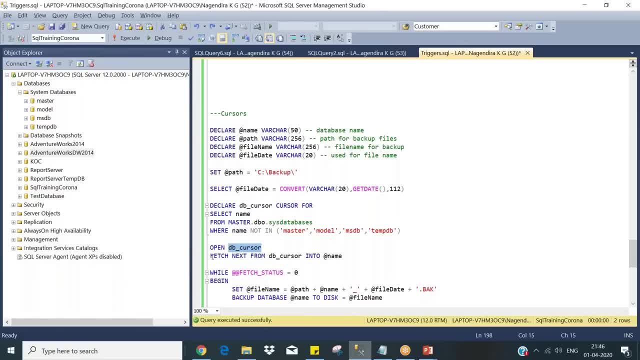 opening a cursor for unbelievable information at your place of the list and you can give any data statement and the data is different to each other, which becomes only the final essentially data I could give. and then here you: ii support the component for each row for fetch next from this cursor and store in that variable. so I 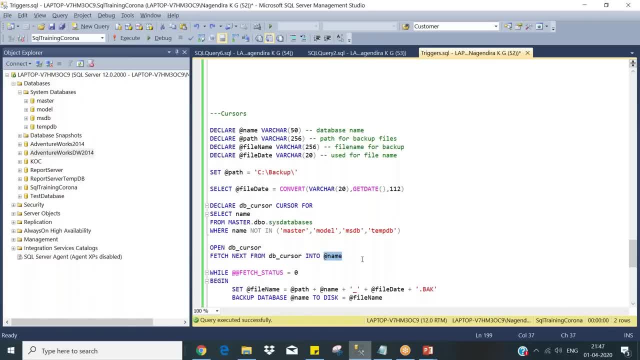 hope you guys remember you worked in any programming language. you need to loop means. for each loop you get a value as 0 to 1, 10 times you 1 to 10. you need to print means. you will specify initial value 1 and the end value as 10 and each. 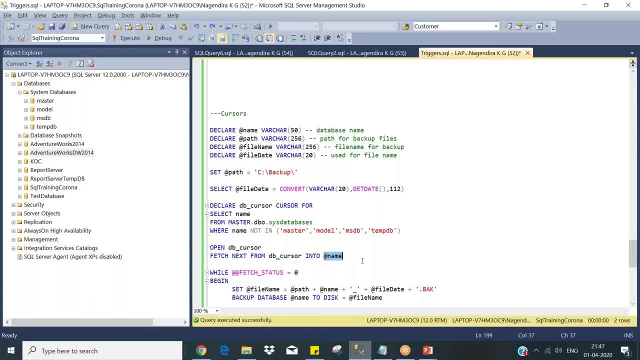 value you loop means each value. you will print 1 and you will assign the value to variable to calculate something and you will assign, then you will look through the increment, the value, then you look through same logic here. so first value you are getting. I mean you assume these: 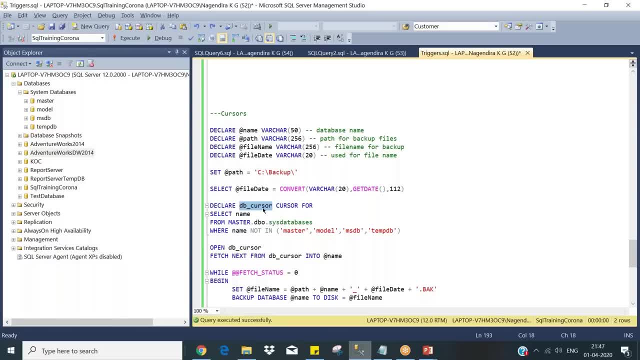 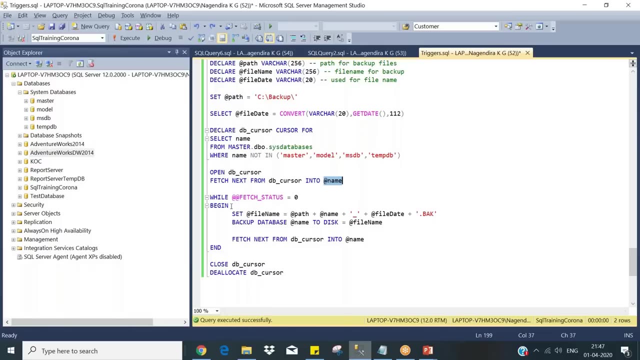 will stick to this example. so four values are stored in this cursor. it is fetching the first value, okay, master, and stored it here. then that master it will keep looping through using a while statement because at that first status, if you declare a cursor, and at that first status, meaning whether the cursor 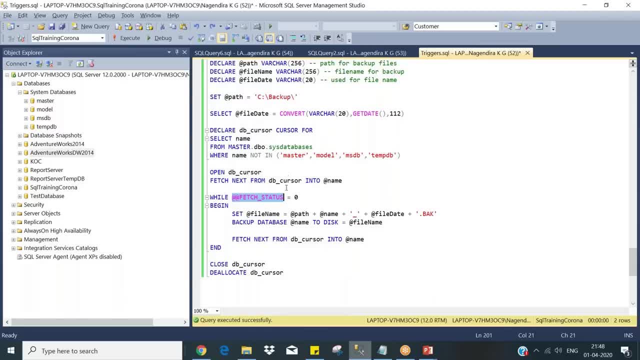 has a value or not. when you say fetch, fetch next from a cursor, it fetch one value. when you say again here, fetch next from cursor, the cursor will point to next value. I will explain that little better in Excel. now stick to this example. master is stored here, it will. 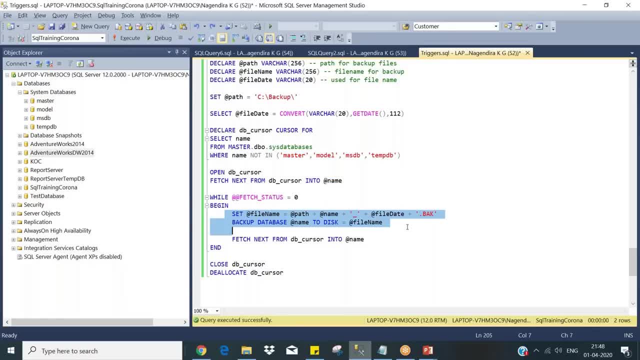 check. this condition is true, then what will happen? this is the code: whatever logics here, only you need to write your logic in the while part. whatever logic, as I said, for thousand customers, we need to take over whoever he has meant. so those information you can write. 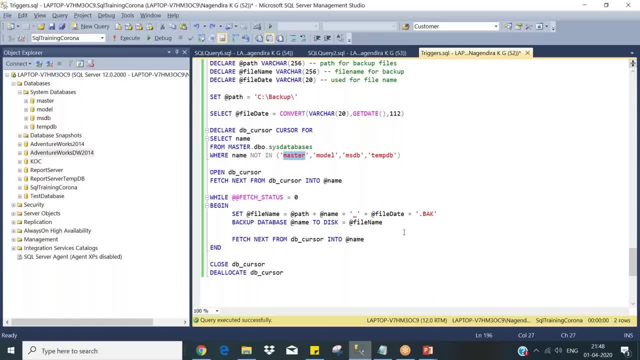 here. okay, so in this case for master, it will generate the path, then this backup database query will be fired, then that will take a backup. okay, then what happens once it has taken a backup? it will go and check model. second value, fetch next from D, because are into name what it will do: it will take model, it will the while. 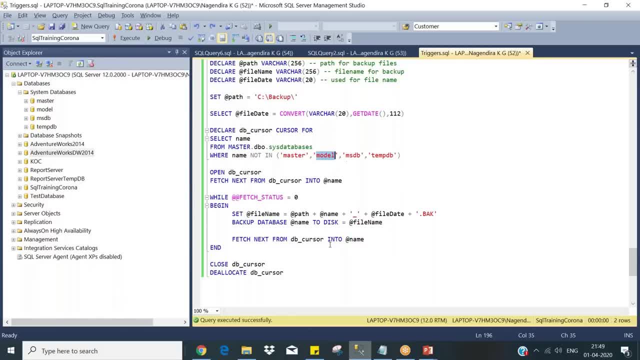 condition is true, then it will take model back up again. this condition will say for MSDB: it will check here. this is also true. this will take back up for MSDB. it keep on going. once temp DB is taken back up, fetch next from DB cursor into. 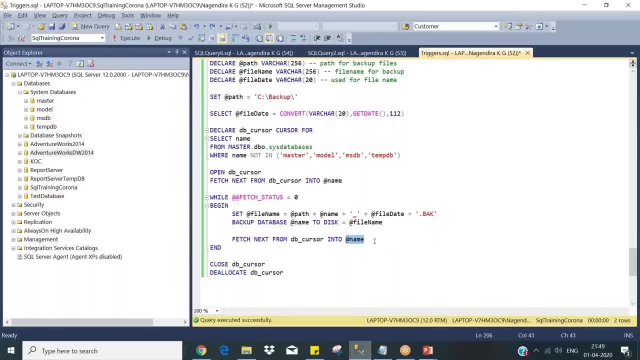 name. this will return zero or null value. okay, it's not an onboard channel, then it is still defined, and then it will exit, because when a, let's say the javascript here so same that it's not an in Den shitty, doesn't. so here we just took it out and immediately. 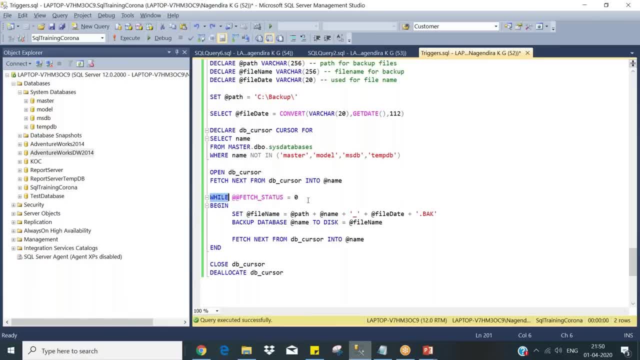 it will now Alec, and then that's the two else question, of course, and it will fail. okay, basically, it's a looping concept case. you need to use the curves because they're nothing, but it will hold the list of values for those, list of values one by one. you. 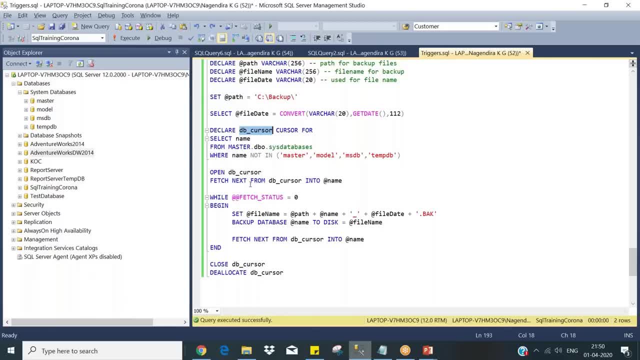 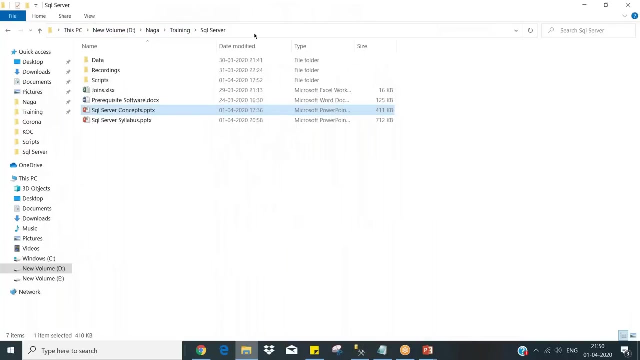 need to process. okay, one after the other. then you will use for each value what operations you need to perform that operation. you need to specify it. it is as simple as that. let us have execute this one. i didn't tried. i need to have, um, the colonizing. maybe training will. we will take backup over here. 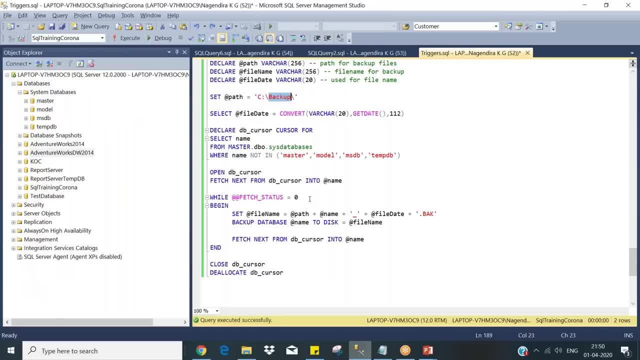 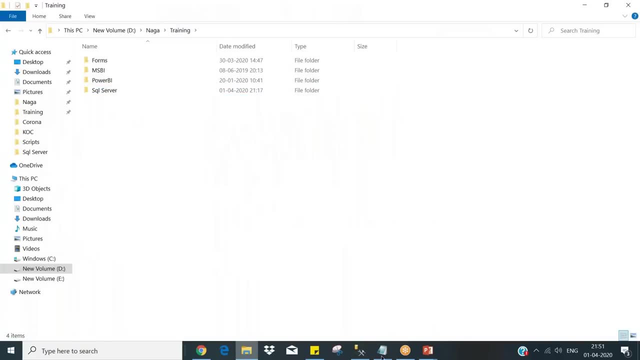 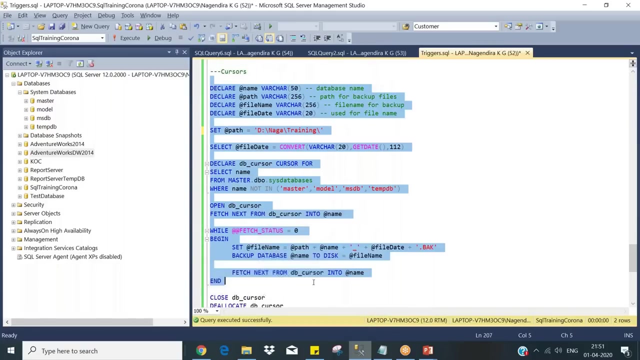 because sometimes the space in the file name will throw error. okay, i want to take back up in the colon training naga. let us see whether it's there. nothing was there. let's try to execute. i'm running it for the first time. i hope it should work. 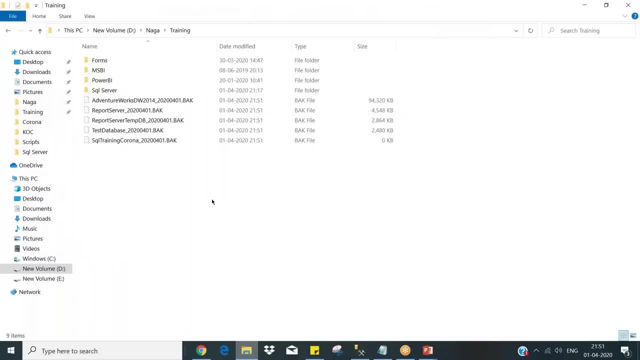 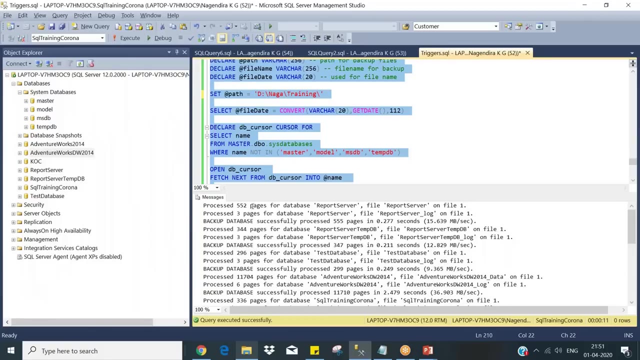 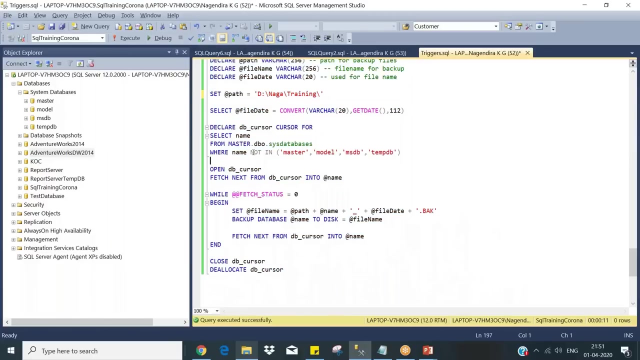 there you go. oh, my god, i'm running it for the first time. it has taken backup for all other things. okay, i think inside each thing it has taken master database backup, possess, for example, server. okay, okay, okay, okay, fine, guys, see, the code is not uh, in it is saying it's not these four conditions. 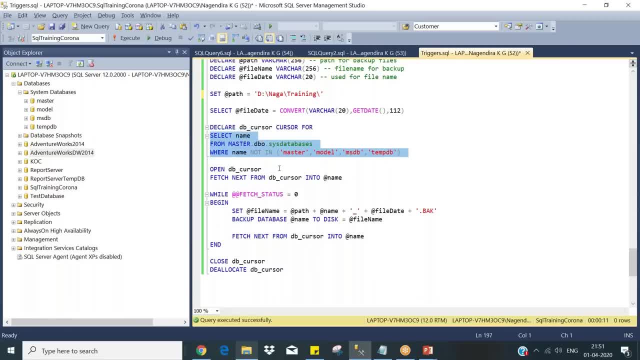 it is not in, Not In means whatever names it has selected. don't take the these four database. you take all other strings. i have done it the way it was not specific table. there are only four mounting other database, so that's why i've taken all these things. our example is correct, only so adventure. 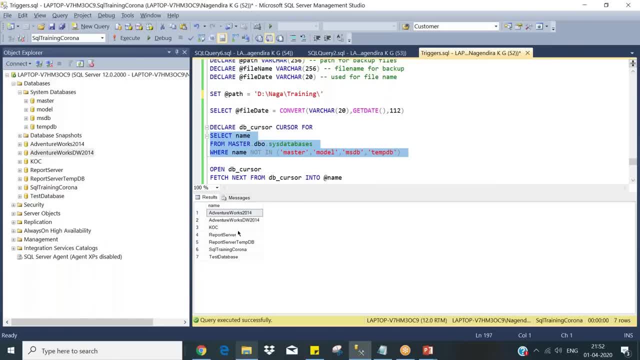 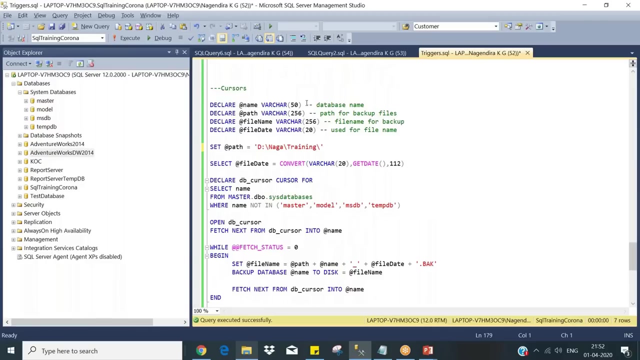 works. so there are seven databases. we have, okay, this list. they have taken one, two, three, four, five, six, seven. okay, you got it guys. now you you see the practical example of it courses how it works. so it will be really confusing for you guys when to use procedures, functions and you have a triggers. 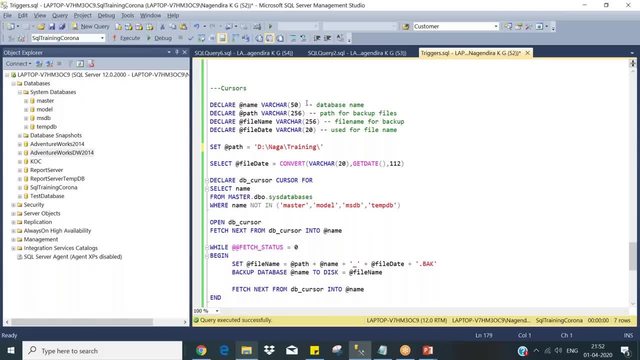 causes. okay, you all came through it. i mean, once you have experienced this one, different scenarios will come into place. at that time, you need to be in a position to choose between either of them. either we need to go for triggers or we need to go for courses. which one fits in that scenario? 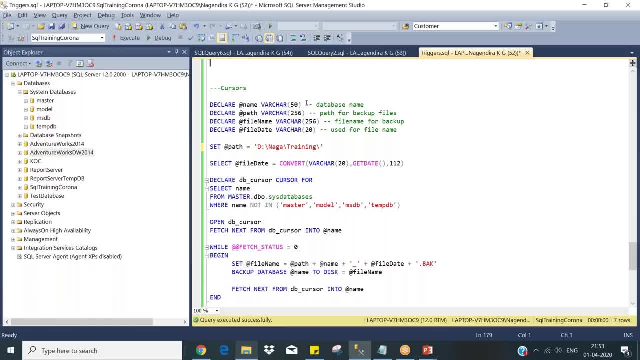 okay, at that time you will you have to decide, but you need to know what are the different things, what is the purpose of procedure, function, triggers and causes. got it guys any doubts? no, okay, a few guys, uh, having no doubt. then i will explain the joint spot today's session. i'm fine, i mean, i'm 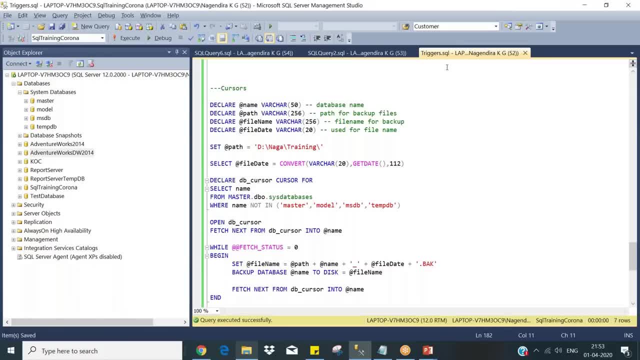 done with today's session. let's focus some time on joints, or you want to take it tomorrow as a beginning? today is at the end of the class. you guys are very feel bored. mother, yeah, i'm having a lot of fun today, so i'm working on that. yeah, good. so, guys, uh, what do you think? guys, uh, can we have? 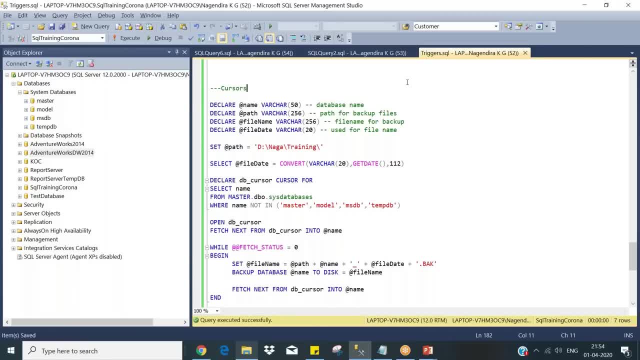 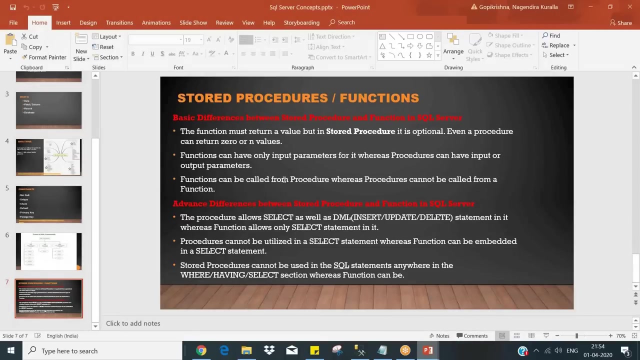 our joints now. uh, tomorrow, hello, no suggestions tomorrow. i think two options tomorrow. then we can have tomorrow because we will start fresh. then it will be easy for you guys to understand. okay, let me summarize uh today's session then. so we started with um, uh functions and a little bit of short procedures. what are the difference between uh, these two when to use? okay, 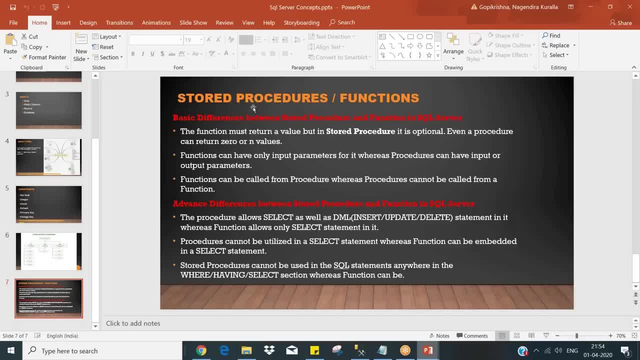 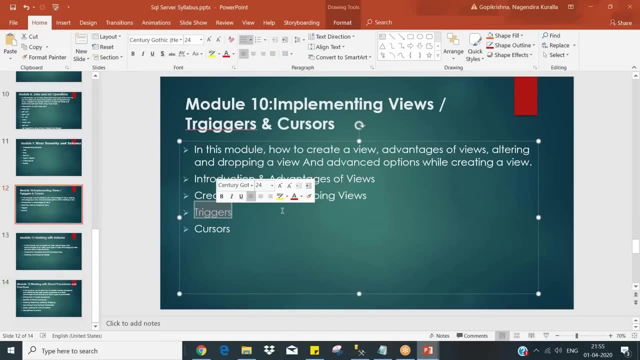 these are the combinations. you should not confuse with stored procedure triggers, causes, short procedures or functions. either of them, which one to choose? okay, then we uh worked on um triggers, so triggers which used to trigger some of the operations based on certain operations that happen in any of the object. okay, cursors when you want to loop. 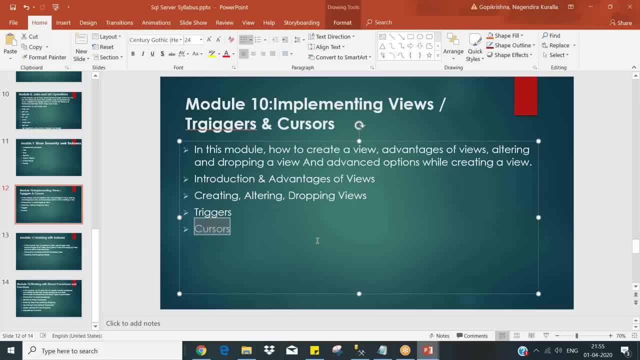 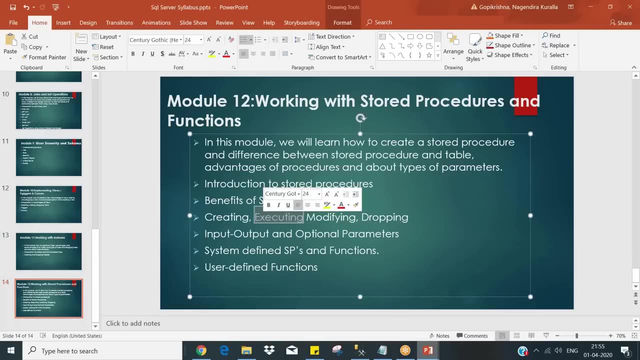 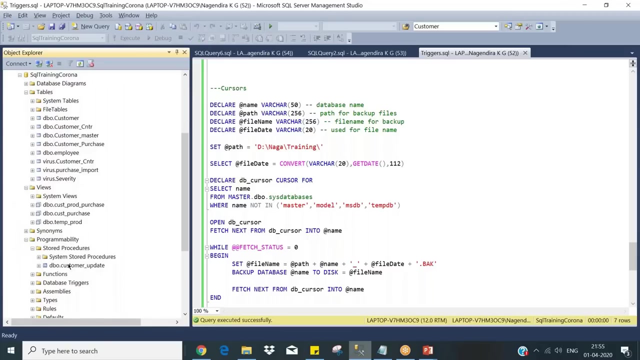 through. uh, you want to go row by row operations? okay, in that case you need to go for courses and i hope, uh, i covered everything: creating, executing, modifying, uh, so these things, uh, it is very simple, it's one-liner, like we had a function uh procedure here. 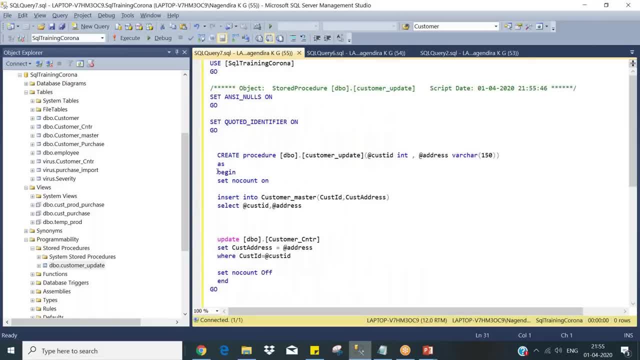 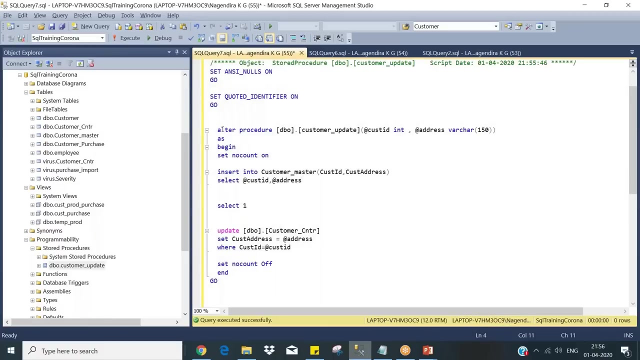 so yesterday itself we saw this, so create procedure instead. if i say alter- okay, this is i- i say like: i want to amend some code here, so i have modified something, whatever it can be, so it's modifying. okay, it's as simple as that. i don't want this. uh, procedure means drop. 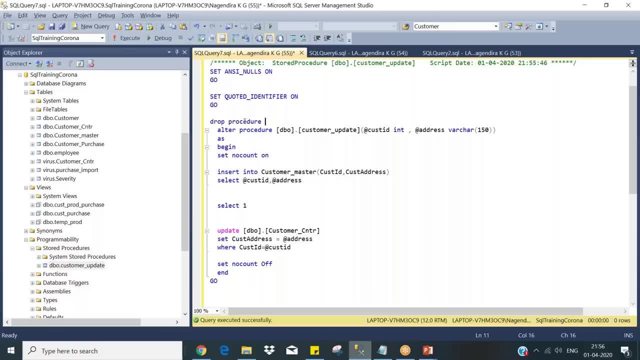 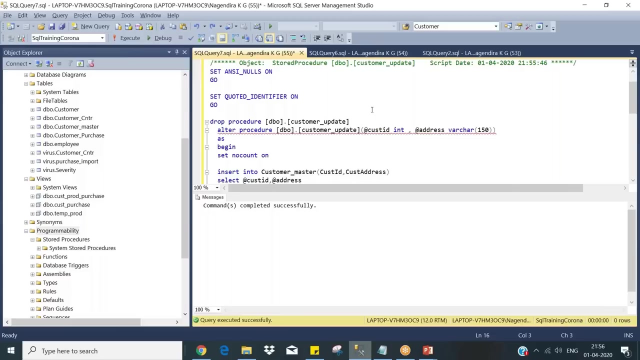 so drop procedure procedure name. even you can delete it. this is the code: drop procedure procedure name. so once i do that, you see here you have customer update. it will be gone. you won't find it. i can recreate. that will be useful because no need to store this content. 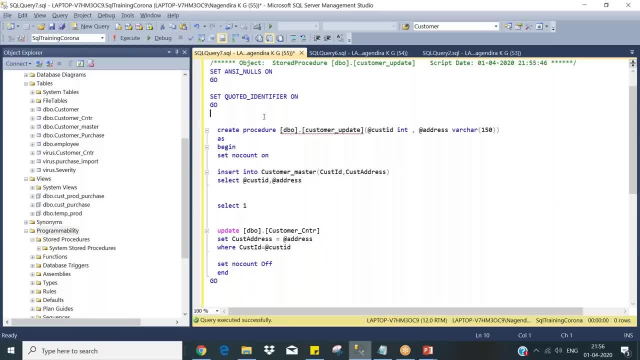 once you have a procedure or view defined, no need to store physically as a script, you just need to have it in your database, keep your database safe, take backups regularly. i got my back, so these are the things as any object you go for, create procedure, alter procedure. in this place you can have view or table, whatever, then use. 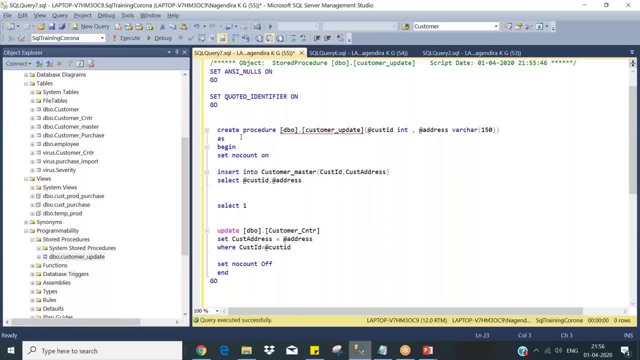 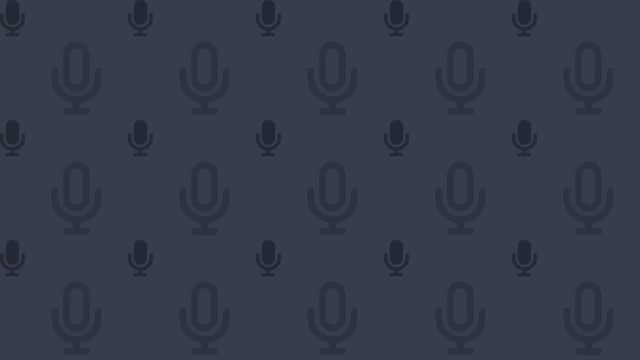 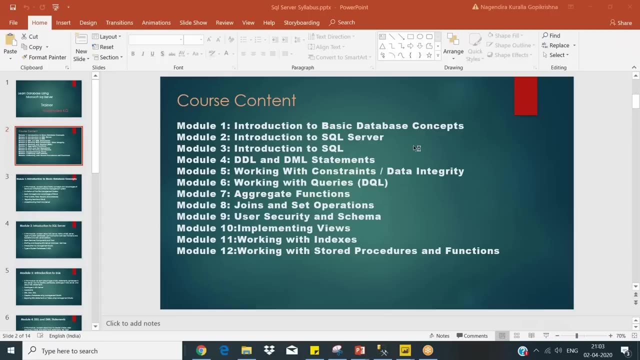 that appropriate objects. this is what. okay, so about that, then. this conference will now be recorded. okay, so, guys, so this is our syllabus. we have seen from the beginning and the topics almost I have covered. just, we will quickly go through it so that you guys will remember what are the things. 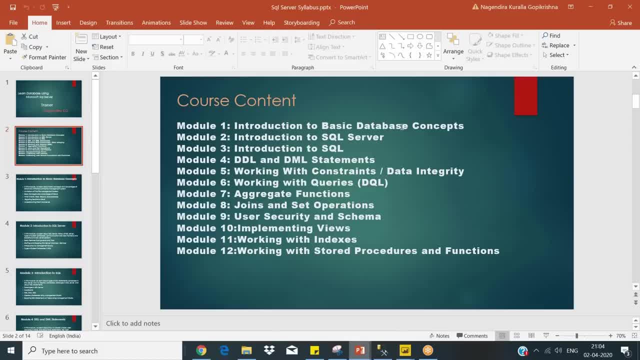 we have some so basic stuff for database concepts. like you know, you have to have a lot of information. you have to have a lot of we see about. what is the purpose of for database, what are the disadvantages of your file systems? all of the steps we have seen in this and introduction to 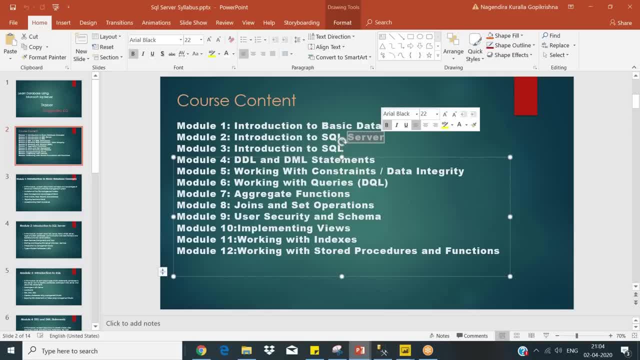 skill server. and here in this module we have seen about our DBMS relational database management system. what is the purpose of it? each table is a relation and management studio, how to log into your client, how server client is architecture. then in this module we saw about the purpose. 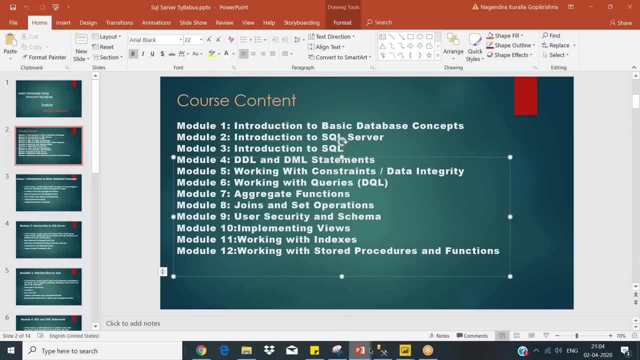 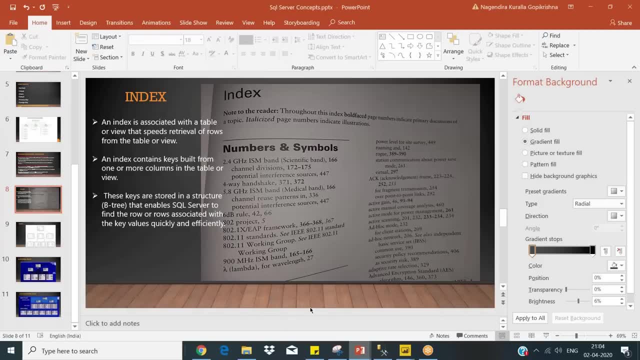 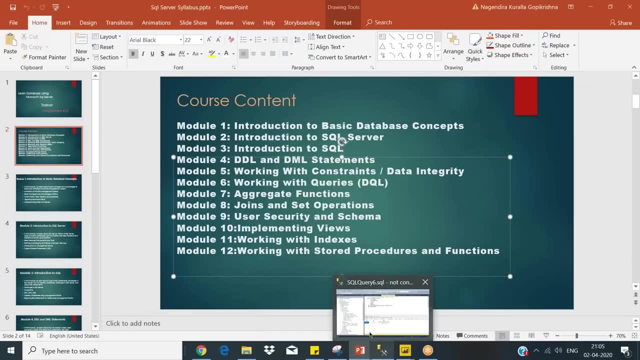 of SQL, the structured query language. this is the language. use it to communicate between you are and hello, Deepak. I'm just going through the syllabus, whatever we saw, so that we are in sync. what are the topics we have covered? it's just a refresher session, so 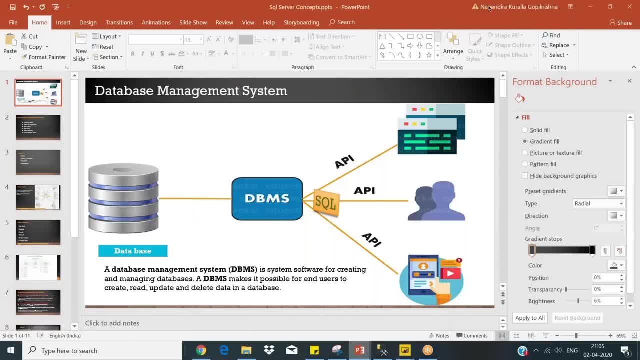 we learned about. yeah, he learned about databases and I hope warrants adjourn, weren't it in China? let me see, I'm sure, why you didn't join. that's fine, let's continue. so we saw about a skill, the purpose of a skill. a skill is a. 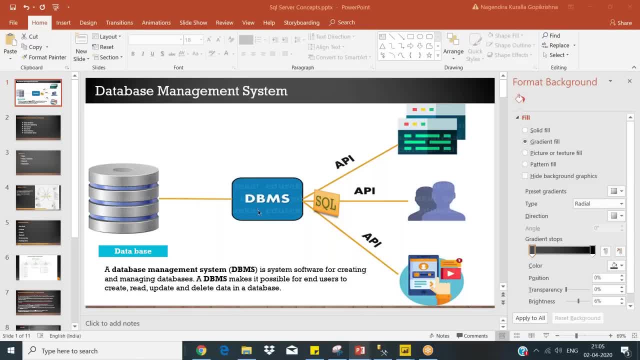 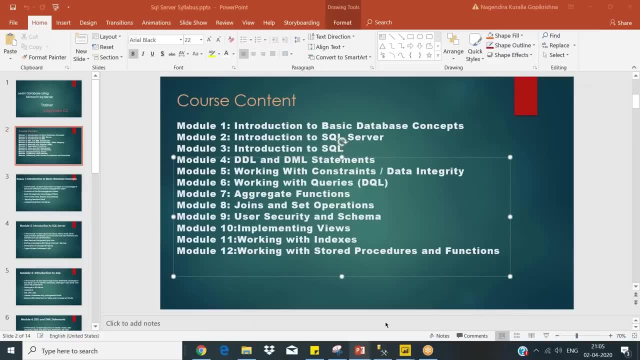 structured language that is used to query your DBMS database and it will return the results to your client applications and we have a DDL statements, DML statements, DDL data definition language that is to create and modify, drop your tables. DML. you need to manipulation language like insert all of the steps and you have a DQL data. 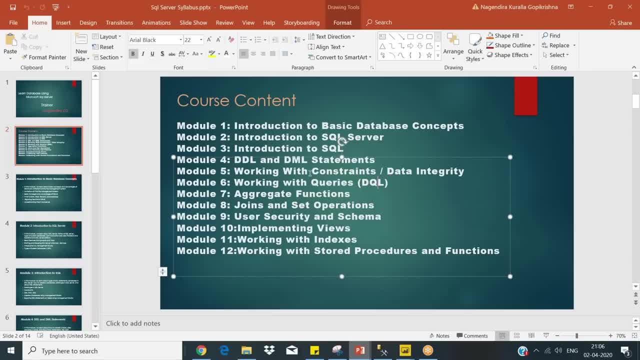 coding language. it should be coming here. we have come to the end of the session, so thank you very much for watching and we will see you in the next video. bye, bye, Ver, that one. so these are these different statements we have seen. then constraints to have data integrity constraints. you guys remember like we 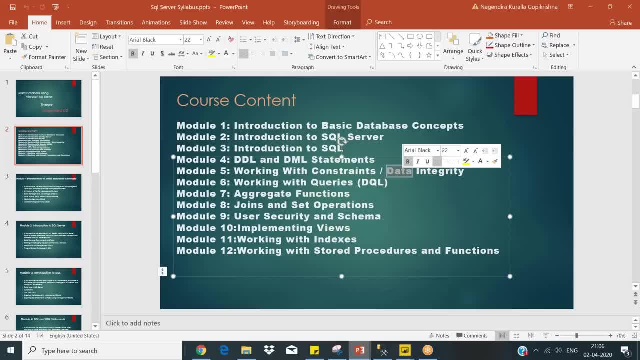 had a non constrain, not now can shine unick constrain, primary key, foreign key. so these are the constraints: check constrain to ensure that there should not be greater than 18 or any combination. so those kind of constraint to define your, your data integrity. then we saw about aggregate functions, some average max you need to use group. 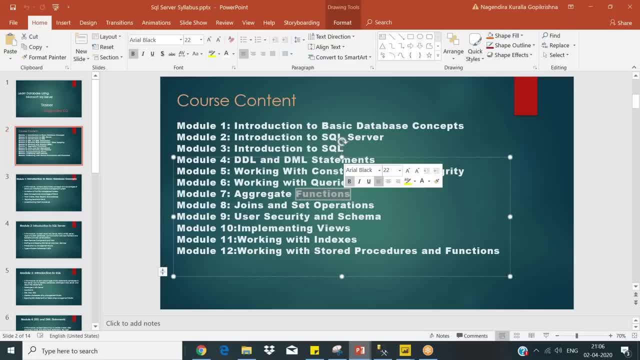 by. when you want to aggregate, you need to use group by and we saw what joins joins. in order to get information available in another table, you need to use joints- i'm going to cover this right now- and user security and schemas. so we have created a user and it is not all the users who 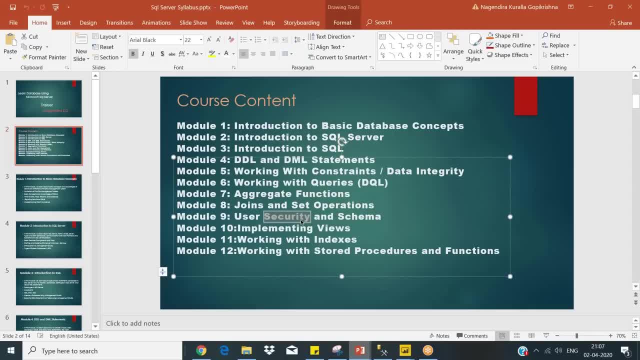 logs into the database we need, can access the table we need to create certain tables- i mean users- and give respective rights to him. so we see, like one of the user we have created who has access only to three tables, he can able to select. remember it. and we saw about user security and schemas, schemas, grouping of objects, you know. 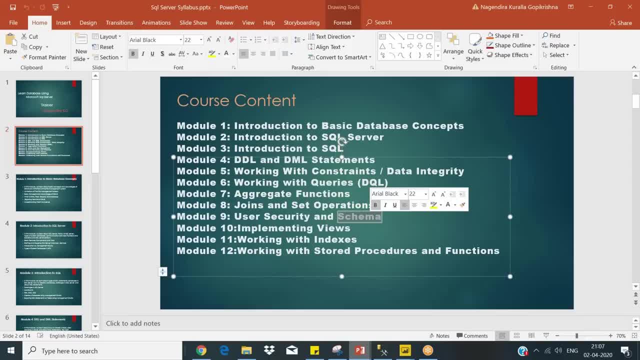 you can create a schema. schema is nothing, but you are like a functional area for human resource. you create one schema. all of the objects you create there, you can map it there. it's like a folder. then views. we have covered use purpose and virtual table. the data won't be stored there. it's like you can combine multiple tables. 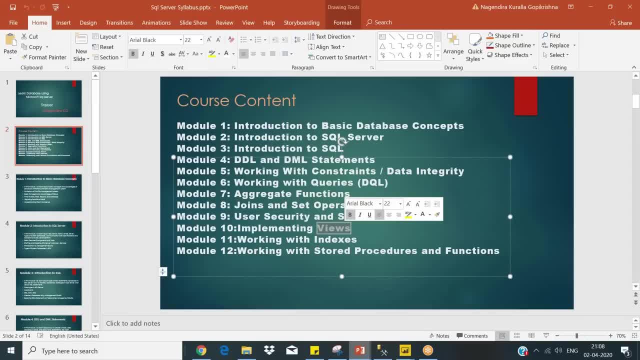 as a query, then store it there. the data won't be stored there, just a query will be stored. another purpose of use is to give you a security. like people should not access to the tables. instead, you give multiple tables in a query, then you can access. i mean people. 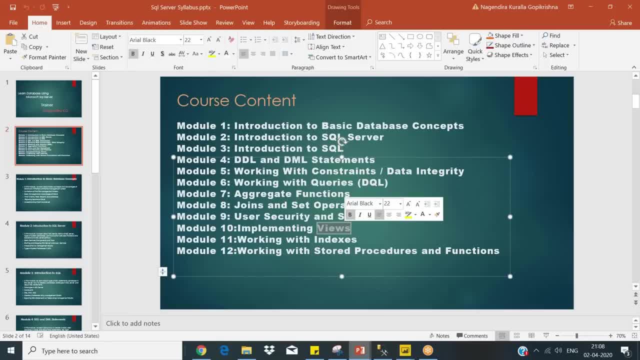 can access the view instead of four tables. so both the purpose of sharing data with with other tables, basically so that way you can provide the same kind of information to the user in the same way you do the above here. we can provide some data in this way, so i will tell you how it works. 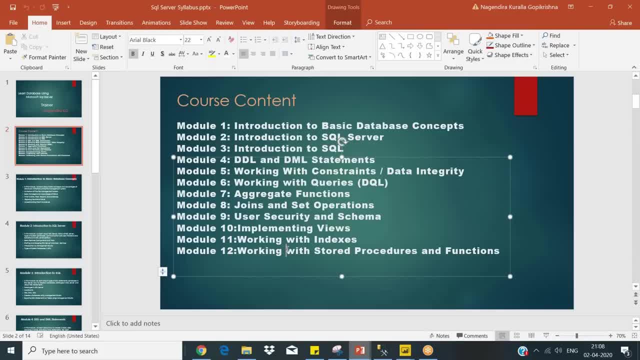 so, for example, we have a score chart on a block, so we don't need to do a fixedval score chart. we could have a fixedval score chart. we could have a fixedvel score chart. based on that, you will write, write your logic inside your procedure. that will do the respective. 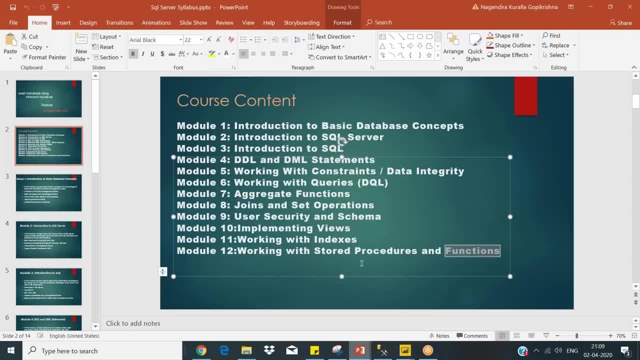 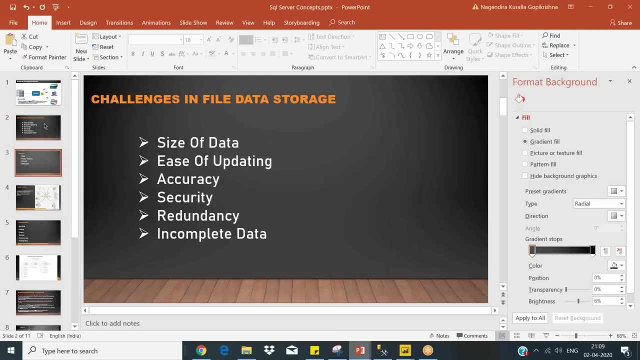 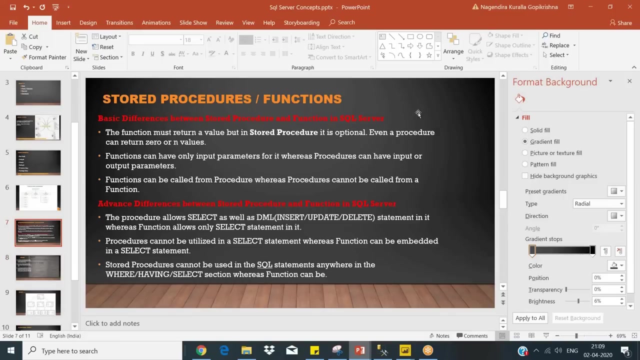 task functions, any calculations. so yesterday we saw deep difference between short closure and functions. i'm going to share those. this ppt about the ppts which i have. this contains a syllabus and another vpt contains some of the key concepts like this: so these are the things we have covered. so today's focus is mainly very good topic. 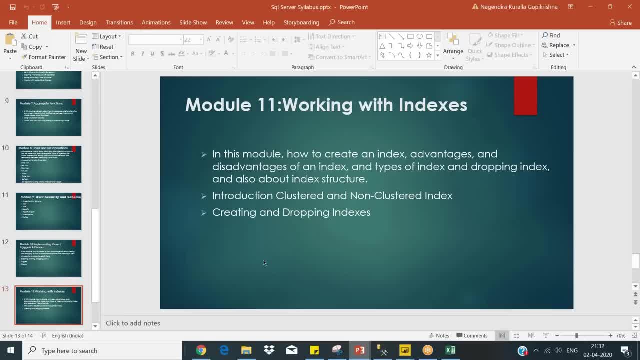 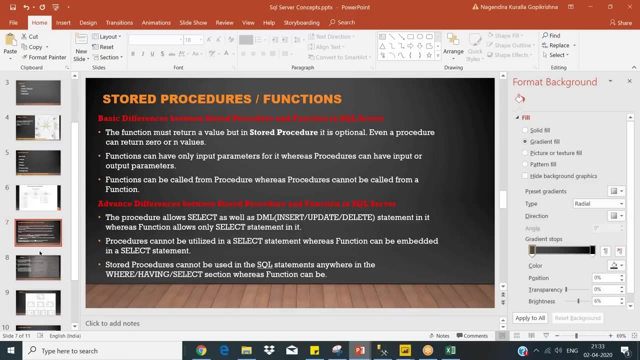 indexes. so any idea before starting index, what is the purpose of index? here it says how to create all those things. so what is index? what is the purpose of it? any idea? no idea, okay, fine, that's okay. i hope everyone is familiar with books while we are reading. 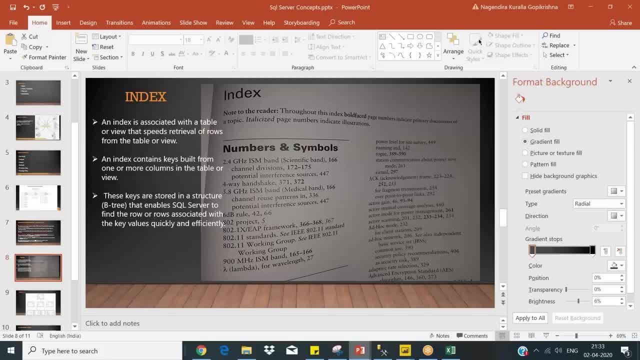 if you guys remember this one index in your books in college, it's the same concept like at the end of your book you will have some index like working group which is available in this particular page number. this if you see: 201, 232, 233, 234. if you want to study about active scanning then you need to. 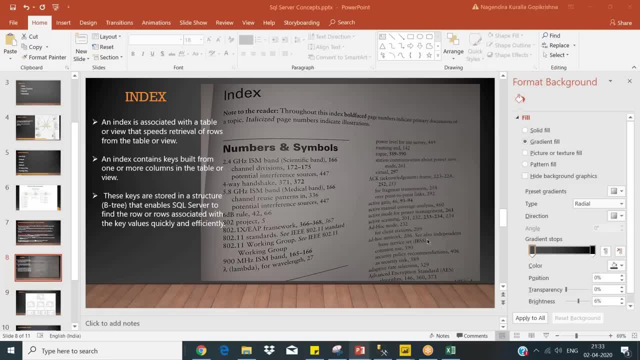 go to this particular page, then you can refer that one. okay, some topics alphabetically, it guys arranged like adhoc network 206, common use. i mean basic services, something like that. so it's like searching criteria where your records are stored. so this is the concept behind the index. the same logic applies in your database level as well. 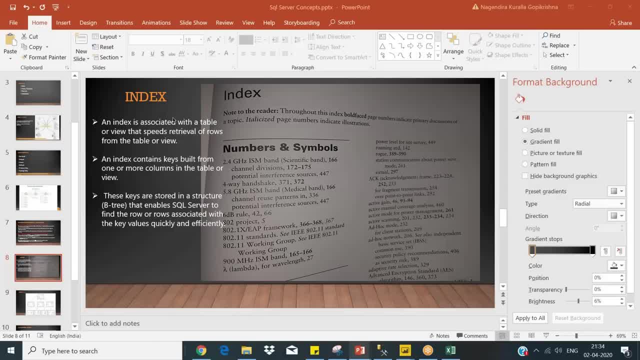 so here is the definition: an index is associated with the table or view. that speeds up retrieval of rows from a table or view. okay, it is basically you can create index for a table and rows which helps you to retrieval very fastly. okay, that is the purpose of your index. 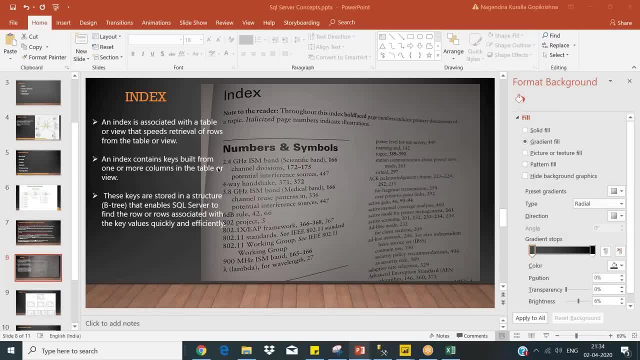 an index contains keys built from one or more columns in the table or view, it is same. i mean you can create index for more than one column. okay, that is what it mentioned how it is stored. it's stored in a b3 structure, so forget about this. it will make you complex to understand. 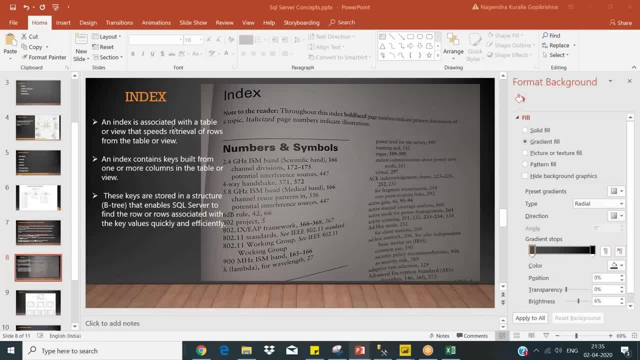 basically, index is used for query retrieval faster. so how it will be fast. say, for example, i'm storing, i want to store customer one to ten thousand are now. you see facebook users, all other users. you have millions of users. okay, so as soon as you log in, you are. 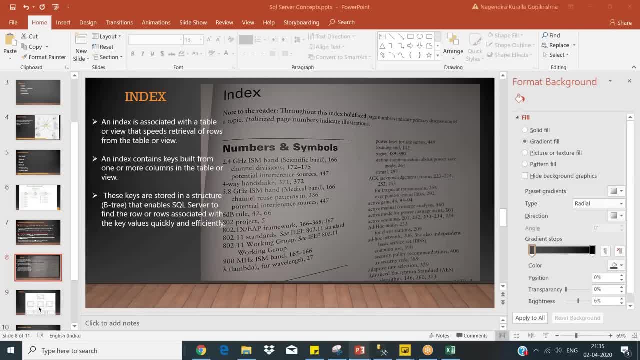 one in one million. so it has to get your information fastly from that one million records. okay, so how it gets it should be very quick. okay, so it has to navigate. as soon as sees your name or you see your password. it, when you hit that button, it should navigate directly to that particular place where it is stored. so 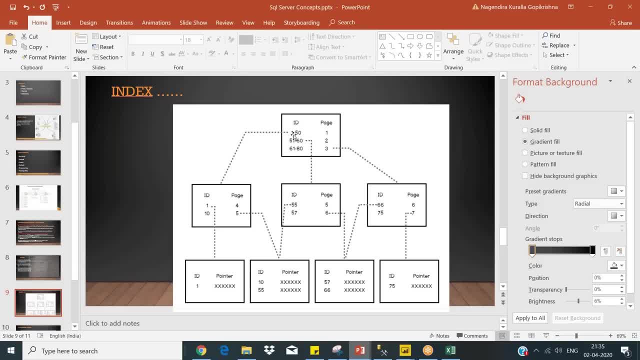 the logic behind this is like this: you assume you have 80 ids. okay, now out of that 1 million- this is like that. i mean now in in our example. here you have ids, 80, users, 1 to 80.. so 1 to 50. there will be a reference, it is stored in page 1, so here it will go 1 to 50. 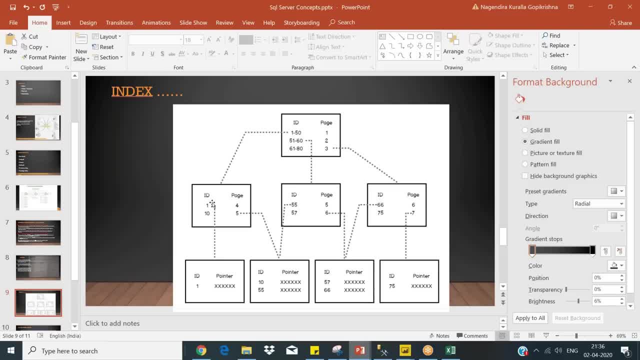 so here in this page 1 you see like 1 to 10. okay, in page 4 i mean you see the difference over here. i mean the 1 to 9 is in page 4 and from 10 onwards it's in page 5, so it will go to page 5. 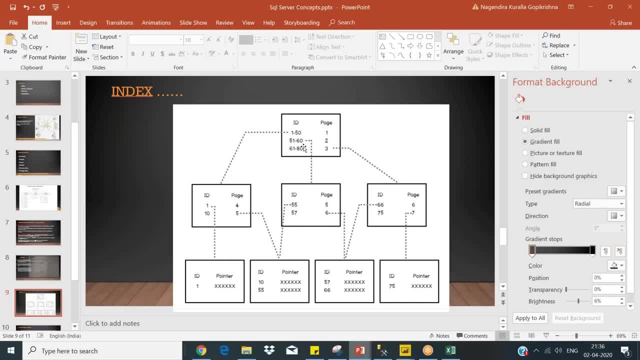 say for example: uh, id number um 56. okay, so it will come and search here: that is 56, 56 is in second page, second page is here. so 56 is uh from 55, so 55 is here. so it will navigate to this particular point easily, then fetches the results and gives to you. so this is what index does. 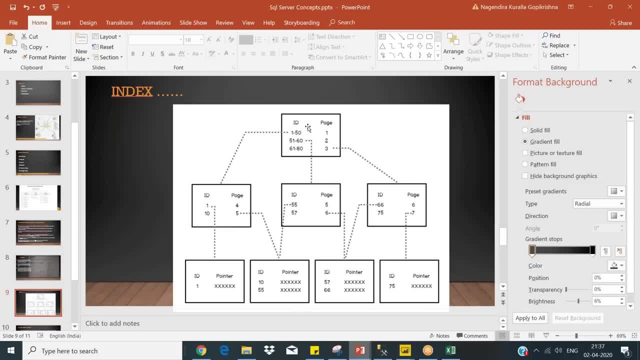 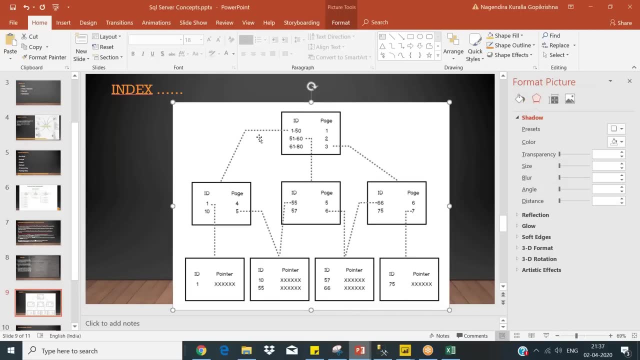 okay, so ids are stored at the bottom level. so even you create a primary key. okay, so that will create a clustered index where your data are stored at this level, at the bottom level over here. so it will create an index structure like this: then your data are stored in this. 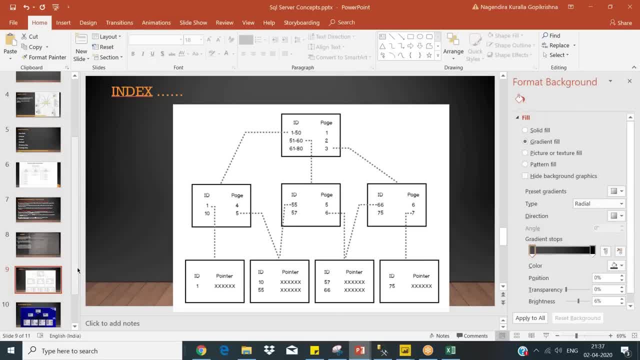 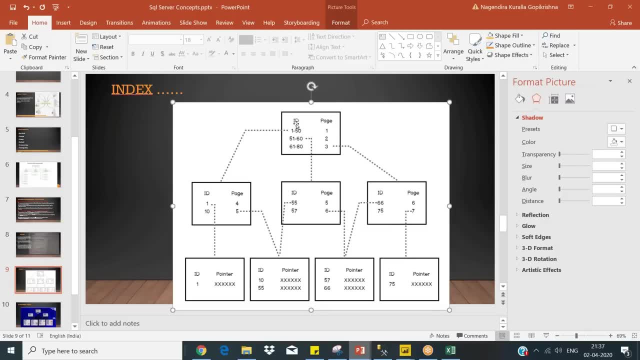 last leaf node. let me show it to you. so this is clear, guys. i think this is very simple. when you have your ids, ids are nothing but customer id, login id unique values, so those unique values will have a value like this: then those informations are stored here, okay. 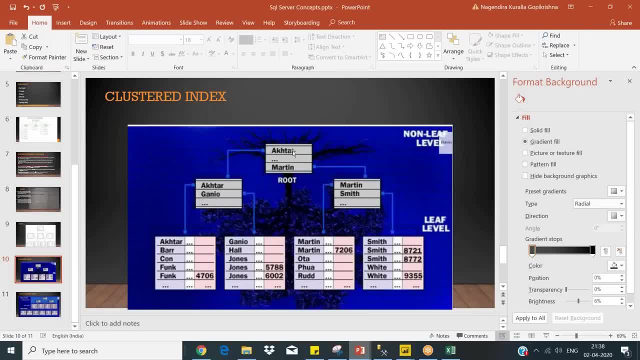 so cluster index, so you have something like id stored, so where from a to uh, say for example a to g, a to g is stored here, send a to g from heather. you have values over here. so this node you have from values from a to g. 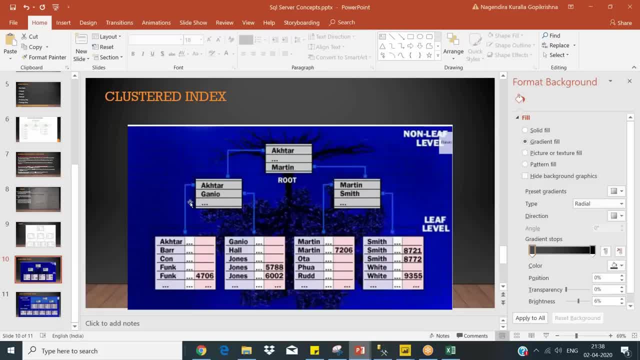 are not from a to g, a to before g. what is that? abcdef, g, h. abcdef till a to f. your values are stored here from g to. is that j? i mean g to j? the values are stored here from m to r. values are stored here from s to, is it? it is stored here, so you, when someone asks my name, naga, then it will. 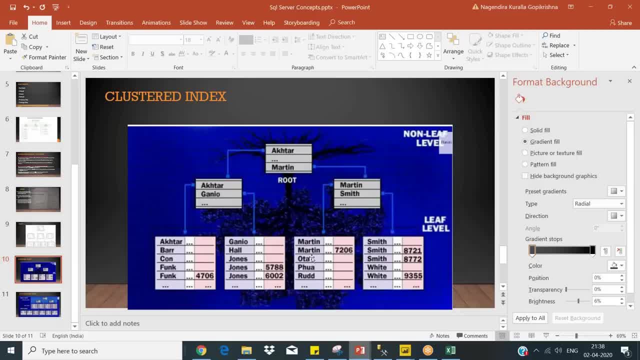 go and check this particular mn, so it will be stored here, some something. so it will navigate this path instead of going searching all the things. okay, so if the index is not there, what will happen? okay, it will go and check in each and every record. uh, it will, if i. my name is naga. 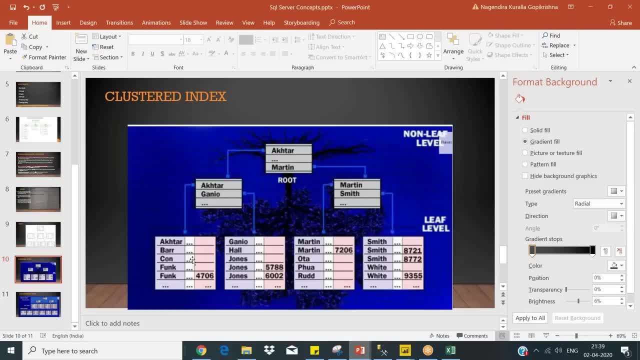 whatever data is stored, from the order it is stored. well, you ask, deepak, i mean a lot of times how it is fetching, how it is retrieving the data. so this is the answer: when you create an index, it will store in alphabetical order. whatever column you have created, the data are stored here. it will be. 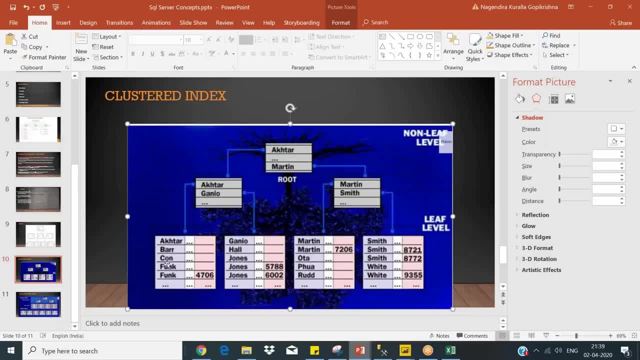 fetched from the page one. this is page one. page two, page three, page four. it is fetched from this order: okay, always okay. when you are not creating an index, it will be inserted random order based on the page availability. if these are concept behind the databases, i mean. 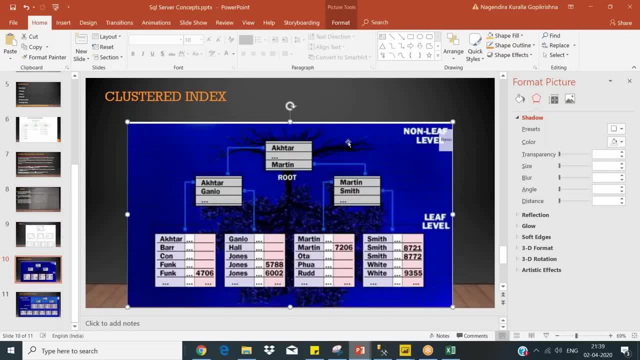 how it is internally stored. okay, so when you are not creating index, the data are stored random order. whatever there will be like storage concept. whether the space is available here, then insert it. whether some space is available, inserted. so if there is no index, naga can be stored here or here. 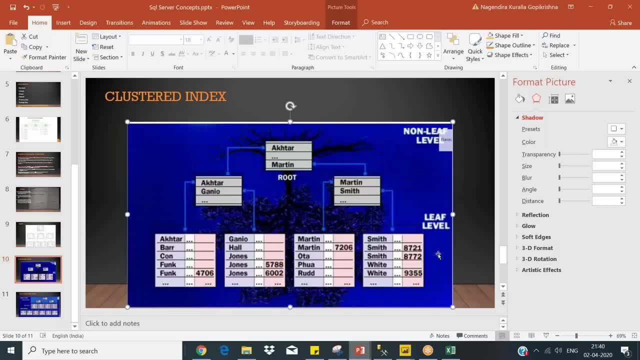 or any other places. it basically will be stored in random order. so if you are not creating an index based on the space availability, that system will decide. there is a huge algorithm behind that, okay, so again focusing on index. so when you create an index, the data are sorted based on the 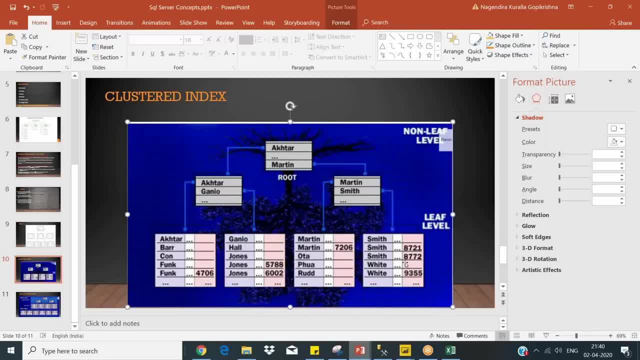 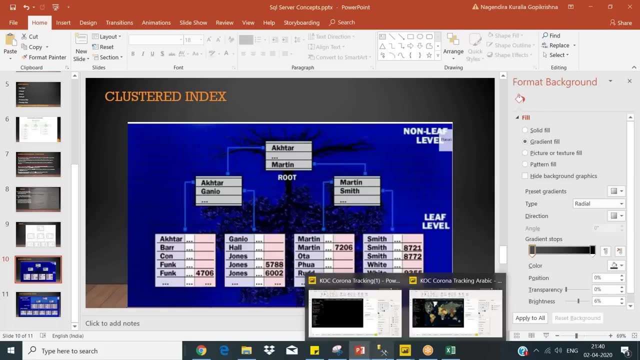 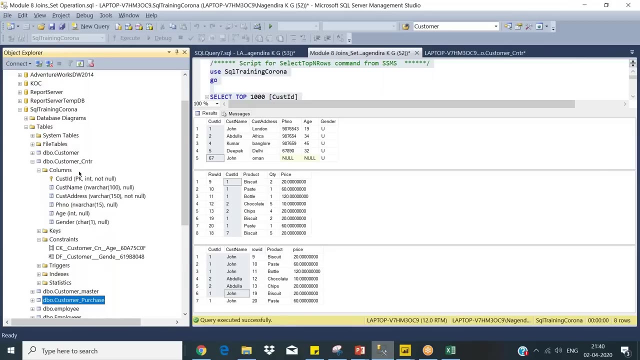 the column you have created index and it will be stored in the least level. this is your cluster index. okay, let us stop this one. uh, before going to non-clustered index, let us focus on cluster index. when you create an index and without an index, how it performs, okay. 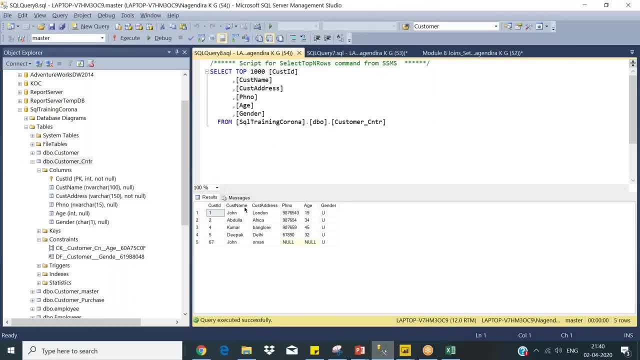 so we have our data over here. now when i select this table, i have index here. whether index is used now or not, let us see that one. so, using execution plan, as i said before, we can see. we can see that the index is used now or not. let us see that one. so, using execution plan, as i said before, we can see. 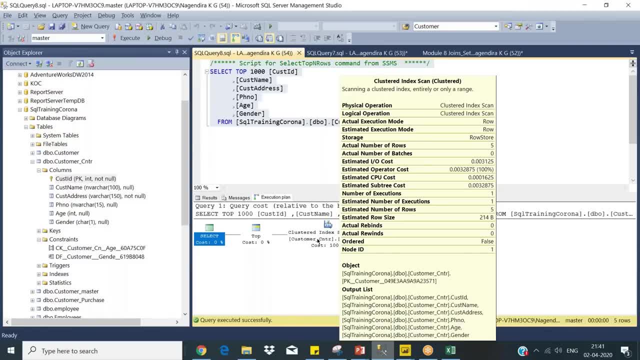 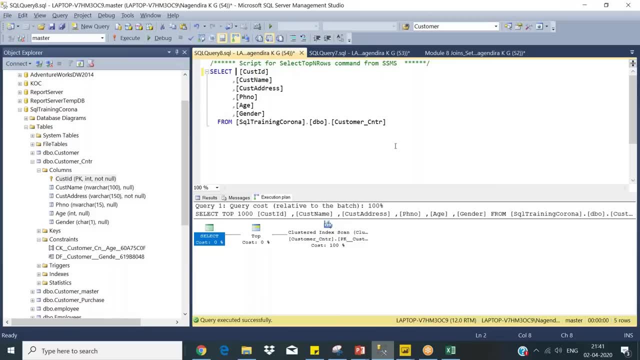 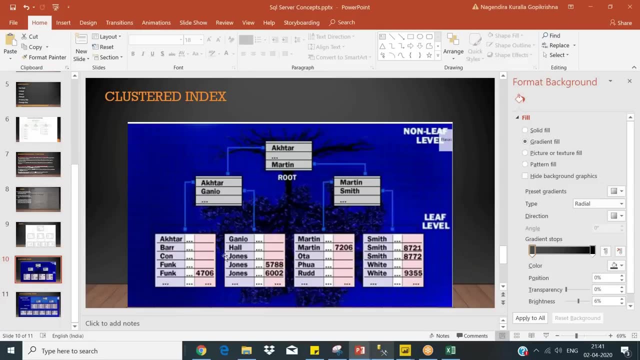 so clustered index scan: okay, when you are not using your index column in your var condition. clustered index scan: okay. when you are not using your index column in your var condition, it will always use a scan. scan is nothing but the entire table from one, two, three, four, all the. 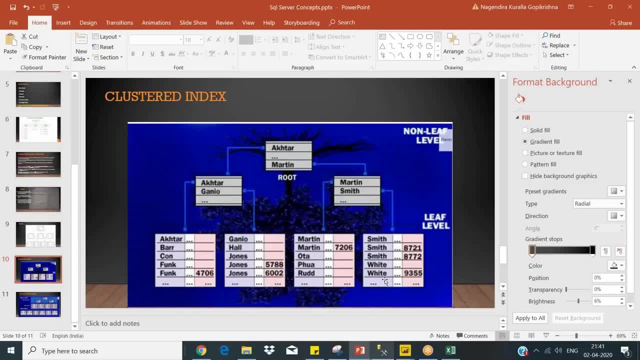 things. it will scan and pick up the results. scan is nothing but row by row, each row, it will go and fetch the results, but whereas when you are not using Changing index column for this textcause, necessarily there is an exception to your voting table, there is a problem at the fundamental table and where, if this row follow by this column, each row, youitate to fetch the results but leaves the table with altering case. 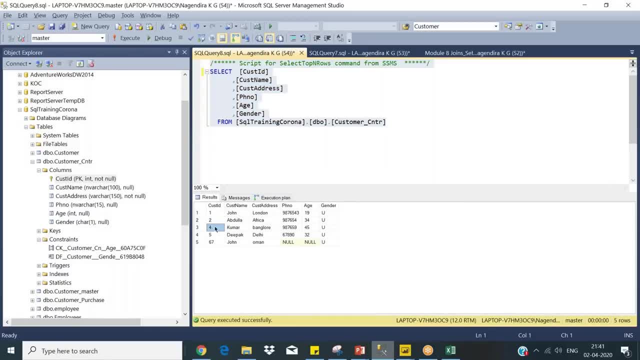 from this example you can see that you have a date knock. your index columnes are killed. install in index column is in practice by the index column었 atими, not extended index column, and what is wrong with them. but whereas when i say customer id, okay, equal to four. 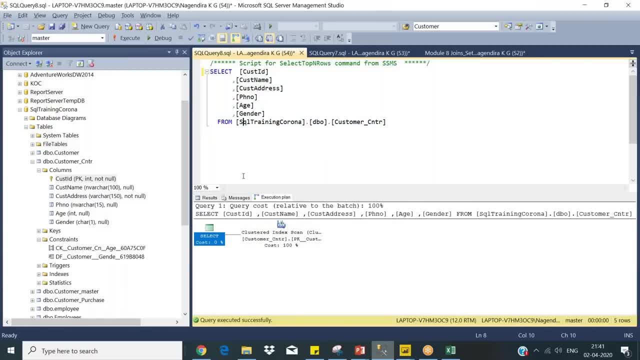 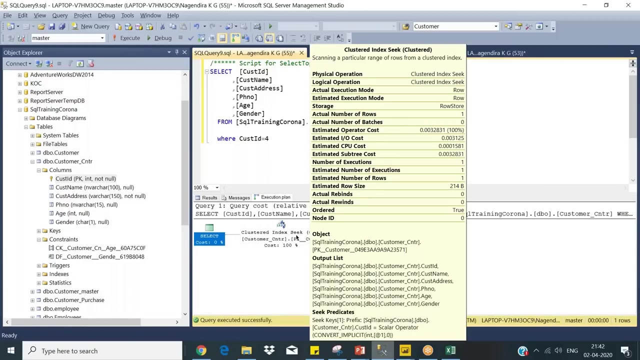 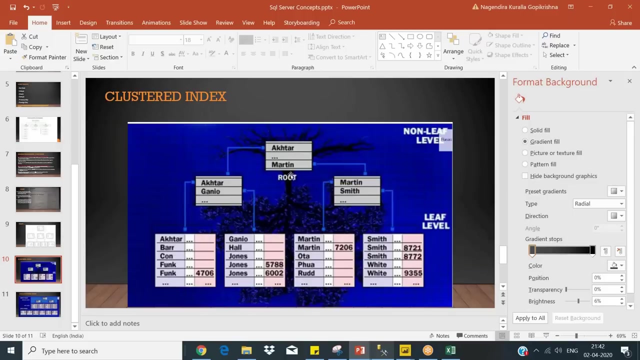 you see the execution plan here, guys, index scan and create a new page. so when i filter using customer id equal to 4, include execution plan. what it does is clustered index seek. seek is nothing, but you are this flow. i have filtered four. so here it is stored with name. so four means naga. assume like naga, so it will go in this path. 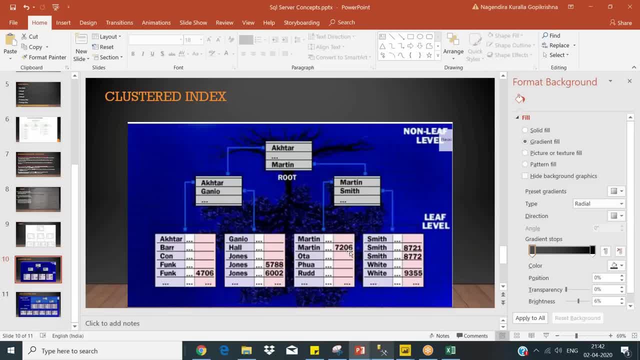 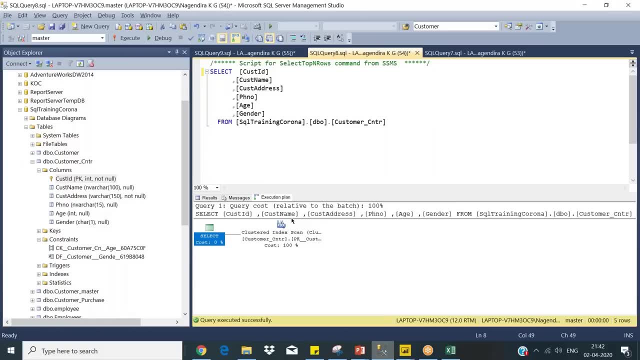 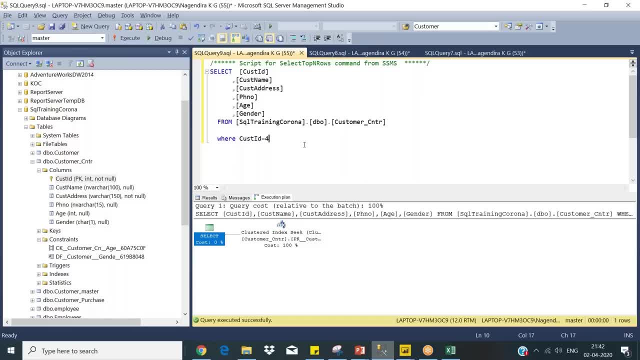 index in the back condition. as i said before, indexing is useful before. indexing is useful before. indexing is useful only when you are retrieving the value, only when you are retrieving the value, only when you are retrieving the value. it is not used for any other purpose. it is not used for any other purpose. 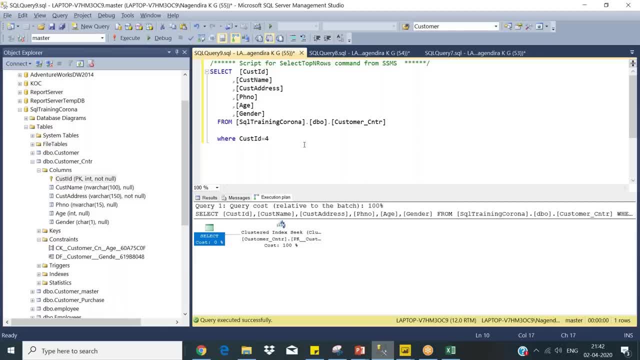 it is not used for any other purpose. basically, when you are coding the 10 000, basically when you are coding the 10 000, basically when you are coding the 10 000 records or 1 million records records or 1 million records records or 1 million records, the response time should be faster, okay. 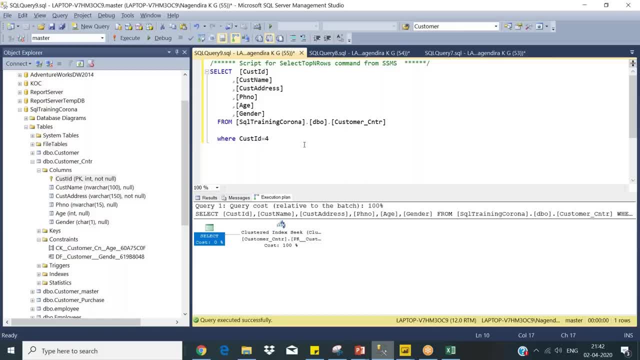 the response time should be faster. okay, the response time should be faster, okay, so when you create an index, so when you create an index, so when you create an index, you need to use it in the bar condition, you need to use it in the bar condition, you need to use it in the bar condition. now let me see if i put instead of: 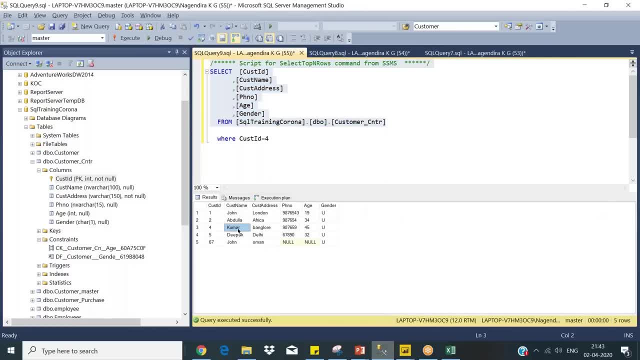 now. let me see if i put instead of now. let me see if i put: instead of four when i see uh instead of four when i see uh instead of four when i see uh instead of index column. i'm not putting the index, index column. i'm not putting the index. 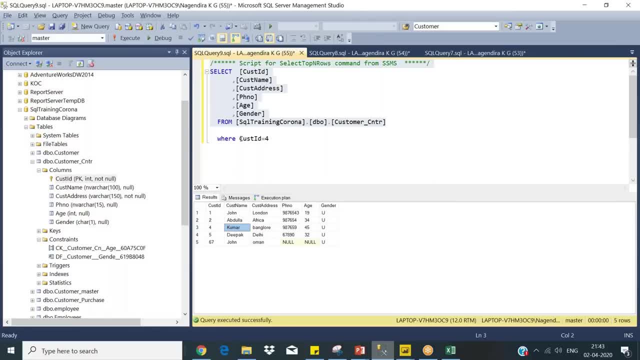 index column. i'm not putting the index column in a bar condition column in a bar condition column in a bar condition. i'm putting non-index column kumar when i i'm putting non-index column kumar when i i'm putting non-index column kumar when i search with kumar. 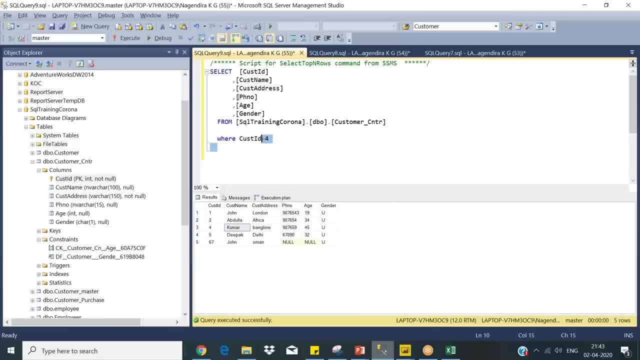 search with kumar. search with kumar: what it shows. even i'm not familiar with this thing, let us see, even i'm not familiar with this thing. let us see, even i'm not familiar with this thing. let us see, definitely it will not do index seek. 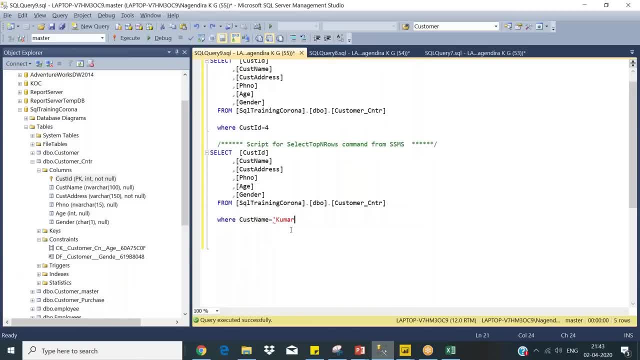 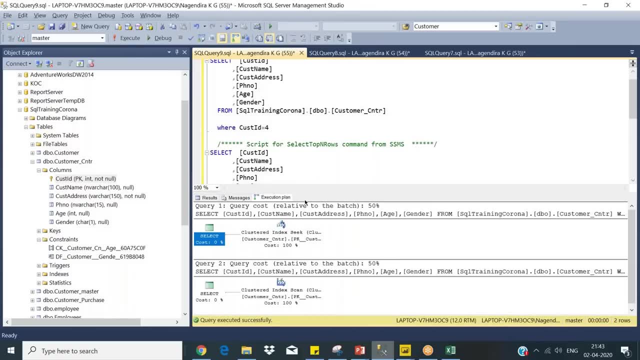 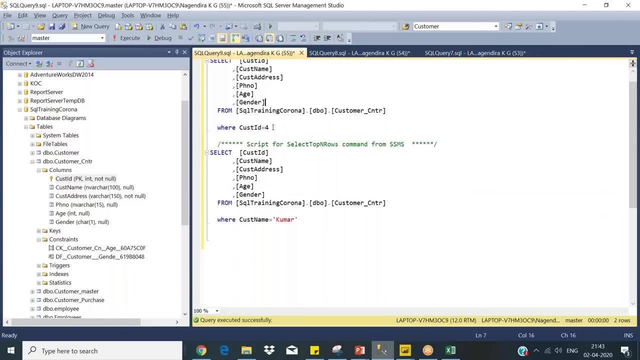 definitely it will not do index seek. definitely it will not do index seek. let us see. so include execution plan. okay, see, okay, see, okay, see. now the first query, now the first query. now the first query is using a primary key column, the primary is using a primary key column, the primary. 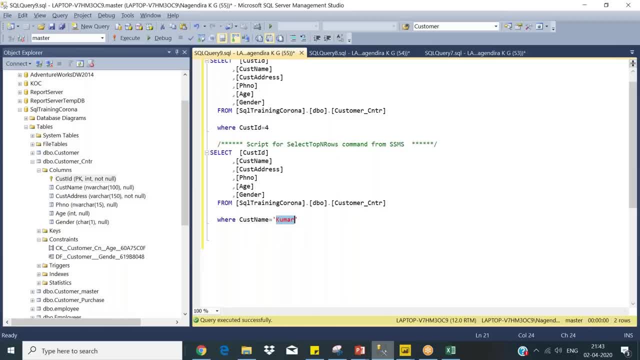 is using a primary key column: the primary column in the var condition. the column in the var condition. the column in the var condition. the second query. second query. second query: customer name. customer name in the var customer name. customer name in the var customer name. customer name in the var condition. 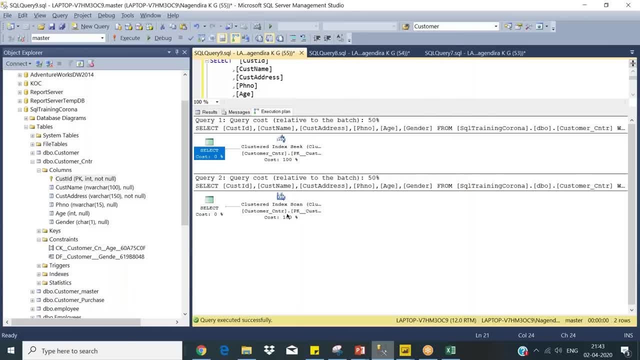 condition: condition: first query. it is seeking. that is finding first query it is seeking. that is finding first query. it is seeking. that is finding the path, the path, the path. the second query: it is scanned, so there is the second query. it is scanned, so there is the second query. it is scanned, so there is no use at all. 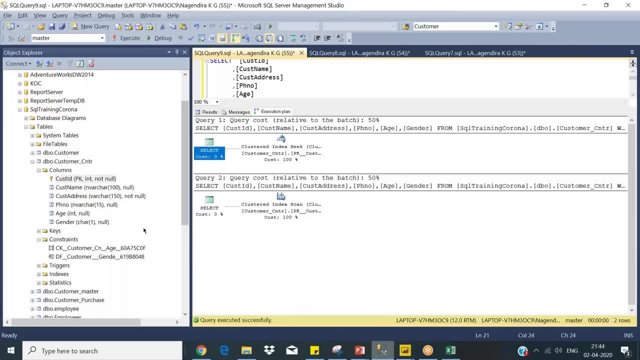 no use at all. no use at all. okay, i mean even you create an index. it is okay. i mean even you create an index. it is okay. i mean even you create an index. it is not that you create an index and use, not that you create an index and use. 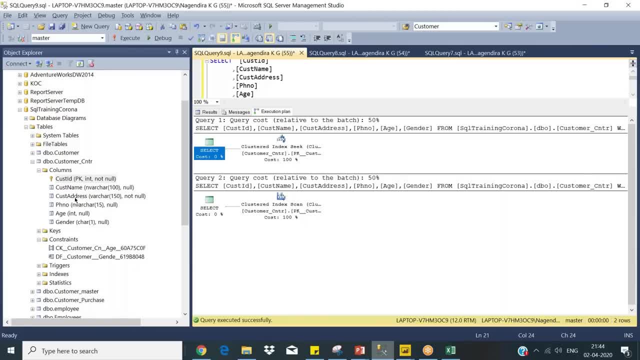 not that you create an index and use other columns in a var condition, that other columns in a var condition, that other columns in a var condition, that will work out, will work out. will work out whatever column you create in an index, whatever column you create in an index. 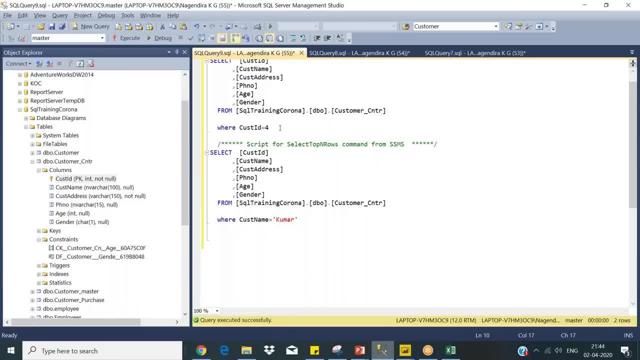 whatever column you create in an index, that particular column you need to use, that particular column you need to use that particular column you need to use explicitly okay, then only it will work explicitly okay, then only it will work explicitly okay, then only it will work. otherwise it is normal even. 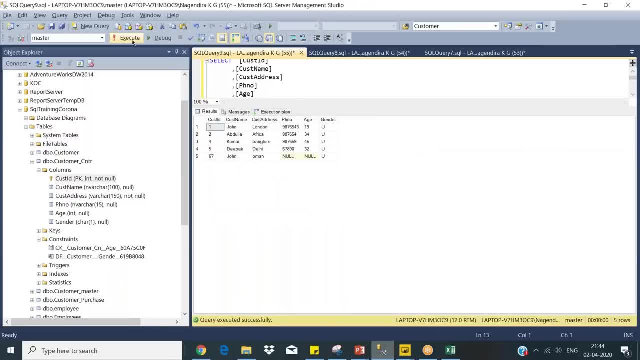 otherwise it is normal. even otherwise it is normal. even some other column, even if you select some other column, even if you select some other column, even if you select without this one, it is same without this one, it is same without this one. it is same. first, what it will do now, it will fetch. 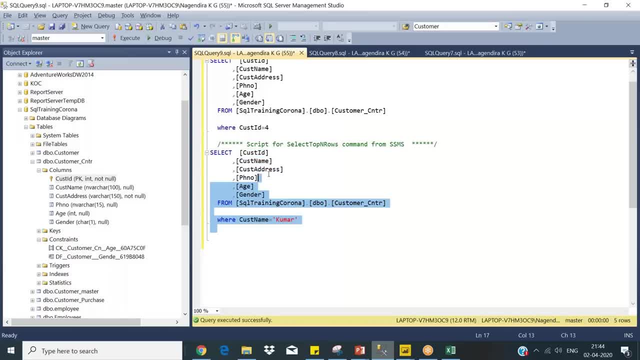 first what it will do now. it will fetch first what it will do now. it will fetch this results first, this results first. this results first. from this. it will pick up, kumar, what this query will do. it will not fetch what this query will do. it will not fetch. 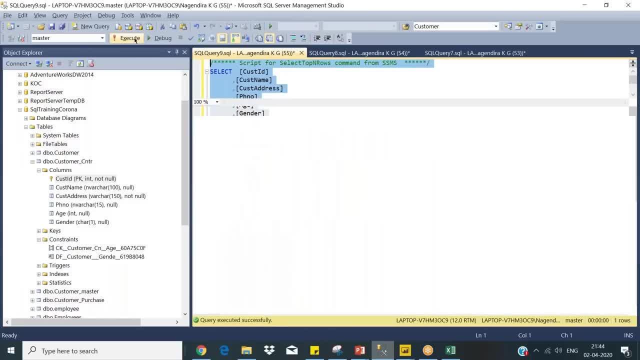 what this query will do. it will not fetch the results. i mean the the results, i mean the the results, i mean the all the records first, then it will all the records first, then it will all the records first, then it will filter, instead it will go and check. 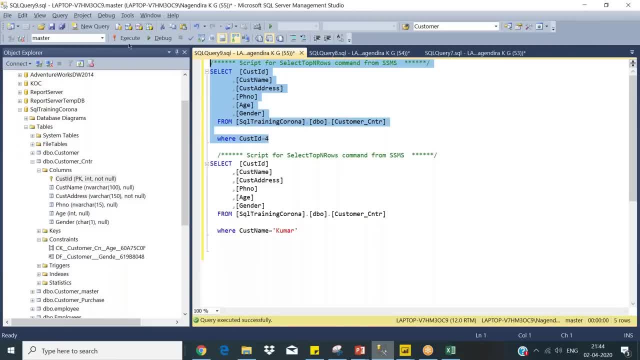 filter instead, it will go and check filter. instead it will go and check where is this four exists. it will pick where is this four exists. it will pick where is this four exists. it will pick up only the record. fourth record up only the record. fourth record. up only the record. fourth record as a whole. it will be resulting only one. 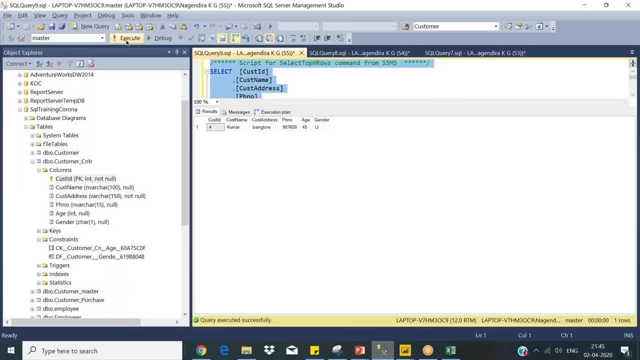 as a whole. it will be resulting only one as a whole. it will be resulting only one: uh one. one input output operation only uh one. one input output operation only uh one. one input output operation only. this is the thing, guys. this is the thing, guys. this is the thing, guys. so this is about your. 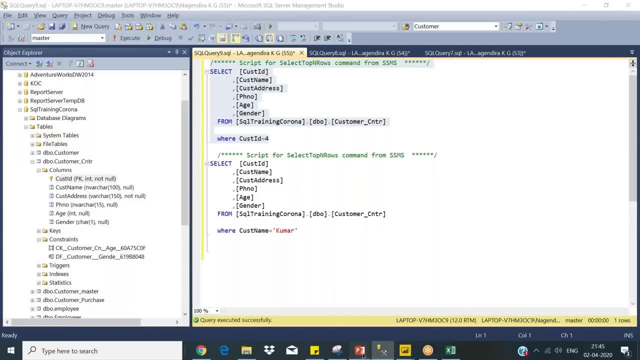 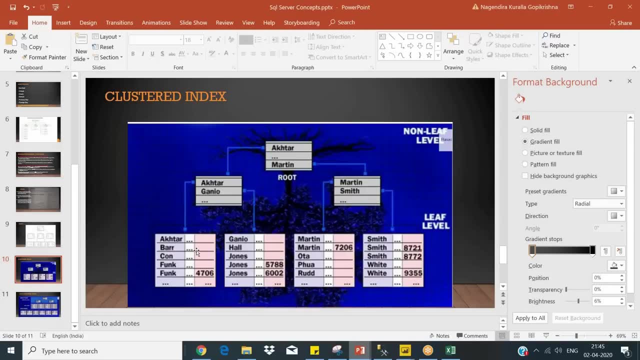 so this is about your. so this is about your cluster index. why? because your data is stored in the same order as i. your data is stored in the same order as i. your data is stored in the same order as i said, the cluster index. when you have. 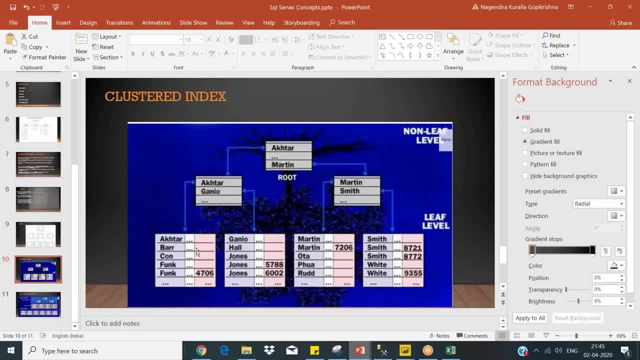 said the cluster index, when you have said the cluster index, when you have in a single table, i mean a table single in a single table, i mean a table single in a single table. i mean a table single table can have only one table can have only one. 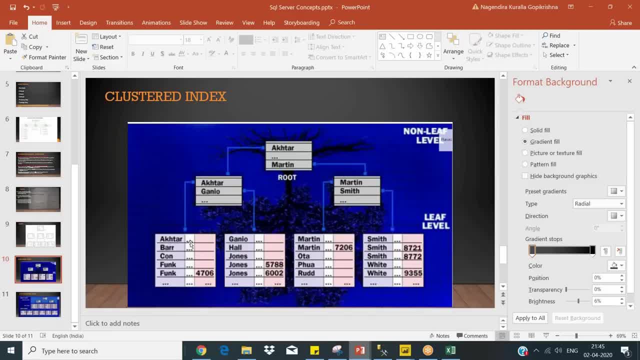 table can have only one cluster index, because your data all the cluster index, because your data all the cluster index, because your data all the columns, columns, columns. okay, it is not only ids your name, okay, it is not only ids your name, okay, it is not only ids- your name, address, everything will be stored along. 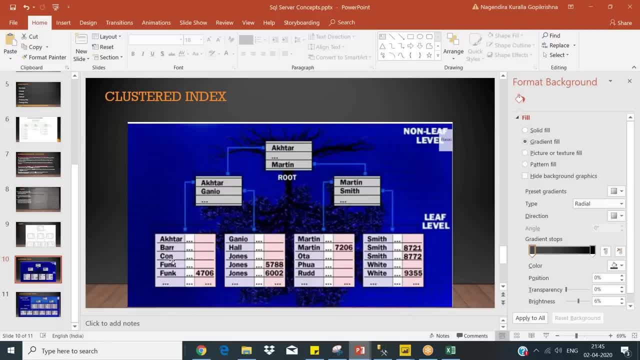 address. everything will be stored along address. everything will be stored along with your, with your, with your clustered index, in this clustered index, in this clustered index, in this last leaf node. this is your cluster, last leaf node, this is your cluster, last leaf node. this is your cluster index. 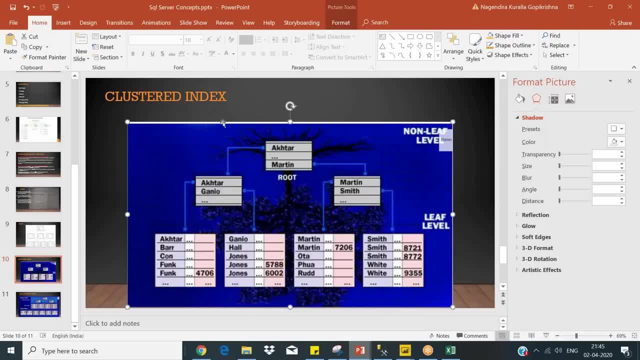 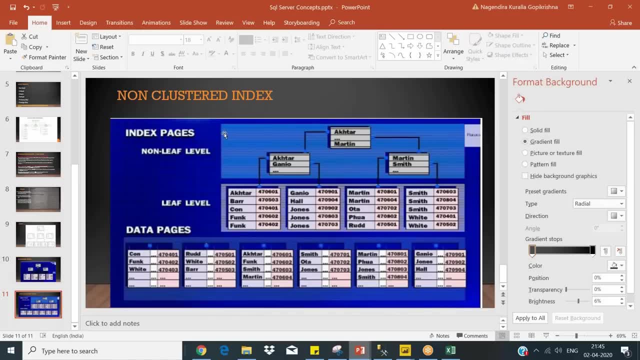 index index. and i said like not, there are multiple. and i said like not, there are multiple. and i said like not, there are multiple non-clustered index: you can create non-clustered index. you can create non-clustered index. you can create. what is that? so here, you have like. 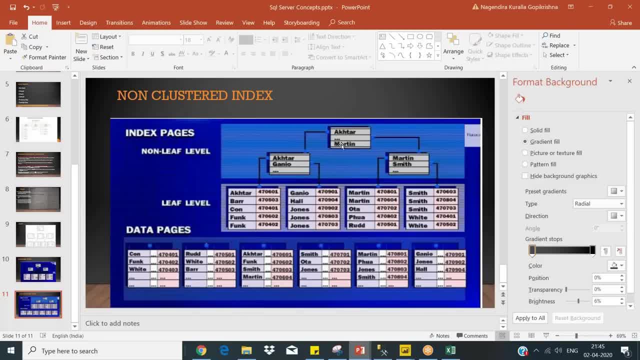 so here you have like, so here you have like non-cluster index. it is same example, non-cluster index. it is same example, non-cluster index. it is same example. so say for example. so say for example. so say for example: naga after mn, it should be stored here. 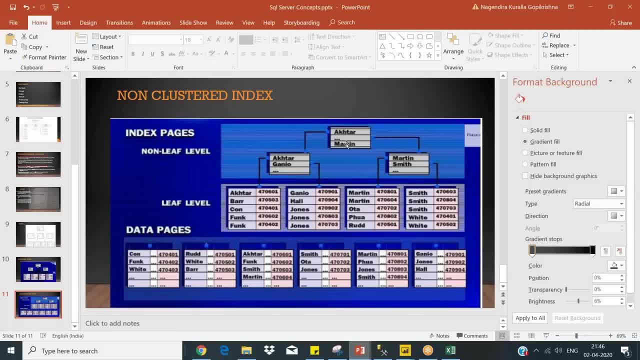 naga after mn. it should be stored here. naga after mn, it should be stored here. maybe we say ota only, maybe we say ota only, maybe we say ota only. so ota. so ota means after m it comes, so ota means after m it comes. 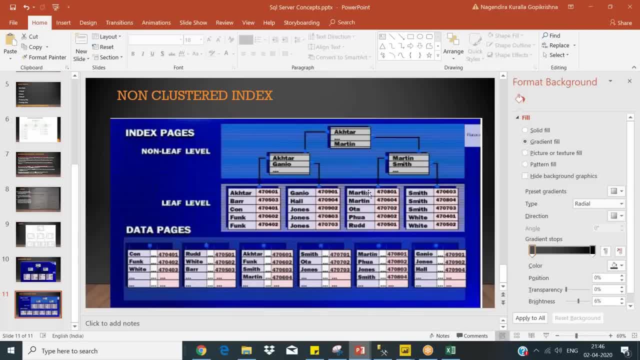 so ota means after m, it comes after m, so it will go here after m, so it will go here after m, so it will go here. and before yes, so it will go here. so, and before yes, so it will go here. so, and before yes, so it will go here. so ota. 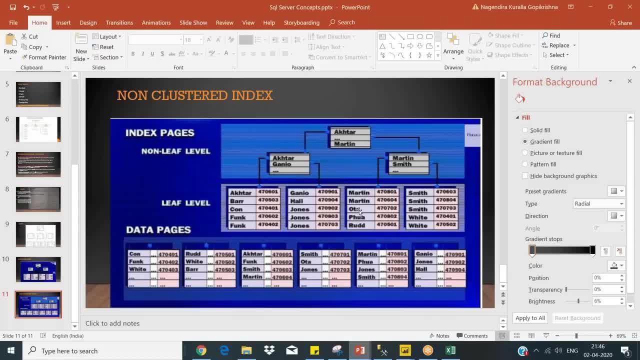 ota, ota and what happens? this is the leaf node and what happens? this is the leaf node and what happens? this is the leaf node here, here, here, the data for ota will not be stored as we. the data for ota will not be stored as we. 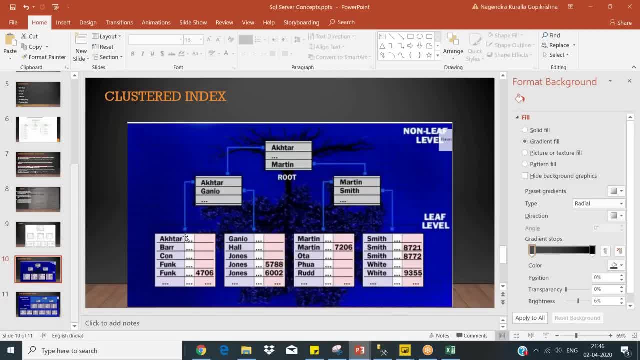 the data for ota will not be stored, as we see in this example. see in this example. see in this example the entire row for other. that is the entire row for other. that is the entire row for other. that is address, phone number. everything is stored. address, phone number. everything is stored. 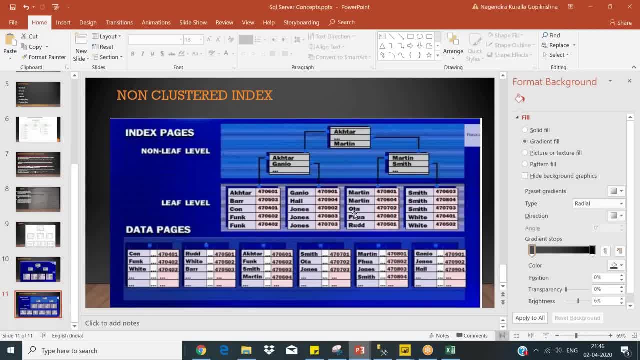 address, phone number. everything is stored here so easily. we can pick up here so easily. we can pick up here so easily. we can pick up instead, what happens for him, instead, what happens for him, instead what happens for him. it will have one reference for this row. it will have one reference for this row. 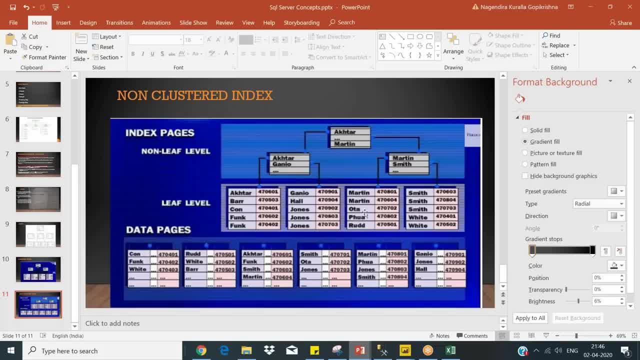 it will have one reference for this row: id: id id. where the other informations are stored, where the other informations are stored, where the other informations are stored: for rota, it is 470702. for rota, it is 470702. for rota, it is 470702. so here, 470702 only. the reference is. 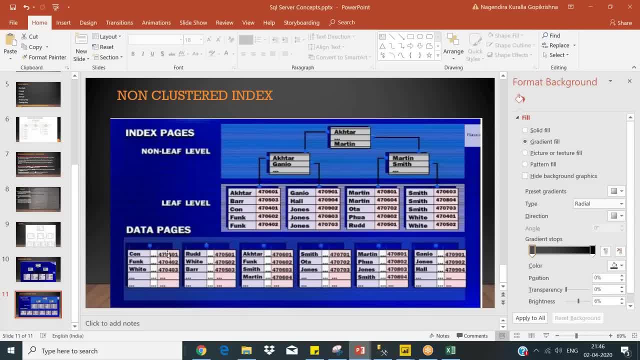 so here 470702, only the reference is, so here 470702, only the reference is stored, stored. stored, so based on the cluster index. it can so based on the cluster index. it can so, based on the cluster index, it can say a table can have, say a table can have. 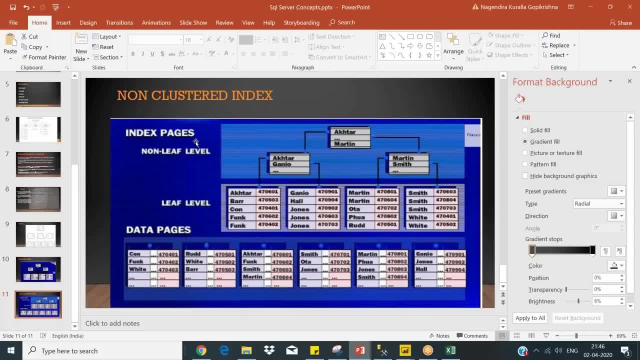 say, a table can have only a cluster index. a table can have only a cluster index. a table can have only a cluster index. a table can have only the non-cluster index, only the non-cluster index, only the non-cluster index if it is a non-clustered index. 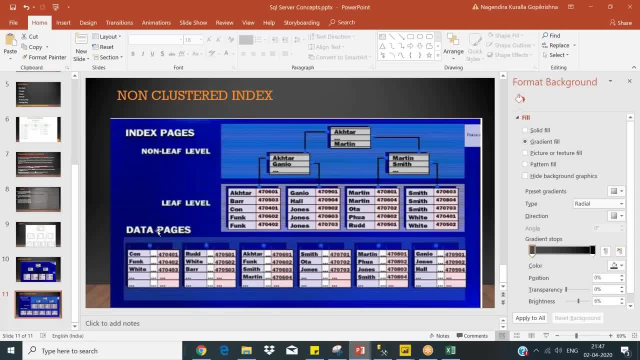 if it is a non-clustered index. if it is a non-clustered index, data are stored in random order. okay, i, data are stored in random order. okay, i data are stored in random order, okay, i mean. i mean, i mean, i assume there is no index at all in a. 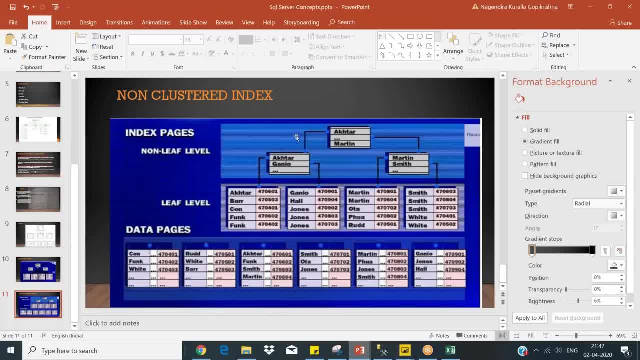 assume there is no index at all in a. assume there is no index at all in a table. you are creating a table. you are creating a table, you are creating a non-clustered index, then while you are non-clustered index, then while you are non-clustered index, then while you are inserting, data are stored in a random. 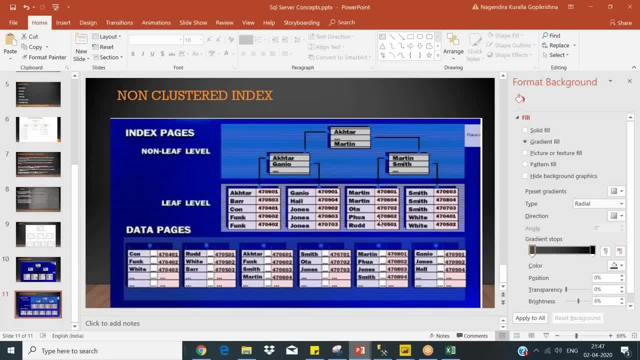 inserting data are stored in a random inserting data are stored in a random order: only here. order only here. order only here: in this data pages, then the in this data pages, then the in this data pages, then the non-clustered column. it will have that non-clustered column. it will have that. 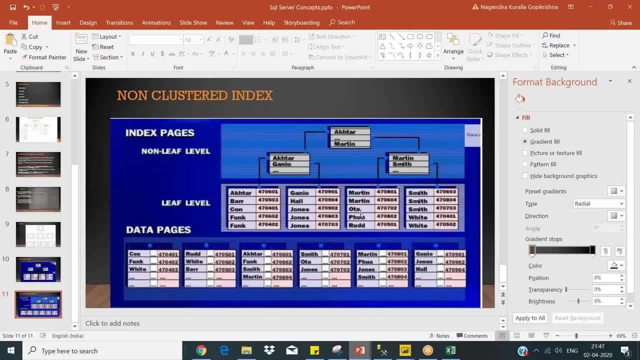 non-clustered column. it will have that reference, reference, reference where that reference is so at least when. where that reference is, so at least when. where that reference is, so at least when you query with this, you query with this, you query with this, it will go and fetch the water and the 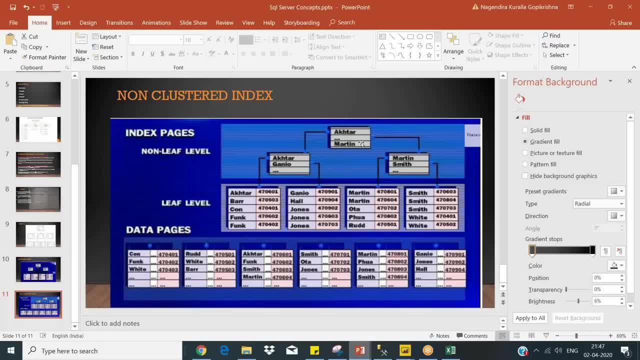 it will go and fetch the water and the. it will go and fetch the water and the reference number. it will pick it up and reference number. it will pick it up and reference number. it will pick it up and show it to you, show it to you. show it to you. so somewhat better than your previous. 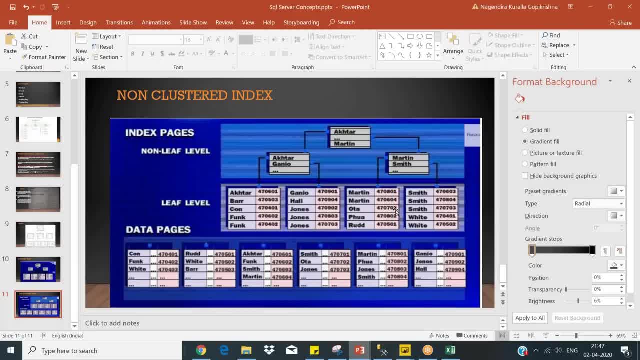 so somewhat better than your previous. so somewhat better than your previous, because it is stored for a column, because it is stored for a column, because it is stored for a column for ota, it is only 470702. for ota, it is only 470702. 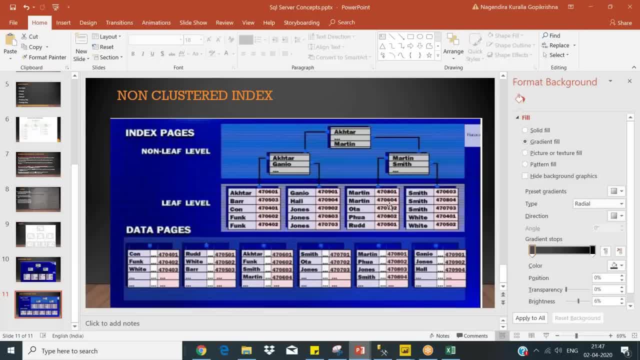 for ota it is only 470702. okay, you can have another non-cluster. okay, you can have another non-cluster. okay, you can have another non-cluster. index, index, index. so that particular reference also will, so that particular reference also will, so that particular reference also will point to this row. 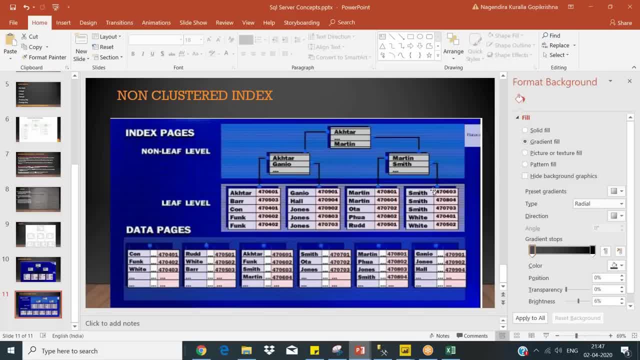 point to this row. point to this row. say, for example, you are creating a for a say, for example, you are creating a for a say, for example, you are creating a for a phone number, phone number, phone number. so this column in this water you will. so this column in this water, you will. 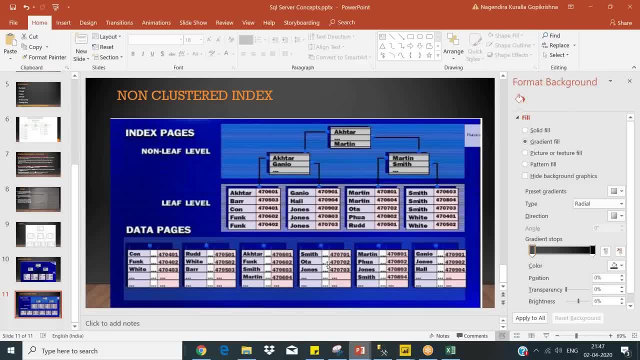 so this column in this water. you will have a phone number. phone number will have a phone number. phone number will have a phone number. phone number will have 470702, have 470702, have 470702. that will have a same reference so this. that will have a same reference so this. 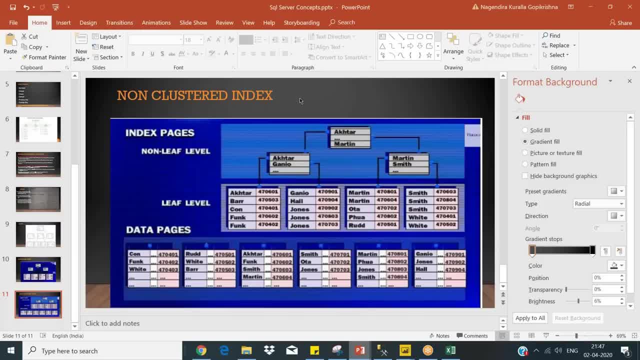 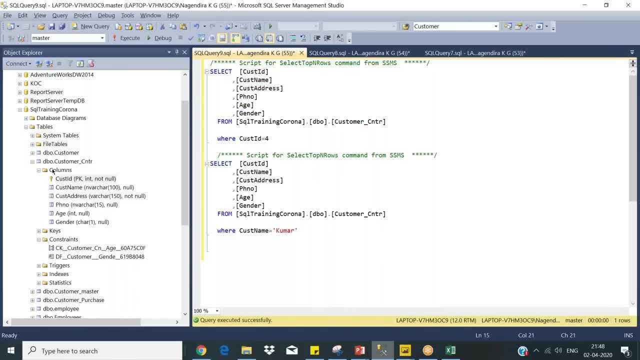 that will have a same reference. so this is what your non-cluster index is, what your non-cluster index is, what your non-cluster index. okay, let's see. okay, let's see. okay, let's see how it behaves. let's create one non-cluster index for a. let's create one non-cluster index for a. 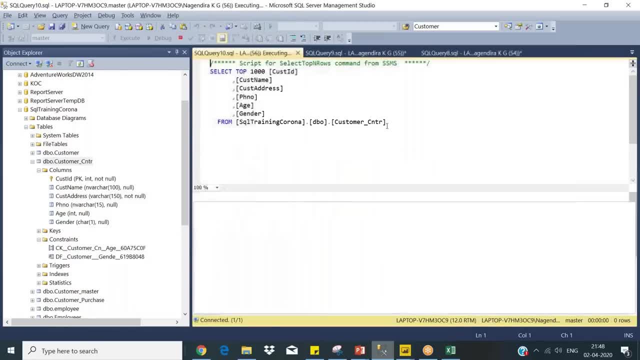 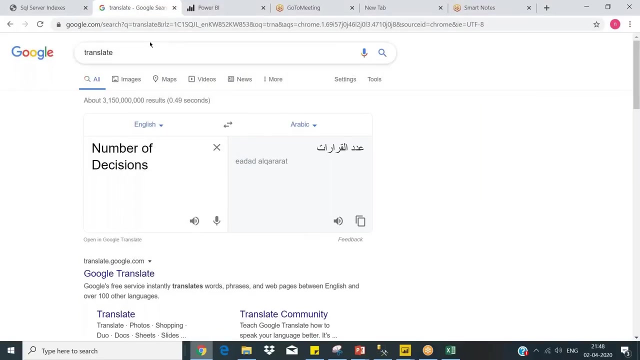 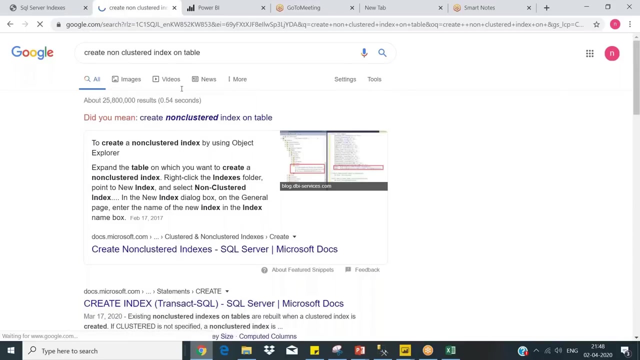 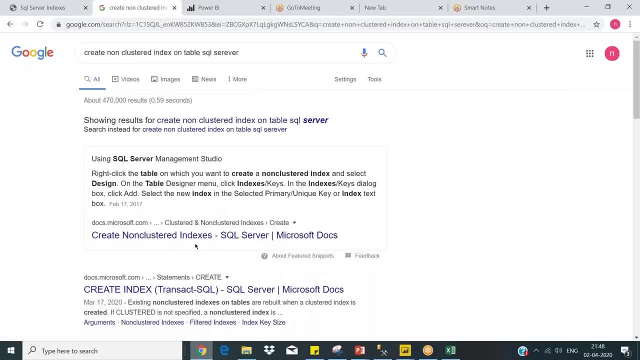 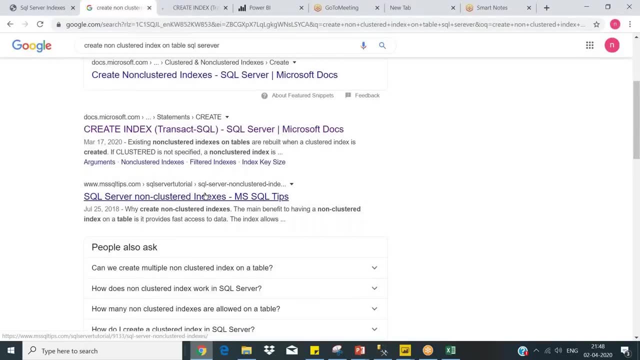 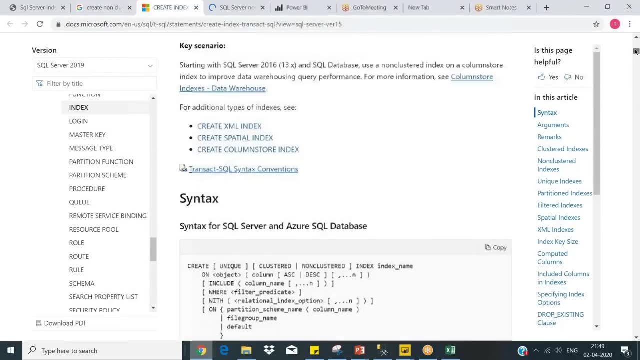 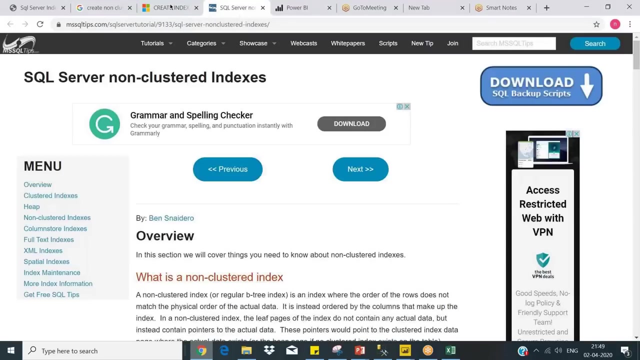 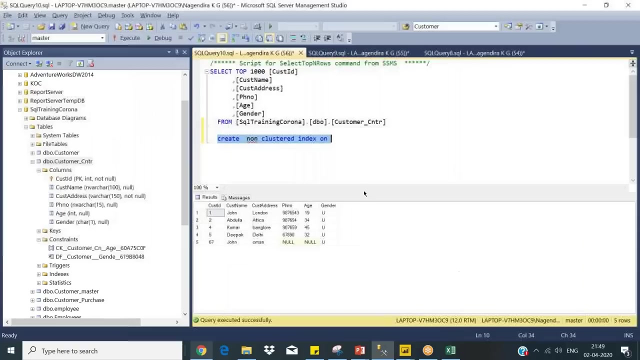 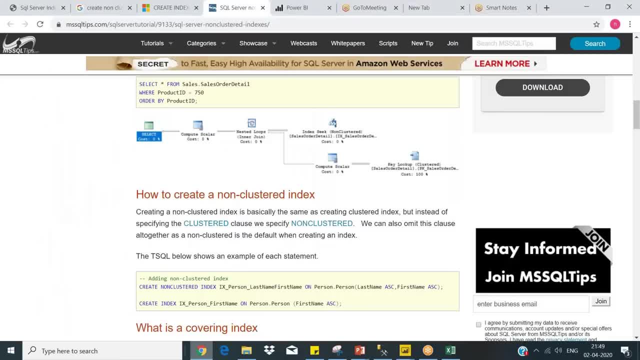 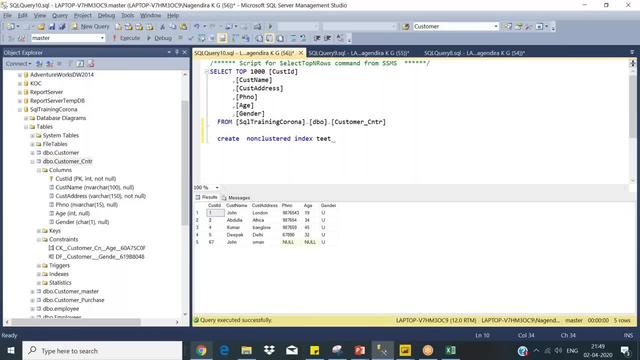 okay, create without space. okay, create without space. see, these syntaxes are not very. see, these syntaxes are not very. see, these syntaxes are not very pathetic, pathetic, pathetic: index, index, index. i'll put some index name, i'll put some index name, i'll put some index name. okay, test. 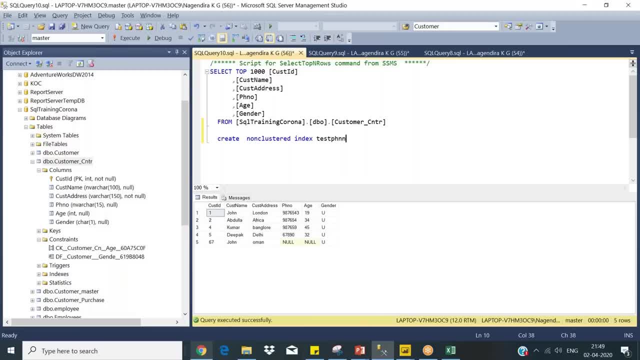 okay, test. okay, test phone number. phone number on phone number. on phone number. on the table name: the table name, the table name for the column: okay. the phone number for the column: okay. the phone number for the column: okay. the phone number okay. the phone number: okay. that's all i think. 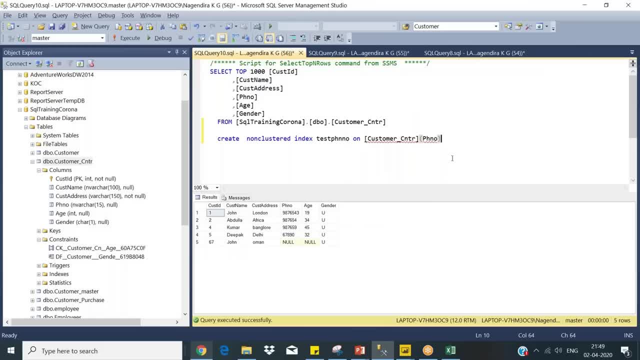 that's all, i think. that's all i think now what order it should be. we are in some other database, that's why we are in some other database. that's why we are in some other database, that's why throwing other, throwing other, throwing other. okay, now you see. 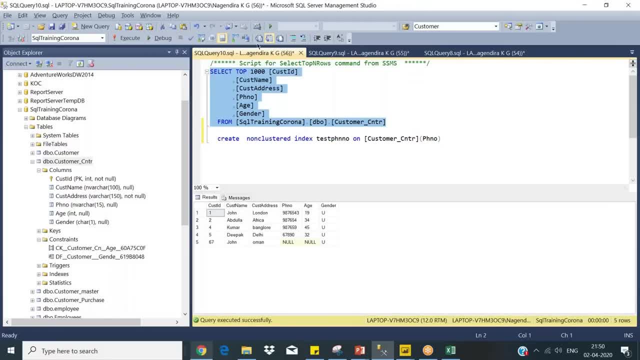 okay, now you see. okay, now you see here. see, you cannot see all these things here. see, you cannot see all these things here. see, you cannot see all these things. how it is stored, all of the purpose. how it is stored, all of the purpose. how it is stored, all of the purpose, okay. 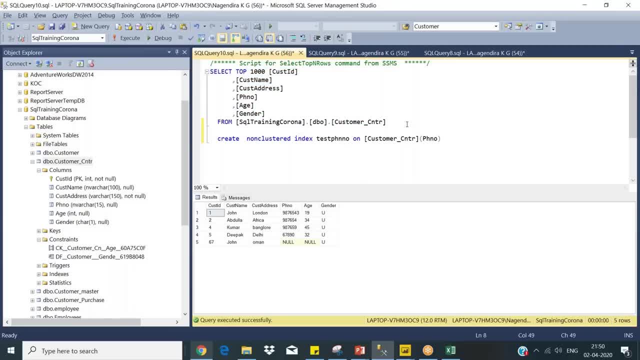 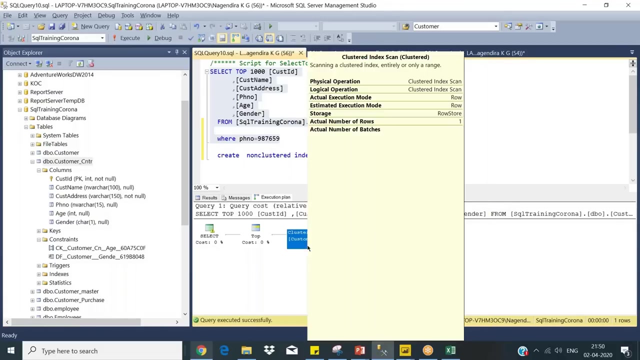 okay, okay, uh, okay, uh, okay, uh, okay, now, now, now, i'm searching using, i'm searching using. i'm searching using a non-clustered index column, let us have. it is doing a clustered index scan. it is doing a clustered index scan. it is doing a clustered index scan. something new: 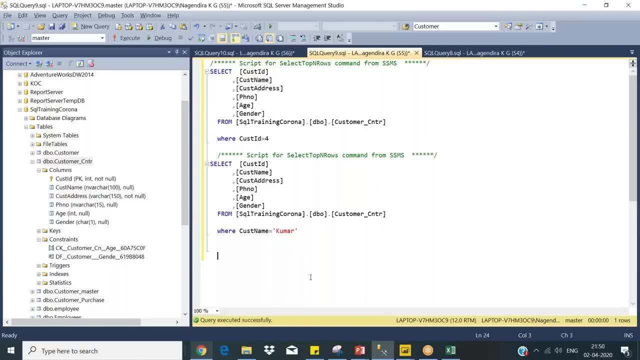 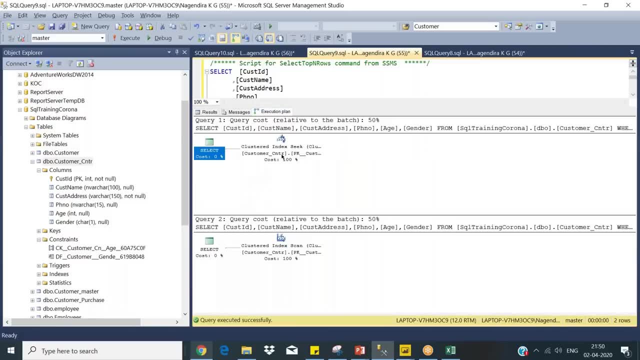 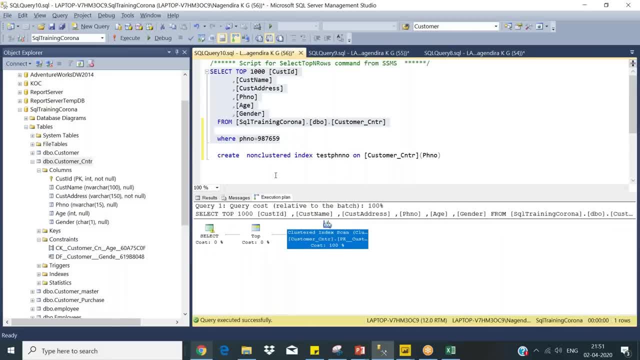 clustered index can okay. clustered index can okay. clustered index can. clustered index can. okay. clustered index can. clustered index can okay. clustered index can. whereas here, whereas here, whereas here. clustered index can again. clustered index can again. clustered index can again. so, so, so, if you use that one, i mean uh. 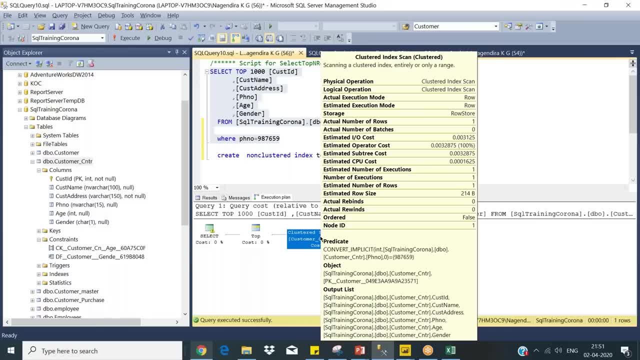 if you use that one, i mean uh, if you use that one, i mean uh, non-clustered index column. non-clustered index column, non-clustered index column. it will, it will, it will give you the cluster index, can only, give you the cluster index, can only. 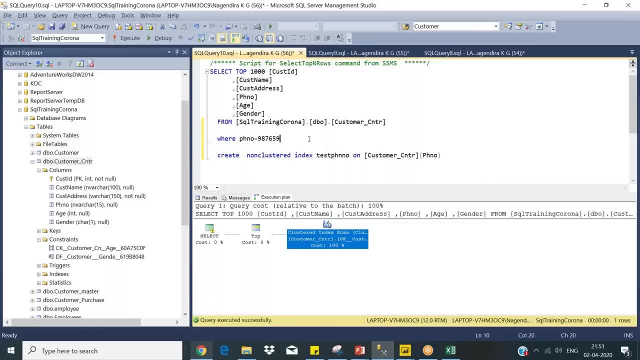 give you the cluster index can only okay. so that is the thing, guys, so, so that is the thing guys, so, so that is the thing, guys. so the main purpose, you got it right. the the main purpose, you got it right. the the main purpose, you got it right, the main purpose. 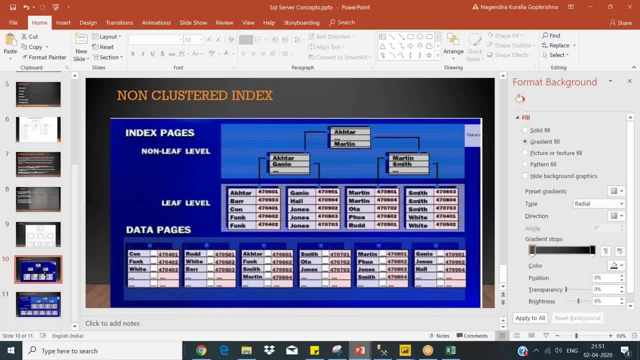 main purpose, main purpose behind this clustered index and behind this clustered index and behind this clustered index and non-clustered index is that non-clustered index, is that non-clustered index, is that cluster index can be a only one per cluster index can be a only one per. 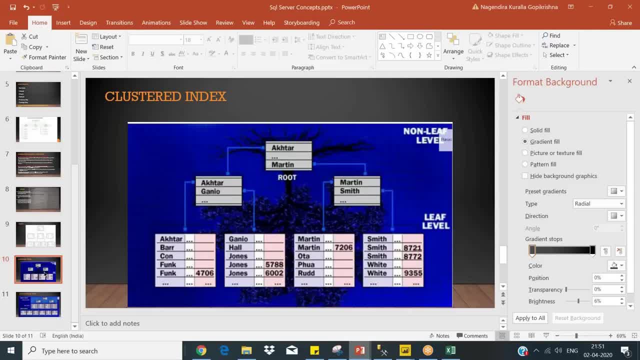 cluster index can be a only one per table. table. table that is using your primary key. if you, that is using your primary key. if you, that is using your primary key. if you want, want, want it to be a single, i mean a unique, it to be a single, i mean a unique. 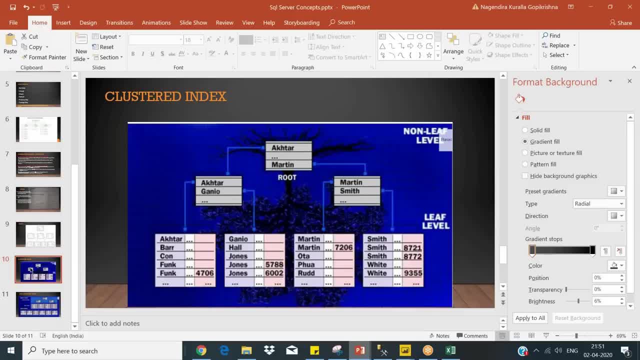 it to be a single, i mean a unique kind of paper. that column kind of paper, that column kind of paper, that column: go for clustered key, then a non-clustered. go for clustered key, then a non-clustered go for clustered key, then a non-clustered column is like you are any. 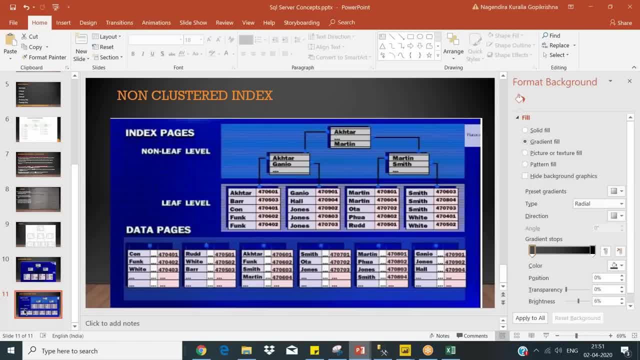 column is like you are. any column is like you are. any frequently used to that condition, like frequently used to that condition, like frequently used to that condition, like: address the location whichever you want. address the location whichever you want. address the location whichever you want. the multiple columns location can be: 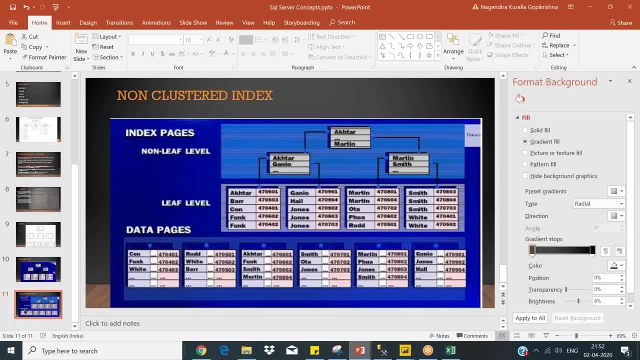 the multiple columns location can be, the multiple columns location can be in the customer. then another thing is in the customer, then another thing is in the customer, then another thing is like like, like, what is his salary? you can have a. what is his salary, you can have a. 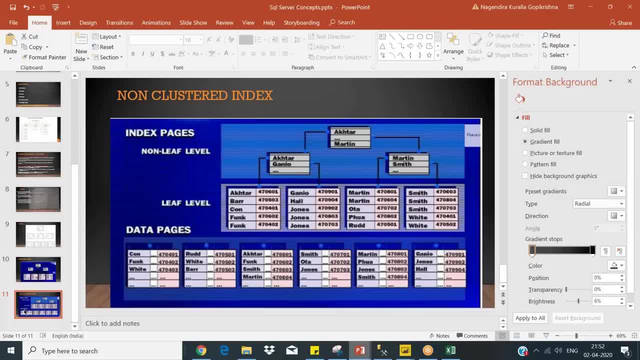 what is his salary. you can have a numeric value also. numeric value, also numeric value also. usually people will query: what is the? usually people will query what is the? usually people will query what is the salary of it, what is the salary range, salary of it, what is the salary range. 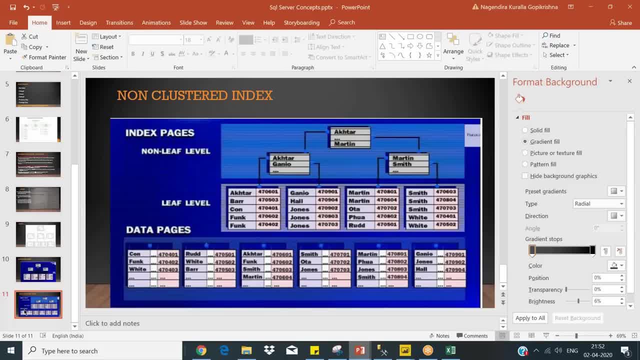 salary of it. what is the salary range? something like that, and phone number, something like that. and phone number, something like that, and phone number, obviously, even other card, obviously even other card, obviously even other card. multiple, uh, um, multiple, uh, um, multiple, uh, um. you have, uh, you have, uh. 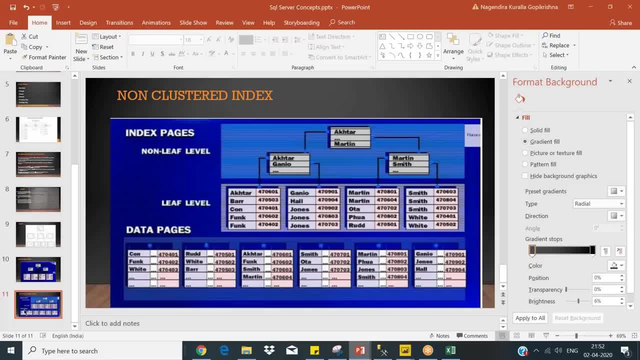 you have, uh, some addresses so these kind of things. some addresses so these kind of things, some addresses so these kind of things. whichever you use in var condition, whichever you use in var condition, whichever you use in var condition, so you can have multiple non-clustered, so you can have multiple non-clustered. 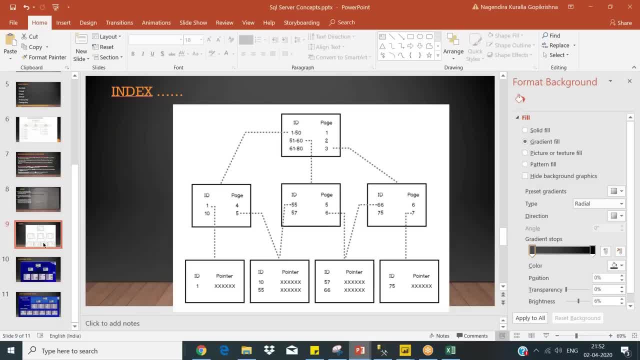 so you can have multiple non-clustered index index index. so this is the code difference between. so this is the code difference between: so this is the code difference between your clustered and non-cluster index, your clustered and non-clustered index, your clustered and non-clustered index. this is about your indexing. 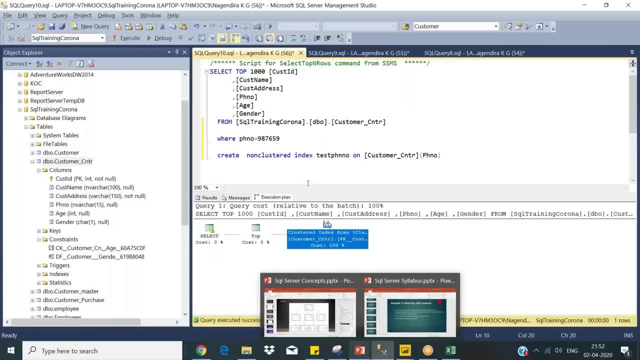 okay, guys, now let us see. we thought i will drop. now let us see, we thought i will drop. now let us see, we thought i will drop this index, this index, this index. how to drop this one and query this one. how to drop this one and query this one. 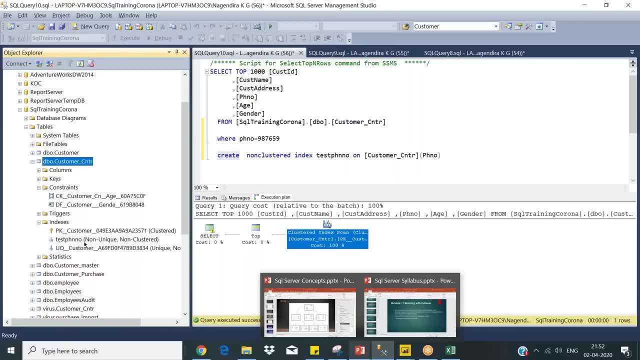 how to drop this one and query this one how it works. indexes: test phone number. indexes test phone number. indexes test phone number: non-clustered- non-unique- non-clustered- non-unique- non-clustered- non-unique. i can't drop it. i can't drop it. 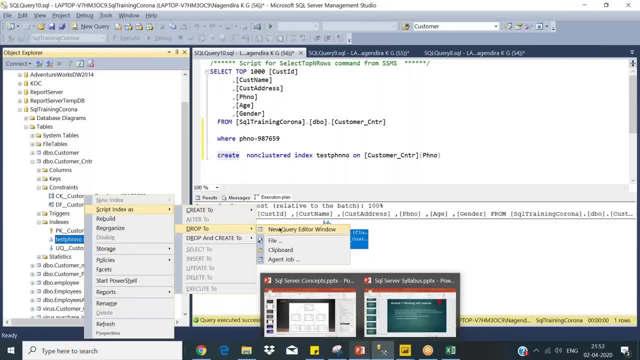 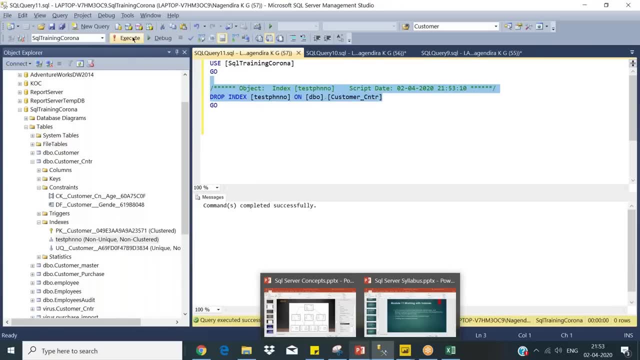 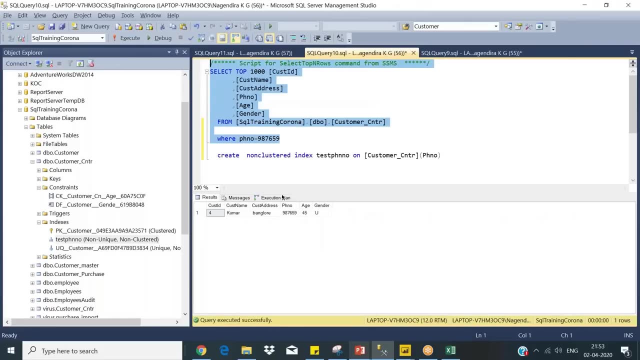 i can't drop it. drop to see here everything we can get. drop to see here everything we can get. drop to see here everything we can get. drop index index on. i think if you have your clustered index, i think if you have your clustered index, i think if you have your clustered index on. 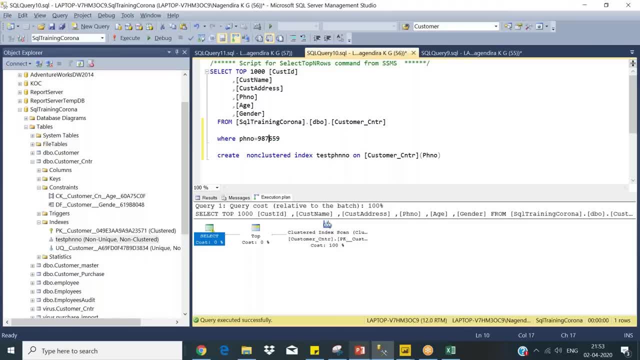 on, on, then using, even if you drop it, it then using, even if you drop it, it then using, even if you drop it, it results the same, results the same, results the same. so what i'm saying, so what i'm saying, so what i'm saying saying is, if you have your non-clustered 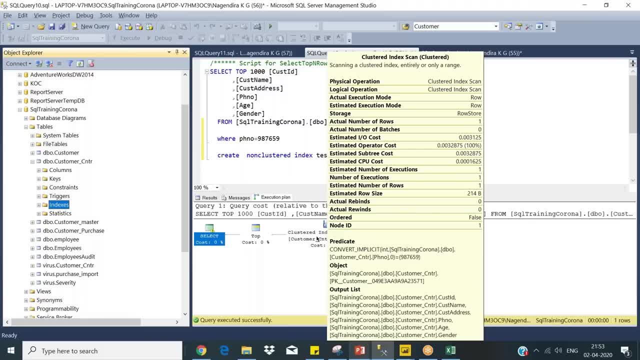 saying is: if you have your non-clustered saying is, if you have your non-clustered index in place, index in place, index in place, that alone will give you some differences, that alone will give you some differences, that alone will give you some differences if this table contains both your. 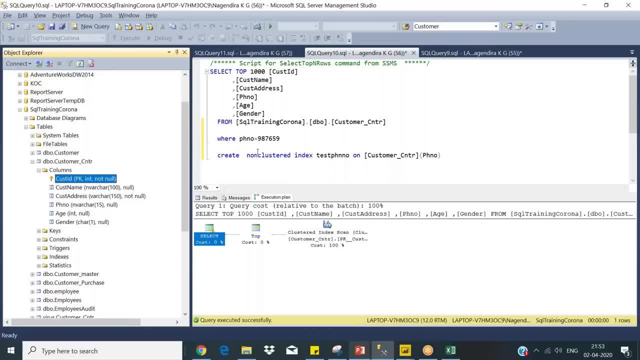 if this table contains both your, if this table contains both your cluster index and non-cluster index, just cluster index and non-cluster index, just cluster index and non-cluster index. just now we drop, but we now we drop, but we now we drop. but we created, okay, but core logic behind this. 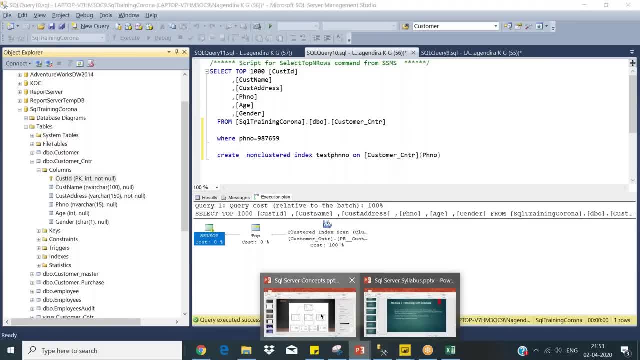 created okay, but core logic behind this created okay, but core logic behind this is this one only is this one only is this one only. i mean it will have, i mean it will have, i mean it will have your data stored in separate pages only. your data stored in separate pages only. 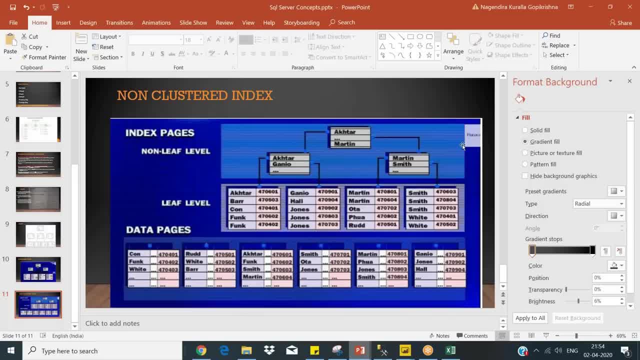 your data stored in separate pages. only the references will be. the references will be. the references will be referred here. okay guys with this note, uh, i am done. okay guys with this note, uh, i am done. okay guys with this note, uh, i am done. i hope, uh, you have got something out of. 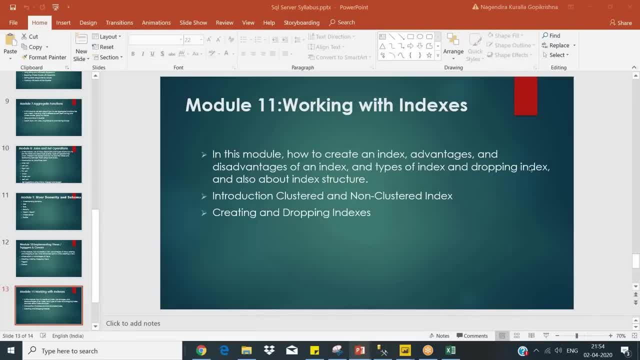 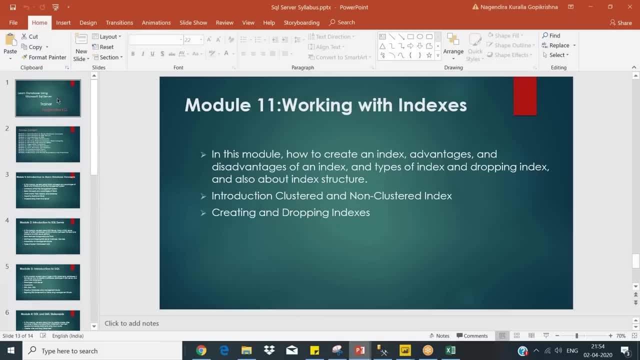 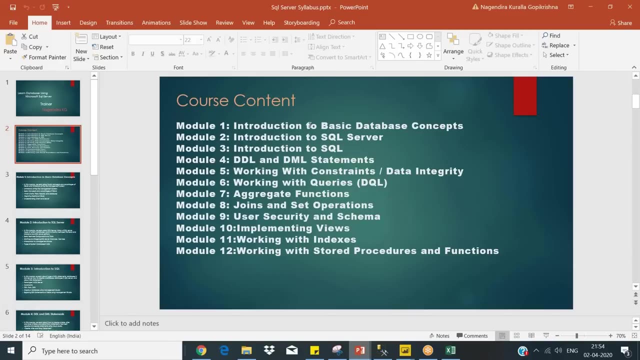 i hope, uh, you have got something out of. i hope, uh, you have got something out of the sessions, the sessions, the sessions, the sql class. any doubts, guys? hello, hello, hello, hello, hello, hello, hello, naga, naga, naga. okay guys, okay guys, okay guys. fine, i hope we have utilized somewhat. 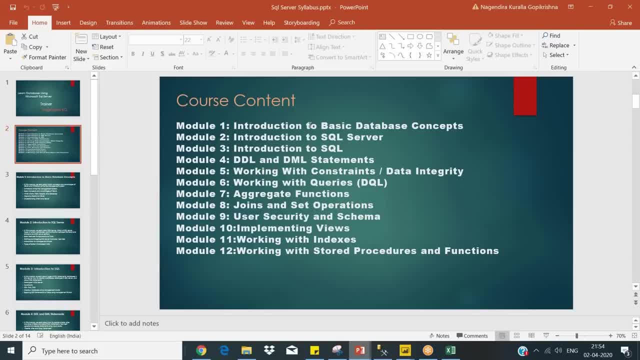 fine. i hope we have utilized somewhat fine. i hope we have utilized somewhat better in learning sql. better in learning sql, better in learning sql. thanks for participation. thanks for participation. thanks for participation. uh, when there is an application has. uh, when there is an application has. uh, when there is an application has been created. 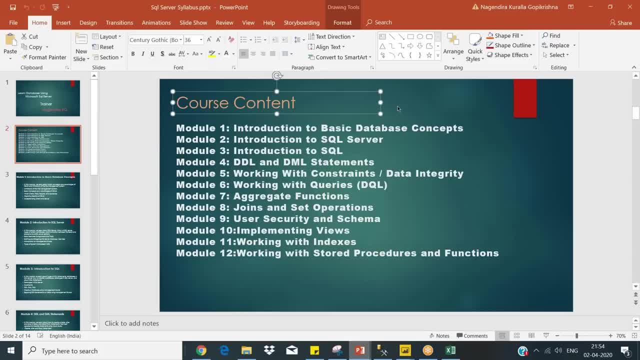 been created, been created okay, and those application data has been okay, and those application data has been okay and those application data has been stored in the database, stored in the database, stored in the database. so these uh index okay at so, these uh index okay at so, these uh index okay at which point in time they will create. 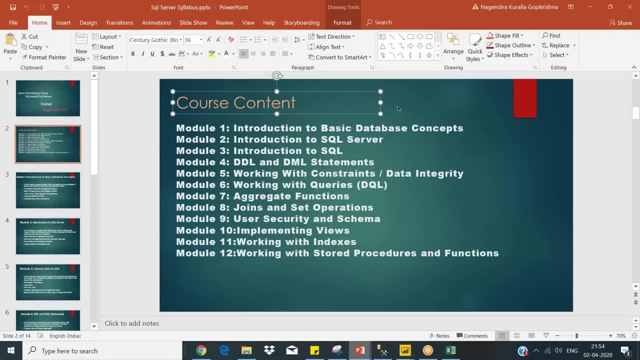 which point in time they will create, which point in time they will create this index after all, this index, after all, this index after all. the completion of application completely, the completion of application completely, the completion of application completely. yeah, so, basically, uh, when you. yeah so, basically, uh, when you. 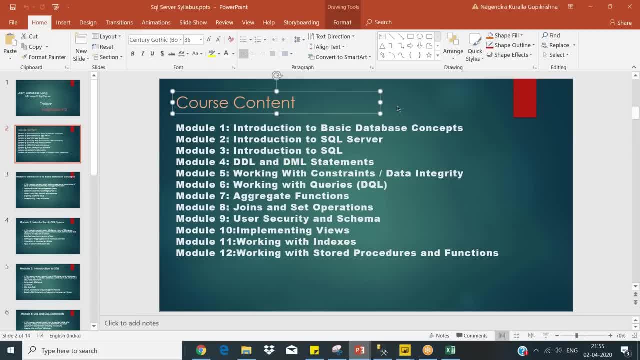 yeah, so basically, uh, when you, when you, as soon as you log in, or when you as soon as you log in, or when you as soon as you log in, or whatever, the, whatever, the whatever, the transaction is going to have okay. so, transaction is going to have okay, so. 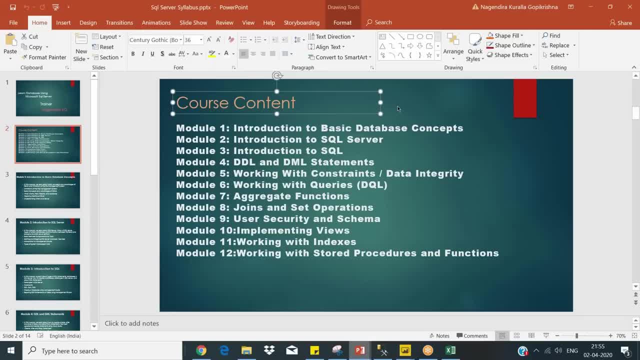 transaction is going to have. okay, so indexing, basically we have some idea. indexing, basically we have some idea. indexing, basically we have some idea. initially, initially, initially, we thought we will be in a position like we thought. we will be in a position like we thought we will be in a position like we will. 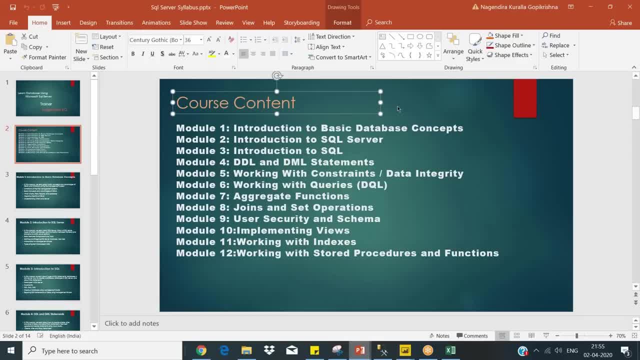 we will. we will use a phone number, other number, based on use a phone number, other number based on use a phone number, other number, based on our assumption, we will create the index. our assumption, we will create the index. our assumption, we will create the index, but going forward. 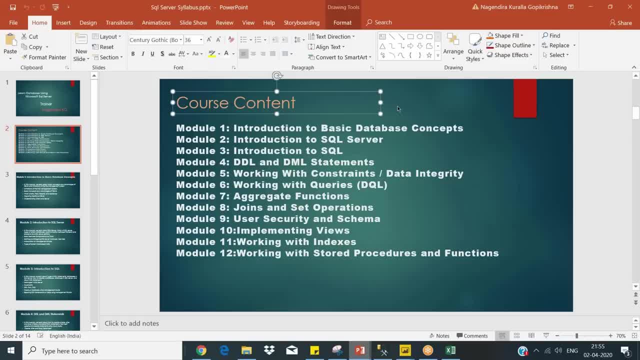 but going forward. but going forward. okay, after some time people will ask some: okay, after some time people will ask some: okay, after some time people will ask some other things also, other things also, other things also. so you can add some more indexes on that. so you can add some more indexes on that. 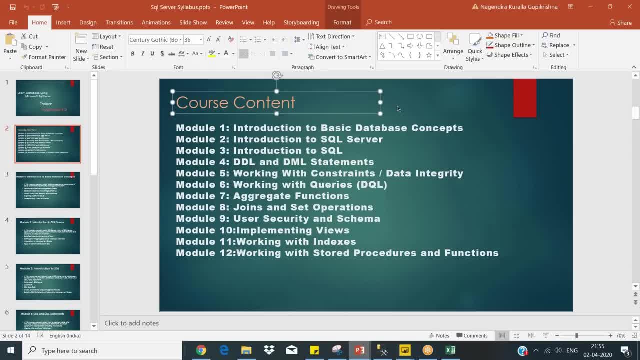 so you can add some more indexes on that. so initially, we will so, initially, we will so, initially, we will based on our assumption, we will create based on our assumption, we will create based on our assumption, we will create while creating the database structure, while creating the database structure. 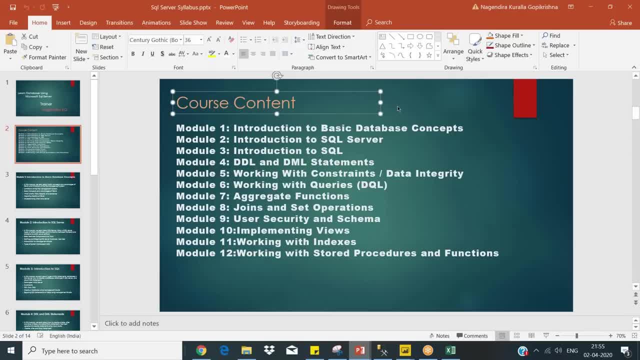 while creating the database structure itself itself itself. okay, after your, as you asked after. okay, after your, as you asked after. okay, after your, as you asked after. application evolves. application evolves. application evolves after few months, six months or one year. after few months, six months or one year. 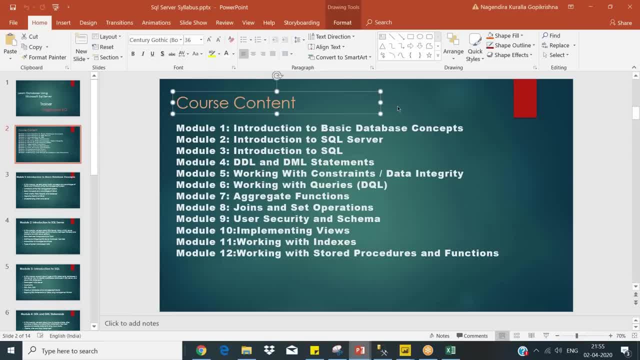 after few months, six months or one year, people will change the application and people will change the application and people will change the application and change the columns also, change the columns also, change the columns also at that time, if they use those columns at that time, if they use those columns. 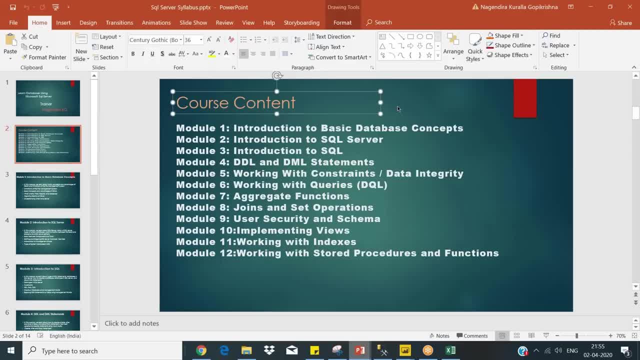 at that time, if they use those columns. we can amend the indexing and based on: we can amend the indexing and based on: we can amend the indexing and based on the user queries: the user queries, the user queries. we can do that, so it is not. we can do that, so it is not. 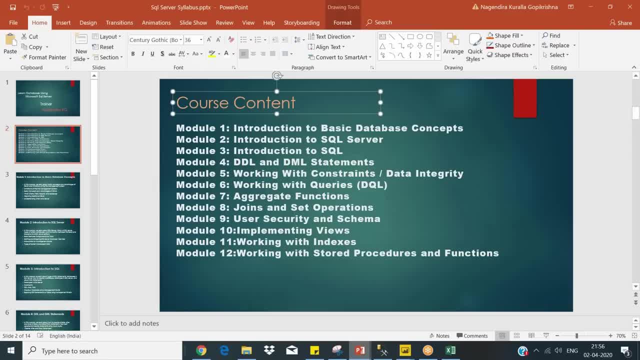 we can do that. so it is not the fixed one once you have. there is no the fixed one once you have. there is no the fixed one once you have. there is no general rule, like you need to create general rule, like you need to create general rule, like you need to create before. 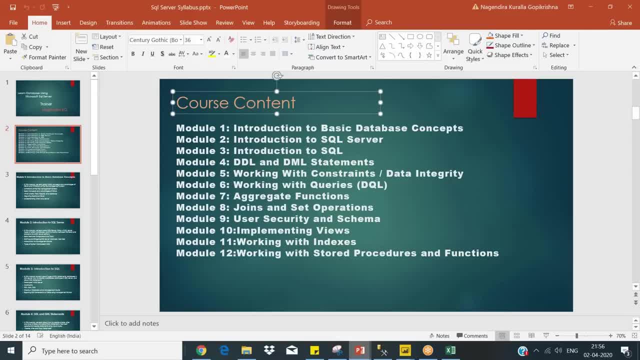 before before. you need to create after something like that. you need to create after something like that. you need to create after something like that. usually we will create and based on. usually we will create and based on. usually we will create and based on our assumption. this will be the things. 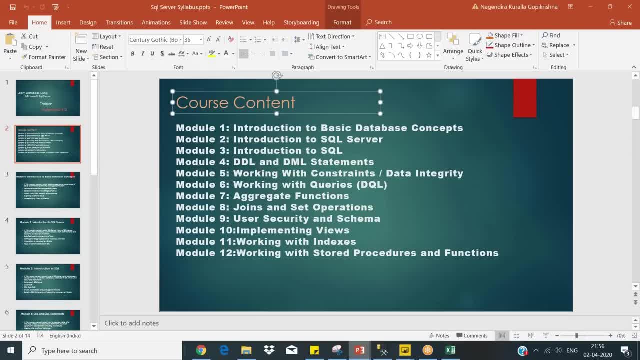 our assumption: this will be the things. our assumption, this will be the things. but as you asked the application, but as you asked the application, but as you asked the application, whoever queries in some application, they. whoever queries in some application, they. whoever queries in some application, they will. 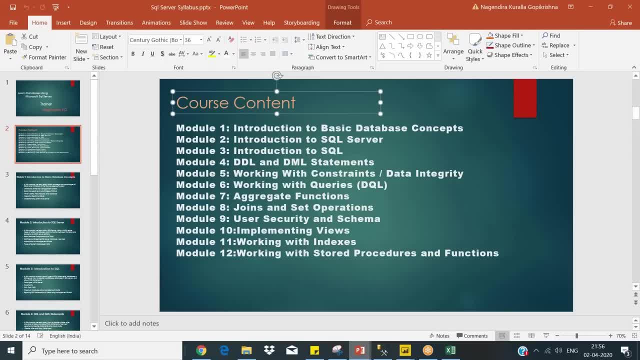 will will query phone number in some application. query phone number. in some application query phone number. in some application they query the location. they query the location. they query the location based on the application. it varies. so based on the application it varies. so based on the application, it varies. so based on that, we will decide and 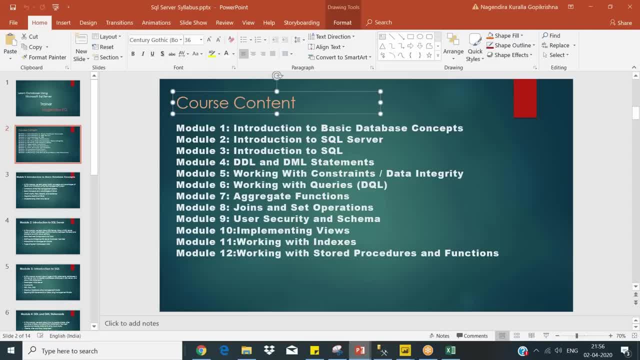 based on that, we will decide. and based on that, we will decide and keep on creating the index, the non. keep on creating the index. the non. keep on creating the index. the non cluster index, cluster index, cluster index. but the cluster index we need to create, but the cluster index we need to create. 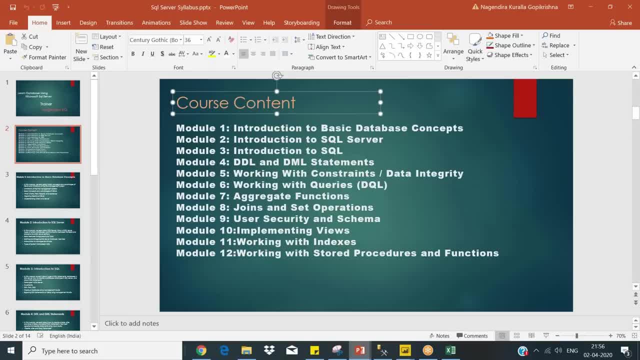 but the cluster index we need to create one, one, one. okay, okay, okay, fine guys. i think, uh, i'm done, fine guys. i think, uh, i'm done, fine guys. i think, uh, i'm done. almost everything covered, we did it in. almost everything covered, we did it in. 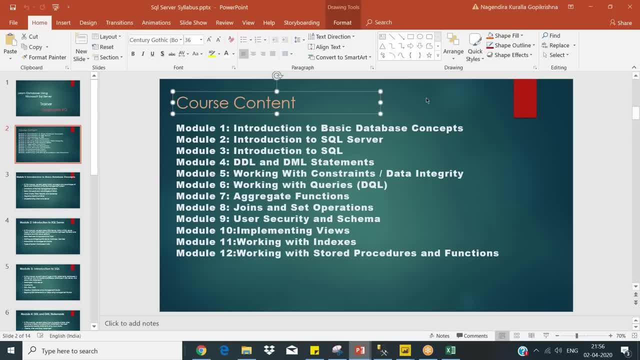 almost everything covered. we did it in days, only days, only days only, because uh you guys are not so, because uh you guys are not so, because uh you guys are not so, responding, responding, responding. uh, in case you didn't ask much, uh, in case you didn't ask much. 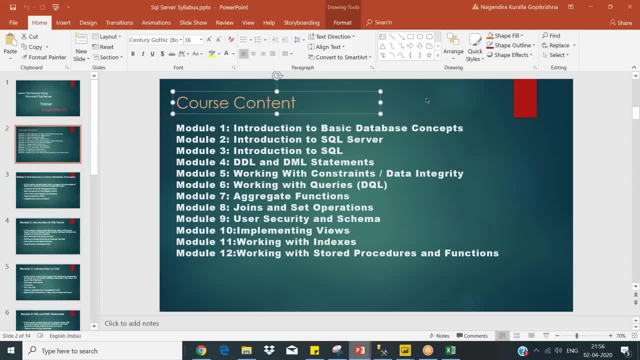 uh, in case you didn't ask much questions, usually it will be questions, usually it will be questions. usually it will be like two and fourth, like two and fourth, like two and fourth. when i keep continuing the session, when i keep continuing the session, when i keep continuing the session, people will stop me and you will ask. 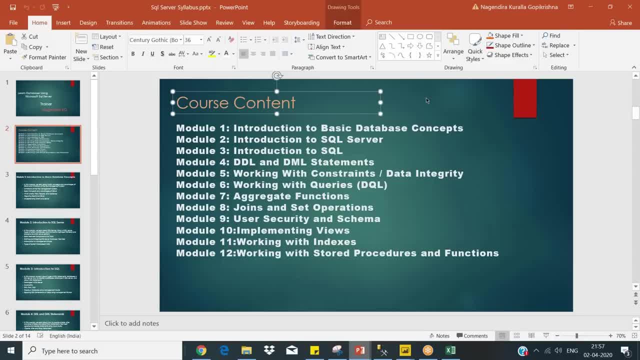 people will stop me and you will ask. people will stop me and you will ask questions. so that will take some time. questions, so that will take some time. questions, so that will take some time. but now it is not in this batch, so, but now it is not in this batch, so 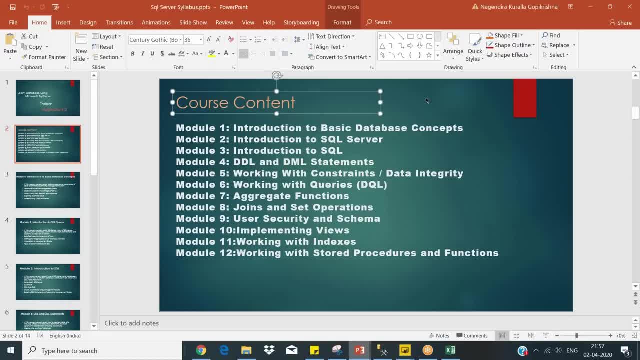 but now it is not in this batch, so that's fine, that's fine, that's fine. okay, uh, okay, uh, okay, uh. you can reach out to me anytime, uh, and you can reach out to me anytime, uh, and you can reach out to me anytime, uh, and i would suggest. 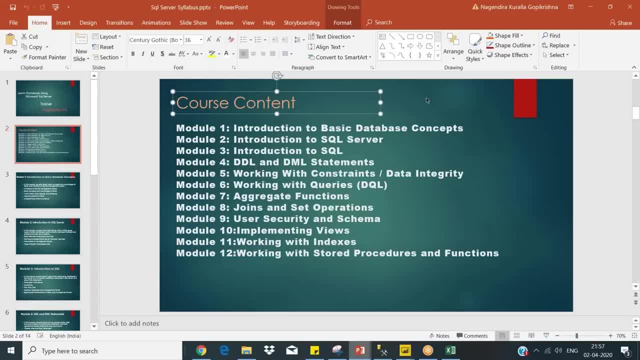 i would suggest. i would suggest: maybe, if i can create a form, just give. maybe, if i can create a form, just give. maybe, if i can create a form, just give me a feedback. otherwise, just give me me a feedback. otherwise, just give me me a feedback. otherwise, just give me your feedback in: uh, what's up? okay, 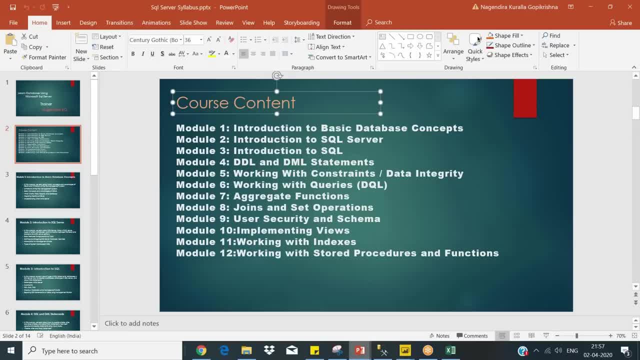 your feedback in: uh, what's up okay? your feedback in: uh, what's up okay? and try to practice, otherwise you can't. and try to practice, otherwise you can't. and try to practice, otherwise you can't learn, learn, learn. definitely will forget in within few days. definitely will forget in within few days. 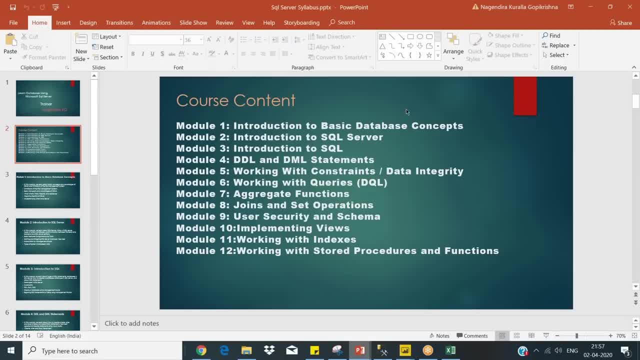 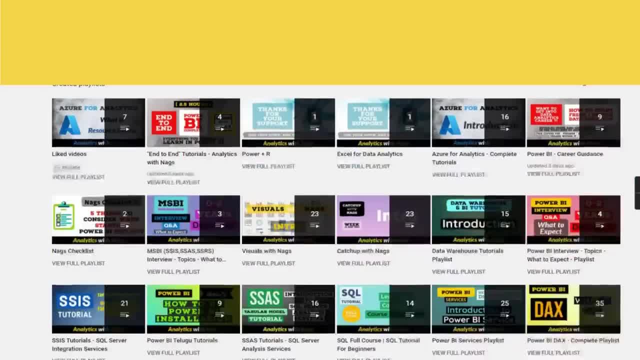 and this channel contains inr 75 000 worth. and this channel contains inr 75 000 worth- a thousand dollar. a thousand dollar. a thousand dollar. um free content, just utilize it as you can. um free content, just utilize it as you can. um free content, just utilize it, as you can see from this.